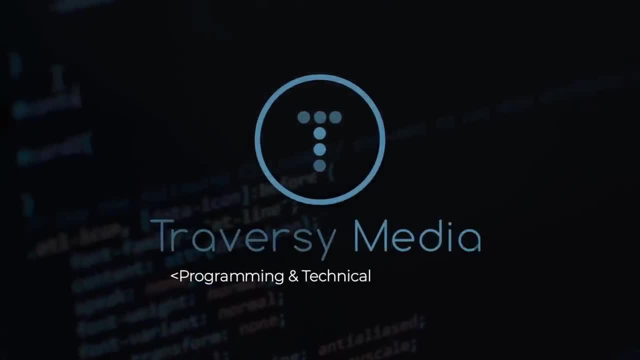 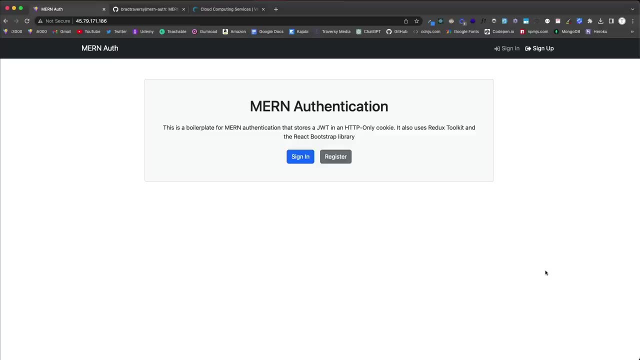 What's going on, guys? So this week I have a pretty good size project for you. This video will probably be two, maybe even three hours long, I'm not sure, but we're going to be building a full stack application using the MIRN stack, MongoDB, Express, React and Nodejs. We're also using 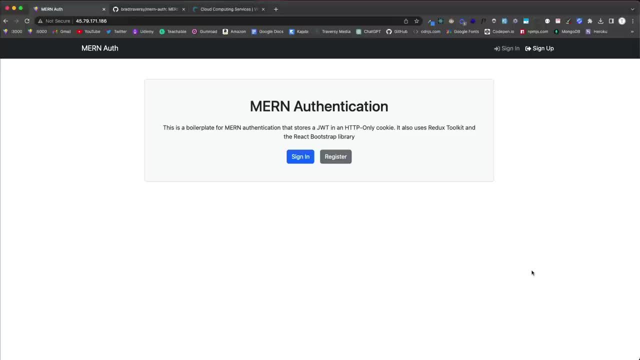 Redux Toolkit for state management, And the main focus for this is authentication. I want you guys to be able to have this as kind of a starting point for any application where you want to implement JSON Web Tokens and authentication. Now, there's easier ways to do this. You could use a. 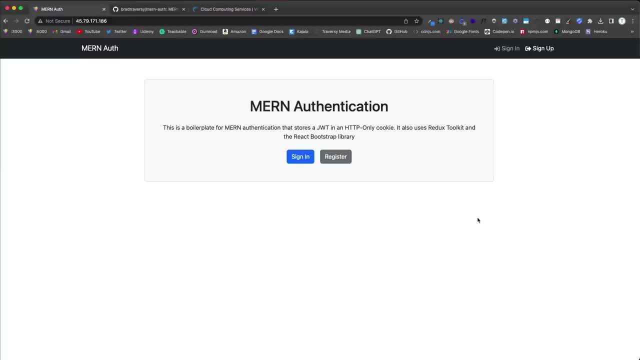 third-party service like Auth0, and that's fine, but I think it's important for you guys to know how to do this from scratch. So we'll be using JSON Web Tokens, but instead of storing the token in local storage, like you see so many tutorials do, including some of my own past tutorials. 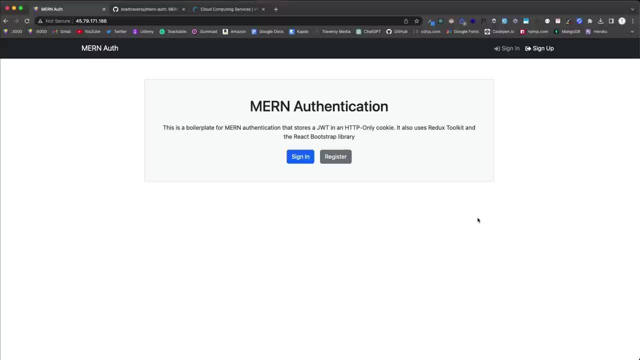 we're going to use JSON Web Tokens. We're going to store it in an HTTP-only cookie, which is it's more secure and less susceptible to things like cross-site scripting attacks. All right, so we'll start off with the back end, creating an API with register, login, logout and then profile routes, And then we'll. 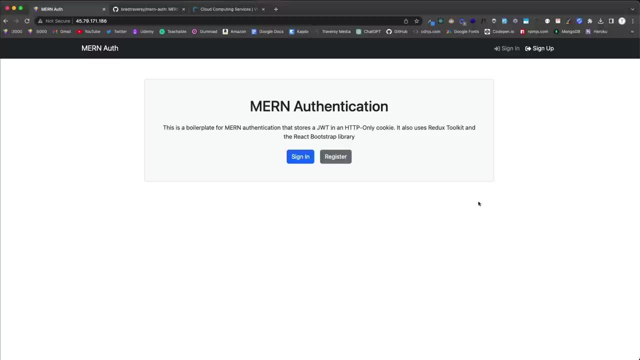 move to the front end and we'll build the user interface. And you can see, it's very simple. We're using the React Bootstrap library, So if you want to customize the look and customize it, you can do that, And then we'll move to the front end and we'll build the user interface And 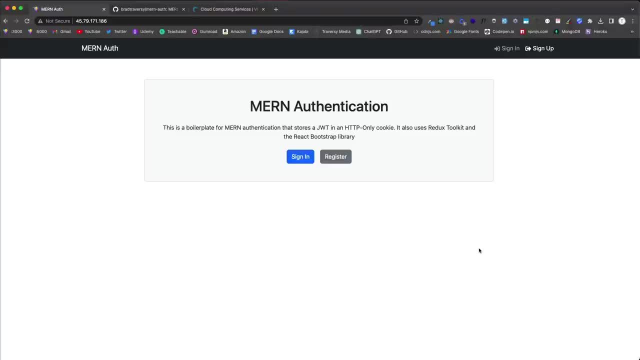 of course you can do that, And then we're going to deploy it to Linode, which I'll talk about in a second, But just to give you a quick demo. we have the homepage, which is very simple. We have a sign. 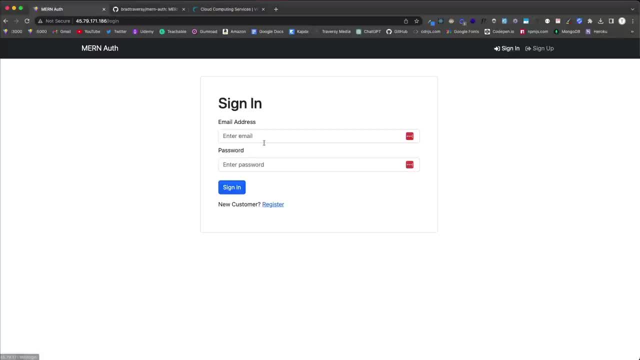 in page, a register page, So let's just go ahead and sign in, And we're using React Toastify for, you know, messages and things like that, So I'm going to sign in with john at emailcom. Okay, so now you can see we're logged in, because up here 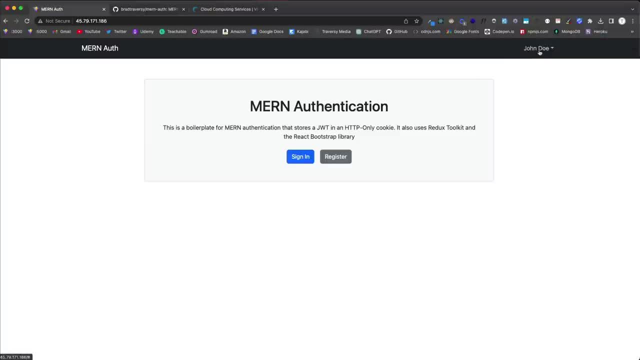 we no longer have the sign in, sign, you know, sign up links. we have the username john doe, And if we click on this we have a drop down with profile And from here it'll just give you the profile name and email address And you can update any of these, including the password. Okay so, 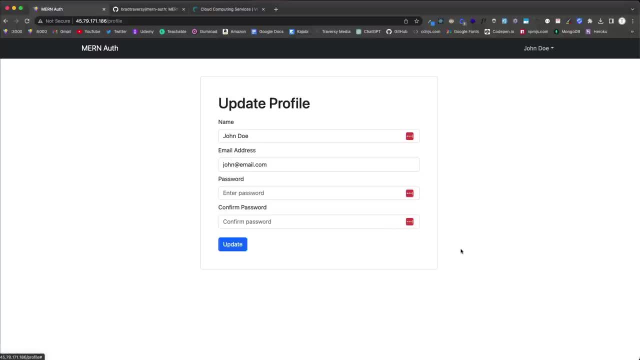 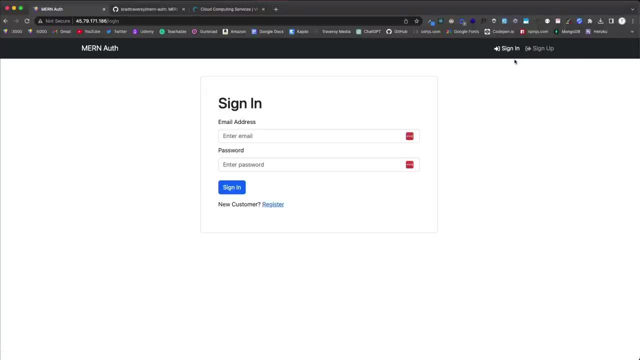 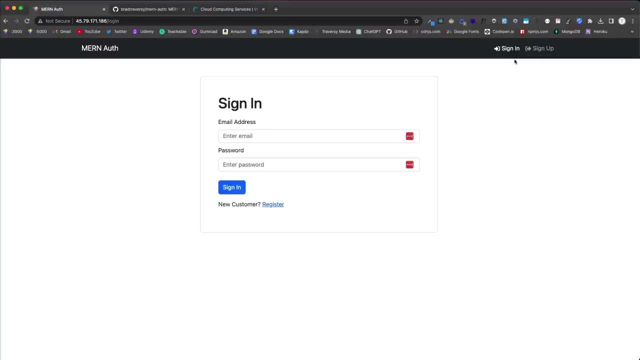 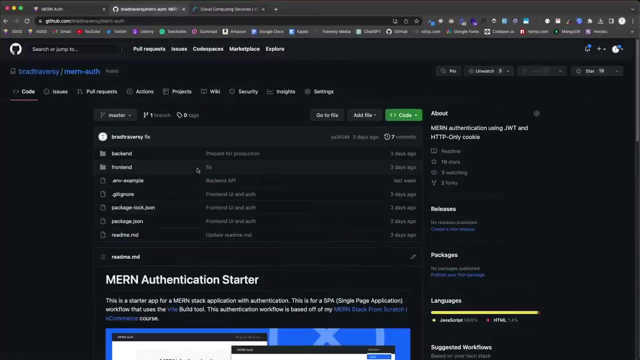 Redux toolkit to manage state. So this is also kind of like a Redux toolkit crash course as well, And I'll have all the final code here in this repository And I'll have that link in the description as well as a link to a couple blog posts. that will basically be a written version. 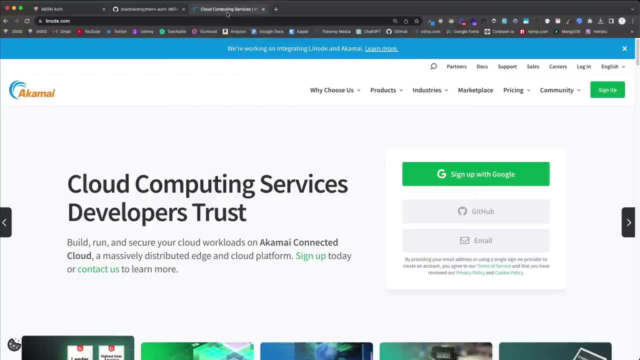 of this, this entire project. Now, like I said, we'll be deploying to Linode, who recently integrated with a company called Akame And they're sponsoring this video And we've been working with Linode for years And they're my go to for any project where I want complete control of my server. you can install. 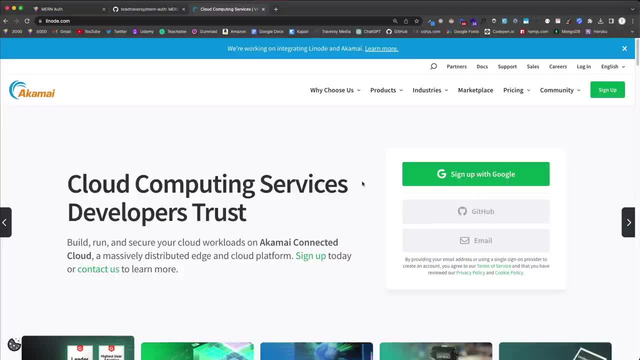 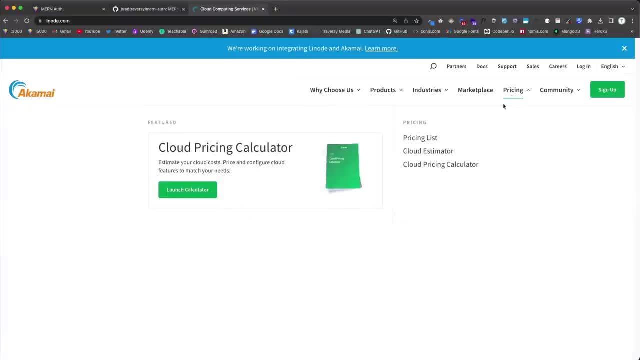 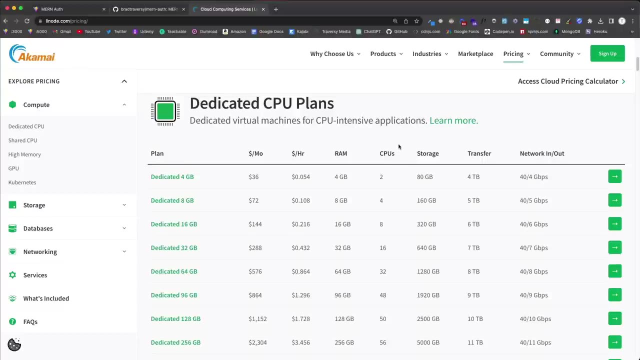 and customize everything down to to the operating system itself, And they have a ton of one click apps and stacks to get you up and running quickly. Now, when it comes to pricing, what really sets them apart is is, with a lot of cloud hosting providers, you end up with all these strange charges and it ends up 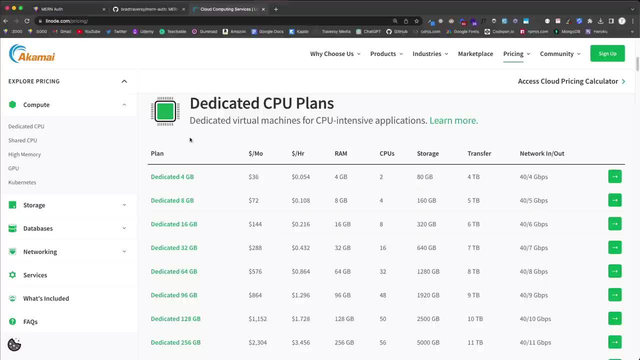 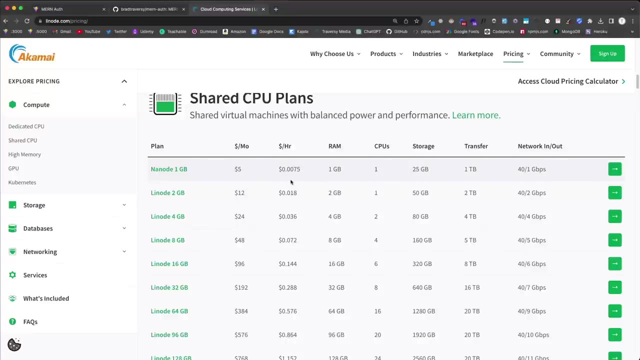 being a lot more than you thought. where, with Linode, slash, Akame, there's caps on Pat on these plans. So this dedicated four gigabyte plan isn't going to go over $36 per month. And these are dedicated CPU plans. They're shared CPU plans for much cheaper. you can see $5 per month, But what? 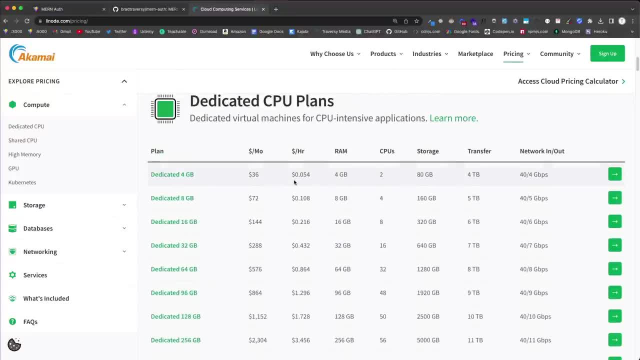 I'm going to do is put a link in the description that's going to give you $100 credit over 60 days, So you can follow along with this tutorial. you can deploy your own projects absolutely free. And I can't say enough good stuff about Linode. We've been working with them for years. they have 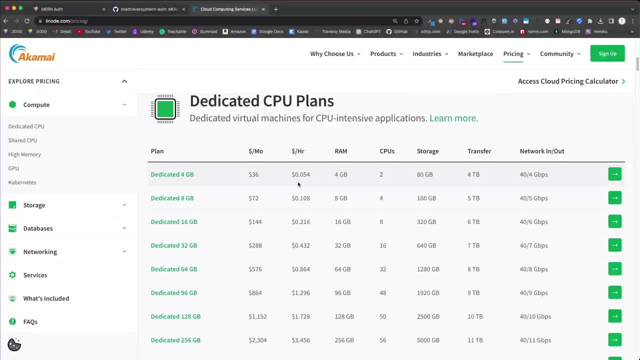 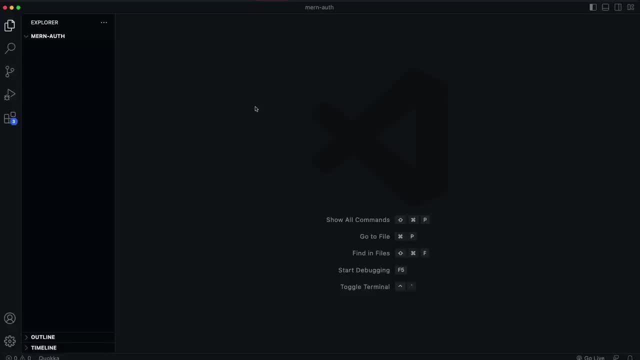 phenomenal support. they have very reliable servers. So check them out- links in the description: for $100, free over 60 days, And let's get started with our project. Okay, so we're starting from absolute scratch. you can see I just have an empty folder called Mern off And I'm using VS code. But 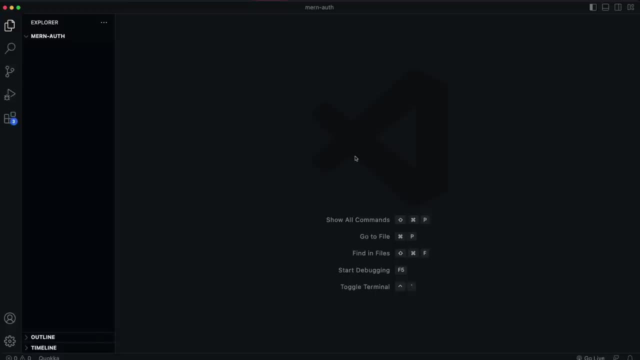 of course, you can use whatever you'd like. So let's get started, And this is going to take a while. It's a pretty big project relative to YouTube tutorials And I would suggest that you follow along with me. you know, get a tea, get a coffee. 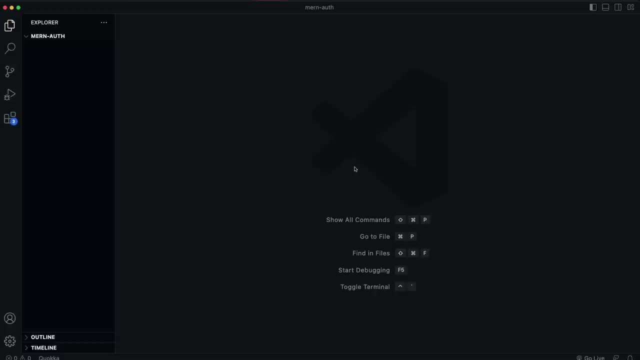 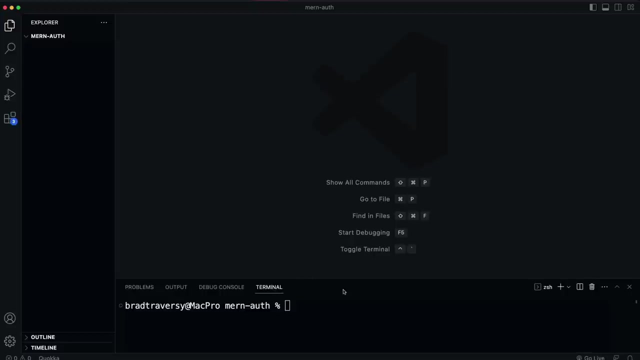 sit down and just follow along, And if you need to do it in multiple sessions, of course that's fine. But yeah, we're going to start from scratch. So let's open up a terminal, And I do expect that you have a little bit of experience with React And with nodejs And express. I'm going to hit the button here And I'm going to just go ahead and type in my URL And then I'm going to go ahead and click on the button And then I'm going to hit the button, And then I'm going to hit the button And then I'm going to. 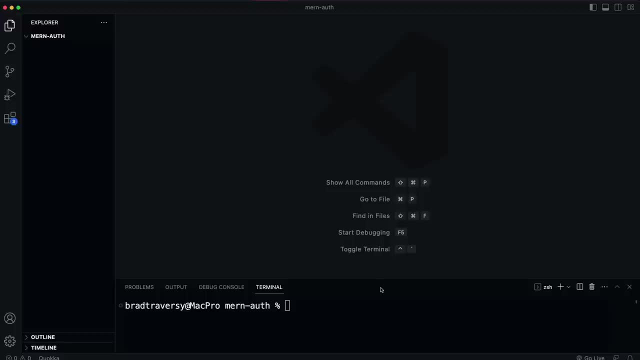 with React and with Nodejs and Express, At least you should be able to create a route. you understand how HTTP works. you should be able to create a React component, things like that. You don't have to be a senior developer or anything. 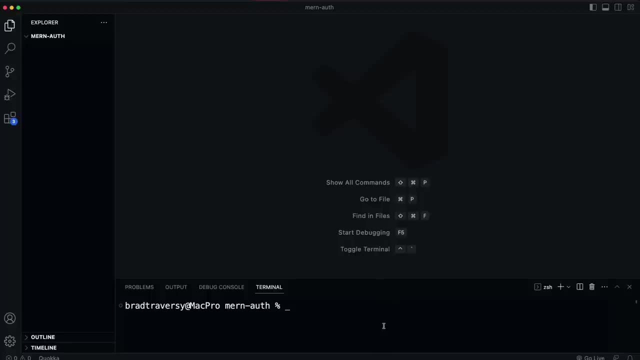 but you should have just a little bit of experience. I would say, if you watch my React crash course along with my Express crash course, then that would be enough. So I'm gonna start off here by running npm init to generate a packagejson. 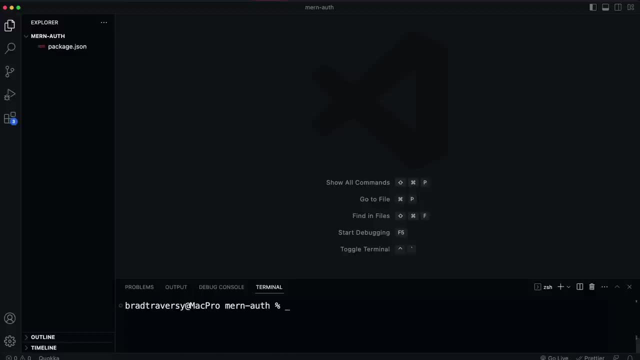 and we'll just say dash y, so we don't have to answer the questions. And then what we're gonna do is install our backend dependencies. Now, the way that this is gonna work, or the structure of our folders is gonna be, the route, will have our server-side packagejson. 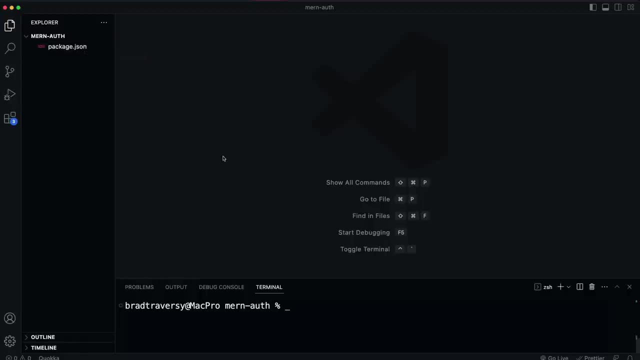 So Express, everything like that, is gonna be listed in here. Then we'll have a backend folder that's gonna have our models, our controllers, things like that- all of our backend source code And then later on when we get into React. 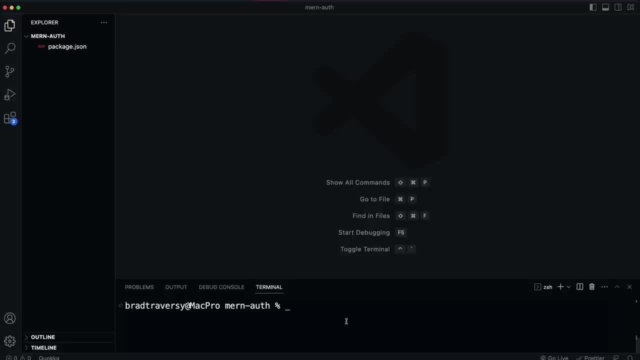 that will all be put in a frontend folder, So we'll have a completely separate folder for frontend and backend. That's just how I like to structure my single-page application projects, And you might wonder why I'm not using Nextjs or Remix. 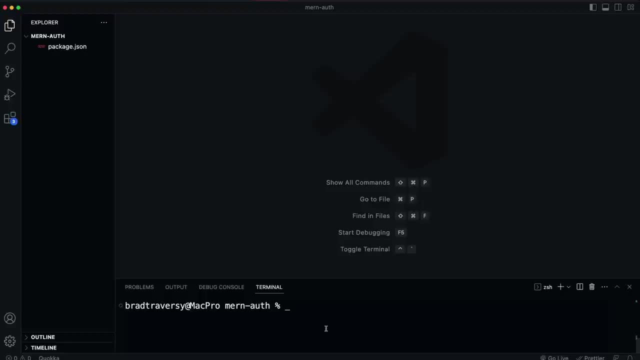 something like that, because I think that it's important to learn. if you're gonna learn React, I think it's important to learn how to build single-page applications first, because that's what React was initially intended for. I know things are changing now. 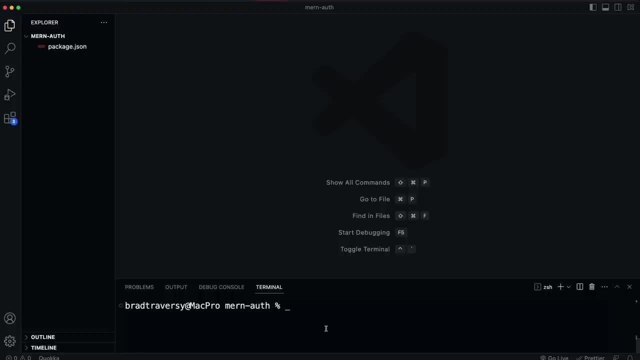 and server-side rendering is really popular and I definitely would suggest learning Nextjs or Remix, but I think that it's important to learn the basics of React first and state management and all that, And you could definitely redo this in Nextjs if you want. 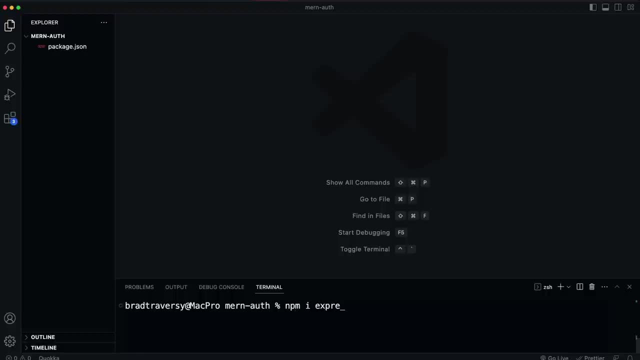 So, as far as our server-side dependencies, we're gonna install Express, which, of course, is our web framework. We're gonna be using env, which will load environment variables from a env file, Mongoose, which we're gonna be using. 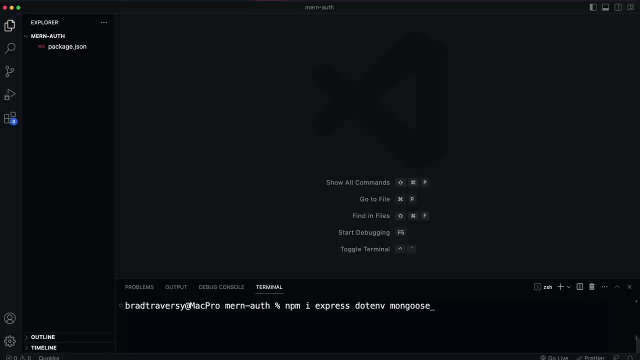 to interact with our MongoDB database. when we get to that, We also want bcryptjs for hashing our passwords And then JSON web token, because we're using JWTs for authentication And we're gonna, like I said, we're gonna be storing them. 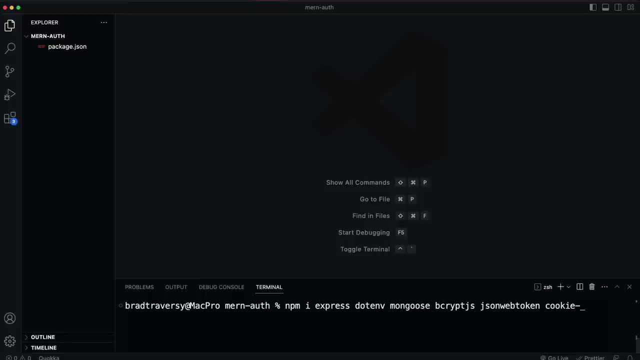 in a HTTP-only cookie. so we're also gonna install cookie parser so that we can parse our cookies. All right, so let's go ahead and install those, Okay? so once those are installed, we're gonna just create a very basic Express server. 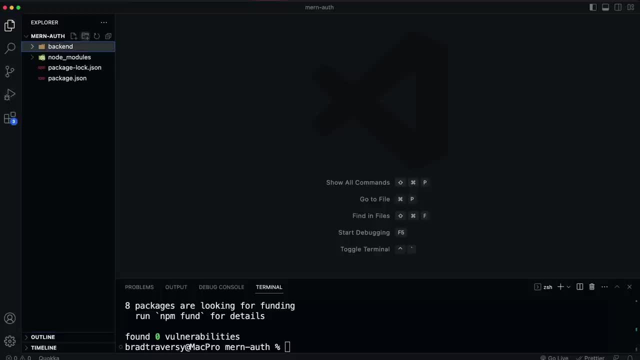 So, like I said, I'm gonna have a folder called backend And then in that backend folder we're gonna have a file called serverjs. This is the entry point for our server, for our backend, for our API, whatever you wanna call it. Now, instead of having a server, we're gonna have a serverjs. This is the entry point for our server, for our backend, for our API, whatever you wanna call it. This is the entry point for our server, for our API, whatever you wanna call it. 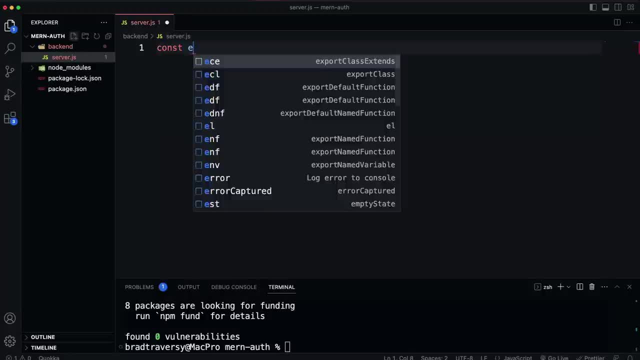 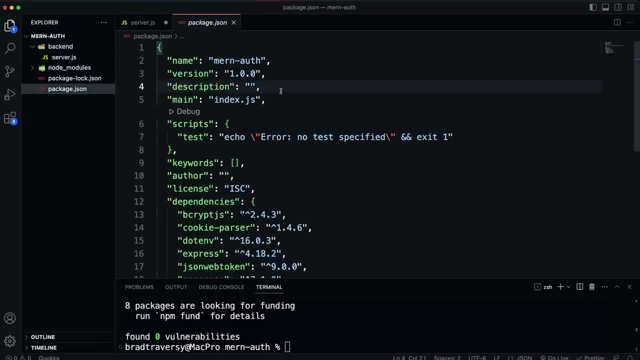 Instead of using CommonJS, where we say: const express equals require express. lately I've been using ES modules in the backend, which is really simple to do. now All we have to do is in our packagejson we're just gonna add: 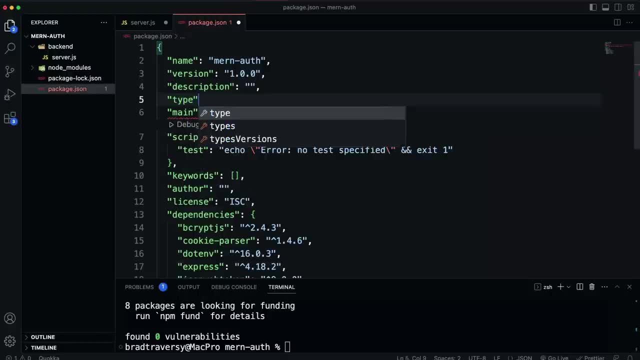 we can put this anywhere, but right here I'm just gonna add type And we're gonna specify: instead of CommonJS, we're gonna specify module, So that will allow us to use the input import syntax, which I prefer. 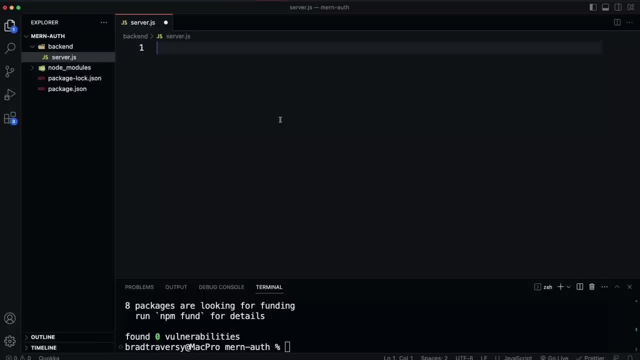 And it's good to use because that's what you use on your front end, so it's good to have them match. So we're gonna import express from express And for now I'm just gonna put the port number directly into a variable. 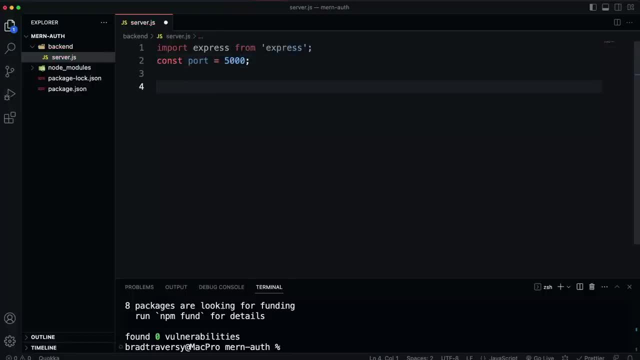 We'll use our env file in a few minutes, but for now we just wanna get this set up. So then we want to initialize our app variable, set that to express, And we wanna listen. so applisten on the port. 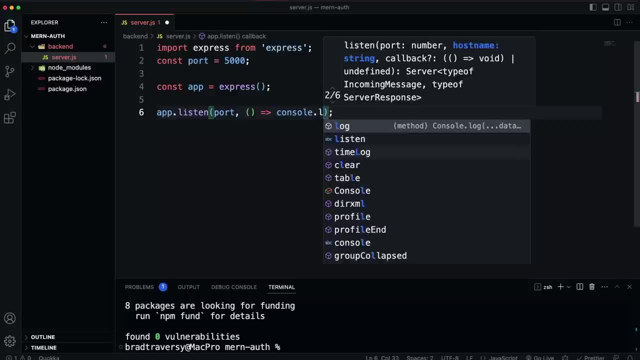 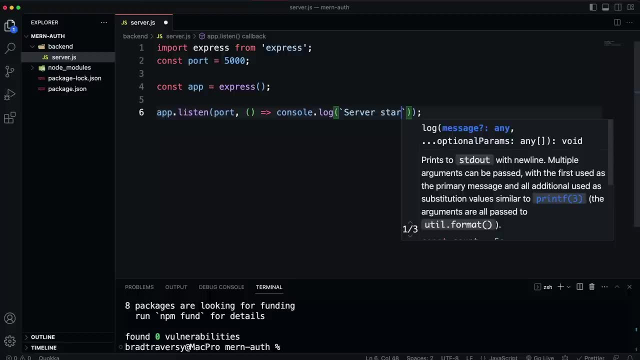 And then I'm just gonna have an arrow function with a console log, And in the console log we'll put some backticks And let's say, server started on port And then we'll put in that port variable. Okay, now as far as a route. 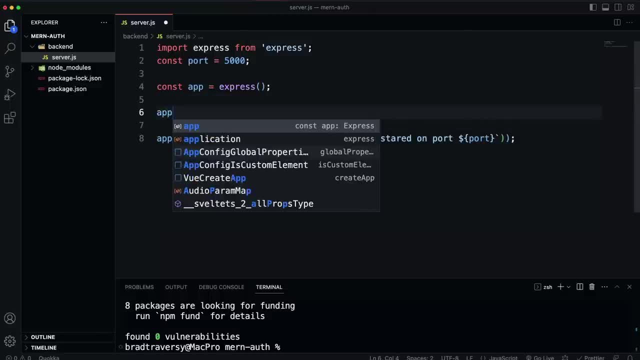 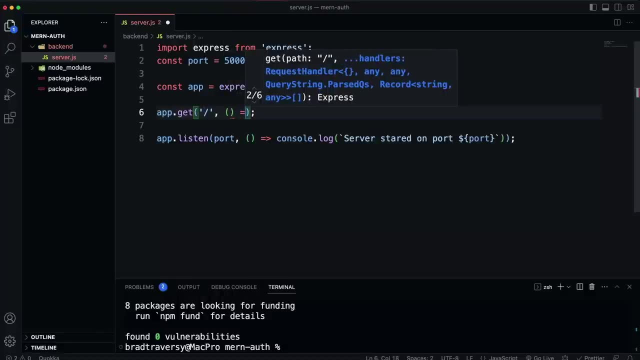 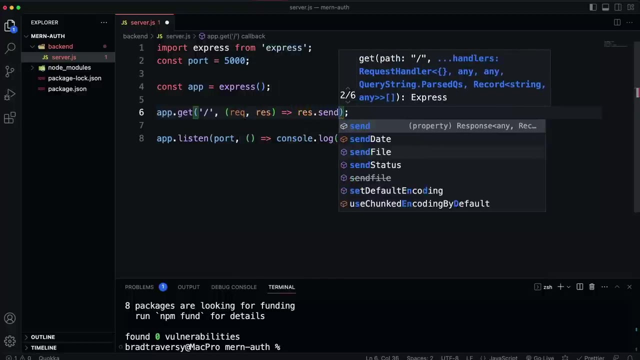 I'm just gonna add a route to the index for now. So appget, And that's just gonna go to slash. Then we'll have our callback And we want request response And I'm just gonna respond by sending just a string back. 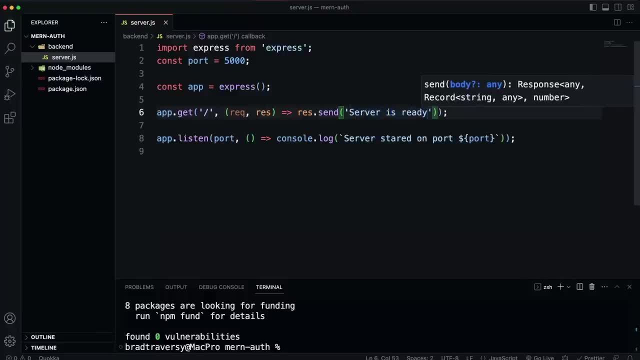 and say: server is ready, Okay, so just that. should. we should be able to run this with node and then backend slash serverjs And you can see it's running. So I'm gonna stop that. Oops, I'm gonna stop that. and in our packagejson. 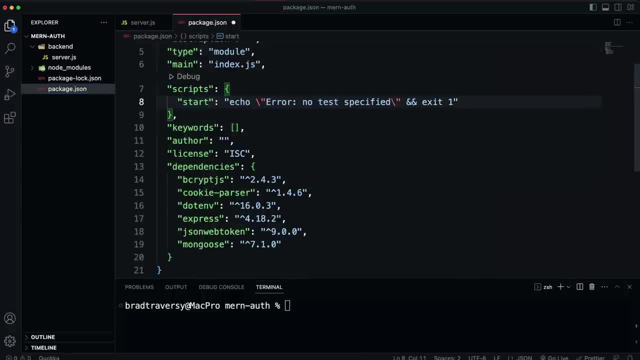 we're gonna add a couple scripts here, So we'll have a start script and that's gonna run what I just did, So it'll run. remember it's in the route. so we need to specify the backend folder- slash, serverjs- And then I'm also gonna install nodemon. 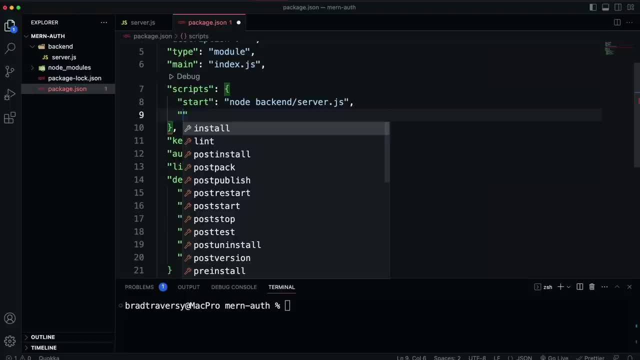 so that we don't have to keep restarting our server every time we make a change. And that's gonna be a script called server. I'm not gonna call it dev because we're gonna have a front end as well- and the dev script will run both the front and the backend. 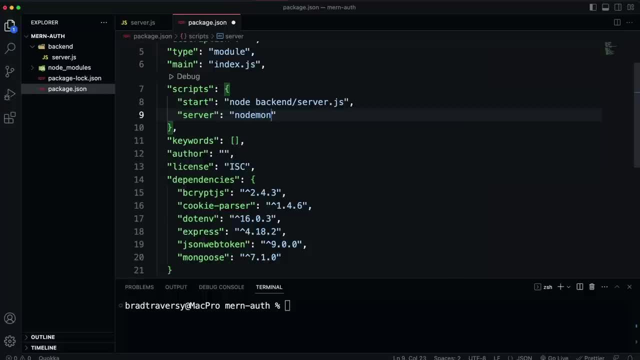 Server will run just the backend with nodemon. So let's say nodemon and then backend slash serverjs. Okay, now of course we have to install nodemon. So I'm gonna install that as a dev dependency. So I'm gonna use uppercase D and then nodemon. 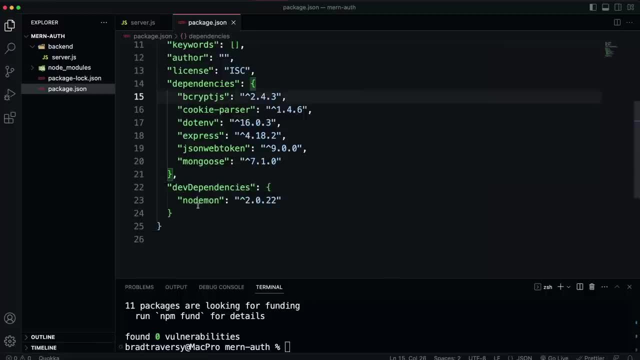 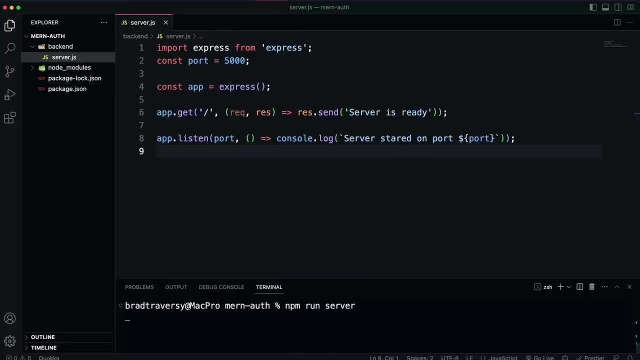 And we should see that get added There. it is as a dev dependency. All right, so now if I go ahead and I run npm run server, it should run our server using nodemon. So next thing I wanna do is implement env. 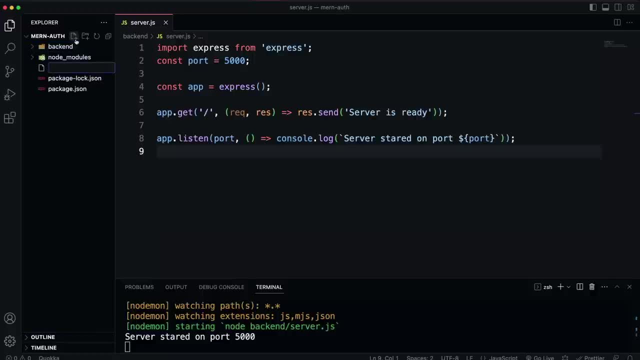 So in the route- not in the backend, but in the route- I'm gonna create a file called So, period and then env. Okay, and from here I'm gonna add two things. One is gonna be my node, env, which I'm gonna set to development. 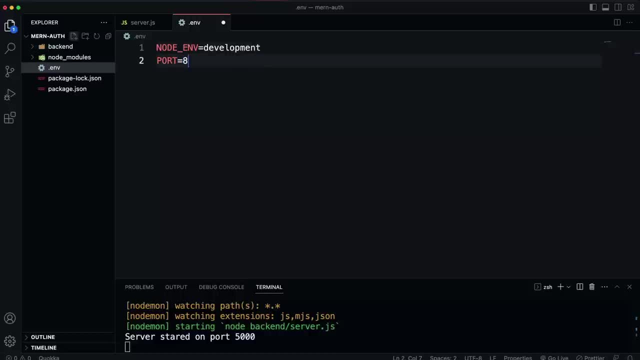 And then we're also gonna have our port, which I'm gonna set to, for right now I'm gonna set it to 8000, just so we can make sure it's working. So, back in our serverjs, we need to do a couple things. 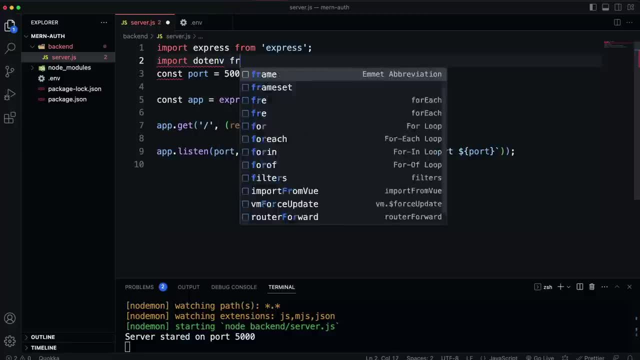 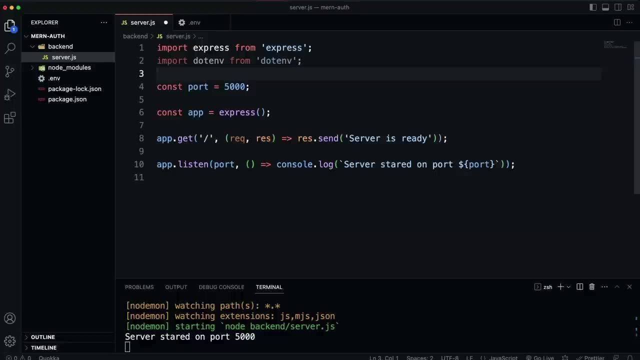 We're gonna import env from env And then we have to run the config method, So we could just do envconfig like that. And then here, where we're setting the port, what we're gonna do is say, first, look in processenvport. 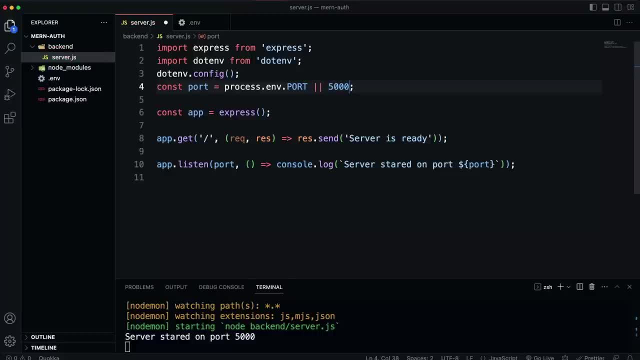 or if that's not there, then use 5000.. So if I save, you can see down here. usually we have to restart this, but I guess not. So server started on port 8000, because it's looking at that environment variable. 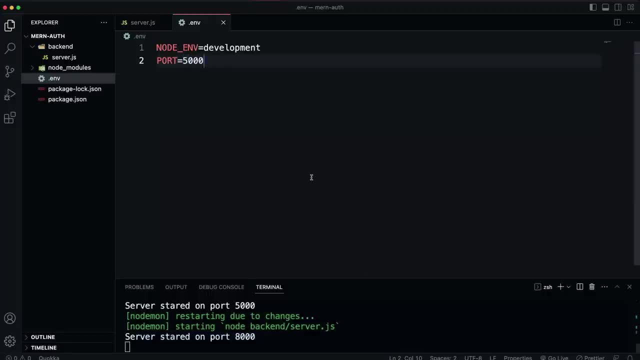 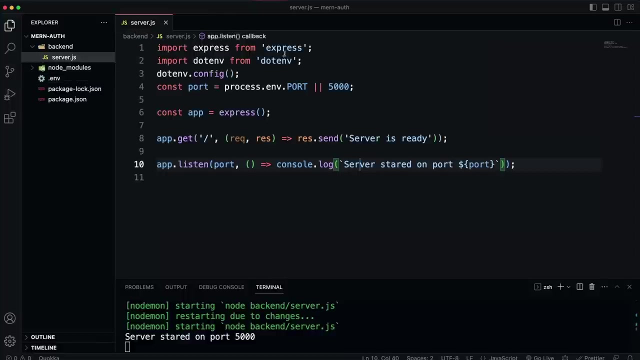 But I'm gonna set that to 5000.. And now you can see, now it's running on 5000,. okay, And now we can use processenvnodeenv whenever we wanna get the environment we're in, whether it's development or production. 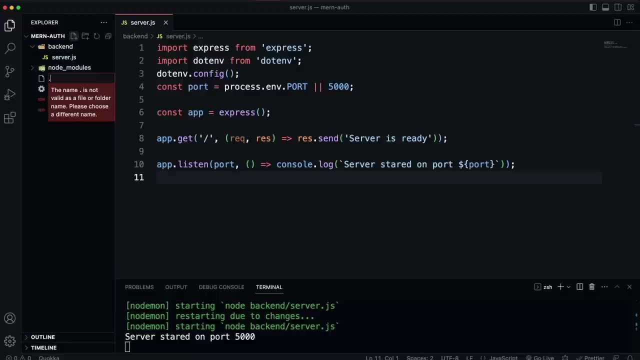 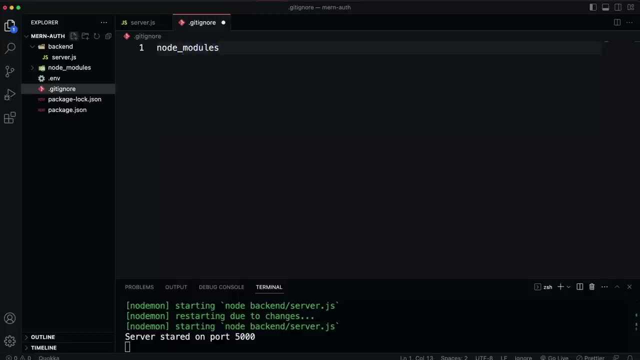 So another thing we should do is, in the root, create a gitignore, And here we wanna of course add our node modules, because when we push to GitHub or wherever, we don't want node modules included. I also don't want the env included. 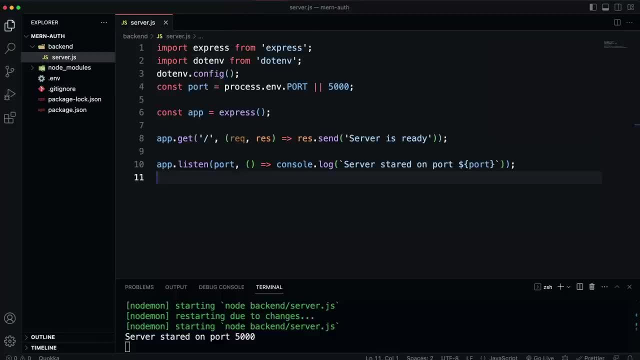 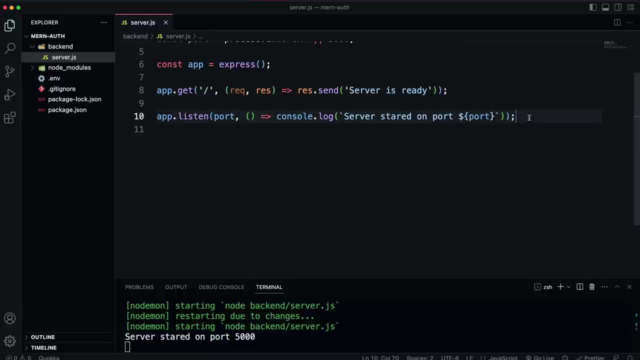 So we'll go head and add those two files. All right, now the next thing I wanna do is start to create our routes Now, just to show you real quick. you guys don't have to type this out, but I just wanna show you the actual routes. 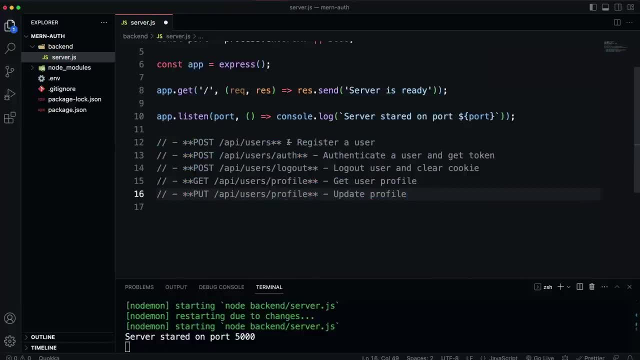 that we'll be creating. So, first off, we're gonna have a route to register user. That's gonna be a post request to API. slash users To authenticate or login to set our token. that will be a post request to API- Booksuserscom. 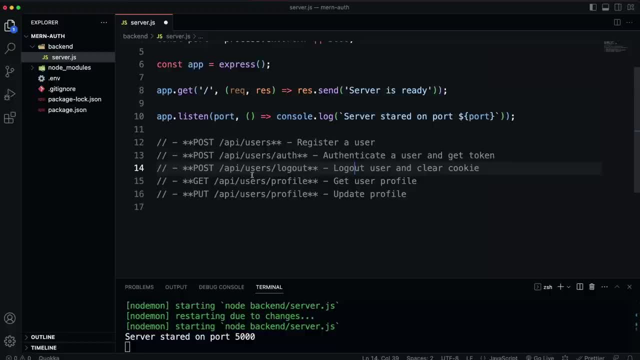 API users off And then to log out or clear the cookie will be API users. log out to get the user profile, which will be a protected route, will be API users profile get requests. and to update will be a put request to that same URL, API users profile. So those are the what is it? five routes. 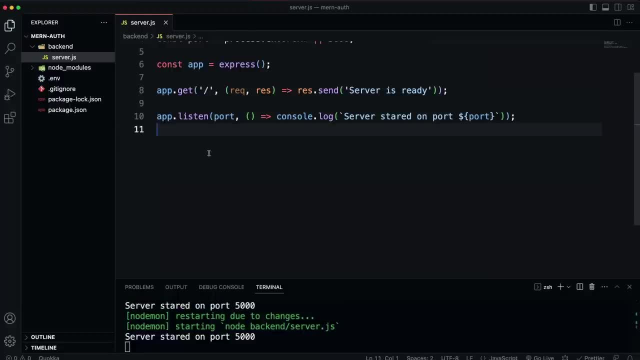 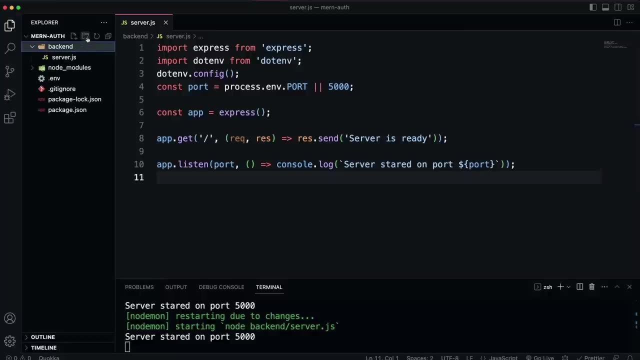 that we want to create, our endpoints that we want to create. So obviously we don't want to put all of that in the server j s. So what we're going to do is, in the back end, we're going to create a folder called routes. All right, now in here we're going to have a file called user routes dot j s. 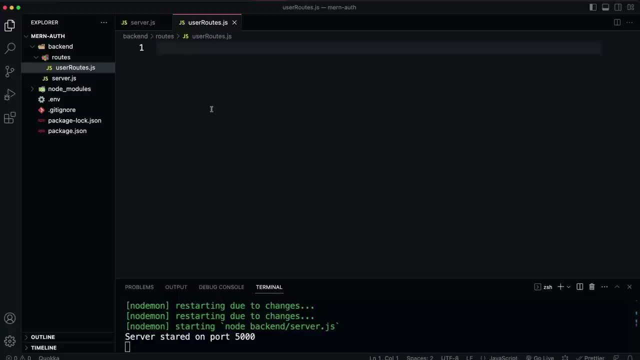 Now we could put all of our logic in this file, But I think it's good practice to have your logic in a controller. So we're also going to create in the back end a folder called controllers And inside that we're going to create a file called the user controller dot j s. All right now in our user. 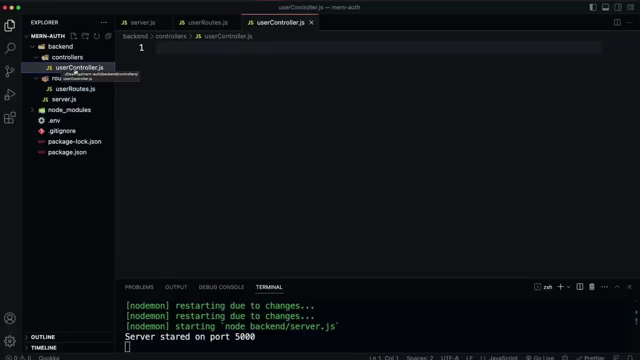 routes. we're going to basically link to our controller function. So let's start off in our controller and create those functions. So the first one will be to authenticate a user or login. I'm going to call it off user And I'm using an arrow function. you don't have to, but that's how. 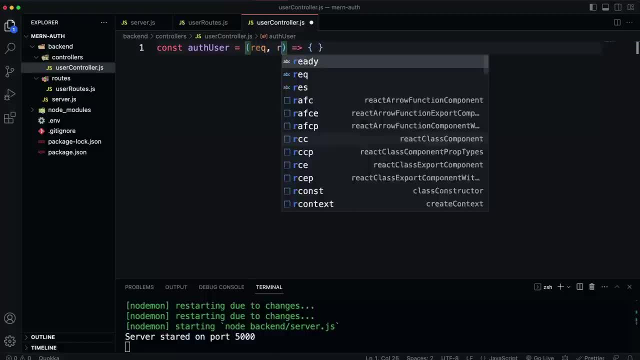 I'm going to set these up And all of these are going to take in the request response, And then we're going to create a file called user controller, dot j s. All, right now, in our user routes, we're going to create a directory called포意思공개, and that's what we're going to do here. So here, 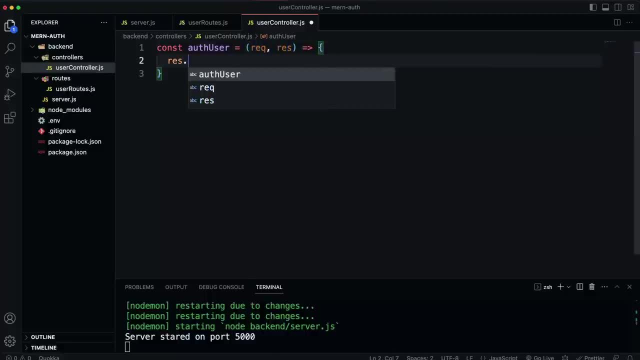 I'm going to say split a response, And then all I'm going to do for now is just do a rez, dot JSON. Actually, I like to do the status as well, So we'll say status 200. And then dot JSON, And then 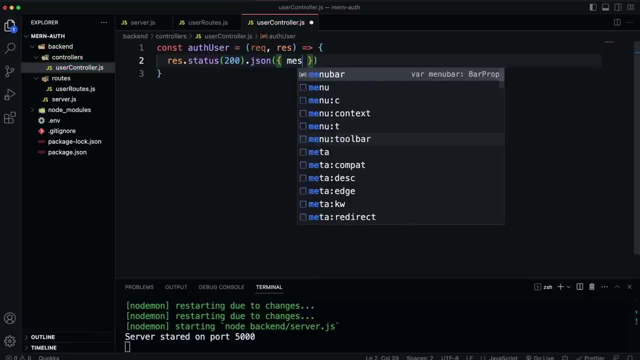 we'll have in here just a message for now. say message and we'll say off user, just whatever the route does. okay, just just to get started Now. But what I like to do and if you guys have taken any courses from me where we use Nodejs: 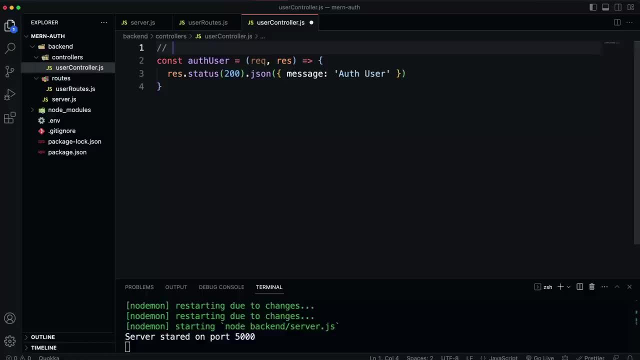 and we use routes. I like to create a couple comments here. So first is going to be the description of what this does. So we'll say auth user and let's say slash set token, And then I also like to put the route, what the route is going to be, which in this case. 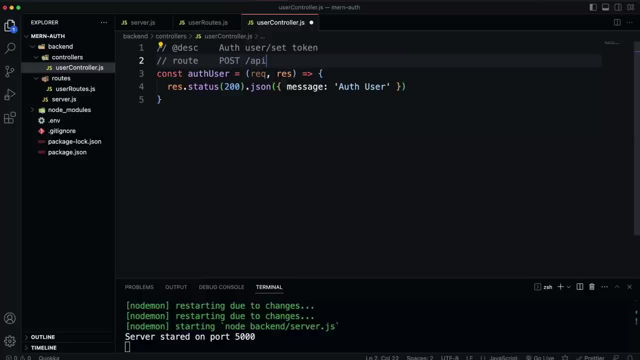 is going to be a post request to slash API, slash users, slash auth, And then also the access. So is it protected or not? Is it private? So this one is going to be public, And that just means that you don't have to be logged in to access this route. 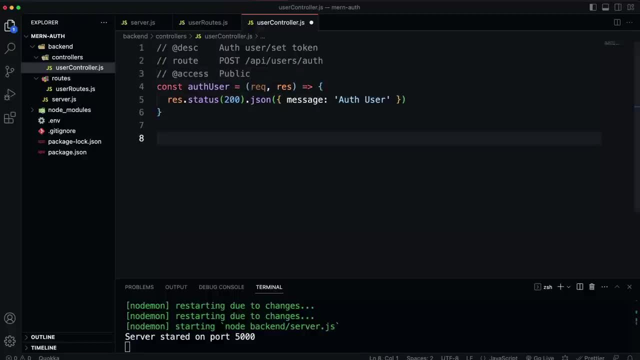 It's not protected. So before I create any other routes, I just want to export this one. So I'm going to say export And we're going to say export, So we're going to be exporting a bunch of functions from here. 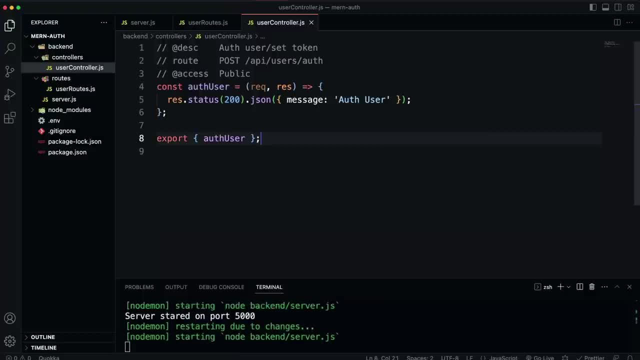 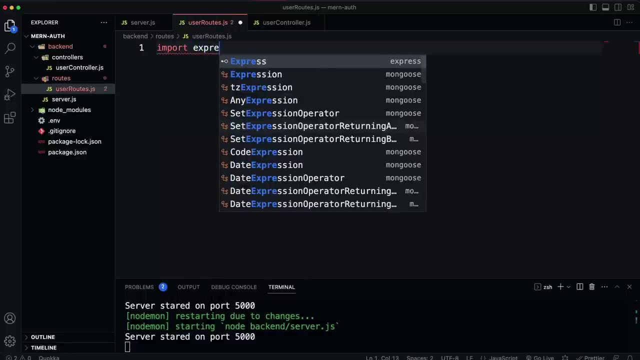 So we're going to use curly braces And then let's export auth user And then what we'll do is go into our user routes And in order to use the express router, we first need to import express from express And then we can create the router. 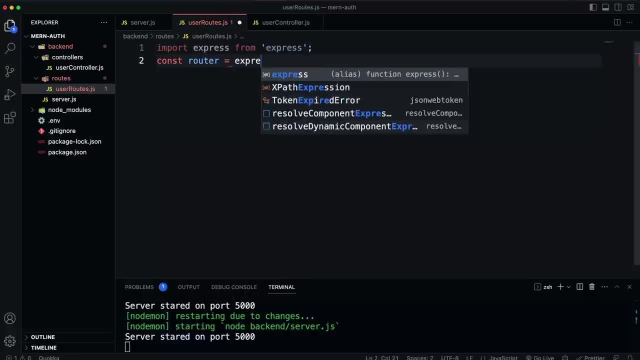 So let's say const router equals express dot router with an uppercase R, All right, And then, And then this needs to be exported. So let's say export as default router, And then what we'll do is say router, We want to handle a post request to slash auth. 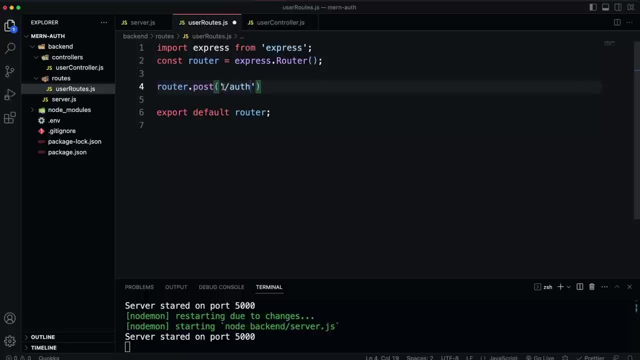 And the reason I'm not putting slash, API slash users, slash auth is because API slash users is going to be connected to this whole file, So we only need to put whatever would be after that And then I'm going to have my auth user. 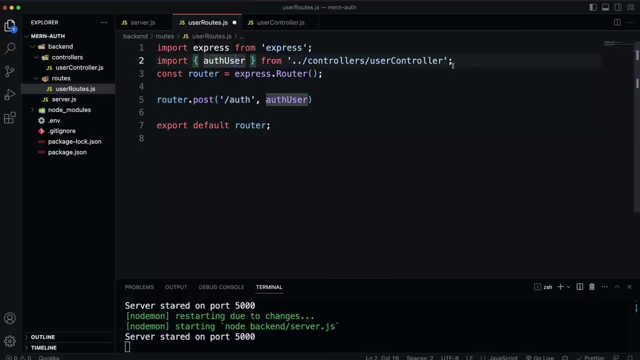 My controller function here which I just auto imported as our callback And I'm just going to move this down. And one thing I want to mention is that since we're using ES modules on the back end by putting type module in the package dot JSON. 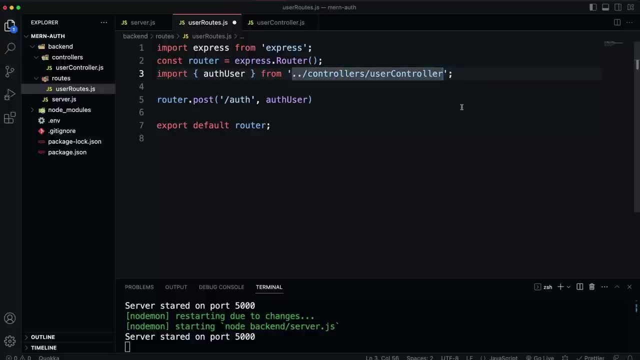 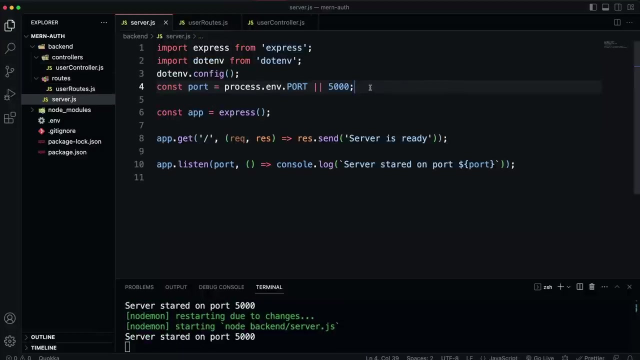 when we use the import syntax and we're importing our own JavaScript file, we do have to add the extension or it's going to give us a module not found error. So just be aware of that. So we'll go ahead and save, And the last thing we need to do to try this route is in the server JS. 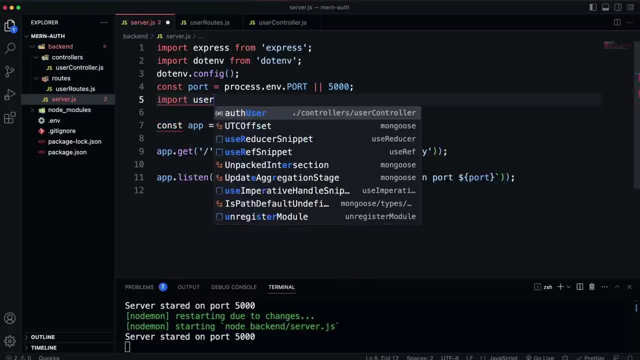 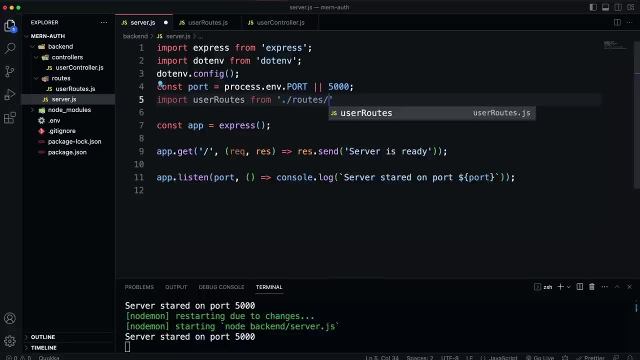 We're going to import our user routes, So user routes, And that's going to be from dot slash. Let's see Routes slash- user routes- And be sure to add dot JS onto it If you're using the import syntax, like I am. 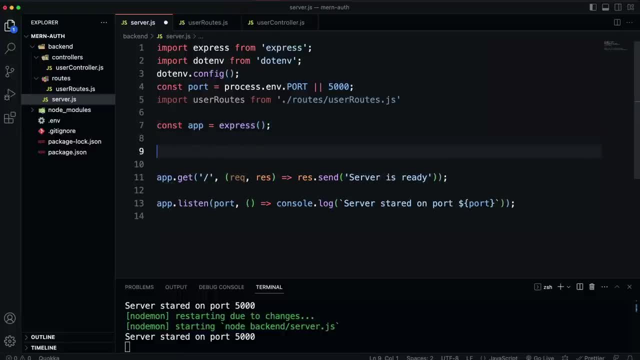 And then let's go right above the app dot get here And we're going to say app dot use And save And save for anything where we go: API users. That's going to be connected to the user routes. Now I'm going to be using Postman to test everything out. 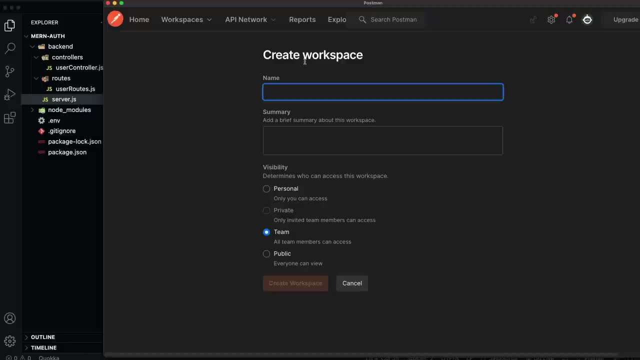 So I'm going to open that up And I'm going to create a new workspace, which you don't have to do. You can simply just open up a new tab and send the request. But I like to set it up like this: 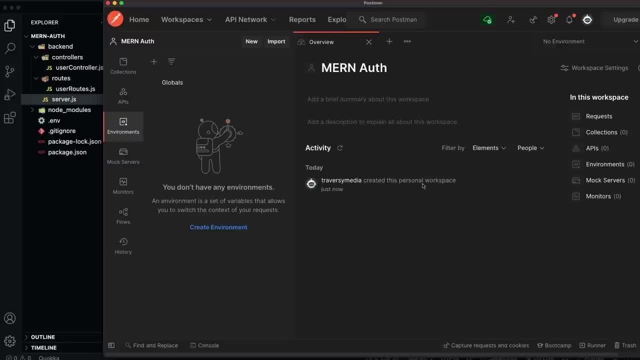 So burn off. I'm going to make it personal, Create workspace And, like I said, you can just open up a tab and make a request, But what I'm going to do is create a new environment. So right here under environments, let's say new. 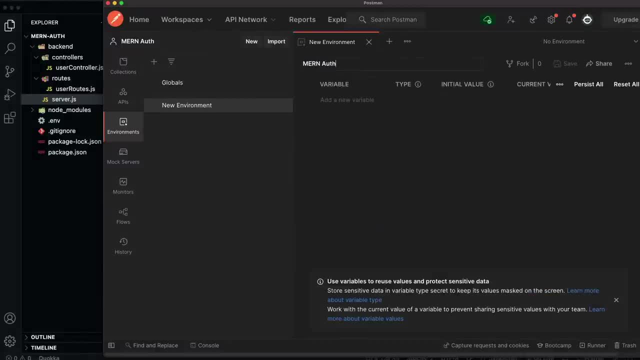 And then environment, And I'll call this mern auth, And I'm going to add a variable for the API URL. So we'll say, actually we want to put the name of the variable here, So base URL, And then here we're going to put HTTP, local host, port 5000 or whatever port you used. 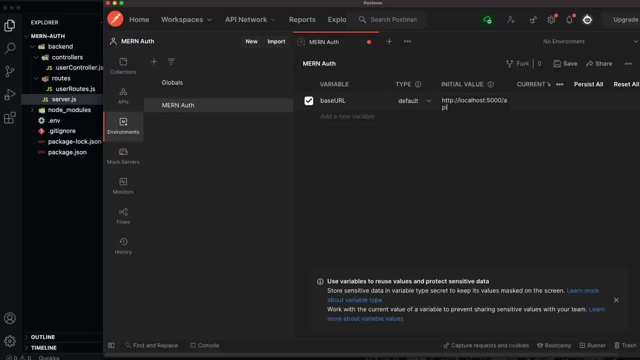 And then slash API. Okay, I'll put that there, And then, for the current, we're going to put the same thing. So, HTTP, local host, port 5000, slash API. All right, Now what we'll do is save this, first of all. 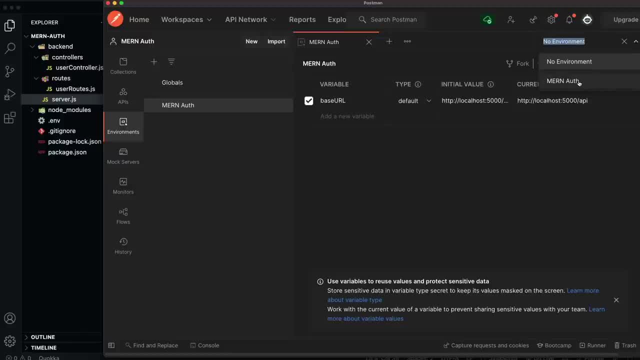 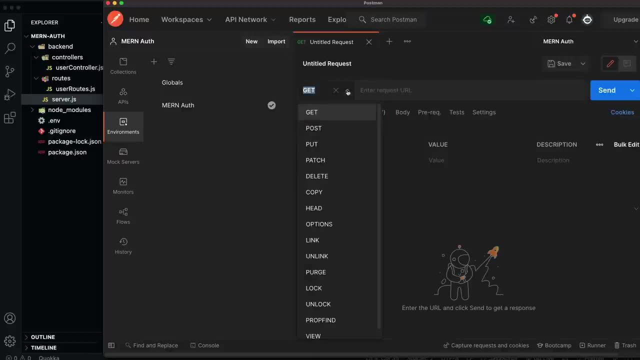 So click save And then on right here, where it says no environment, I'm going to choose mern auth. So now what I should be able to do is create a new request and make it a post request, And I'm going to do double curly braces and then base. 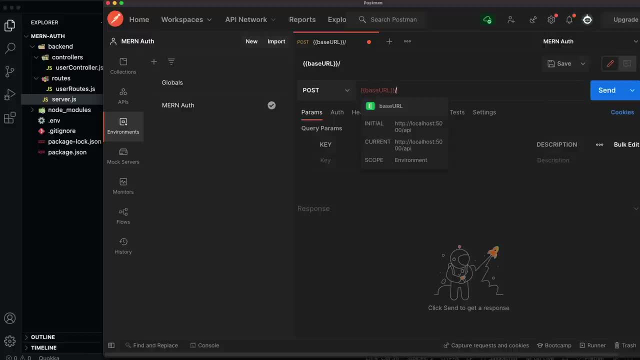 And you'll see it comes right up base URL And then all I have to do is slash users slash auth, Because the local host slash API is already in the base URL, So let's send that. Make sure it's a post request. 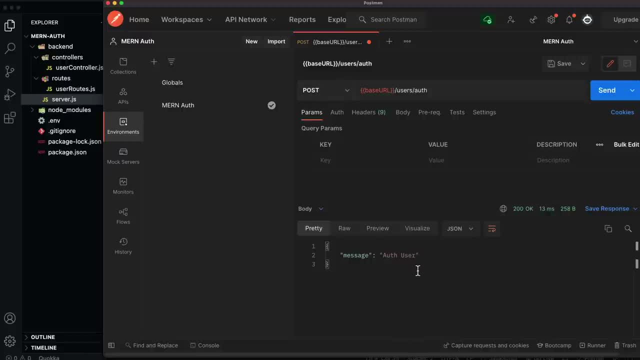 And you should see message auth user, Because obviously we have no functionality yet. It's just going to give us this message object. All right, Now I like to save my requests in collections As well, So I'm going to go to collections and say new. 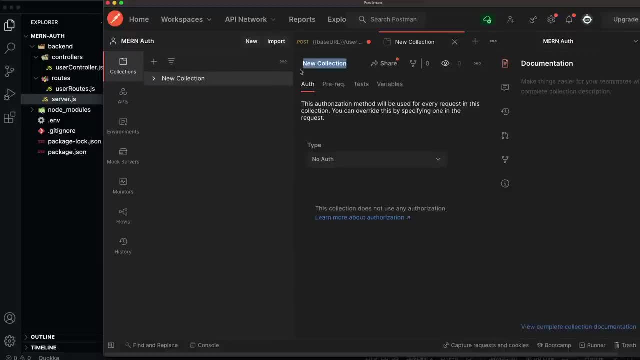 And collection And we'll call this users, And yeah, I think that should do it. So users, And then inside collections is where I want to save this request. So let's see If I go right here and say: save as. 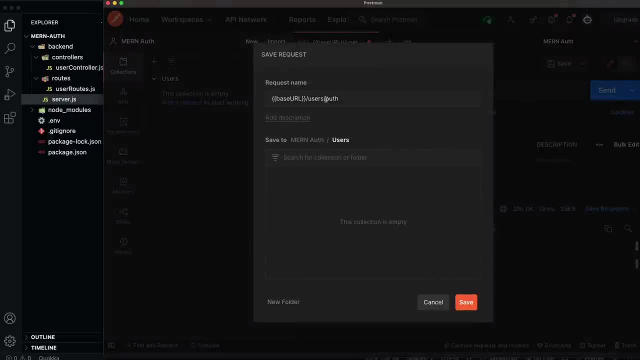 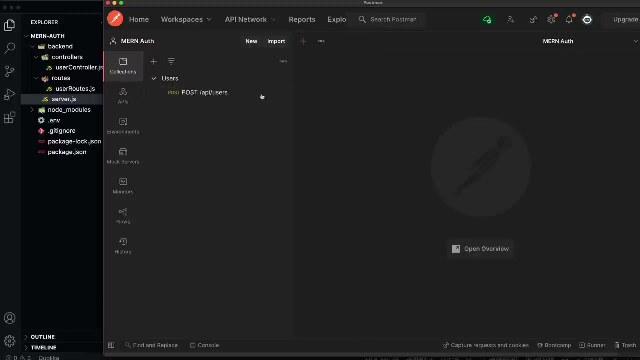 And then choose users And then the request name. What I'll usually do is save And then I'll say like post and then whatever the- let's say- API slash users. So now I have this request saved So I can always just come to it and I can make that request. 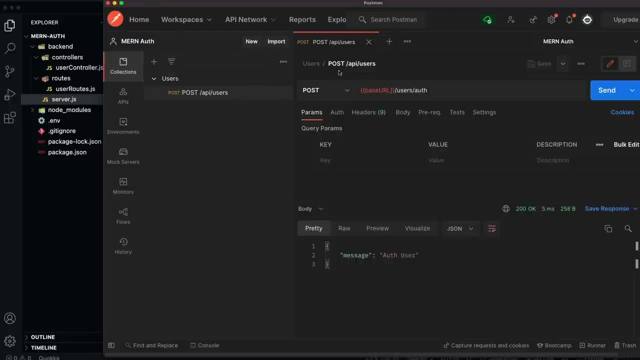 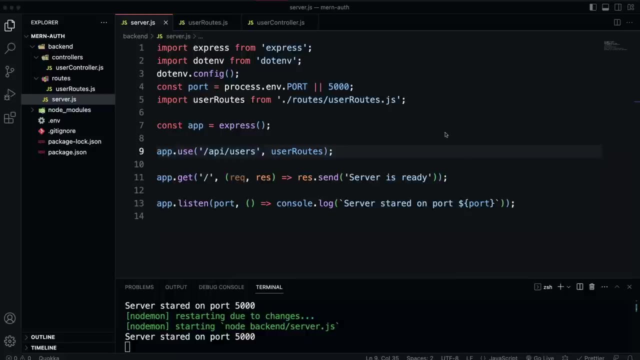 All right Again, you don't have to do all that set up. You can just pop open a new tab and use it. All right, Cool. So let's see The next thing that I'm going to want to do before I add the rest of my controller functions. 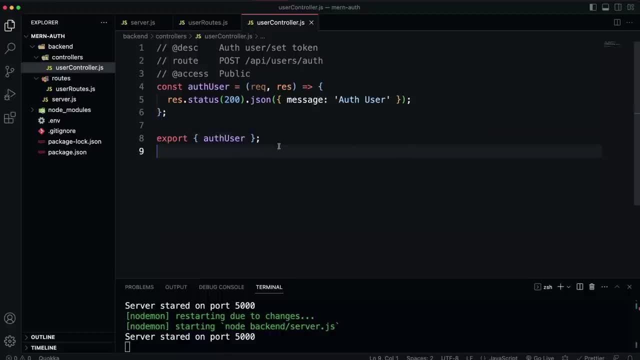 we're going to use an async handler because the mongoose methods that we're going to be using within these functions return a promise And I want to use a sync await, So we're going to be making all of these async, Okay, So we'll put that there for now. 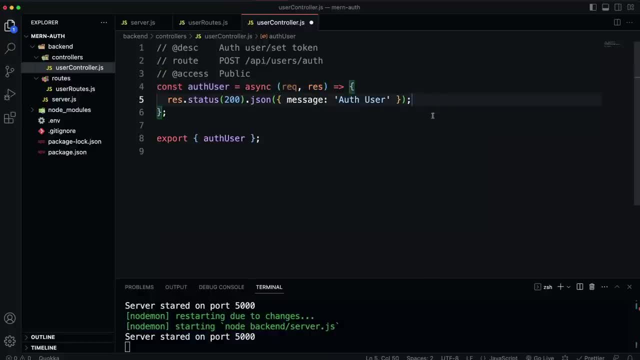 And we don't technically have to use an async handler. We could just put you know a bunch of try catches, But what the async handler will do is we wrap it around each controller function and it will handle the errors And it will allow us to use our custom error handler, which we're also going to create soon. 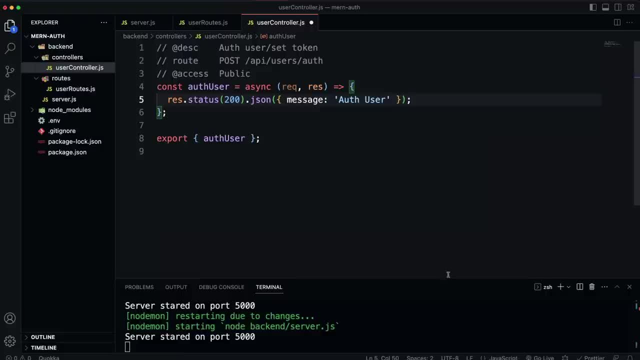 Now there's a few ways we can do this. We could create our own, which is what we did in the e-commerce course, But I'm going to actually just stop the server and install express dash, async dash handler, And then we can run the server again. 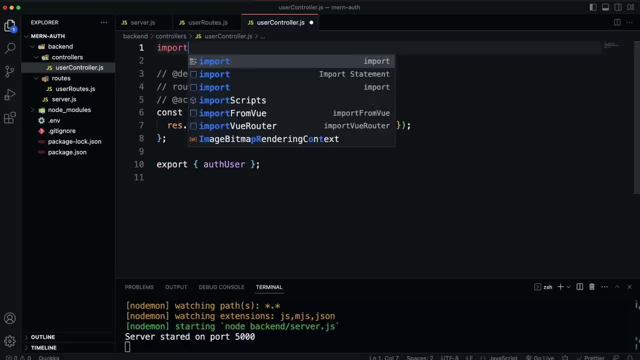 And all we need to do is bring it in. So let's import, say async handler, And that's going to be from express async handler, And then for all these functions we just want to wrap it. So I'm going to go right here at the beginning of async and say async handler, and then an open parenthesis. 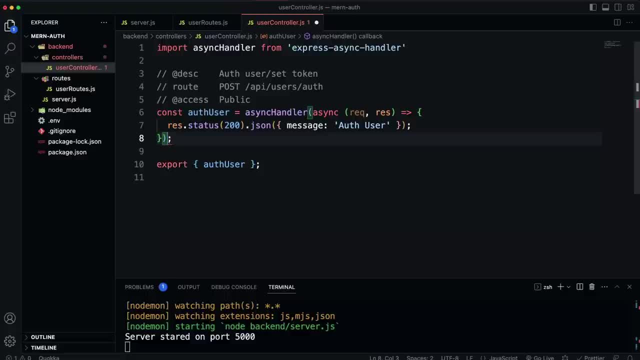 And then just put the ending parenthesis at the very end here after the ending curly brace, And that's it. So I mean it's not going to make any difference right now, But it will allow us to use a sync await and not have to wrap everything. 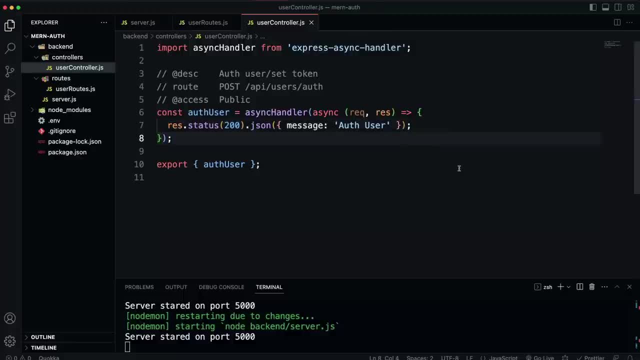 In try catches All right. So now that we've done that, let's create our custom error handler. So we're going to actually create a middleware folder. So in backend let's create a folder called middleware And inside that let's create a file called error, middleware. 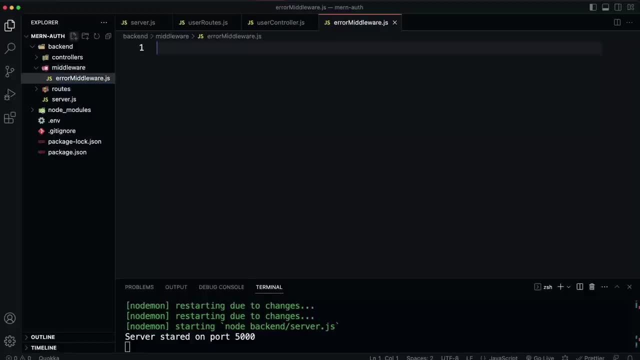 Yeah, error middleware dot JS, Because the default middleware for express it's an 80.. And we're creating an API, So I want our errors to just be a JSON object that has an error message and the stack trace if we're in development. 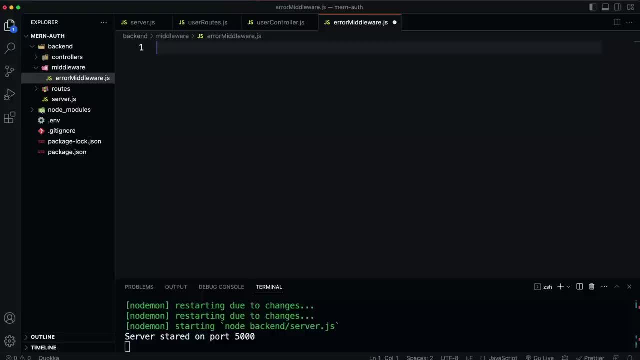 So we're going to create two middleware functions here. The first one will be used as basically a catch-all for any routes that don't exist. So if you go to some route that you know we don't have a controller for, then this will be thrown. 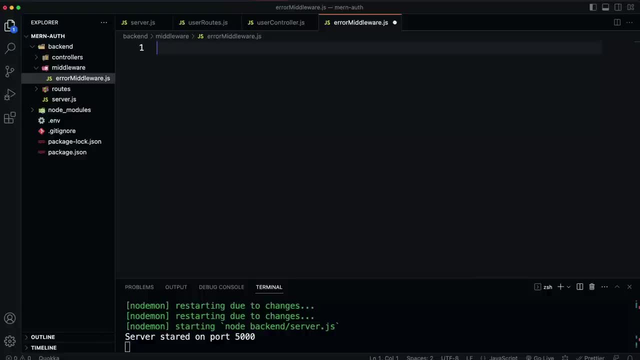 The second will be used as a catch-all for any errors that occur In our routes. So in our routes we'll be able to say throw error, and then put some kind of message in here or throw new error, And that's what I want to be able to do. 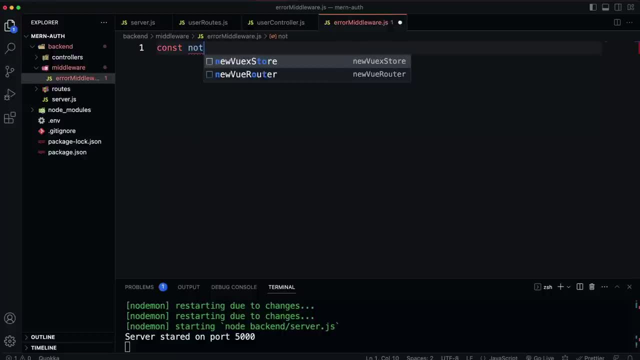 So the first one is going to be called not found, And this is going to be a function that takes in request response, and next, Next, is just the callback that we fire off once we're done And we're basically saying: run the next piece of middleware. 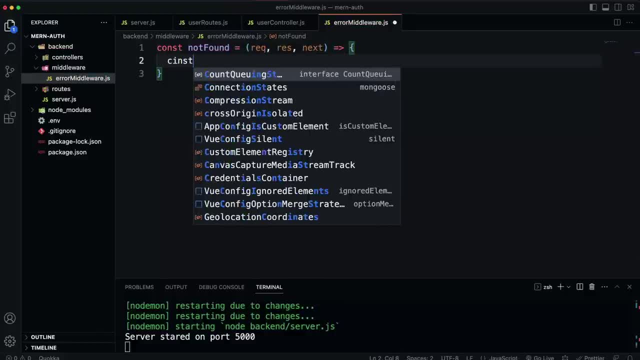 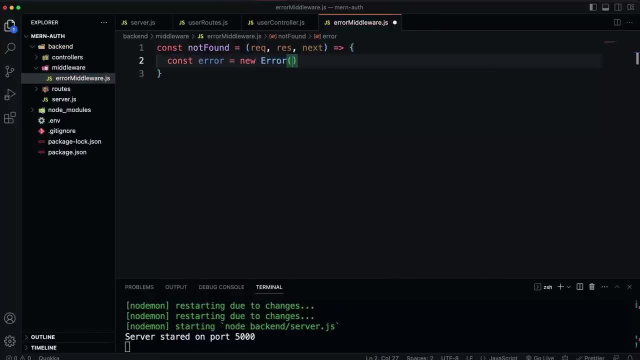 So all I'm going to do Here is say const error and say new error, And in backticks here we'll say not found dash, and then whatever the URL is. So request on the request object: we have an original URL property. 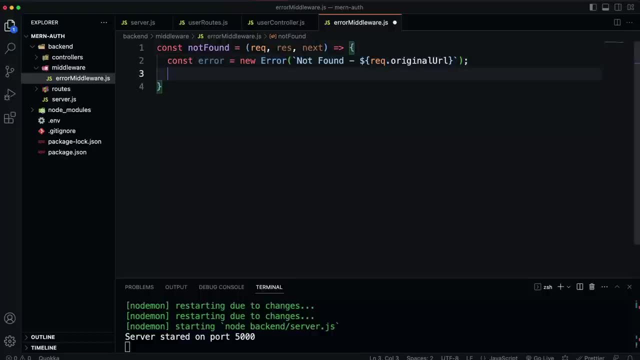 So we're just going to output that And then we'll set the status. So, resstatus, We'll set that. We'll set that to 404, which means not found, And then we'll go ahead and call the next piece of middleware. 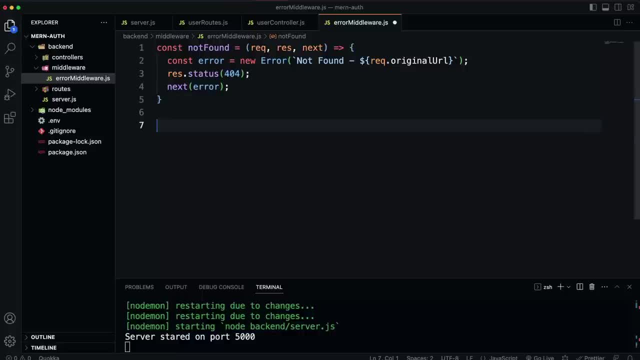 And we're going to pass in that error. OK, So that's the first one. The next one we're going to call error handler And this is going to take in in addition to request response. next, it's going to take in the error as the first argument. 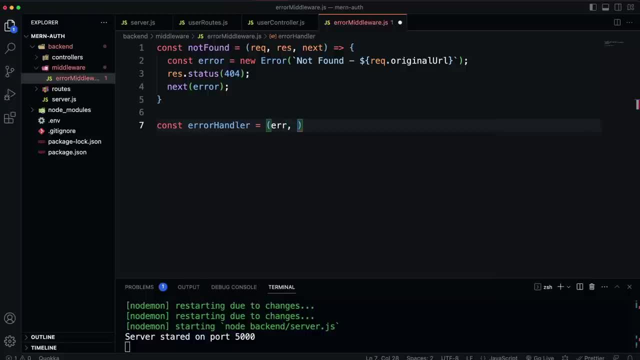 And if you do that, Express knows that this is your custom error middleware. So let's say request response Next, And then we'll have our function here And I'm going to just initialize a variable called status code And basically we're going to set this to resstatuscode. 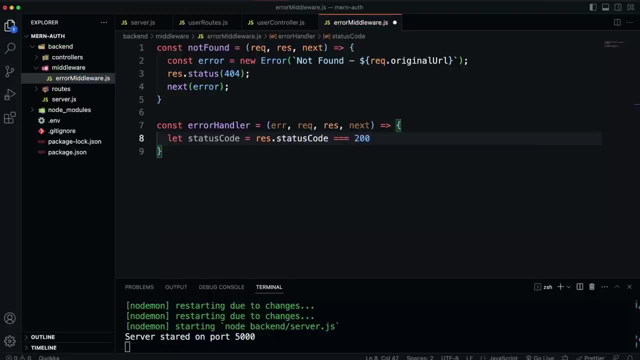 And we're going to check to see if that's equal to 200. Because if we throw an error, a manual error that we're creating, the status might still be 200. But if we're throwing an error we don't want to. 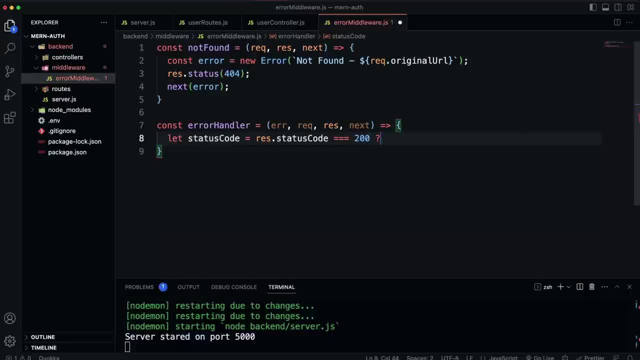 We don't want it to be 200. So we're going to say: if it's equal to 200, change it to 500. Else then, just use whatever resstatuscode is. So if it's not 200, just use whatever it is. 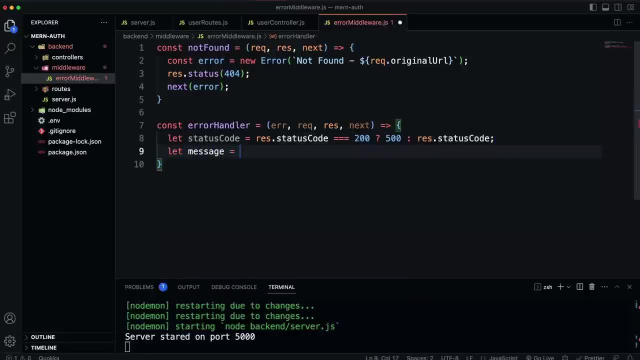 All right, Then we're going to initialize a message variable as well, which we'll set to errormessage. OK, So the message that's on this right here. Now, with Mongoose, we have a specific type of error called a catch. 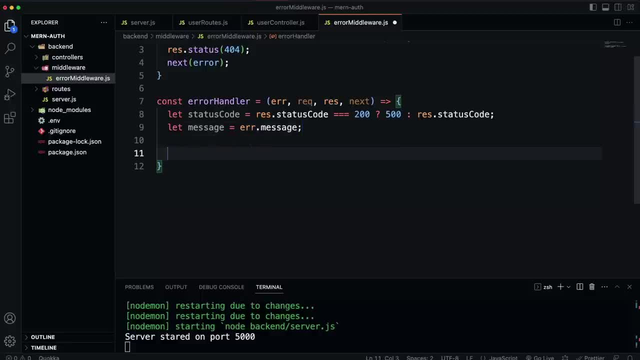 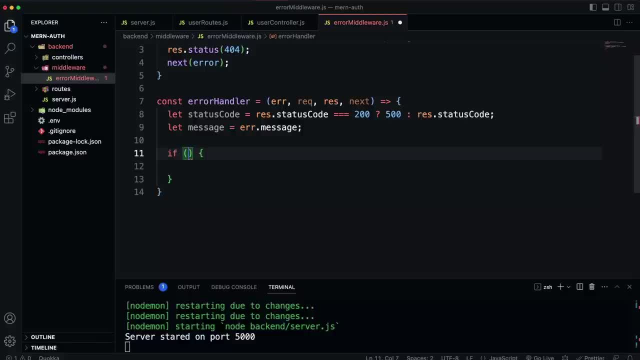 So I actually want to check for that. So we're going to say if the errorname because it has a name property and if it's equal to castError and we can check the kind It has a kind property as well. 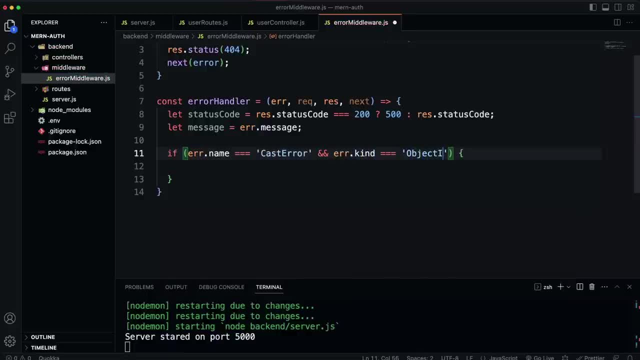 And we want to check that for objectId. So, basically, if you try to get a user with an objectId that doesn't exist, then this is going to fire off, And if this does happen, then I want to set the status code to 404, which is just a not. 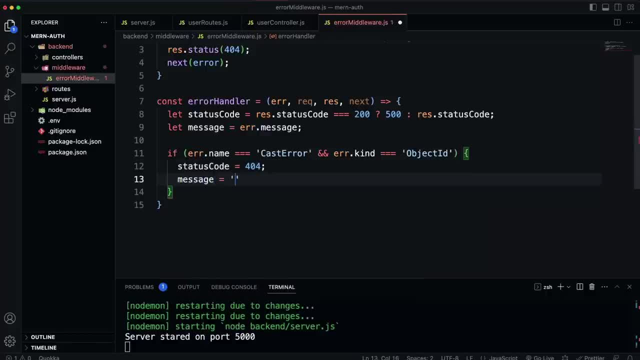 found. And then I'm going to set the message equal to, let's say, resource not found. OK, So we're just adding on to these variables up here that we initialized. And then, finally, we want to set a status, so resstatus, whatever the status code variable. 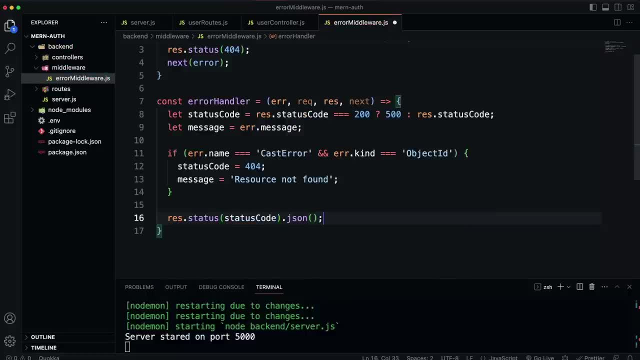 is, and then json, And what I want my errors to look like. like I said, I just want it to have a message, which is going to be whatever the message is And, of course, since these are the same, we can just do that. 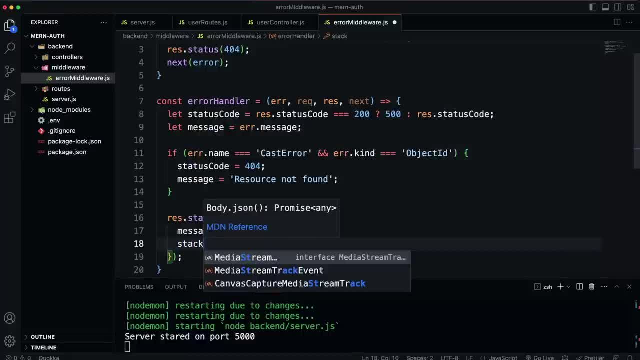 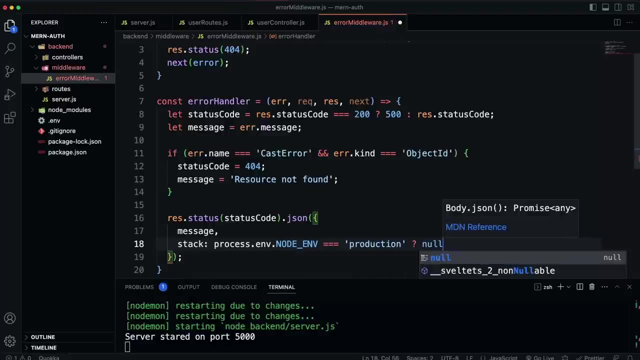 And then also we'll have the stack trace if it's in development. So I'll say stack and then processenvnet Node underscore env. If that is equal to production, then I want this to be null, else then I want it to show. 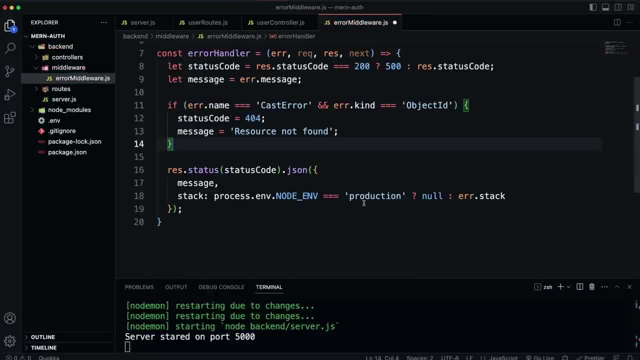 the error stack, which can be helpful, showing you the line numbers and stuff like that- files and line numbers- And then, finally, we just want to export both of these. So we're going to export the not found and we're going to export the error handbag. 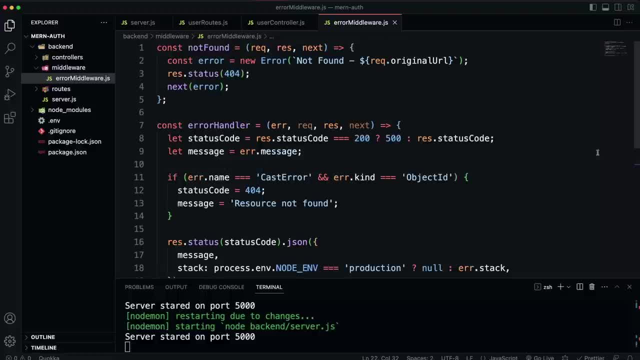 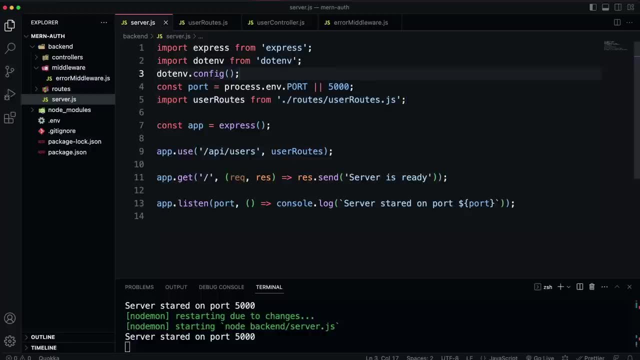 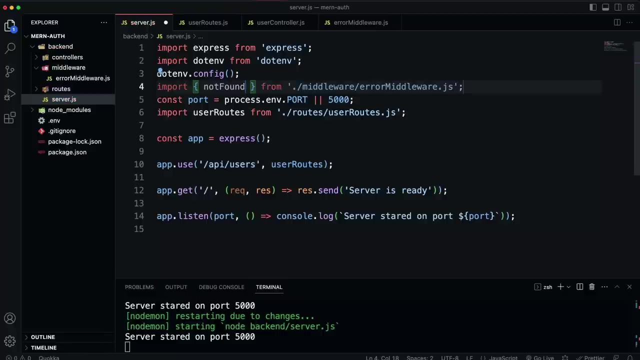 All right now. just creating these isn't going to do anything. We now have to bring them into our serverjs and add them as middleware. So I'm going to go right here and I'm going to import: not found and also error handler. 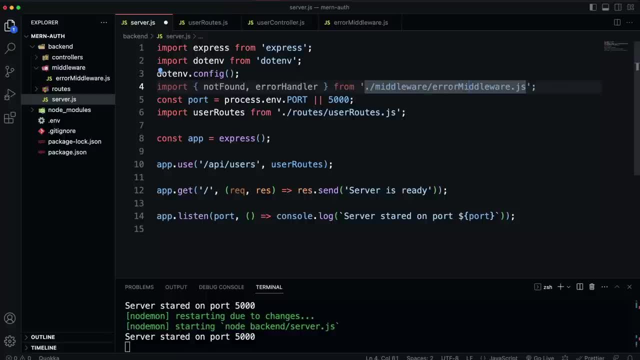 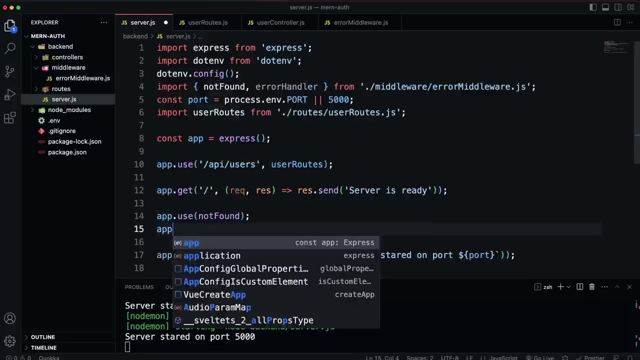 from the middleware slash error middlewarejs, And then we just have to pass those into appuse. So I'm actually going to put this down at the bottom right here and say appuse and not found and then also appuse error handler. OK, so that should do it. 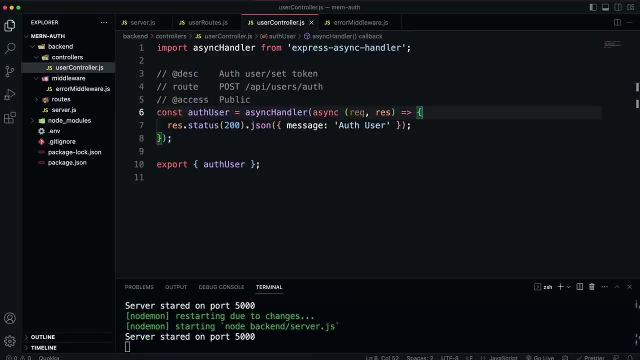 Now, if I were to go into my controller here and let's say something happens here where we want to throw an error, well, first I would set the status, So I'd say resstatus, And let's say I don't know, 401, which is a user error, a client error. 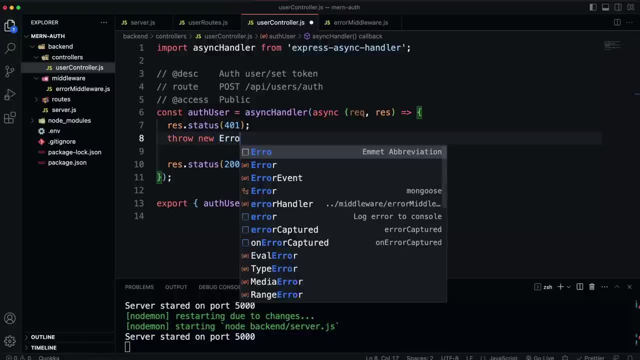 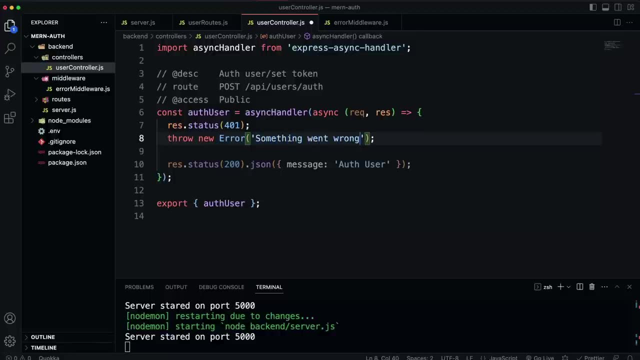 And then we could say: throw new error. And then I could put whatever message in here. I'll say: something went wrong. So now if I save that and I go back over to Postman and I send to that route, you'll. 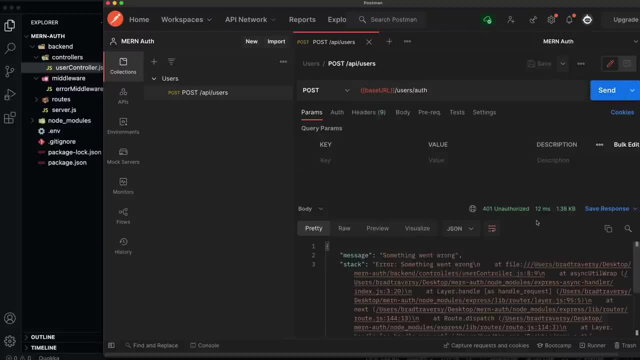 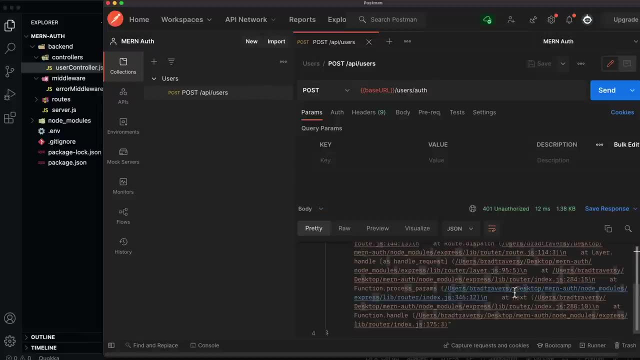 see I get back a 401, unauthorized- That's what it is, unauthorized- Which is still a client error, And then message: something went wrong. And then I also see the stack trace because I'm in development, right, And this would be null if I was in production. 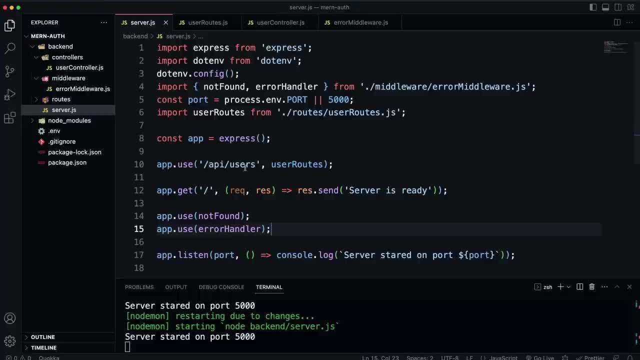 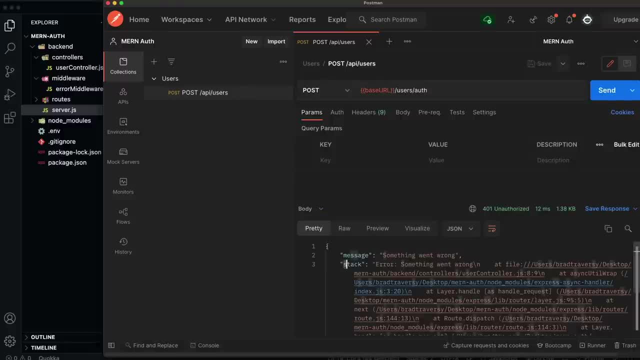 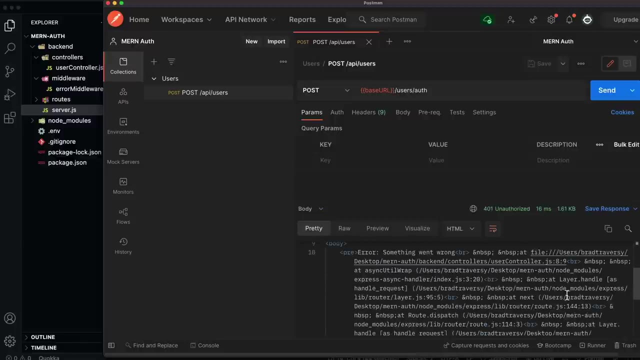 So that's pretty helpful. If we weren't using that custom error middleware- like if I comment these two lines out and then I go back to Postman and I send that- we get the default error handler, which is an HTML page, which of course we don't want. 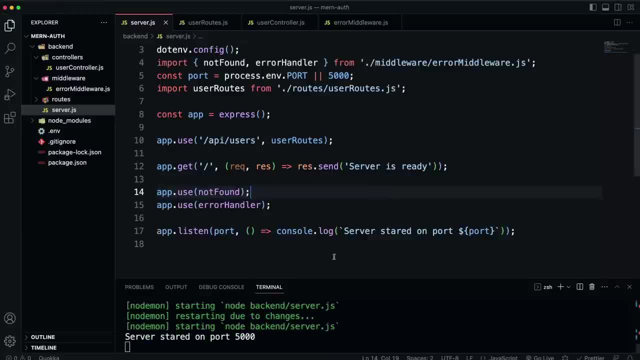 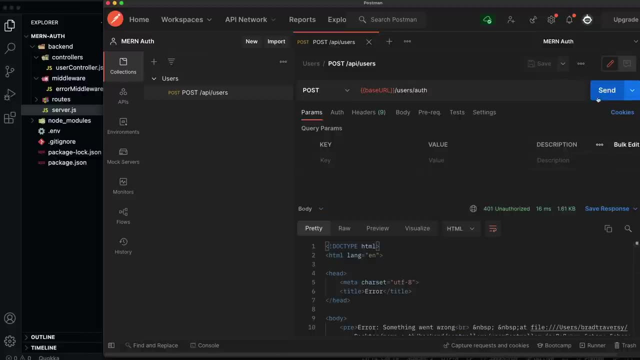 OK, So that's why I created a custom error handler, And you can do a lot more. This is just kind of the base error handler that I like to use in pretty much all of my APIs. But let's go ahead and we can close up the error middleware. 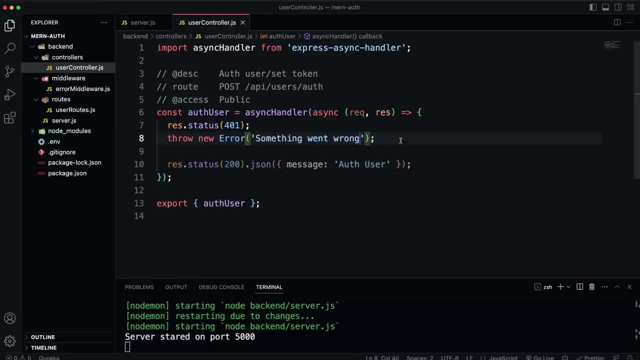 We can close up the routes for now, And let's get rid of that, what we just did, that error, And now I just want to create the rest of our routes And for now they'll just output a JSON object with a message. 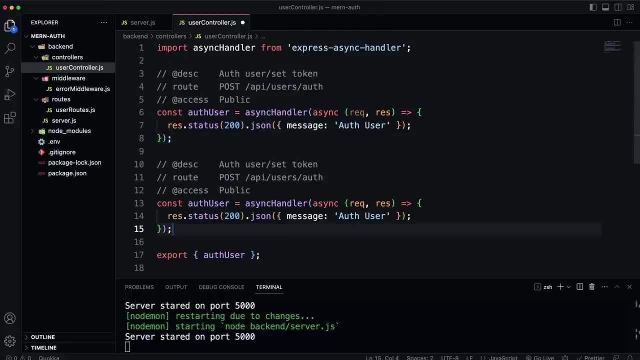 So let's copy this. So the next one is going to be to register a user. So let's get rid of this for the description and we'll say register a new user And the route is going to be a post request to API slash users. 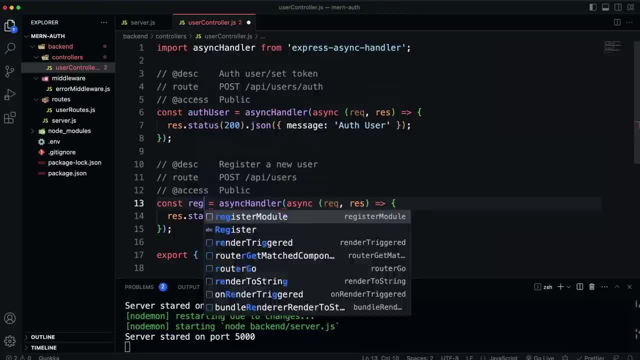 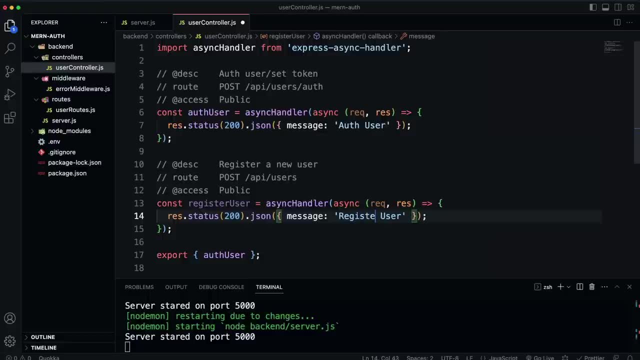 It's going to be public And let's change the name of the function to register user, And then, for now, I'm just going to send out a message that says register user. OK, And then we'll go ahead and add another function. 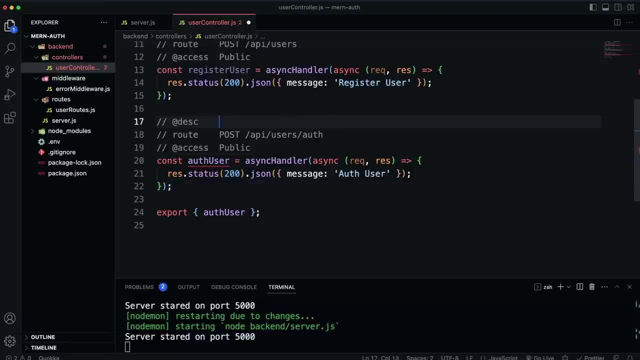 This one is going to be the log out. So let's say log out user And then we're just going to change the route here to slash log out And we'll change the function to log out user And then let's just change the message here. 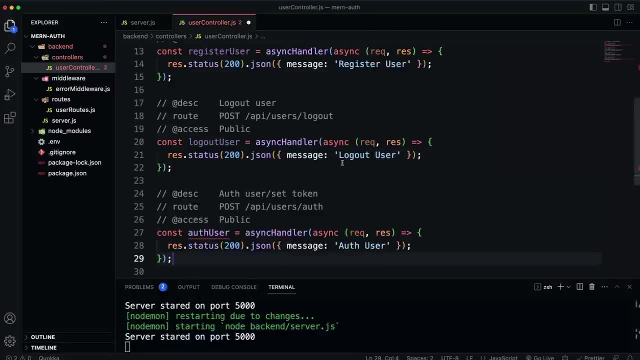 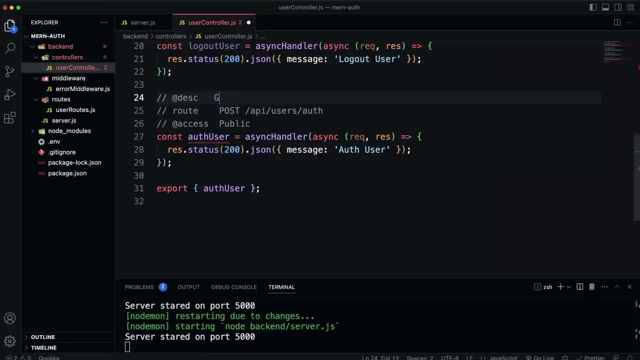 Log out user. All right, Then the next one is going to be to get the user profiles. So let's say, get user profile. It's going to be a get request And then it's just going to be API users slash profile. 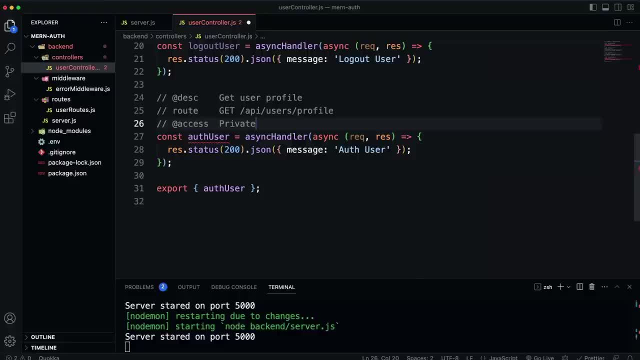 And this is going to be private. So let's say private meaning you'll have to have a token, You'll have to have a valid JSON web token for this. And let's make this: Say get user profile and say user profile. 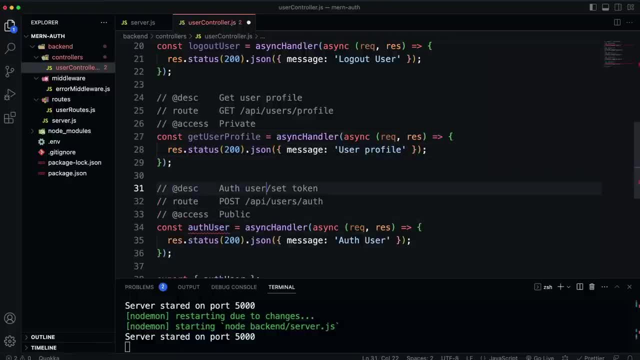 And then the last one is going to be to update the user profile. So let's say, update user profile, And it's going to be to user slash profile, just like the one above, except it's going to be a put request because we're updating. 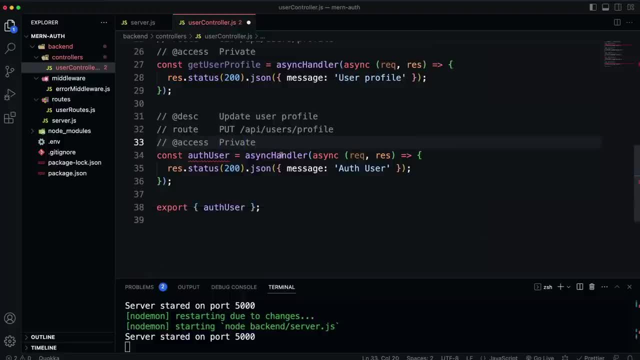 And that's also going to be private. Okay, And then we'll change this to, let's say, update user profile and change the message here. Okay, And then we just need to export all of these. So I'm just going to put this on the next line. 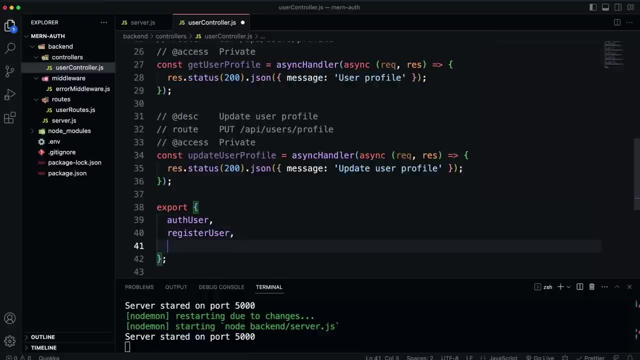 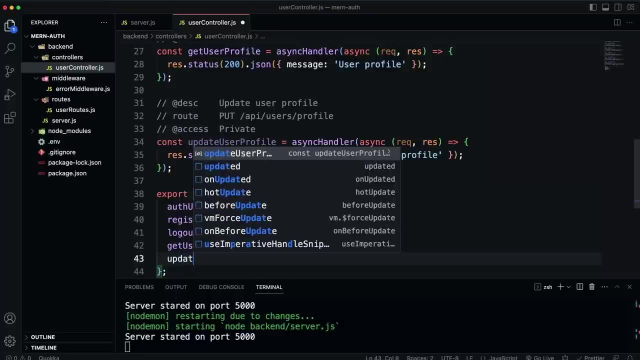 And then let's see: We have auth user, We have register user, We have log out user, All right, So we're going to do the same process for the other two lines of the same string. I'm just going to say: add user profile. 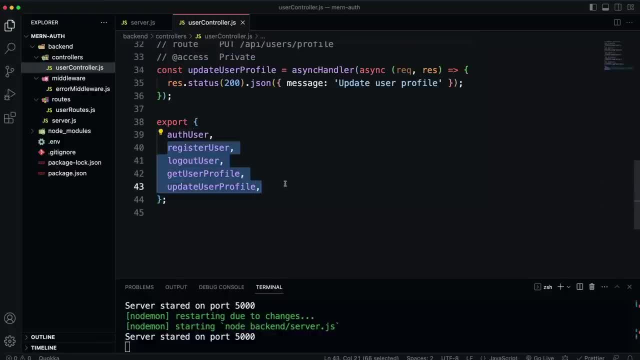 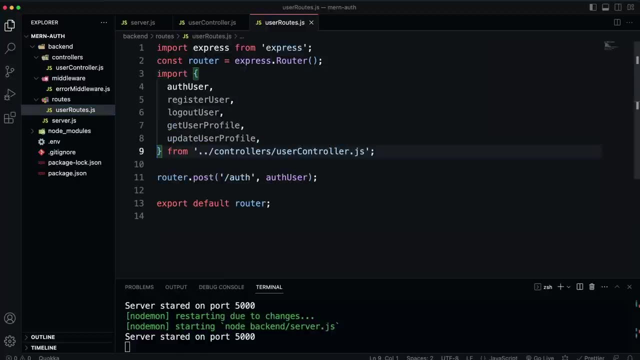 Get user profile and update user profile- Cool. So I'm going to copy these because we need to import them into our routes. So let's go to our user routes and right here, we'll just go ahead and import all of those, And now we just want to basically connect the routes to those functions. 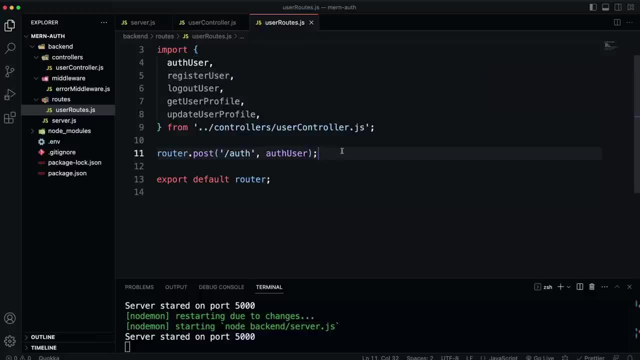 So let's see. I'm sorry for the register, So I'm going to copy that down Now. the register is just going to be to slash, because it's a post request to slash API, slash users. All right, so that's going to. 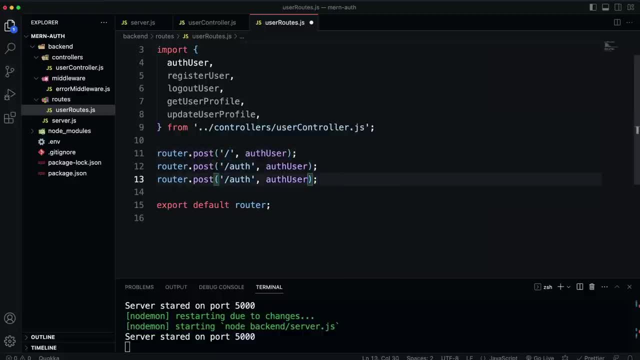 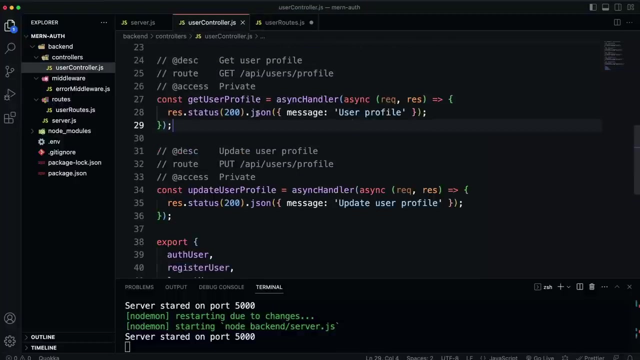 handle the register And then the logout. Let's copy that down. Let's say: logout users. So this will be slash logout and it will be a post request, So we can leave that. And then let's see, the slash profile is going to have two, two different methods, right? So 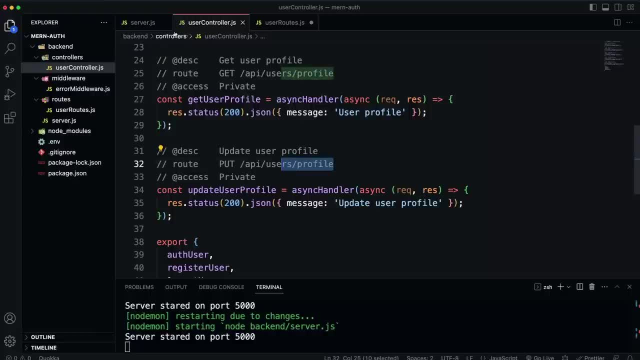 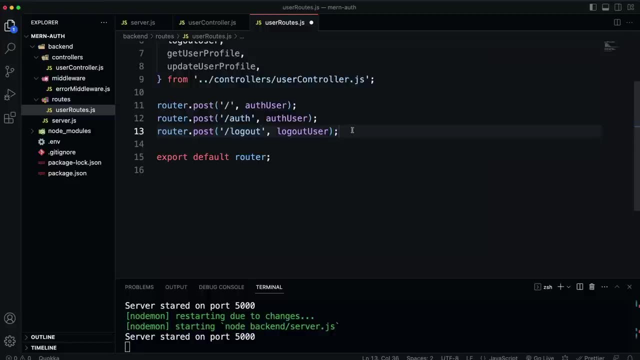 slash profile, slash profile, but one is a get and one is a put. So I could create two separate lines like router dot get and router dot put. Or we could do this: we could say router dot route and then put the endpoint which is going to be slash profile, and then just attach get. 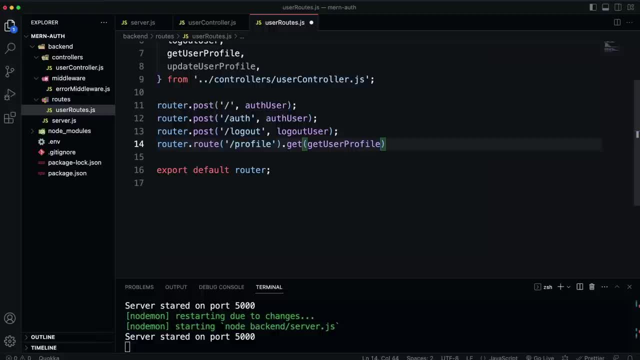 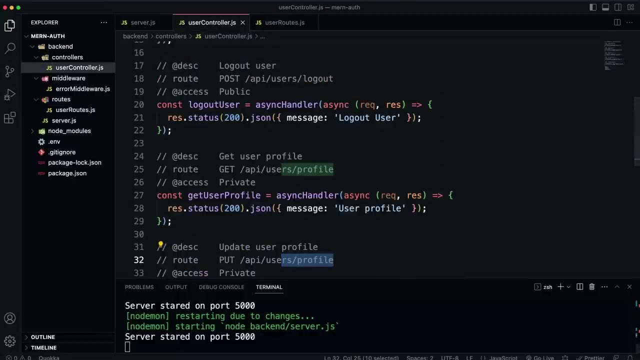 and whatever function i want for that which is going to be get user profile, and then i could also just chain on to that dot put and then in there i want update user profile. all right, so all of our routes should now be connected to these, um, to these functions in the controller. so we can test that out by going to postman and we can create these requests in our collection. and i'm actually going to rename this just so this is more readable. so we know that this will authenticate our login, let's say login user, for that route, and then right here for where the user's collection is. 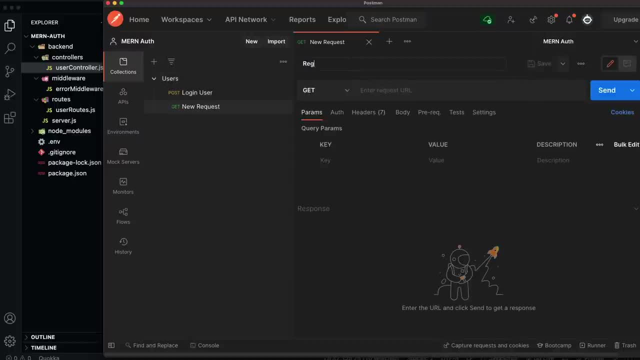 let's say add request and let's call this one register user and then that's going to be a post request to our base url, so base url, and then slash users. let's see, yeah, just slash users for the register. and if i send, let's see auth user. did i not change? 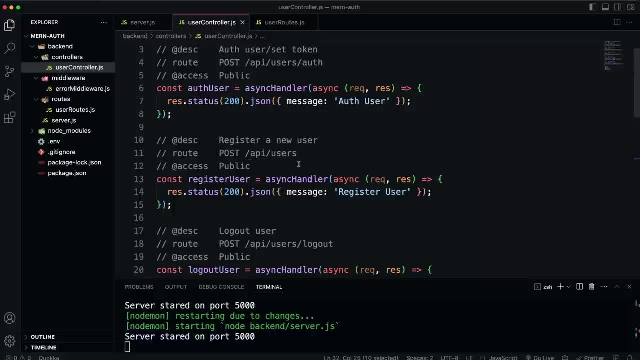 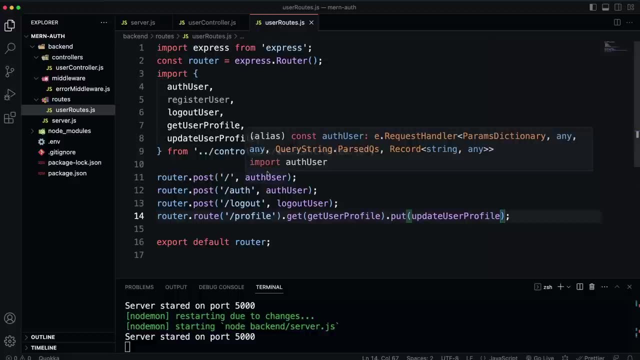 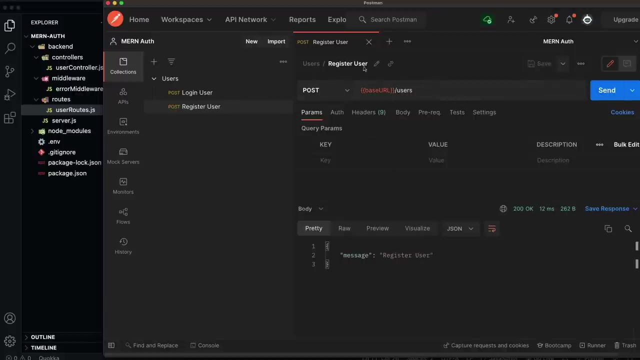 wait a minute. so registers a new user, post request to api slash users and then in our routes, routerpost. oh so, right, here this should be register user. okay, so now if i go back to postman, i send that again. now we get register user, which is correct, and i'm just going to save this all right. now let's create another. 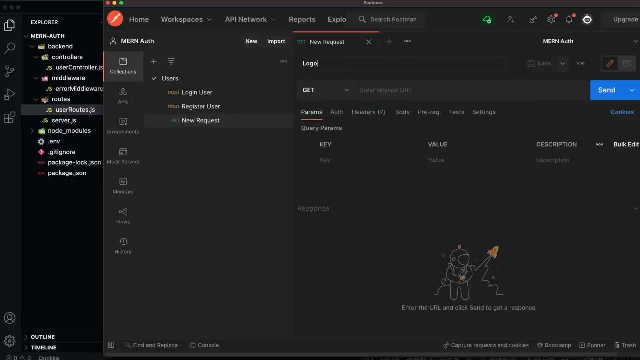 request. so this one, let's say log out user, which is going to be a post request to our base url and then slash users, slash logout, send it. we get log out user. i'm going to save that. now let's create another add request. this is going to be, let's say, get. 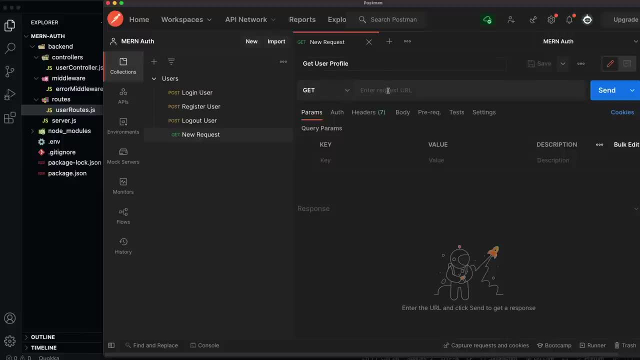 get user profile and it's going to be a get request to our base url: slash- users slash profile. okay, that works, let's save. and finally we have the update route. so let's go to add request and say update user profile. that's going to be a put request to our base url: slash- users slash profile. send that we. 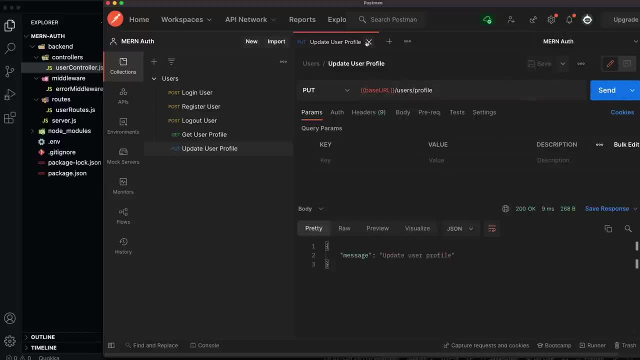 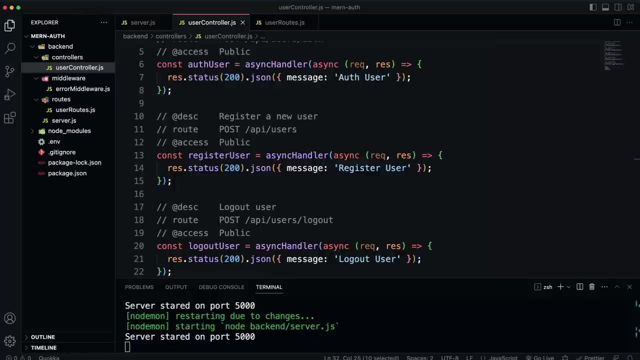 get update user profile. we'll save that. so now we have all of our authentication routes here that we can easily access and easily make those changes, those requests, okay, so now that we're set up with this, what I'd like to do in the next part of this video is set up our database and you can do that at. 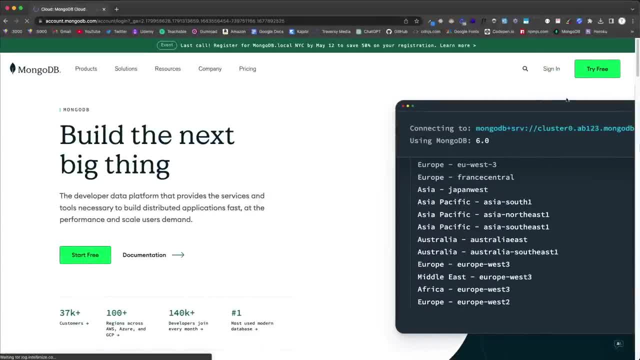 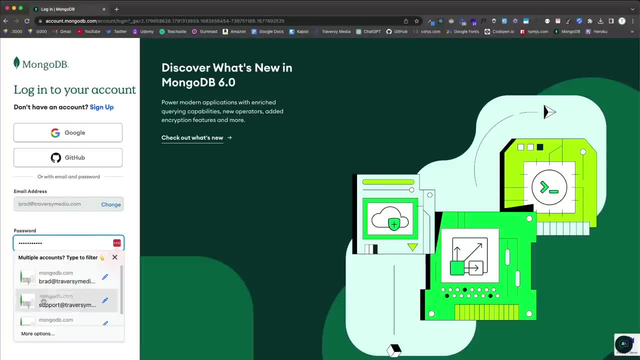 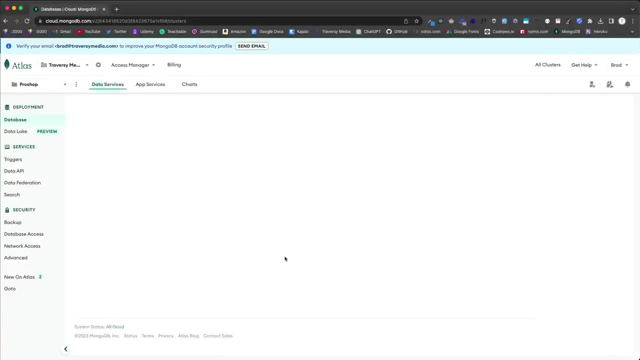 MongoDB comm. so you just want to sign in, sign up and sign in. I'm gonna use this. yeah, I'm gonna use this login here and I already have a database set up, but I'm just gonna go through and create another one. so, basically, when you sign, 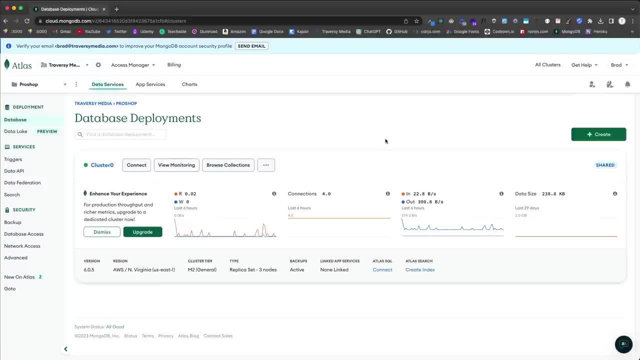 up and you sign in. you're not going to see anything. here. I've already created a cluster. so first thing you're probably going to be asked is to create an organization which I've created- Traversee Media- and then from there you'll create a project. you can see, I have one called ProShop, but I'm going to 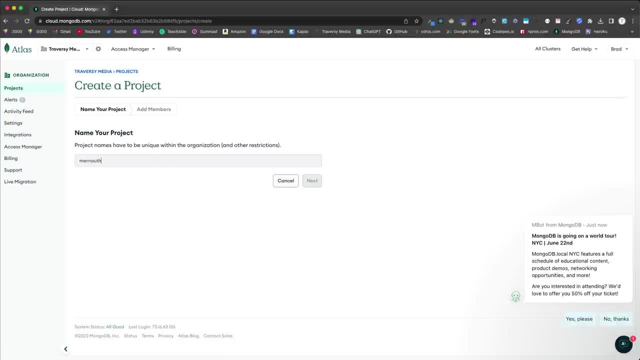 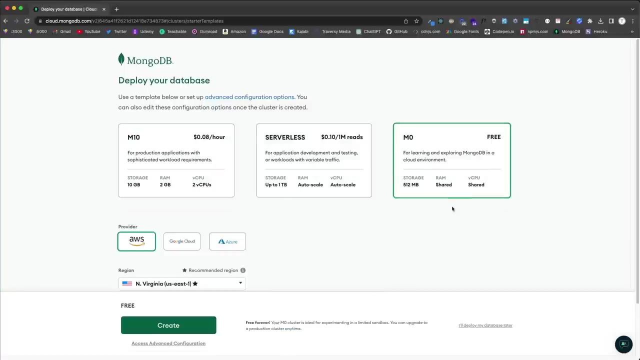 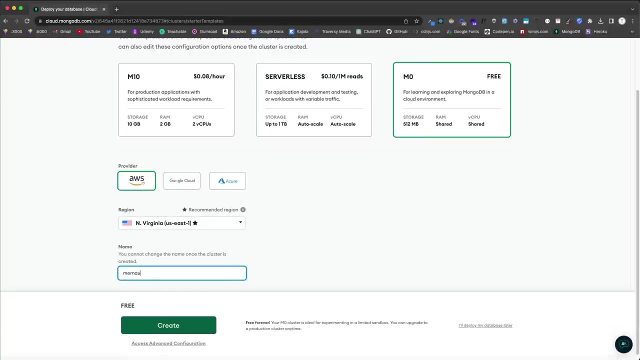 create another one here and just call it murn off and click Next and create project. okay, so once that's done, we can then build a database and I'm gonna choose the free package here. I'm gonna keep AWS is the provider. you can rename your cluster if you want. just call it murn off and then create. see some of these. 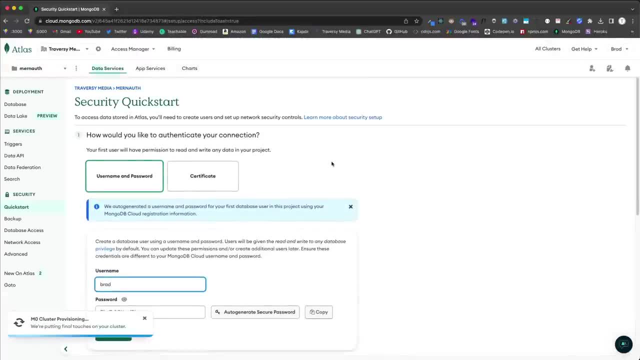 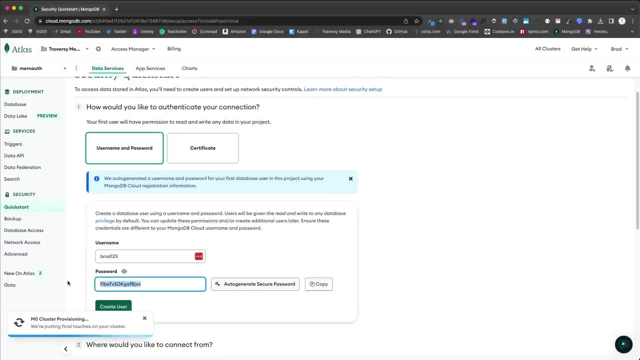 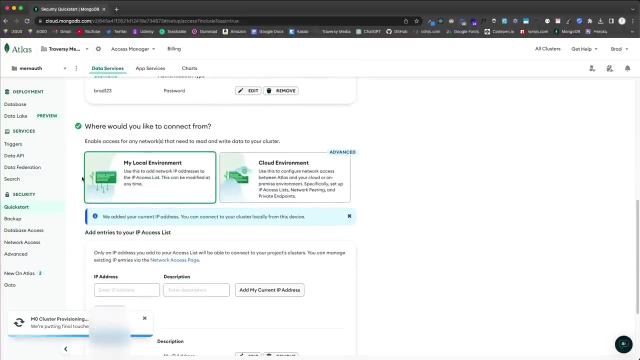 are just crazy. that one's an alright okay. so now you want to create a database user, so I'm gonna call mine just Brad, two, three password. i'm just going to do brad one, two, three for now, and then make sure you click create user and then from here you want to add your current ip address and it should already. 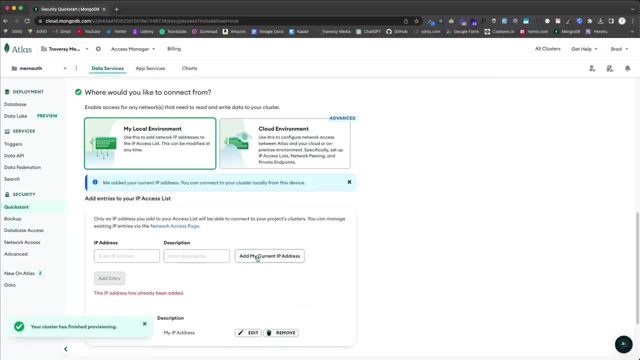 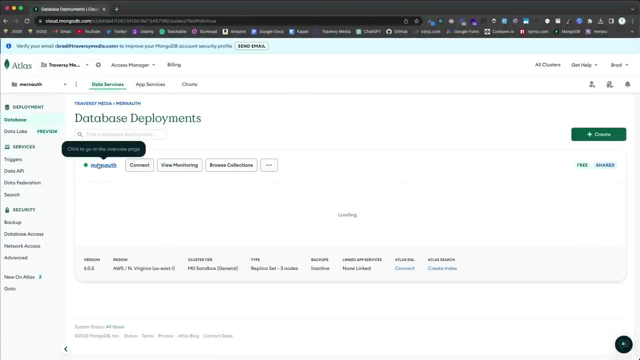 be added. if not, you can click on this and we should be good. so click, finish and close and then go to databases. and now you can see i have my mern off database and it's still being set up right now, but we should be able to still do some stuff, and what i want to do is go to browse. 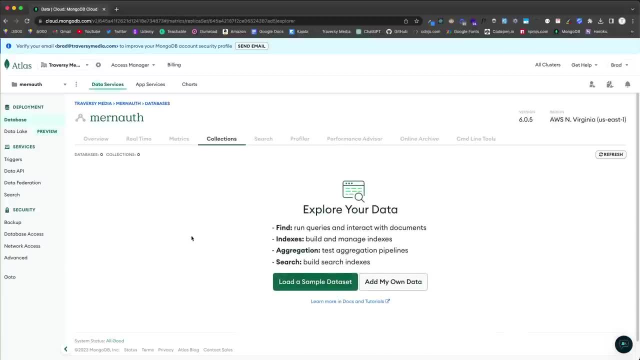 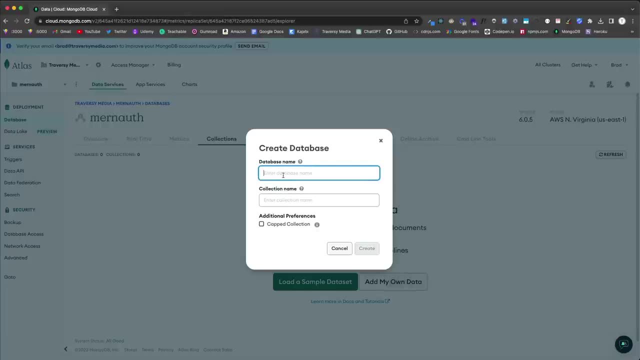 collections, and if we had data here you would see it. we don't, but i'm going to click on add my own data and here i'm going to give the database a name, otherwise it's just going to be called test. so i'm going to call it mern off and then a collection name. we're going to have a collection. 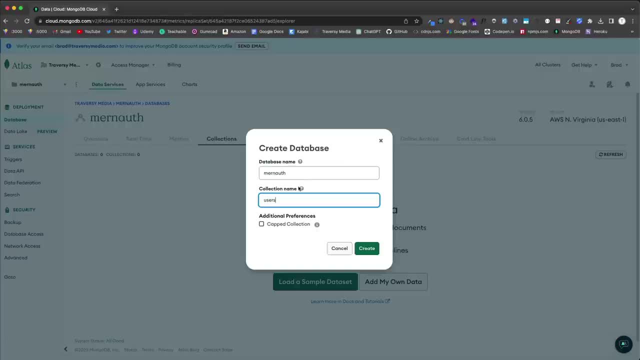 called users. so with collections you don't have to manually create them like this every time. you can just do it through your code. no, sql databases are very you have a lot of freedom and they're they're not strict at all like relational databases, where you have to, you know, create every table with all of the different columns. 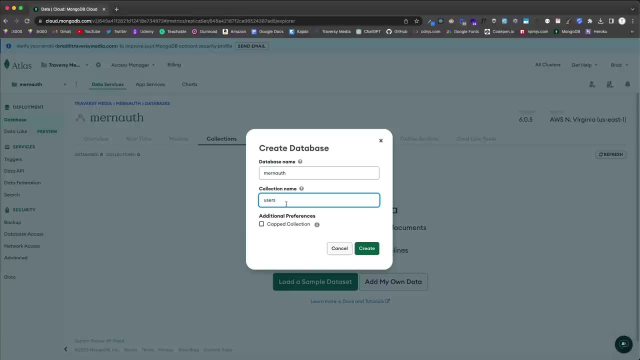 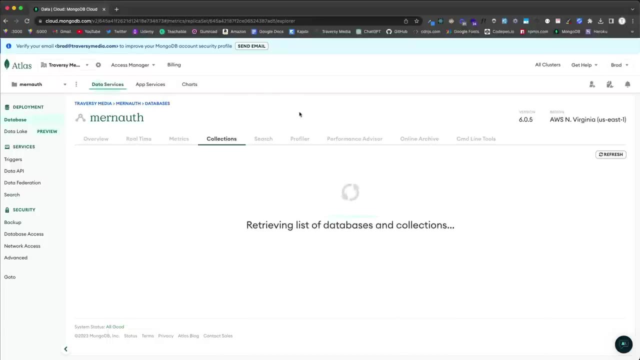 all the fields and the field types. they're there. you get much more freedom with no sql. you can do do all that at the application level. so let's click create and now we have a database called mern off with a user's collection. so now what we want to do is go back to this screen here. 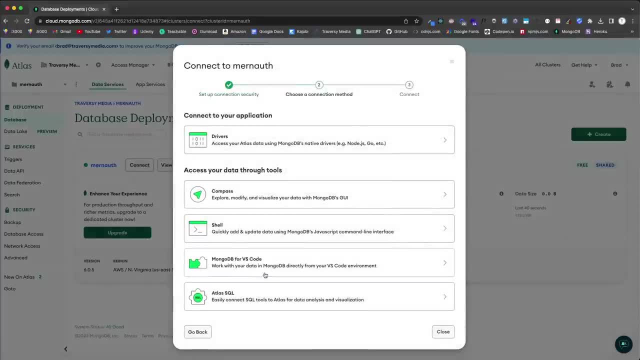 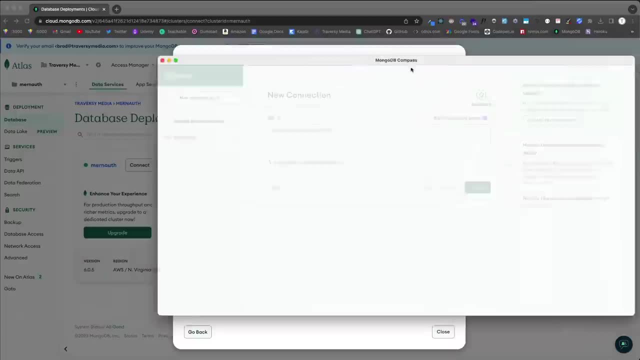 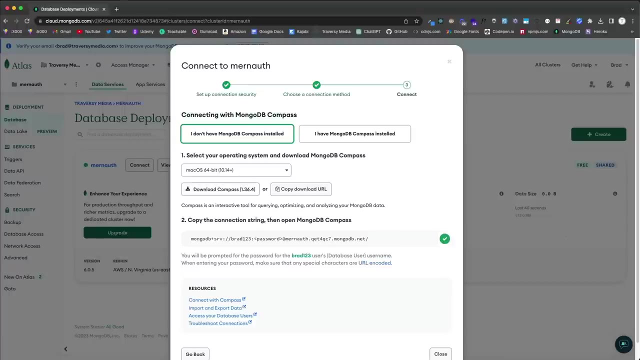 and click on connect and if you want, you can download mongodb compass. just google mongodb compass, download it. it's a desktop and if you want to connect to that, what you can do is open it up and right here where it says compass, you can click on that. copy that connection string. 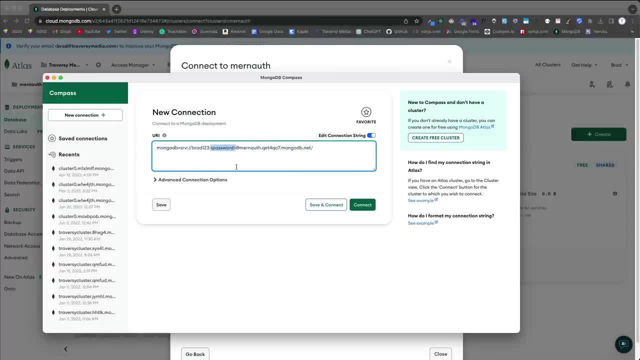 and paste that in here, and you just got to replace your password. this is optional. this is only if you want to use compass to see your data directly. so if we do that, i believe that should be good. all right, and over here you'll see mern off. 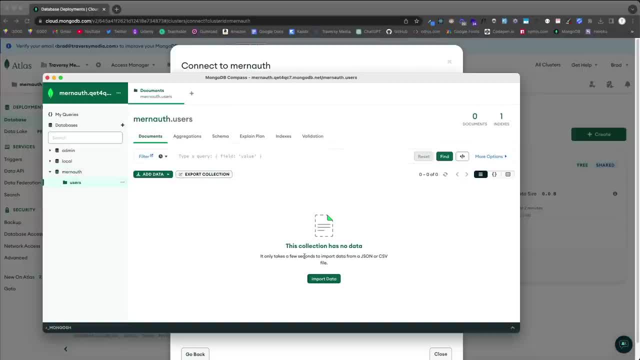 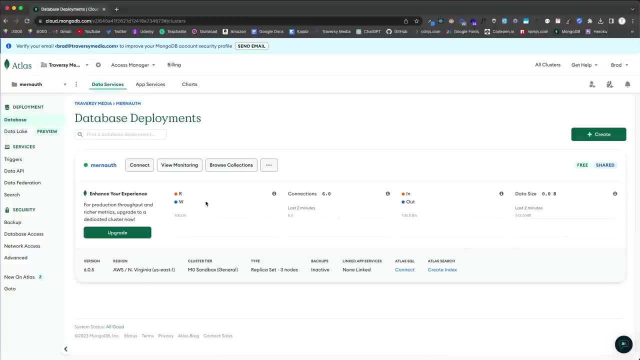 and we have our users collection. so if i had any data, it would show here, and i'm just going to keep this open, just in case we need it. so to connect, connect to our application. you want to again click connect, and this time you're going to click on drivers. 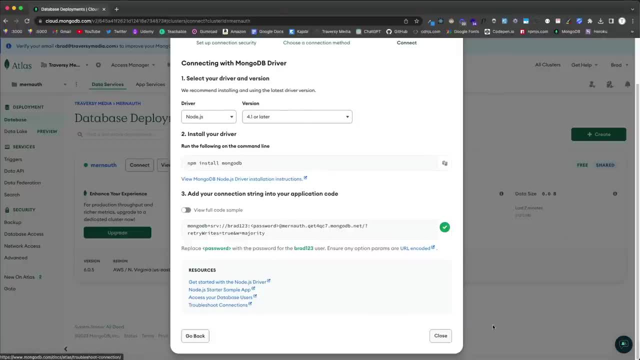 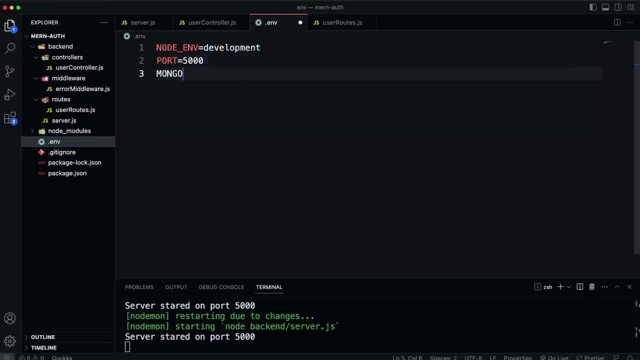 and we're going to grab this connection string right here and then we're going to go into our project and then the dot env, we're going to create a mongo underscore uri environment variable and then paste that in. now we have to change some things here, such as the password. so let's say 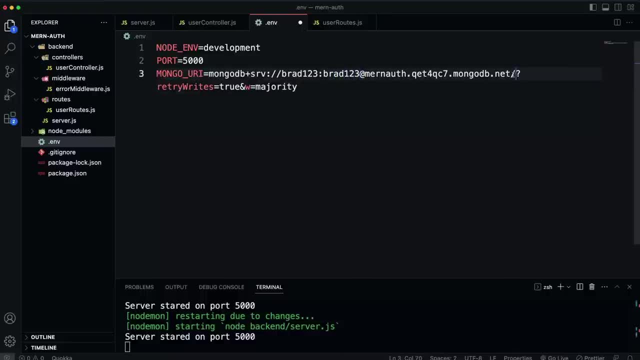 brad123 or whatever. your password is also right here. this: after this slash, you want to put the name of your database, which i called mine, mern off. okay, so we'll save that, and now we should be ready to connect to our database. so in our back end, 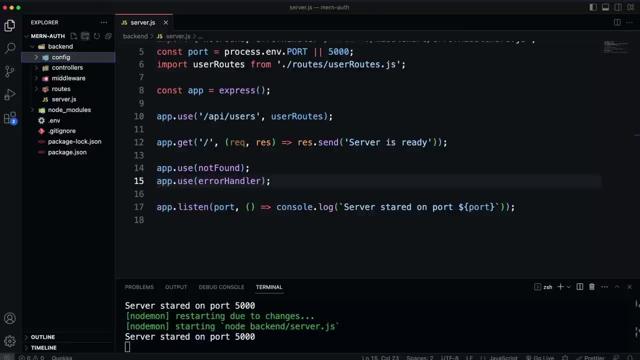 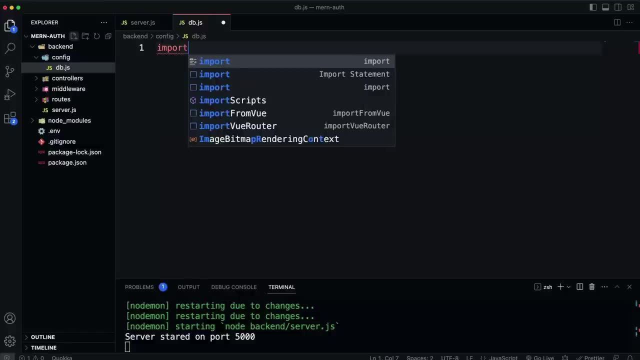 folder. i'm going to create a new folder called config and then in config i'm going to create a file called dbjs and we're going to use mongoose here, so let's import mongoose from mongoose, and we're going to have a function called connect db and this is going to be an asynchronous function. 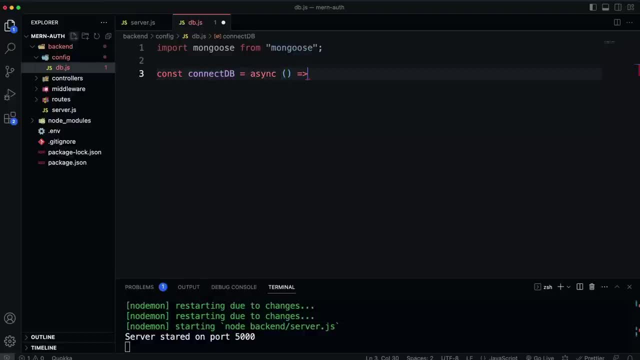 because everything we do with with mongoose is going to be asynchronous and we'll just have a try catch in here and let's create a variable called con. and this is just standard. you know, standard connection function. we're going to await on mongoose dot connect and that's going to take in our mongo uri which is in our env file. so let's say process dot env. 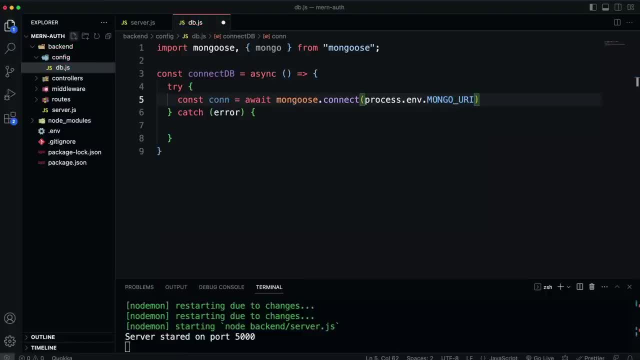 dot and then mongo, underscore, uri, all right, and then underneath that i'm just going to do a console log and let's put some back ticks in here and we'll say: mongo, db connected, and i also want to put the host. so i'm just going to do colon and then we'll put our variable in here which is going: 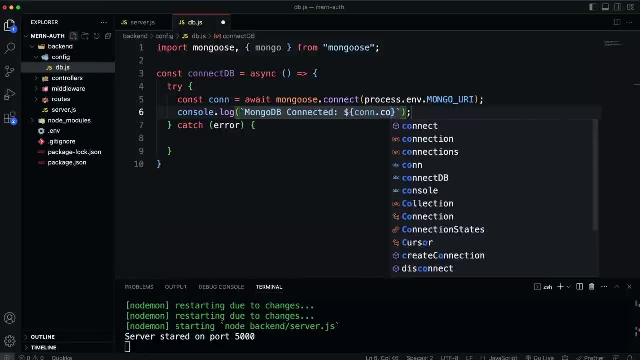 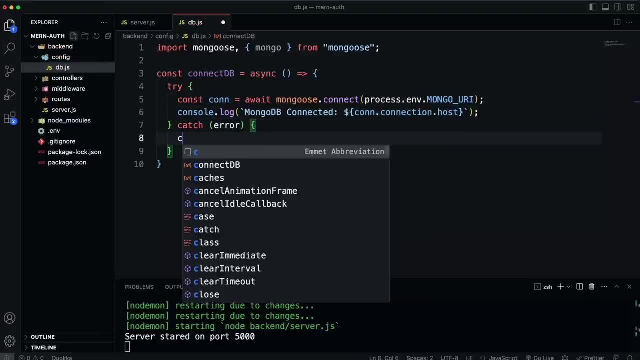 to be that con object and then in that we have connection and then we have host and then if error, what we'll do is just do a. we'll do a console error. actually i don't think i have that. yeah, it's just console dot error and we'll put some back ticks in here, say error. 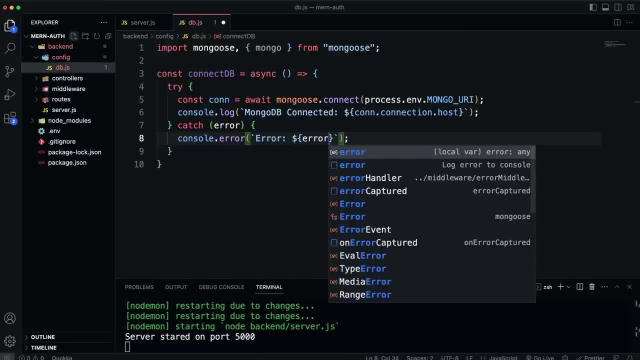 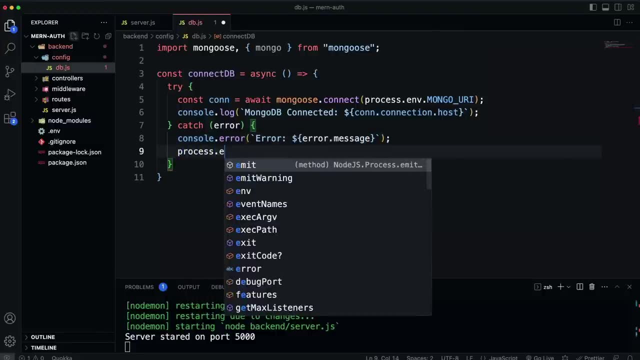 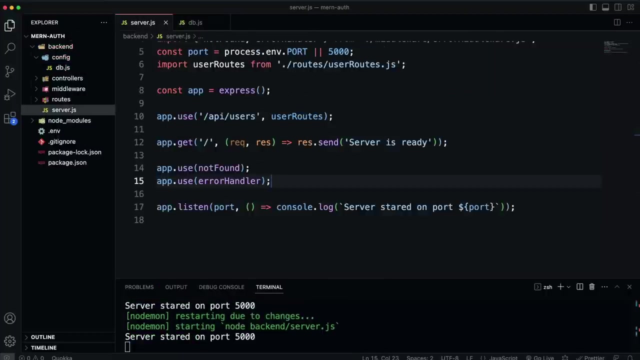 and then whatever message is on that error object, so error dot message, and then we're going to exit with failure. so process dot, exit and pass one in there. all right, and that should do it. so we just export default connect db. so now we want to call that in our server js. so let's go to server js. 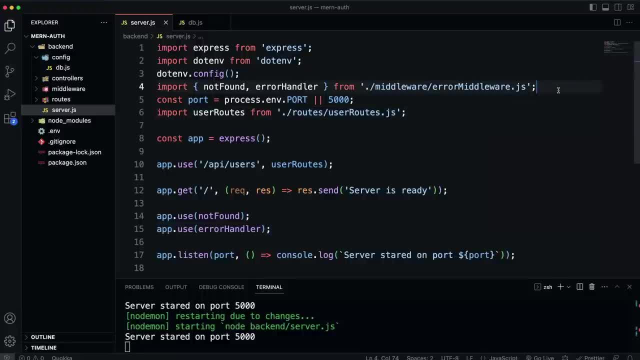 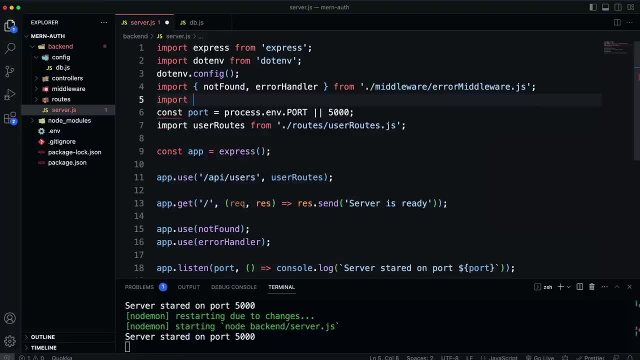 let's bring it in. we'll bring it in. uh, just bring it in right here, i guess. uh and let's. yeah, we're going to import, connect db from config dbjs and then we're going to run this. you can really do this anywhere. i'm just going to do it right above, where we 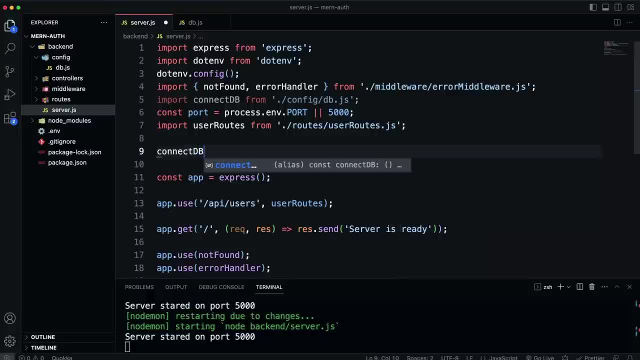 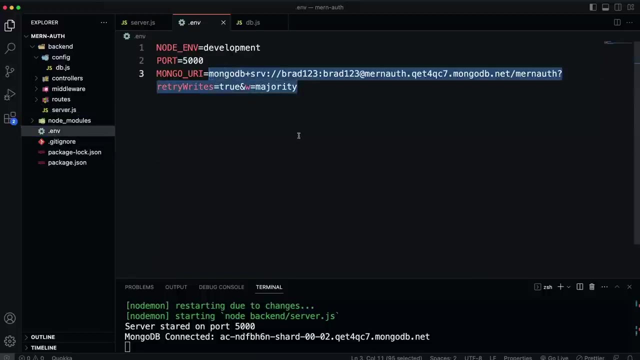 initialize express. so connect db. so when you save now you should see down here in the console mongodb connected and the host. if you don't, it's most likely an issue with your string. so you want to make sure that this is perfect, that it has the correct password, has the correct database and. 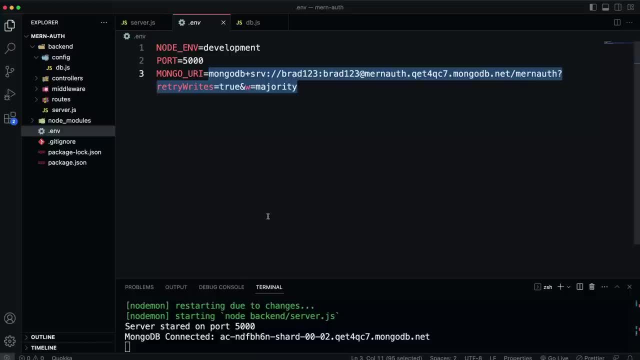 then in mongodb atlas, you want to make sure you have your user set up, you want to make sure that your ip address has been added, and you want to make sure that your ip address has been added. um, you can also set it so that any ip address can connect. so next thing we're going to do is create. 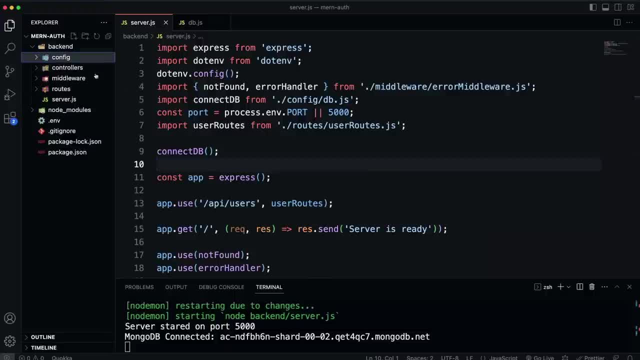 our data model for our users. so, with mongoose and mongodb, instead of setting this stuff up at the database level, like you would with, let's say, mysql or postgres, you do it within your application and in our back end we're going to have a folder called models, and this wouldn't just be for users. 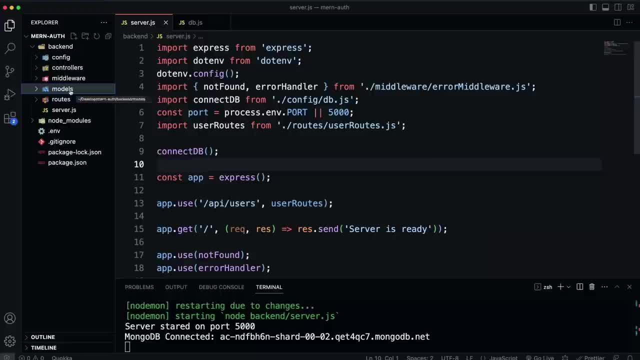 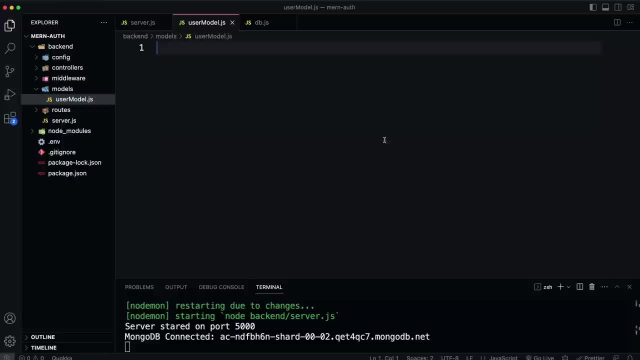 we're going to have a folder called models, and this wouldn't just be for users. we're going to have a folder called models, and this wouldn't just be for users. we have a model for products, we have a model for orders and so on, so let's call this user modeljs, and a model consists of a schema which is going to basically 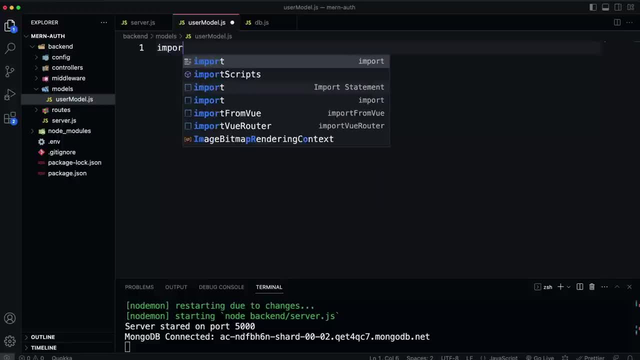 just the fields that that piece of data will have, so like name, email password. so let's import mongoose and then let's create our schema. so we'll say const user schema and we're going to set that equal to mongoose dot uppercase s schema and then inside that we pass. 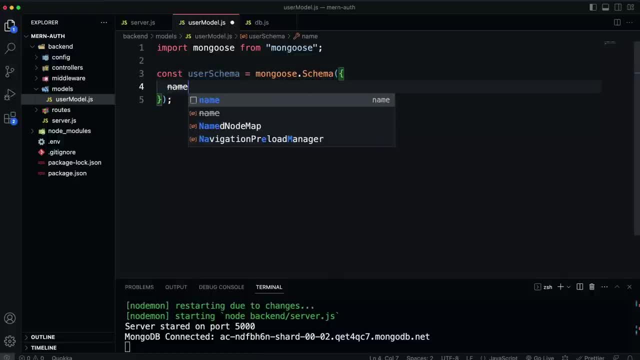 in an object with our fields. so we're going to have a name. uh, did i do that right schema? yeah, so we're going to have a name. now you can just do like this name string. but if you want to have other things, like if it's required or not, then you can make this an object. 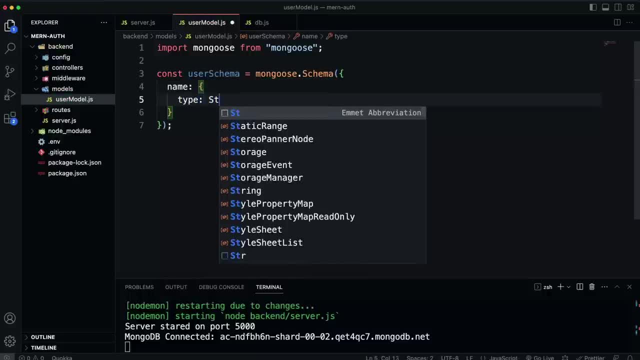 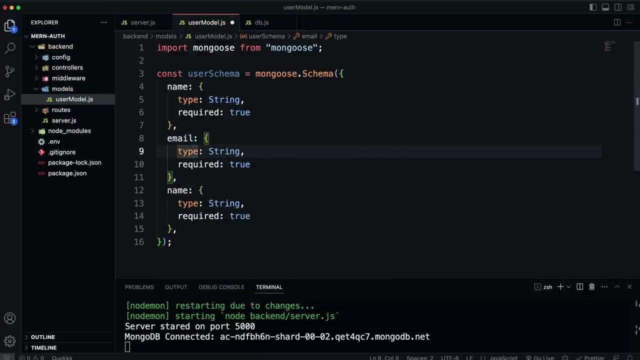 object, then we'll say type and the type will be a string, and then i also want it to be required. so we'll say required, required is going to be true. and then let's, we'll just copy this down two more times. so we have name, we have email, type is going to be string. required, true, and 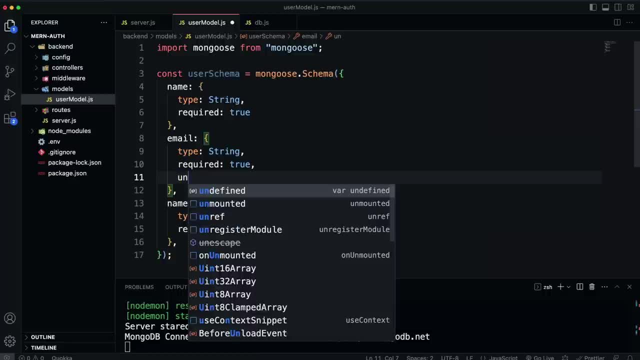 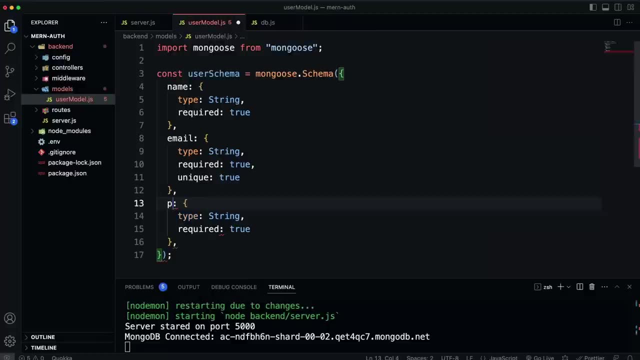 i also want this to be unique. no one should have the same email address. so we'll say unique and set that to true, and then for the password: obviously it'll be a hash password, but it's still going to be a string and we want that to be true. 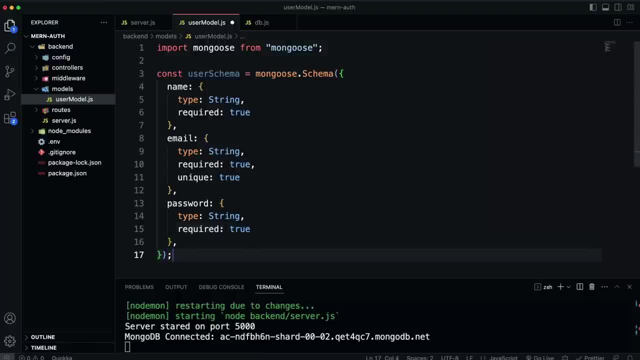 now i also want timestamps, meaning if a user is added, i want the date- the create date- and if it's updated, i want the updated at field. so instead of manually adding them, we can go past this last curly brace here and put it in and add them to our♡. 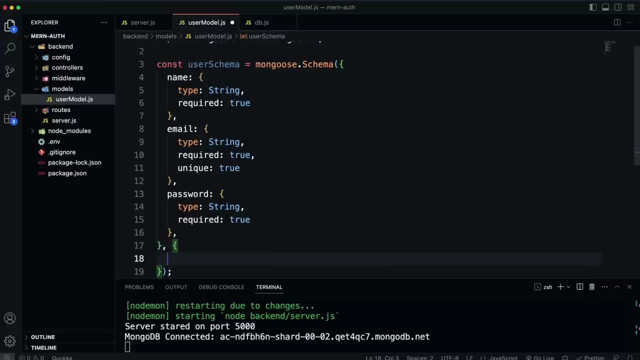 and put a comma and then open up another set of curly braces and we can say timestamp and set that to true timestamps plural, and that should do it. now we're just going to create a variable here called user and set that to mongoose dot model, which takes in a model name which we'll 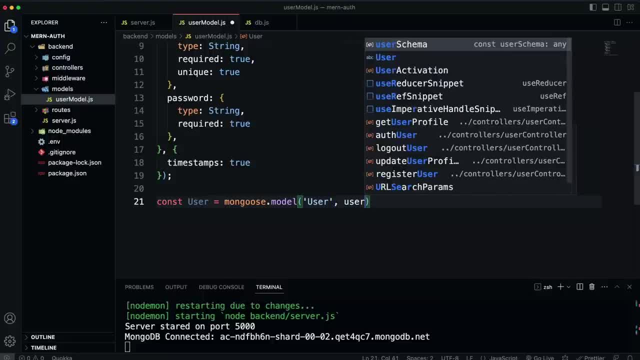 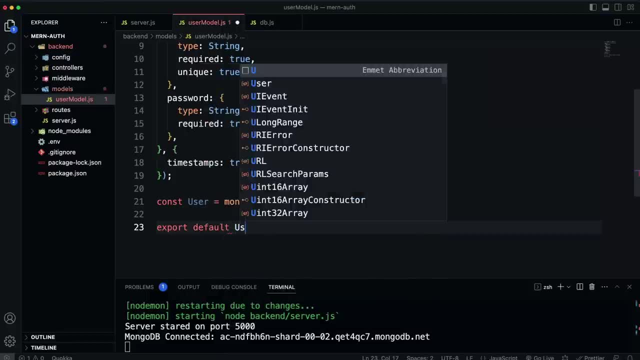 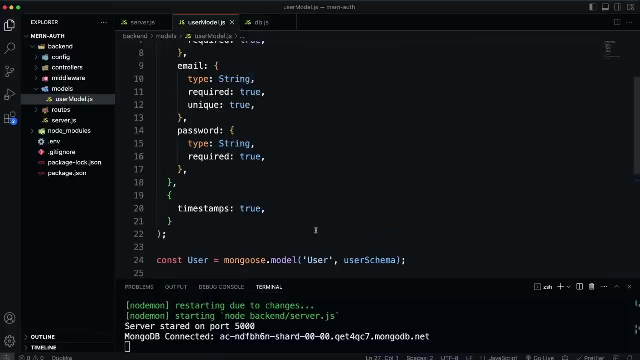 call user with an uppercase u and then it takes in our schema, which is our user schema, and then we simply want to export as default that user model, so then we can bring it into our controller. and then we can call mongoose model methods like find and save and all that stuff. all right, so we 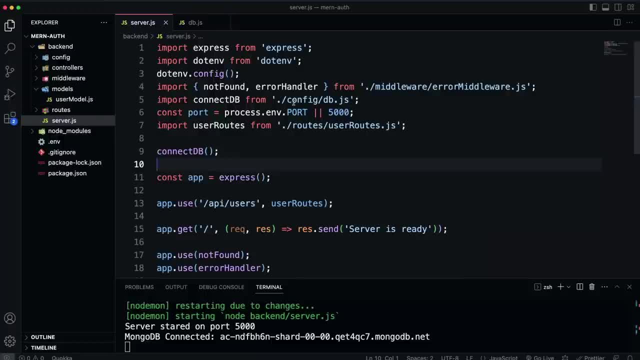 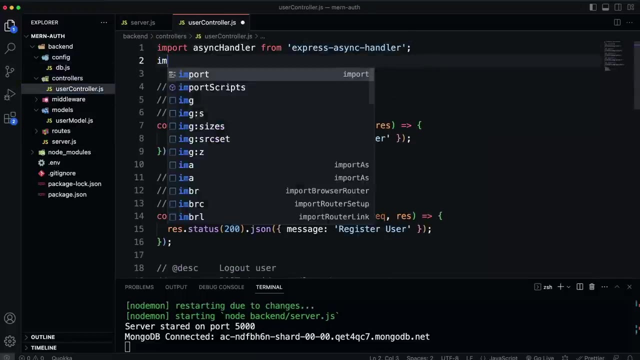 shouldn't? well, we should. we'll go back into our model later when it comes to um, uh, like hashing, passwords and stuff like that. but we're good for now and we can close this dbjs and we're going to go into our user controller and then we're going to bring our user model in. so let's say, import user, uppercase u and. 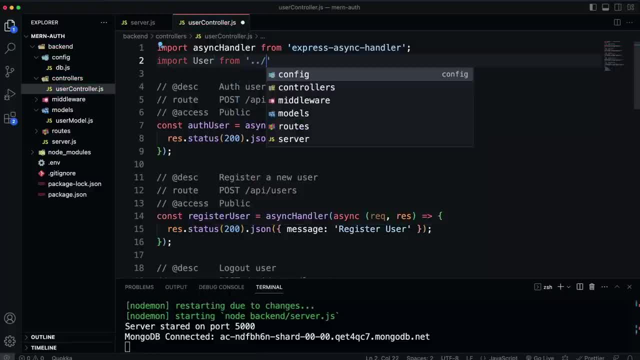 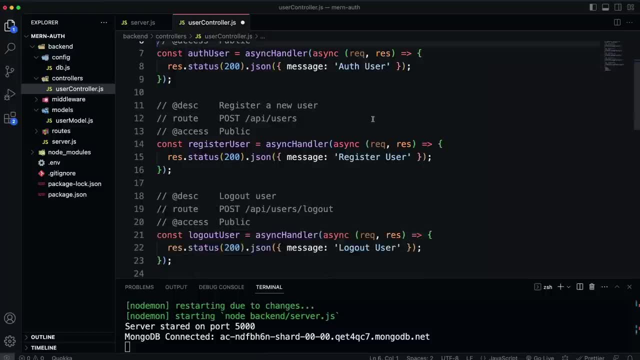 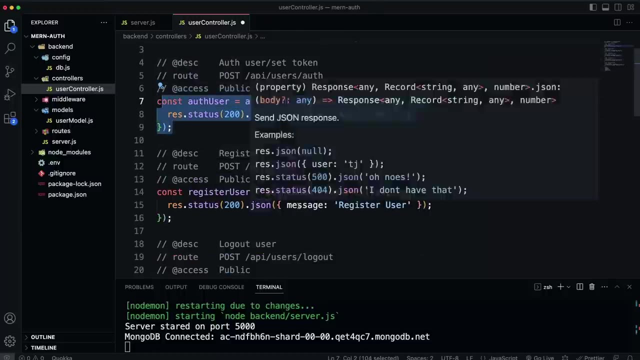 that's going to be from our model, which is going to be up one level into models, and then user model dot js. now i think the first thing we should do here is the register route, because right now we don't have a user to try to authenticate. so when we register, it's also going to authenticate. it's. 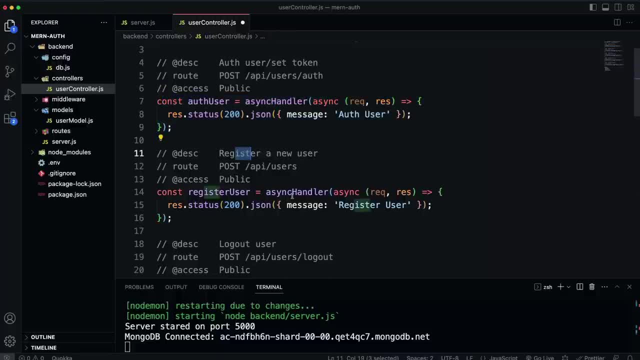 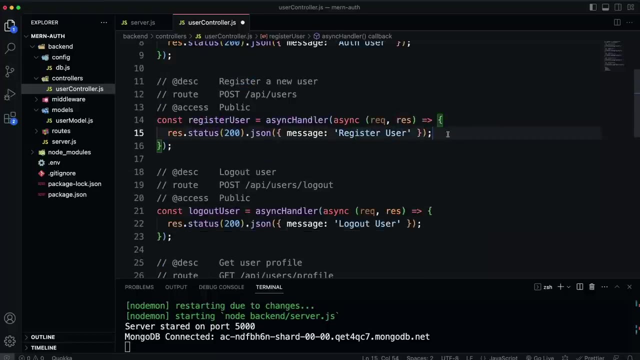 going to be very similar to auth user, except with register we're creating a new user instead of, you know, authenticating one, but ultimately we're going to end up with the json web token in the http only cookie. so let's go into register user and we want to be able to get the body. so right now i'm just going to leave this. 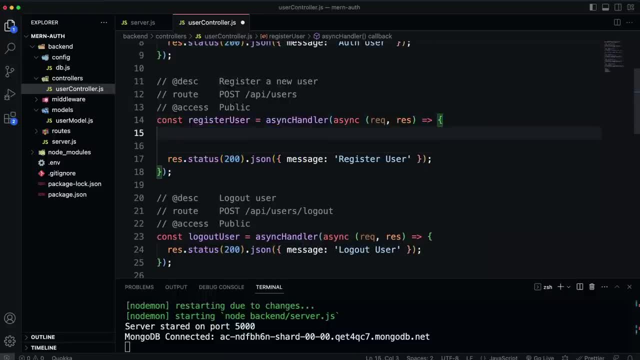 response. but we want to be able to get- let's just do a console log of request dot body, because that is the data that's sent in the http body and we're going to be able to get the body and we're going to get the body. so the the name, email password, that stuff will be here. uh, however, right now, if i try, 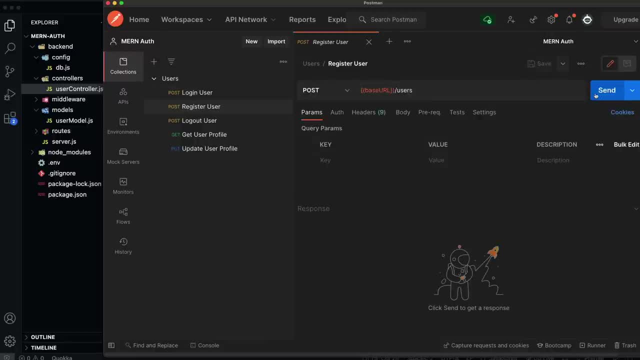 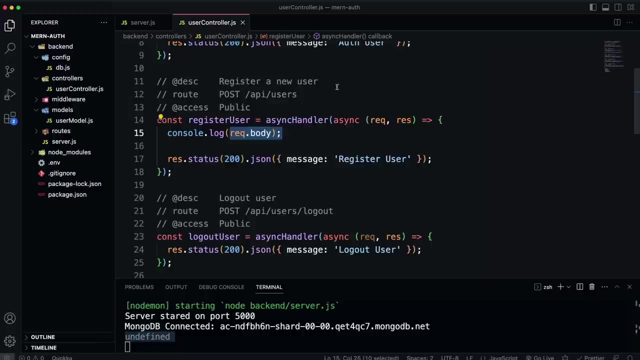 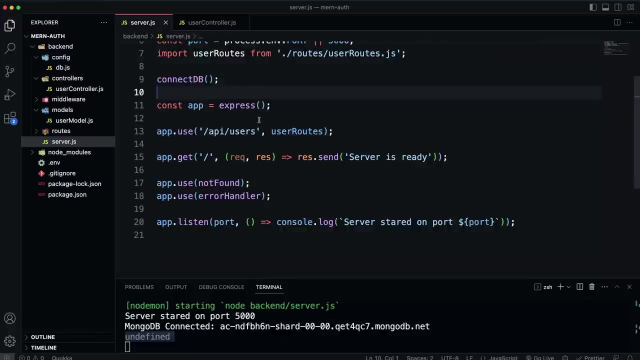 to console log that and i go to my register route and i send and we look down in the console you'll see it's undefined. that's because to use this we need to add the middleware, the body parser middleware. so let's go into our server js and we're going to add that right here. let's say app. 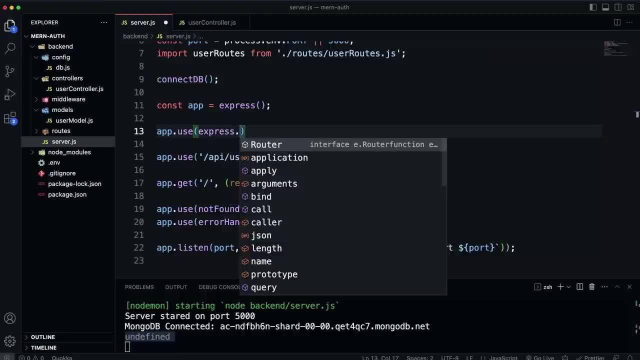 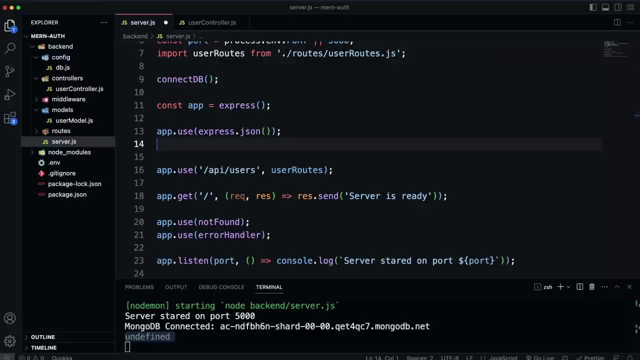 dot use and we're going to do that, and we're going to do that, and we're going to do that, and we're going to do express dot json. so that will allow us to parse just raw json. and then i also want to add app dot use and then express dot url encoded and that's just going to take in an object with 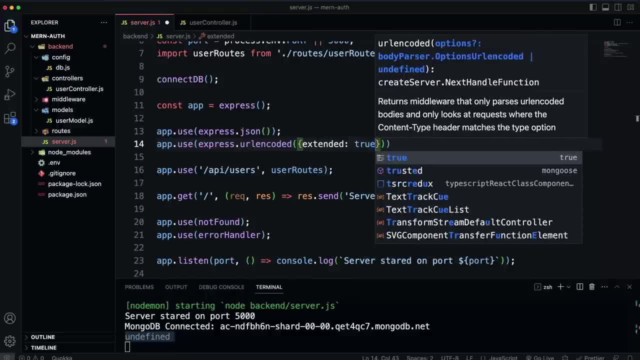 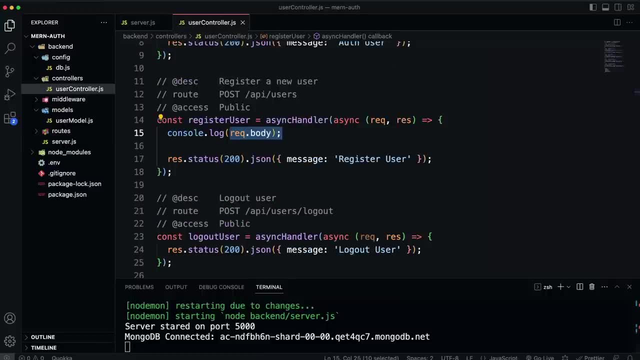 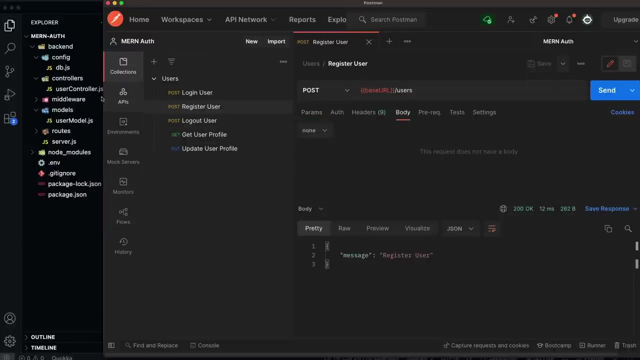 extended and set that to true, so that will allow us to send form data as well. all right now, if we go back to postman and send that again and then we come down here and look, you'll see, we just get an empty object. now to send body data, we can go right here into body. and let me just make this a. 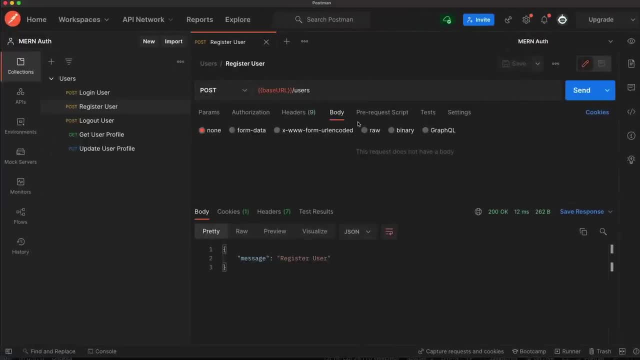 little bigger so that we can see. yeah, so we can see those, and we can choose to send raw json or this form url encoded, which is what i'm going to do. so for the key, i'm going to send name and we'll say john doe, and if i send, and then i'm going to go back to postman and i'm going to go back to postman. 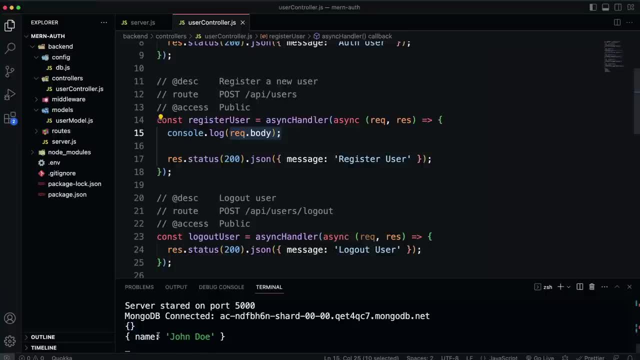 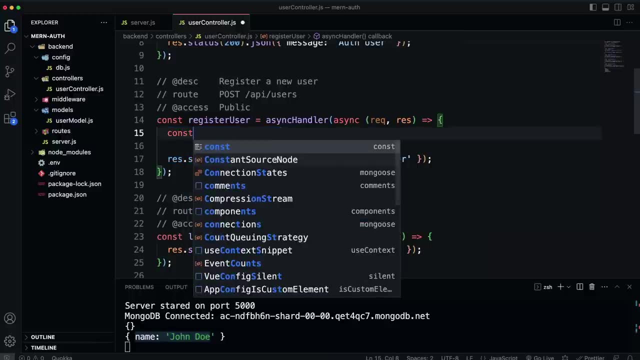 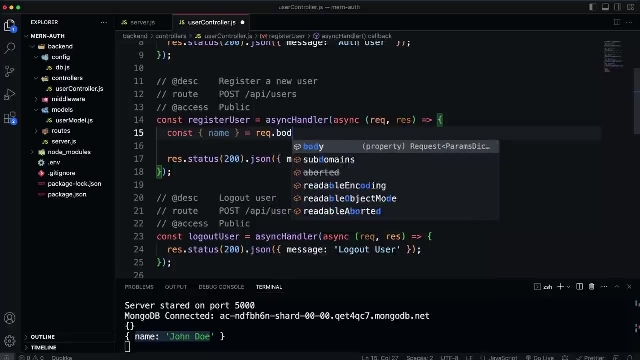 and then i look at my console, you'll see i have an object with the name of john doe. now if i want to get that value, i could destructure it so i could say: const, open up some curly braces, say name and then set that to request dot body and that will pull that out. so now if i were to send again, 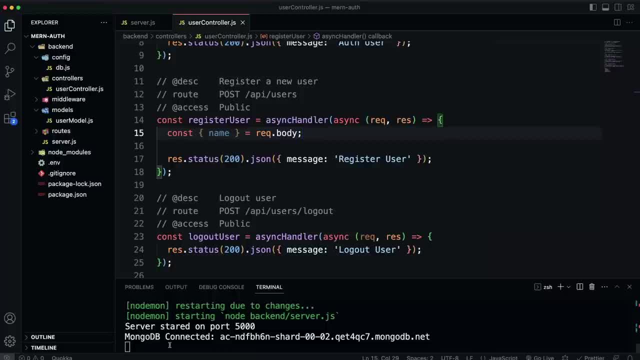 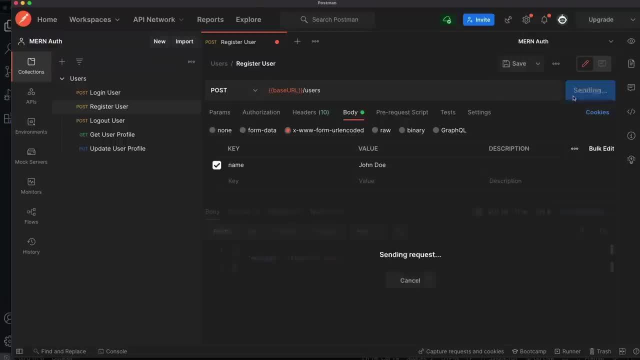 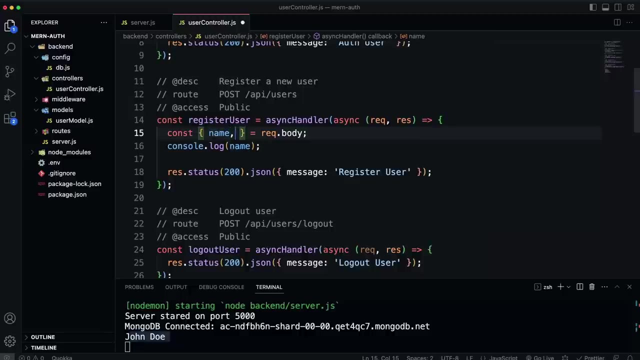 and look at the console, uh well, we should probably console log it. that would help. so console log name and then send it again, check it out and we get john doe. all right, now we want to be able to take in the name. we also want email and we want password. all right, because we're. 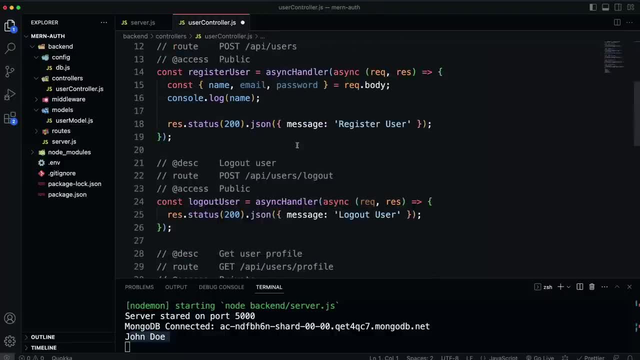 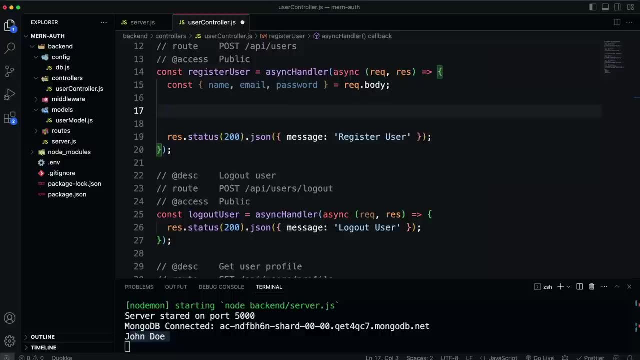 registering a new user. whoops, and that's what we want to get. so let's get rid of that console log. and then the first thing i want to do after we get that data from the body is see if the user exists. so we'll say: const user exists. 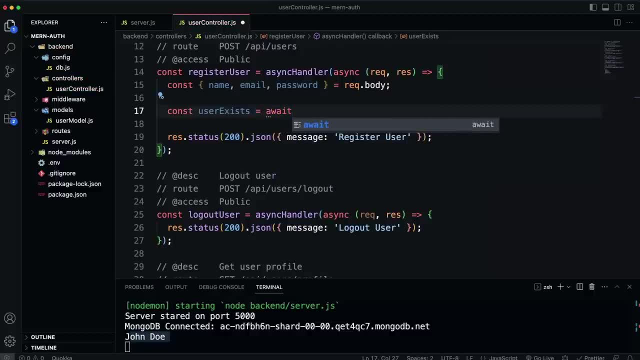 and, And we're going to set that to await because, remember all these model methods- they return a promise. So we're using a sync await, And then user, and there's a method called find one, And basically what that'll do is just 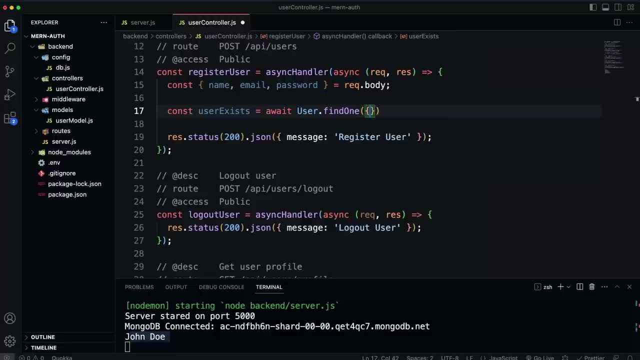 find a single user by whatever I put in here And I want to get it by email, And this is the same as doing this. So I'm basically just saying, if the email matches this email, that's being sent. But we can cut that down to just email. 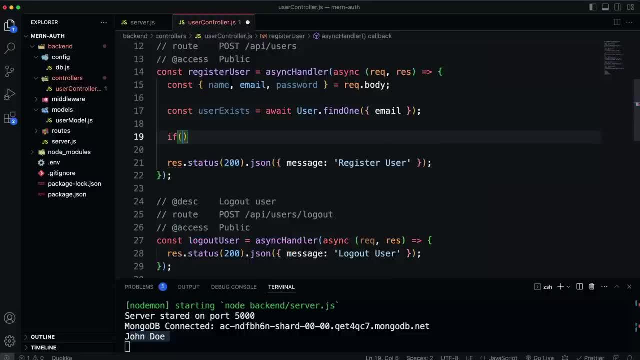 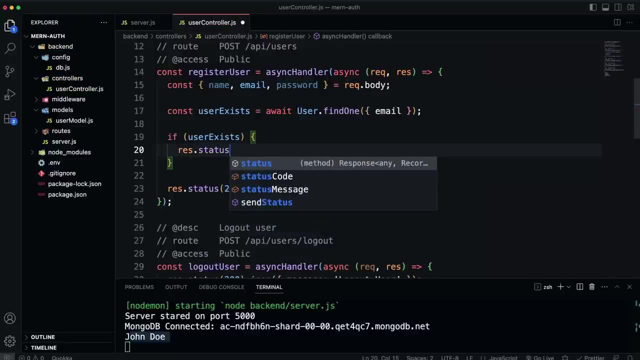 So if that user exists, let's say if the user exists, then I want to throw an error. So remember, we can set the status- Status is going to be 400, which is a client error, And then we can say: throw new error. 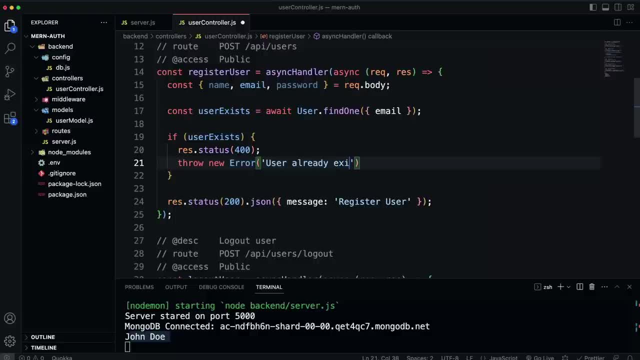 And then just say user already exists And this will use our default error handle that we created a little while ago. So, outside of that if statement, now we want to create the user because obviously they don't exist if they're passing this validation. 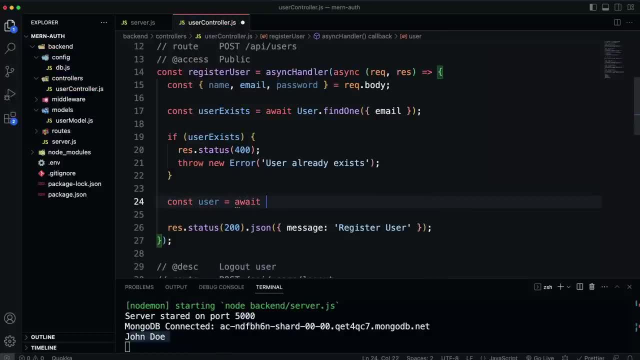 So let's say, const user, set that to await and then usercreate And we're going to pass in here. We want the name, the email and the password. And you're probably saying, well, that password is just plain. 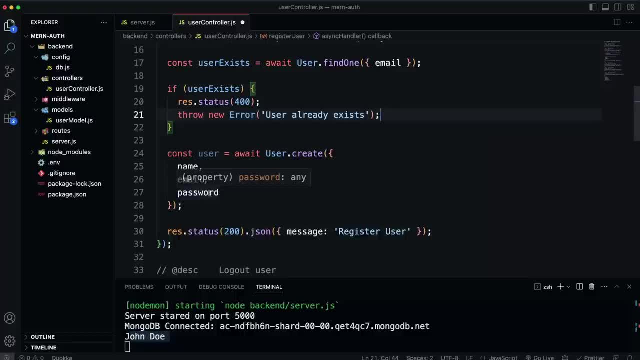 text It is. So, after we do this, we're going to go into the model And we're basically going to add a little hook that says, before we save this password, we want to hash it using bcrypt. We'll do that in a second. 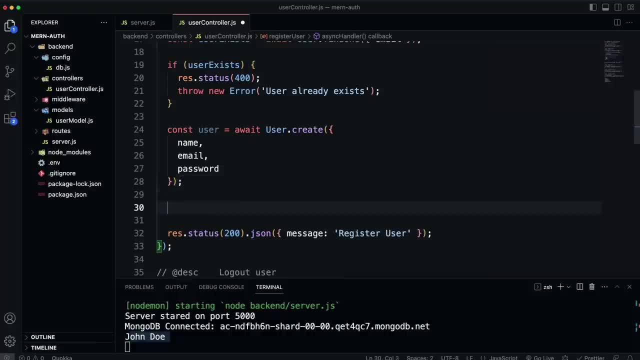 But let's go down here after we create that user And we'll check to make sure the user was created. And then we want to do a resstatus, And let's do a 201, which is successful, but something was created. 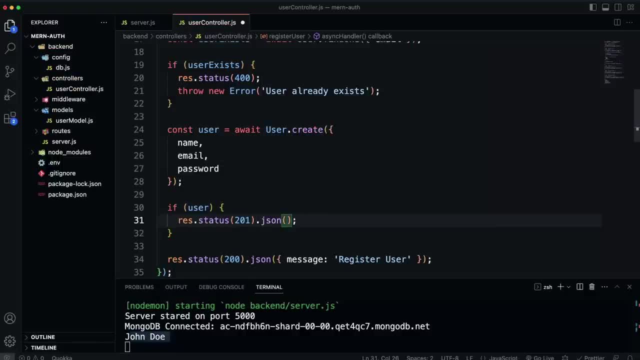 And then json, and in here we'll pass an object that has the user say underscore ID. Set that to the userunderscore ID And the name, so username And the email, which will be the useremail. 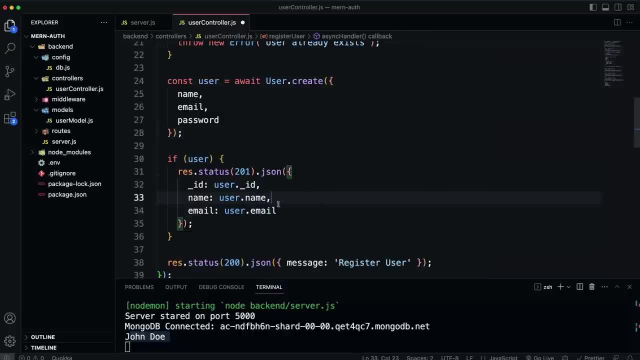 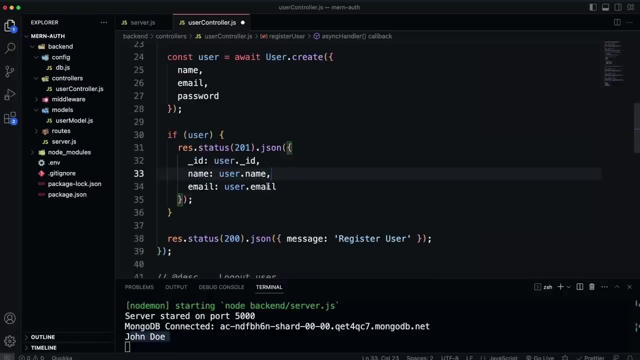 We're not sending the token. I know that in some tutorials you'll see where they send the token, But we're not doing it that way. We're still going to store the token in an HTTP-only cookie, Now if there's no user here. so if something goes wrong, 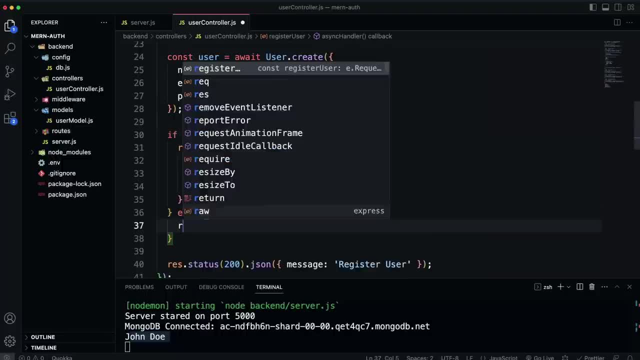 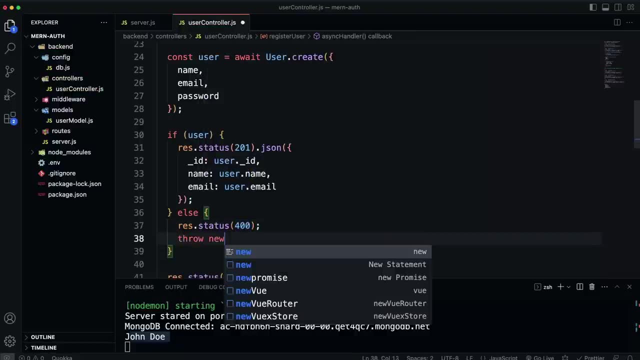 then we're just going to say else And let's set a status, so resstatus of 400.. And then we'll throw a new error And we'll just say invalid user data. And then this very last, this right here: 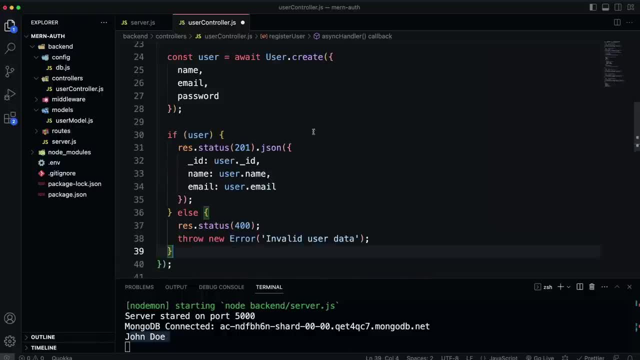 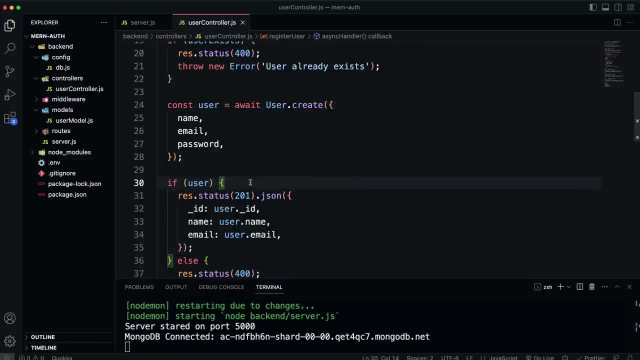 we want to get rid of that. All right, Now I'm going to save this And before we try it out, we want to make sure that we hash the password. Now you could bring bcrypt into the controller and do it here. 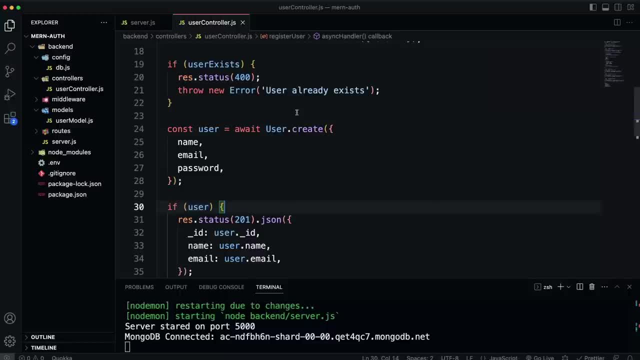 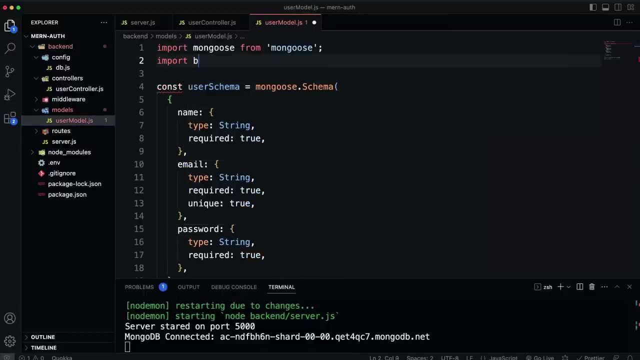 But I think it's neater to keep it in the model and try and keep your controllers really light. So let's go into the user model And first of all we're going to import bcrypt. So let's say import bcrypt from, and then it's. 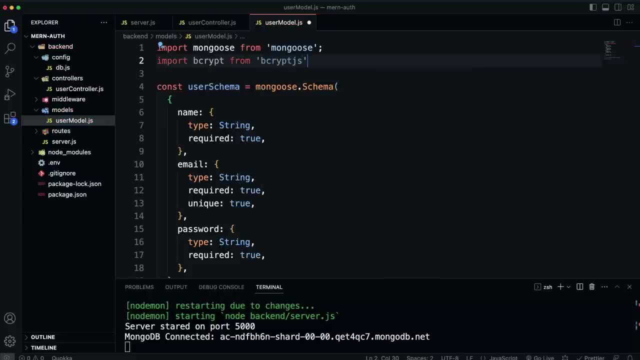 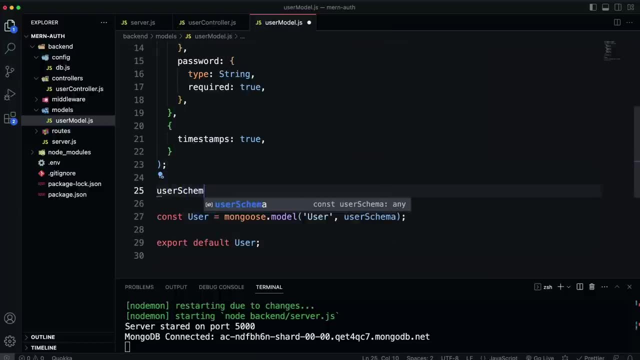 going to be bcryptjs, OK, And then down here under the schema we're going to add a piece of middleware So we can actually add onto user schema. there's hooks for pre and post, So pre means obviously before. 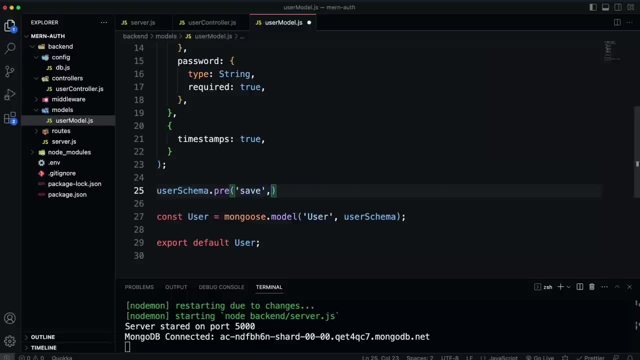 So we want to say: before we save, then we want to run a function. Now, this function, we're not going to use an arrow because of how this keyword works, because we will be using this, So we're going to say asynccd. 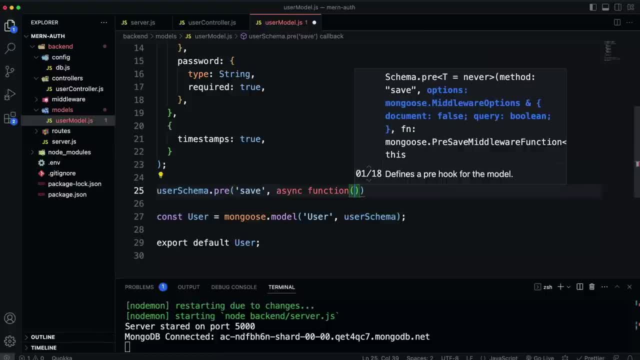 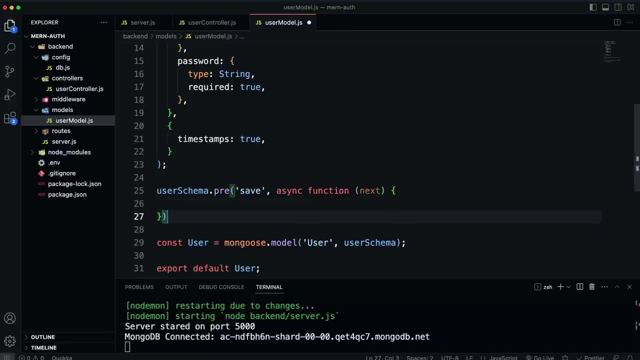 OK, All right. So we're going to say async and then function, And that takes in a param of next, because this is middleware, so you want to be able to move to the next piece of middleware. Now, inside here, what I'm going to do is have an if statement. 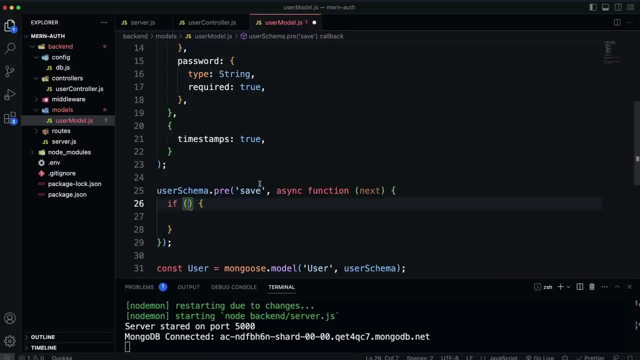 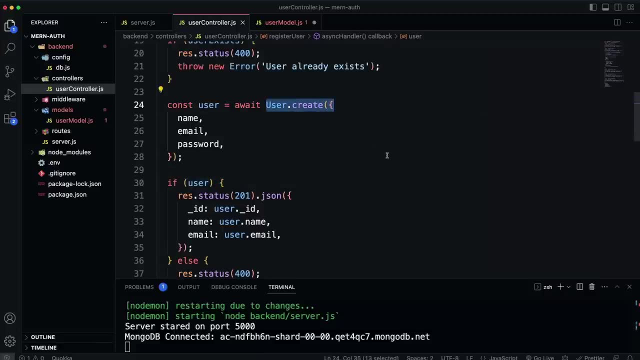 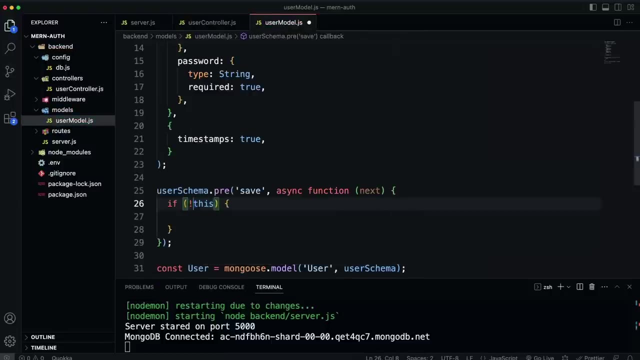 And, like I said, we're going to use the this keyword, And this just pertains to the user we're saving right. So in our controller, when we say usercreate or usersave, that is what this means. OK, So I'm going to say actually, if not this, and on this, 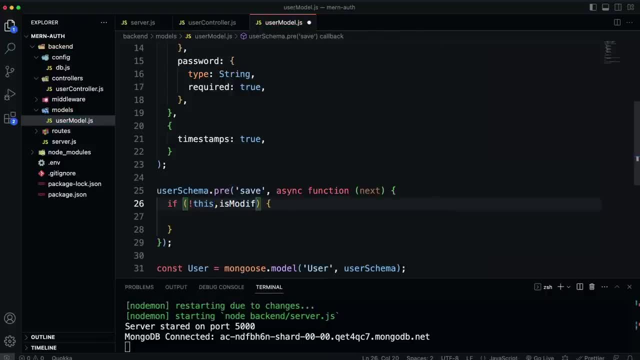 we have certain methods And one of them is is modified. So I'm going to say, if this, that should be a dot, So if this dot is modified, and then we can pass a field in here. we want to check for the password. 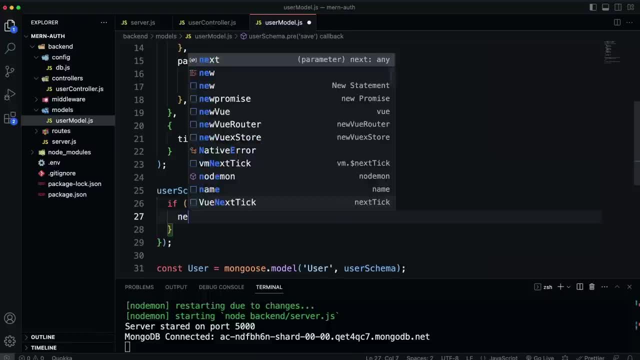 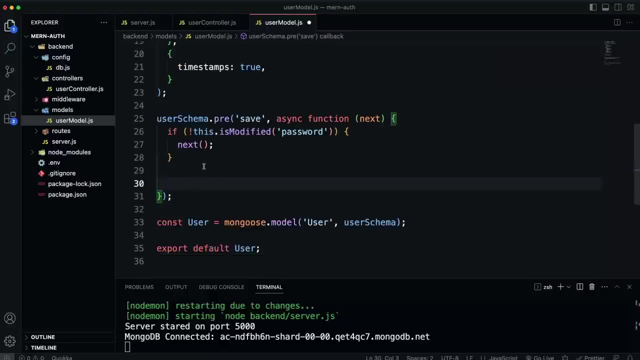 So basically, if the password isn't changed in any way, then we just want to move on. So we're just going to say next: OK, If the password is modified, or if we're just creating it like we are now, then we want to hash it. 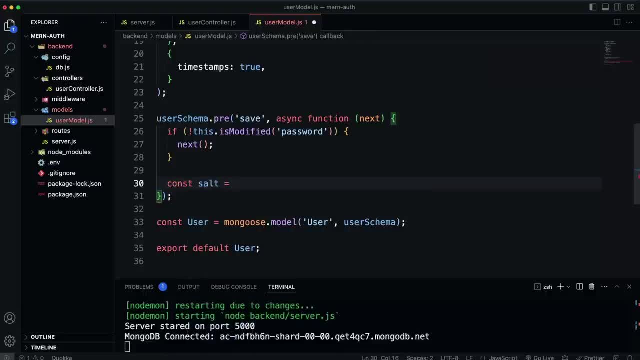 So, first thing, we have to create a salt which is like a key that we use to hash the password, And we can create this with, let's say, await, And then bcrypt has a method called gen salt. so generate salt. 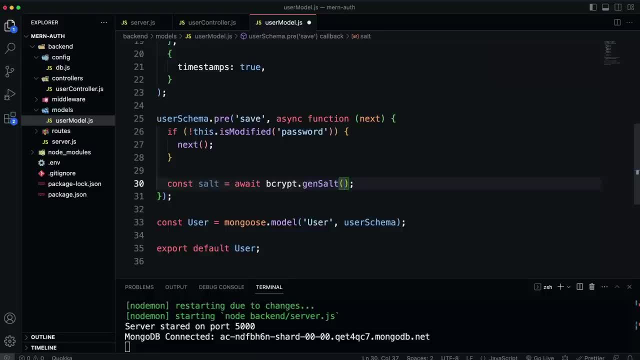 And it takes in the number of rounds, which is basically the number of characters, And I think it can be like 1 to 20, or something like that. So we're going to say 10,, which is right in the middle. 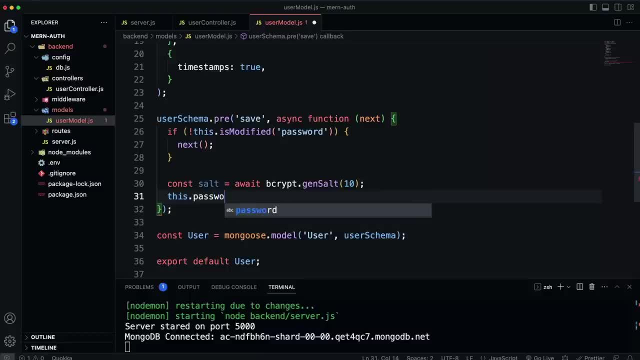 And then we can then say this dot password, because you can access any of the fields. Right now this dot password is just plain text, So that's why we're now changing it to be hashed, And we can do that with bcrypt dot hash. 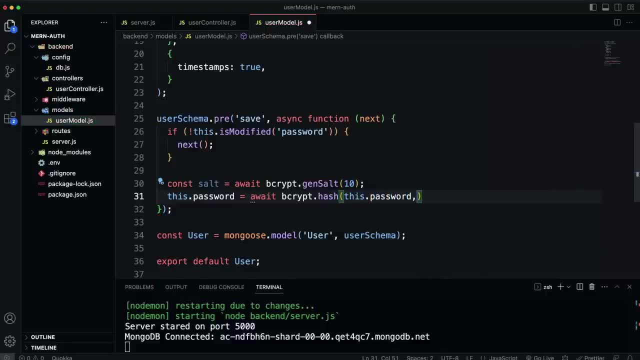 pass in the plain text password, which is this dot password and also the salt, So that will hash the password before it's saved into the database. So we'll go ahead and save the file, And now we should be able to try this out. 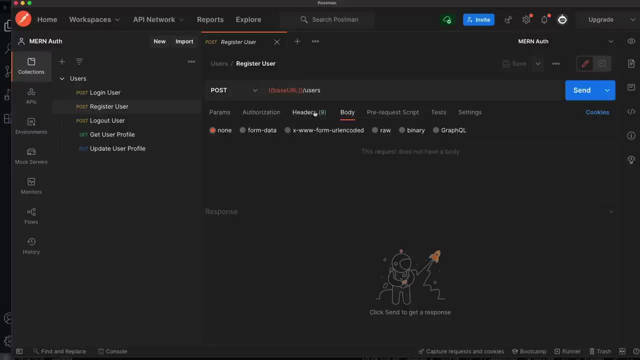 So let's go into Postman, go to our register route And in the body I'm going to have name, which I'll say John Doe, We're going to have email, which I'll do john at email dot com, And then password. 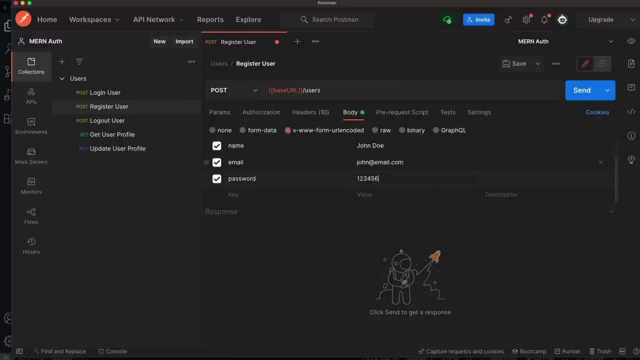 Which I'm just going to do: 1,, 2,, 3,, 4,, 5,, 6.. But it should get hashed because of that middleware in the model. So let's say send And we get back a 201 created. 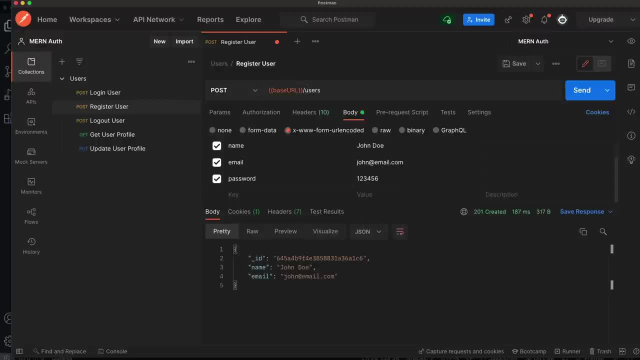 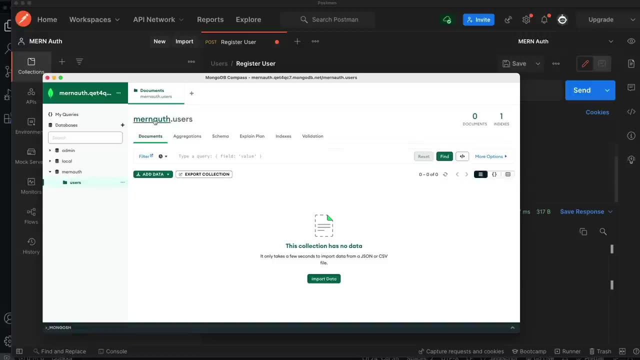 And it gives us the ID, the name and the email Now to check this: if you have Compass installed, you can use that Now you do have to just reload. So you guys can't see my context, my menu. 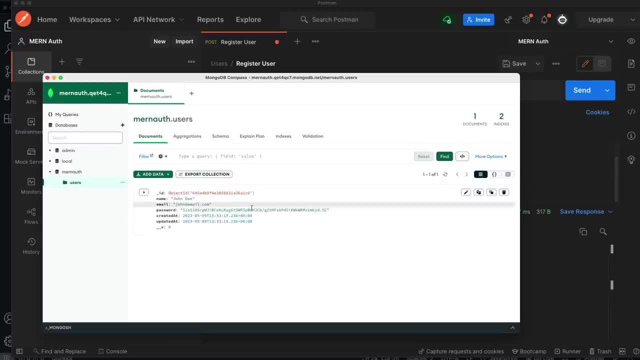 But I'm going to go to View and Reload Data And there it is, There's my user And you can see the password is hashed And we also have created that and updated that because of that timestamps that we put in the model. 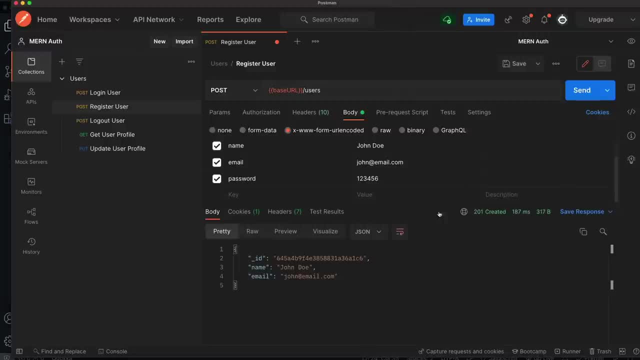 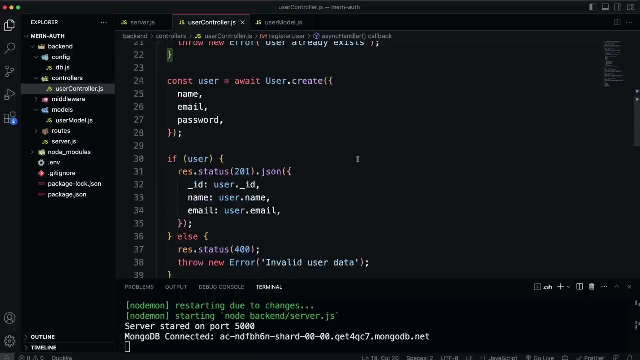 So we're now able to register users. Now, that's only half the battle. We also want to generate a JSON web token and also save that in an HTTP-only cookie. So to do that, let's go to our register user And we could put all the code here to generate the token. 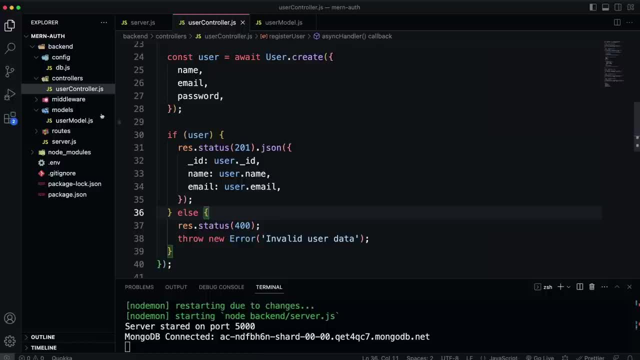 and so on. But we're going to be doing the same thing in the auth route, So I'm going to put it in a separate utility file. So in back end let's create a folder called utils And then in utils we'll create a new file. 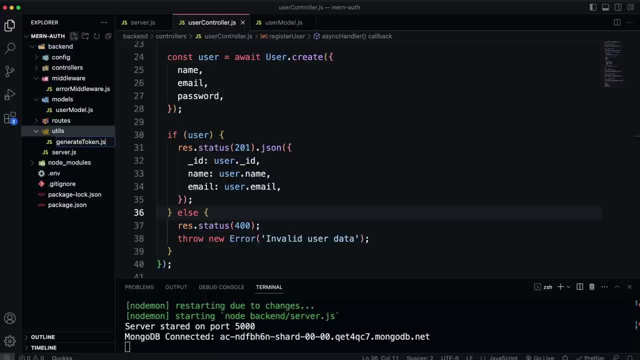 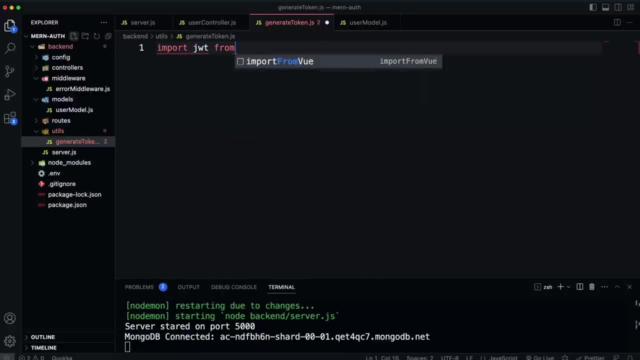 And let's call it generateTokenjs. OK, And in here we want to bring in our JSON web token. So we import JWT from JSON web token And then we're going to create a function here. So, const, we'll call it generateToken. 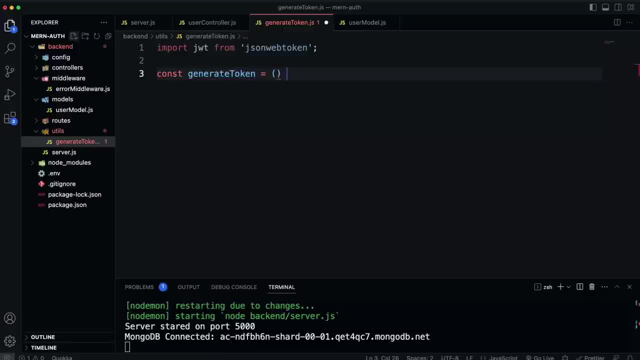 And make it an arrow function, And this is going to take in two things: It's going to take in the response And then it's going to take in the user ID. Now, the way that JSON web tokens work is you can add something into the payload, right? 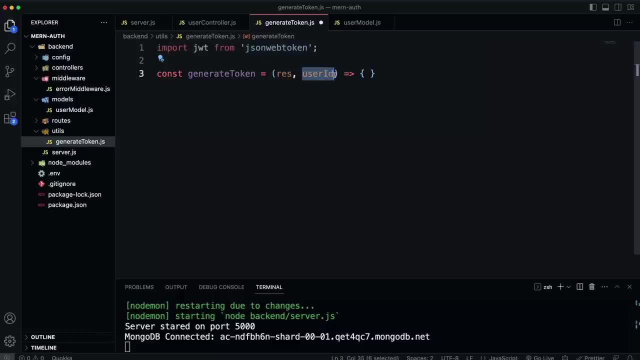 And what we want to add is the user ID. because we need the user ID, Because we need that when we validate the token right, We need to be able to pull that user ID out so that we can do whatever If we're getting the user as profile or whatever it is. 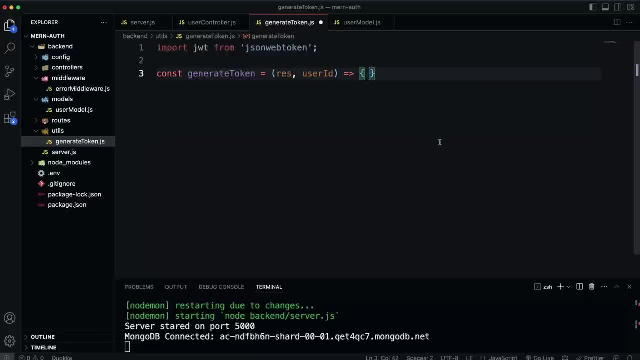 we need that user ID. So we're going to add that as a payload. So let's go ahead and create, let's say, token, And the way we create a token is use our JWT package And there's a method called sign. 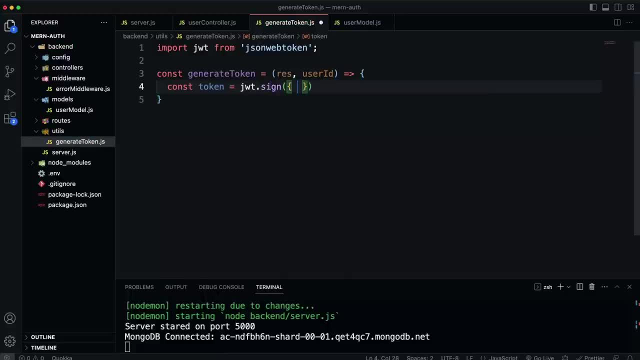 And then sign is going to take in an object with the payload, which, for us, is going to be the user ID that's passed in, all right. Then the second thing we want to pass in here is the secret which we're actually 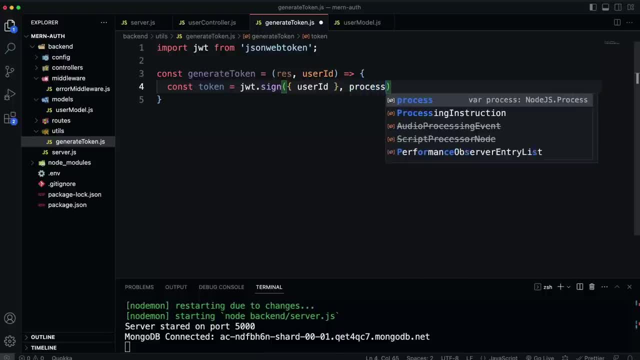 going to put into our env file. So let's say processenv and then JWT underscore secret, And we'll add that in a second And then the next thing. so another comma. the next thing is an object where you can have some options. 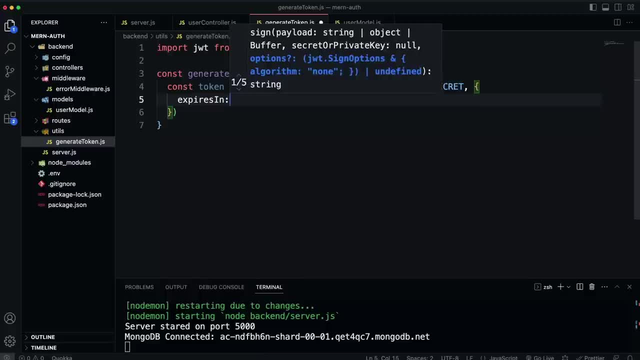 And the option I want is expires in, So you can decide when you want this token to expire. I'm just going to say 30D, 30 days to keep it simple, But of course you could make it a lot sooner than that. 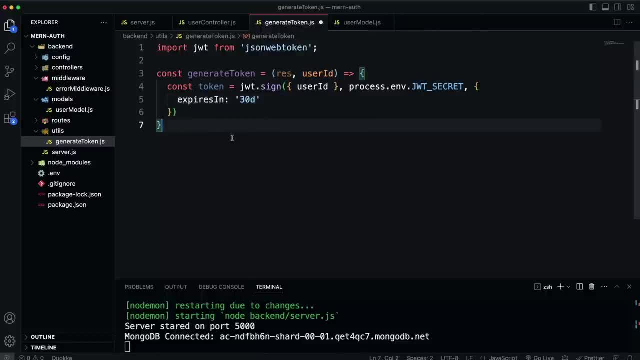 You can make it a day or an hour, whatever you want. All right, now let's add this secret. So I'm going to go to my env And let's say JWT underscore secret And I'm just going to set it to ABC123.. 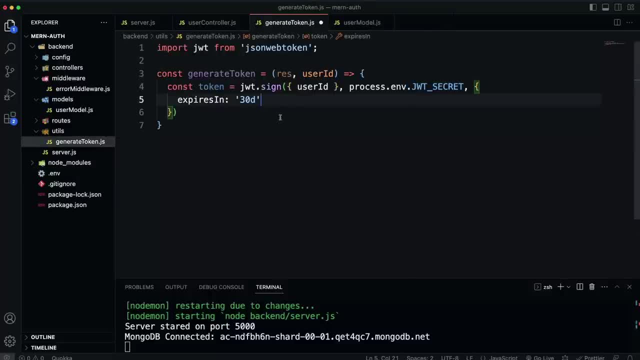 But of course you can set it to whatever you'd like. All right, so that will create the token. Now we need to save it in a cookie. So to do that, let's go under where we created the token And we're going to say rescookie. 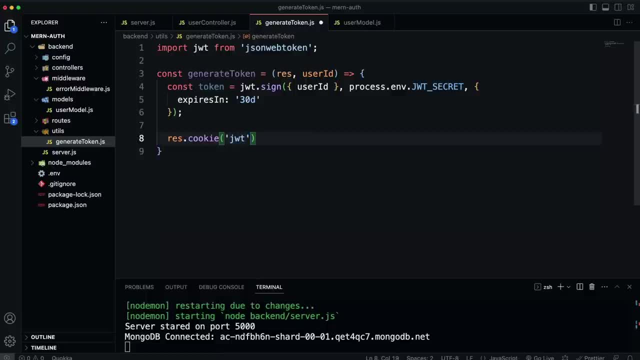 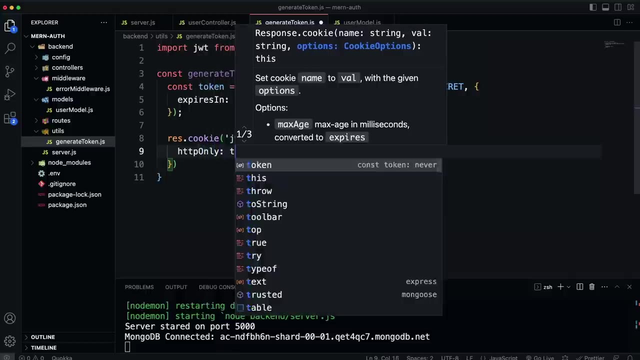 And we're going to call it JWT. And then we want to pass in the token- That's the data that goes in the cookie, And then we also have some options. So we want to pass in some curly braces. We're going to set HTTP only to true. 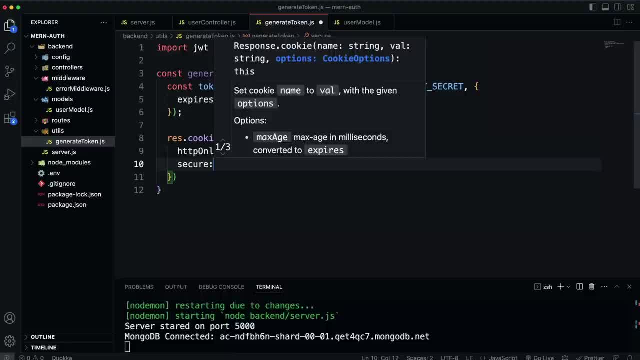 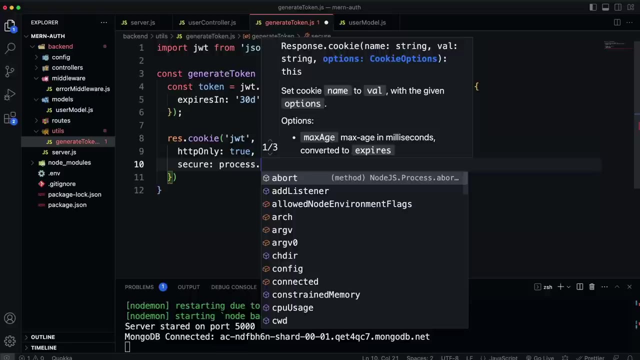 And we're going to set secure. So basically, with secure, the site has to be HTTPS. Now we only want this in production Because obviously when we're in development, we're not using HTTPS on our local host. So what we can do is we can say processenv. 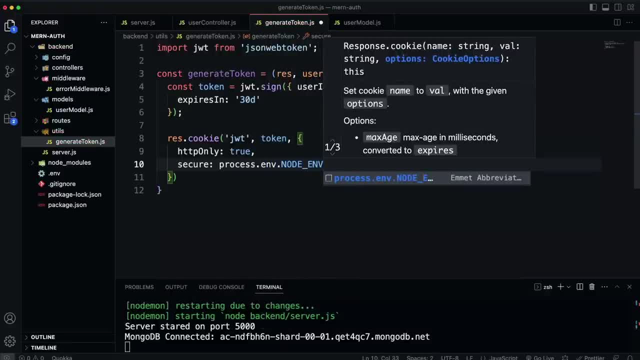 And we're going to check our node, underscore ENV and say if that is not equal to development, OK, so if we're in development, then this will be false. If we're not in development and we're in production, then secure will be true. 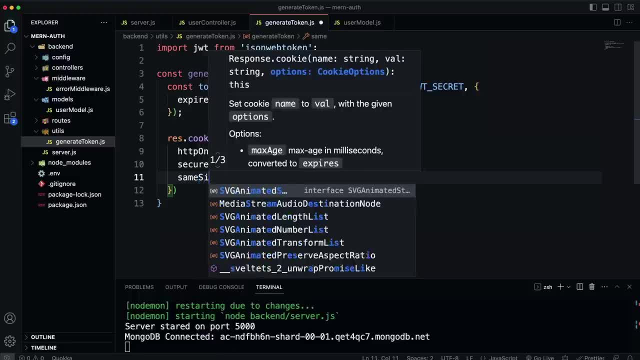 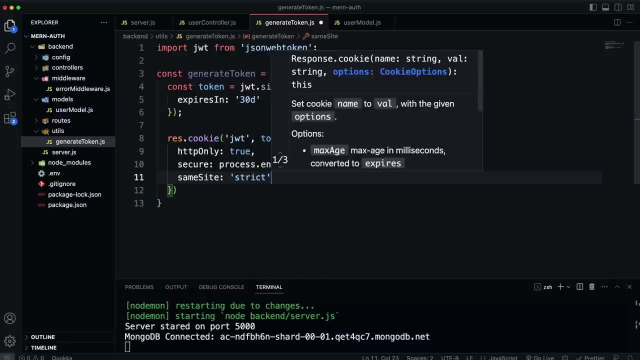 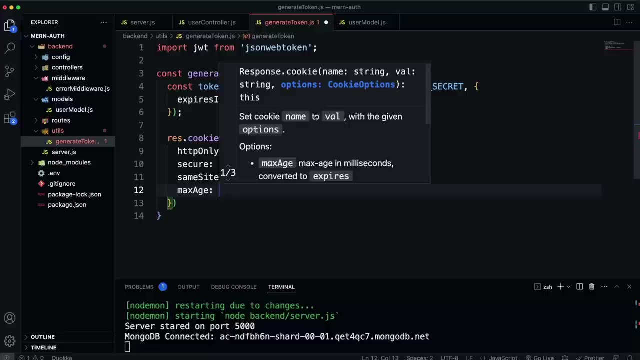 And then we're also going to add same site. So, basically, this will prevent CSRF attacks. We're going to set this to strict And then we want to put a max age. So, basically, when does this expire? I'm going to set it to the same thing as the token, which. 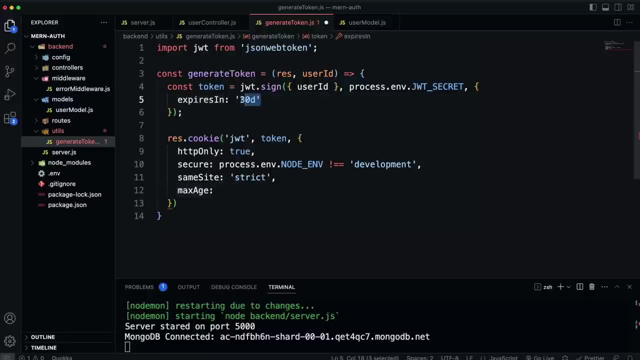 is going to be 30 days. Now this takes in seconds. You can't use something easy like this: 30D. So we're going to do 30 times 24 hours in a day, and then times 60 minutes in an hour, times 60 seconds. 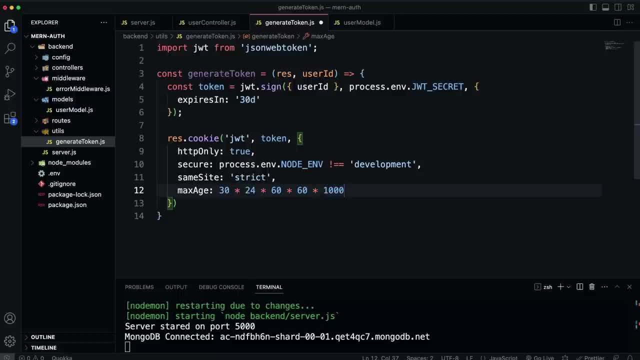 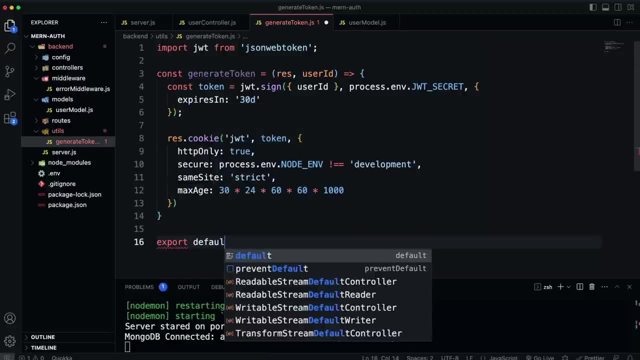 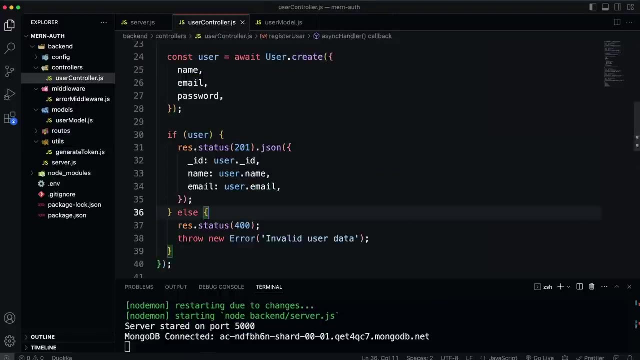 and then times 1,000.. I think that's right. Yeah, so that should be 30 days, And then we're going to export this as default generate token. OK, so now we should be able to use this in our controller. 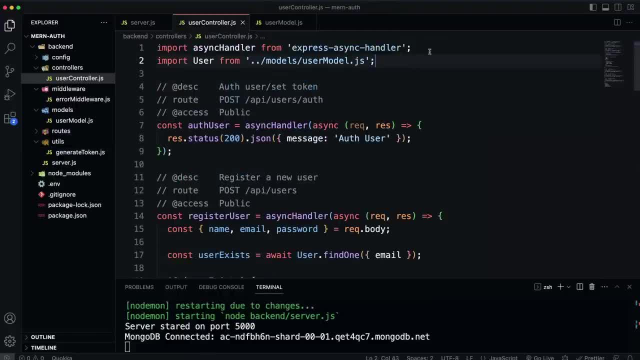 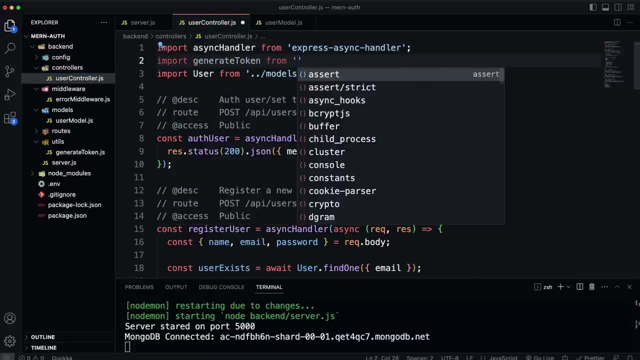 So I'm going to close that up And then we're going to import it at the top here. So let's say, import, generate token And that's going to be from, And we want to go outside of controllers into utils and generate token. 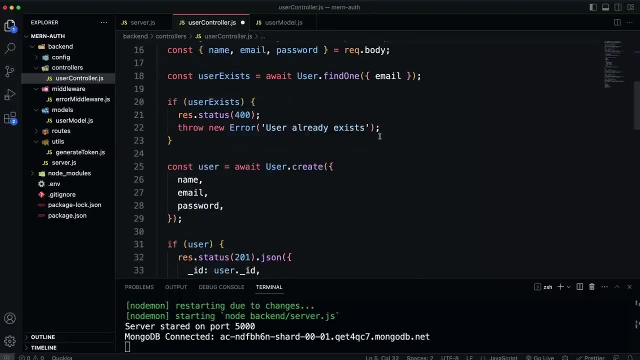 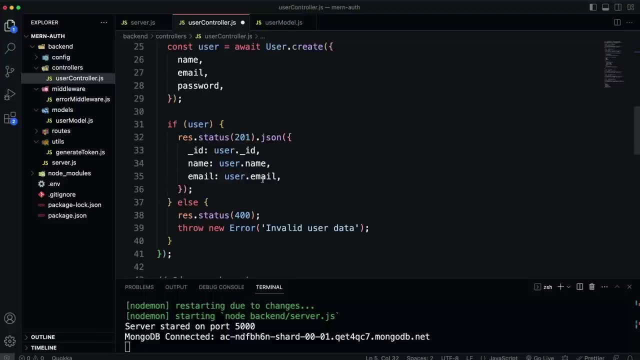 Make sure you add the dot js. So now we just need to go down And add this And let's see We're going to put it right. before we put our response right here, We're going to call generate token. Now, remember it takes in the response, so res. 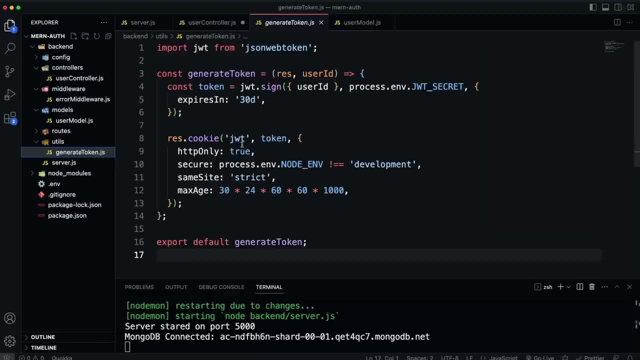 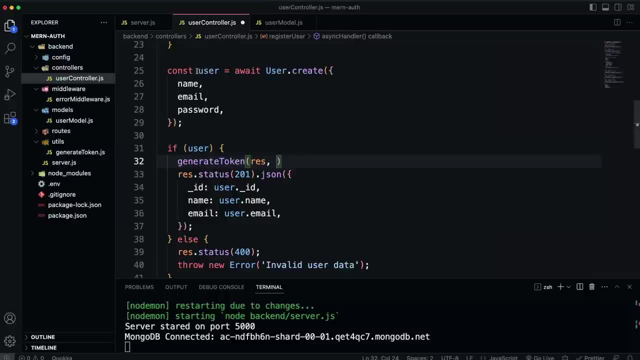 And the reason we do that is because we set the cookie with rescookie right. And then the second thing is the user ID, which we are getting the user Here right, So it creates the user And then it puts the result in user. 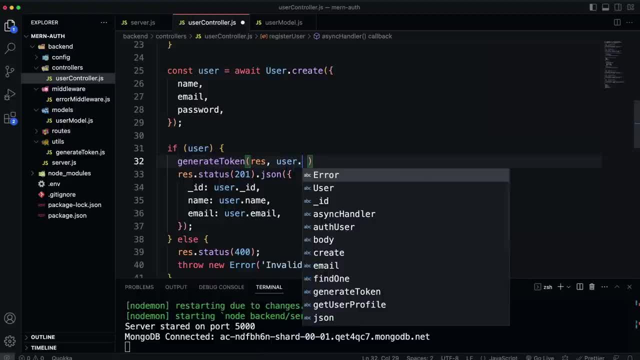 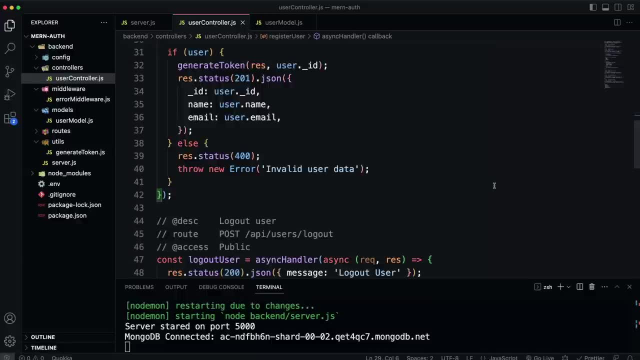 So we should be able to just pass in user dot underscore ID And that should do it. So we'll save that. Now let's check it out. So I'm going to go to Postman And I'm just going to. actually, you know what? 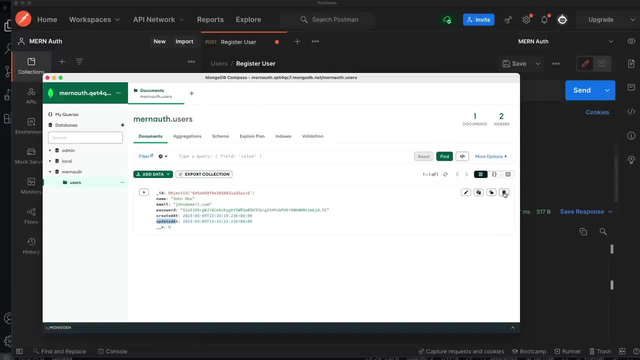 I'm going to go through Compass and delete the user I just created, just so I don't add up a bunch. OK. OK, I've added up a bunch of users here, And then I'm going to go ahead and send this again. 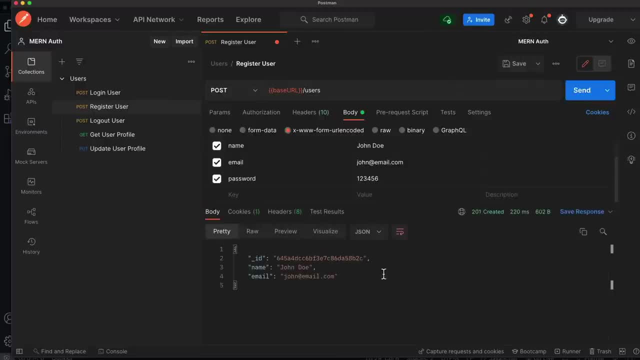 and register John Doe, And now notice that where we have these cookies, we have one in parentheses And if I click on that it shows we have this JWT cookie, which is set to true for HTTP only False is set to secure. 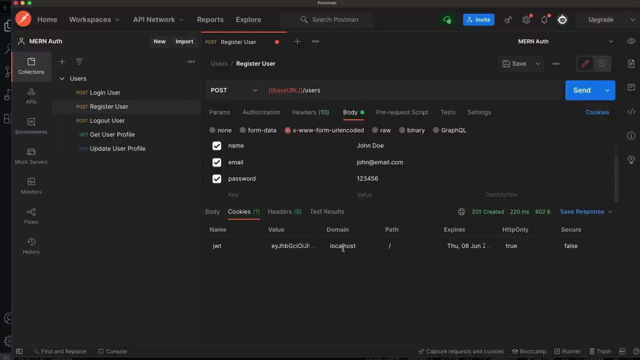 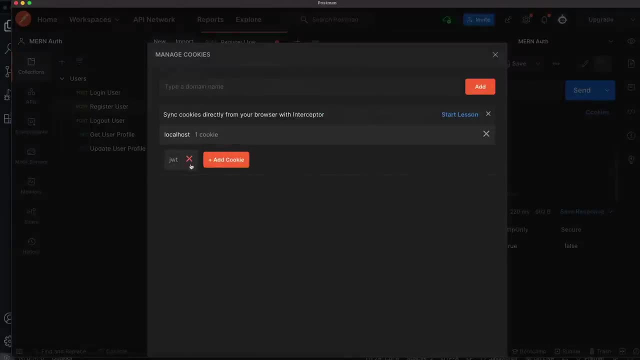 Secure is set to false because we're not using HTTPS, because we're in development, But this is how you can tell. You can tell that the cookie was set. Also, if you click right here, you'll see JWT, And if I delete that, then that cookie will go away. 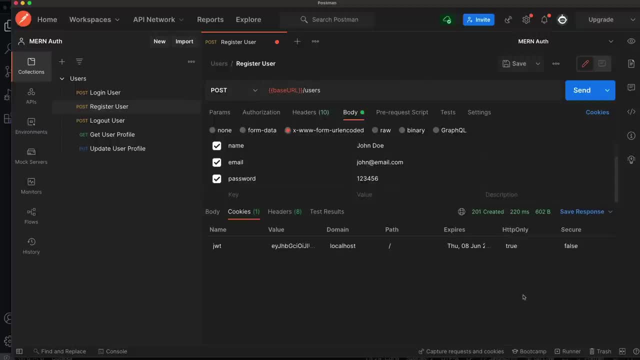 But that essentially means we're logged in if that cookie is set with the JWT value, which is this: right here Now we don't have a log out yet, So I'm just going to go ahead and delete the cookie right now. So right here I'll hit the X And it should be gone. 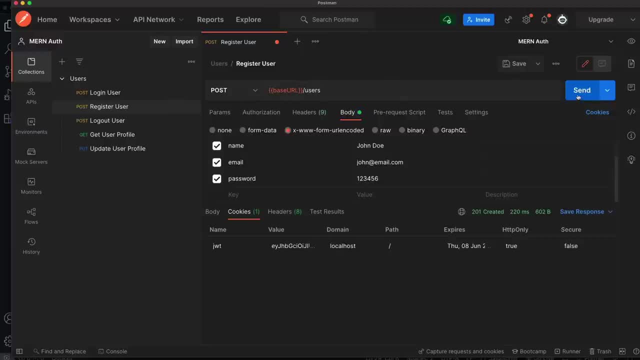 It does still show right here, But I just want to show you. If I were to send this again, you'll see the cookies. that one is gone. But if I look in the body it says user already exists, because I'm trying to register someone with the same email. 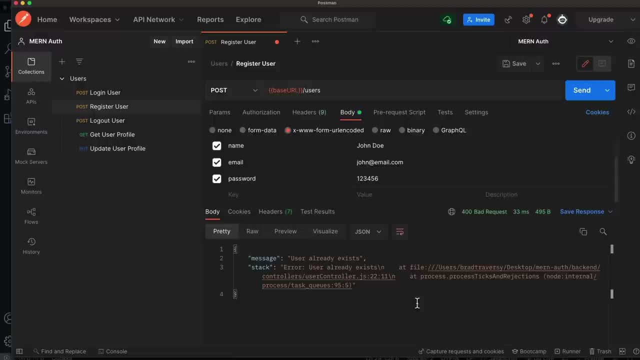 And it's formatted as our custom error handler wants, which is the message and stack if we're in development. So now let's create the login route, the auth route, And I'm just going to save this route. So if I click Save, it'll actually keep this data in here. 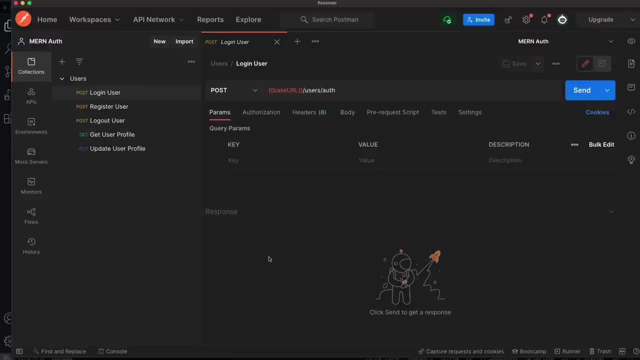 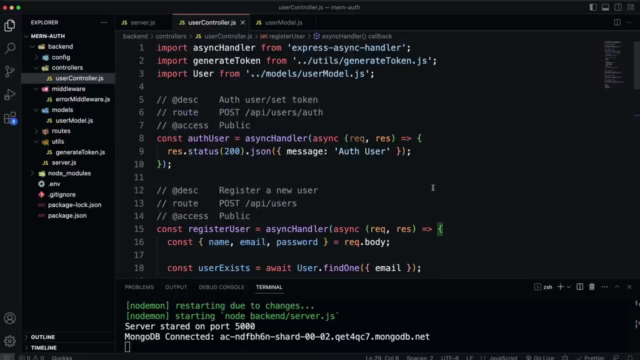 So I want to be able to log in now with John, because right now I'm logged out. I got rid of the cookie, So let's go back into the controller And let's go up to the auth user function, And this is going to be really simple now. 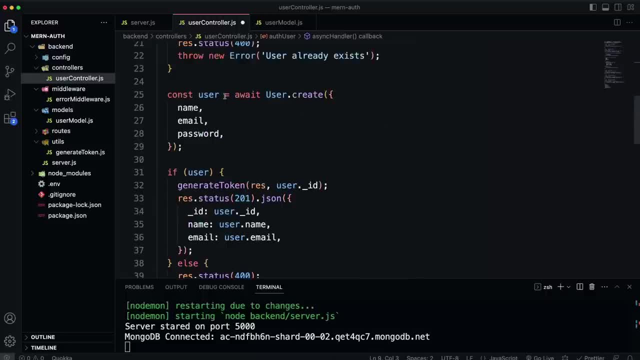 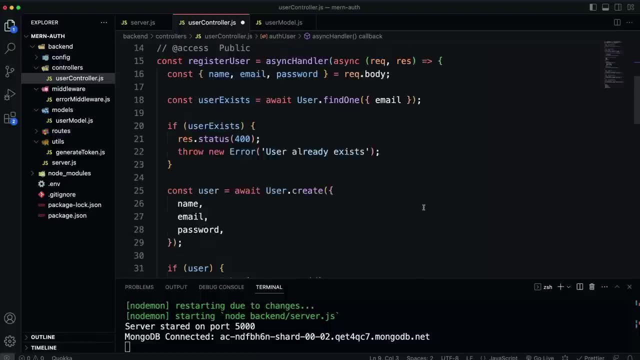 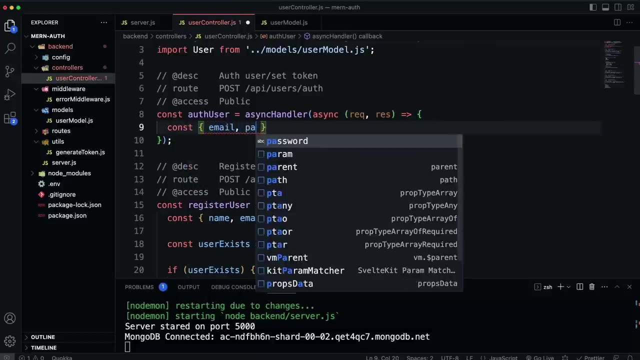 that you understand what we've done here as far as sending back the user and generating the token and storing it, And we'll create the middleware that validates that token after we do this. So let's get from the bottom. So we want to set that to requestbody email and password. 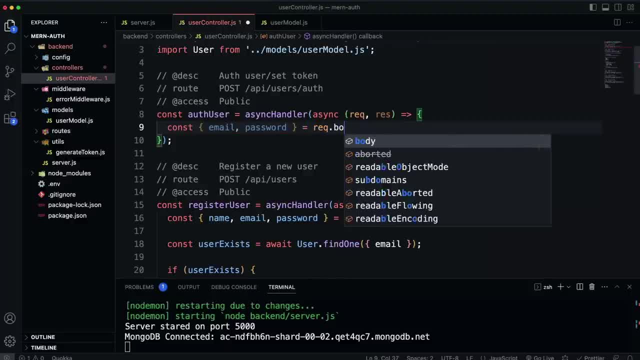 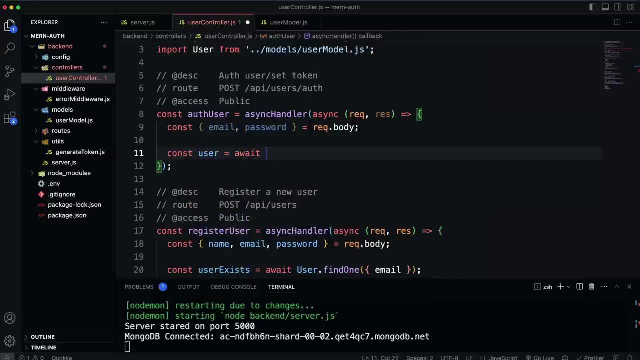 because we have to validate that, to authenticate. So we want to set that to requestbody And we want to get that user with that email. So let's say user equals await And then our user model we can use find1.. And we want to find the user by email. 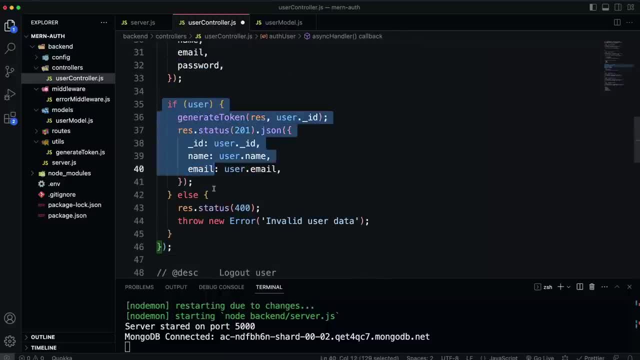 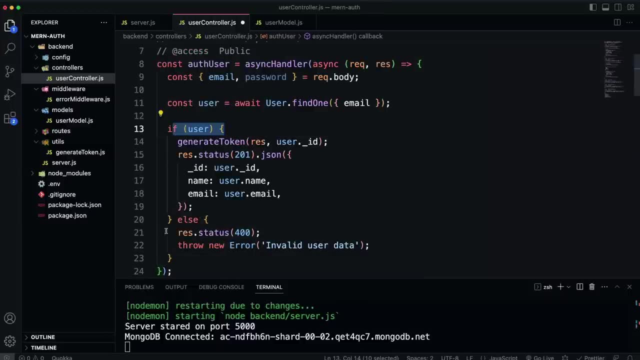 And then we're going to check for the user- And I'm just going to grab this right here, because we're doing the same thing- So after we get the user, we're going to check for it. If it's not there, then since they're trying to log in- 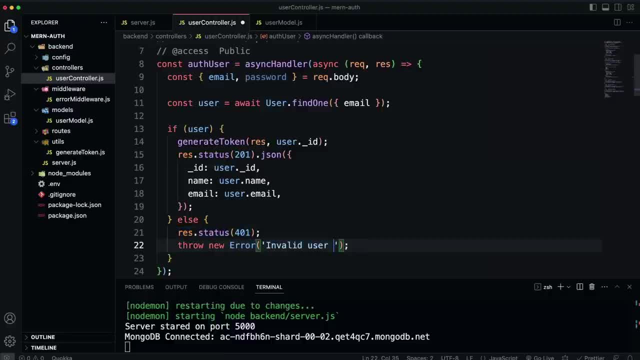 then we're going to do a 401,, which is unauthorized, And we're going to say invalid email or password. You don't want to let them know which one is which, Like you don't want them to be able to validate to see if a certain email exists. 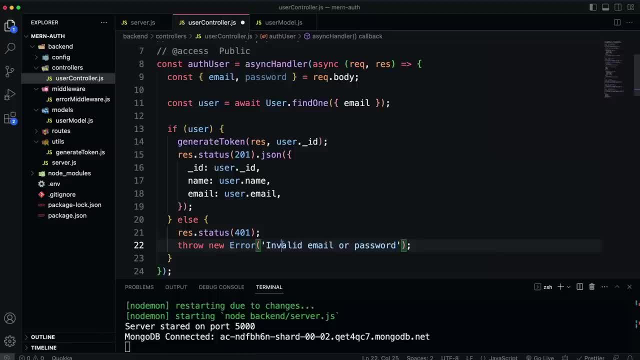 So even if the email does exist, it's going to say invalid email or password. So obviously this is not checking for the password. We're actually going to do that in the model. So in user model, let's open that up. 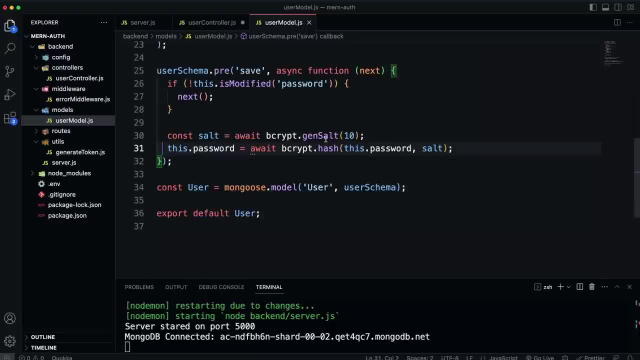 And we're going to. let's see, we already brought in bcrypt And what we need to do is match the password that's sent, which is obviously going to be plain text. We have to match that to the hashed password. So bcrypt has a method called compare that allows us to do that. 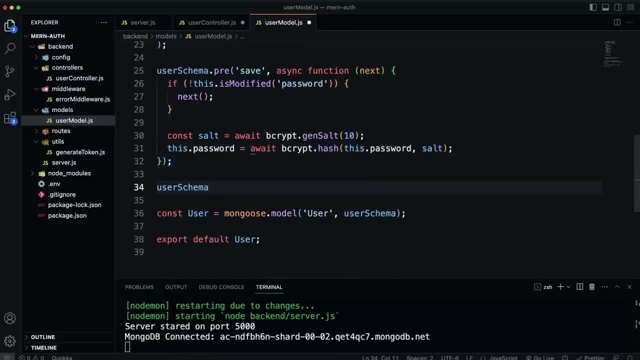 So what I'm going to do is, on the user schema, we can say methods, So we can add methods directly to the user, in this case, And I want to call this match passwords, And we're going to set that to an async. 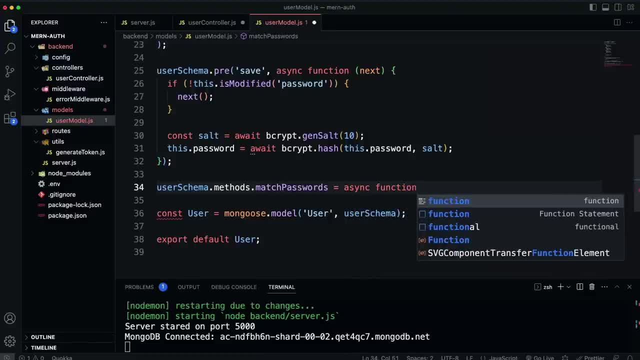 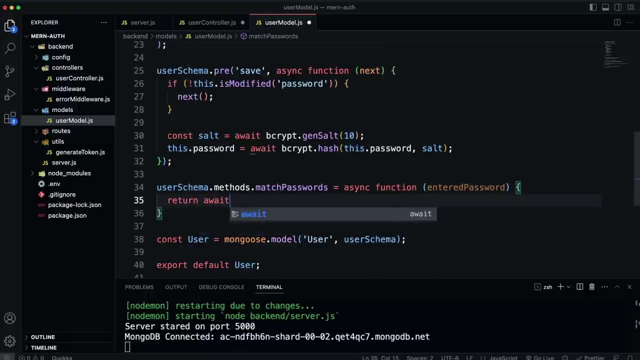 And we're going to use function here, because again we're using this keyword, And what that's going to take in is the entered- Let's say entered- password, which is going to be the plain text password, And then we're going to return, await and then bcrypt. 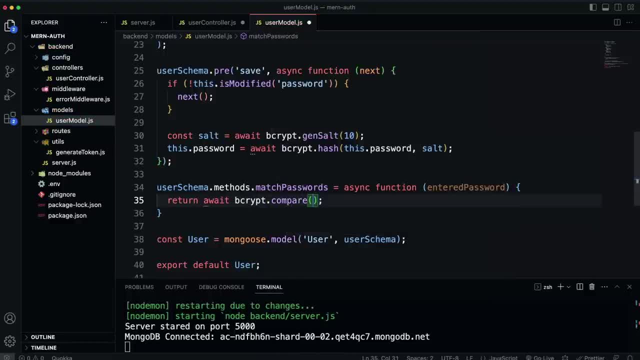 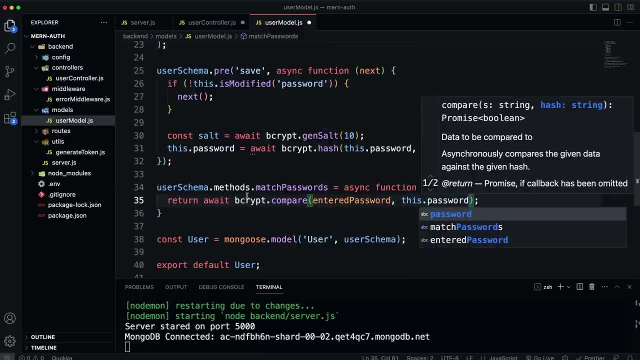 And then, like I said, there's a compare method. So this will return true or false, based on if the entered password matches this dot password, which is the hashed password that's in the database. So if these match, then it's going to return true. 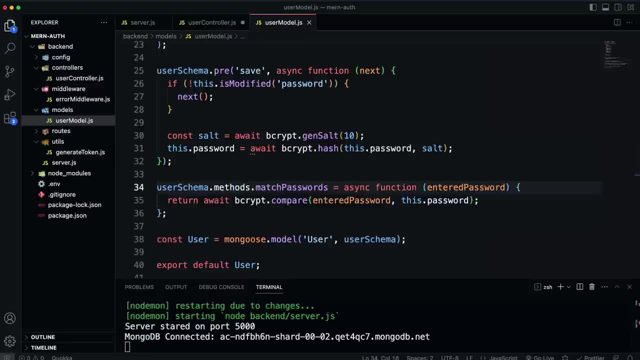 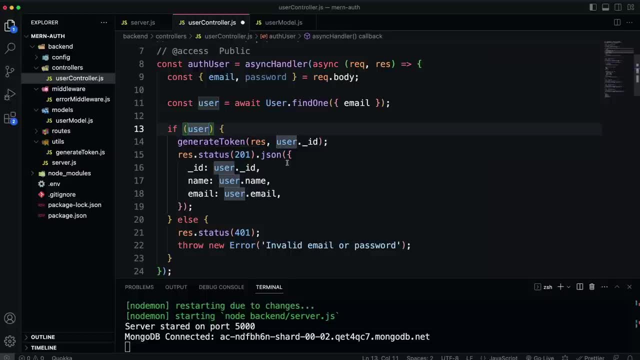 If they don't, it's going to methods, It's going to return false. So now let's save that And let's go back to the controller And, in addition to checking for the user, we're going to say and: 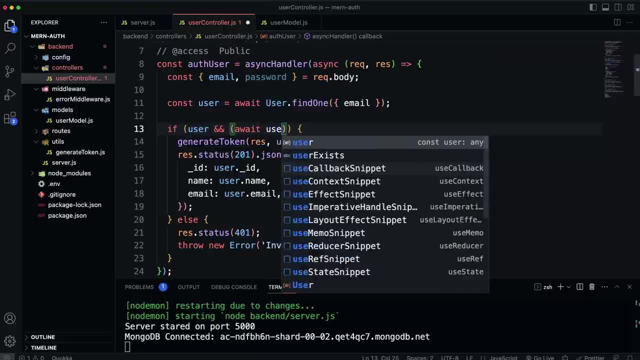 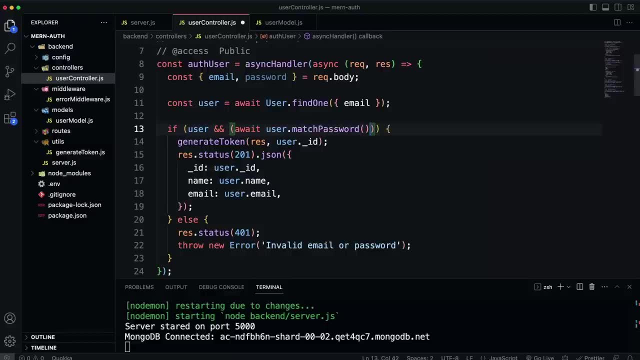 And then I'll just put some parentheses here And we'll say await. On the user itself. we can then call match password, which is the function or the method that we just added, And we're going to pass in password, which is the plain text password. 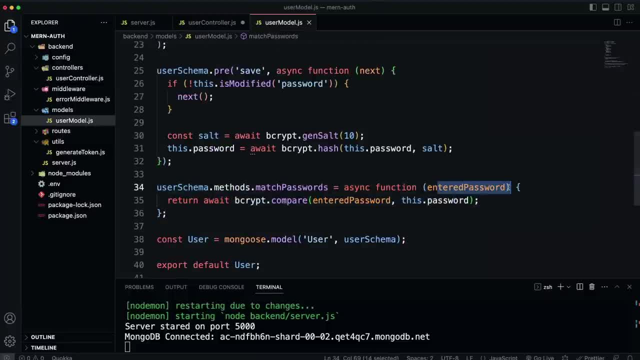 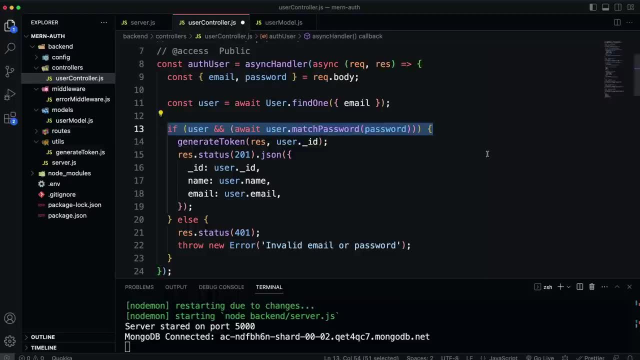 So this right here is going to Is going to call this. It's going to take in the entered password, match them, return true or false. So now we're checking for both the email and the password. So let's save that and then make sure the user model is saved as well. 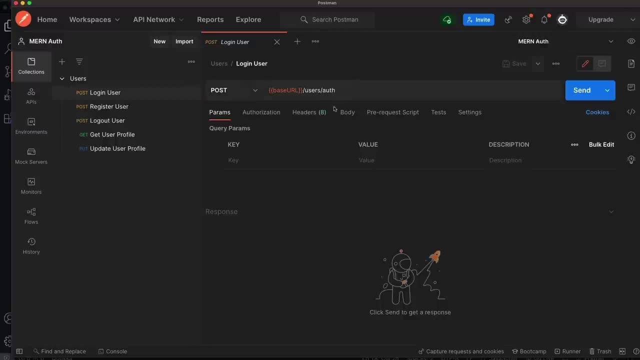 And we can open up Postman And let's go to our auth And if I just send it as is, I get invalid email or password. So if I go to my body and I go and add email, Let's see, Let's say John at emailcom, and then password. 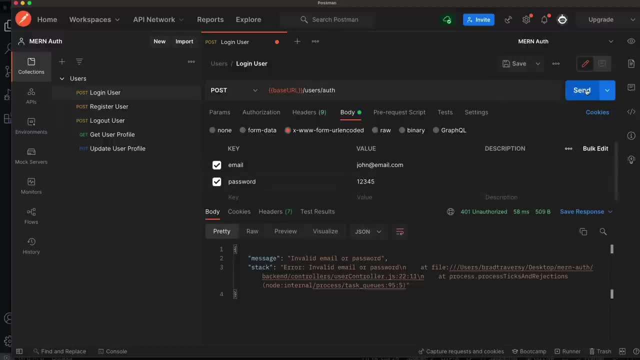 And I'm going to put the wrong password in. I'm going to do one through five and send OK. so it looks like we've got an issue here. User match password is not a function. So what did I do? Wait, user match password. 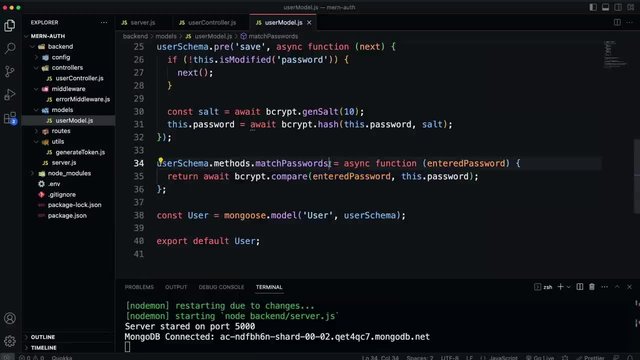 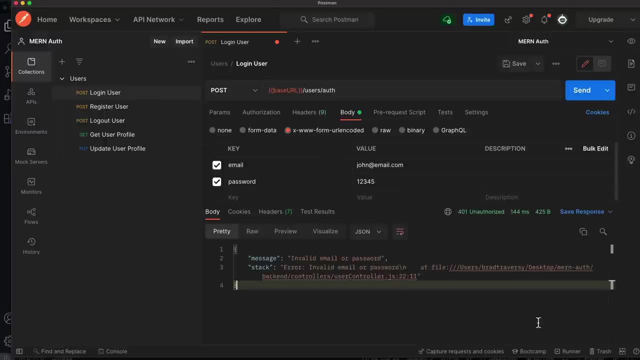 If we look in our model, we have- oh, I put passwords, Let's do just singular match password. All right, let's try that again. OK, so now we get invalid email or password. Now let's go ahead and do the right password and send. 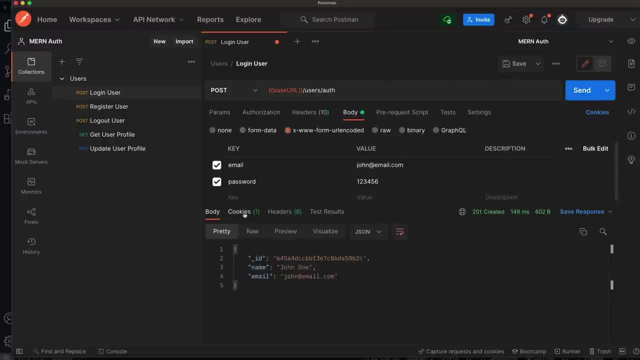 And now we're authenticated And you can tell because of the cookie right here. All right, we have our JWT cookie And if you click right here, you can see it as well. All right, cool. Now we want to be able to log out. 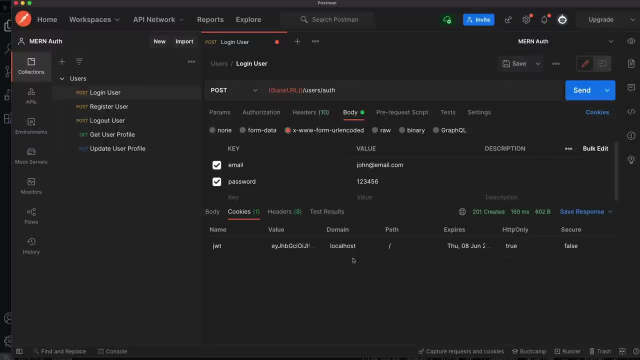 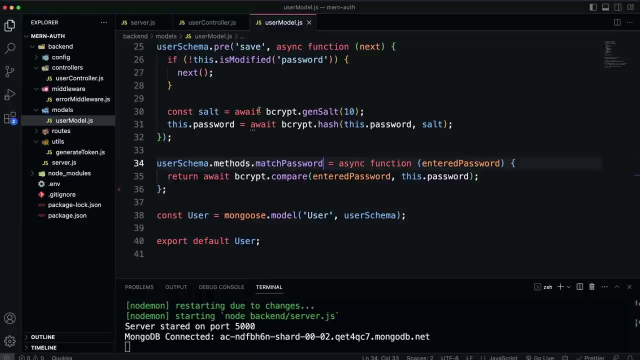 Which means distribute, All right. So we're destroying that cookie. So, instead of going to cookies and x-ing this out, I want to have a route to do that. So let's go back into our controller here And we're going to create a log out user with our controller. 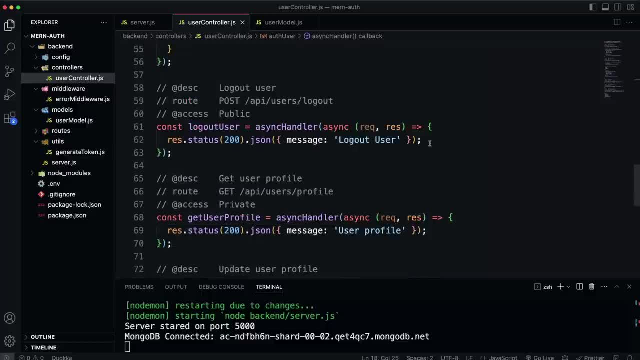 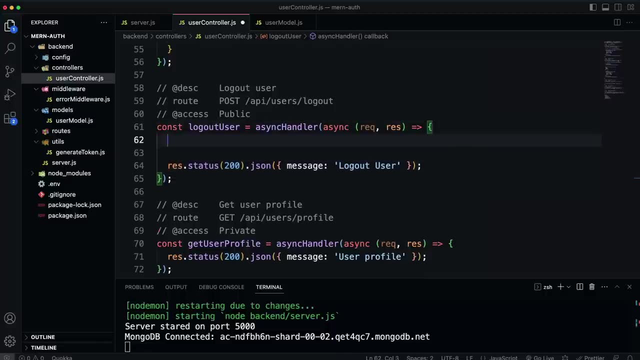 We actually already have the function, So we're just going to add the functionality, which is actually really simple. So we can leave that. And the way that we can destroy this is by saying rescookie And we want the name of the cookie, which is JWT. 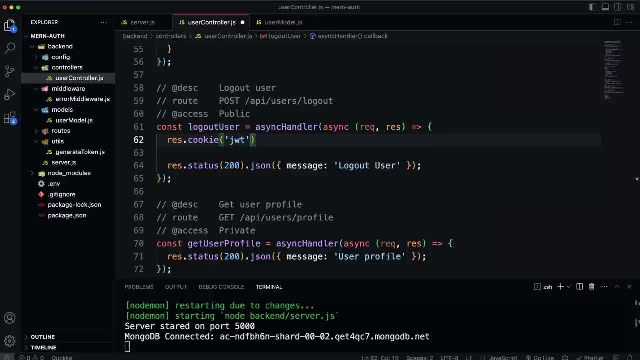 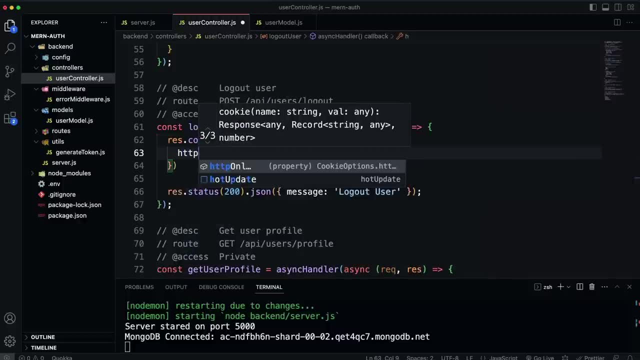 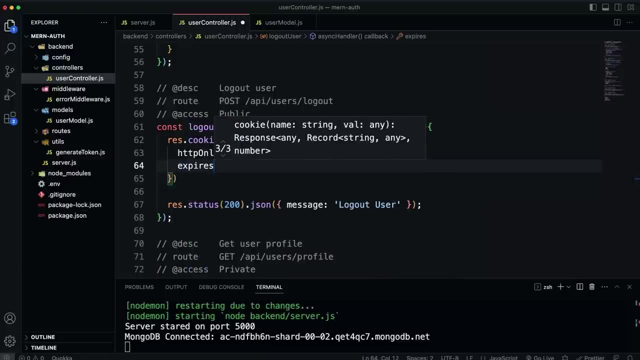 And you could call it anything. If you want to call it token or whatever, that's fine. We're going to set it to nothing And then in the options we're going to set, still set HDB only to true And then for the expires we're going to set that to new date and then zero. 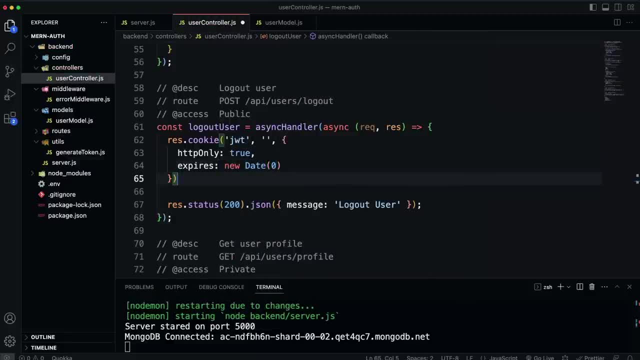 So it's just going to expire right away And then we'll keep this status here. But let's change the method to we'll say logged or we'll say user logged out. Okay, so let's save that one And let's go back to Postman. 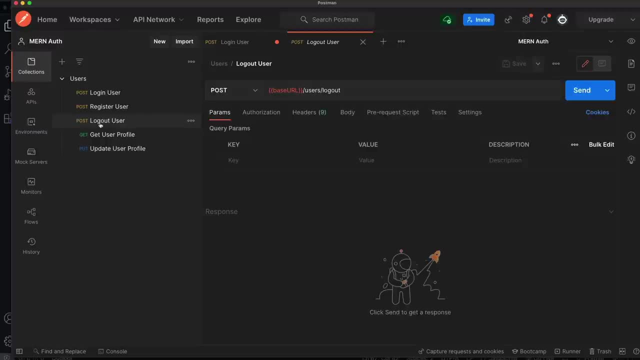 I already have a log out route. So if we open this up and then I click send, we get user logged out. And now if we look in cookies, you can see there's no JWT. Okay, if I come over here, you can still see it here. 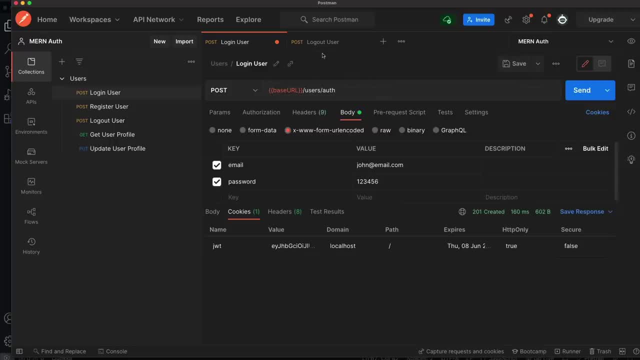 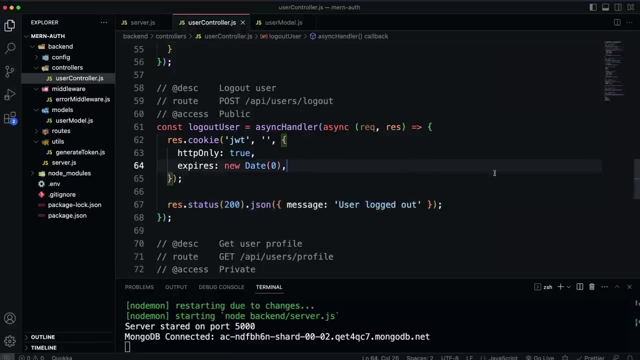 But if we look in cookies here, it's not there, So we're now logged out. So now that we're able to register, log in and log out, we need to now be able to actually protect our routes, Because right now it's kind of useless, right. 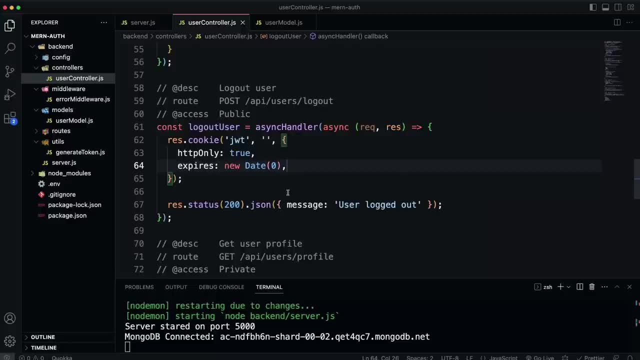 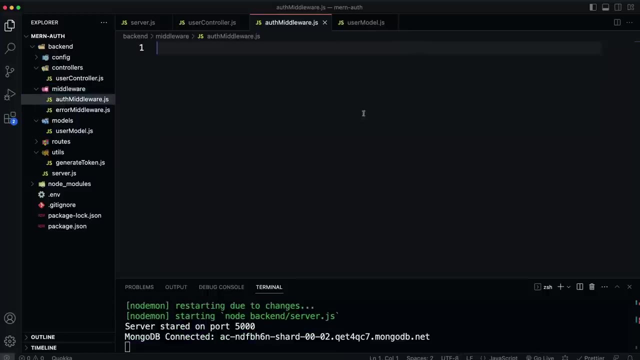 It's just setting the cookie. We need to do something with that cookie. So that's where the auth middleware comes in. So in the middleware folder Let's create a file called auth middlewarejs. Now in this file we're going to need to check the cookie. 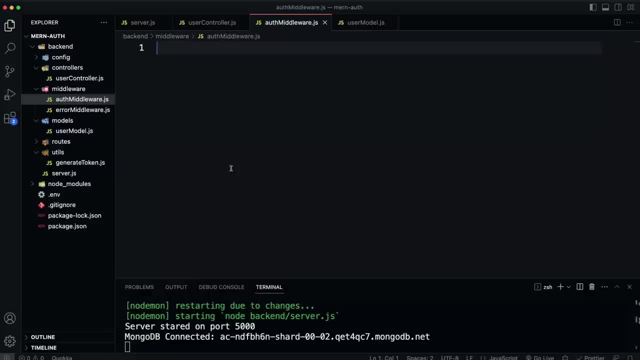 We're going to need to parse the cookie, which we're going to use, the cookie parser package, for which you should already have installed, as you can see here in packagejson, And it's just a one line of middleware we need to add in the serverjs to be able to do that. 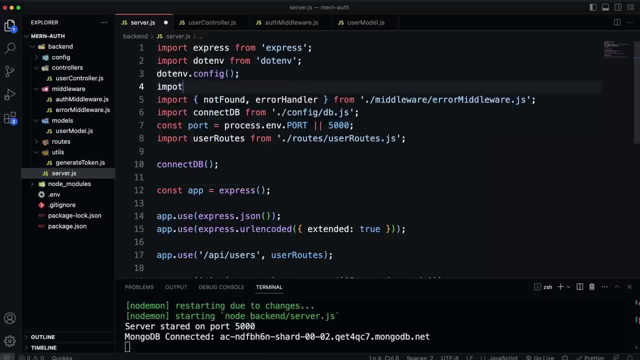 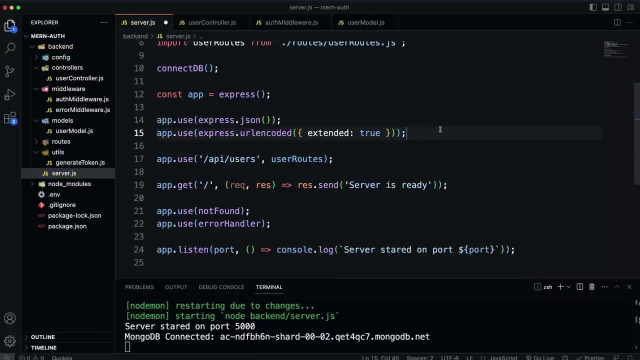 So first off, let's import The cookie parser. So we're going to import cookie parser And then I'm going to add the middleware right here. We'll say appuse, And we're just going to pass in here cookie parser. 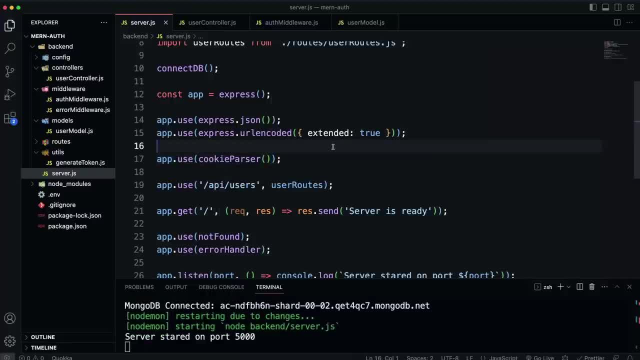 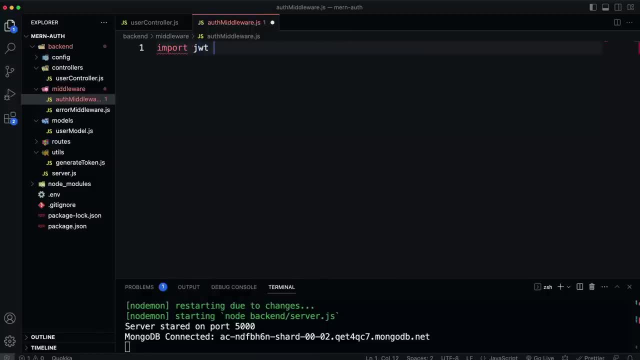 Make sure you add your parentheses as well. Okay, So now we close that up, Close the model up, And now, in auth middleware, we're going to bring a couple things in. First off is the JSON web token, Because we need to get that. 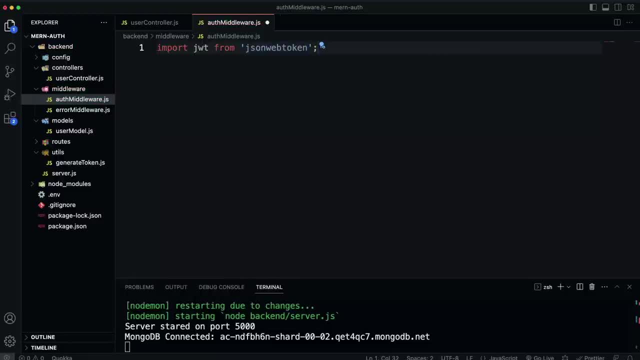 We need to get the payload from the token, which is the user ID. So there's a method called verify that will verify the token and enable us to get the decoded, you know, the payload information. And then we're also going to use the async handler. 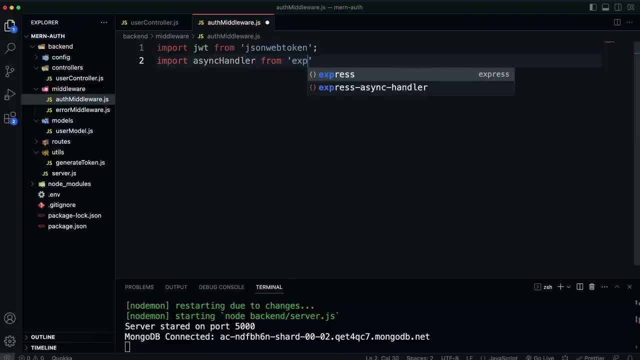 So let's bring that in from express async handler And let's also bring in the user model That's going to be from dot dot slash models, slash user model. Make sure you add the dot JS, All right, So we're going to have one function in here called protect, because that's what this is going to do. 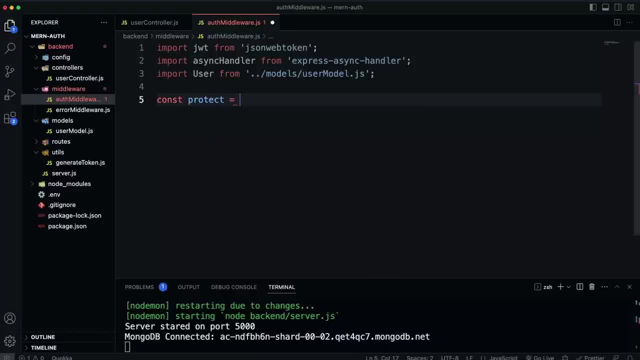 It's going to protect routes so that you have to be logged in to access that route. So this is going to be wrapped in the async handler, So let's add that first And then in here we're going to have an async function- arrow function. 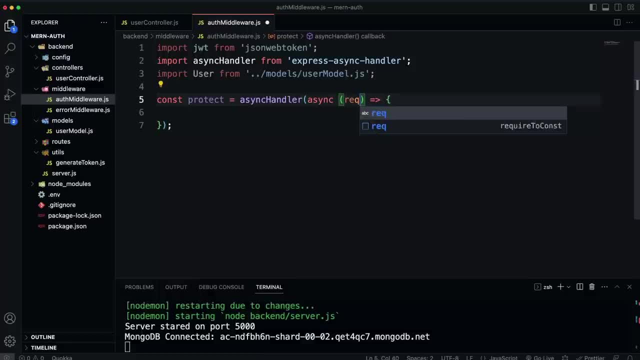 Okay, And this is going to take in request response, and next, because it is oops, these should be commas, because this is middleware, So we need to call next when we're done. Now I'm going to initialize a variable called token. 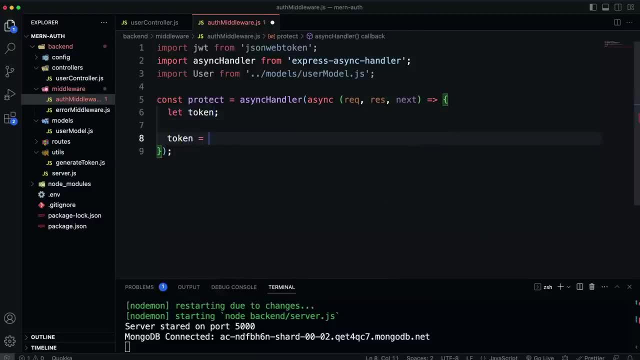 And then we're going to set token to request dot cookies and then the name of the token, which I call JWT. So just make sure if you called it something different, you put that here And this. we're allowed to do this because of the cookie parts. 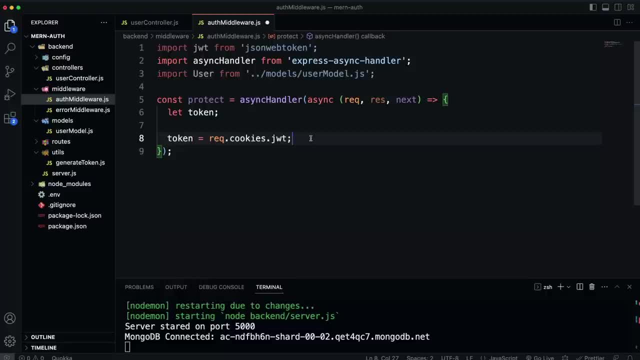 So if you don't have that installed and set up, then you wouldn't be able to use this. So that will get the token. So we want to check for the token, All right. So basically we're checking for the cookie. So if it's there, then actually let's add our else first, because this is pretty simple. 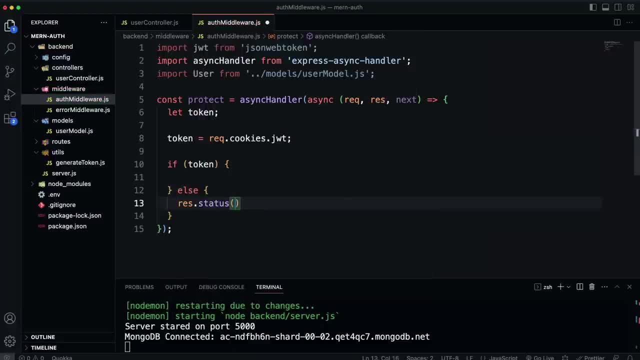 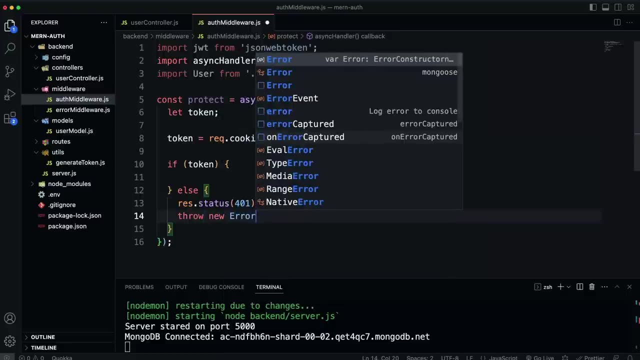 We're just going to return a status of 401, which is unauthorized, And then we'll throw an error. Okay, So throw new error And let's say not authorized, And I'm just going to say no token, All right. 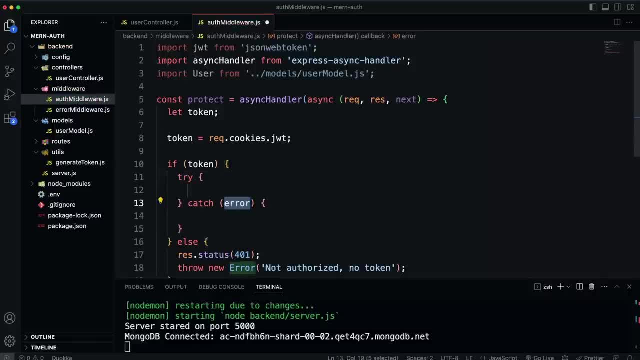 Now inside here I'm just going to use a try catch And in this error I'm going to say resstatus 401.. And we're also going to have an error that says not authorized, But I'm going to say instead of no token. 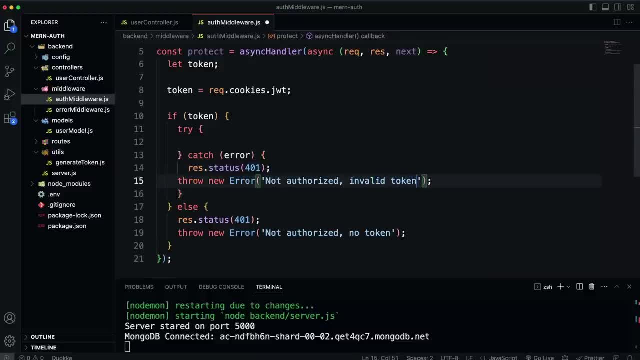 I'm going to say invalid token. Okay, Because here it is there, The token is there, It's just not valid. Now in the try, let's go ahead and create a variable called decoded And we can set that to our JWT verify method. 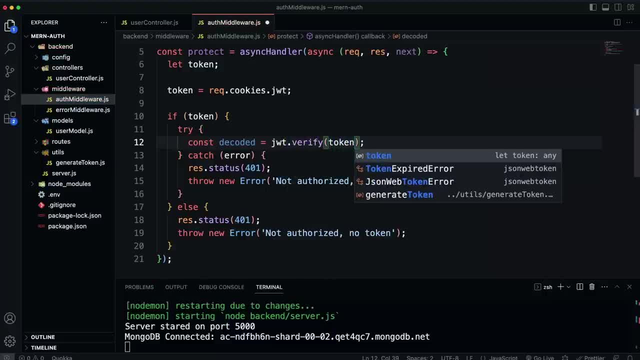 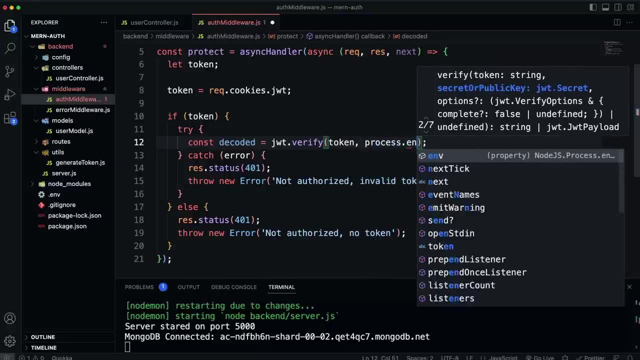 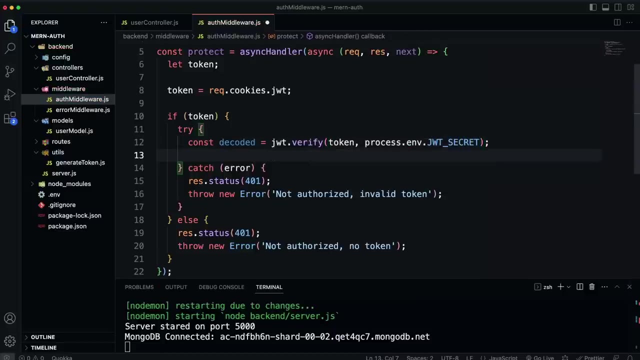 And that takes in the actual token that we're getting from the cookie, And it also takes in the secret. So we want to do processenvjwt underscore secret. Now that decoded object should have the user ID in it. So what we want to do, the ultimate goal here, is to set requestuser to the user of the token. 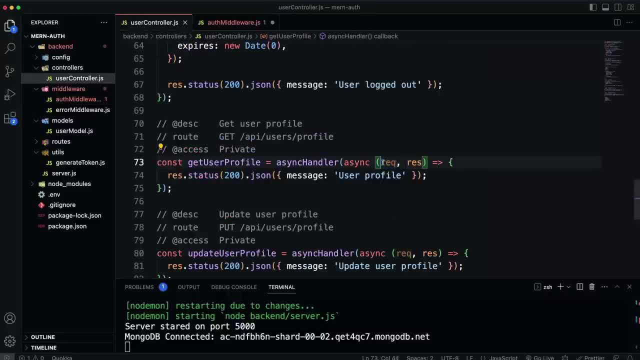 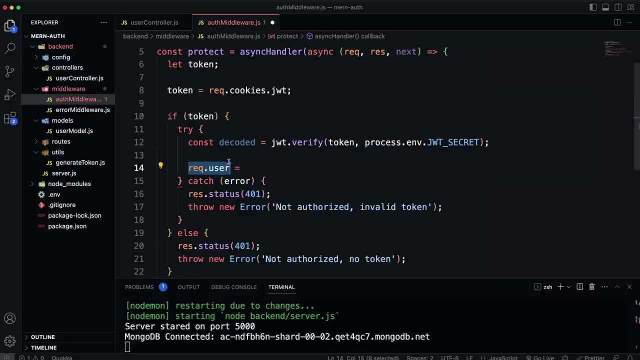 Because this requestuser we can access from any route. So requests here, any of these, we should be able to say requestuser And that will be whatever user is logged in And you can, you know, do whatever you want from there. 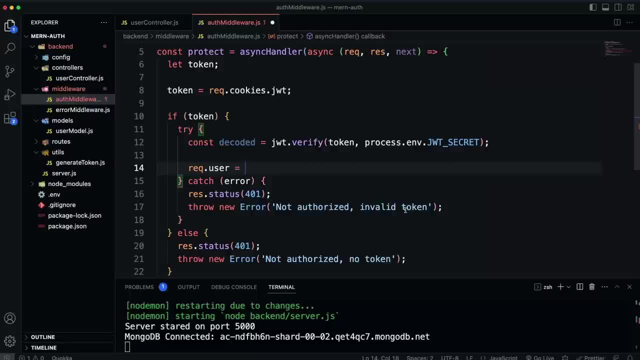 Whether you want to fetch their products or orders or whatever it is you want to do, Get their profile. So let's do await And then with the user model we can say find by ID And that ID is going to be in that decoded object. 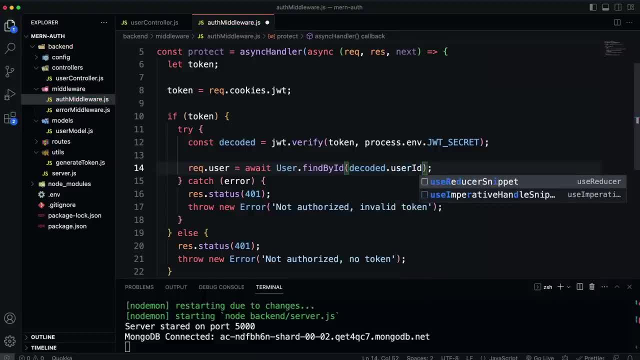 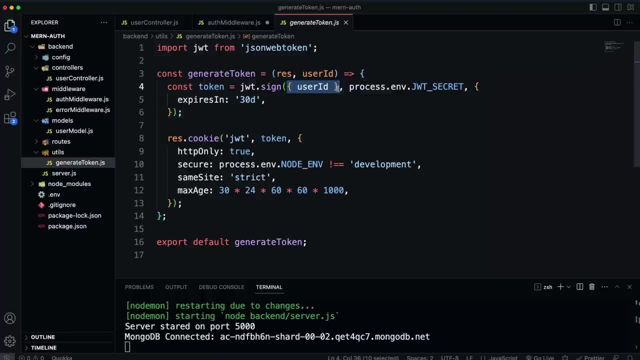 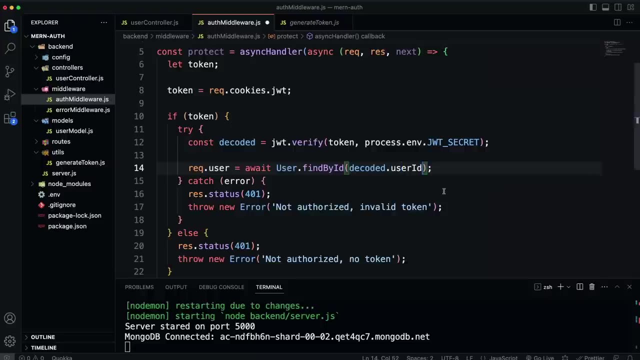 So decodeduserID, All right, And the reason it's there is because when we generated this, the token we called the sign method. we passed in the user ID And you can pass anything you want in here as a payload and then access it from here. 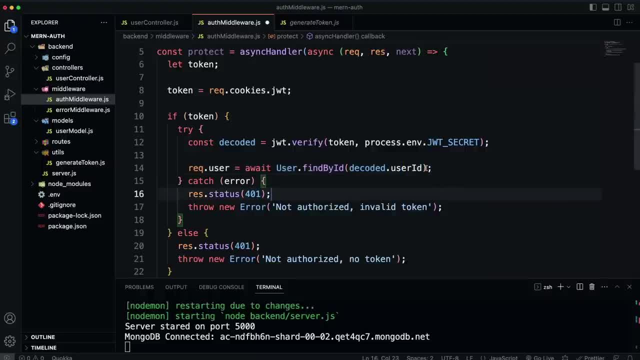 Now, this will get us the user, but it will also include the password, And even though it's hashed, I still don't want to return it, So we're going to add on select and then pass in a string of minus password. 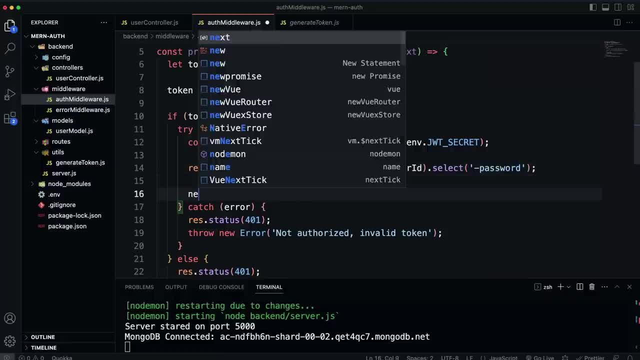 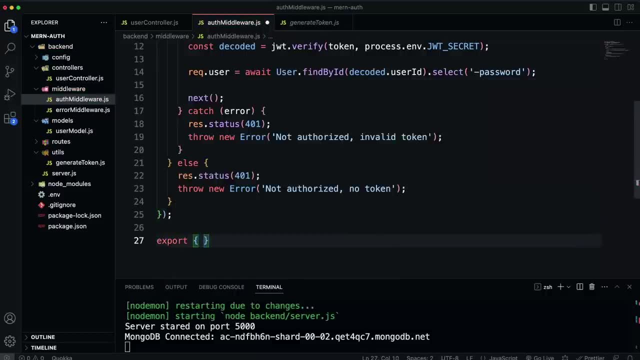 And that will make it so the password doesn't get returned, And then we just simply want to call next. Okay, And that's it. So now down here, we just want to export the protect middleware, And I'm not going to export as default, because you might want to add in some other authentication middleware. 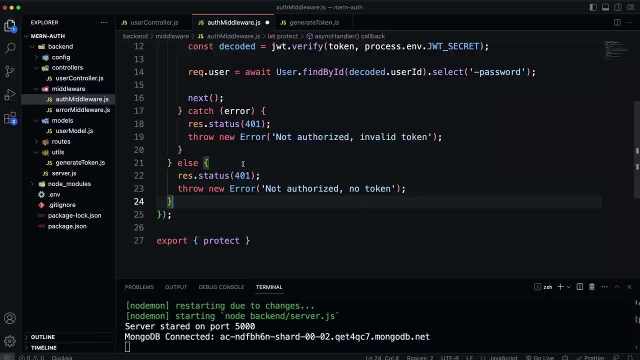 Like, for instance, in the e-commerce course. we have an admin middleware to check to see if the user is admin, Because some routes you might only want admins or some other role to access. So to use this, let's go. Actually, before we use it, I just want to show you. 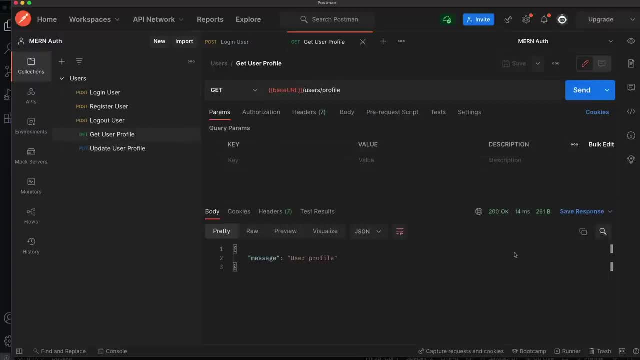 If we go to get user profile And I send And I'm not logged in right now. If I go to cookies, there's no JWT, I'm not logged in, but I can still access this route. So what I want to do is protect this route and the update route. 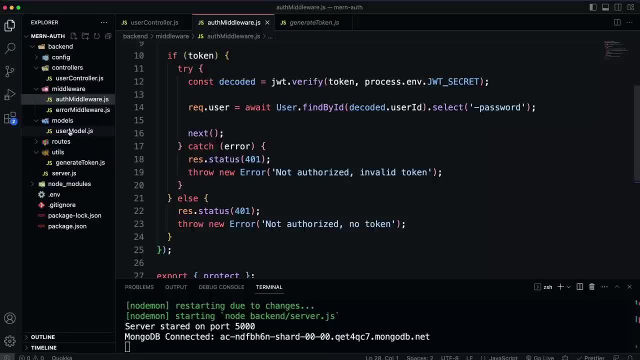 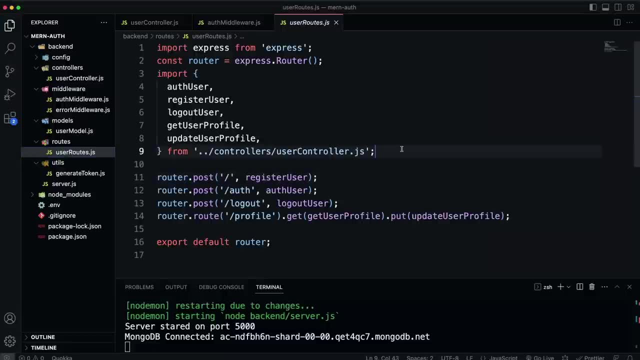 So let's go to the user routes file And what we're going to do is bring in the protect middleware. So let's say import Protect From our auth middleware, And if we want to use it, we simply add it as a first argument. 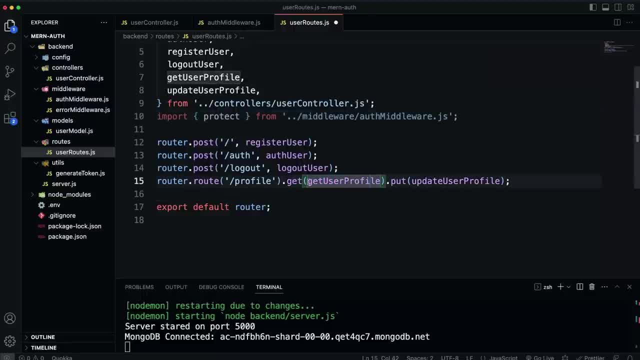 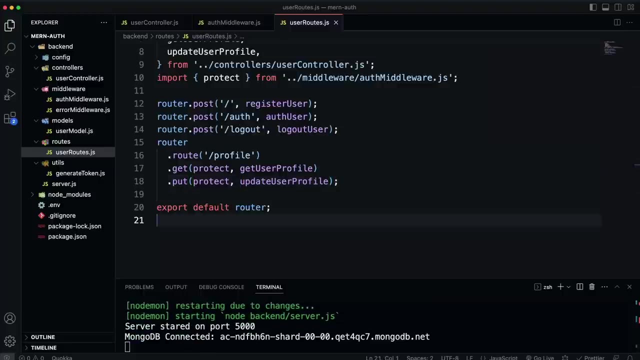 So right here, where we have our get request to get the user profile, I'm going to add in protect as the first argument. Same thing with the update. So right here we'll say protect, Save that. Now let's go back over here. 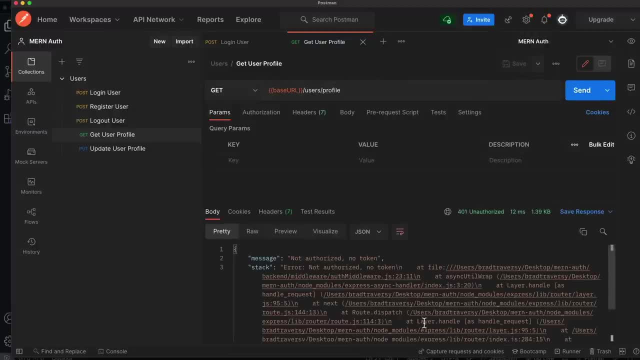 And I'm going to try to access this. And it says not authorized No token If I go to my update And I send Not authorized No token. So now, if I log in, right, I'm going to go to log in user. 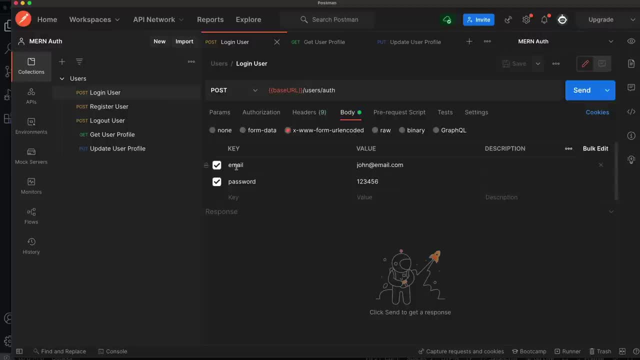 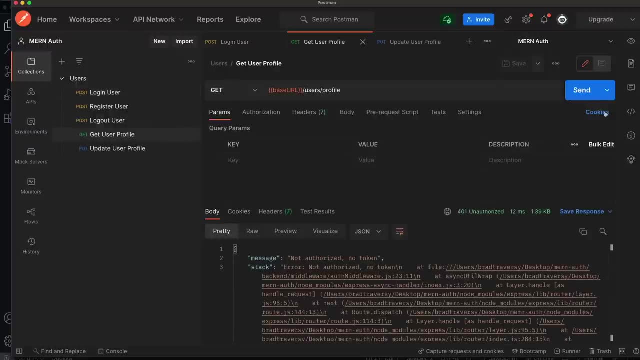 I have the correct info in here. Email password I'm going to send. Now I'm logged in, meaning that cookie is there. So if I go back to get user profile and send, it works Because that auth middleware it goes through that first. 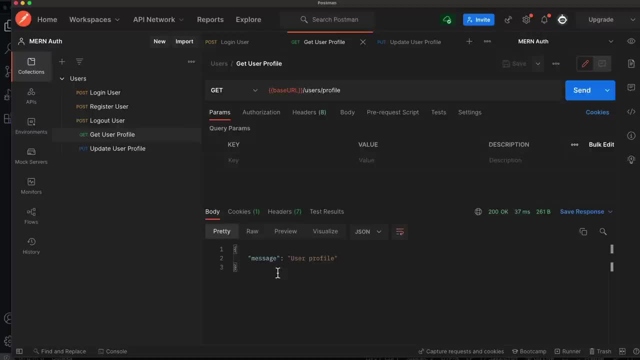 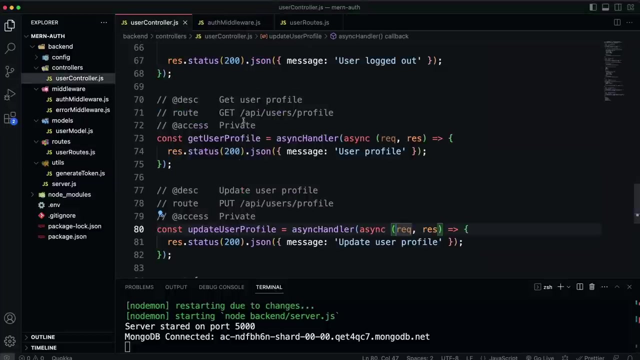 And it checks to see: is there a token? Does that JWT in the token? Is it the right one? Is it verified? If it is, then we can go ahead and get the user. Now, not only that did we protect it, but if we go into our controller, into our get user profile, we have access to that user through requestuser. 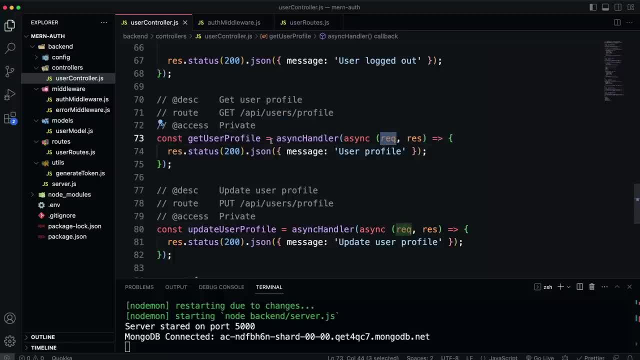 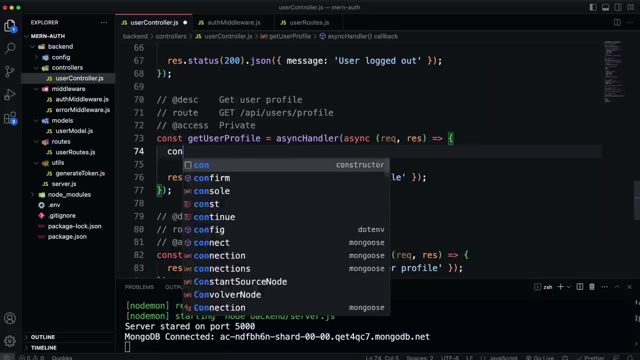 So let's say you have a get orders function right And you want to get just the logged in user's orders, You can just simply add in requestuser Underscore ID into a query. So what I want to do here is just, let's say, const user. 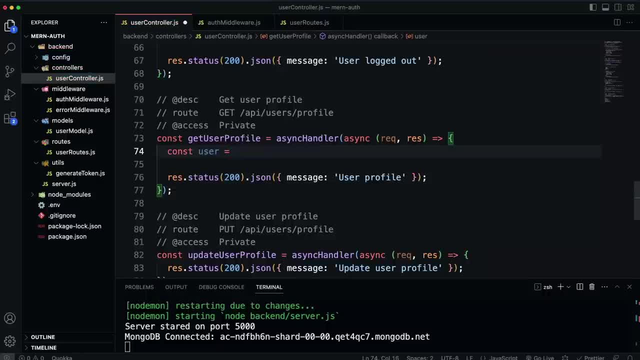 I don't want to return requestuser directly because there might be some fields that I don't want, even though the password isn't being returned. Actually, let me just show you what it does return. So we'll do a console log of requestuser. 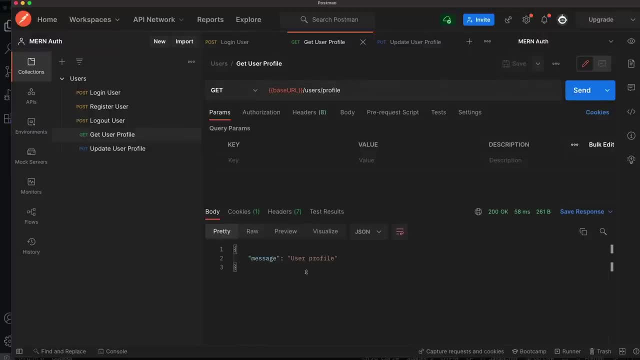 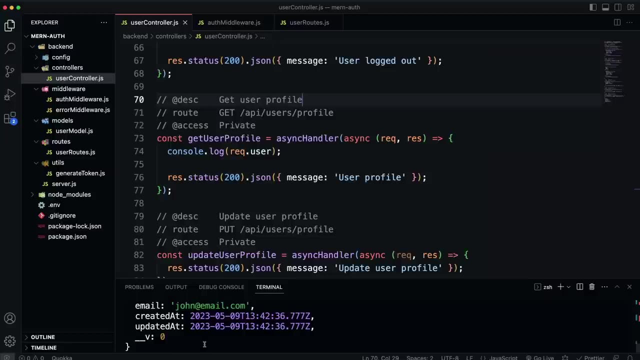 And then let's go and hit that route, get user profile And then we'll come back over here And you can see, this is what it gives me: the ID name. email created at updated at version. So the password is not here. 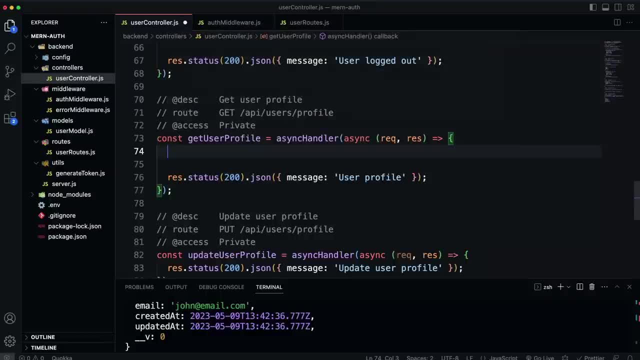 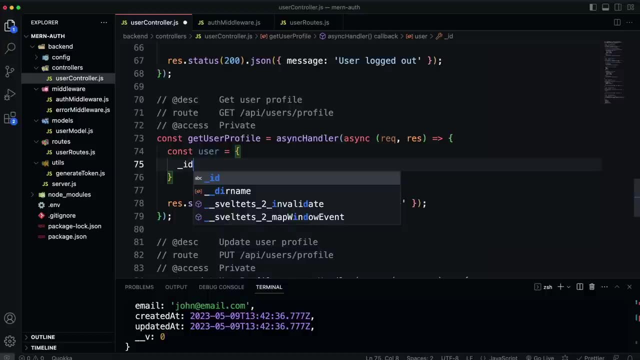 So I could just return that. But what I'd rather do is just construct, let's say user equals and we'll say underscore ID. Or you could just do ID Depends on how you want to set your application up. But let's say requestuserunderscore ID. 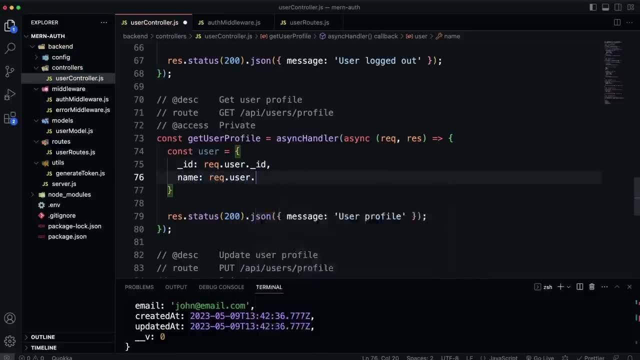 And then name requestusername, And then email requestuser. Okay, and then I just want to return that. So right here, let's get rid of this message And say JSON. And then we want to just pass in our user. 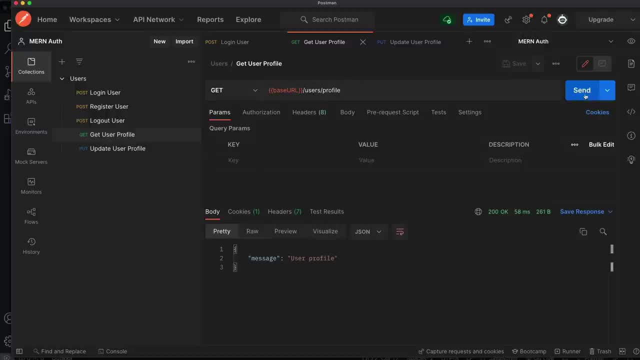 So let's save And go back, Send, And now we're able to get our user data through this route And, of course, if I log out, Go ahead and log out And then I go back to my get user profile route. 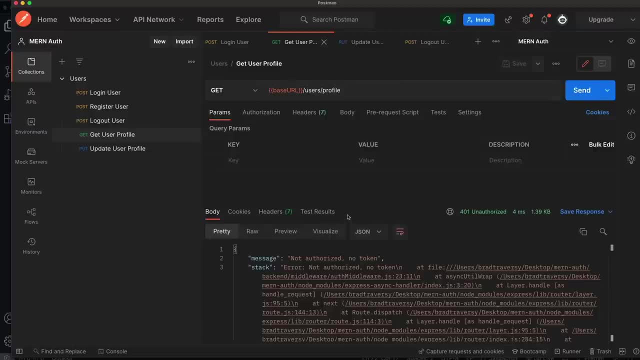 And I try it, Can't do it because I don't have the token. All right. So the very last thing we need to do in the back end- I shouldn't say the very last, But the last before we move on- is the update, right. 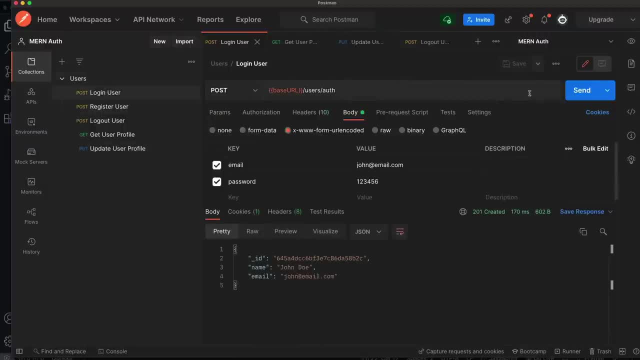 We want to be able to update a user, So let's log back in, And now I should be able to access this put request, This update route, Which right now is just returning a string, But we're going to go ahead and change that now. 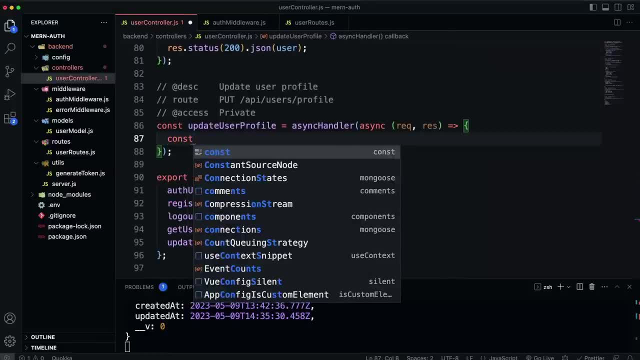 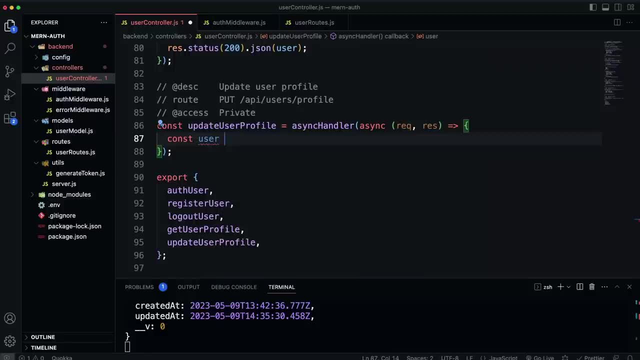 Now the first thing I'm going to do in this function is get the user, And I know we have the user in requestuser, But we don't have the password And I want to be able to update that. So we're going to say: user equals await. 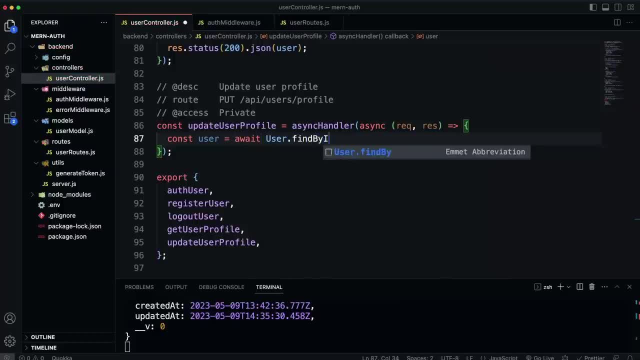 And then userfindById And pass in here the requestuserUnderscoreId- Okay, And then we're going to check for that user. So say if that user, and else If it's not there, then we'll do resstatus 404.. 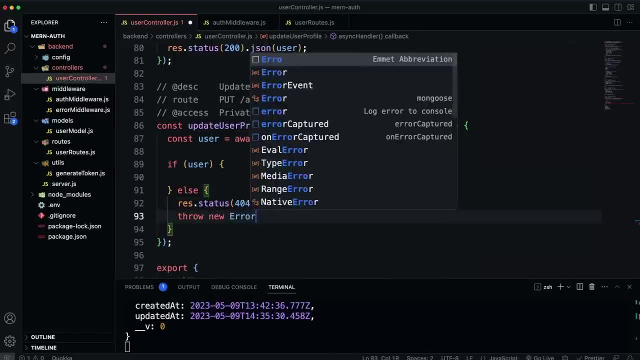 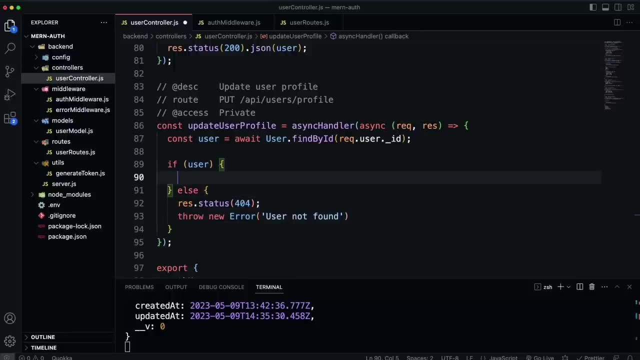 And then let's throw, Say throw new error And we'll just say user not found. All right, Now, inside here, what I'm going to do is say the username equals the requestbodyname Or username, Because if that name isn't included in the body, then I just want to have it. you know, stay what it is. 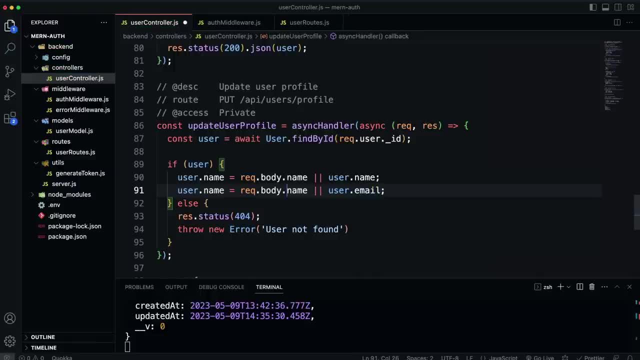 And we'll save that for email as well. So email Email, Okay, And then Let's check for the password Now. you might not want to have them update their password here, Or you might. It's really up to you. 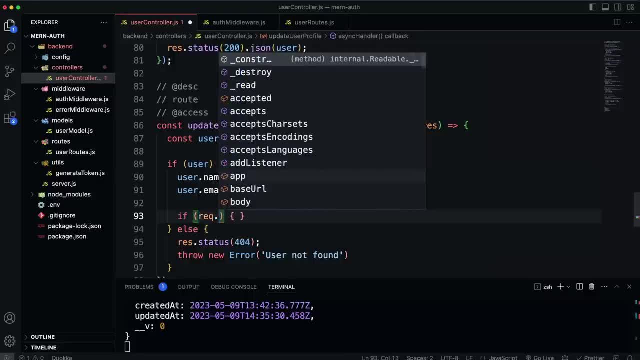 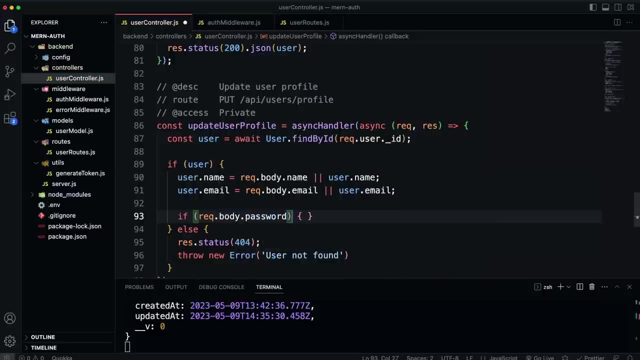 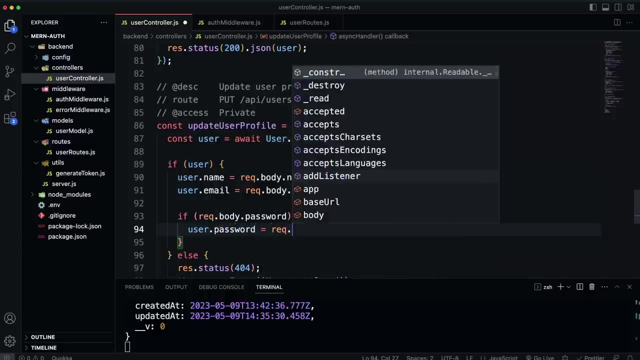 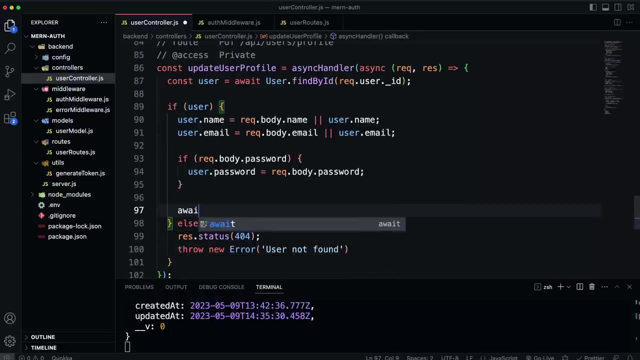 But I'm going to choose to let them. So we'll say request. Yeah, If requestbodypassword, Then let's set the userpassword to requestbodypassword. Now we're going to save the user, So we want to await usersave. 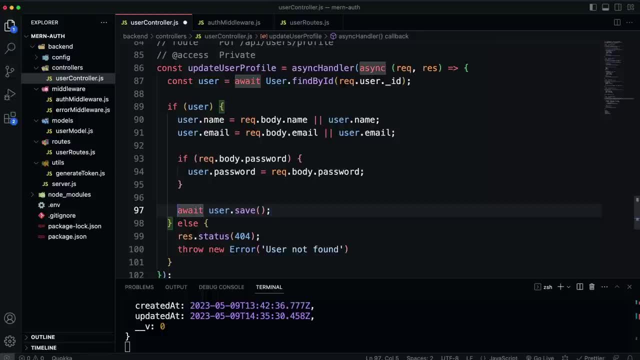 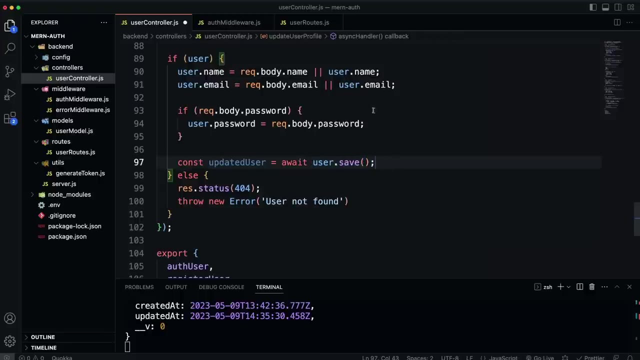 And that will save it with the new data. But I do want to get that new data to respond with it. So let's put it in a variable, So we'll say const updated user And set that to whatever the save gives us, which will be the user with the new data. 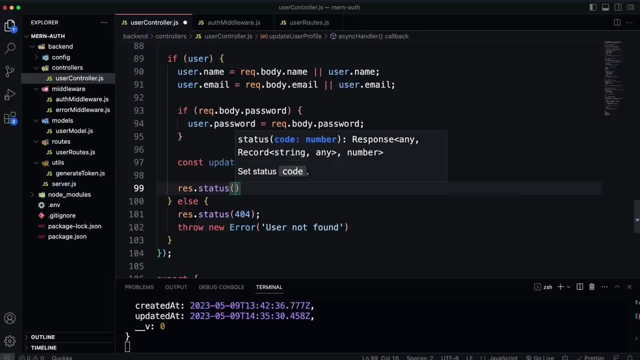 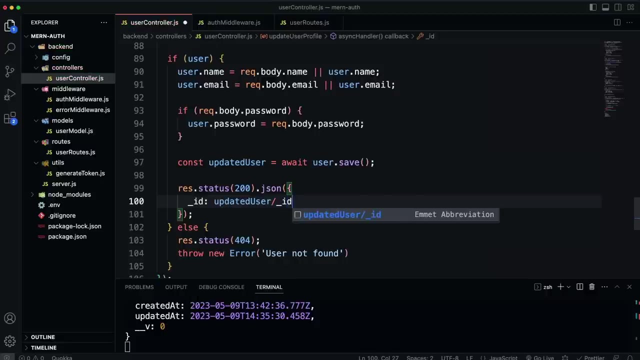 And then we're going to respond So resstatus200.json, And we'll pass in an object here with underscore ID Which will be the updated user. Dot underscore ID. Okay, And then we're going to do the name of the updated user. 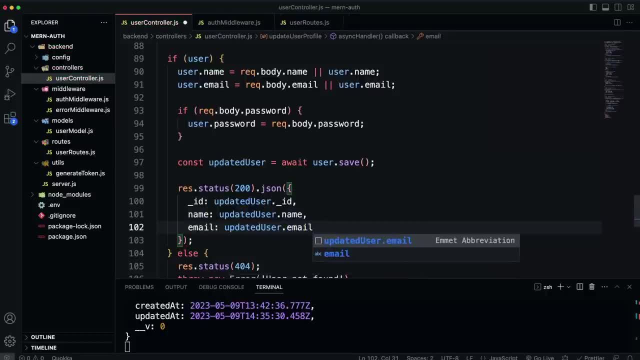 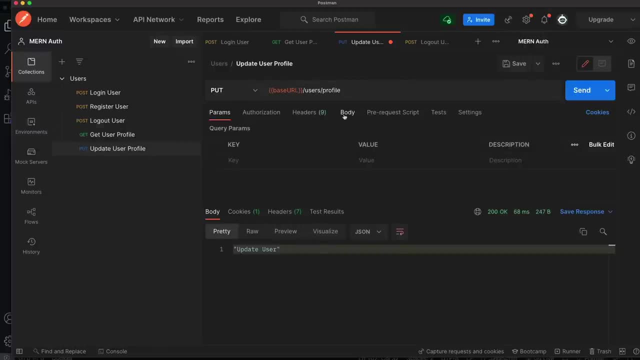 And the email And I think, yeah, that should do it. So let's save. Then we're going to go to Postman and go to our update user profile And go to the body And I'm just going to add or I'm just going to change. 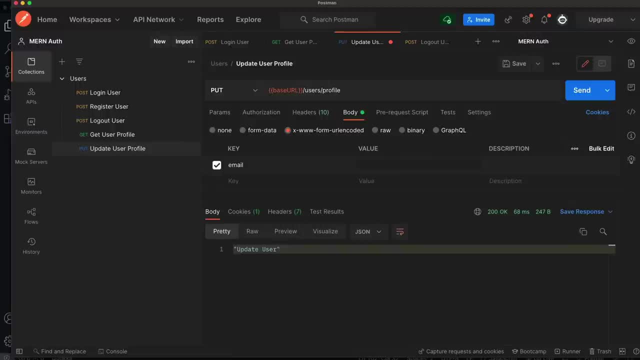 Let's do the email. So right now it's john at emailcom- At least mine is. Yours might be different, But I'm going to change it to john, let's say, at gmailcom, And then I'm going to send. 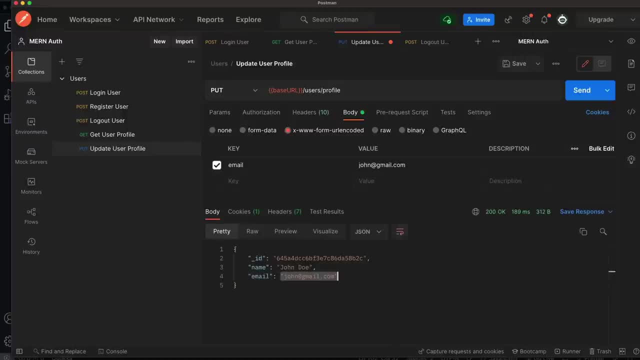 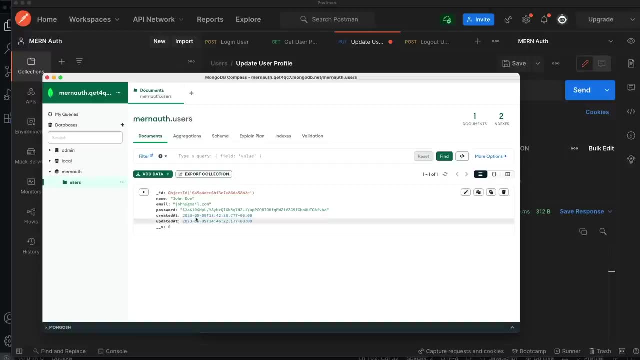 And now I get back the new user, John at gmail. Okay, And if I go to Compass And let's see Reload data, Yeah, So it's changed in the database- John at gmail. To change the name, I could add on to this and say name. 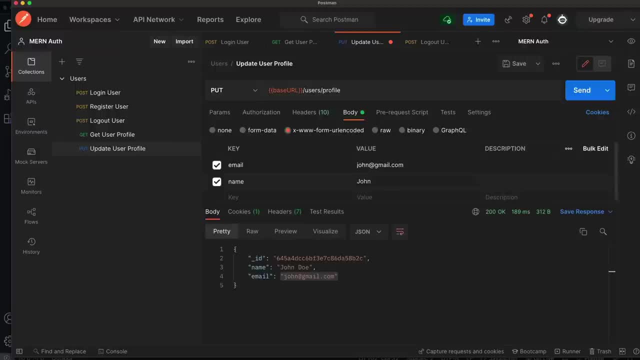 Let's say John- I don't know, John, James, And send that- Okay, Get that back Now. remember, if you're going to log in again, you have to use the new email And the new password If you're going to change that. 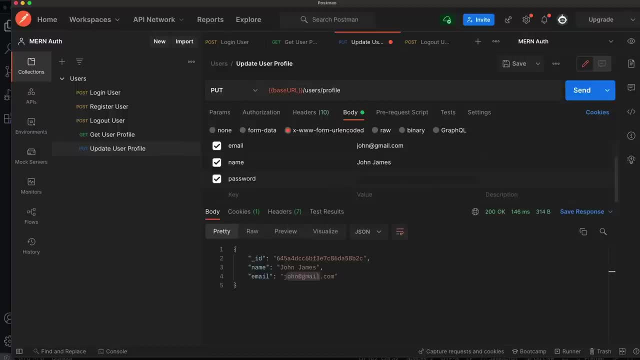 So let's change. Let's try that too. So password: I'm going to change to 12345.. All right, So now I'm going to log out. Go to the log out, Clear the cookie. And now Excuse me. 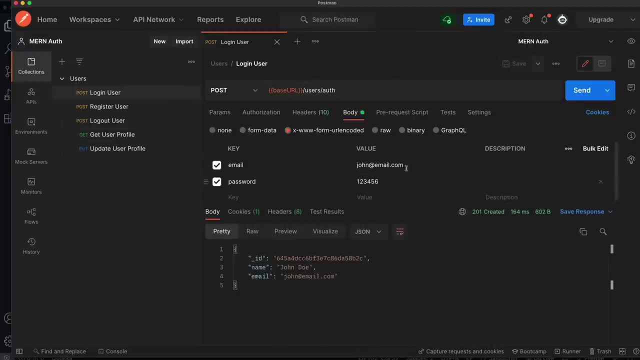 I'm going to go back to the login And I'm going to try to log in with the old info. Doesn't work Now if I change it to john at gmail, Let's see if that works. No, I changed the password as well. 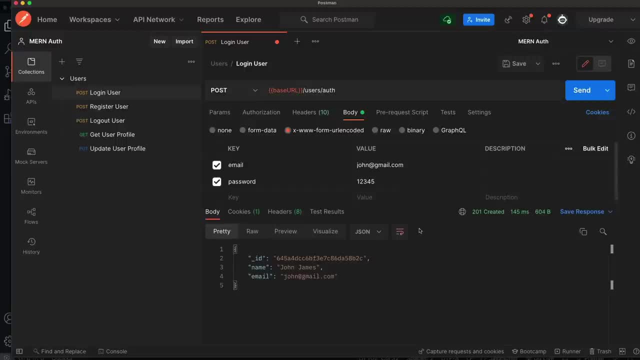 So let's do 12345.. And now I'm in. All right, Cool. So our authentication, Our back end API, is completely working And all set And you could use this with any front end. You know, If you want to use view, 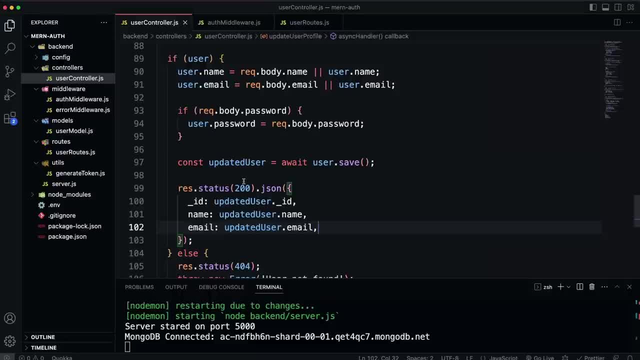 Or svelte, Or build a mobile app Or whatever- Anything that can send HTTP requests, Then you can use this API. All right, But we're going to start on the second part, Which is this one, And we're going to use this one. 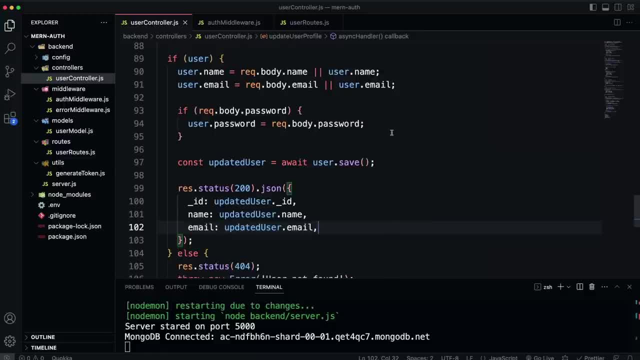 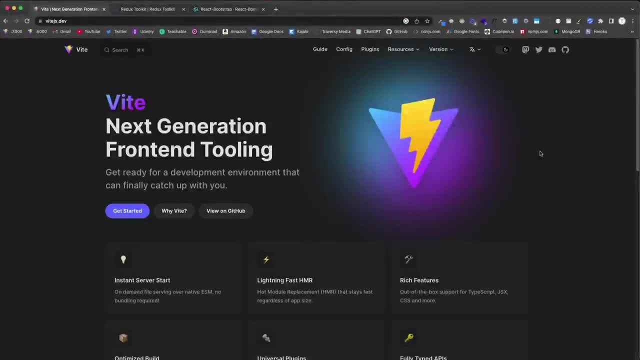 Okay, So now we're going to start on the front end And I just want to go over some of the tools that we'll be using. So, as far as just a starting point, A boilerplate, We're going to be using Vite. 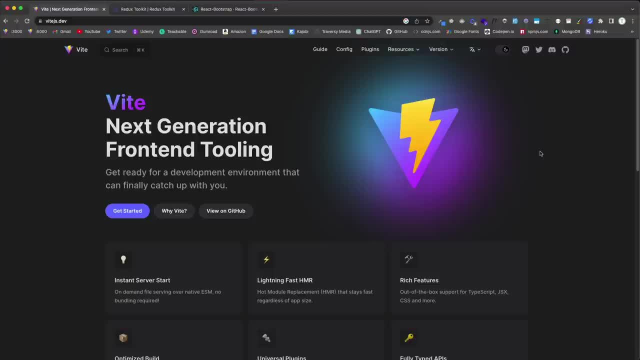 Which is a modern build tool, And I'm using it instead of Create React app. If you want to use Create React app, that's fine. That's actually what we used in the ecommerce course, But no matter which one you decide to use. 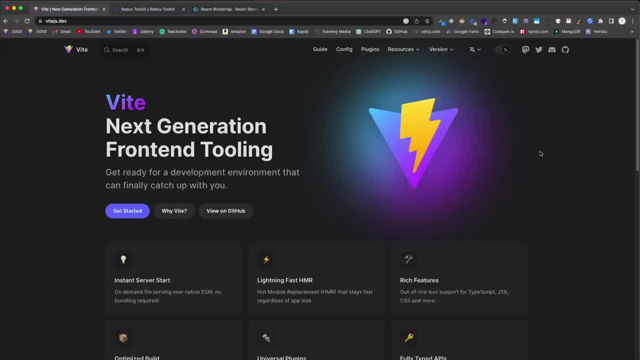 once you get it set up, the rest of the code will be the same, So it's up to you on what you want to use. Vite is is ultimately faster And it's just. it's a more modern. it's not a module bundler. 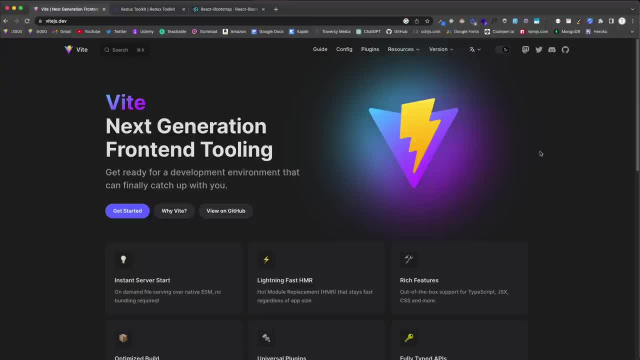 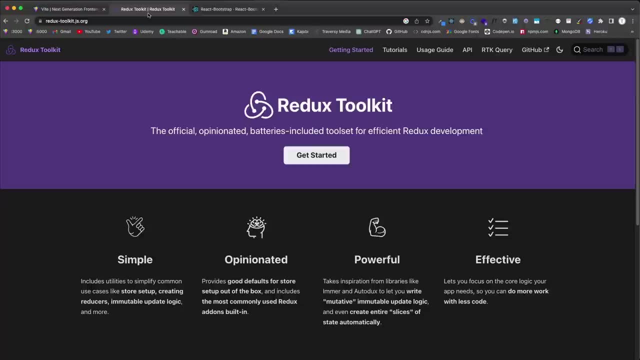 So you know, it's not like Webpack or anything like that. It actually uses ES modules in the browser, So it's very, very quick. So that's what we'll be using as far as getting set up. Now, as far as state management goes, we're going to use Redux and Redux toolkit And Redux toolkit. 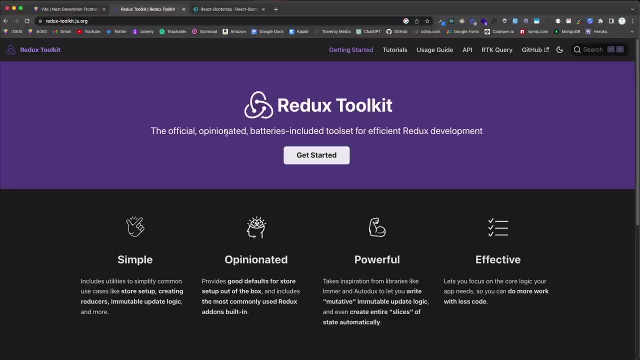 just makes Redux easier and more enjoyable to work with. For those of you that have used just vanilla Redux, you know that it can get quite messy when you're, you know, creating your actions and your reducers. and all that where Redux toolkit basically puts everything into what we call a 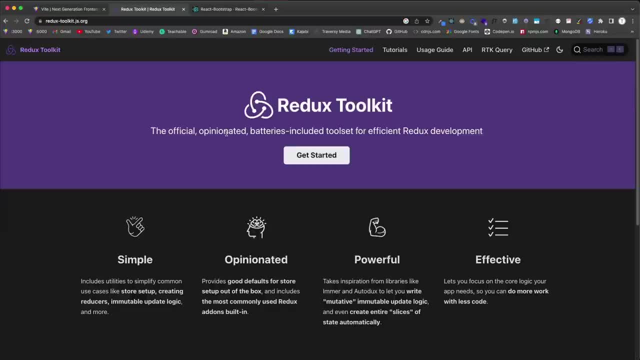 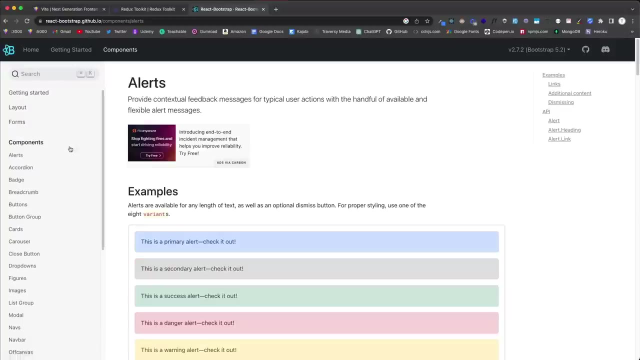 slice, And your slice holds your state and your reducers for that particular resource, whether it's users, products, blog posts, whatever it might be. And then we're also using React bootstrap for the UI. So basically, we have all of our bootstrap components, For example, buttons, we have 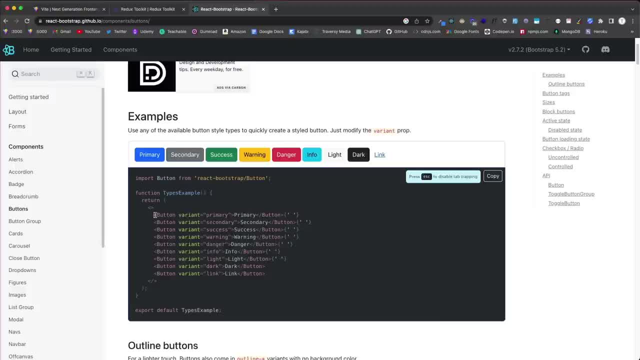 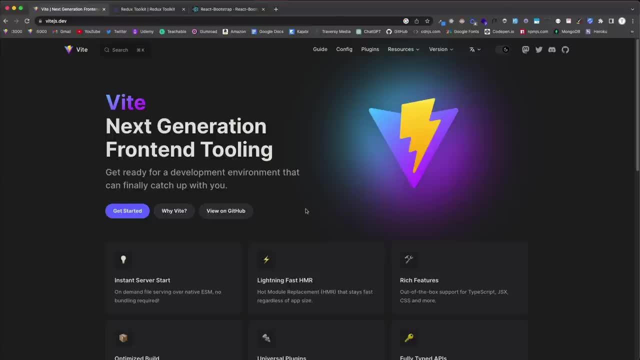 available as React components, So we can just bring in a button, we can use it, and there's different props that we can pass in. So those are the three main things that we'll be using, But we'll have some small packages like React, toastify and some other things as well. 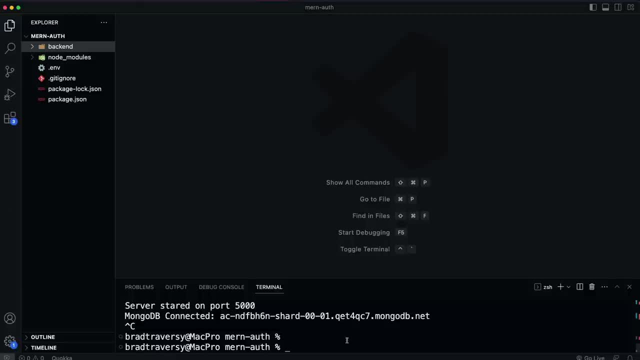 So let's get started. I'm going to go back into my project here and I stopped my server and I'm in the root And what I'm gonna do is run npm create, And then we're going to do Veet at latest, And I'm 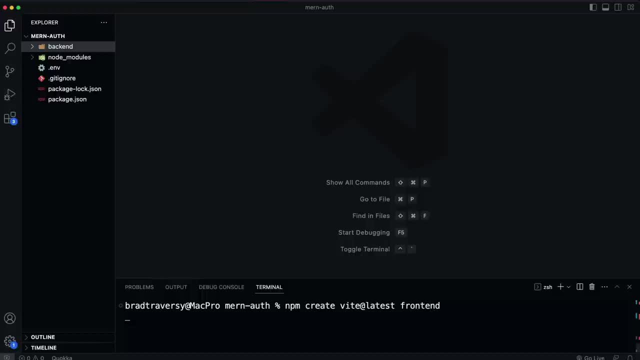 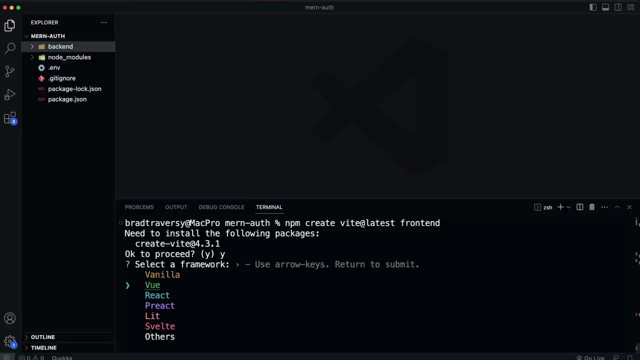 going to put everything in a folder called front end. So basically, this is going to create our React application in a folder called front end. let's say yes, Okay, now we're going to get some questions here. let me just make this bigger. so v you can use with vanilla: vanilla, javascript. 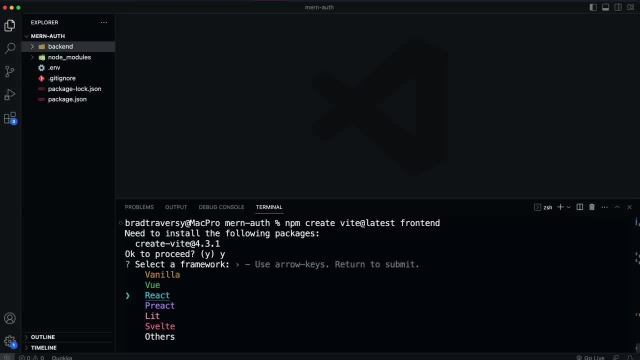 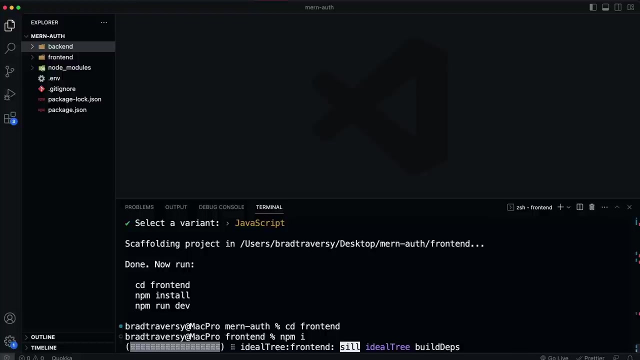 view, react pre-act, lit, svelte and others. i'm going to choose react and i'm not going to use typescript for this project, but you can if you want. so now what we need to do is cd into the front end and we have to install our dependencies. so npm install or npm i. now it's really important. 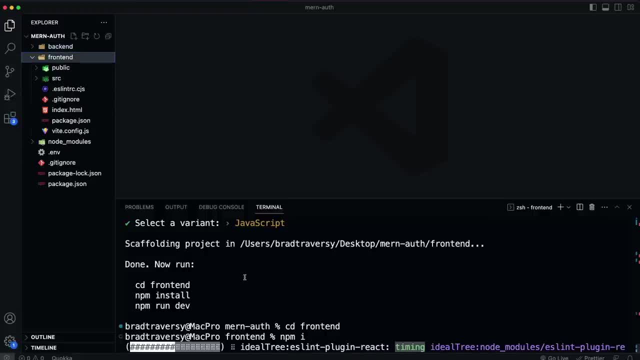 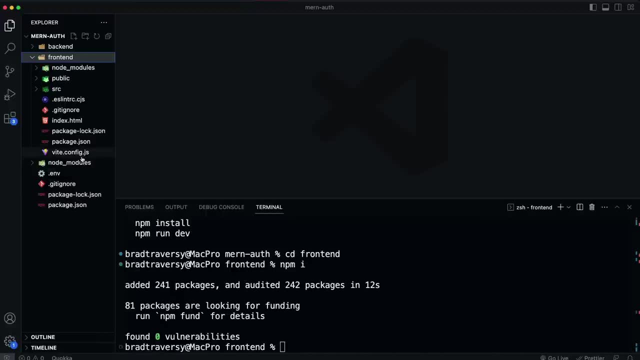 to know where you're at in the terminal when you're installing stuff like, for instance, we're going to use react router. you want to make sure you're not in the root because you don't want to install react router on your server. so what i would recommend is having one terminal open. i'm 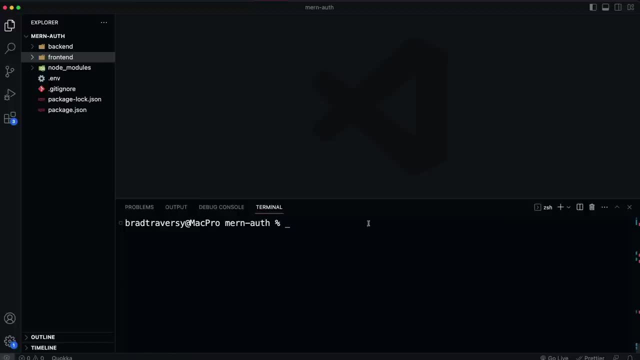 just going to go back to the root for this. so this terminal is open in the root and then i'm going to open up another bash terminal and actually i know i want zsh. i'm going to open up another z shell and then this one i'm going to cd into front end. okay, that way. 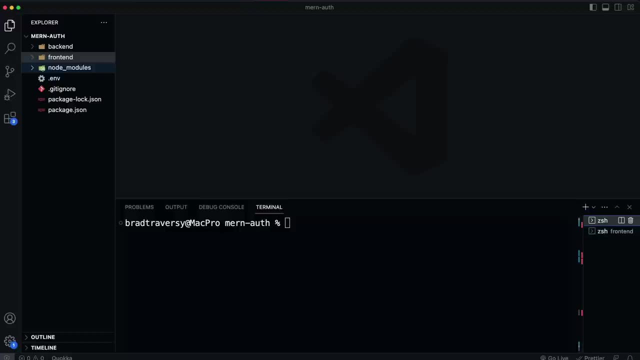 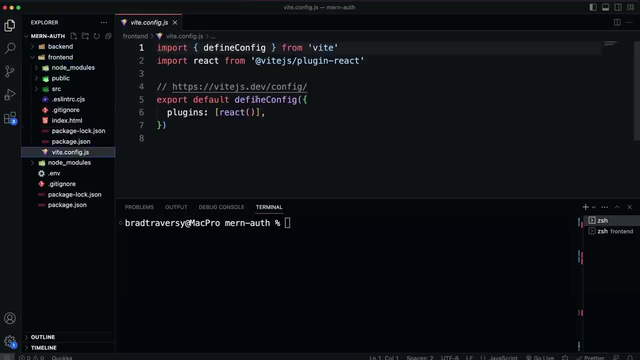 i have two terminals, one open in each. now, as far as veet goes, i'm going to do a little bit of customization, so i'm going to go in the config and basically, this is just: we're using the react plugin because we chose to use react, but i'm going to go under the plugins here and we're going to 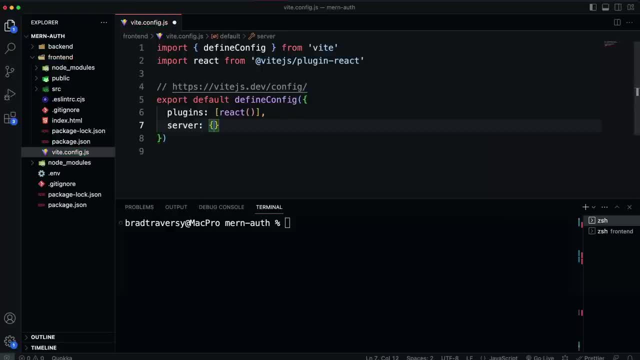 put in a server object and i'm going to set the port. the default, i believe, is like 5137. i like to set it to 3000. that's of course, that's optional, and then we're also going to add a proxy because our api is on. 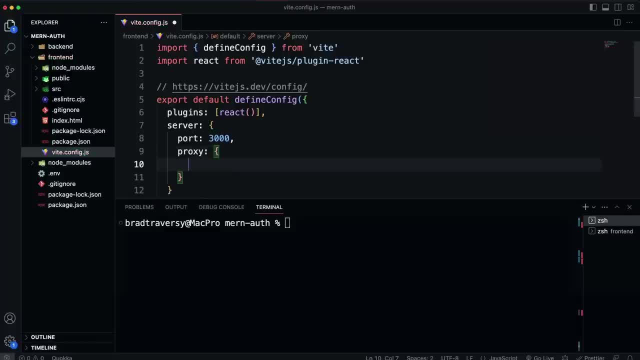 a different domain. it's on localhost 5000, where our dev server, our front-end server, is on localhost 3000. so when we make requests to our back end i don't want to have to put you know, hdp, localhost 5000. so we're going to add a proxy here saying that whenever we go to anything that 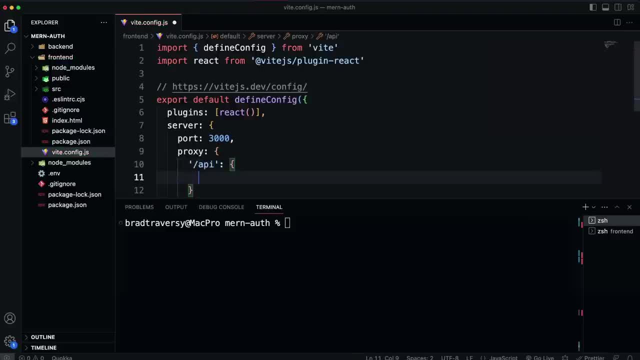 has slash api, then we'll open up an object here. then we're going to have a target and that target is going to be hdp, localhost, port 5000, which is our back-end server. okay, and then we're just going to add: change origin and set that to true. so this is the same as if you use create react app and you 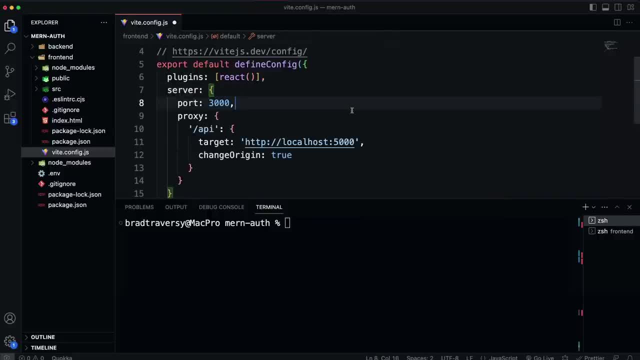 add a proxy in the package json file. okay, so if you're using create react app, then you're going to want to do that, so that should be it as far as config goes. now i want to be able to run the front-end reactor dev server from the root directory, so i'm going to go into my root packagejson where we have 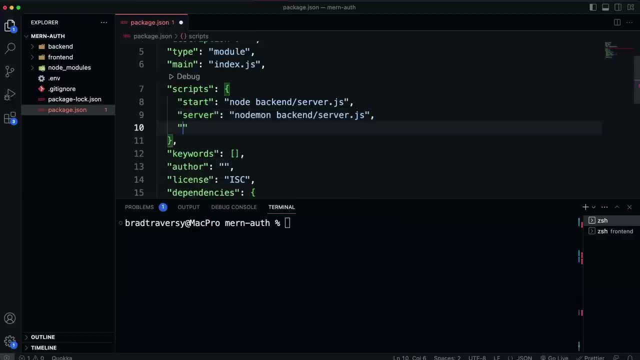 our start and server and let's add on to this a client script and what this is going to do is run a client script, and what this is going to do is run a client script and what this is going to do npm start. is it npm start? i think let's see front-end packagejson is 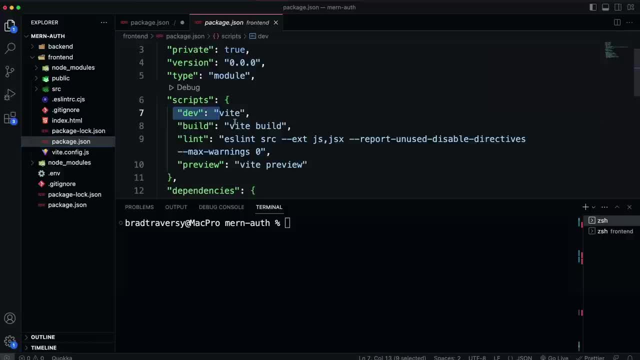 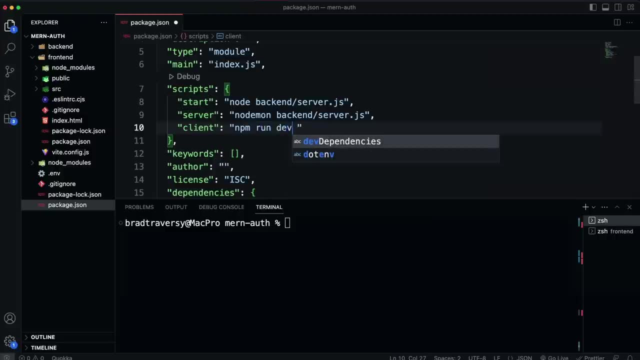 no, it's npm run dev, it's npm start if you're using create react app. so i want to do npm run dev and then just add the dash dash prefix and then front-end, because i want to run it in the front-end folder. all right, now, that will run the client. we can test that out, if we can go. 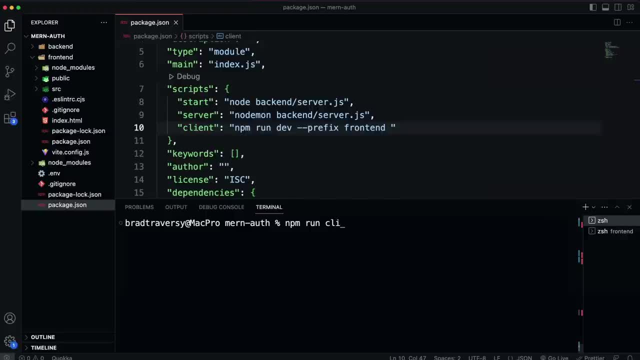 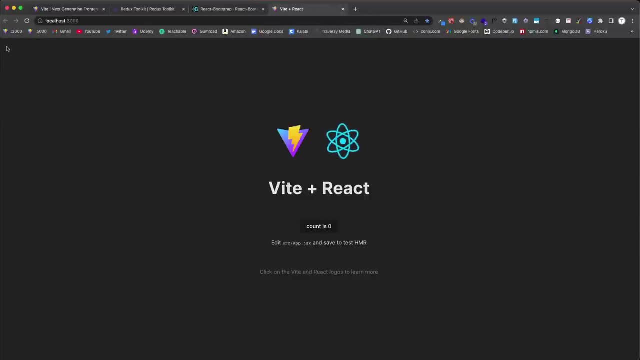 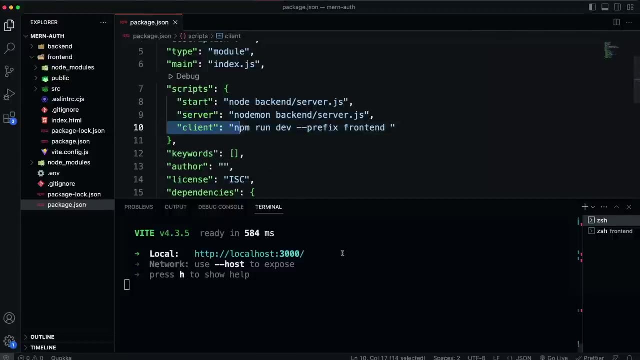 to the root and say npm run client. okay, so that runs on, opens up 3000. good. so so far so good. but i want to be able to run both the back-end and the front-end, so both of these scripts, without having to open up another terminal and run npm run server. so the way we can do that is with a 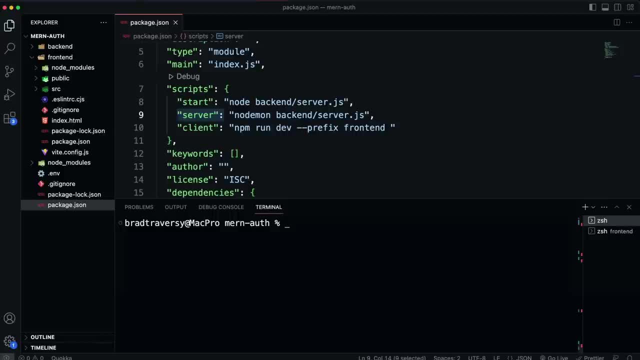 package called concurrently. so in the back-end here, or i should say in the root directory, let's install dash uppercase d concurrently, and that will allow us to run both scripts again. make sure this is in, not in the front end. you want to install concurrently in the server, in the root? all right. so now what we'll do is create another script. so let's put. 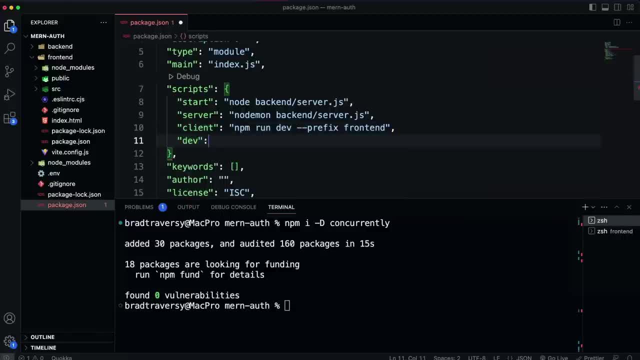 a comma here and i'm going to call this one dev. okay, because this is the main dev script. it's going to run both the client and server. so the way we do that is we say concurrently, and then i'm going to do slash, slash and then double quote: npm run. 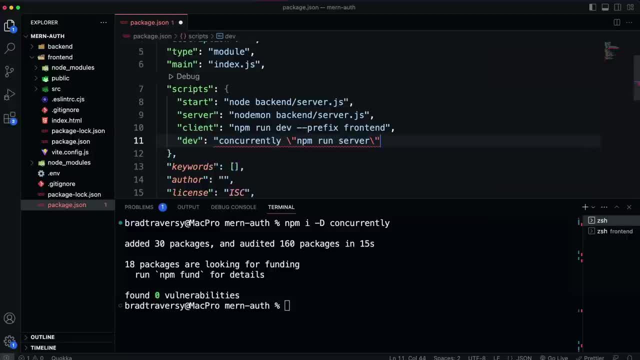 server and then slash- because i'm escaping the, the um double quote here- and then i'm going to do another slash, backslash and then double quote, and then npm run client and then another backslash double quote and then the final closing double quote. so this is going to run both of these. 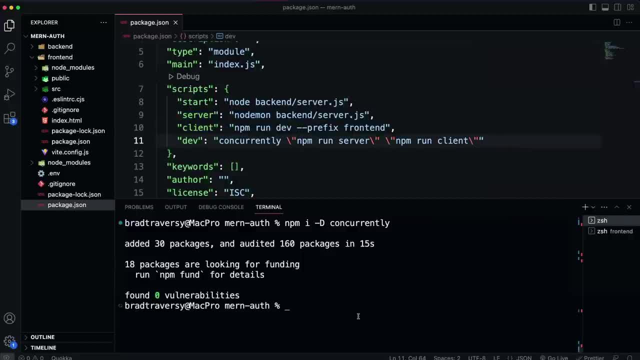 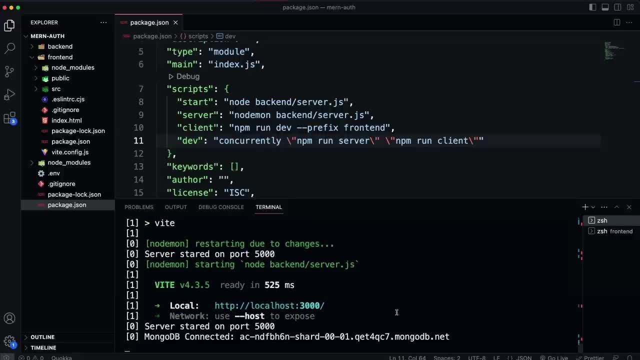 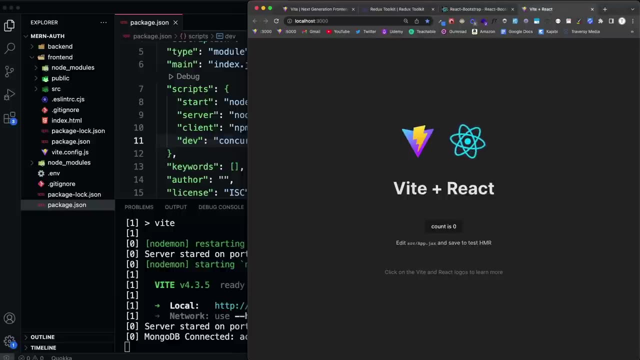 the front end and the back end. so now, when we want to run our development environment, we simply do npm, run dev, and you can see port 5000. the server is running and the front end is running. so i can go to 3000. that's our front end and i should still be able to go. um, let's see, we can try. go to postman. 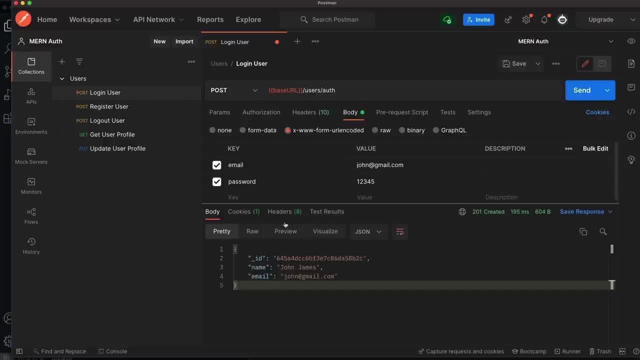 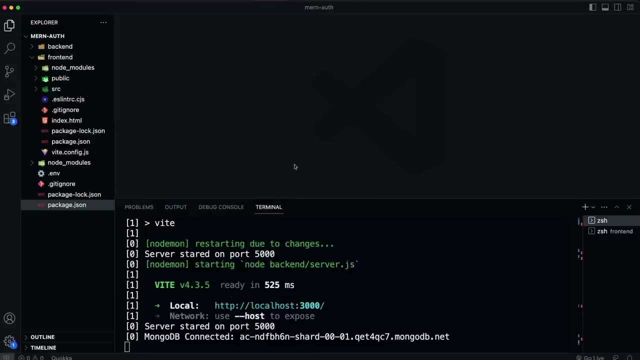 and i should still be able to- you know- authenticate and i should still be able to use the api here as well. all right, so now we'll start to do a little bit of cleanup. now with v there's not that much to clean up. so if we look in the source folder, this is obviously where all of our 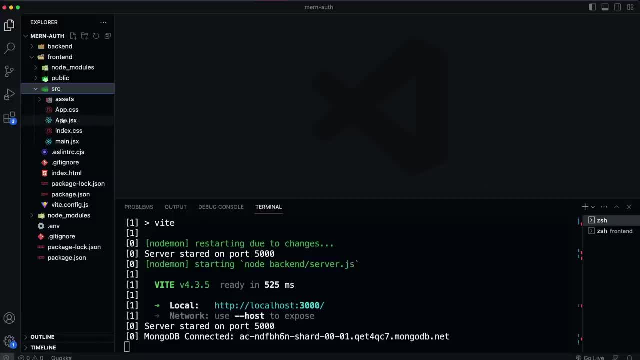 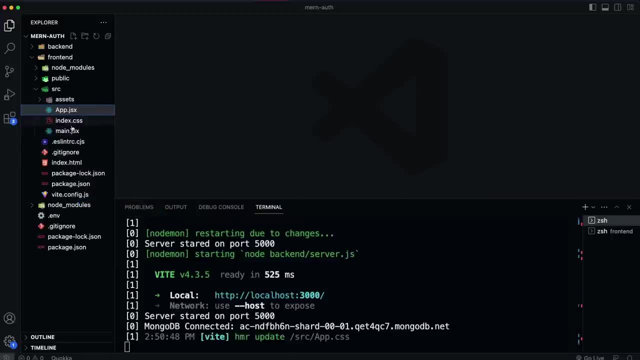 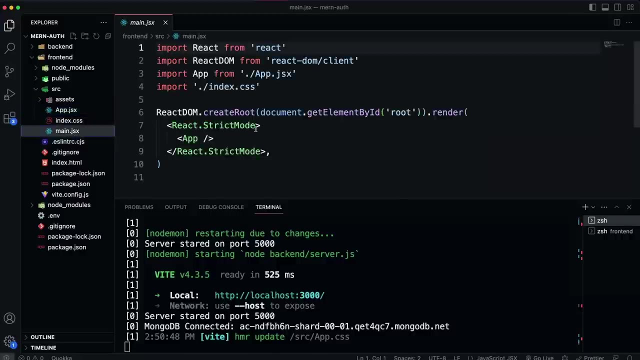 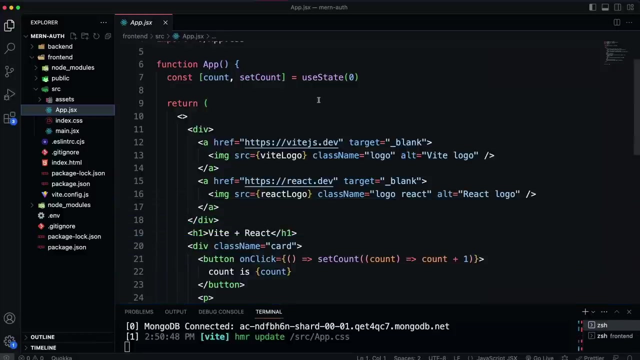 components and stuff go. all i'm going to get rid of is the app css, so we can get rid of that and we can go here into our. let's see, we have our main dot jsx and our app jsx. the main jsx we can leave alone, and then the app jsx, which is our main app component. all i'm going to do here is actually: 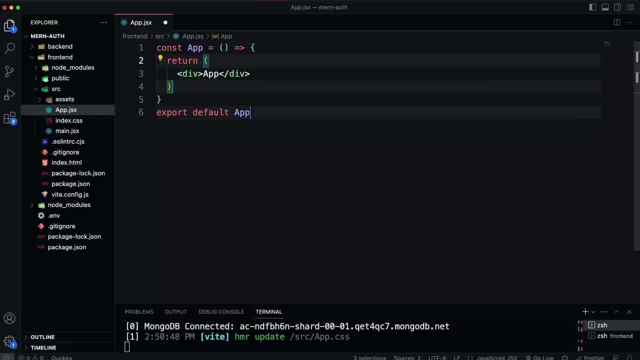 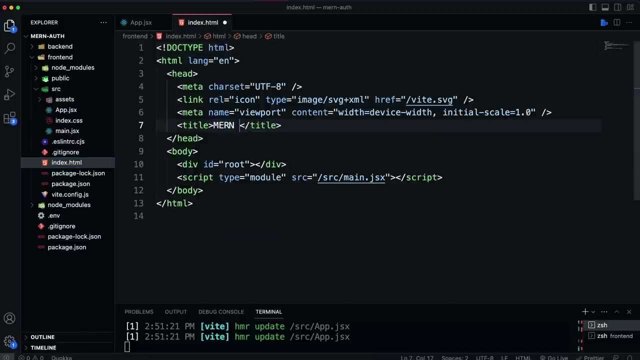 i'm going to get rid of everything and just do a simple arrow function component and we'll just have a fragment here and then an h1 and we'll just say, uh, i don't know. we'll just say my app. and then i also want to go into the indexhtml and just change the title here to murn off. 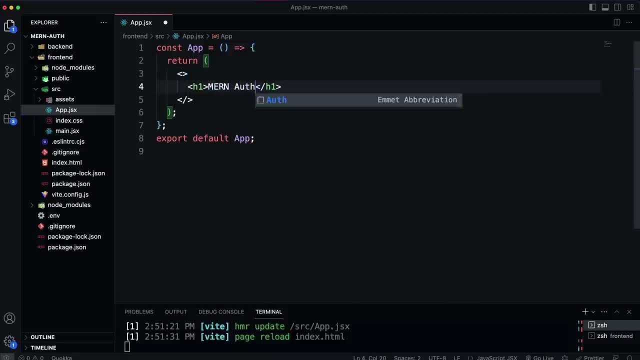 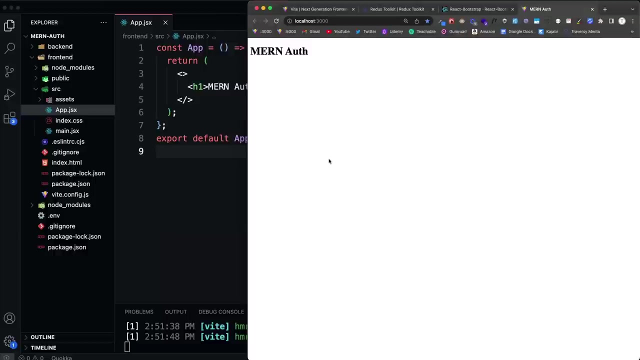 actually we'll just change this to murn off as well. so now, if we go back to our localhost 3000, we can see this. now we do have some CSS from this index CSS. I'm just gonna clear all that out, because we're gonna be using bootstrap. so clear that out and 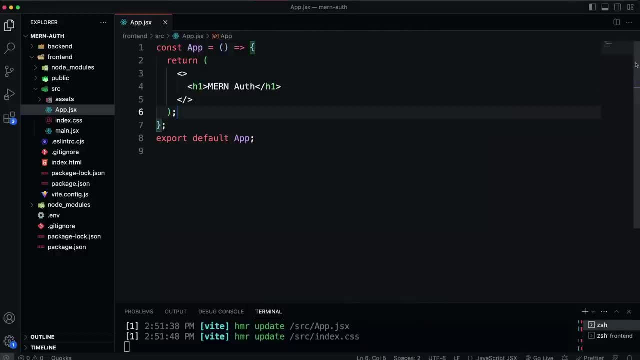 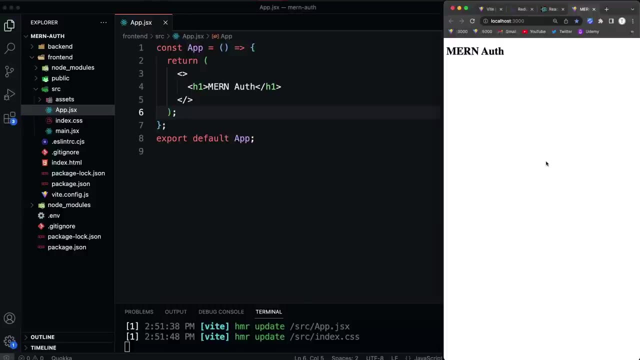 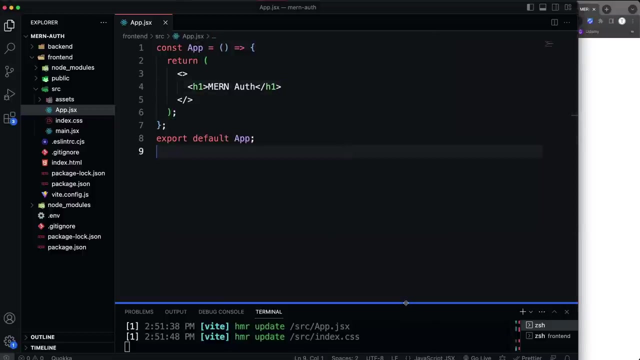 you should just see this for now, and we'll make this a little bit smaller. alright, so we now have just a brand new, clean front-end that we can start working on. now, as I said, we'll be using react bootstrap for the UI library and you want to make sure you install this in the front end, so this terminal, that's. 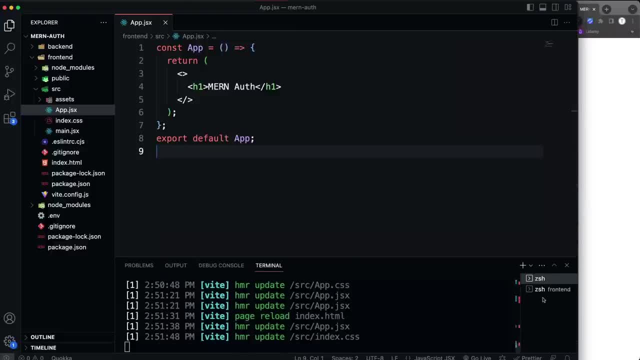 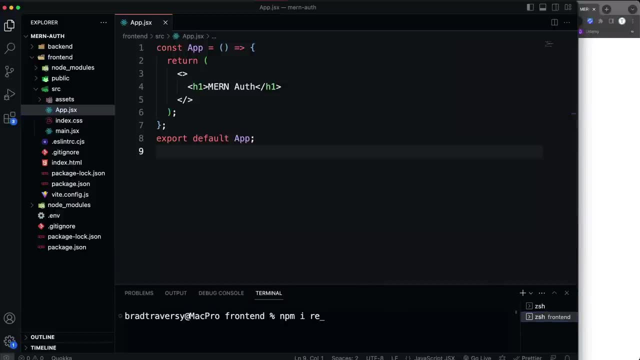 in the route. I have the server running npm, run dev. so I'm gonna let that keep running and I'm gonna go into my front end terminal now and from here I'm gonna say: npm, install react-bootstrap, and I'm also going to install react-icons so that we can use font awesome icons. so let's go ahead and install those again. 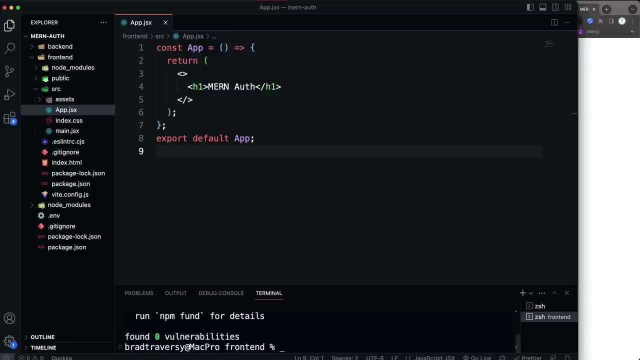 make sure you're in your front-end terminal and you want to make sure you You're using the present venk. traditionally, we're using a front-end right, so now all we'll do is set up bootstrap, which is pretty easy. we're just going to go into our front end entry point, which is maine dot JSX and 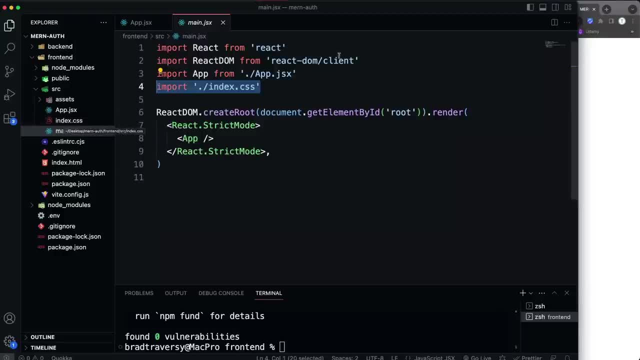 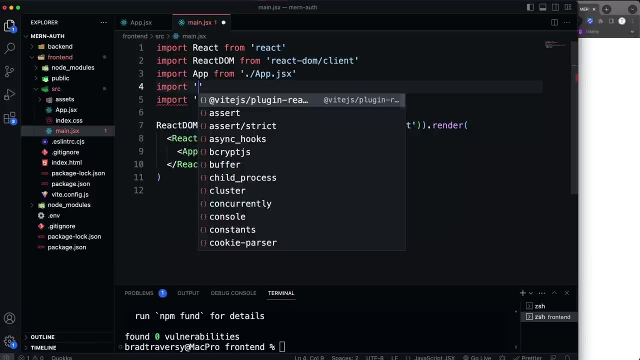 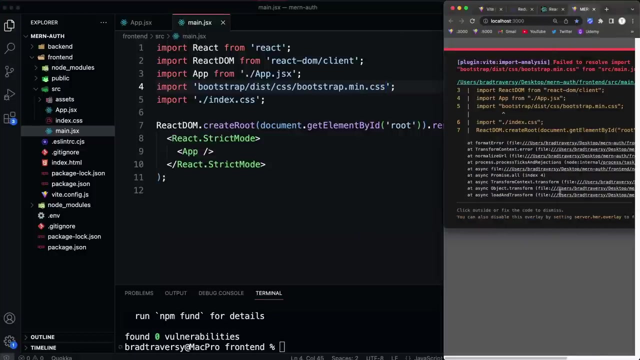 we're going to import the bootstrap CSS right now. we're importing our index CSS right here, which is completely empty. I don't want to delete it. just in case you want to, let's see. we want to import bootstrap slash- dist slash CSS, slash. bootstrap dot min dot CSS. so if I do that, let's see. there's an error here. 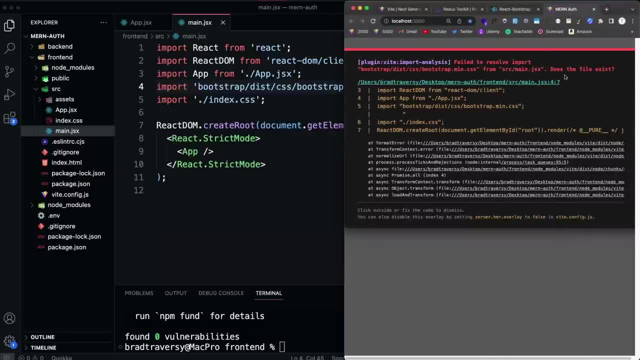 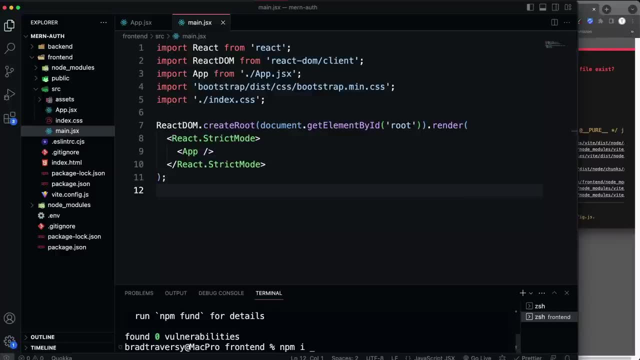 field to resolve import. does the file exists? oh yeah, we need. we need to install bootstrap as well. so when you install react bootstrap, you also need to install the actual bootstrap package. that should fix that, hopefully. so let's reload and there we go, and you can see that the fonts different, the margins, 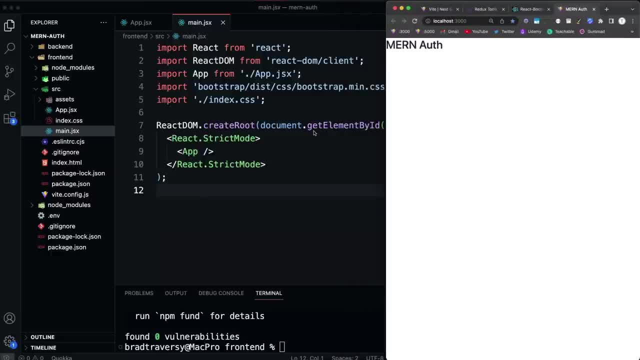 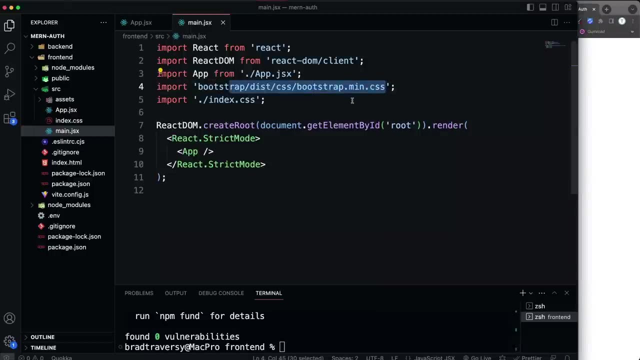 different. so bootstrap is now working. now you can create your own custom themes. I actually used a custom theme for the, the ecommerce course, but for this I'm just going to use the default styles, which is what this is you. but if you want to compile your own SAS and create a custom bootstrap file, where 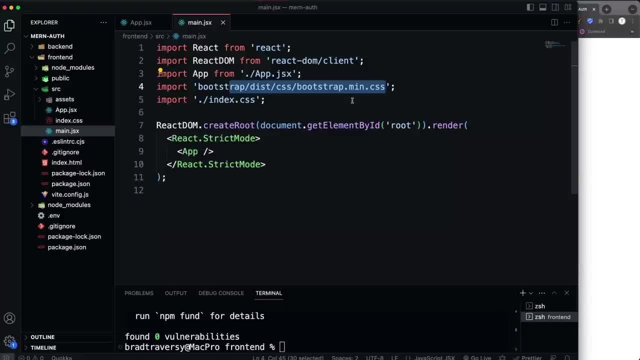 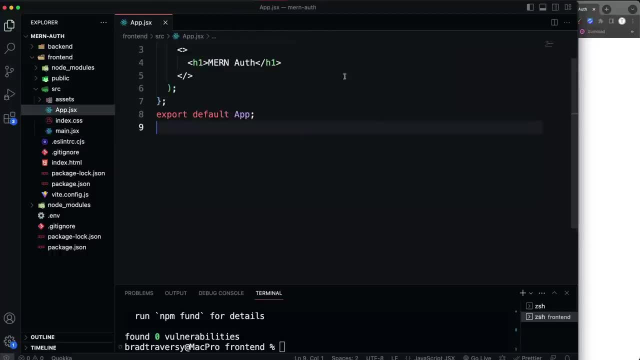 you have custom colors and all that. that's fine, but that's not the focus of this tutorial. so this is going to look very bootstrap II, but again, if you want to customize it, you can certainly do that. so the first component will create is our header, because that's pretty simple. so let's go into source and let's 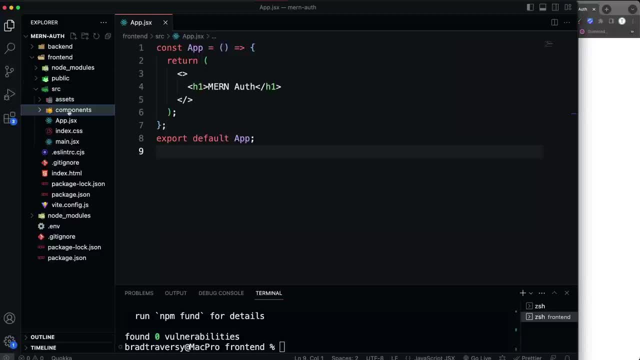 create a folder called components, and this is for any components that are not pages or screens. so let's create a new folder for our screens, but let's create in here a new file called headerjs X or J's, if you just want to use J's or T s or T s X, if 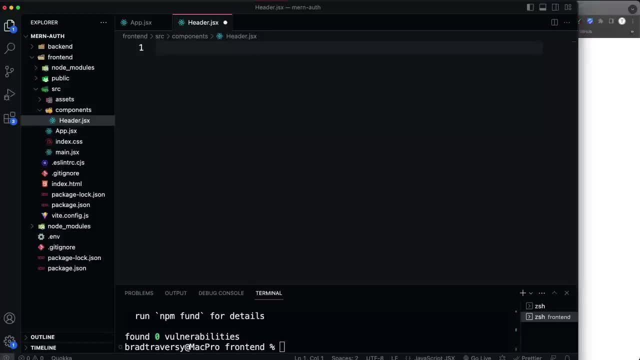 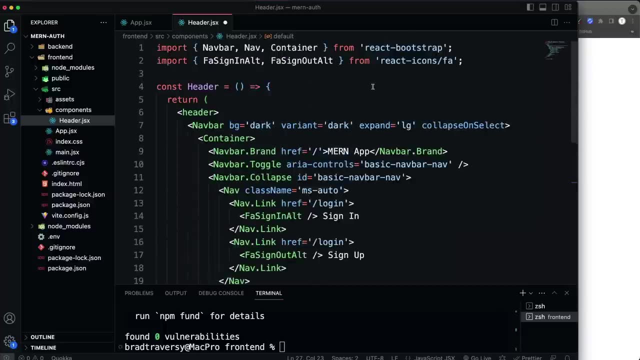 you're using typescript now for something like this, where it's just, it's just output. we're not really doing much here. I'm gonna paste in the J's X and just go over it. so basically we're just bringing in a few components from react. 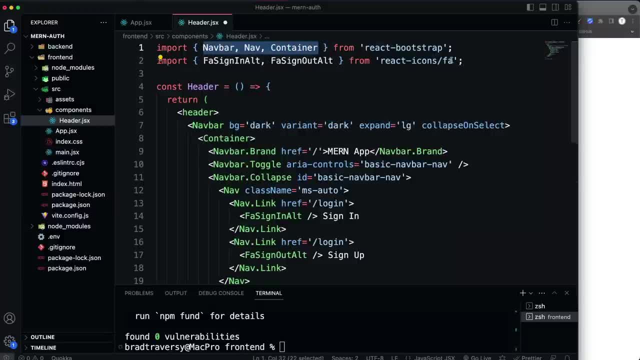 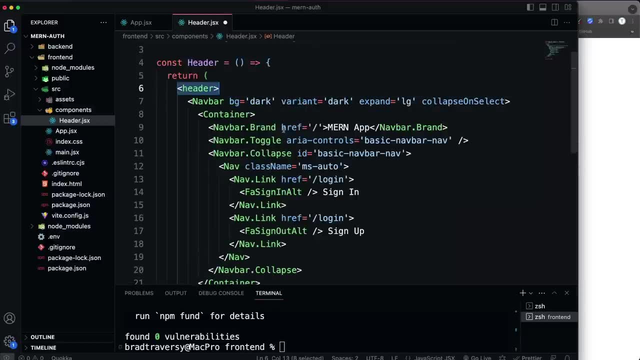 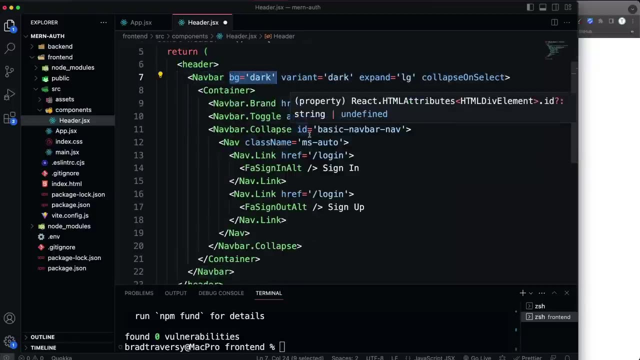 bootstrap the nav bar, nav and container, and then a couple icons for the sign in and sign out links, and then in the header component where we have an html5 header, and then in that we have our nav bar and you can pass in different props. like i want this to be dark, so i'm doing bg dark. 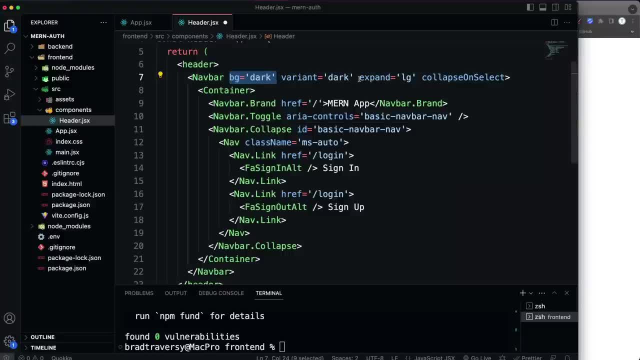 and variant dark expand is basically where you want the hamburger menu to kick in. so i'm saying on large screens and then in the container here we just have the nav bar brand, which is kind of the logo i'm actually going to do. mern off, but of course you can put whatever you want there. 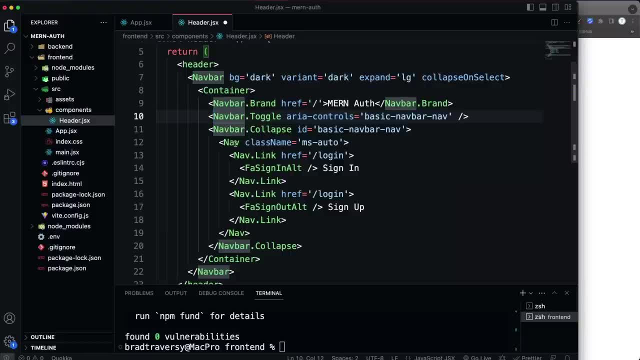 and then we just have our nav bar toggle and collapse because we are using the hamburger menu and then the nav with the nav links which we have login. this should actually go to register. so we have log in and slash register. just have sign in and sign up for the text along with the icons, so you can just copy this and you. 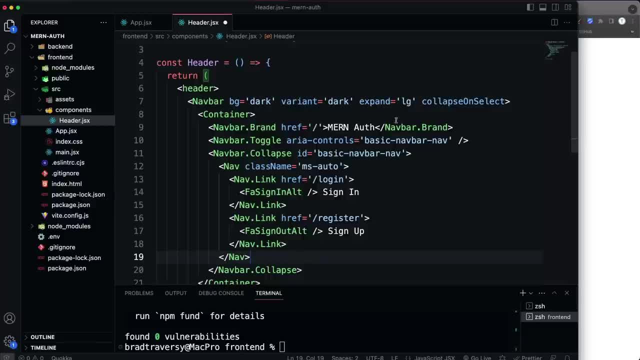 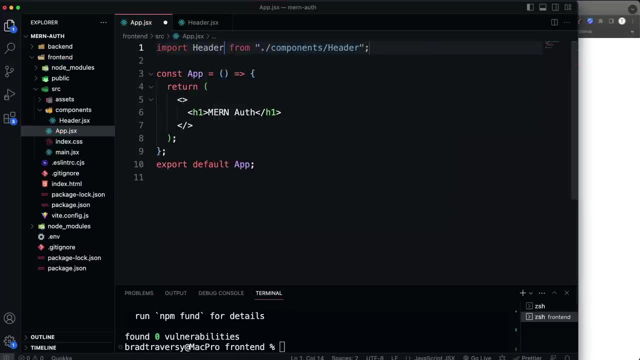 can copy it from the repository. well, actually the repository will have other you know the code, the final code, but you can copy it from the blog post. I'll have those in the description as well, so I'm gonna save that and then let's bring it into our app component. so in here we're gonna import the header and I'm gonna 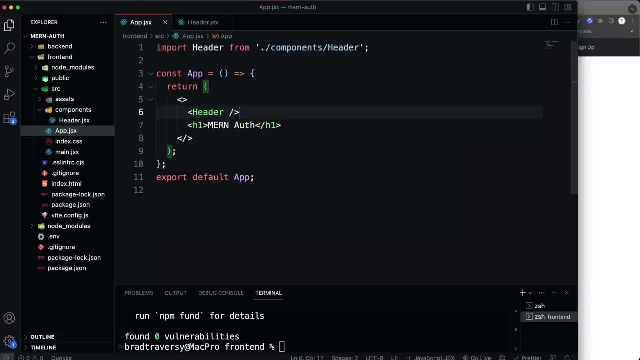 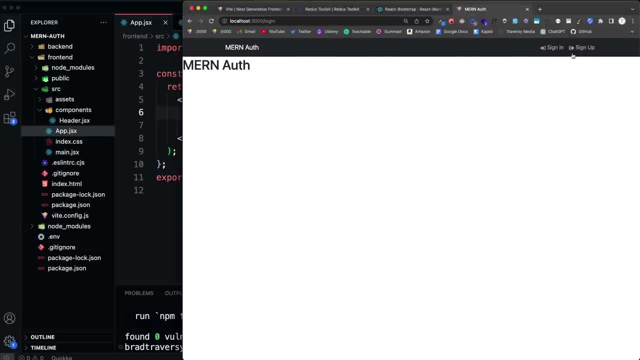 put it right above the h1. so now if we take a look you can see we have our header here. our navbar sign-in goes to slash login, which obviously these aren't gonna. you know it's not doing much because we don't have those routes yet. 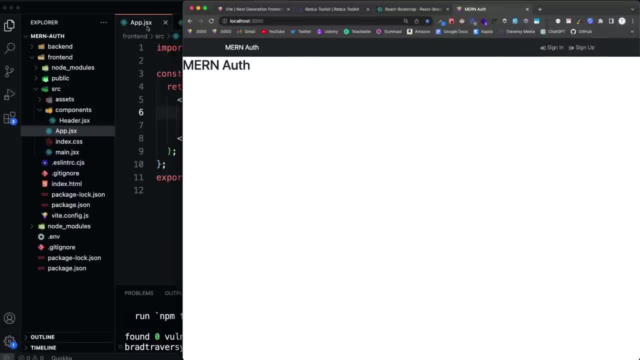 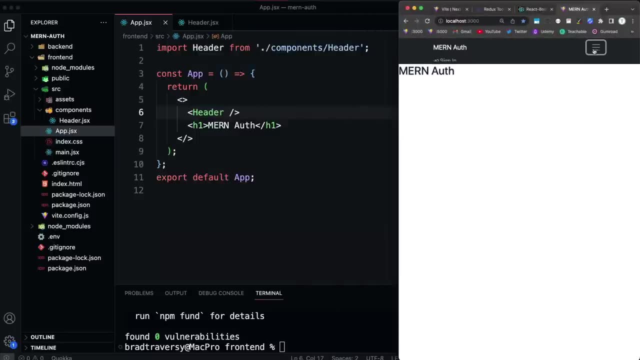 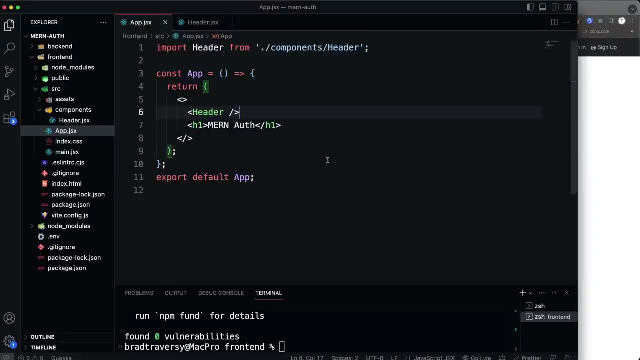 we don't even have the router installed, but at least we have the navbar there, and again, it looks very bootstrap II. but if you want to add your own custom theme, you can do that. we do have the hamburger menu working as well. okay, so the next thing I want to do is we want to do the want to get the router. 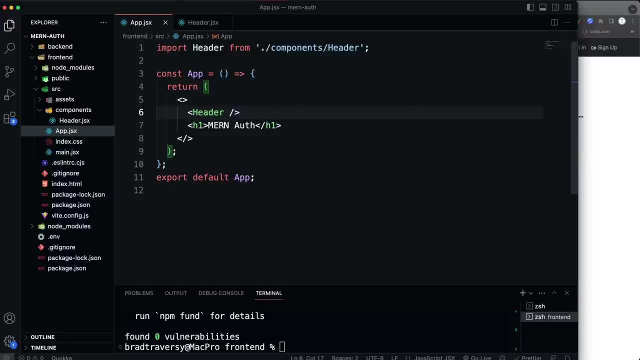 set up. but let's create the home screen first, which is just basically the landing page. so in the source folder in the front end, let's create a new folder called screens, and in here we're gonna have a new file called home screen. dot JSX and I'm using the es7 react redux snippets extension. so I'll just say are. 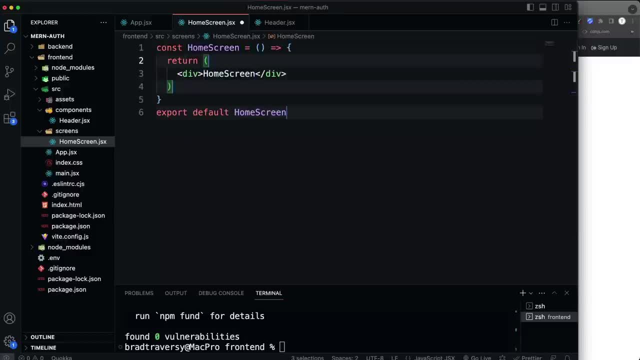 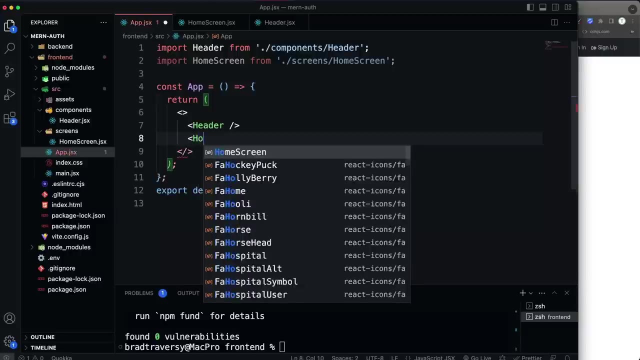 a FCE which will create an arrow function component. and just for now, I'm gonna save this and bring it into the app folder. I'm sorry, app file. so import home screen and we'll replace the h1 with home screen, and we should just see that. 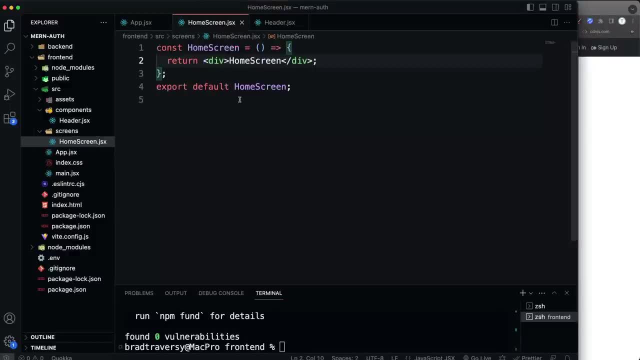 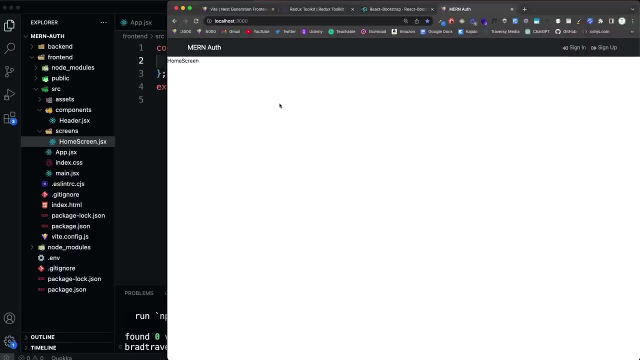 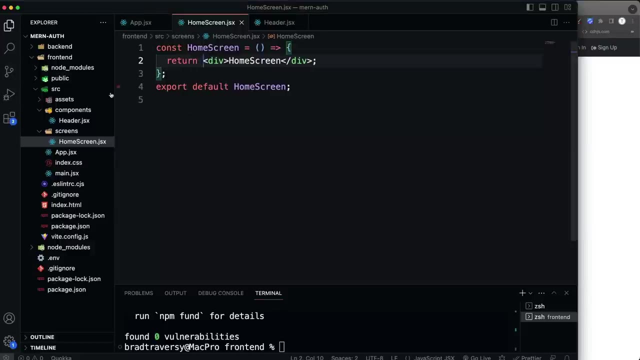 the text home screen there. so in here, what I want to do is just render a component, a hero component, just a, you know, an area, a showcase area with some text and also some buttons to the sign-in and sign up page. so I could put it directly in the home screen, but I'm 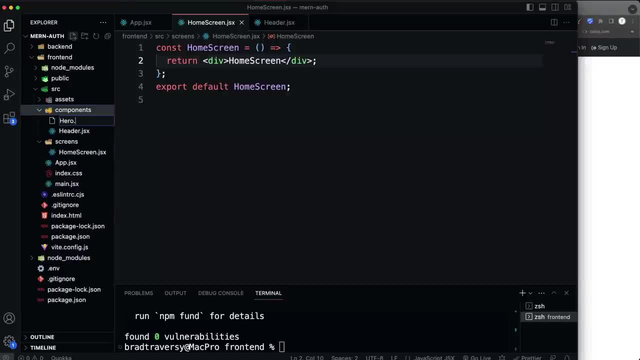 going to choose to put it into a component called hero jsx. so let's create that, and for this, I think I'm just gonna paste this in is what and as well, and just go over it. so again, we're just bringing in some stuff from react. 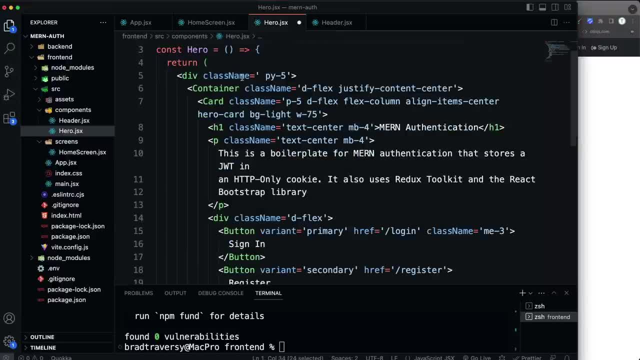 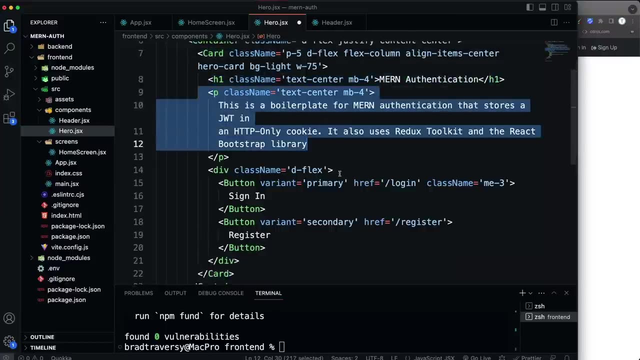 bootstrap, container, card and button, and we have some class names like py5 is just padding on the y-axis, so basically top and bottom, and then we have a container, we have a card in that container with an h1 paragraph and then we have the sign in and register buttons. let's say sign up, sign in and 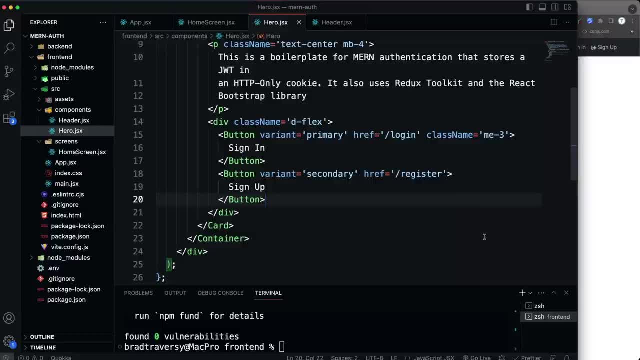 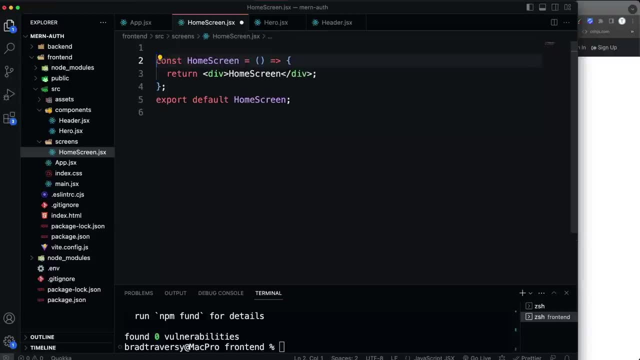 sign up. i mean, it doesn't really matter, this page is really irrelevant to what we're doing, but i just wanted to have something here, so let's save that and then in the home screen we'll go ahead and bring in that hero component and then let's show that we could even get rid of this div. 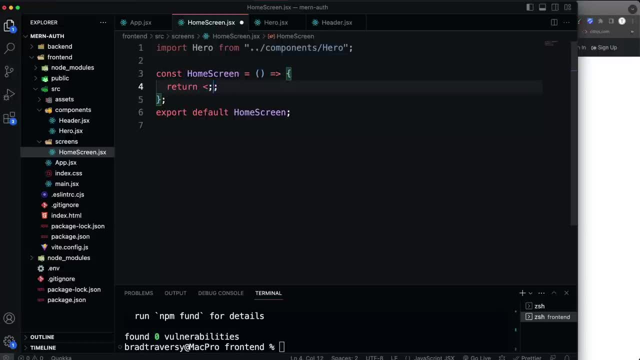 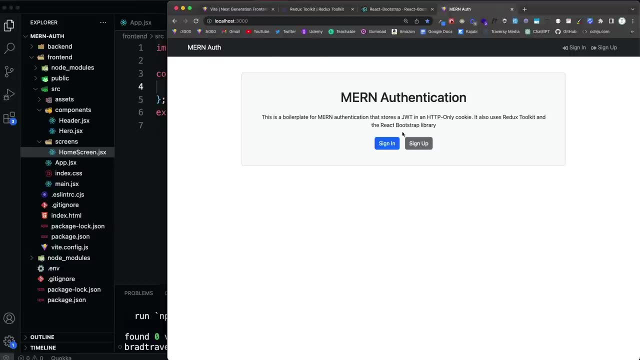 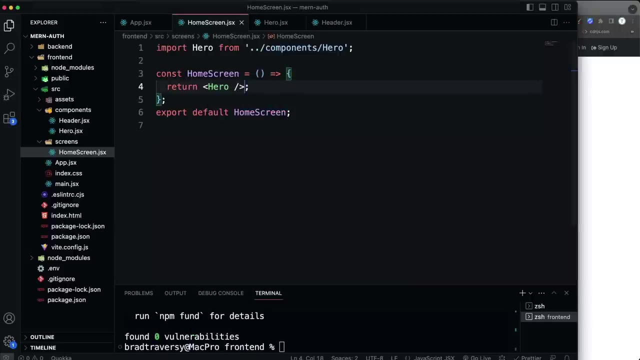 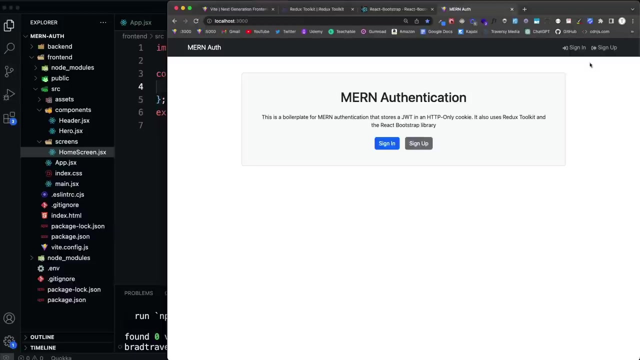 we could just return the hero component, okay, so there we go. we just have this little box sign in, sign up. all right, good, so now. now what we can do is start working on the router, because obviously we have different pages we want, or different screens we want to be able to go to, like sign in, sign up profile. so let's install the 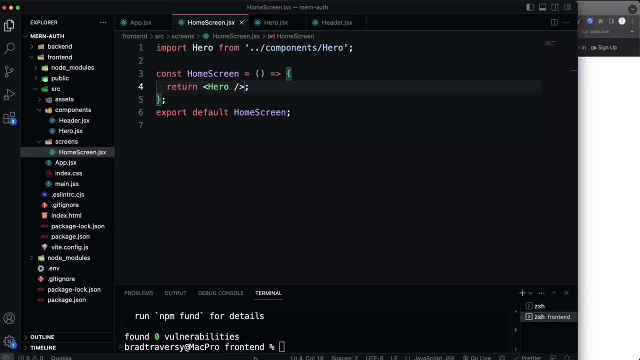 router. now again, make sure you're in your front end. you don't want to install the react router on in your express server, so make sure you're in the front end. let's npm install react dash router, dash dom. now there's also another package that we're going to want to install. 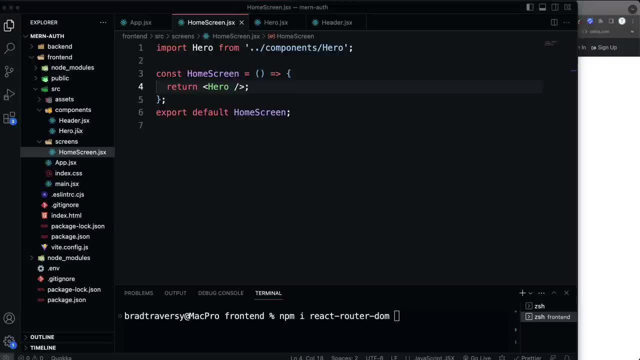 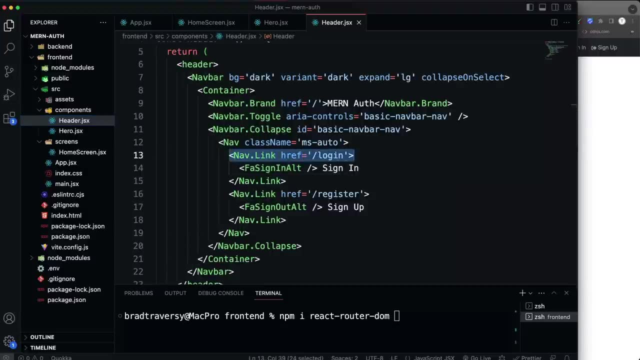 because we're using react bootstrap and with the nav in the header right we have this nav link. so if we want to use the link component along with this nav link, then we need to install, we need to use something called the link container and that's part of a package called react router. 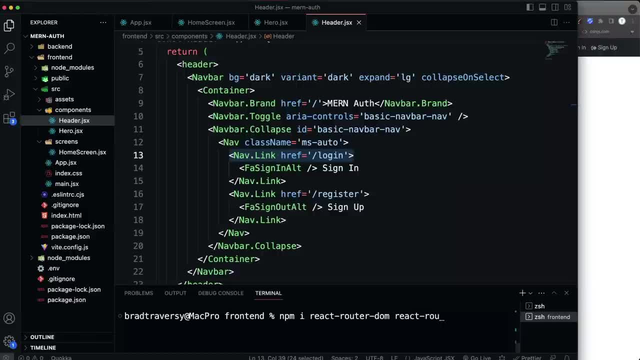 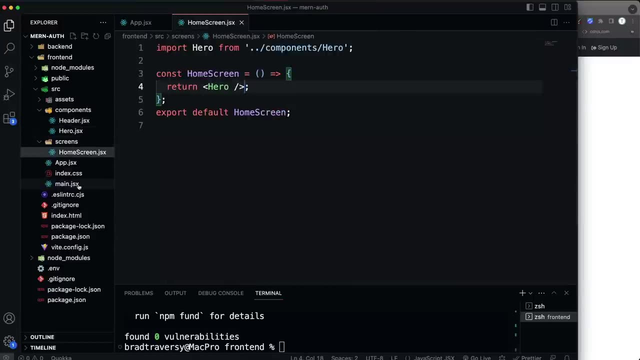 bootstrap. so we're also going to install react dash router dash bootstrap. so let's go ahead and get those installed and we're going to go. we're going to set up our router first and we're going to do that in the, the entry point, which is 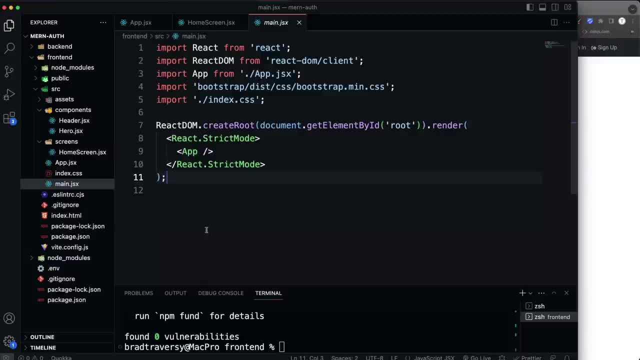 mainjsx. now, if you're using create react app, your entry point is called indexjsx, so you would go to that file. now there's a few things we're going to bring in from react router dom. so let's say import and open up some curlers. 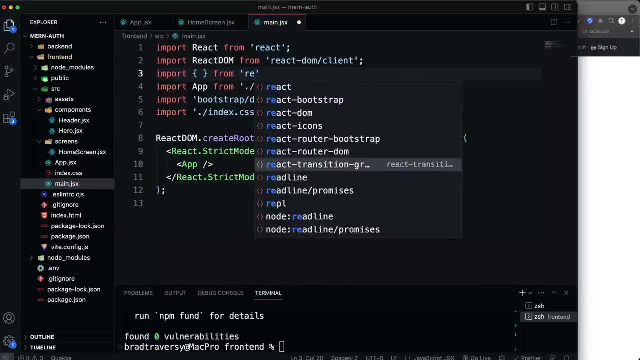 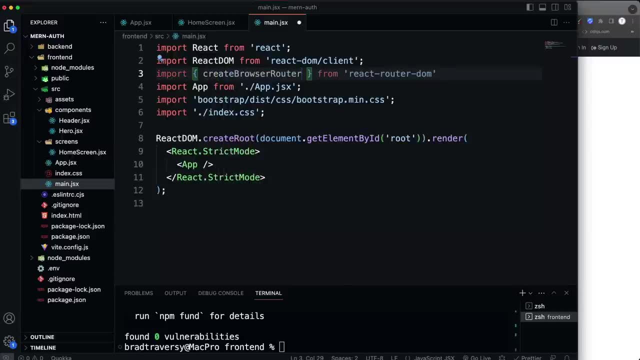 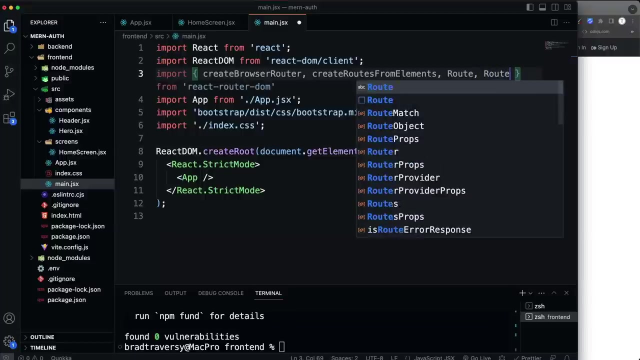 and it's going to be from react router, dom. so there's four things we want to bring in. the first is create browser router, and the next is: create what is it? create routes from elements. and then we want to bring in, of course, the route component and then the router provider. so, router provider. 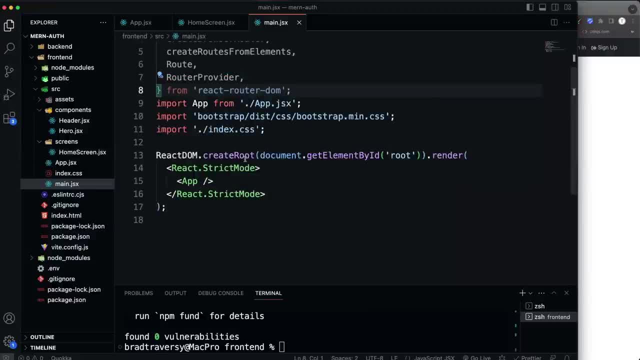 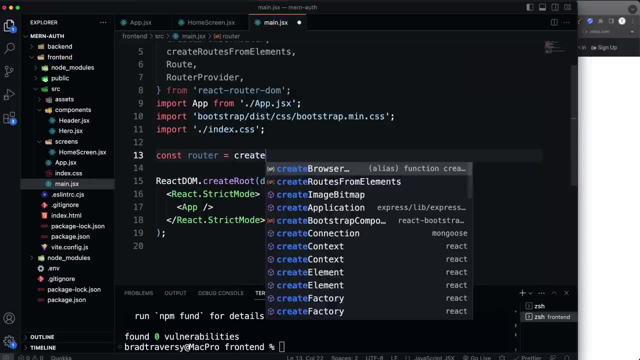 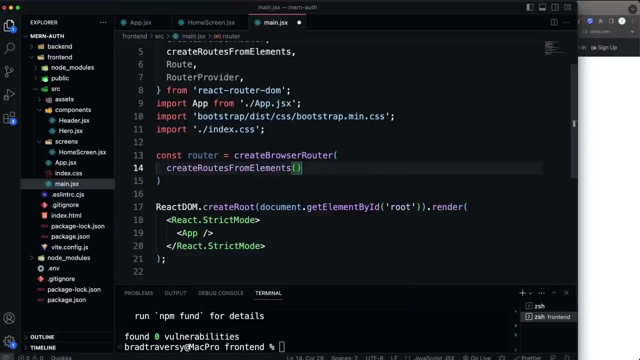 so those are the four things we want and then create our router. let's come down here and we'll say const router and we're going to set that to create browser router which is then going to take in the create routes from elements and then inside that, 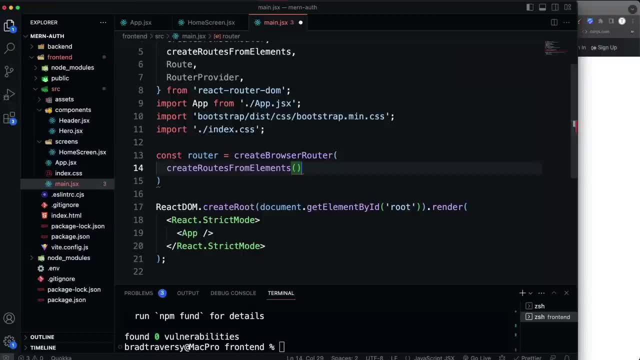 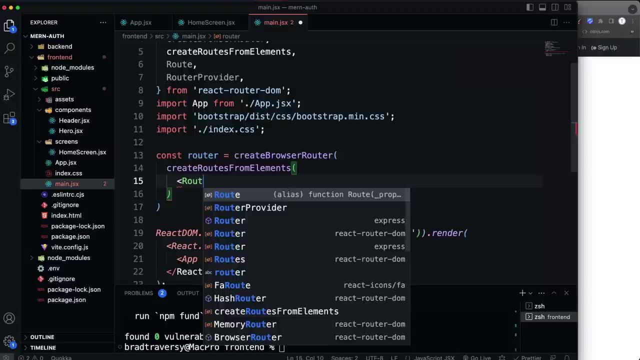 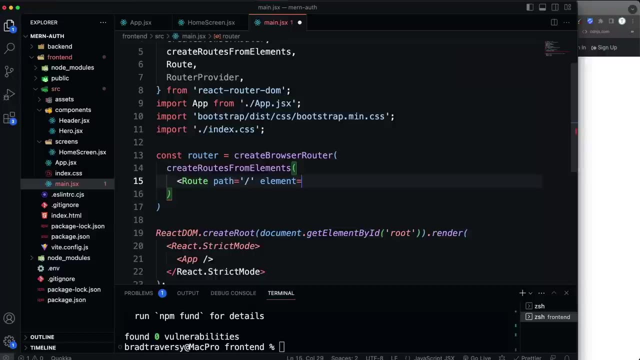 actually we don't want that there. so inside that, create routes or create routes from elements, we're going to have our route component with a path of slash and then the element is gonna be the app element. so in curly braces we're gonna put in app and make sure you put in your angle brackets and all that. and 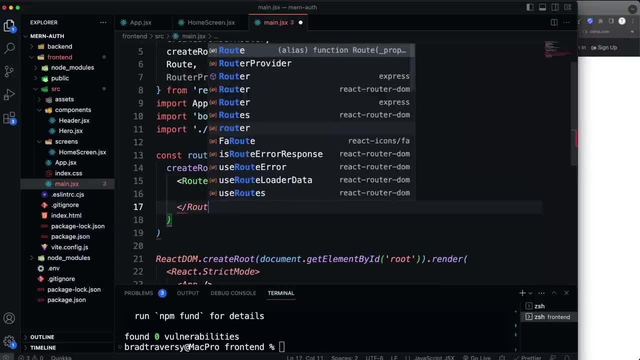 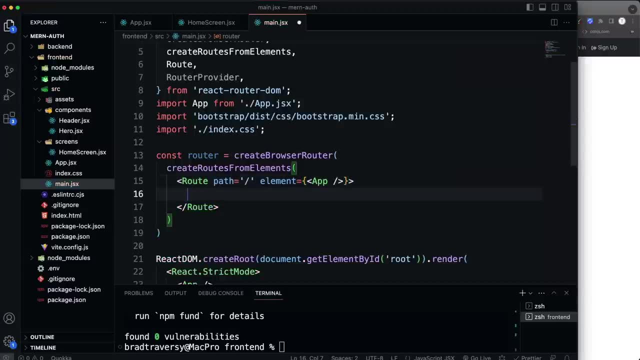 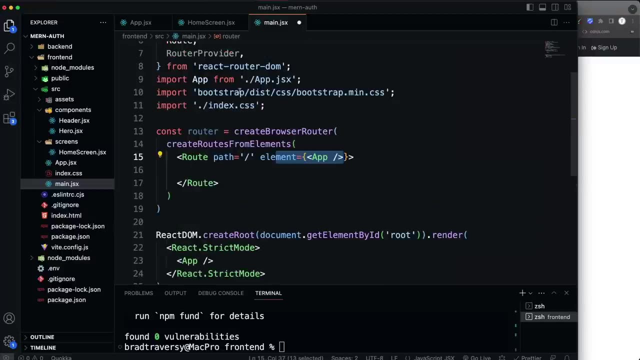 then we're gonna close that route. let's close this as well. now, every, every route we create now is gonna go in here, because it's gonna be a child of this route, which has the element of our main app component, which is being brought in here now. since we're putting the app component here, we don't want it down. 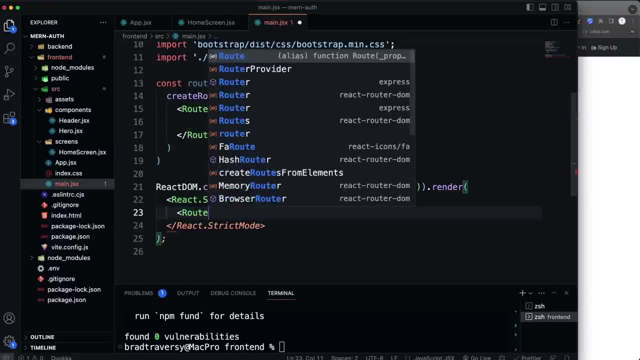 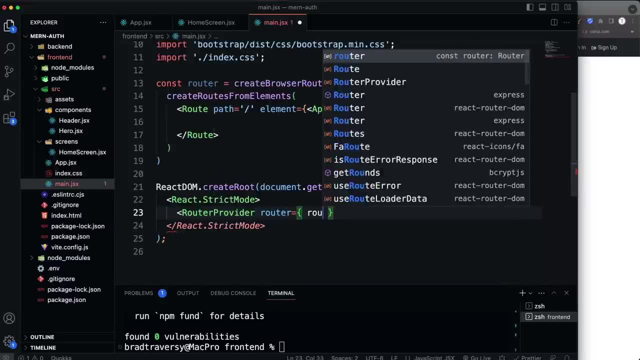 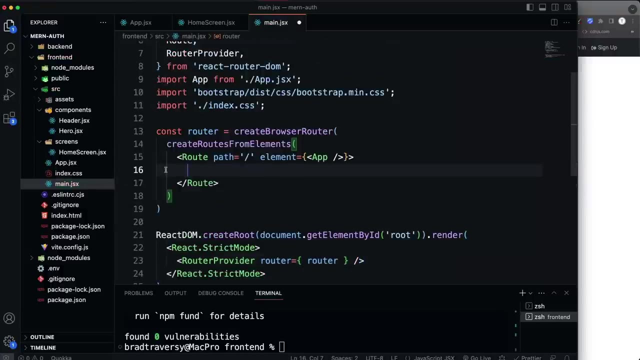 here. instead we want to put the router provider. so here we say router provider, and then we can pass in router equals and set that to our router variable above, which has all of our routes. okay, now, the only route we're gonna have at the moment is the home screen. so let's import home screen and then we're gonna. 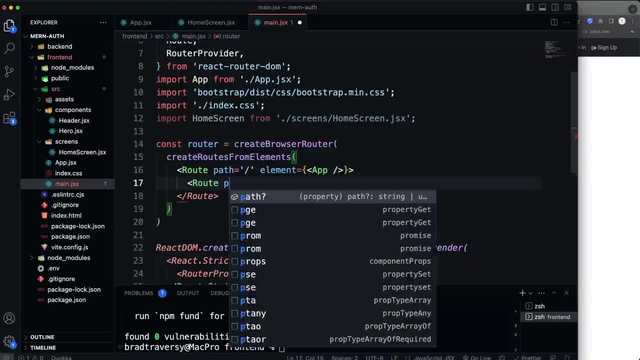 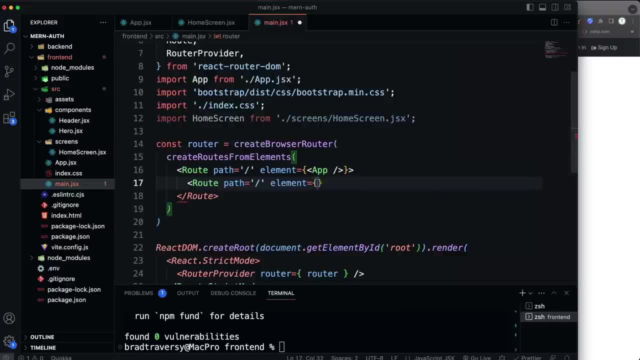 go in here and add that, so let's import home screen. and then we're gonna go in here and add that, so we'll say route, path, and this is still gonna be: just slash the index and then, as far as the element, it's gonna be the home screen. now, just make sure you don't 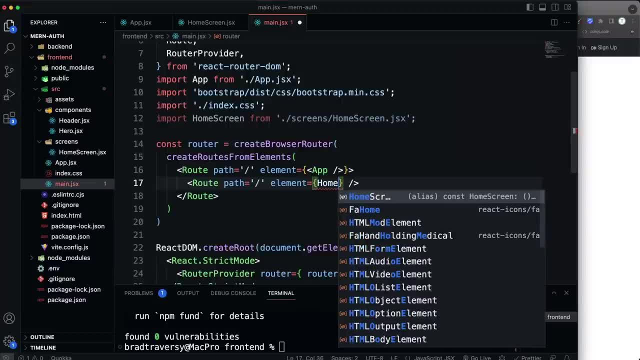 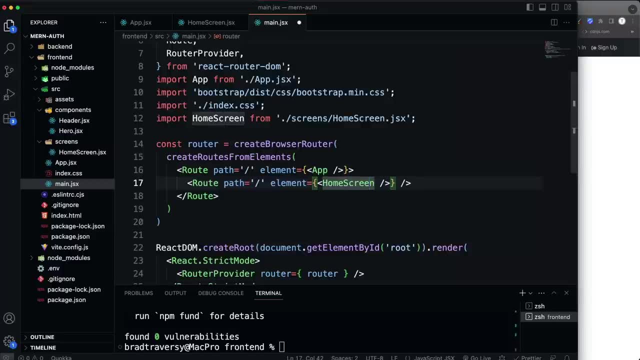 do this. where you just put you know home screen, you have to have your angle brackets as well, because it has to be the actual component being embedded, just like we did with the app component. now, since this is the home page or the index page, we're gonna put index equals. 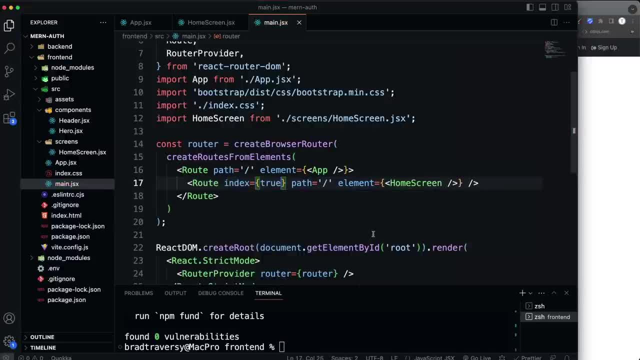 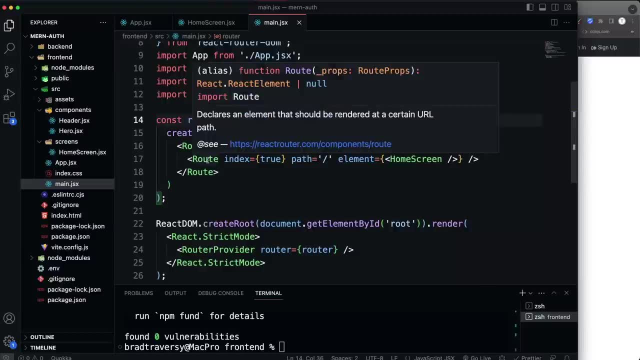 true, okay, so we want to add that, and then any other routes we create, like our login screen, register screen, will go in here, just like this home screen. now, to render whatever, whatever path we're on, whatever screen we're on, we need to go into our appjsx, because right now we're just showing the home screen, no matter. 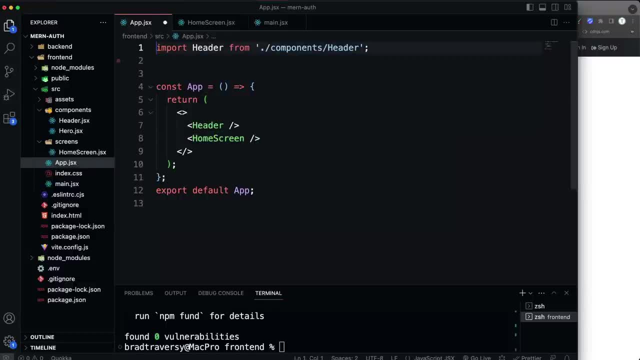 what? so we can actually get rid of the home screen and we want to import the outlet. so we're gonna say: import home screen and then we're gonna save just a outlet from React or DOM and then we can replace. we can come down here and replace that with. 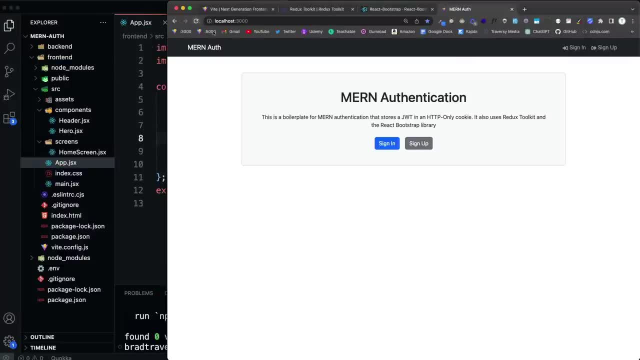 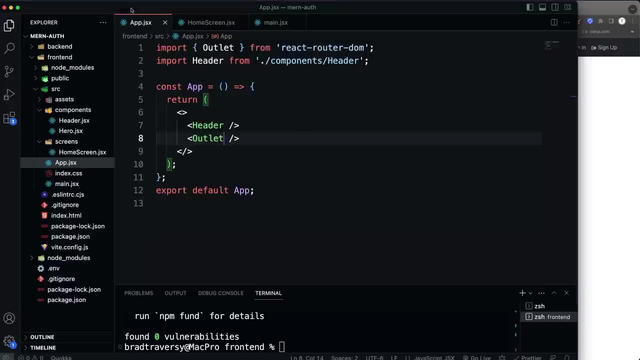 outlet and for now we should see the same exact thing, because we're still seeing the home screen. that's the only, you know, the only route we have. one thing I'm going to do is just wrap a container around the outlet, so I'm going to bring that in from react bootstrap, so let's say, import. 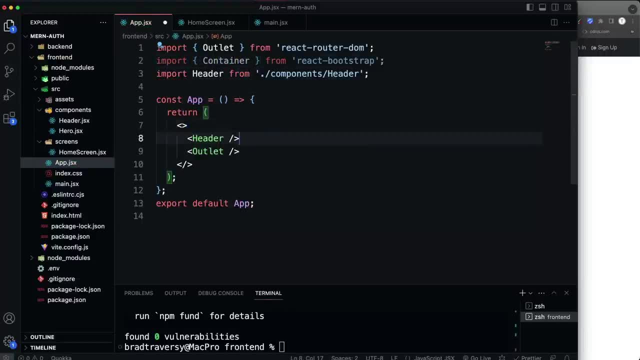 container from react bootstrap, and then I'm going to go under the header and say container and I'm going to give it a class name of my. so just margin on the y-axis of two, and then I'm going to move the outlet into there. all right, cool, now before we move. 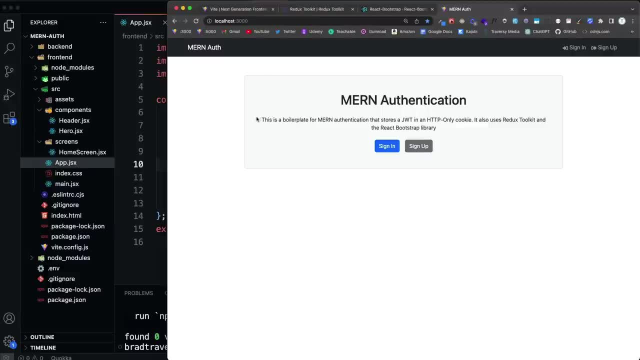 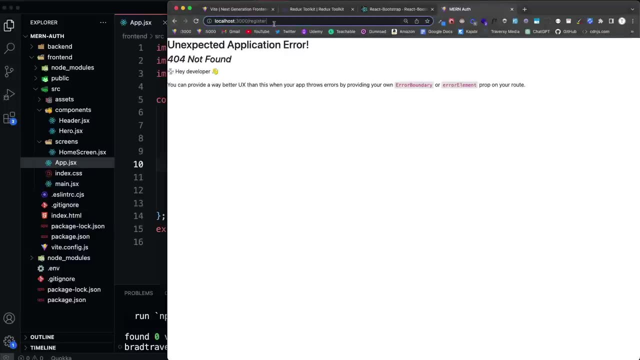 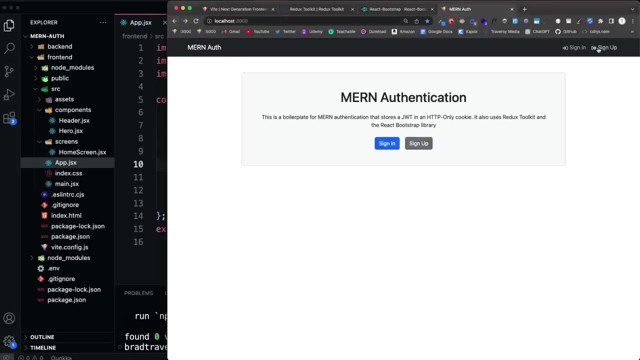 any further. as far as screens and moving to the login and all that, we want to fix it so that these links up here aren't using href. I mean, obviously these, these routes aren't going to work right now, but you can see that when we click you get the little refresh, little spinner in the in the tab, because 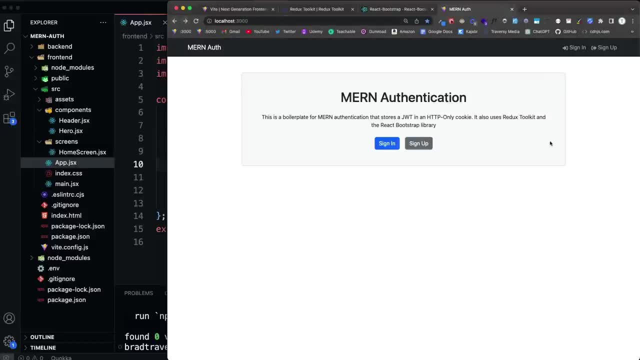 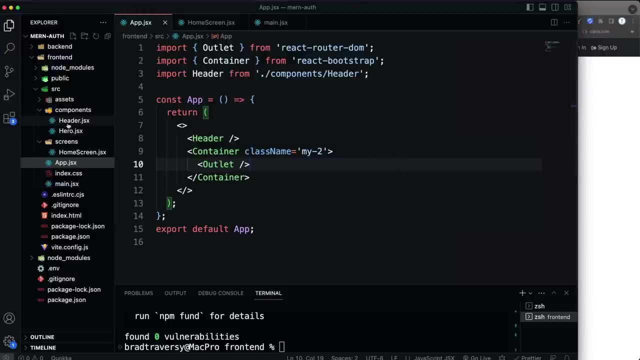 it's, it's going to a different page. well, we don't want to do that because we have a single page application. all of the routes are embedded in our javascript, all the pages and screens are in our javascript. so we want to use the link component from react router DOM and if we're using in the 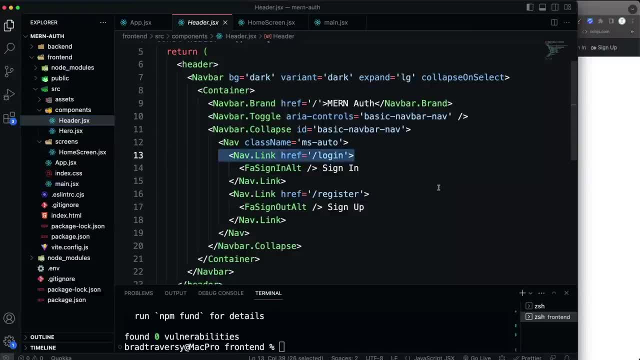 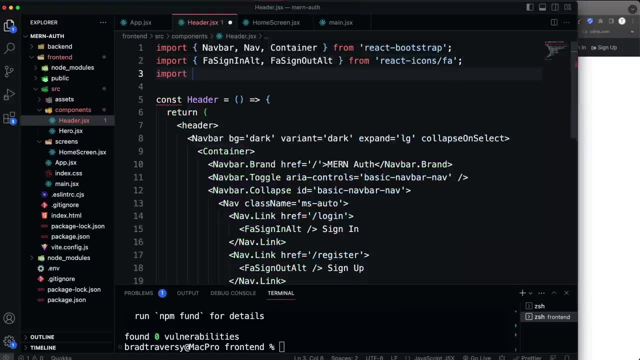 header. if we're using these nav links, then we want to use the link container from react router bootstrap. so let's go to the header and let's import. we want to import the link container and that's going to be from react router bootstrap. now, the way this works is wherever we want to have. 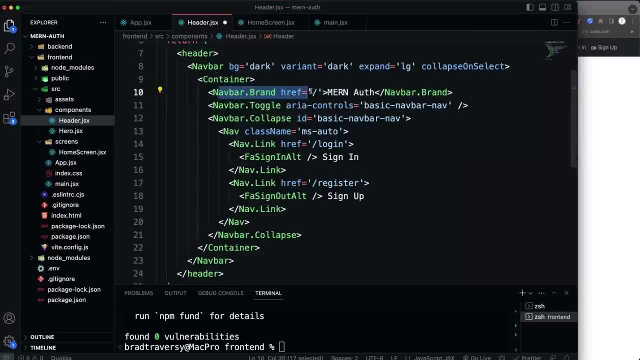 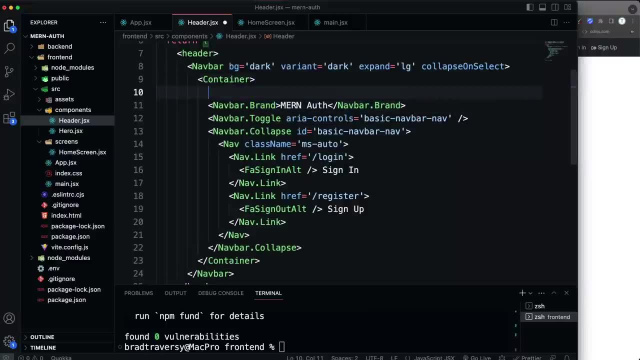 a link like, let's say: right here we have the navbar brand. we want that to go to the home home screen or home page. so we'll get rid of the href and we're just going to wrap this in the link container and that's going to have a to attribute instead of a href. so we'll say to: 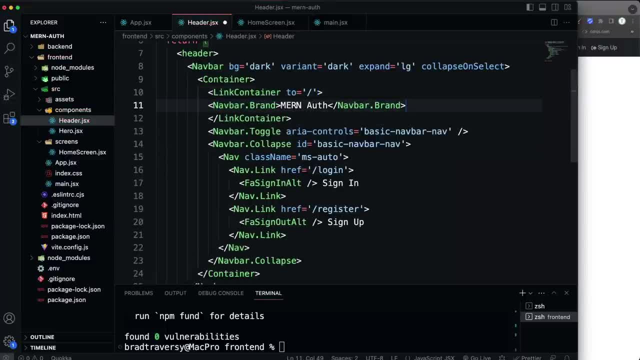 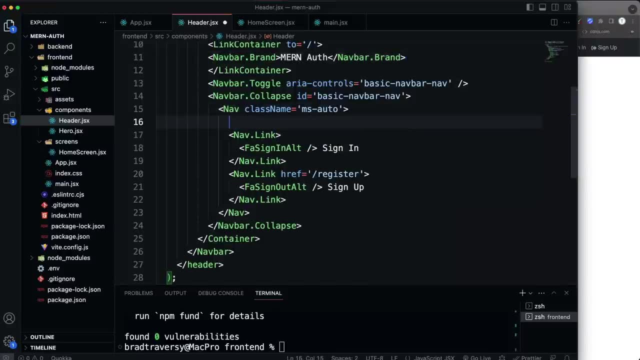 slash and then we'll move the brand into that and then we'll do the same thing down here. so instead of having the href on these nav links, we'll get rid of that and we're going to wrap the whole nav link with the link container you. 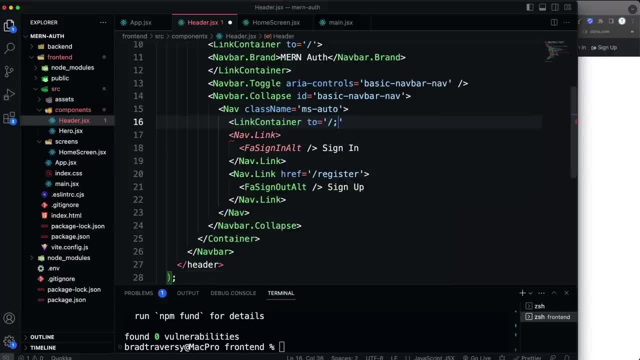 and that's going to have two, and that's going to go to slash login and what we'll do is move this, the whole nav link, into that link container, right, and then we'll do the same thing with the register. so we'll get rid of this href. 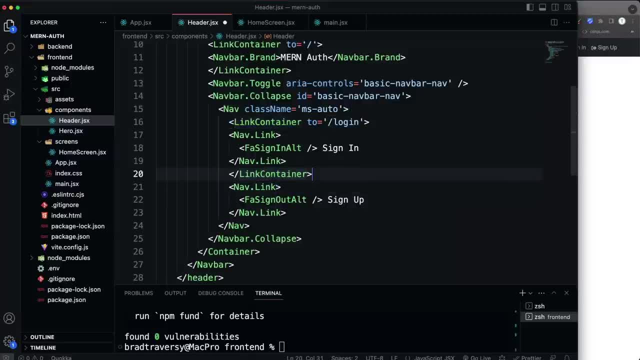 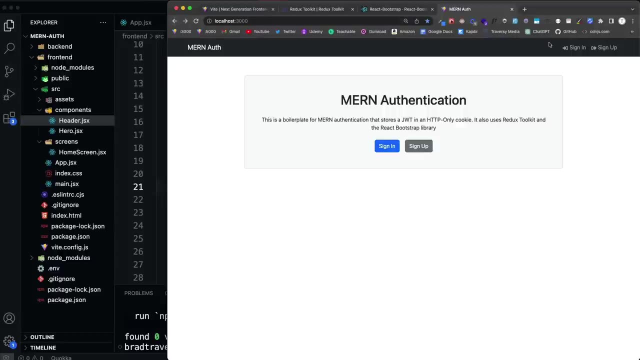 and then let's go right here and we just want to wrap this and change this to register. so if I save that, we come over here, this should still take us to slash login and slash register, except now it's not. it's not a hard refresh. now we also have these buttons which are using. 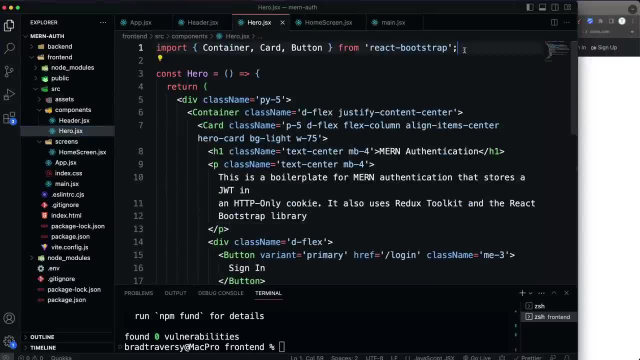 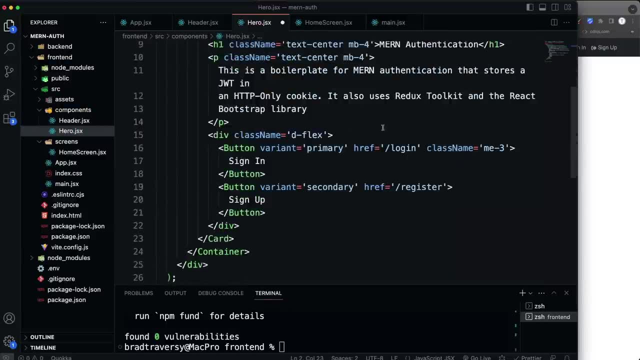 let's see that's in the hero component. so let's bring the link container in here as well. so import link container and then we don't want these hrefs on there. of course you want to��on a special later, just to make sure that we need a reason to type it in. but i'm going to run our channel it with some any in dashboards or whatever vos, for sometimes let me just do an example and then we'll see the next things surface: how we want to be build music with right, so we'll go to href and run it and then we, moving on to whether something else been added and 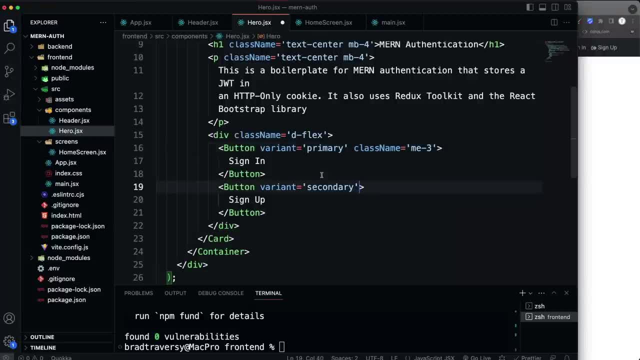 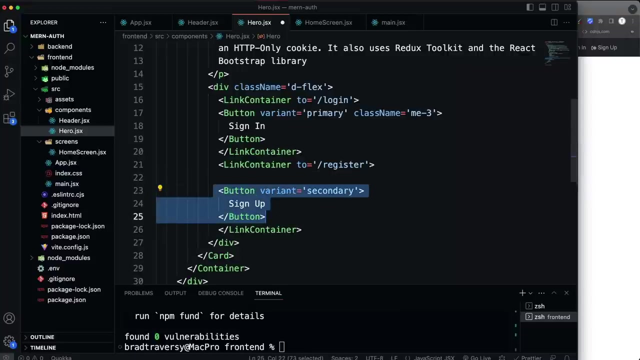 these buttons, so get those out of there. and then we're gonna wrap the button in the link container and let's have this go to slash login and then we're gonna move that button into there and then we'll do the same thing for this button, except that's gonna go to register, and then we're gonna move this into here. 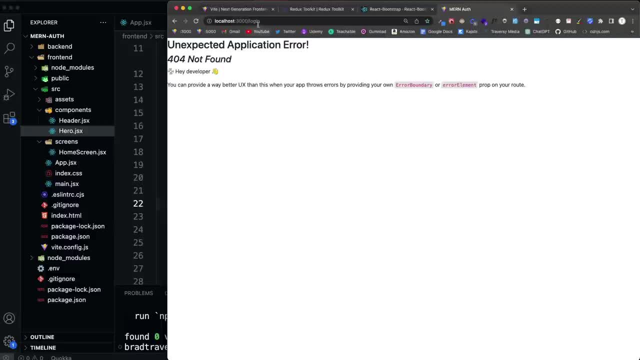 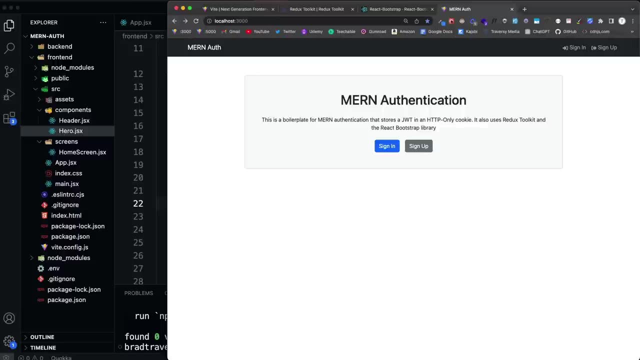 all right, let's make sure that works. okay, that brings us to login. that brings us to register. so now we have the, the navigation, all set. so we're gonna start on our forms now for the sign in and sign up and we'll do the, we'll do the. 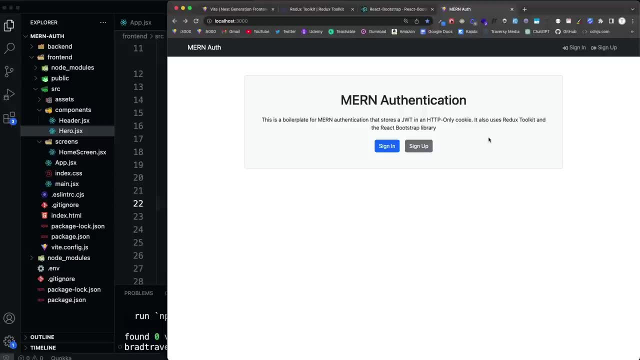 sign in or the login first, and the forms are gonna be a little different. they're gonna have a different layout where they're a little more narrow. they have a more narrow container. so I'm actually gonna create a form container component to wrap both of those forms and the update profile form when we get to that. so in components. 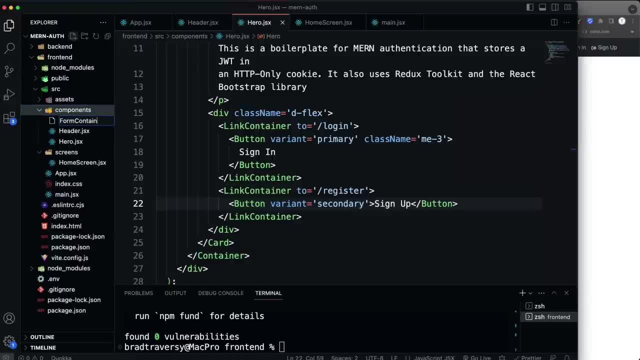 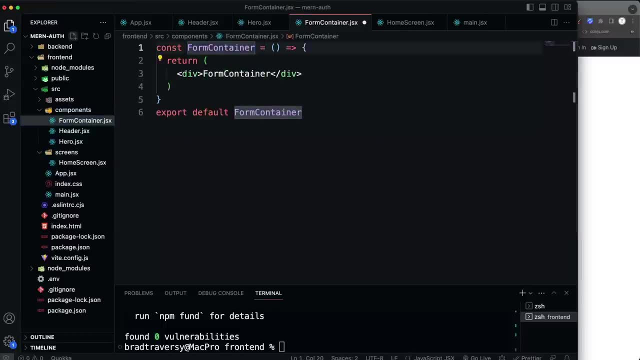 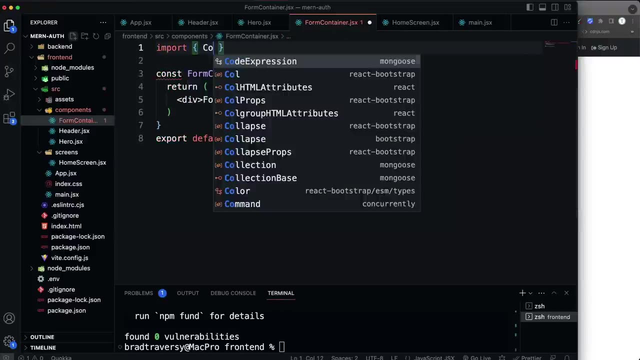 let's create a new component called form container, dot JSX and we'll say RAFCE. okay, so we have our form container. I'm gonna bring in some stuff from there and we're gonna go ahead and create a new component and we're gonna from React Bootstrap. so I'm gonna bring in the container and I'm also gonna 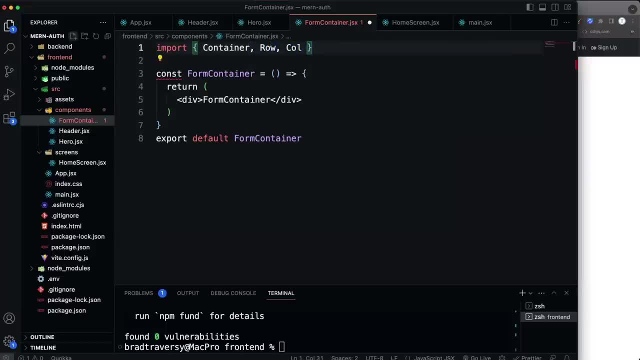 bring in the row and call so row and column and that's gonna be from react-bootstrap. now this form container: it's gonna wrap our login and register form, an update profile form, so it's gonna take in a prop of children because whatever we wrap it, we wanted to display in here. all right, 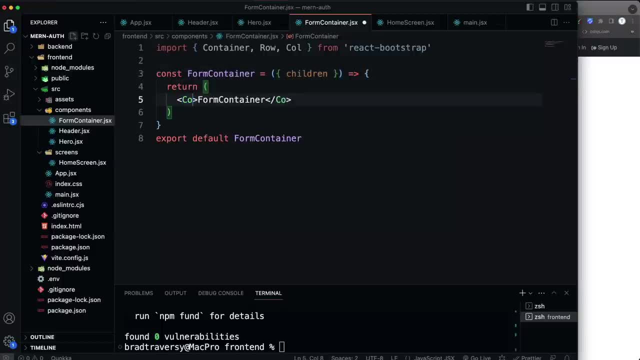 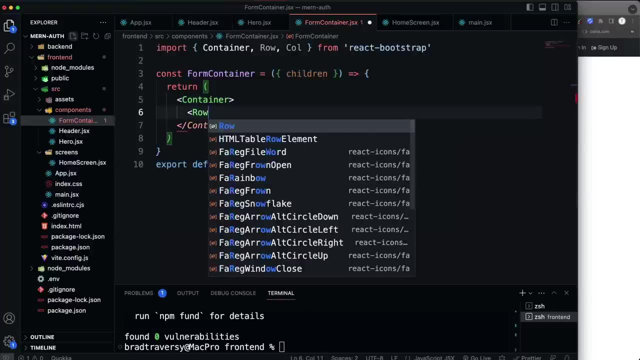 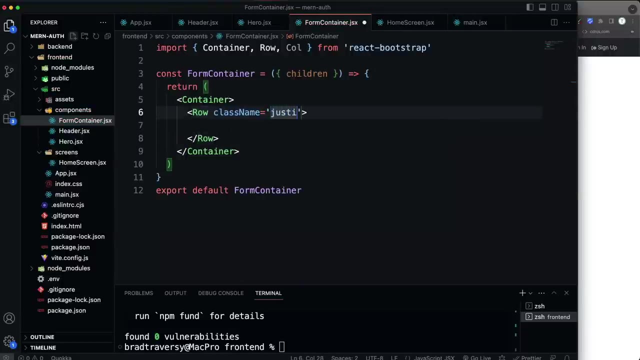 So the outer element is going to be the container. So let's add that, And then inside of that container is going to be a row. Okay, And that row, I'm going to give that a class name of justify, let's say justify-content-md. 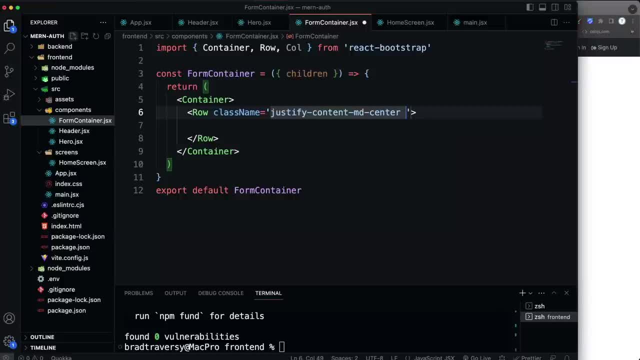 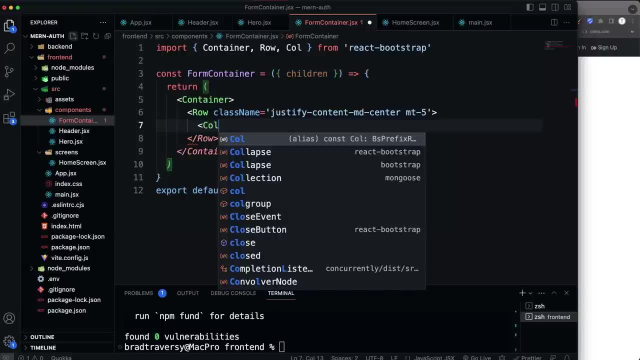 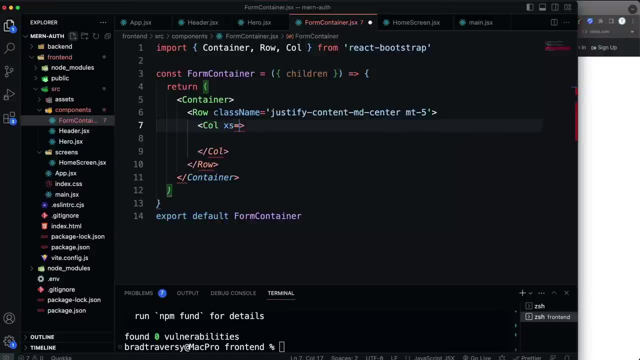 So on medium screens, center and then also margin, top five, And then in that row, let's have a call. Yeah, So we'll have a call and I'm going to add a couple props here. So we're going to do xs, so extra small. 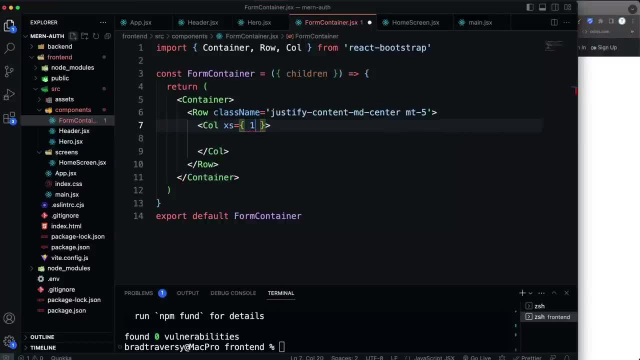 When the screen is extra small, I want the column to take up all 12 slices, basically All right, So I'm going to put 12 here, meaning it's going to stack if it's extra small. If it's on medium screens, then I only want it to take up six of the 12 slices. 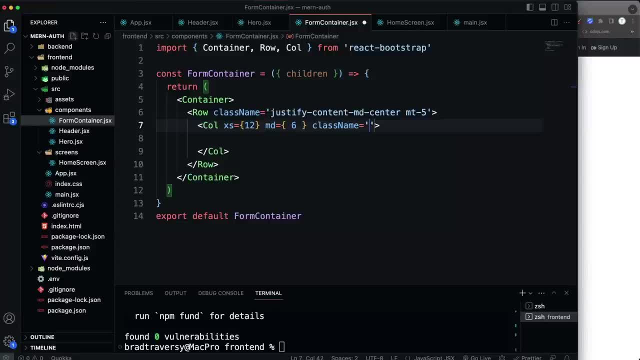 So it'll be half Okay, And then I'm just going to add a class name of card and also padding five, And then in here we'll just have the children. So basically, whatever we wrap, in our case it's going to be the forms. 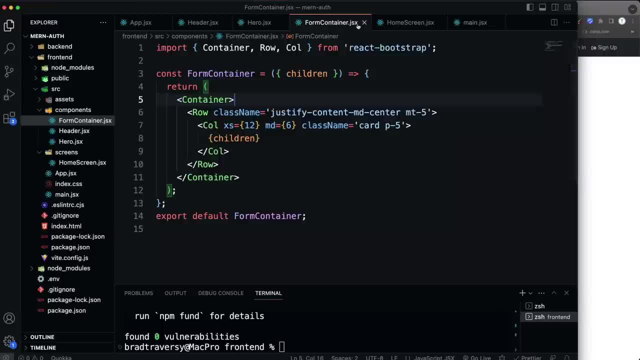 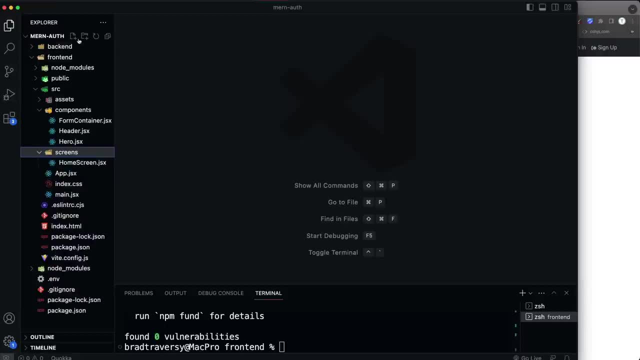 So let's save that And now we can create our login screen. So I'm going to close up everything here, just because this is getting kind of messy, And let's go into screens. Let's create a file here called login-screenjsx. 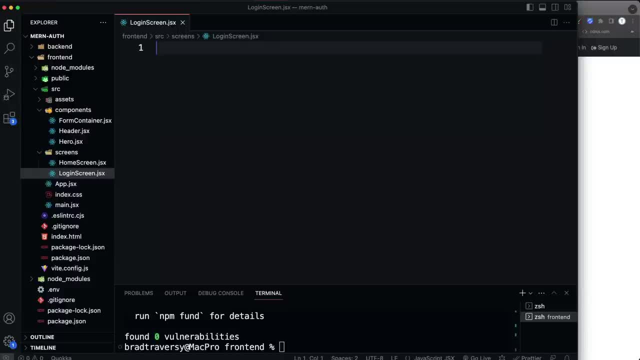 And before we start working with screens, let's go ahead and create a file here called login-screenjsx And let's go ahead and create a file here called login-screenjsx And start making our requests and all that. I just want to have the register and login screens. 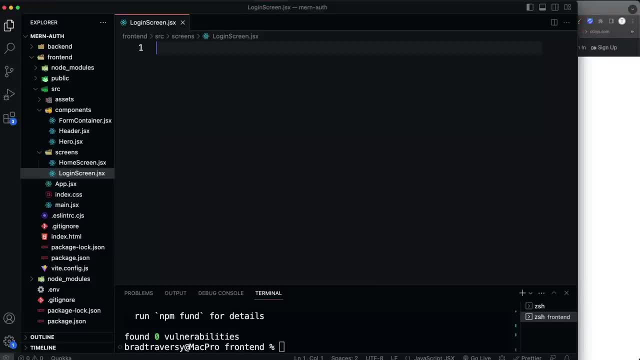 I just want to render them on the page and have our local state, just our email and password state for the form and all that. So first off, let's import use state, since we're going to have local component state And that's going to be from React. 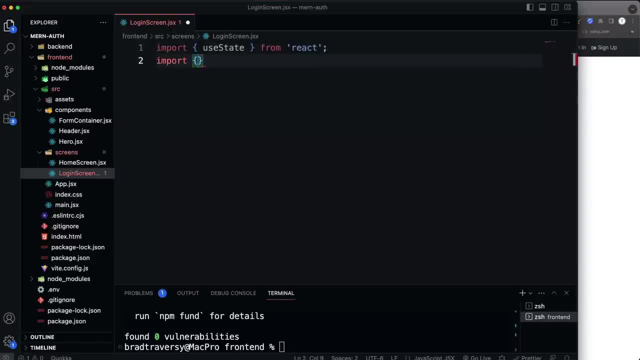 And then let's import. We want link from React router because we're going to have A link to the register page and then on the register will have a link to the login page And then, as far as React bootstrap stuff, we're going to bring in form button row and call. 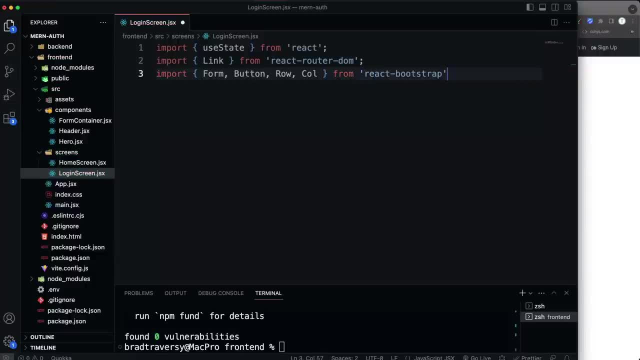 So that's going to be from React bootstrap, And then we also want the form container that we just created. So form container And that's going to be from. Let's see, we're going to go dot, dot, slash components, slash form container. 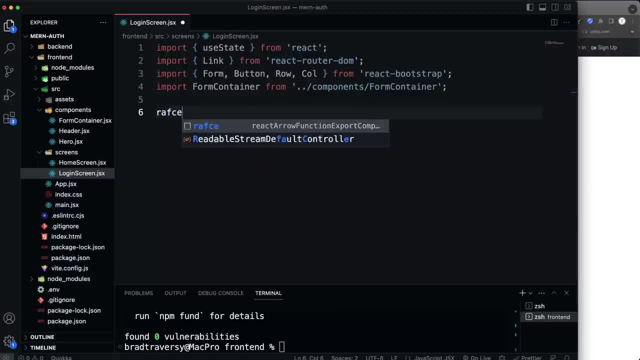 All right. And then let's create a component here called login screen, And I want to create the state first. So let's go up here, Let's say constant, We're going to have email, and then set email is going to be the function to manipulate that state. 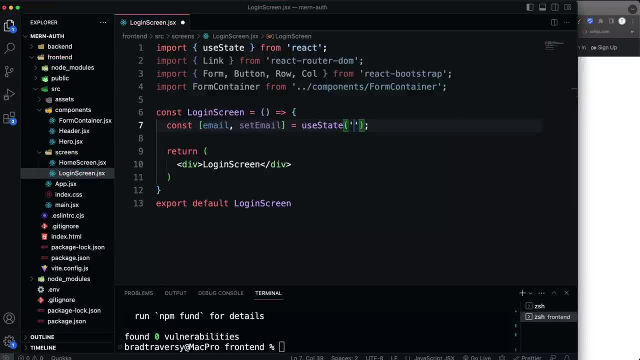 Set that to The use state and then the default- for that is just going to be an empty string. Then we're going to have set Password and Password, because this is this is the login, So we don't need name here. It's not the register form. 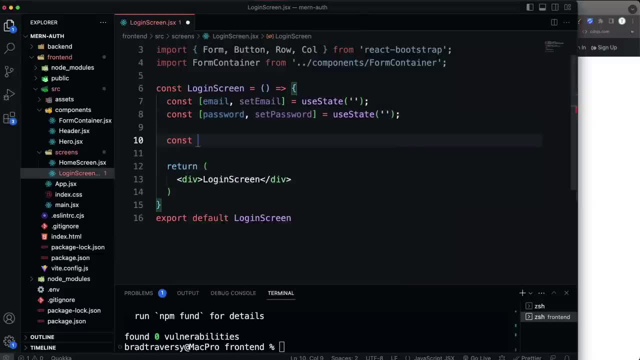 And we might as well just create our submit handler for now. So let's say submit handler And that's going to be. it's actually going to be an async function, Pass in our event Parameter and just for now, we're going to E dot prevent default. 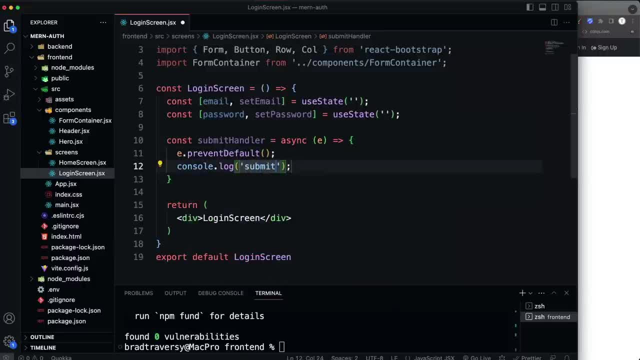 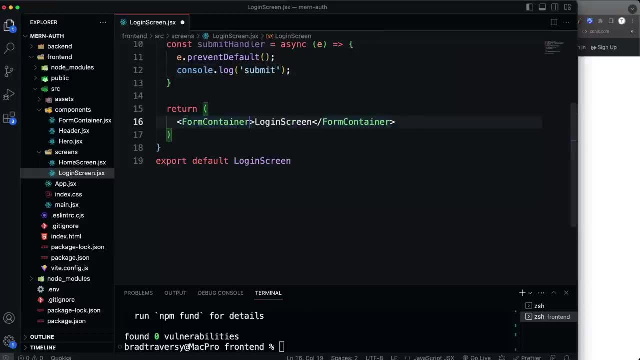 And we'll just do a console log of submit just for now. So now let's, let's do the form output. So the wrapper for these forms is going to be our form container. Okay, so that's going to be the the outer wrapper. then we'll have an H1.. 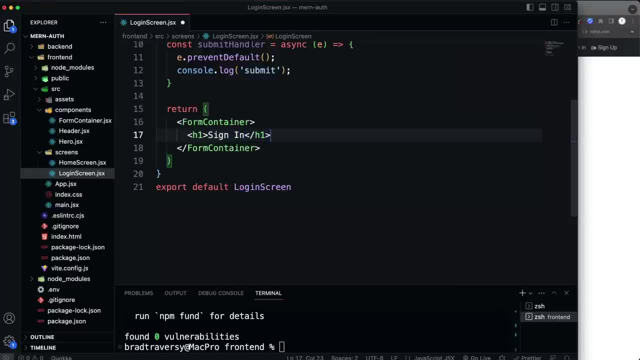 Let's say sign in and under that H1 will be our form And our form is going to have A submit handler. So let's say on submit, set that to the submit handler and then inside the form We're going to have a group for each, each input. 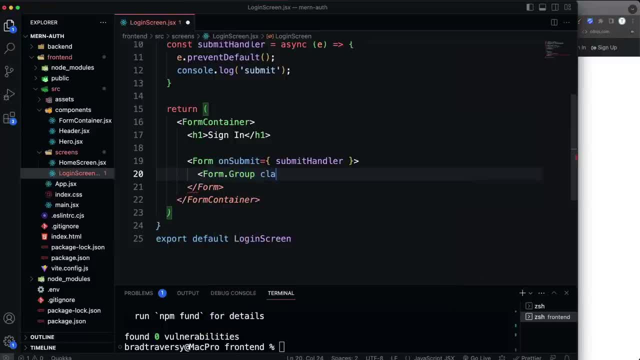 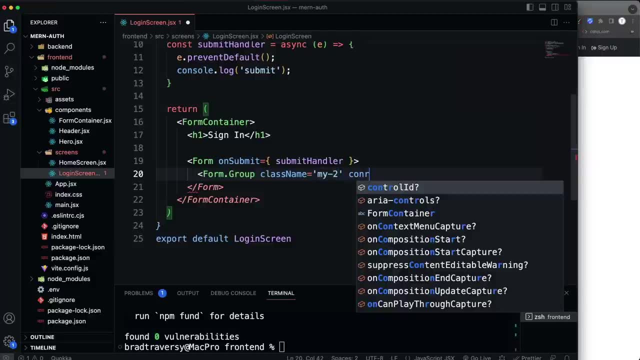 So let's say form dot group and I'm going to give this a class name of my to give it some margin, And it's going to have a control ID And set that to email, because this is for the email field Now in the group. 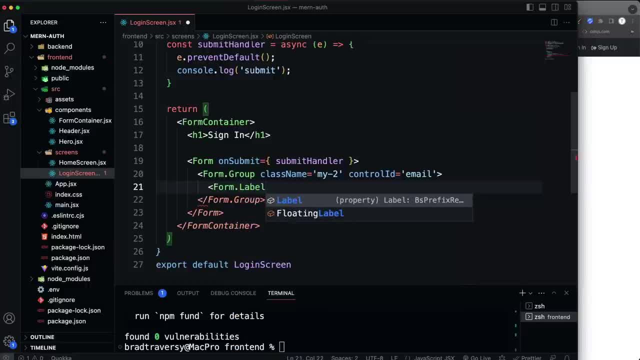 We have a label, so form dot label and that's going to be email address. Okay, under the label We're going to have the actual input, which is a form dot control in react bootstrap and that's going to actually take in some props. 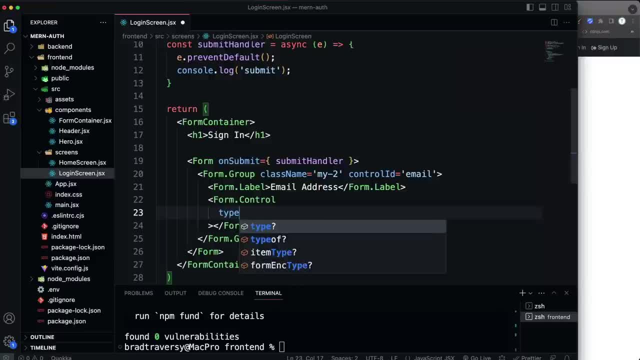 So I'm going to go in here and we're going to add a type- type is going to be email, and we're going to add a placeholder And that will be, let's say, enter email, And then we're going to have a value which is going to be: 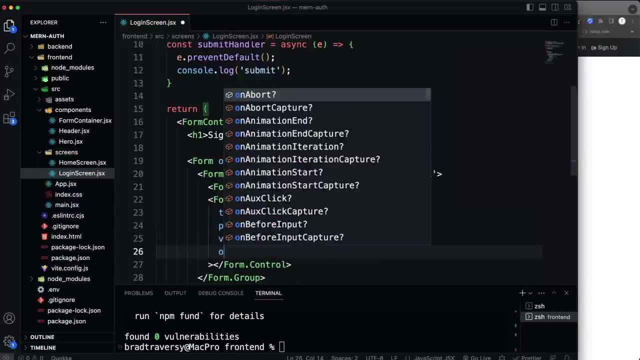 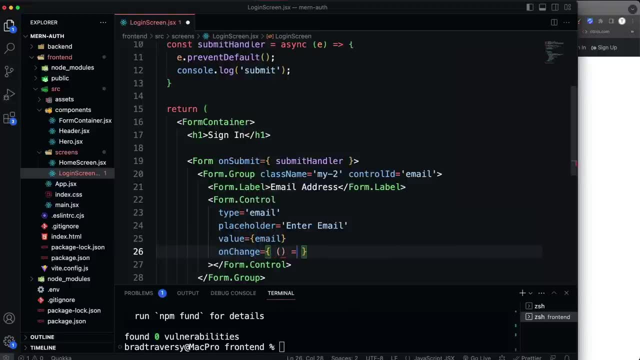 The email state and then we'll have an on change. So basically, when we type into this field, this function is going to fire off. So we're going to have an arrow function with an event parameter and then we're just going to call set email, because this is going to update that state with whatever we type in. 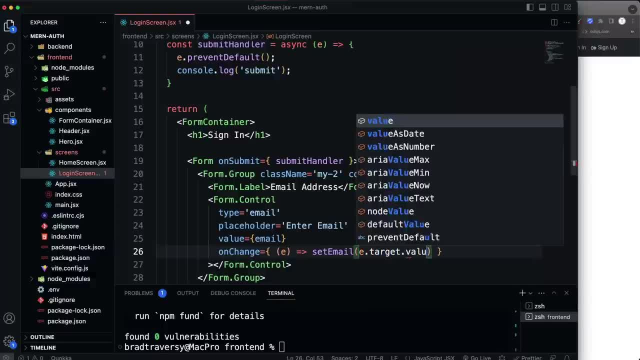 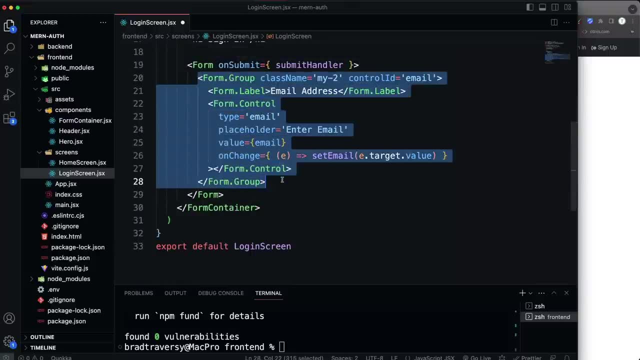 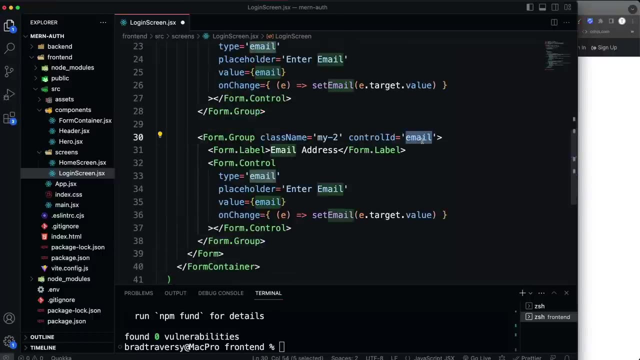 So we pass in Here: e dot, target dot value. All right, so that's the first input. then I'm going to copy this form group and then right under it Let's paste that in. and now we want the password. So I'm going to change the ID here, actually going to change all of these instances of email to password, except of course we don't want password address. 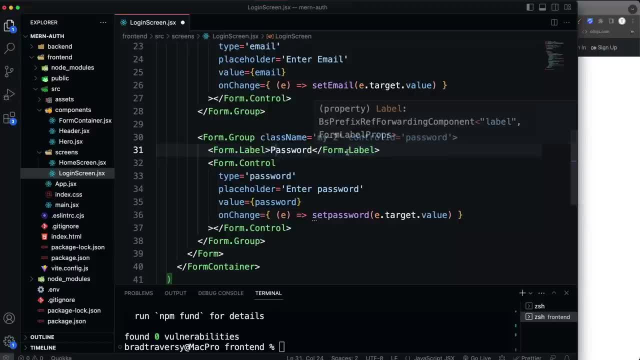 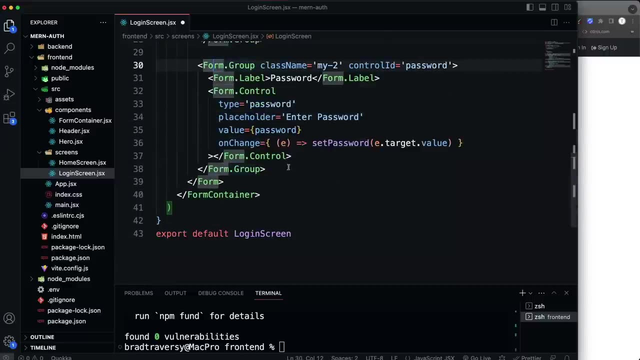 I actually did that in another tutorial. I forgot and I left. I left it as password address. type password: enter password. except, I'll make that uppercase and then set password. This should also be uppercase, All right, then we want our button. So under the form group, let's say button. 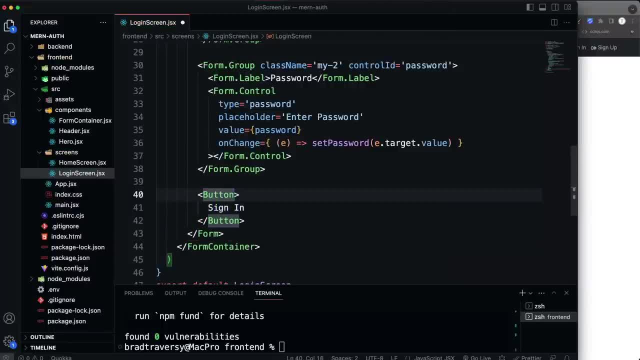 And we'll say sign in. but I just want to add a couple props to this button. So one is going to be the type and we want to set that to submit and then the variant Variant. I'm going to set that to primary and then class name. 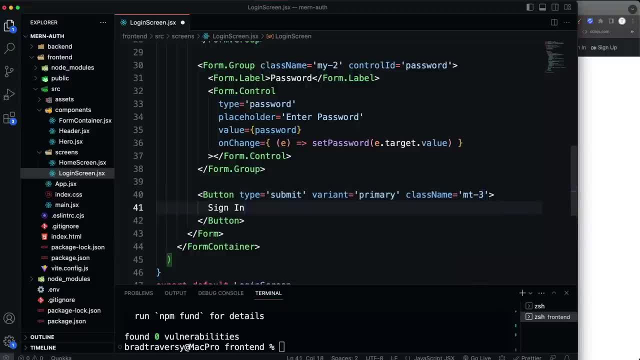 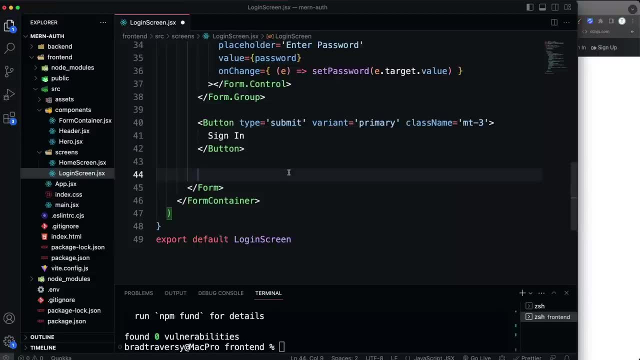 I'm just going to do some margin on the top. Now, underneath that, I want just an area where it says: if you're a new customer, then they'll have a link to register. So I'm going to put that into a row and this row is going to have a class name of py-3. just some padding and then inside there. 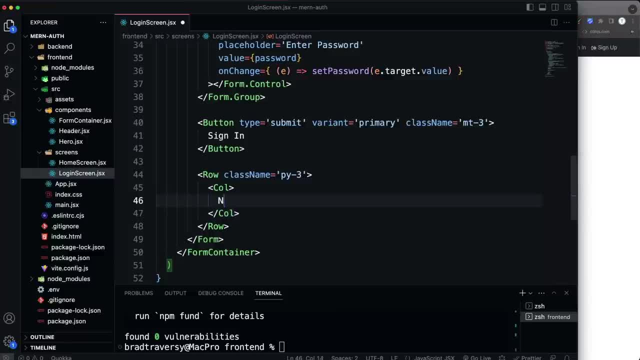 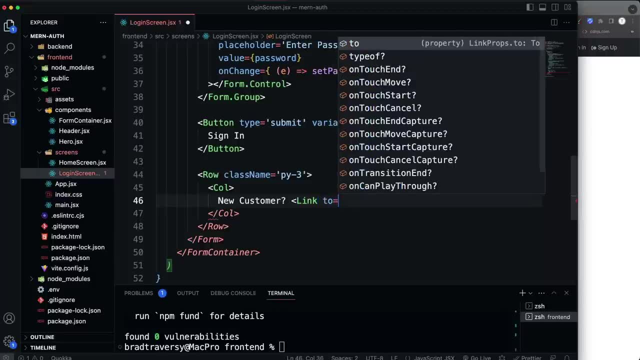 We'll have our call and inside the column We'll say new Customer, with a question mark and then a link, and that link is going to be to What is this going to be to? this is going to be to register, Right, because if they're a new customer, then they need to register, and we'll just put in the text here: register- 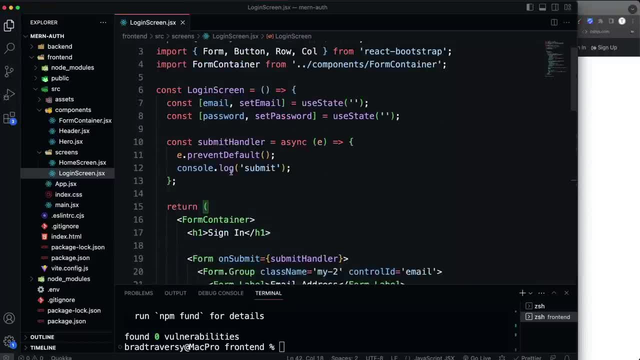 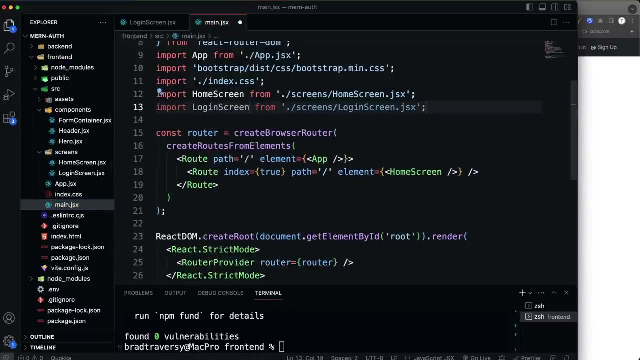 Okay, so obviously this isn't going to do anything yet, It's just going to log submit, but at least we have the, the UI, So let's go ahead and now create a route for this. So we're going to go back to our main dot JSX, where we have our routes, and we're going to import the login screen and then down here. 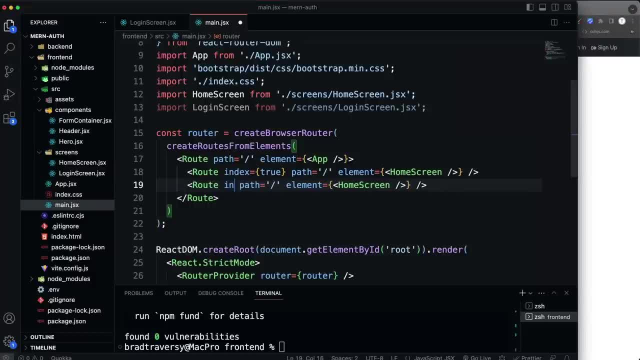 I'll just copy this down, except, of course, we want to get rid of the index- true, because it's not the index. and then the path is going to be slash login and the element that we want to show on that route is going to be the login screen. 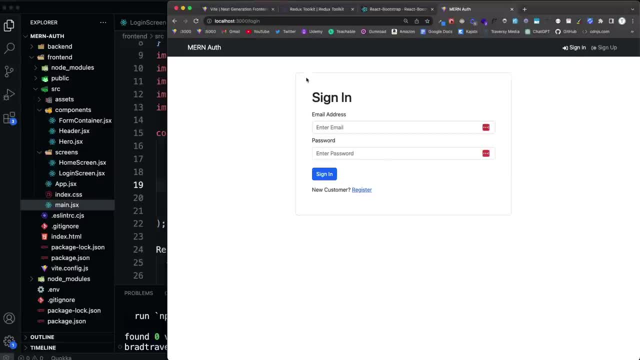 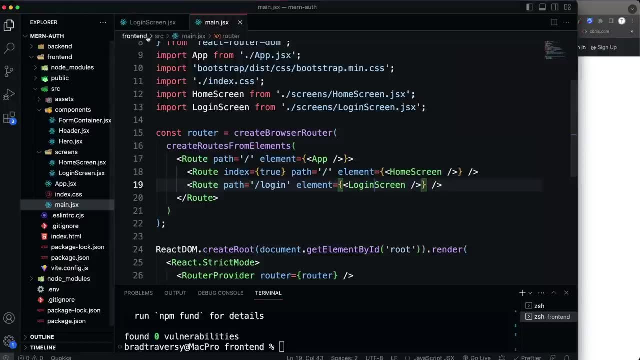 So now let's save that, Let's click on sign in and it takes, Takes us to slash login and we can see our form UI. Now for the register screen. let's do that because I just, I just want to get the output, the UI, there before we start looking at state and functionality and requests. 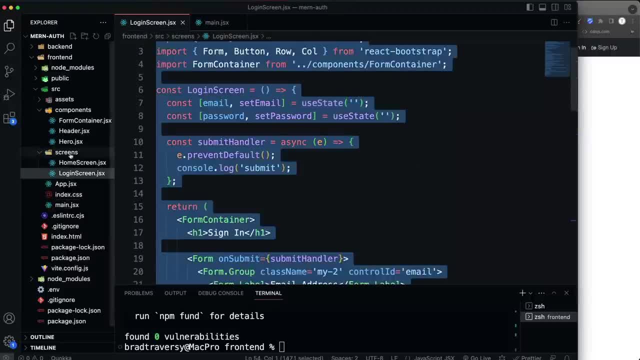 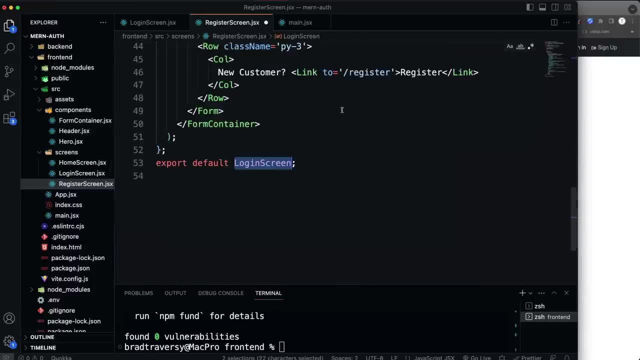 So I'm going to just copy everything from the login screen because it's very similar, and then let's create a register screen. So register screen dot JSX, And we'll paste that in. and just be sure that you change Here this login screen and then down at the bottom change that to register screen. 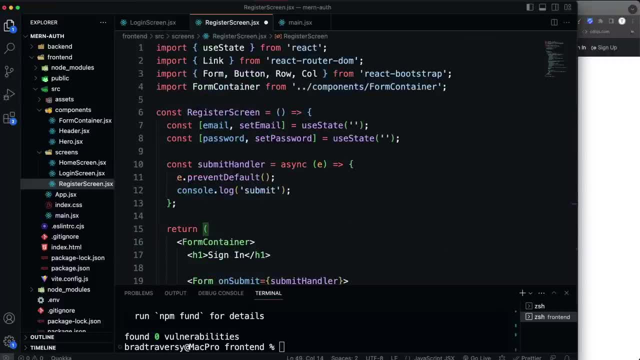 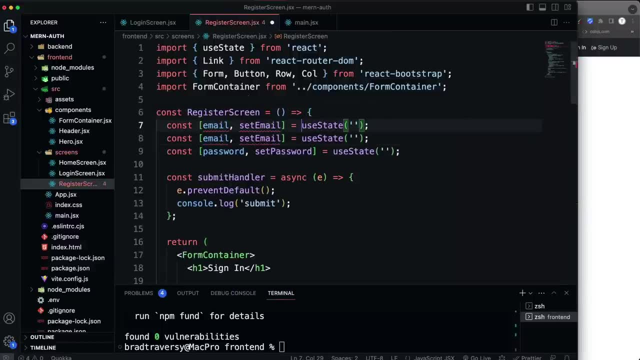 And then we have a couple changes that that we need to make here. So, in addition to email and password, we're going to want the name, Right, So let's change this to name And this is going to be set name, And then I also want a confirm password. 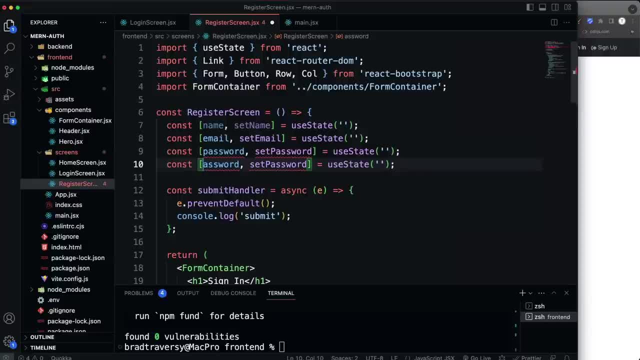 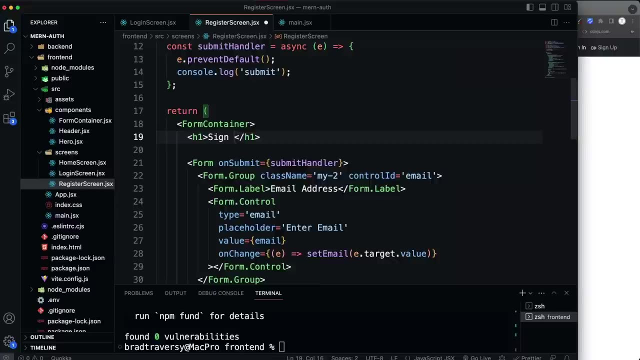 So I'm going to copy this down And this is going to be called confirm password And then this will be set: confirm password. Okay, and then let's see submit handle. We'll just leave that for now. Let's change this to sign up instead of sign in. 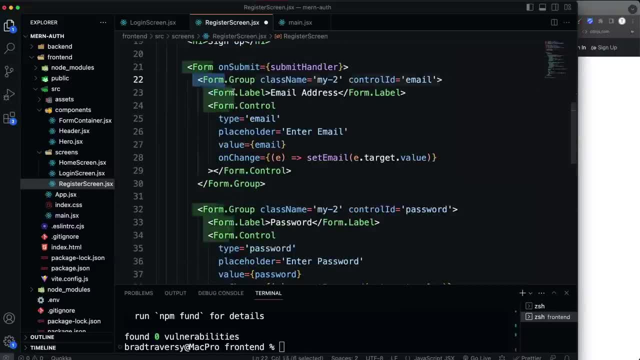 And let's see, we have our email here. I'm going to copy this email form group and then, right above it, We'll go ahead and paste that in and this will be for the name. So I'll just change all this stuff to name. 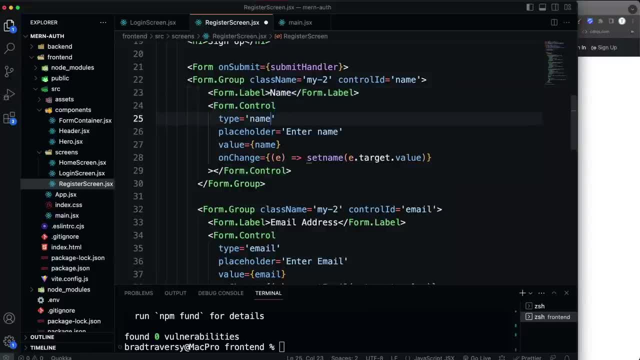 Get rid of that. to make this uppercase type. There is no name type. Let's make that text and we'll say enter name and then set name. That should be uppercase and we should be good there. Now we just want to do the confirm password. 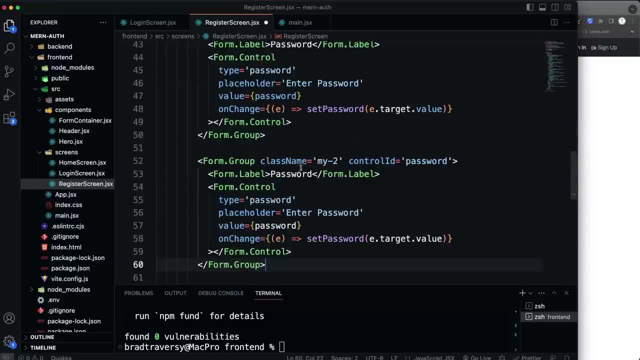 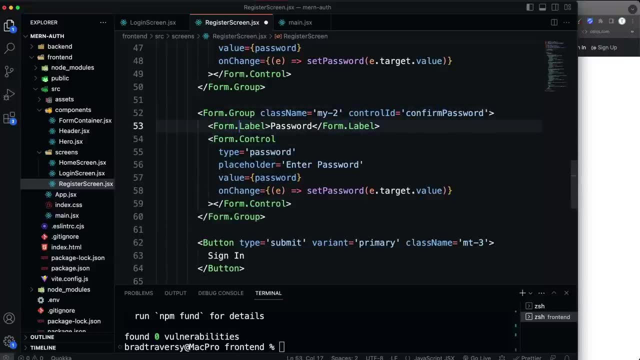 So I'll copy the password form group And we'll change the control ID to Confirm password. and let's change the label here To confirm. the type will be password. here We'll say, instead of enter will say confirm, and then the state is going to be: 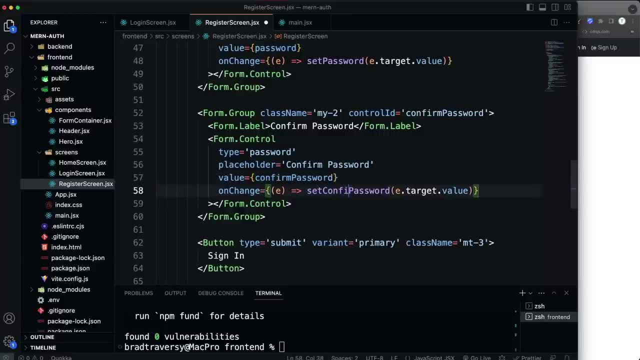 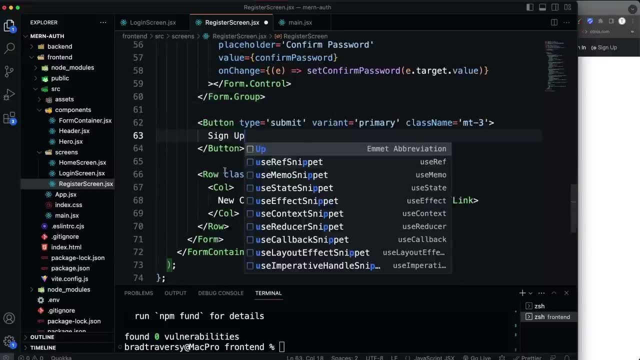 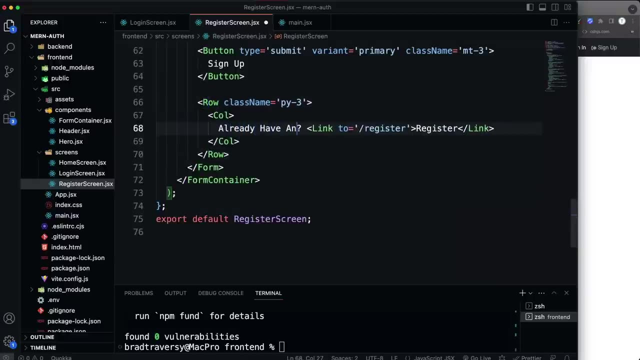 Confirm password and then set Confirm password now down here. Let's change sign in to sign up and let's also change right here It says new customer. Let's change that text to say Already have an account. Or let's not do uppercase will say 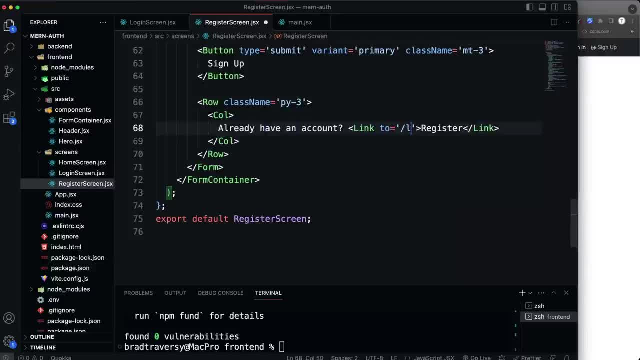 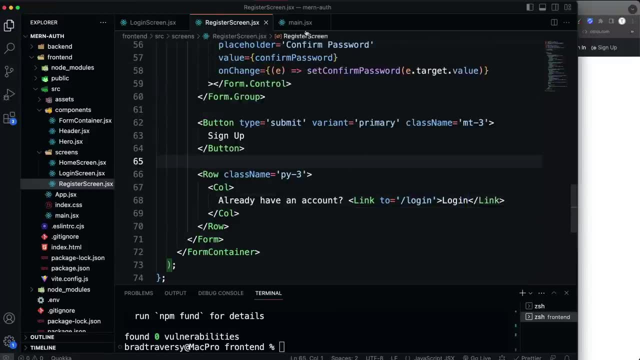 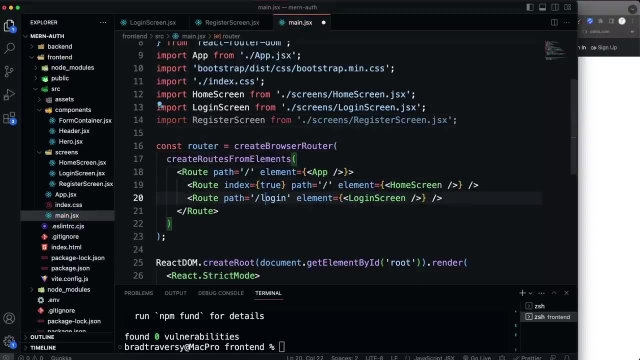 So already have an account and then this is going to go to login And we'll change that to login. All right, so that's our register screen. So let's go back to main JSX and let's import the register screen and then we can add that route. 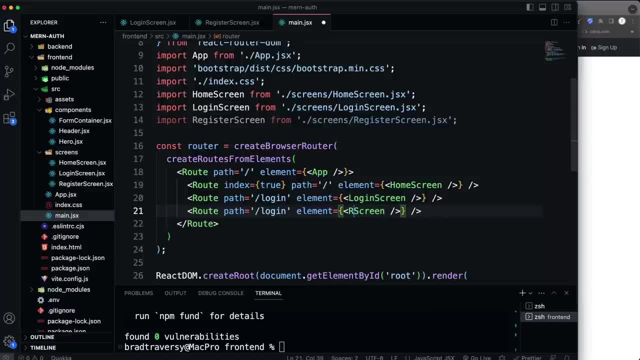 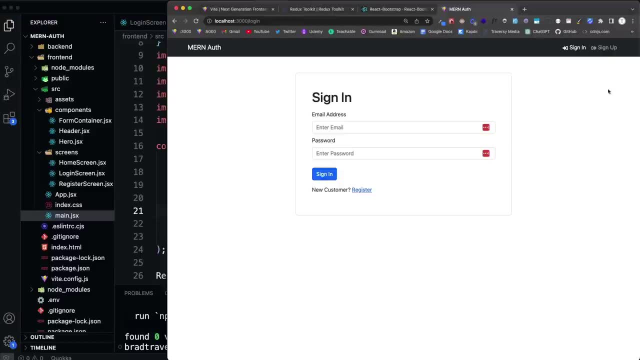 Down here, Let's change this element to register screen and change this to the path to slash register. So now I should be able to click on sign up and it takes me to the sign up UI, the sign up form. So now we're going to get into our global state. 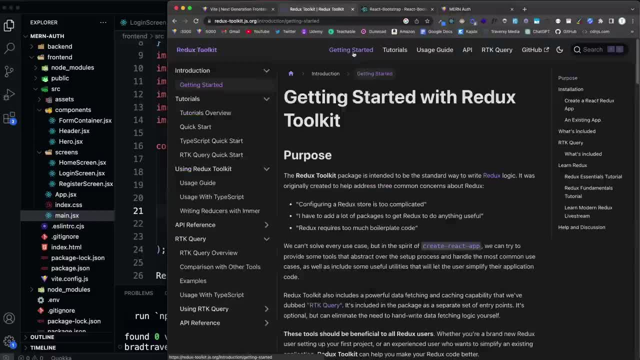 And again, we're going to be using Redux Toolkit and they have guides here, They have tutorials, if you want to use this as kind of a supplement. but basically it makes Redux easier and it makes us not have to write as much boilerplate. 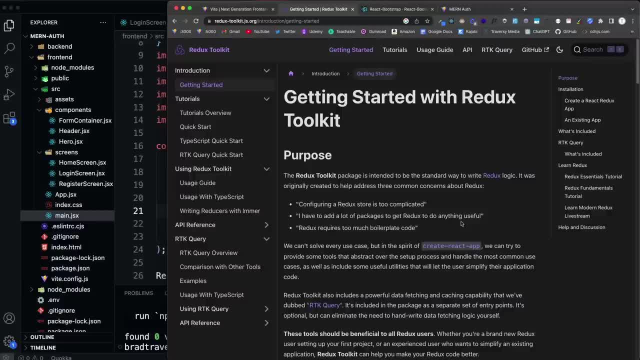 We don't have to create like our custom actions to make our requests and all that. It's as simple as creating a slice and then for any requests We want to make, we just add an endpoint. All right, there is a little bit of set up, but not as bad as if you were using just vanilla Redux. 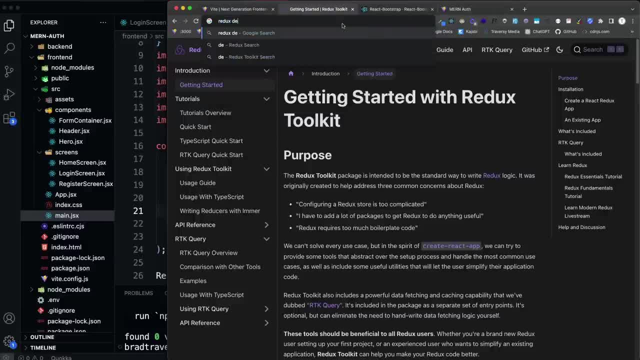 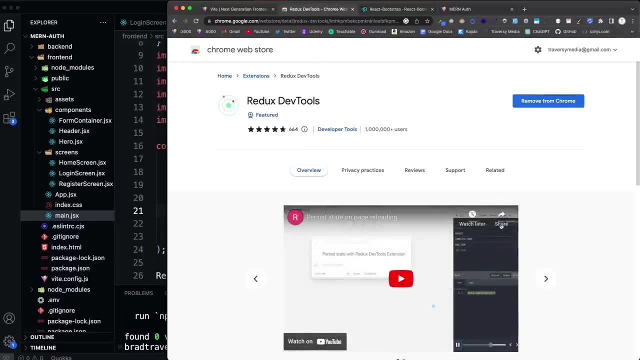 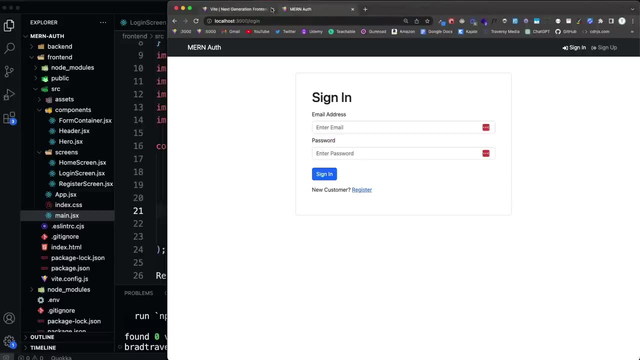 Now I definitely would suggest that you use the Redux dev tools. So, whether using Chrome or Firefox, Definitely get these installed because it helps you. just, you know, see your state and see any actions that are fired off, or anything like that, And I'm just going to close the rest of this stuff up. 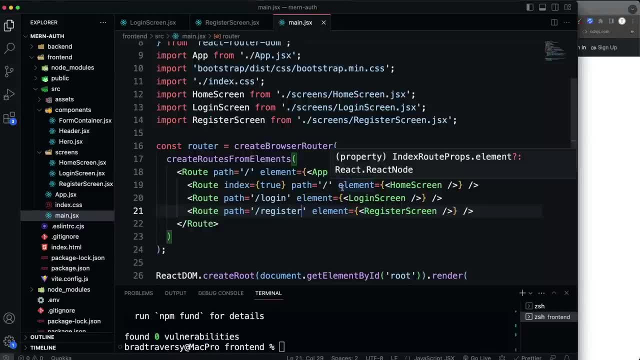 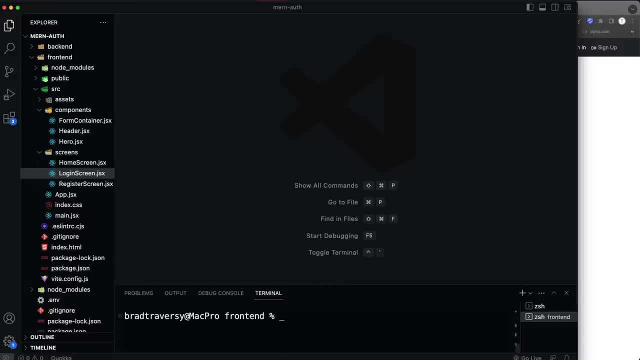 So let's install it. First of all, and again, make sure you install it in your front end. I'm going to close these tabs up for now and down here You can see I'm in my front end and I'm going to run NPM install and then at Redux, JS slash. 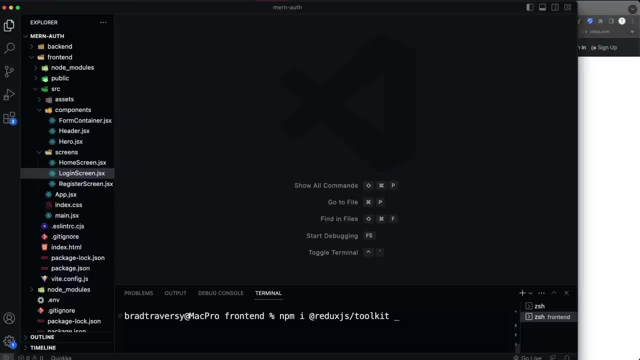 Toolkit, and then I'm also going to install the react Redux bridge, which is called react dash Redux. that just makes it so we can use Redux with react, because you can technically use Redux with with anything really, with vanilla, JavaScript, with angular, with anything. It just goes really good with react. 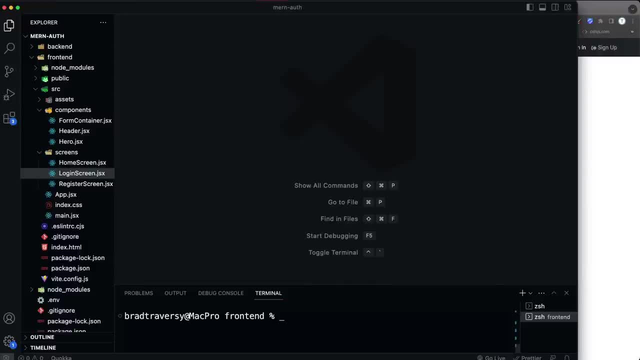 All right. So now we have that installed, The first thing we're going to do is create our store, which is a place to hold all of our state, And then we can And dispatch actions to change that state. We can also subscribe to that store to get the current state. 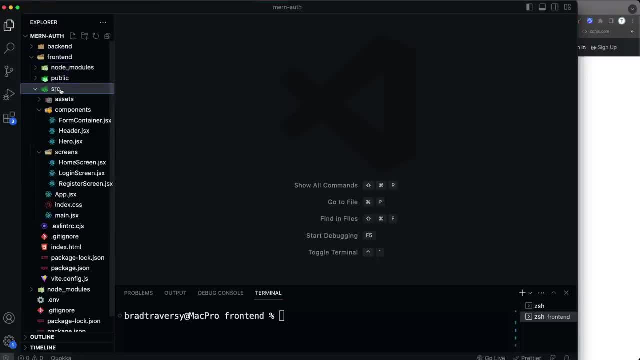 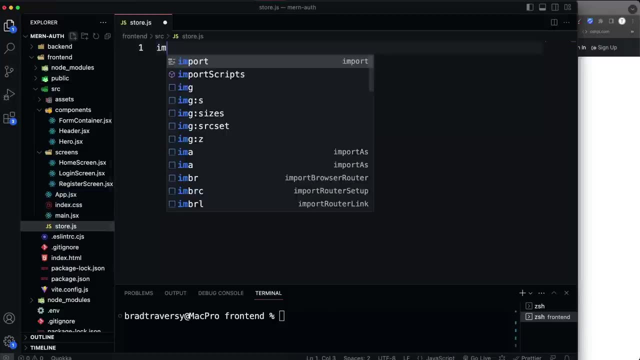 So in the front end folder, in the source folder, let's create a file called store dot JS, And the way we're going to set this up is we're going to import something called configure, Store, and that's going to be from Redux Toolkit. 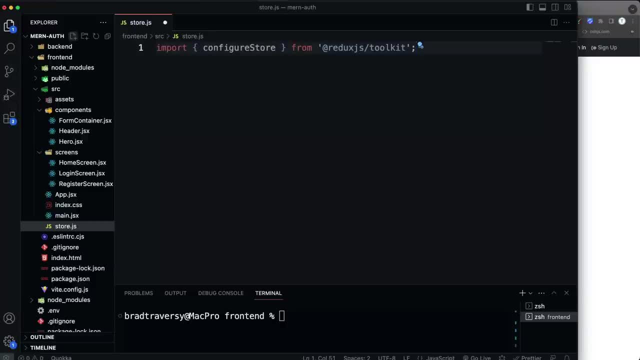 So at Redux JS slash Toolkit, And then the way we do this is we create a variable called store, set that to our configure store And then that takes in an object, And that object we're going to have a reducer object, And this is where we put our reducers right now. 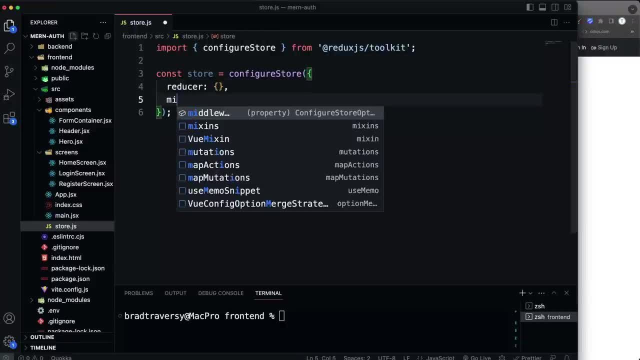 We don't have any, so we're just going to keep it empty. And then we also have our middleware, which I'm going to set that to an arrow function and this will take in A Function to get our default middleware. So it's called get default middleware. 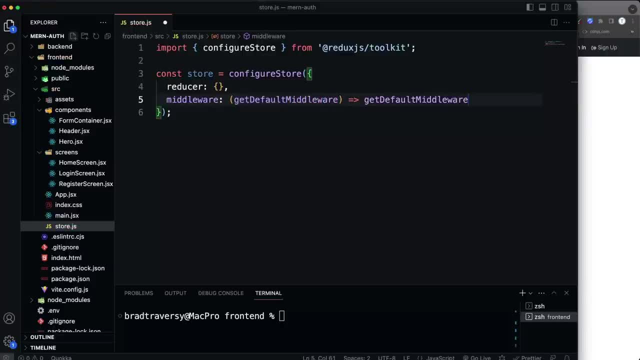 And then we just want to call that. So get Default middleware like that, And then we'll do comma And then dev tools. This is important because you want to be able to use the Redux dev tools, So you have to add this: dev tools- true. 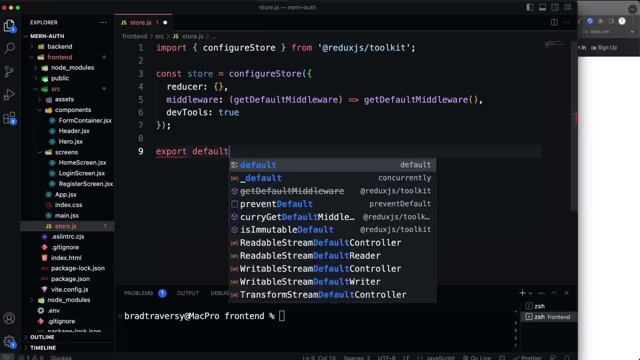 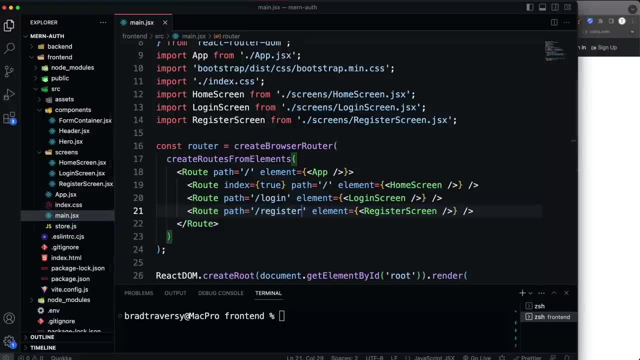 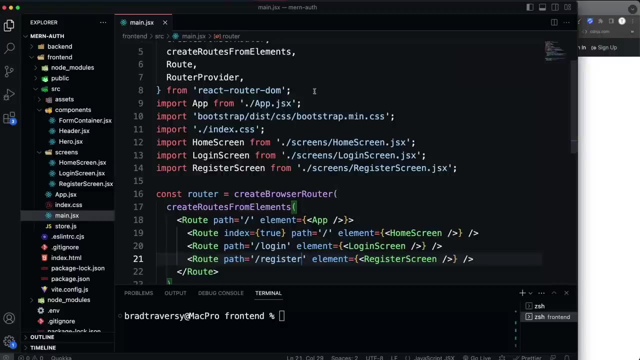 All right, And then we want to just export as default our store And then we can bring that in To our main entry point, which is main dot JSX. All right, So in main JSX we're going to bring in Couple things. let's go. 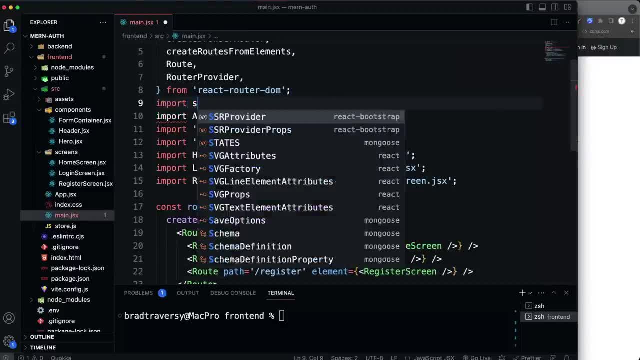 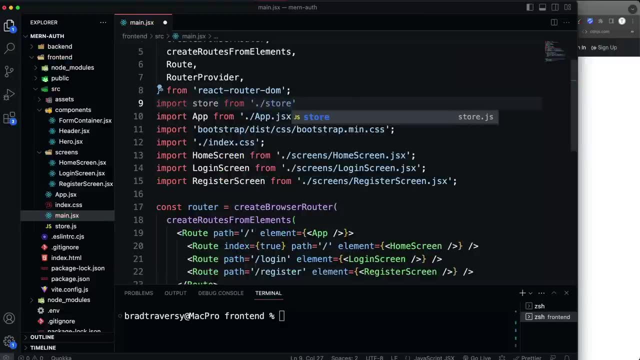 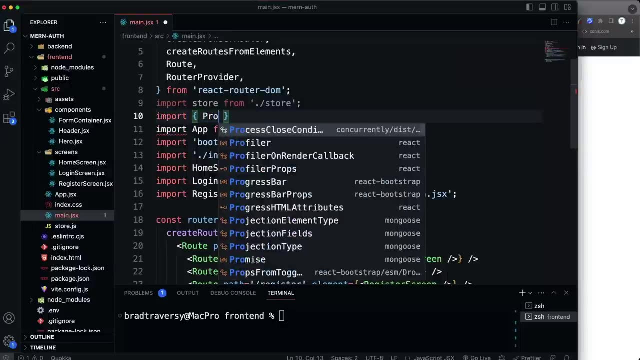 Right here. and let's say import Store and that's going to be from just dot slash store, because that's in the same, on the same level, And then we want to bring in our provider for Redux. So let's say import Provider. 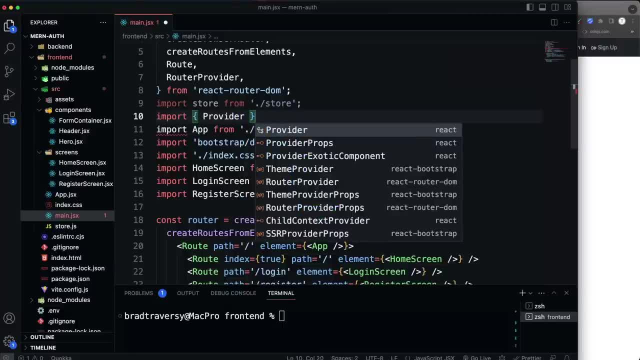 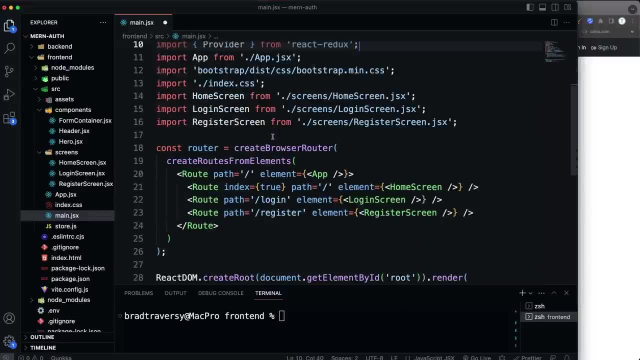 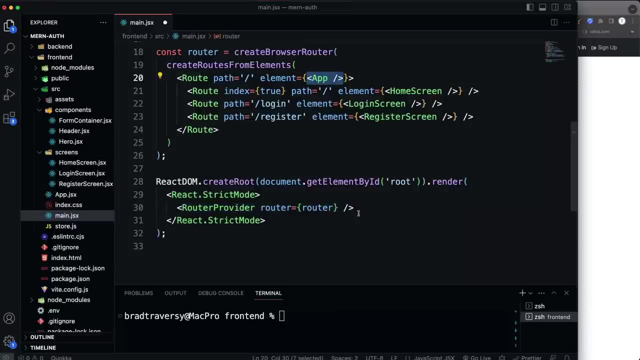 Now the provider is actually from react Redux, which is the bridge, So react dash Redux. All right, Then what we want to do is come down here where we, where we have our router provider, which is essentially our app, along with our routes, And we want to surround that with our provider, will surround the react strict mode as well. 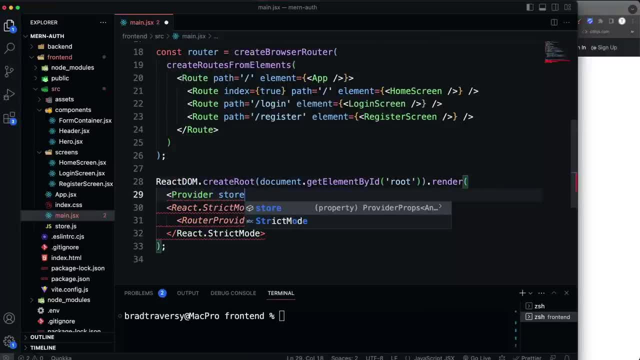 So right here let's say provider, And then that's going to take in our store Here. so the store that we just created in the other file and we want to wrap everything, So let's go down here and put our ending tag. So now our store is is there and it's implemented with our app. 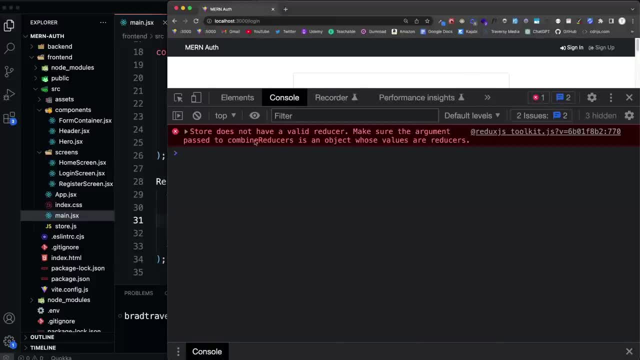 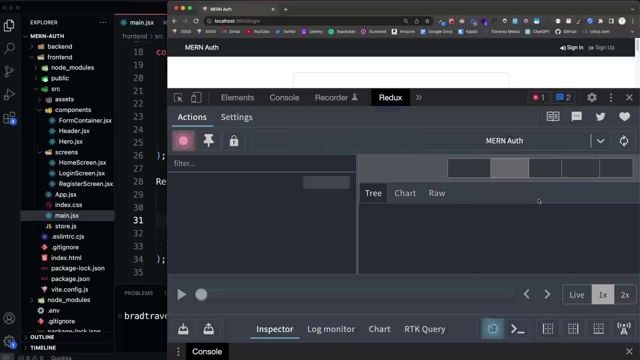 We can open up our dev tools And if you go to your console, you're going to see that it doesn't. we don't have a valid reducer yet because we haven't created any reducers. So that's fine. And if you go to Redux, 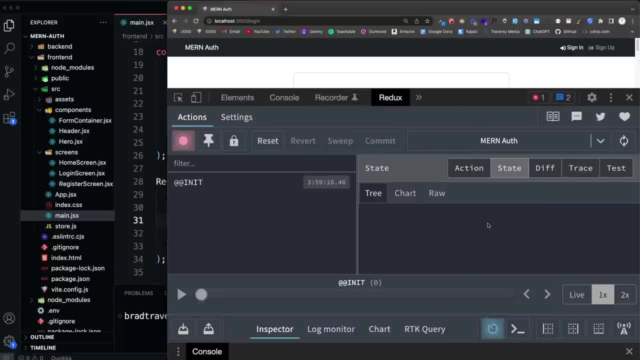 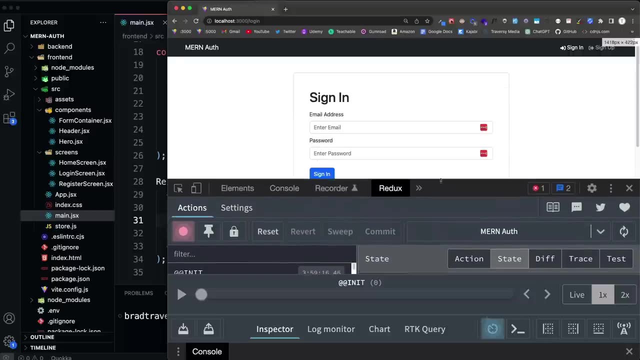 At least You're not going to see anything here yet in our state, because we have nothing. We have no reducers, There's nothing in our state, but this does work, So we do have this working. So the next thing we want to do is create a slice. 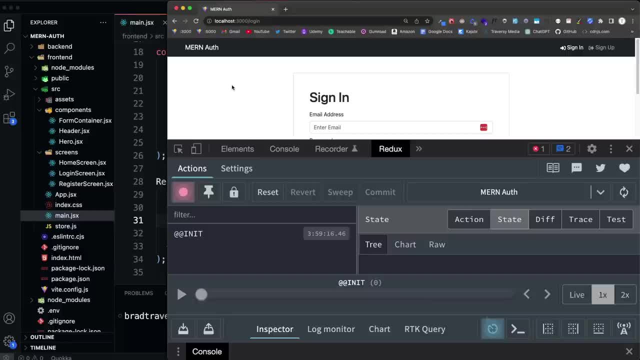 Now, the way that this application is going to work is we're going to have two slices, and a slice is just where you can keep certain pieces of state, as well as your reducers that take in actions, And we're going to have two different slices. 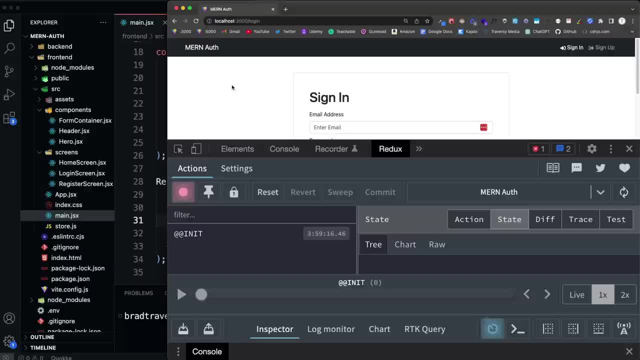 One Is going to be called off slice and it's going to just be dealing with local stuff. So it's going to take the user data that we get back from our API and put it in local storage and also put it in our off state. 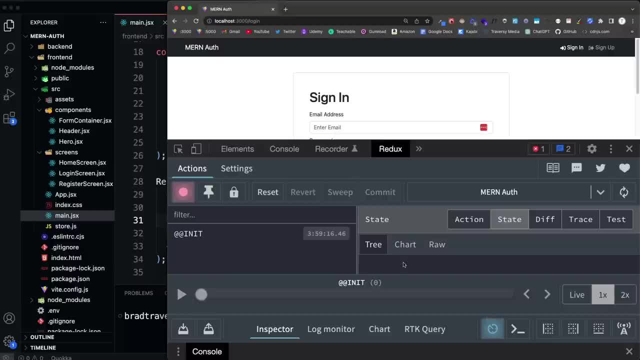 So it'll have the ID, the email and the name, right, not the token. Remember, the token is stored in an HTTP only cookie. It'll also have the log out, where it will destroy it from local storage. But that's really it for the off state. 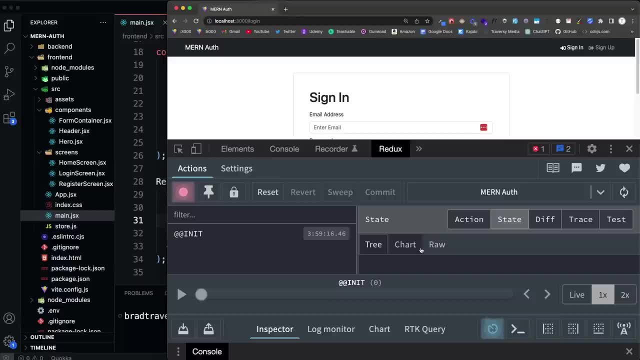 The other slice we're going to have is the user API slice and that's where we actually make the request to the back end to log in, to authenticate where we register, where we get our profile, where we update our profile. That stuff is going to go through the user API slice. 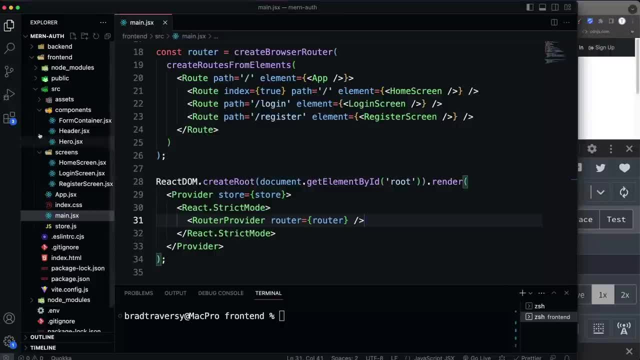 All right. So let's start with the off slice, which again, is just the local stuff. So we're going to create in source, in our front end, a folder called slices And we're going to create a file called off slice dot JS. Okay, 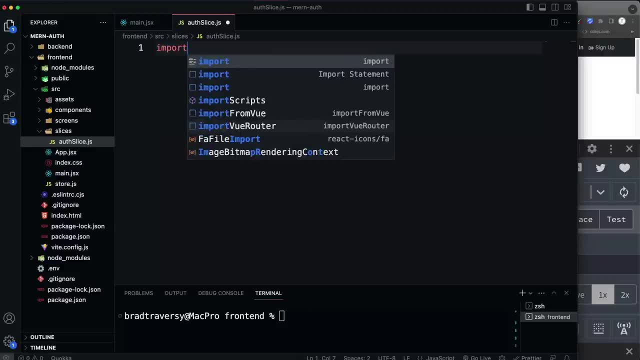 And then we're going to add to this or we're going to bring in create slice. Okay, And there's two different kinds of slices. There's one like this, which is just a local stuff, And then there's an API slice where, where it implements the Redux thunk middleware so that you can make a synchronous request. 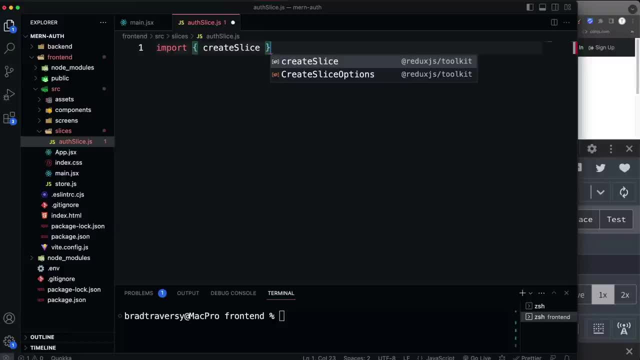 Okay, And if you've ever done anything with vanilla Redux, you know that you need to set up that thunk middleware manually. But here we don't It's. it's much, much easier, as you'll see. So let's say, import, create slice from, and then that's going to be from Redux toolkit. 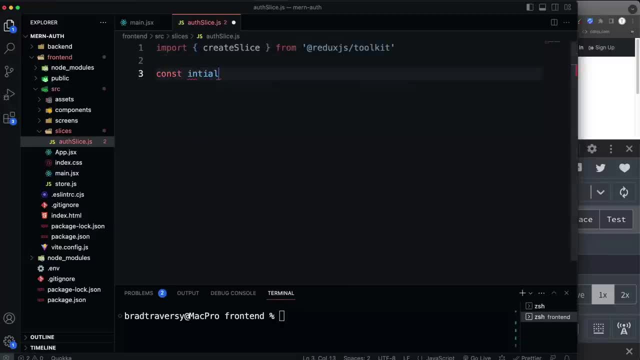 And then we're going to create our initial state And basically our initial state is going to check local storage. So this is going to be an object with user info And for that user info we first want to check local storage. So we're going to say get item and that's going to be called user info. 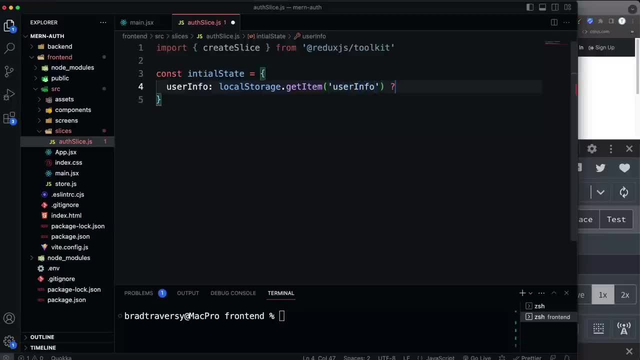 And we're going to use a ternary here because we're saying if that's there, then we want to use that And we also want to parse it. You know, Jason dot parse, which will turn it into an actual JavaScript object rather than just a string. 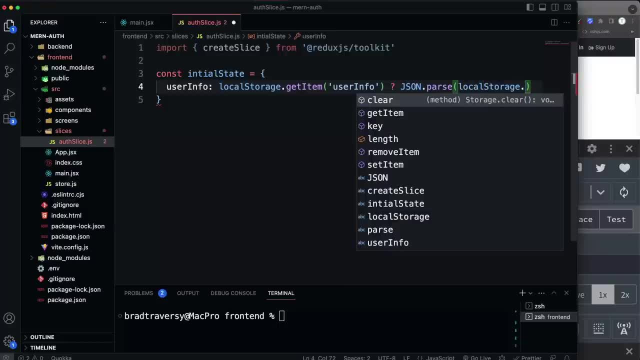 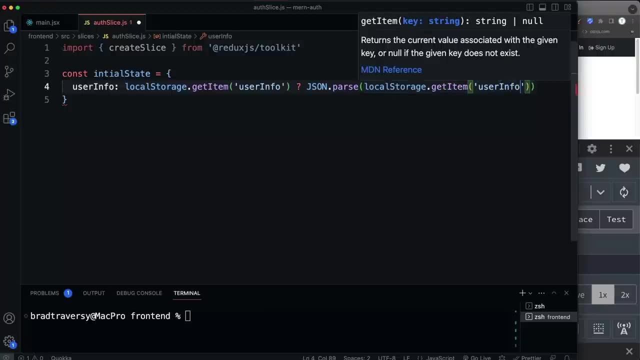 So we're going to pass in here local storage dot. get item. Let's close that up, Okay. So get item and user info, else then this will be no. What did I? did I miss something up here? So Jason dot parse, Oh, wait a minute. 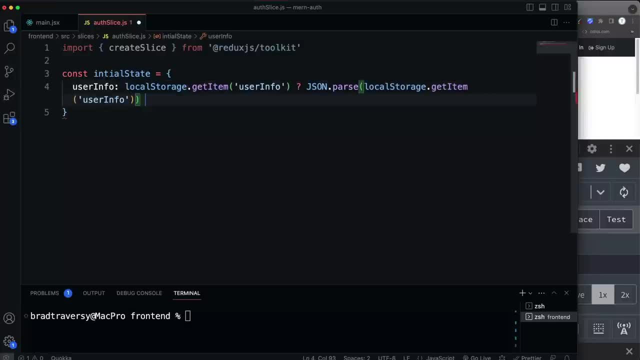 User info. So after both of these, Yeah, Then we want to do else, no, All right. So hopefully that's clear. We have our initial state, which is user info. It's going to check local storage for user info. If it's there, we're going to use that. 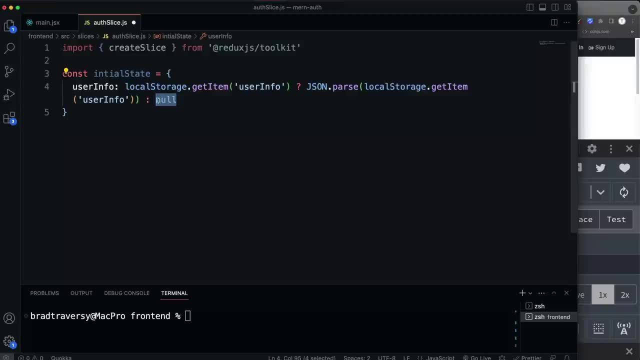 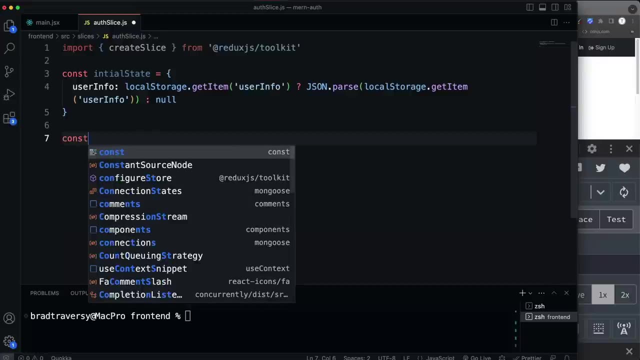 We're going to parse it as well, And if it's not there, then user info is just going to be no, All right. So that's our initial state. Now, down here, we're going to create our slice. So let's say const auth slice. 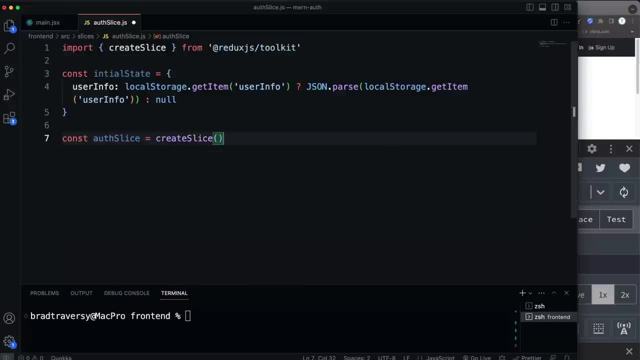 And we're going to set that, to create slice, which we just brought in, And that takes in an object with a name which we're going to set to off, And then it takes in our initial state, which we just set above, And then it also takes in reducers, which is going to be an object with reducer functions. 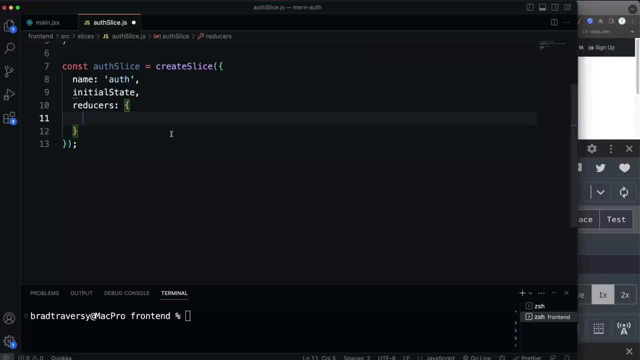 And in this particular slice, we're going to have two functions: Set credentials, which is going to set our user info to local storage, And log out, which is going to take our info off, Take our info out of local storage. So let's say, set credentials. 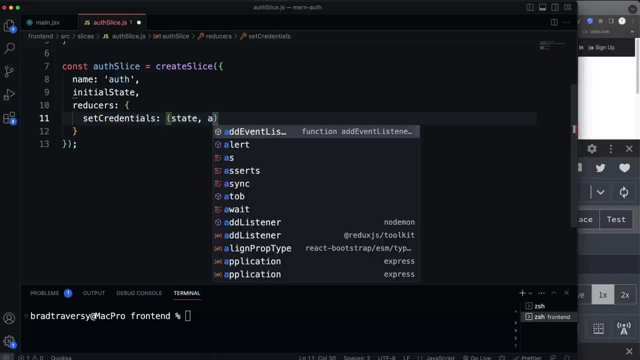 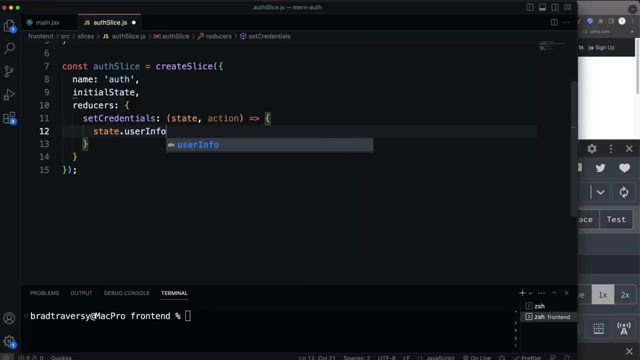 And all of these are going to take in state and an action. Okay, So this is going to be an arrow function that takes in state and action. Now, the action that we pass in is going to be the user data. So I'm going to say state dot- user info. 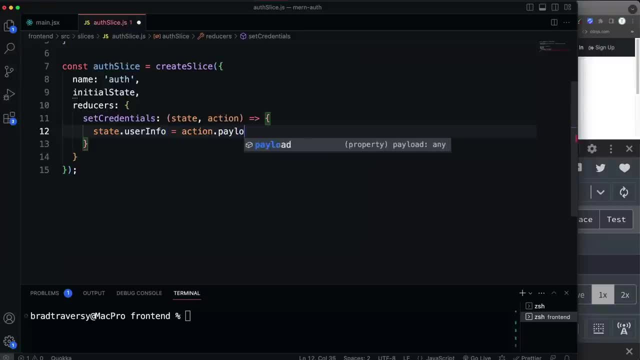 We're going to set that to the action dot payload. Okay, So again going to be the user data, The name, email and ID, And then we want to set that to local storage. So we're going to say set item. 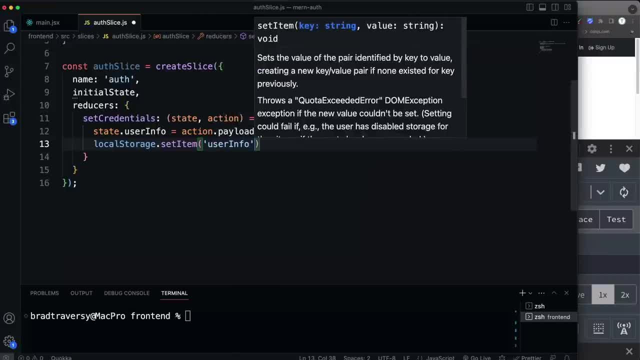 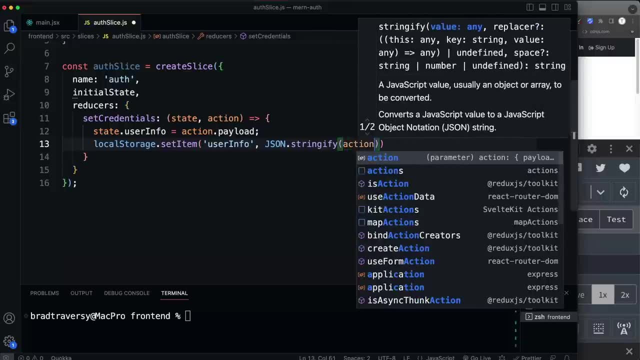 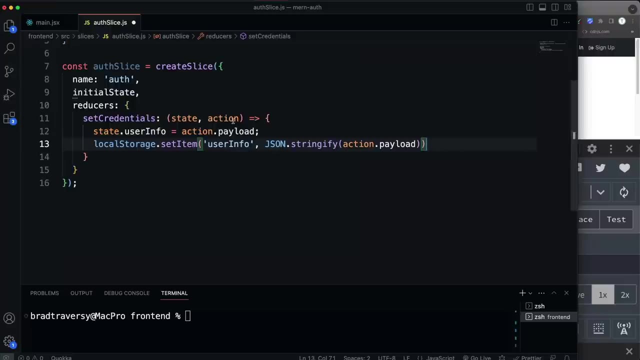 We want to set user info And we just want to make sure we stringify it before we put it in. So json dot stringify And then pass in our action dot payload, Okay. So hopefully that's clear. We're just, we're getting, we're going to have an action, right. 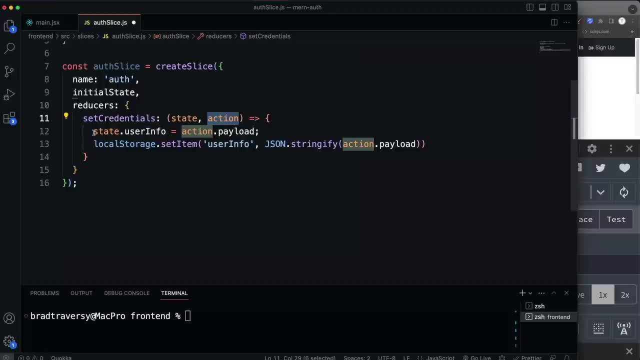 We're going to call this, We're going to pass the user in as the action And then we're going to set it to our user info state And we're going to save that also to local storage And then we're going to have a log out. 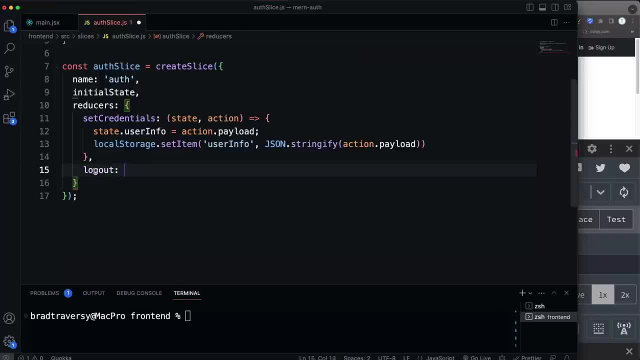 We probably should call this well. I guess it doesn't matter Because we're going to have a log out in the user API slice that makes the request to the back end to log out. This is just basically the front end log out to kill the local storage. 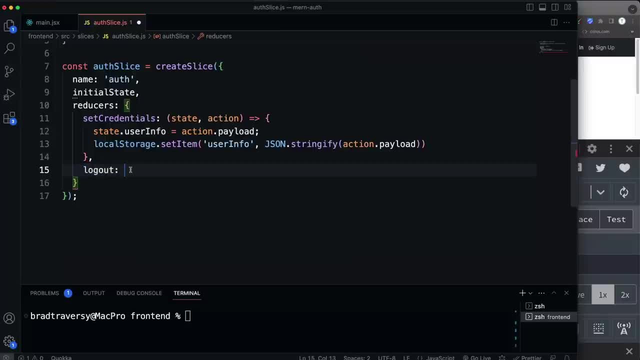 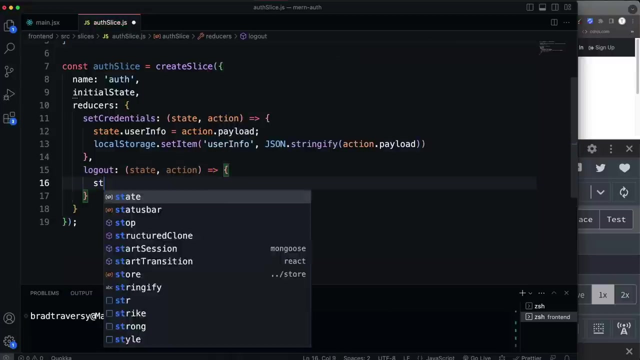 So you could call it like clear credentials. But I'll just keep it as log out. So for that that's also going to take in action. I'm sorry. State and action Right. And then we're going to say state dot user info. 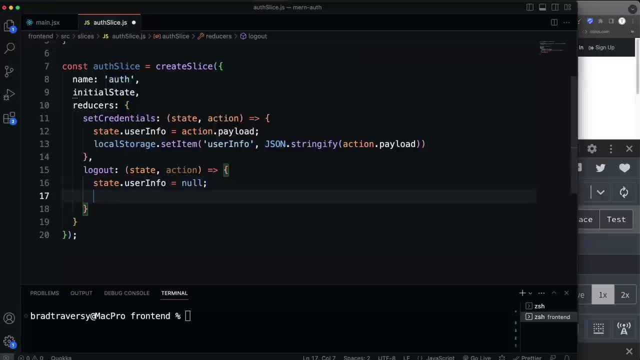 And now we're clearing it. So we're going to set it to null. And then let's say local storage, dot remove item, And we want to remove user info. Okay, So we're clearing it from both our state and local storage. 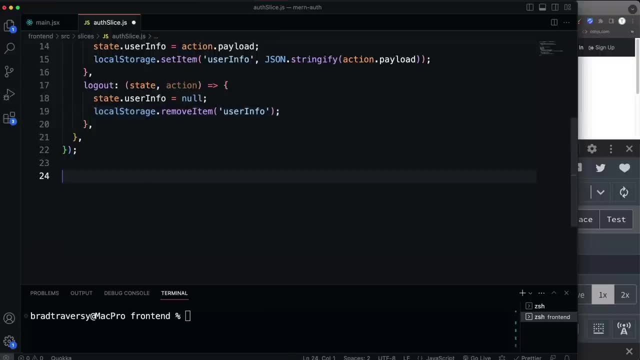 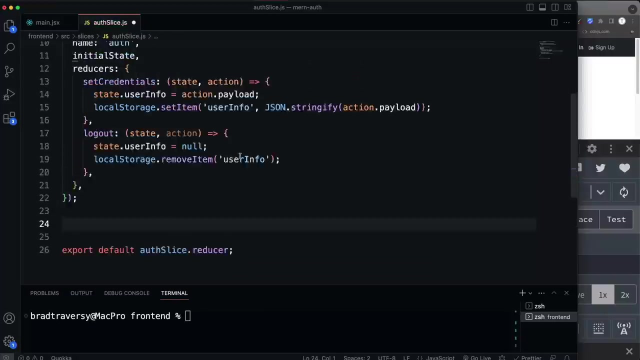 Now we need to export a couple things here. One: we want to export as default the auth slice reducer. So we say auth slice and then dot reducer, But we also have actions right. So when we call these, like if I call this in my login component, my login screen, 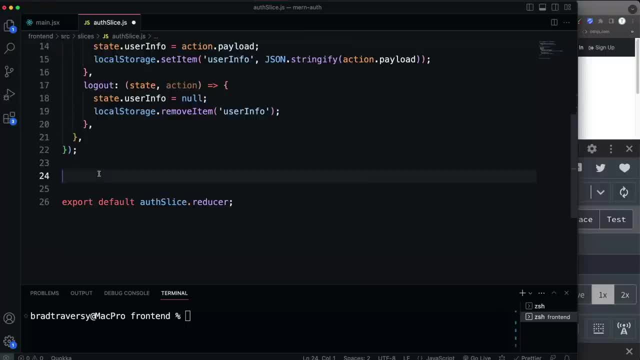 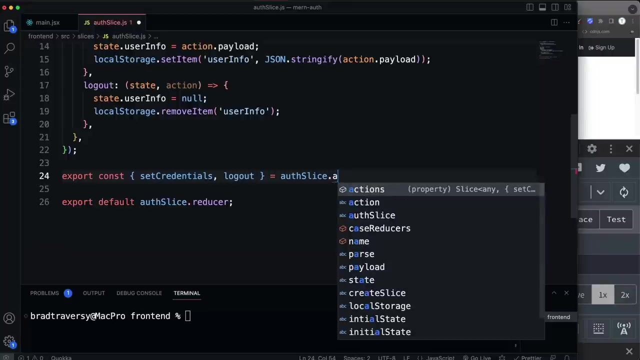 It's an action. So right above that, we're also going to say export const. And then in curly braces we're going to have our set credentials and log out, Okay. And then we say equal auth, slice, dot actions. So actions, when you call this, that's an action. 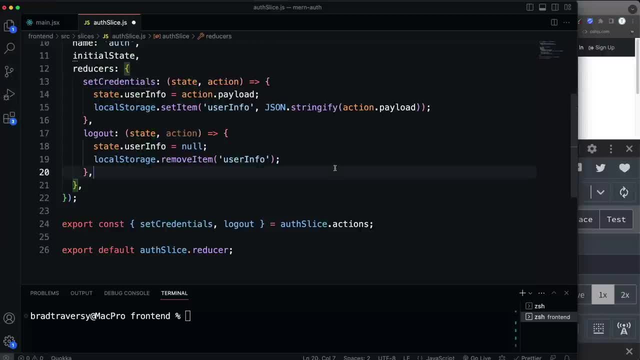 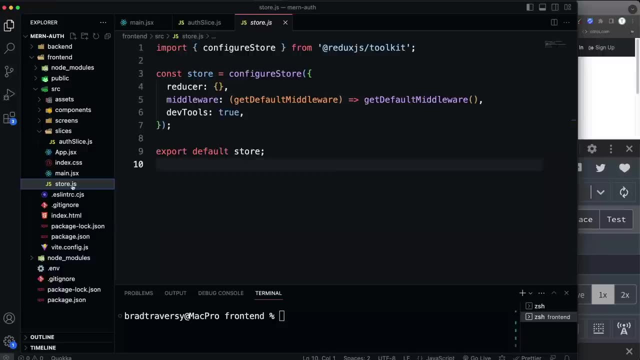 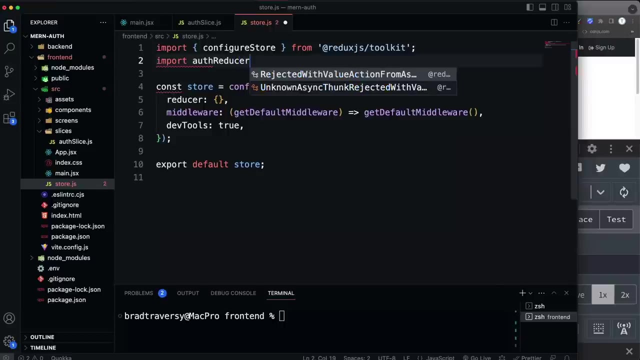 When it changes your state. that's the reducer. So let's save that Now. in order to use this, In order to use any slice, you have to bring it into your store. So let's go to storejs And up at the top here we're going to import auth reducer. 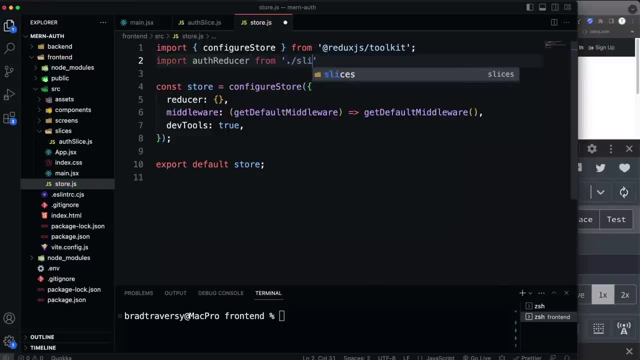 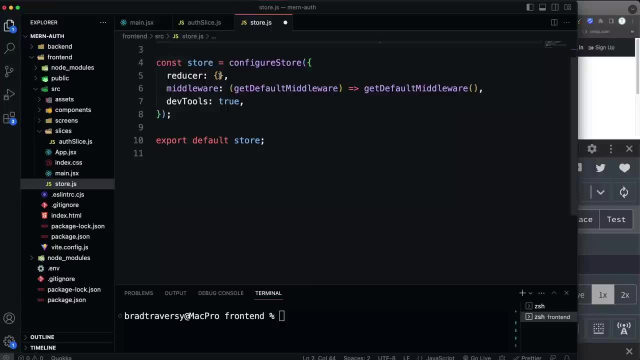 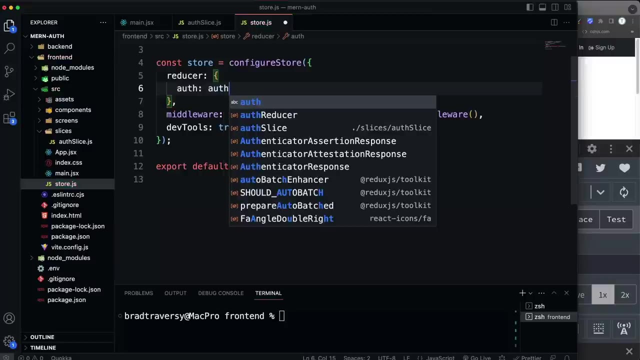 And that's going to be from dot slash slices, slash auth slice And then down here in reducer we're going to say auth, That's going to be the name of this part of our state And that's going to be set to our auth reducer. 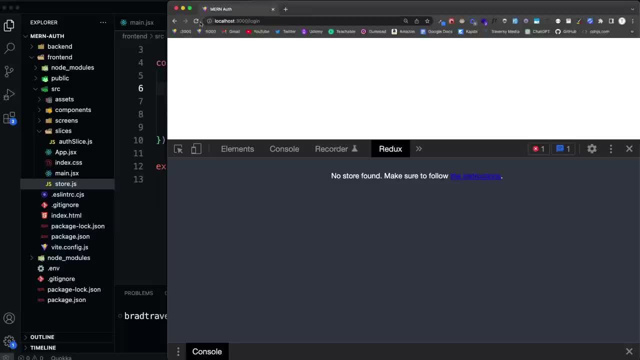 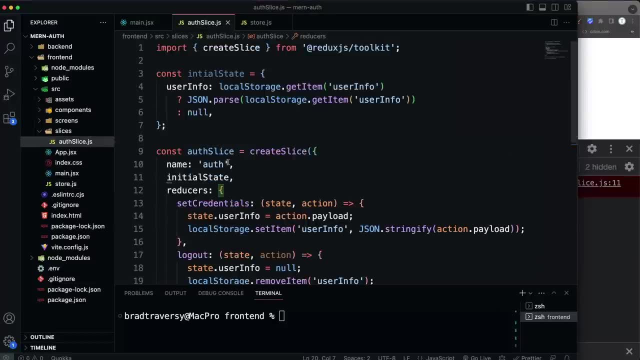 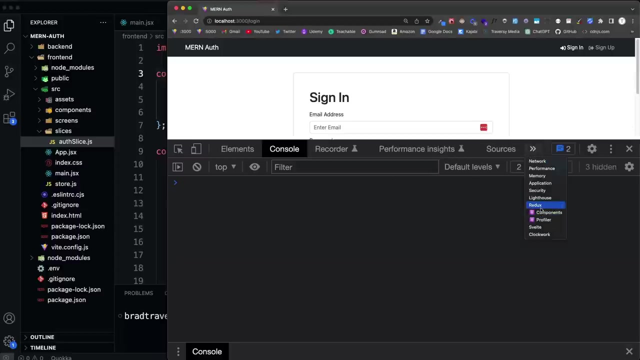 So let's save that. Now let's see what's going on here. Initial state is not found. Oh, I spelled this wrong. Okay, So now let's take a look at our Redux dev tools And now see that we have auth in our state. 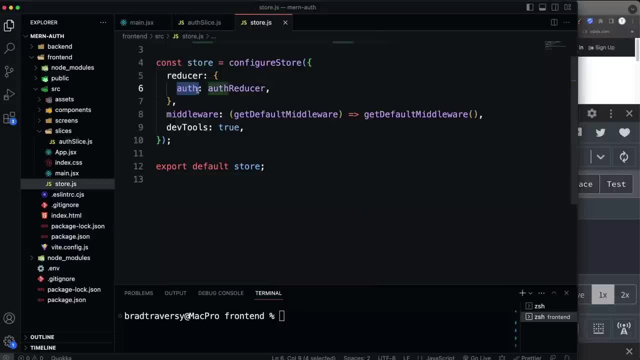 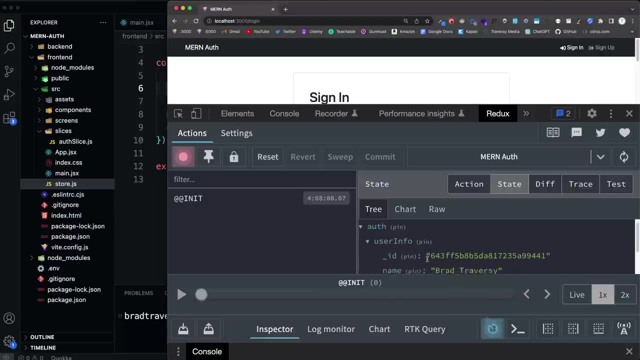 And the reason it's called auth is because in our store we called it auth. Right, If I call this auth one and we look now this is called auth one And then all we have in there is right now- actually I do have a user in there, just because I already had that in this- for localhost 3000.. 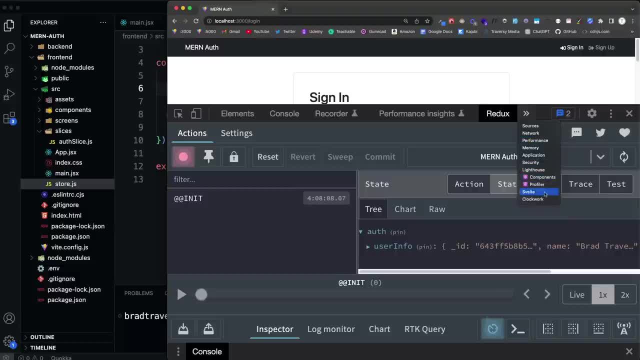 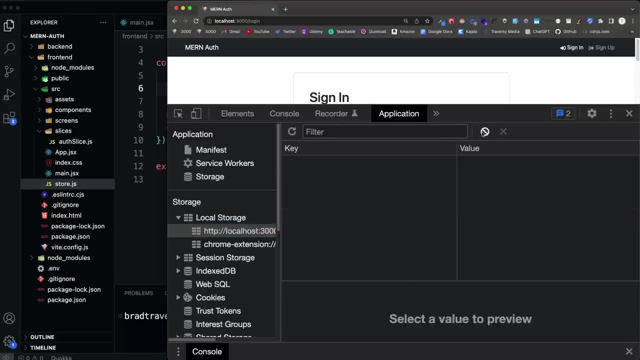 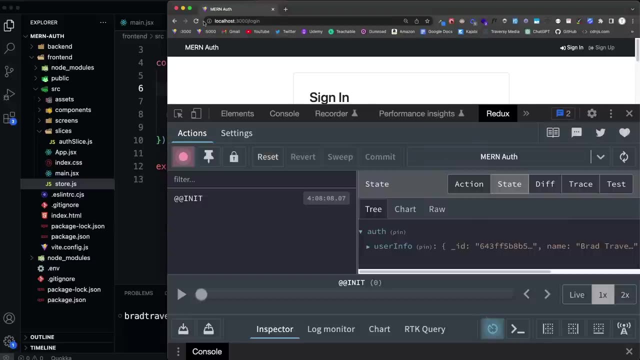 It's in my local storage, So let me just clear that You guys won't have that, So I'm just going to clear it. I'll just- yeah, I'll clear all this out. So now, if I go back to Redux now, my user info is null, which is what you guys should be. 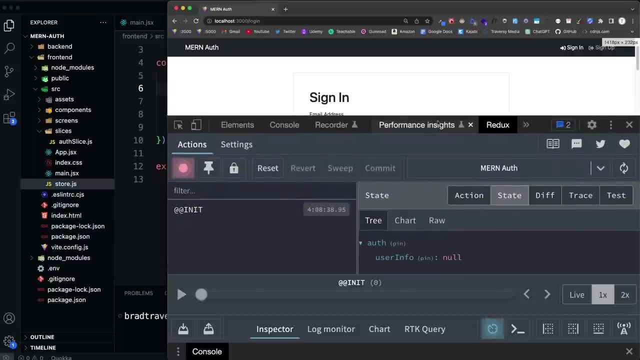 Okay, And then once we go through and we send our request to log in, we make it successful, We get back a response. That user will then be pulled. That user will then be put into this state and into local storage. All right, 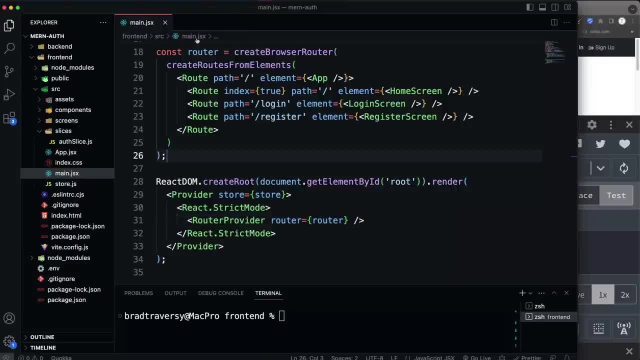 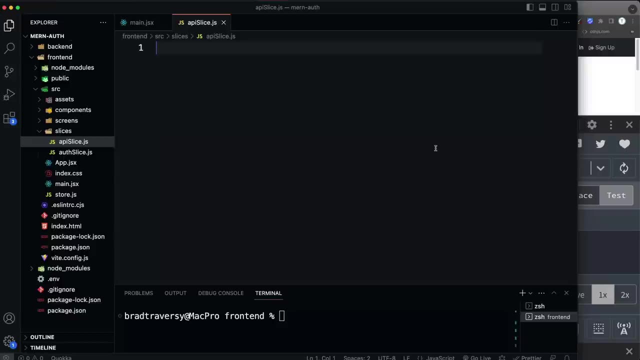 So that's basically the local part of our state. Now we want to have the part of our state that makes asynchronous requests to our back end. So in slices we're going to create another slice called API slicejs. Now, this is going to actually implement the thunk middleware. 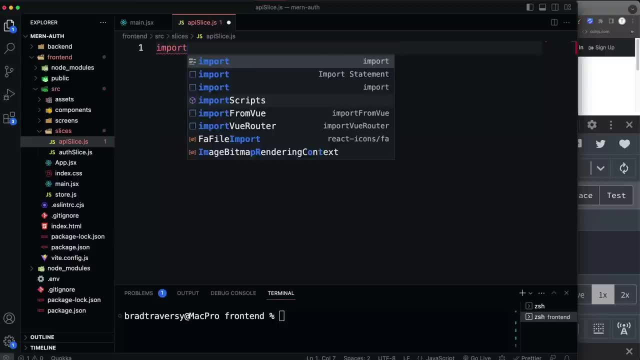 And we don't have to do it manually. Basically, all we have to do here is bring in a couple things. We're going to bring in create API And we're also going to bring in fetch base query. And that's going to be from Reduxjs slash toolkit. 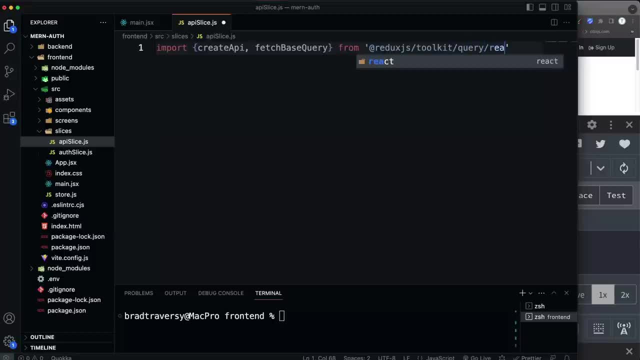 But you also want to do slash query and then slash react, Because under the hood it uses RTK query, which is a library for interacting with the back end API, And the thunk middleware is built in, So we don't have to manually add that either. 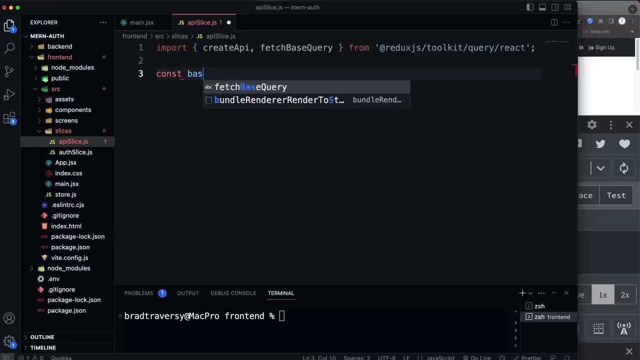 But there is some setup here, There is some boilerplate. So first off, we're going to create a variable called base query. Set that to our fetch base query And in that it just takes an object with a base URL And for us it's just going to be an empty string. 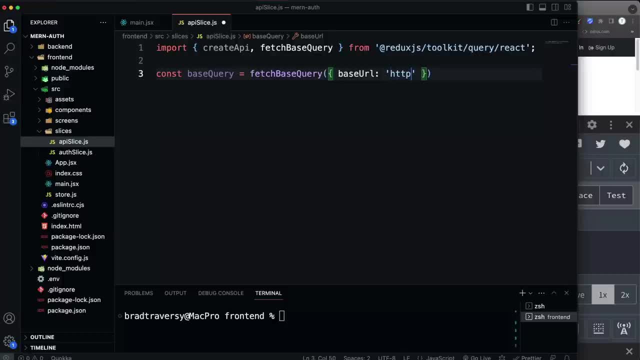 Now, if we didn't use a proxy, we would put like HTTP localhost 5000.. Because we would want that before every call. But for us we're just going to keep that as an empty string because we're using a proxy, And then we're going to export const API slice. 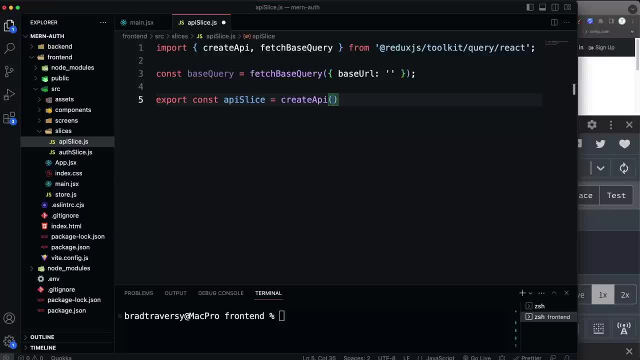 And then set that to create API which is going to take in an object with our base query, So base query. And then we also have a concept of a concept of tag types, And this has to do with caching, Because sometimes you might have like blog posts and stuff. 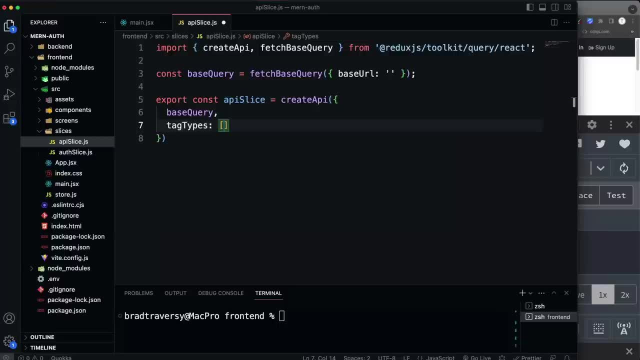 where you don't want to make a fetch every single time. You want to cache them and use that data. So the only tag type we have is user. If we had products or blog posts or something like that, then we would add those as tag types. 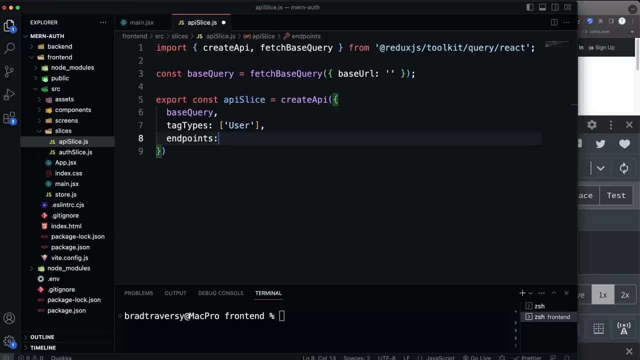 And then we also have endpoints, which is going to be just an arrow function, And this takes in a builder. So basically, there's a built-in builder to make our requests, And when we make our requests, it won't be from this file. 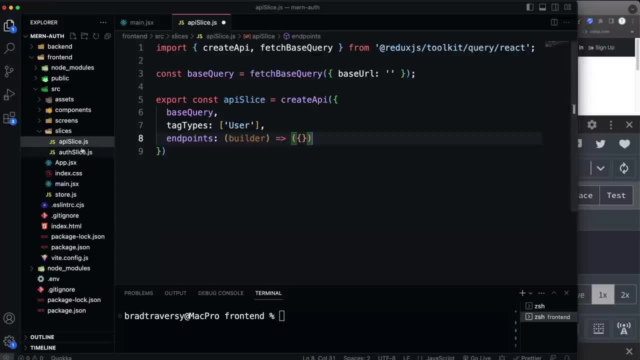 You can think of this as like a parent to any other API slices. So for this particular application we just have a users API slice, But in the course project we have a products API slice, an orders API slice and a users API slice. 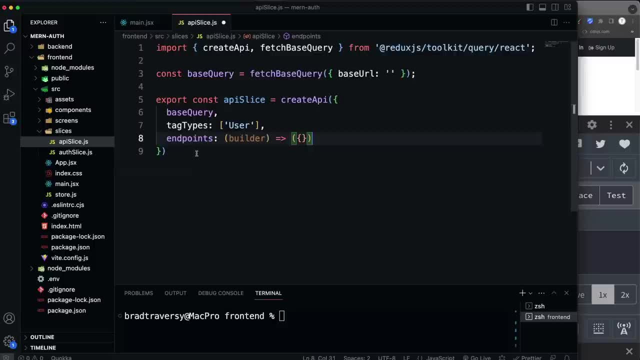 And all those have their own endpoints That you know contribute to the back end Or interact with the back end. So let's save this. That's all we have to do here, And then we just want to bring it into our store. 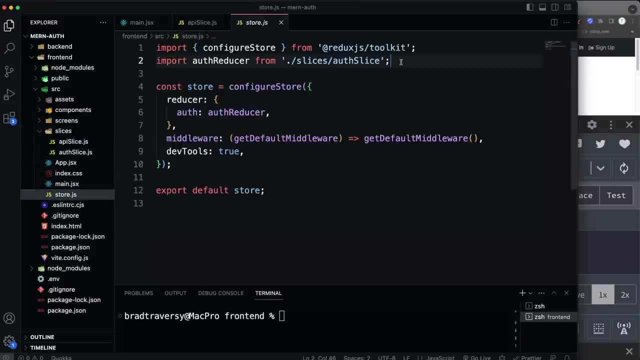 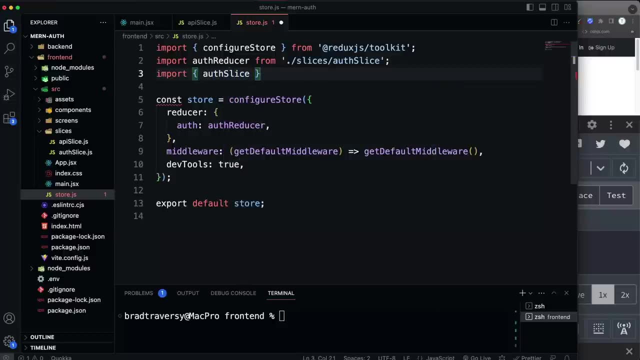 So in storejs we're going to import auth slice- Yeah, I'm sorry, not auth slice, API slice And that's going to be from. and then we want to go: let's see dot slash slices, slash API slice. 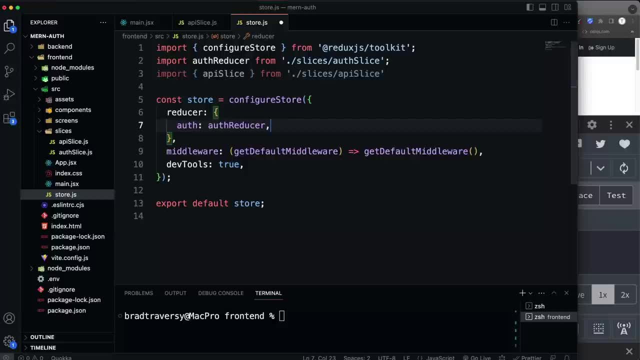 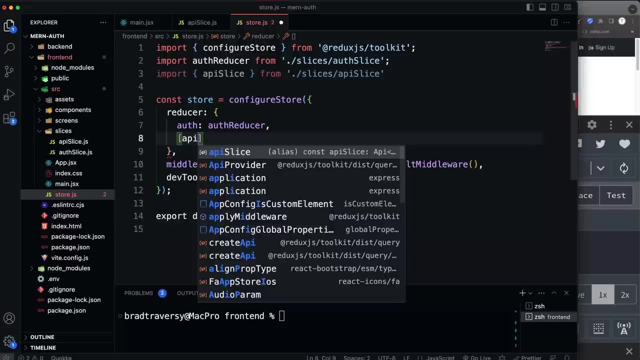 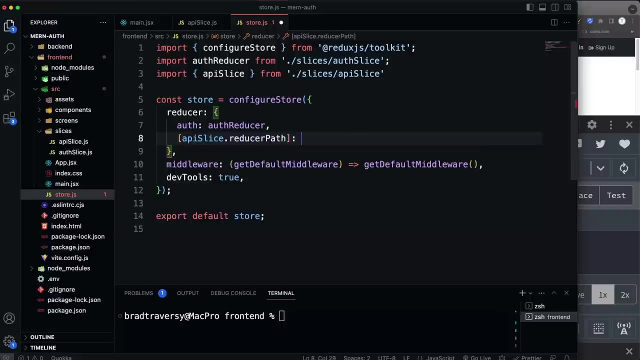 And then to add it, let's go in the reducer object And the way we add it is as an index we do brackets: API slice dot and then reducer path And then colon and then API slice dot- reducer. 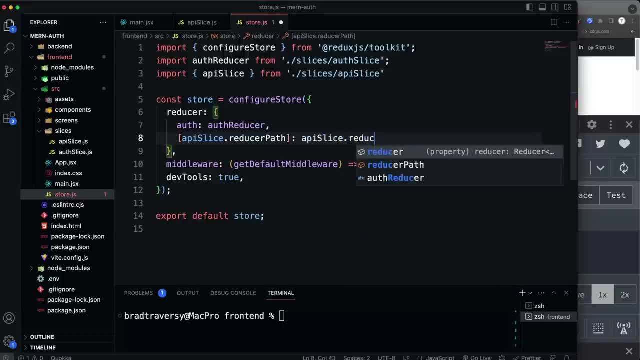 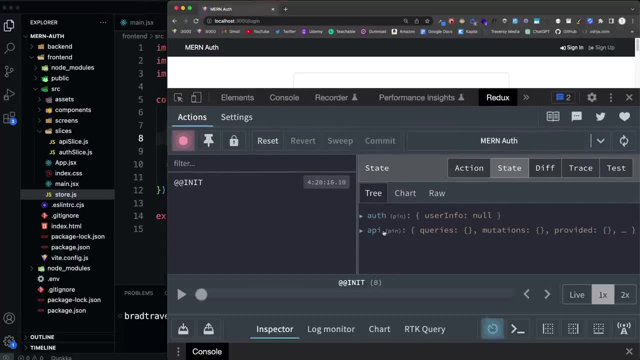 So what that will do is it's going to say: you know so what that will do. if I save that and now we take a look at our state, you can see we have this API And this has a whole bunch of stuff associated with it. 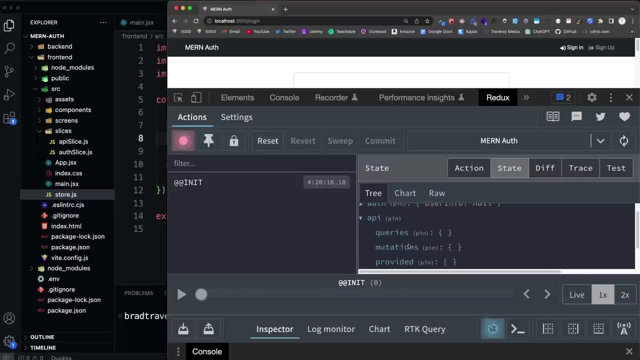 So queries, mutations, subscriptions, So it gives us a lot to work with without us having to do the extra work. And queries are basically, you know, fetching data from the back end. If you're going to fetch your blog, post products, whatever. 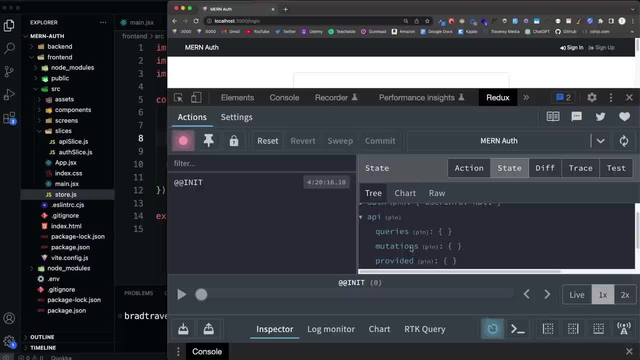 that's going to be a query. Mutations are doing something in the back end, like adding a user, Like when we register or log in. those are going to be mutations, All right, So now that we have our API slice, we can close that up. 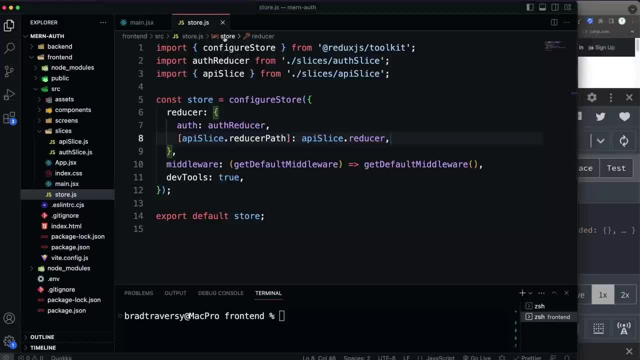 We don't have to touch that again. We don't have to touch. actually, we do have to add the middleware Because, remember, we have the thunk middleware And basically all we have to do here is add on to this. So at the end of this, get default middleware. 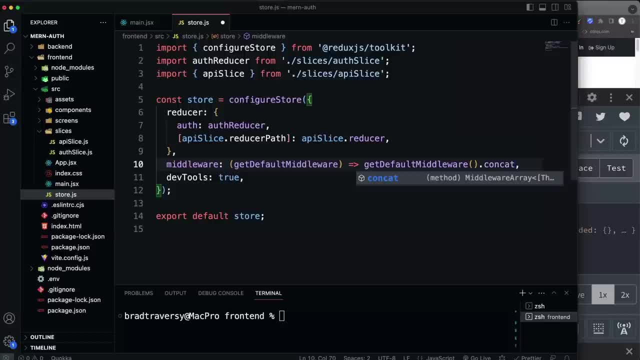 we're going to concat, So let's just say dot, concat, And then we can pass in here API slice, dot middleware, And now we shouldn't have to touch this file again. All right, Now we're going to have another file. 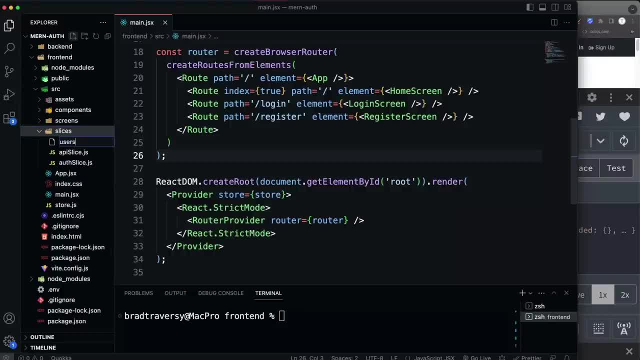 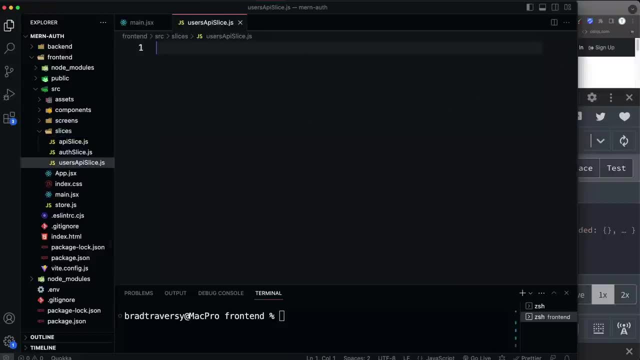 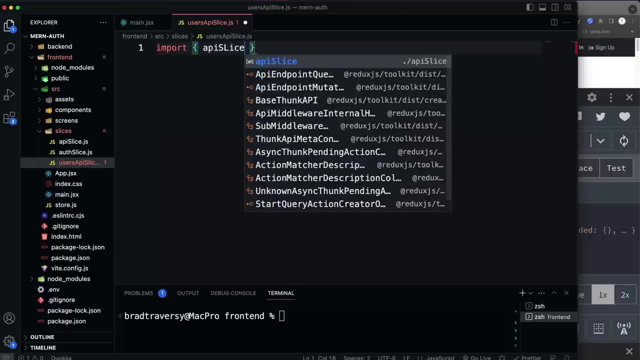 another slice in here called users API slice dot js, And this is where we'll have all of our endpoints to work with the back end. So we're going to import the API slice, Because that's like I said. you can think of that as like the parent slice to this. 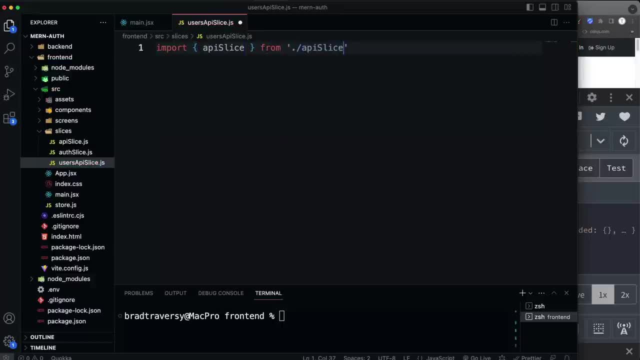 So that's going to be from dot slash API slice, And then let's create a variable for our users URL, So underscore URL. You could put this in a separate constants file if you want, But since we only have one resource, which is users, 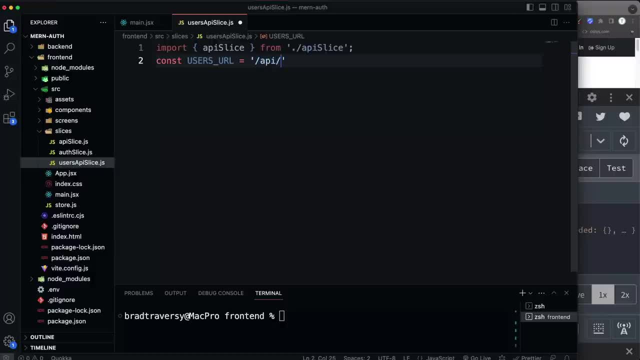 so I'm just going to put it in here And that's API slash, users, Right, Because all of our back end endpoints start with API users. So let's go ahead and create our slice here. We're going to say export const and then users, API slice. 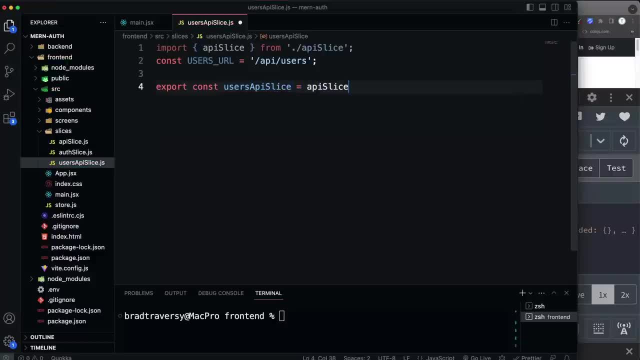 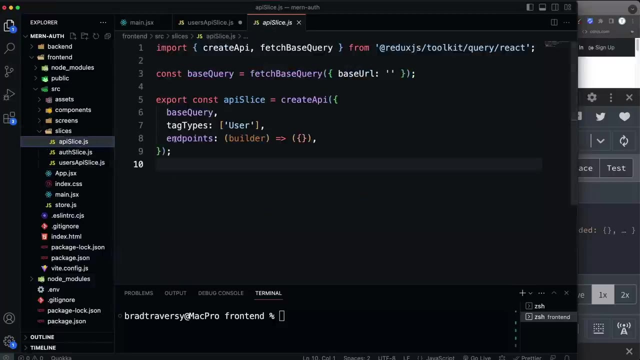 And set that equal to API slice, And then there's a method called inject endpoints. All right, So basically, what this allows us to do is create our own endpoints in this file And it will inject them into this, into the endpoints here. 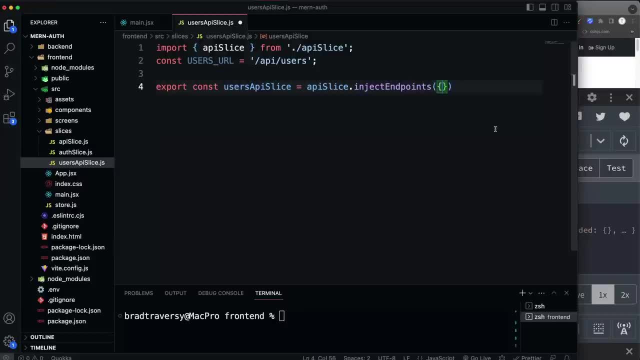 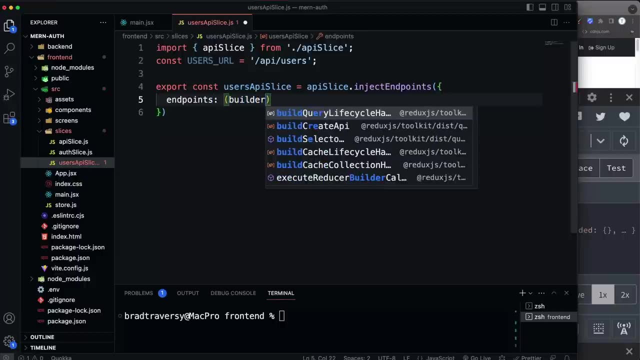 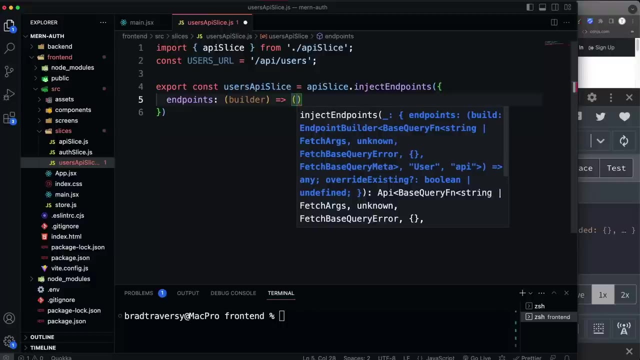 So we're using dependency injection. So in this inject endpoints we're going to have an endpoints function which also takes in builder, So we want an arrow function: pass in builder. We're going to set this to an object, So we want to have parentheses around object. 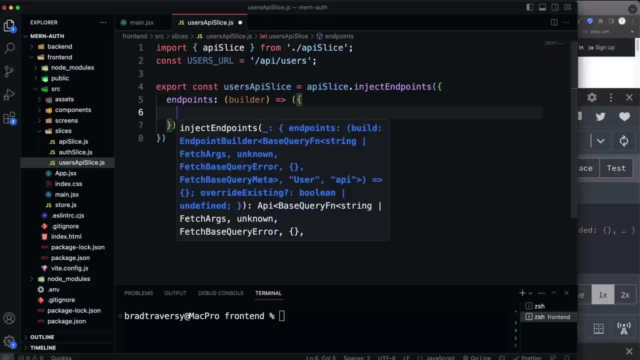 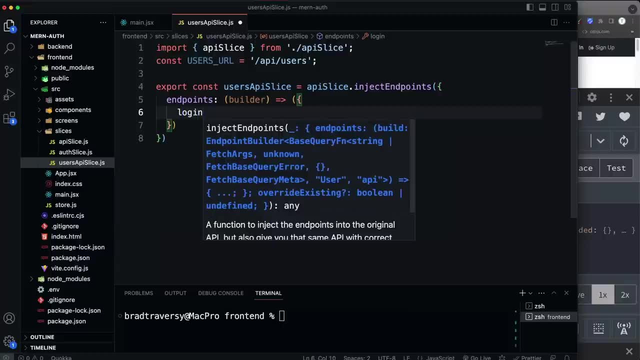 And then we're going to have our curly braces And then in here we can put all of our queries and mutations. So the first thing I want to do is the login. So I'm going to call this login, We're going to use the builder and create a mutation. 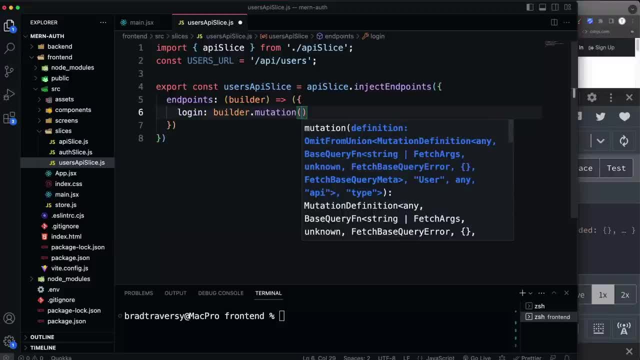 And I know this might be really overwhelming if you've never used this before- But once you see the flow of this, once you see how we add the login and the register and the update profile and all that, you'll see how easy it is to add functionality once all this boilerplate crap is done. 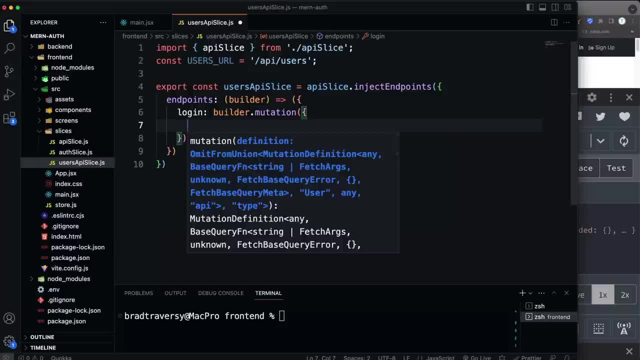 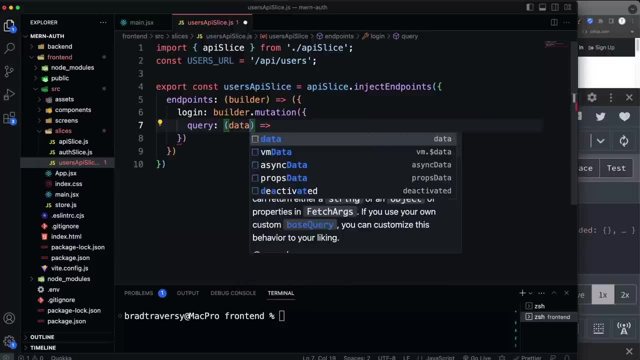 So for this mutation, we're just going to pass in an object And it takes in a query And that's going to be a function And we're going to have data passed in because it's a login. So remember, we're going to be sending an email and password. 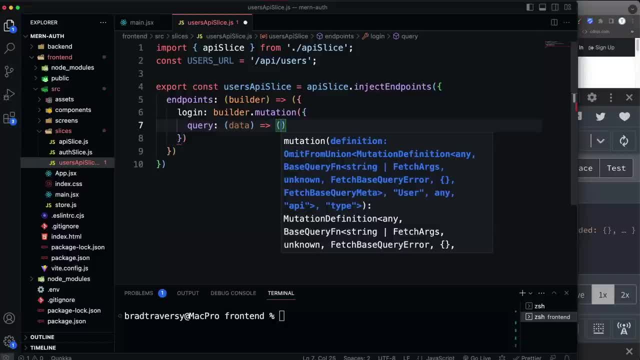 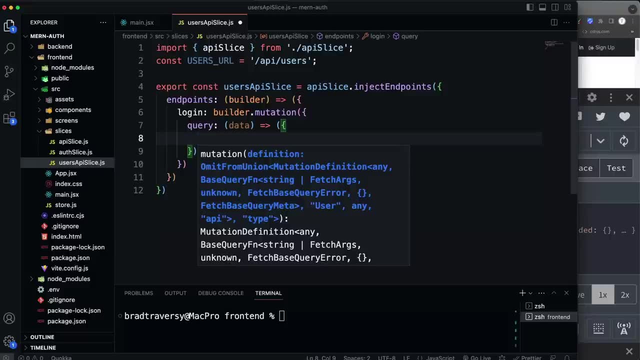 That's going to be what that data is, And then we're going to set that to an object. So parentheses around our curly braces, And in here we're going to have a URL that we want to hit, which is going to be our backend URL. 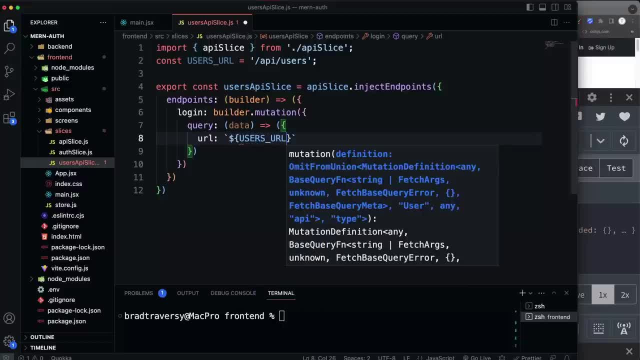 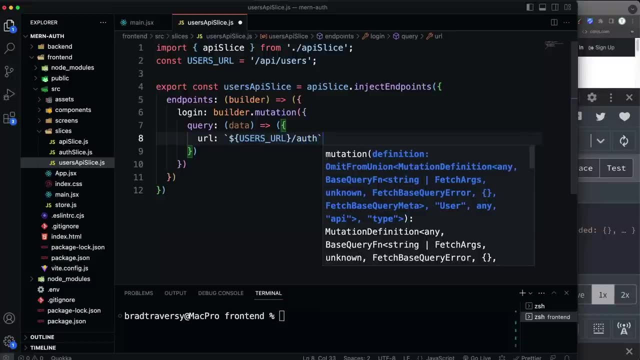 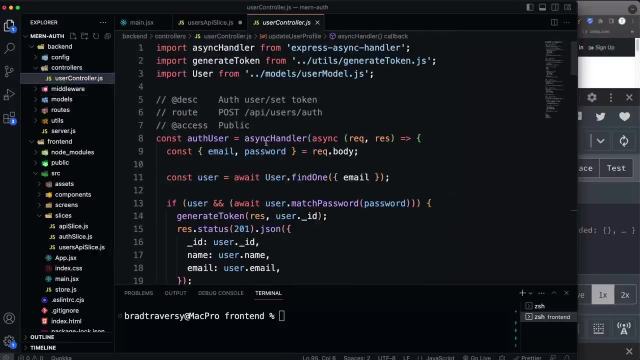 So we're going to have users underscore URL, which is API slash users, And then we're hitting the auth route. So we're going to put slash auth Because, remember, what we're hitting is in our controller, the auth user. that's the route to this auth user. 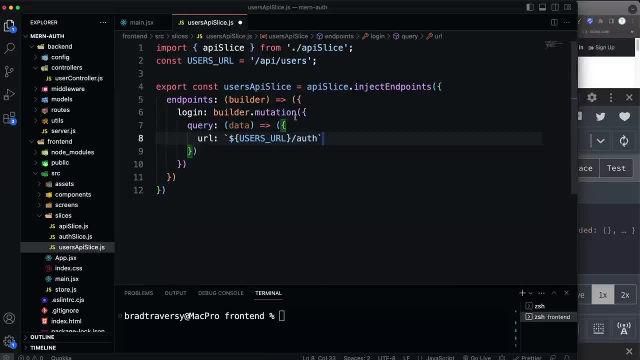 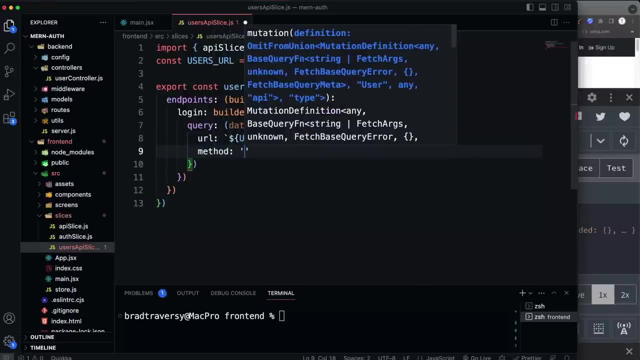 Because this is what I'm hitting right From the front end, from this slice. So we have the URL. Now we do want to specify the method, because by default, it will be a get request. I want this to be a post request. 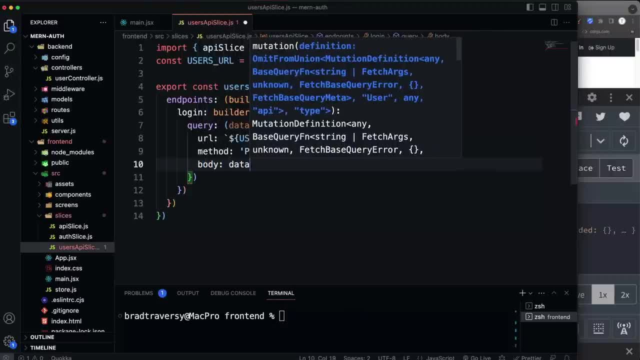 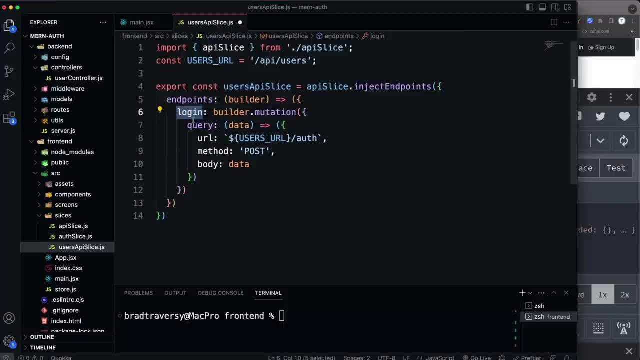 And then we also have. we need to send the body, which will be the data passed in. So now, in our form, we just have to dispatch this login action or this endpoint, But we do have to export it. So let's come down here and say export. 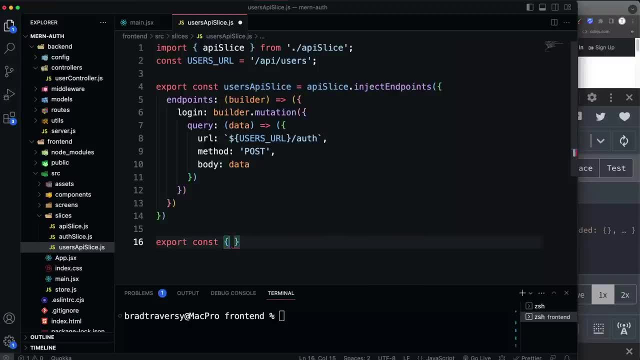 I'm going to say export const. Now there's a specific convention to export these mutations and queries. Since this is a mutation right, We need to say use and then the name of it. So in this case, login And then mutation. 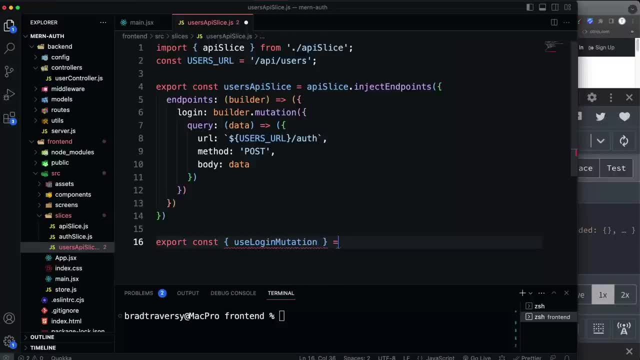 Okay, So that's going to be the name of the mutation, And then we set that equal to user, our user's API slice. Okay, Now if this were a query, like if we said build or query and we were fetching some data? 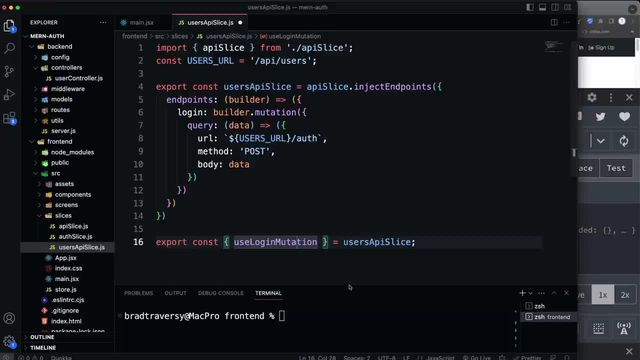 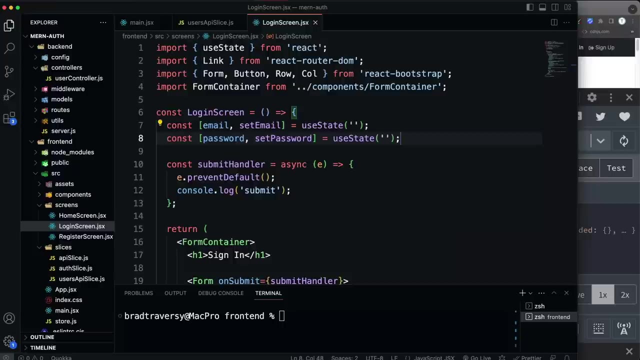 then this would be use login query instead of use login mutation. So it's very important that you use the correct convention. So now we can save that And now we can go back into our login screen and start to implement it. So let's go into login. 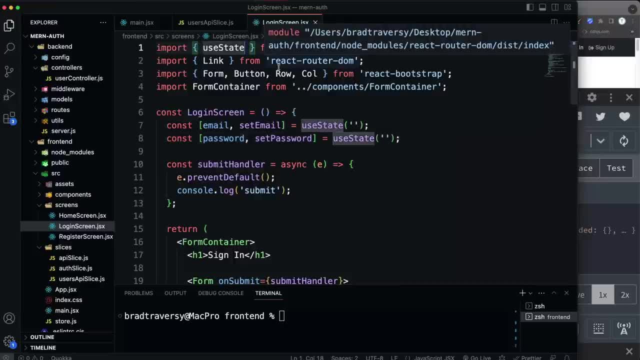 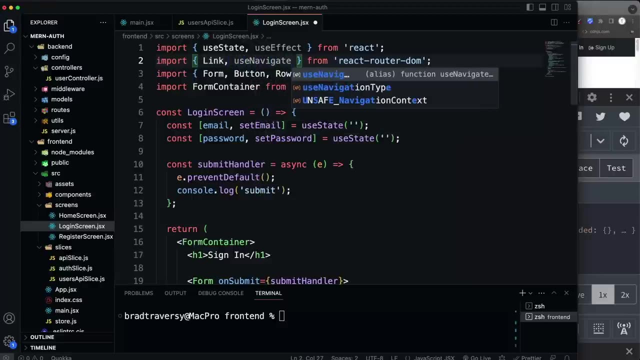 And let's see. we're going to bring in a few more things. We do want a use effect. And then let's see link: We're also going to navigate from, you know, from this page, So I'm also going to bring in use navigate from react-router-dom. 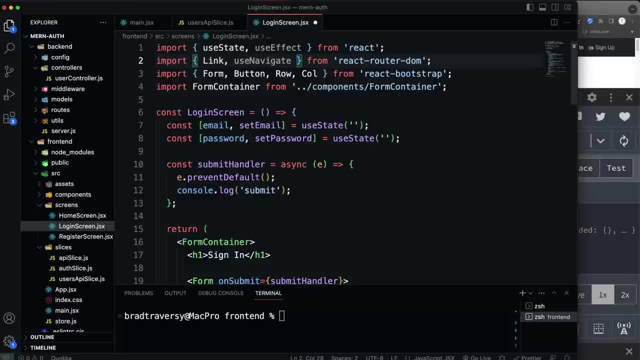 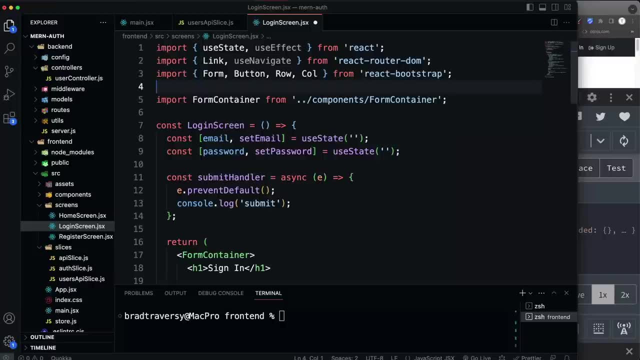 And then let's see we have. We're going to need to dispatch an action And we're going to need to get data from the state. We need to get our user data. So we're going to import two hooks from react-redux. 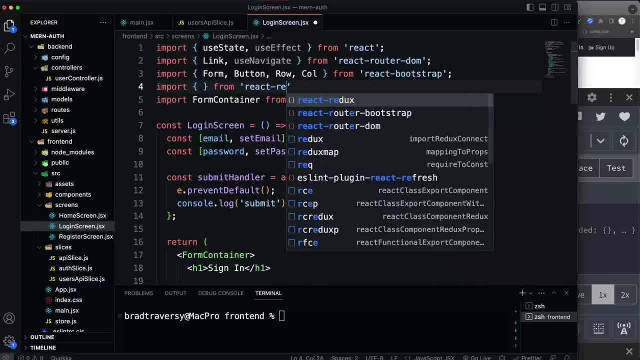 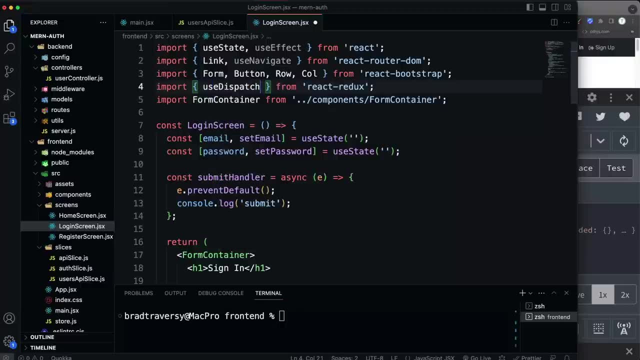 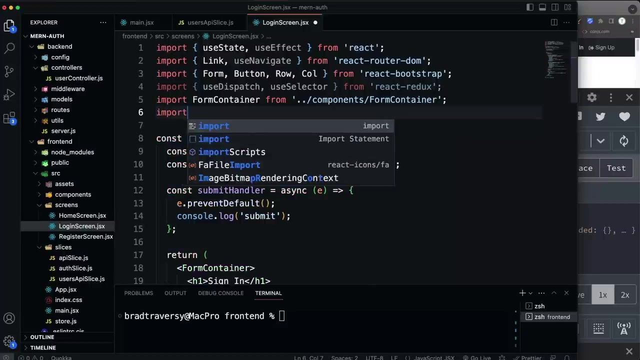 So from react-redux, And those two hooks are use dispatch and use selector. So use dispatch, obviously that's to dispatch an action, And then use selector is to select from your global state. Okay, then we want to bring in our mutation that we just created. 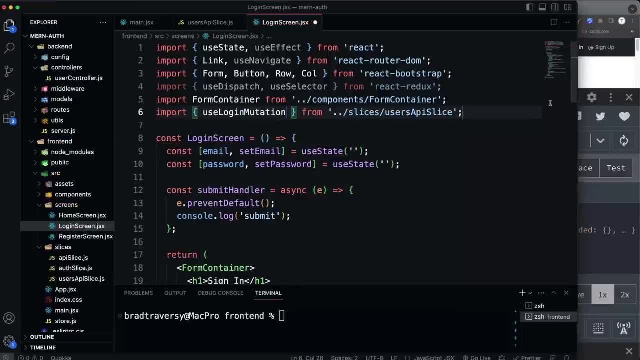 So say, use login mutation. That's going to be from our user's API slice. And then I also want to bring in our set credentials from our auth slice, Because after we hit our backend we get our user data. we then want to call that set credentials. 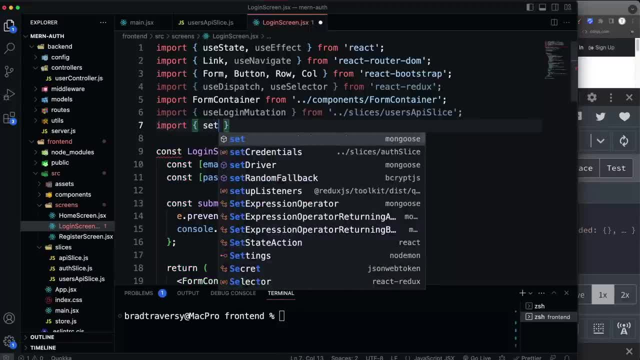 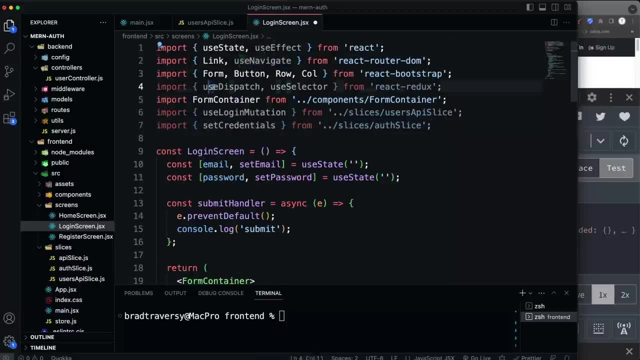 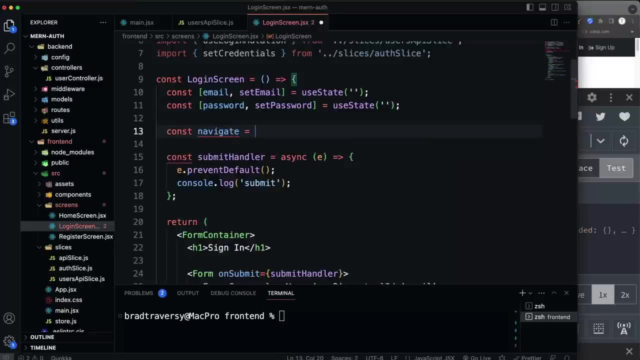 So let's say import set credentials from our auth slice. Okay, now for use navigate and use dispatch. we need to just initialize the variables for those. So I'll say const navigate equals use navigate, And then let's say const dispatch equals use dispatch. 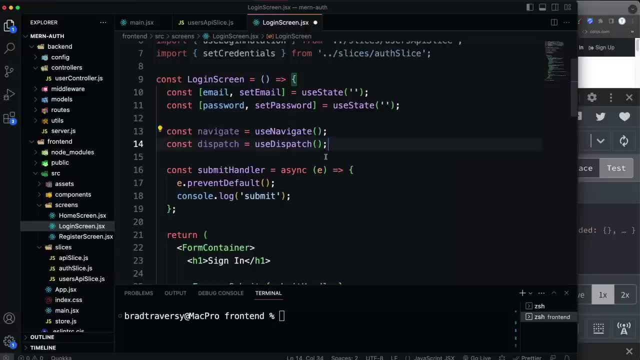 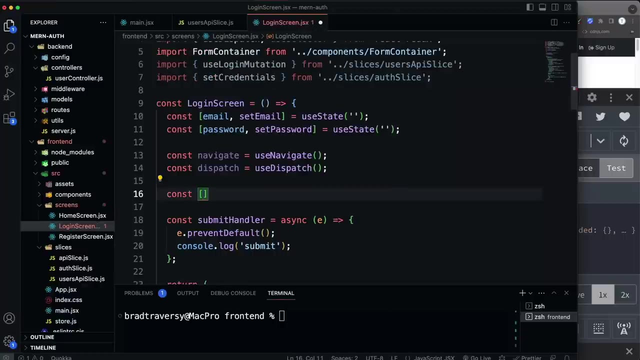 So we can use those functions. All right, now let's see To get the function to call to fire off our mutation. what we'll do is say const and then in brackets and then set that to use login mutation. So in here the first thing we're going to pass in: 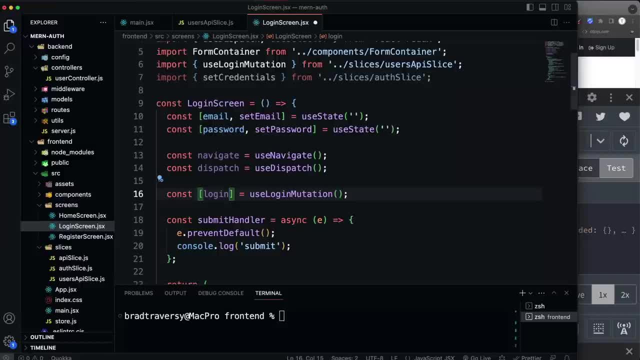 is the name of the function to call, which I'm going to call login. You could actually call this anything. And then what's great about this is we can also, in curly braces, we can get is loading, So we don't have to handle the loading state right. 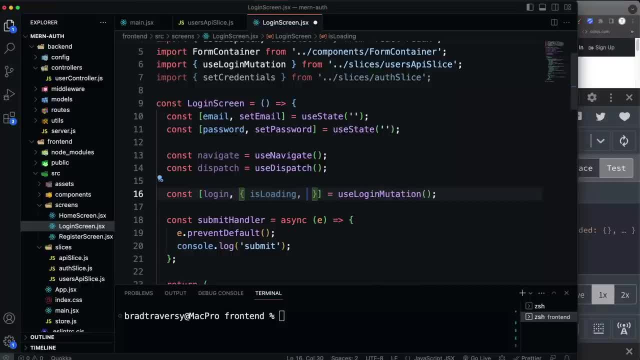 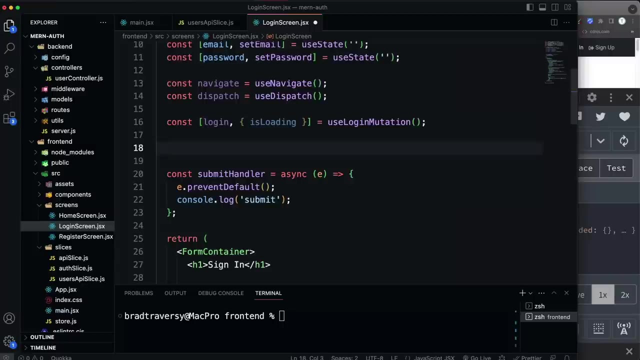 It just. it's there just by default. We can also get the the error if we want. So it's nice because you don't have to manually set all those parts of your state. Now to get the user data, we can use the use selector hook. 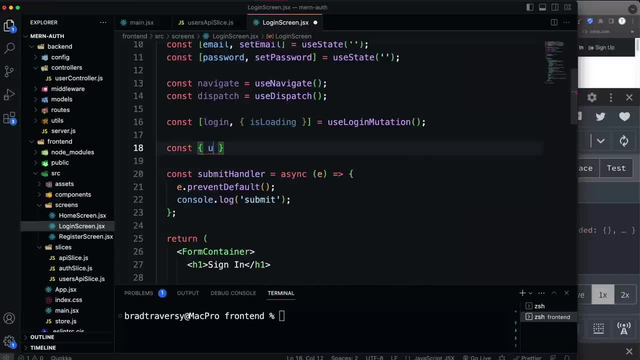 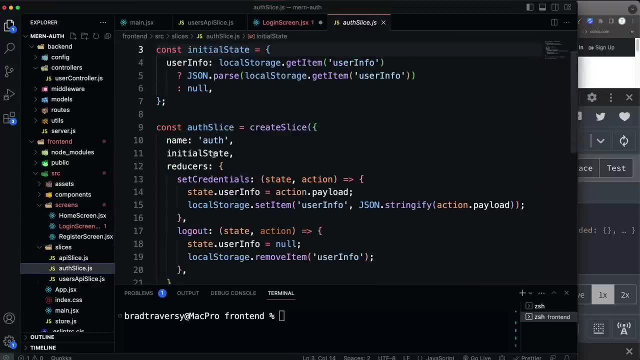 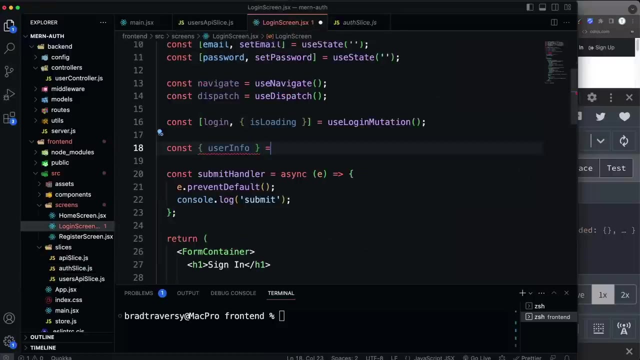 So let's say const, and the state that we want is going to be the user info, which is, you know, if we look in our auth slice, so right here, user info. So in our login screen we can say user info. 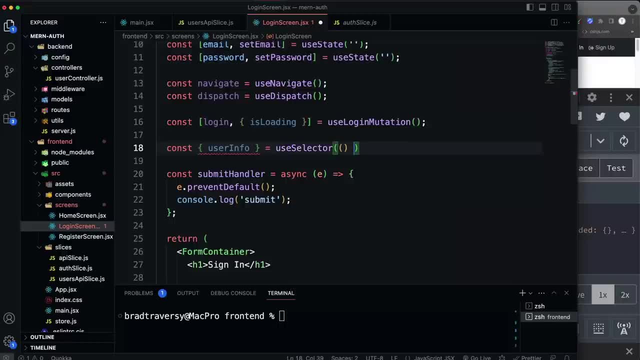 and then set that to use selector That's going to take in a function that takes in our state, and then we just set state dot and then whatever part of our state we want. So we want this right here, auth, because that's what has our user info. 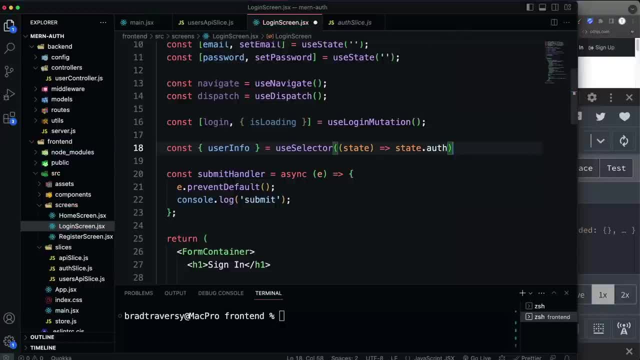 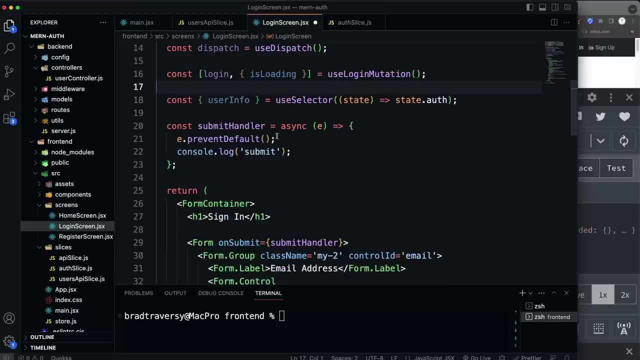 So we just simply do state dot auth. All right, Now let's see. The next thing I want to do is, if there is user info, that means we're logged in. So I want to redirect to the home page if we're logged in. 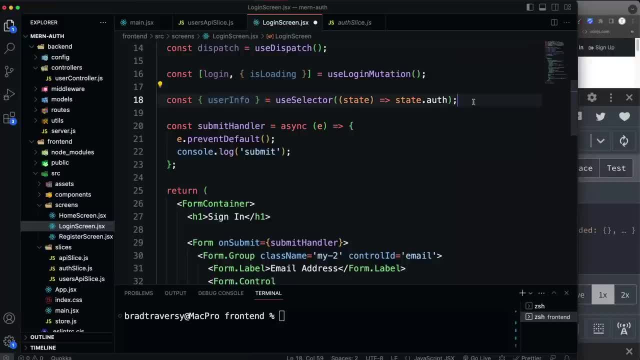 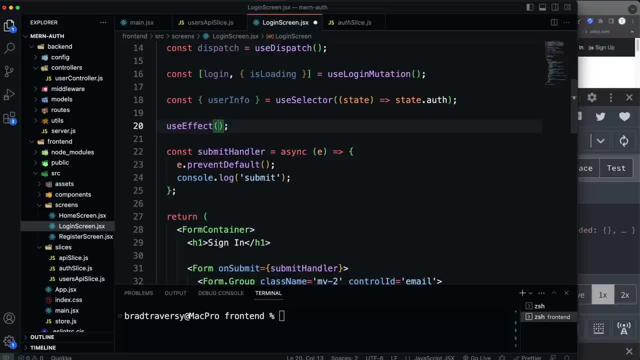 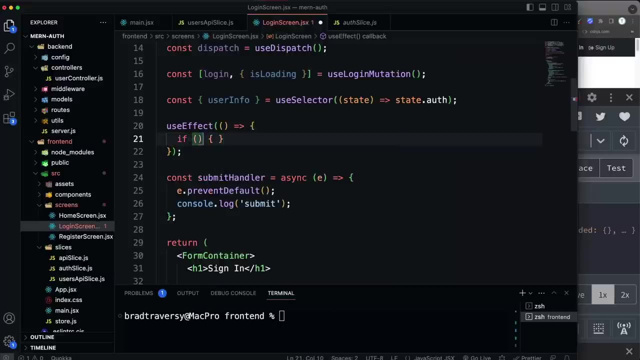 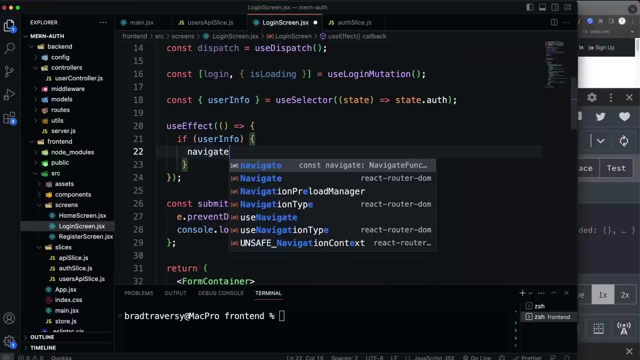 and we go to the login screen. So for that we'll do a use effect. So let's say use effect and pass in our function, and then we're going to say, if so, if user info, then we're going to navigate to the home screen. 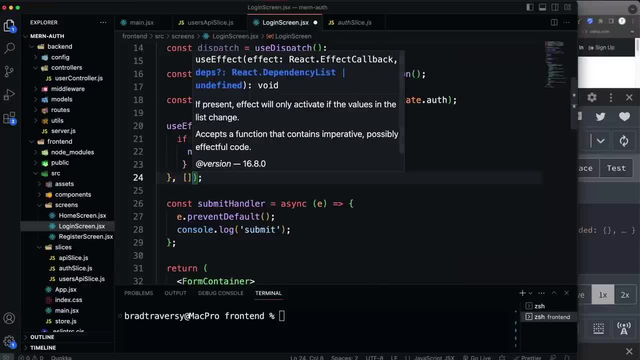 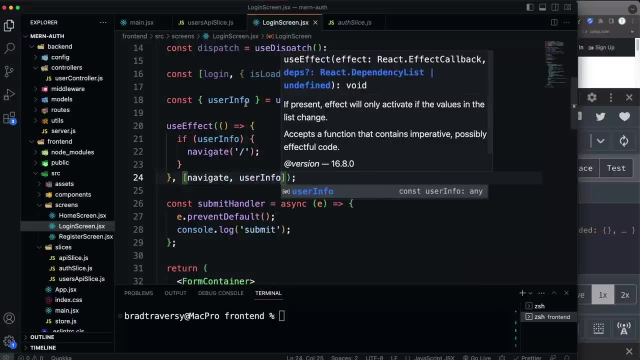 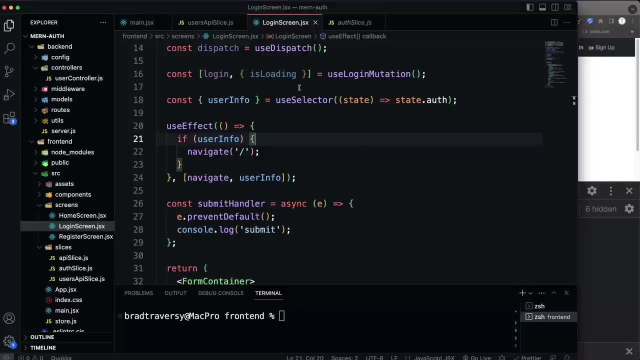 All right, And that's all we need in here. Now we do have to add those as dependencies to our use effect. so we want to add navigate and user info, All right. So if I just save this now, I just want to make sure that we don't have any issues here. 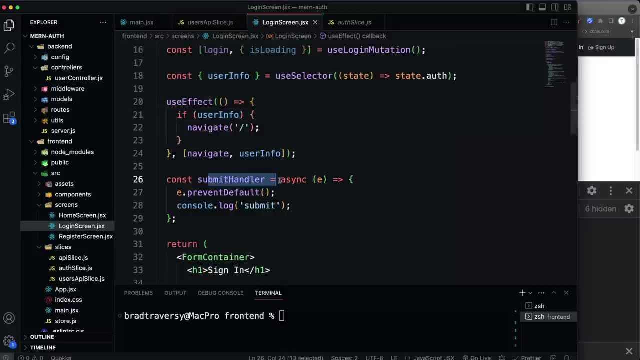 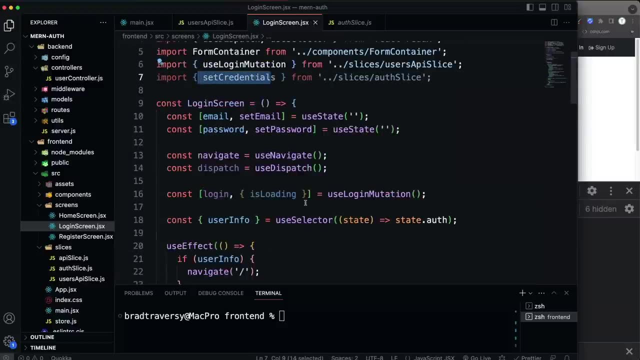 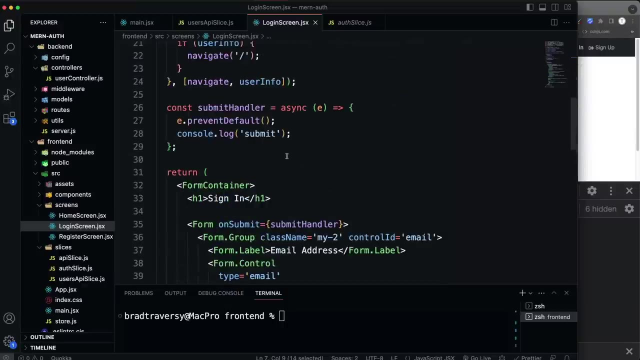 Okay, So now the only thing left to do is to log in to our submit handler. We have login, and then we also have our set credentials that we brought in. So now let's go. let's see, Yeah, we'll just go down to our submit handler. 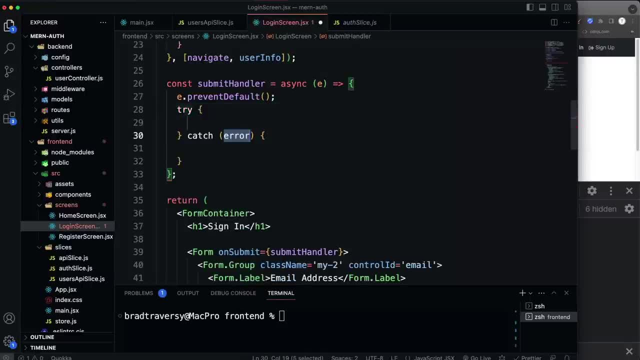 get rid of this console log and I'm going to do a try catch, And in the try we're going to say const res, and then we want to await on login. Okay, So what I'm doing is I'm calling this login. 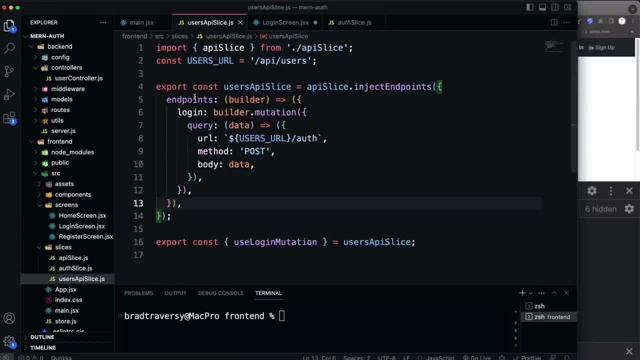 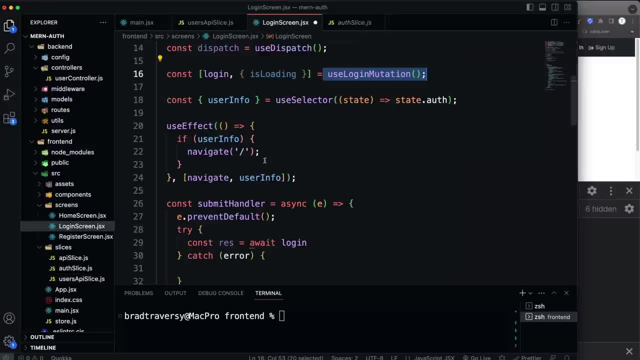 which is from our mutation, which is in our API slice right here. So I'm making, I'm going to make this request, this post request. So back in the login screen, let's say we're going to call login and remember. 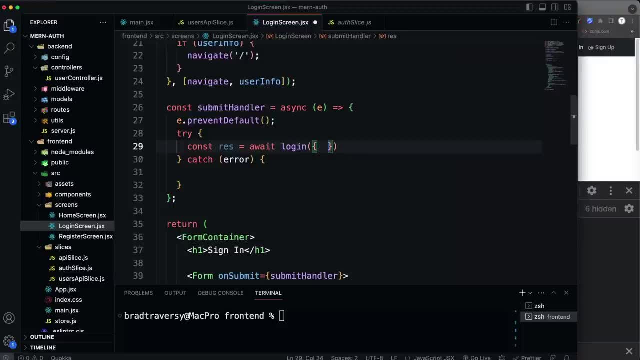 it needs to take in the data of the username and password. So we're going to pass in an object with- I'm sorry, not username, email, email and password, which are coming from the form Right, And then we just want to add on the end of this dot. unwrap. 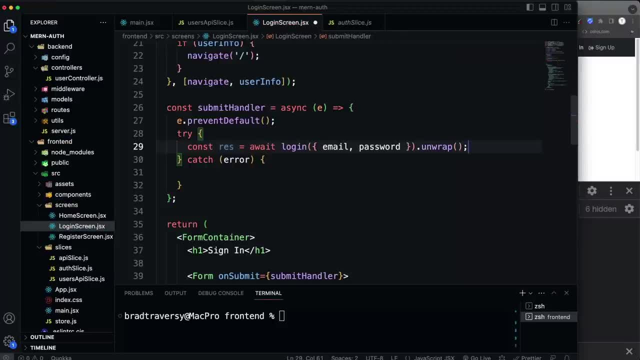 because this will return a promise. So what this basically does is it unwraps that that promise. So that takes care of calling you know, to the back end, And the response from the back end is the user which is going to be put into this res variable. 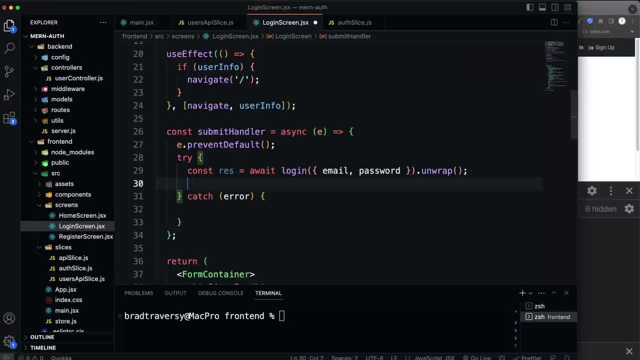 So then what we want to do is then call set credentials, because, remember, that will set it to local storage and to our state. So we want to then dispatch set credentials, And what I'm going to pass in here is just an object. 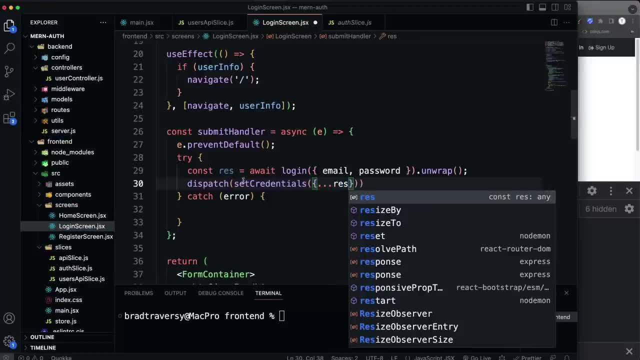 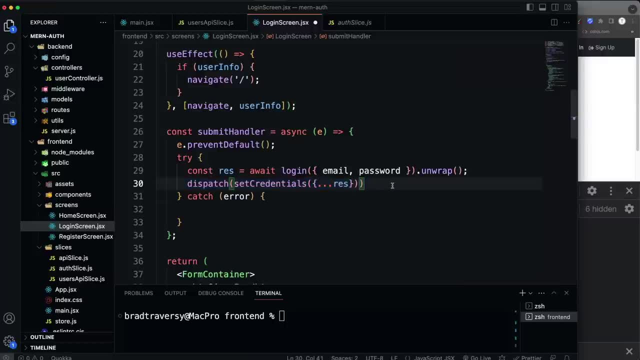 And we're going to spread across that res data, which is the user data. So now we're just setting, setting the user to local storage and to our state, And then, finally, we'll navigate to the home screen. All right, Now if there's an error. 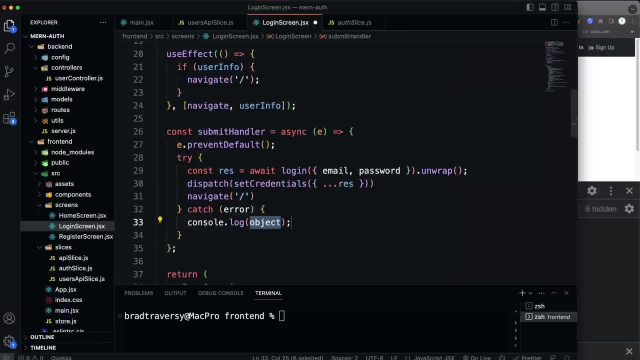 so in the catch, I'm just going to do a console, I'm just going to do a console log of I'm actually going to change this to just err, because we should be able to get errdatamessage or errerror, All right. 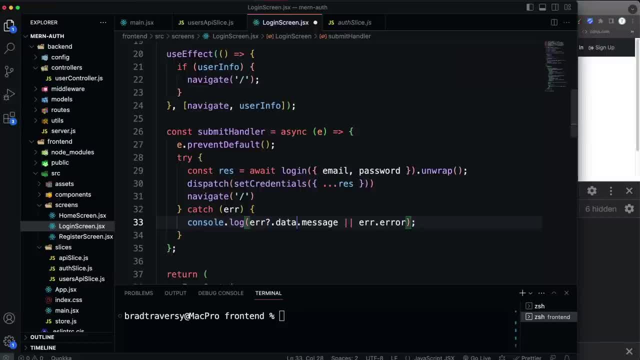 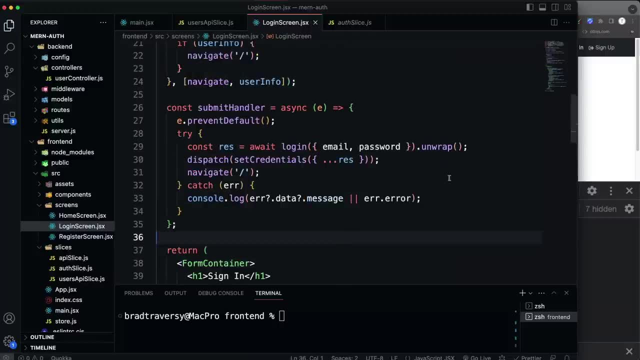 I'm just going to put question marks here, just so, if these so, we can still try to get this message, even if these are undefined. So let's save that. Now we're going to try to log in with the wrong email and password. 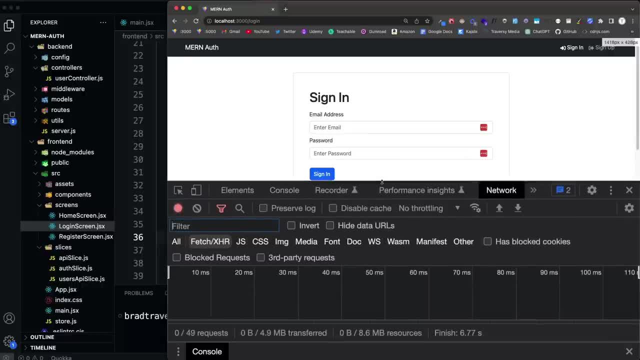 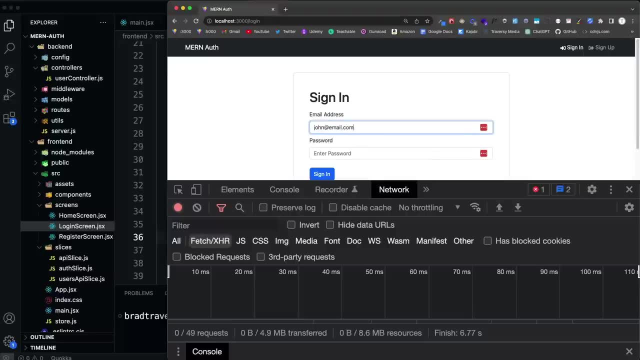 And I'm going to actually have the network tab open, just so we can see exactly what happens. So I'm going to put in here john at email dot com, which is not correct, And then one, two, three, four, five. 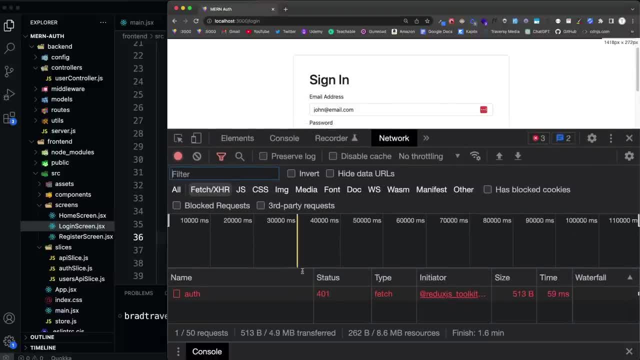 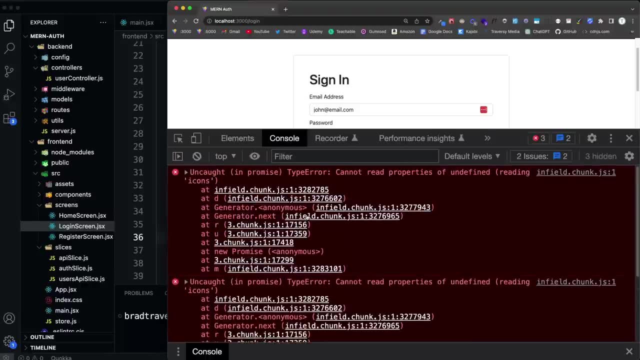 six, which is not correct, And click sign in And down here you'll see we got a 401 and it says invalid email, error, Invalid email or password. If we look in the console, let's see This right here reading icons. 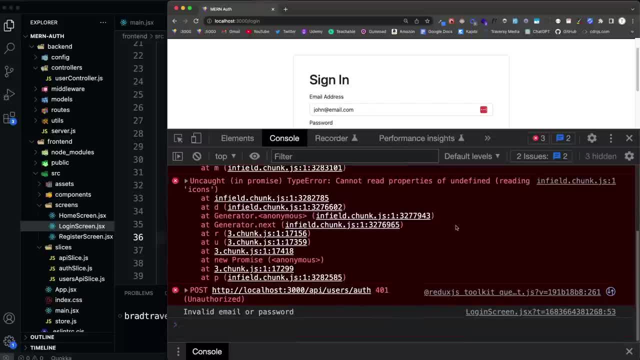 never mind that. That's just for my LastPass extension. You won't see that unless you have LastPass installed. In fact, I'm going to disable it in a second, But this is what we actually have coming from. our app is invalid email or password. 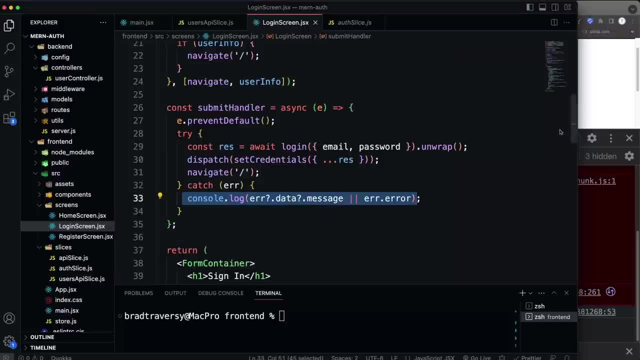 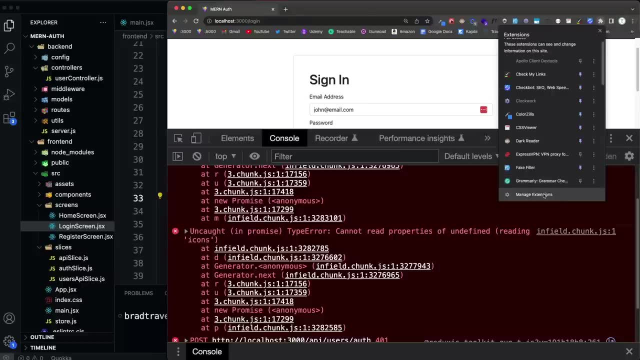 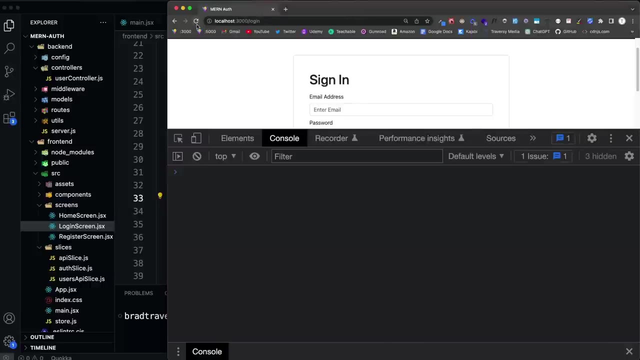 That's coming from the catch from this console log. Okay, So let me just, yeah, let me- disable LastPass real quick. That should make those go away. Yeah, So now if I send? yeah, so now, just seeing invalid email or password. 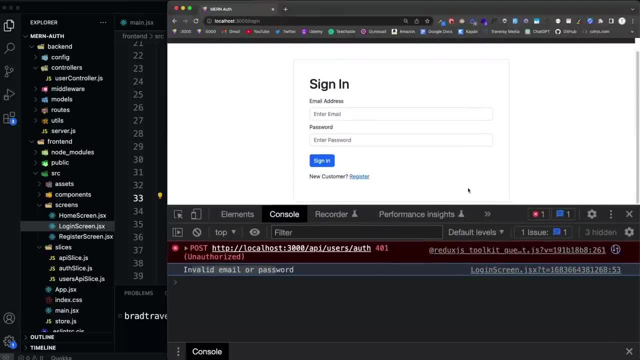 Now, before I try an email and password that works, I just want to set up React Toastify because obviously we want to show the user that you know they're entering. they're not entering the correct information and they're not going to check the console. 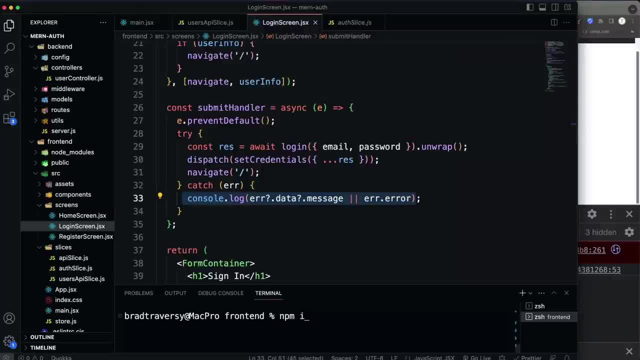 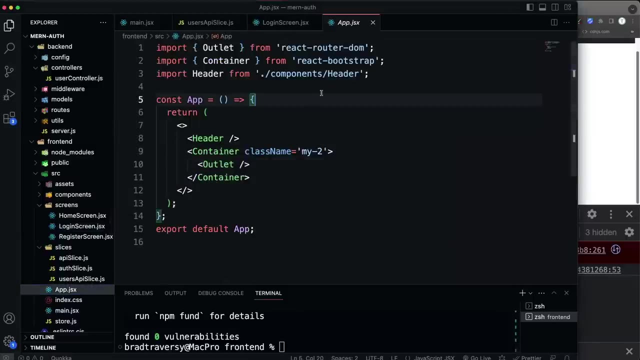 So let's go to the front end and let's npm install react-toastify And there's just a little bit of setup for this. So we have to go to our appjs or appjsx and bring in the toast container and the CSS for Toastify. 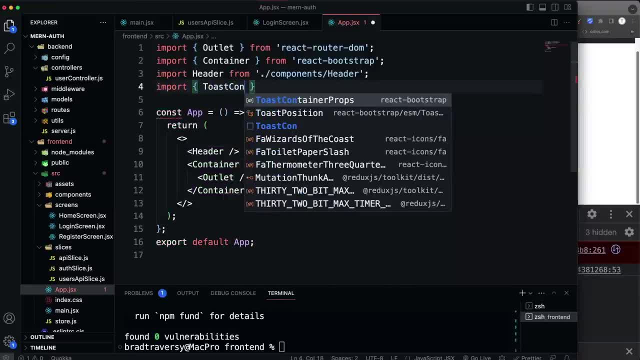 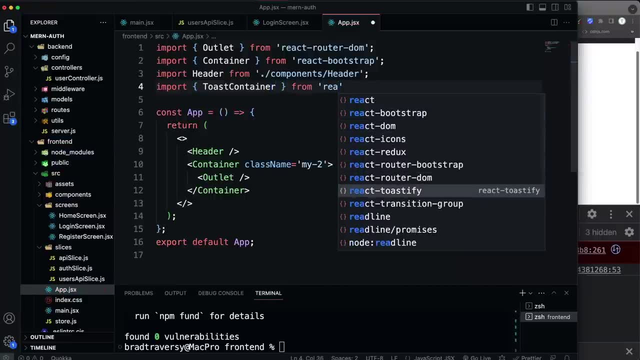 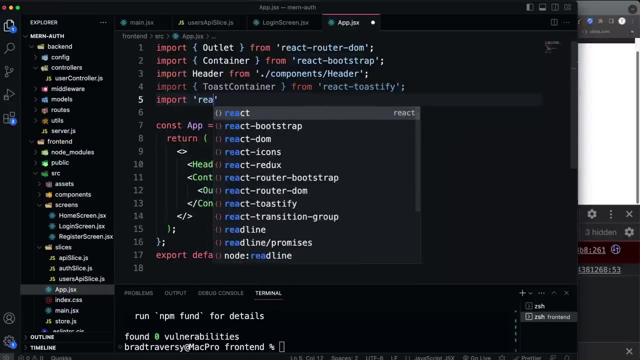 So we're going to import toast container And that's going to be from react-toastify, And then, right under that, I'm going to import the CSS which is in react-toastify: slash, dist, slash, react-toastify. I think that's it. 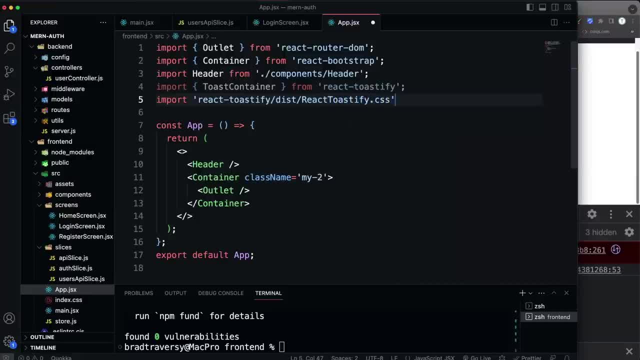 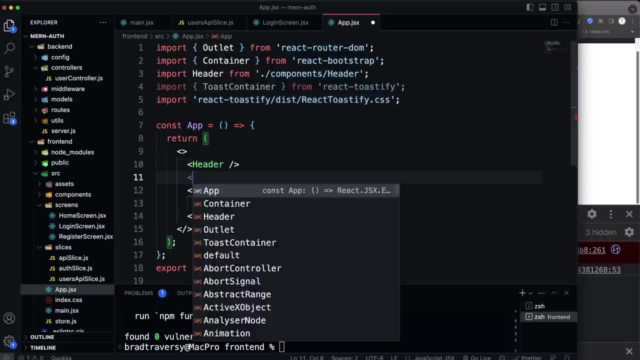 right, Yeah, react-toastifycss, Otherwise it will look really, really crazy. And then the toast container. you can just put that anywhere. I'm going to put it right under the header. So toast container, Oops, Toast container. 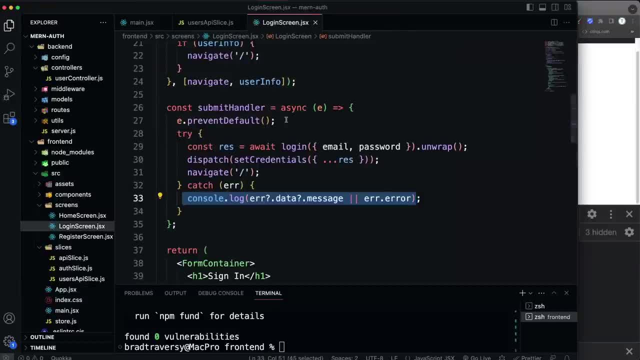 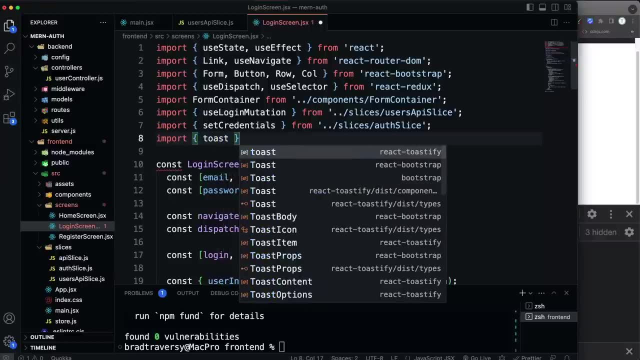 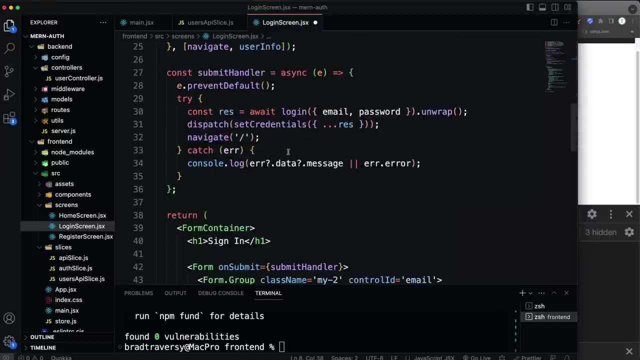 Just like that. All right, So now we should be able to bring in wherever we want. We should be able to bring in toast, which is a function that we call, And that's from react-toastify. So now, instead of a console log for my error. 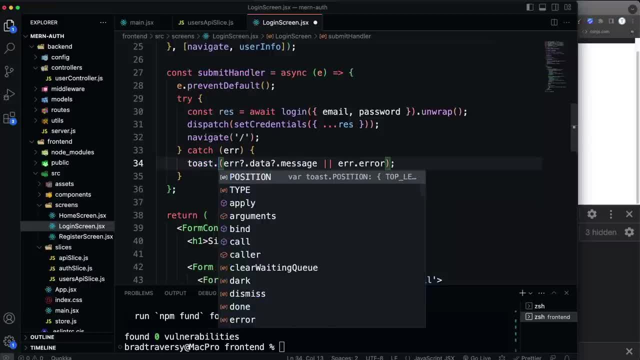 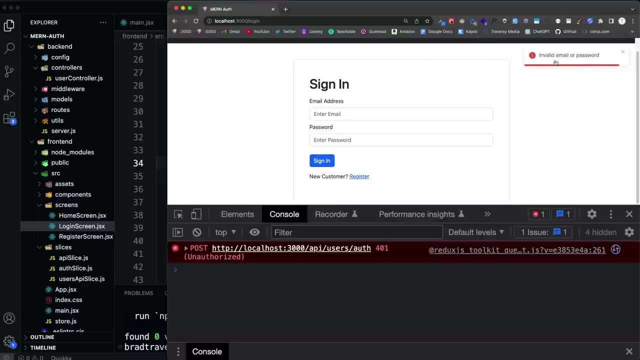 I'm going to change that to toasterror. So now, instead of showing it in the console, you can see, it shows it here in a toast. All right, So we know that the error works right if it's not correct. So now let's try the real login. 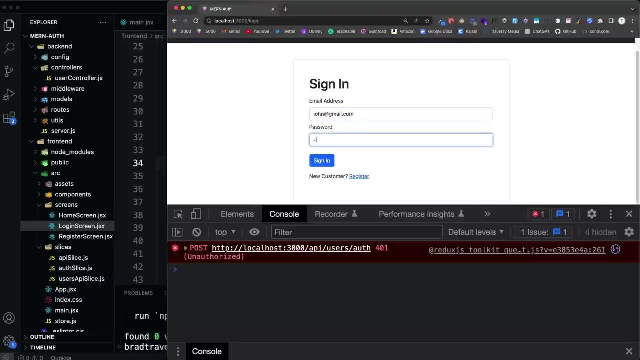 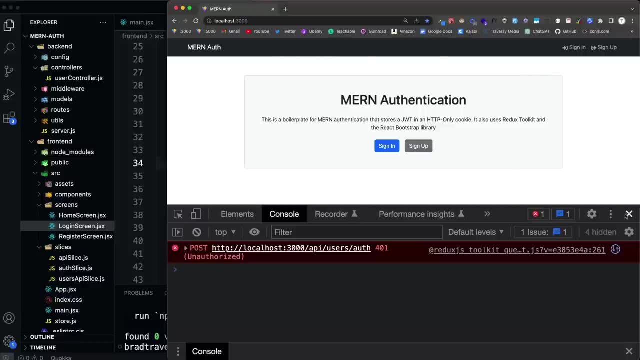 which for me is john at gmail, And then one, two, three, four and notice that I didn't get the message and it brought me to the index page. Now you can see the HTTP only cookie If you go to application. 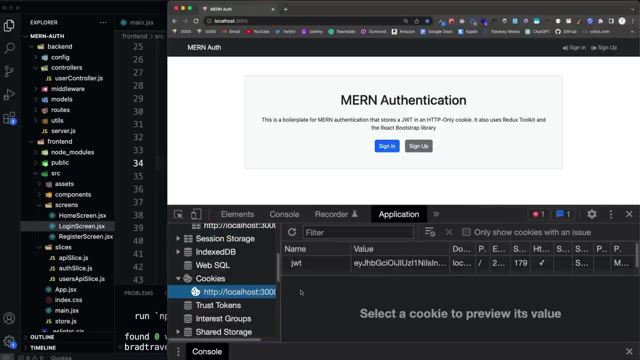 and then you go down to cookies and right here you can see my JWT and HTTP only is checked, All right. So we have that set And that's going to be sent with every request, So we don't have to worry about attaching the JWT. 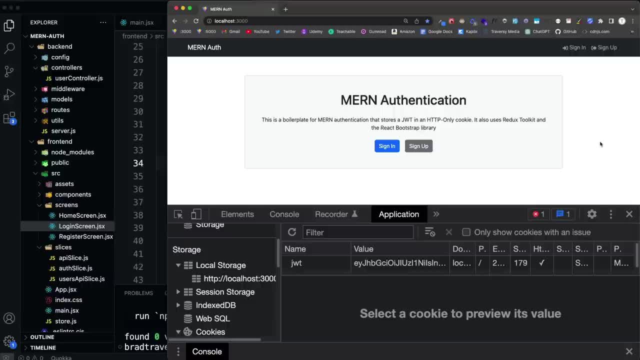 to the request, like you would have to do if you had it in local storage, which is really cool. Now I do want to show if we're logged in or not, So we want to change this menu up to check for the user And if there is a user. 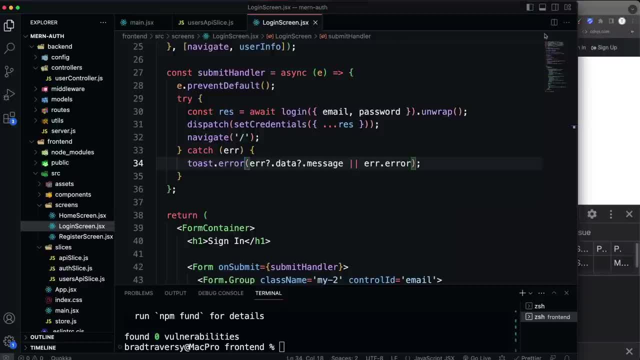 if we're logged in, then we want to show the user name along with a profile link. So what we'll do is go into our header. So, components header JSX, We can close up login screen. I believe we're done there. 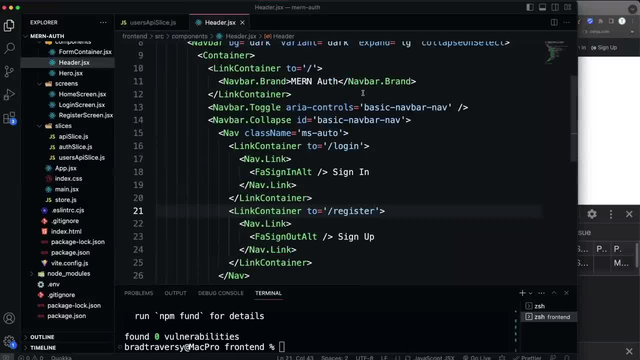 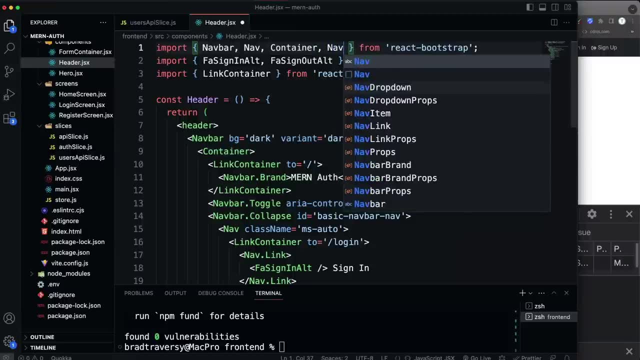 Main JSX. we can close that up for now. So in the header we're going to bring in a couple more things from React Bootstrap, because I do want to have a dropdown. So we want what is it? Nav? Yeah, nav dropdown. 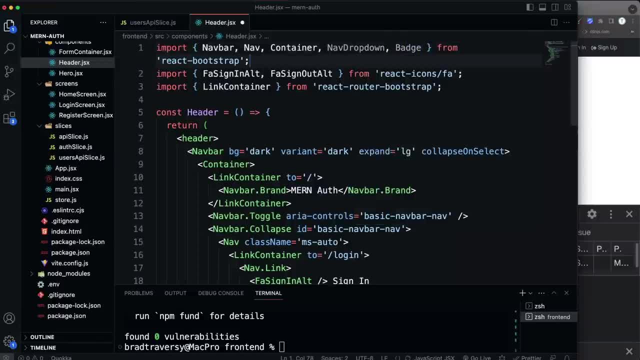 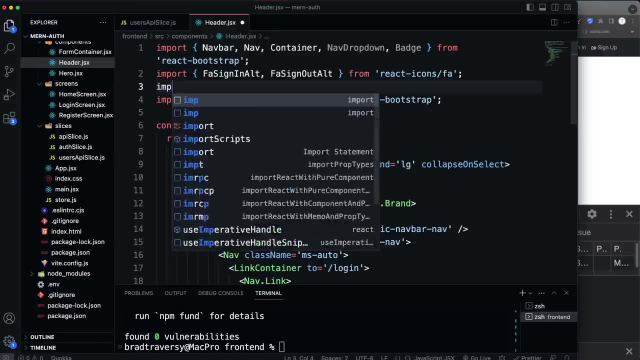 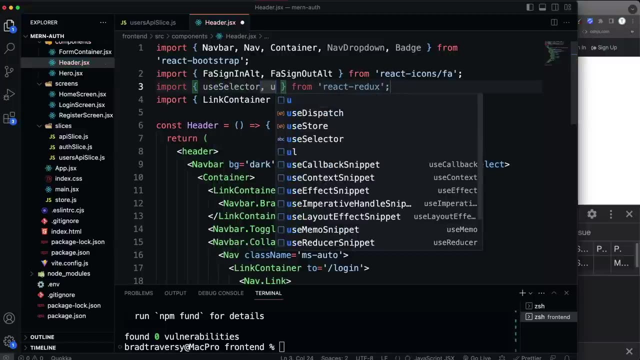 and badge, And then let's see what else we want. We need to be able to get stuff from the state, So I'm going to import useSelector And then we're also going to need useDispatch, because we're going to need to dispatch the logout. 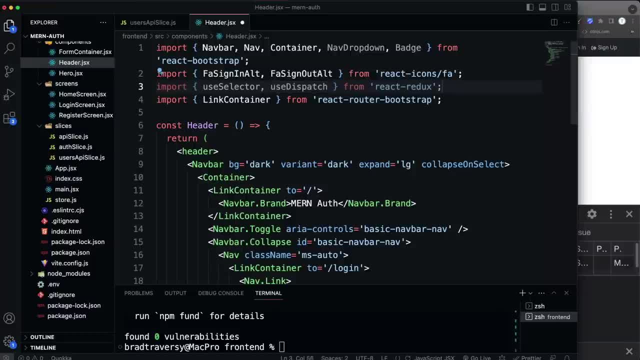 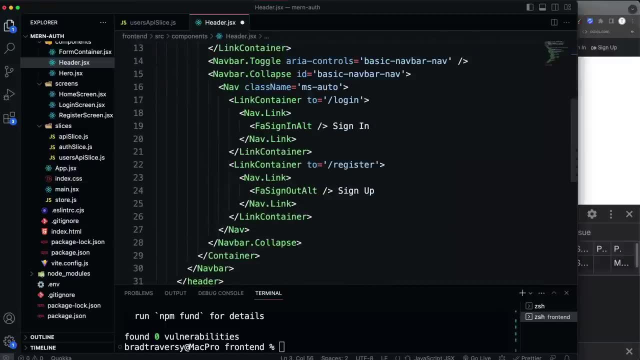 So I'll bring that in as well, And then let's see, I think that's yeah, that's all we need for right now. So let's come down here and go to, let's see, So we have our nav right here. 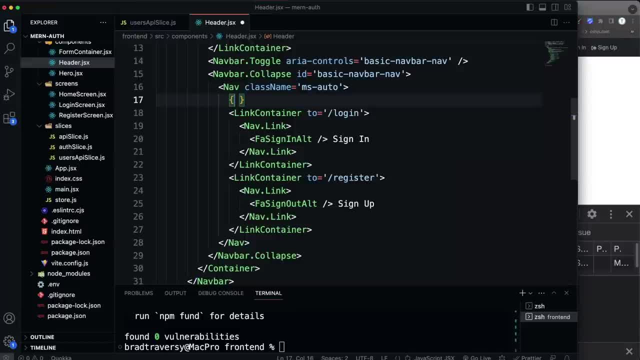 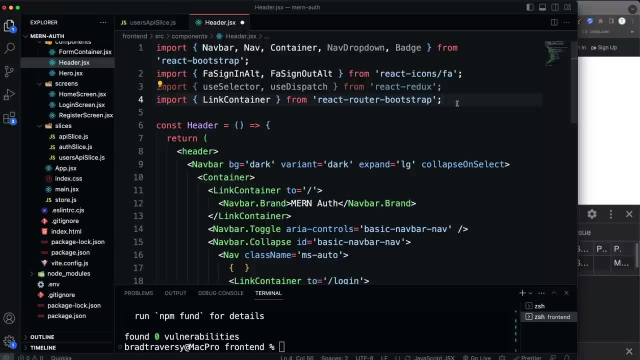 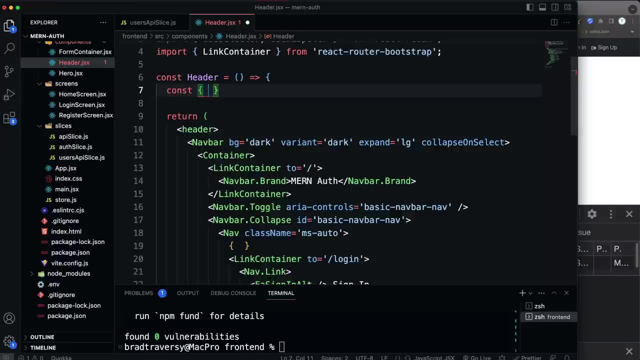 So directly in the nav I'm going to open up some curly braces and I'm going to check for the user info. Actually, before we do that we need to get the user info. So in the component above the return we'll say const- userInfo. 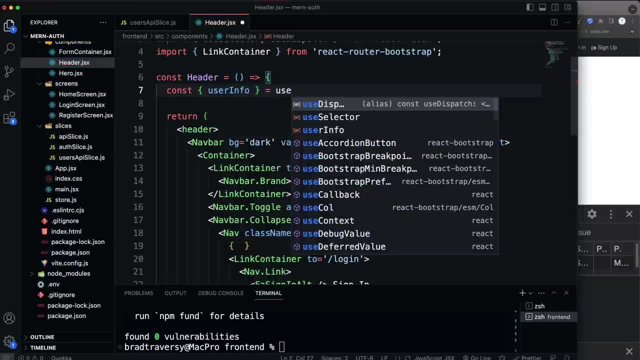 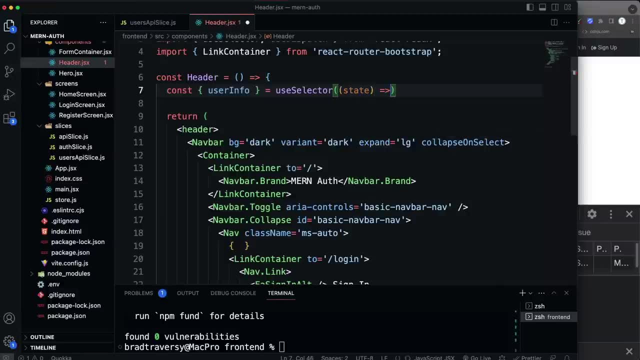 And we're going to get this the same way we got in the other. in the login screen We say useSelector, That takes in a function with the state, And then the part of the state we want this from is stateoff. So now down here. 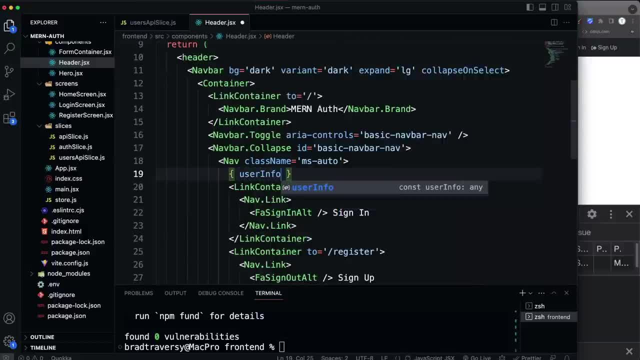 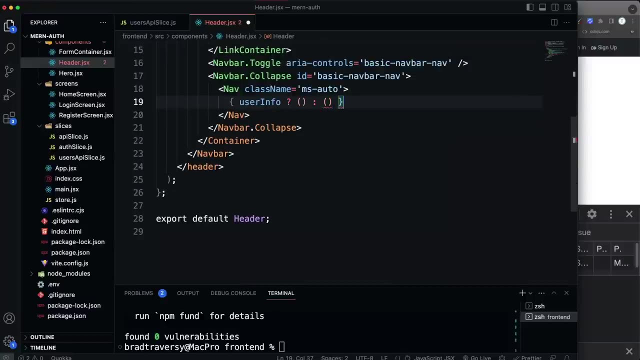 we're going to check for that user info And if it's there, then we'll show something else. We'll show something else Now. the something else is this: these two link containers. So I'm going to cut those, And we do have to have a wrapper around those. 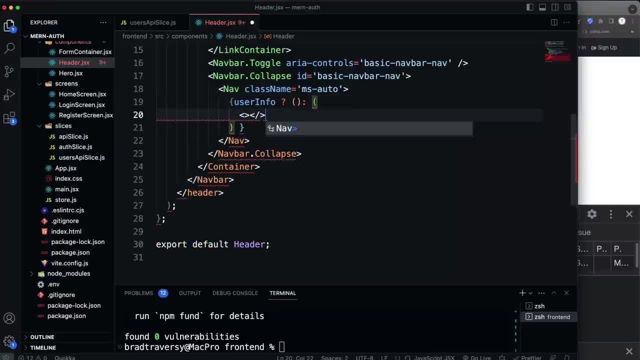 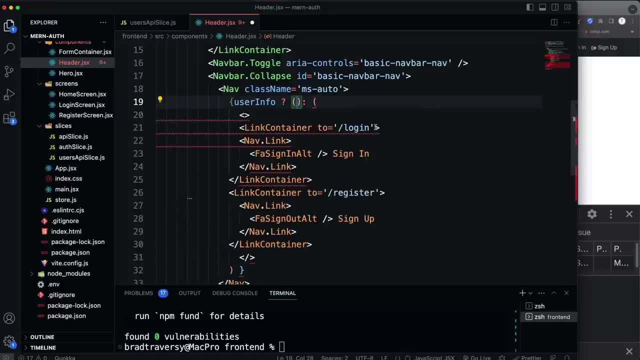 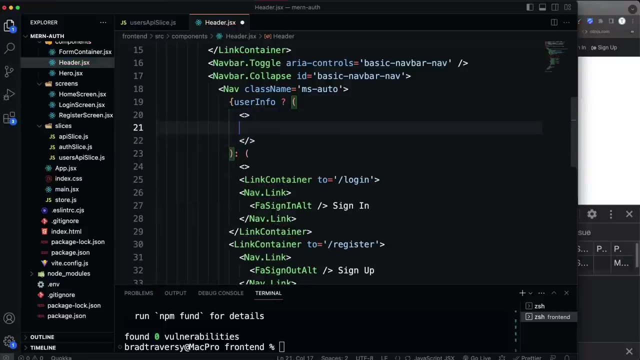 So I'm going to go in the second set of parentheses and add a fragment, And then in that fragment I'll add those link containers And then in the first one, here is where we want to put the dropdown and the username. So we're going to actually wrap that in a fragment as well. 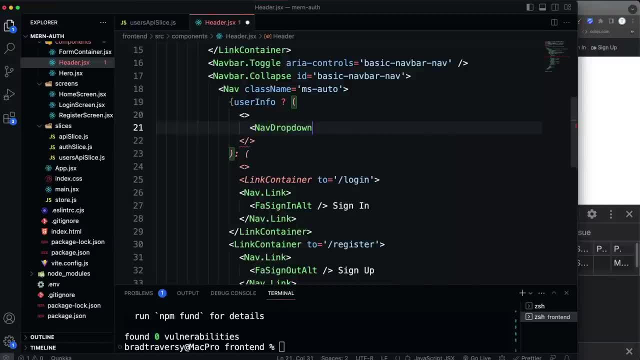 And let's say, nav dropdown. We're going to give it a title. Title is going to be set to userInfoname, because that's what's going to be displayed, And I'll give it an ID of username. All right, Now inside the dropdown. 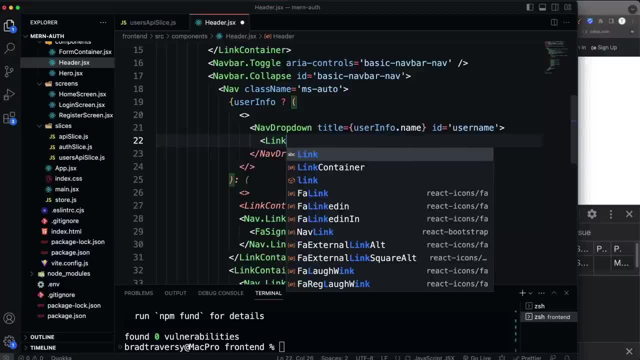 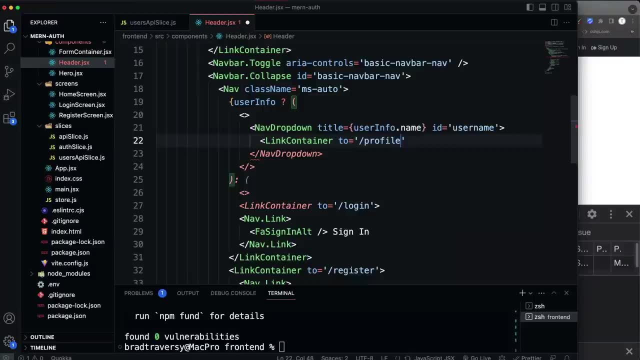 we're going to have the link container For the profile. so let's say link container to and set that to slash profile. And then in the link container we're going to have a nav dropdown item, So nav dropdown dot item And that's going to say profile. 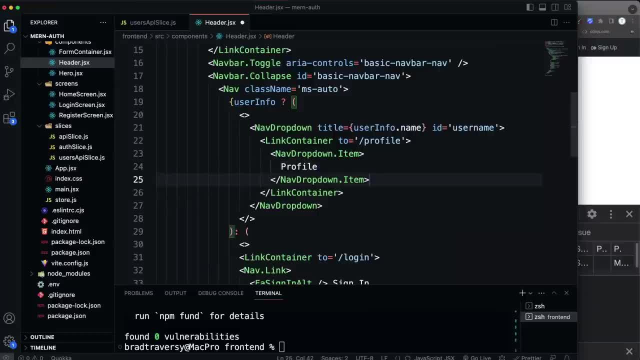 All right, Then we're also going to have a log out. So under that dropdown item- actually, I'm sorry, after that link container- we're going to do a nav dropdown dot item and say log out, Okay, And this will have a log out handler. 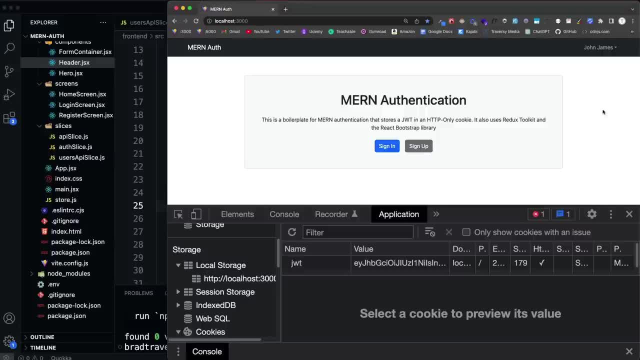 but we'll just add that after. So now, if I save that, we take a look: it says John James. Okay, And then I have my profile, which obviously isn't going to work yet. Log out obviously isn't going to do anything either. 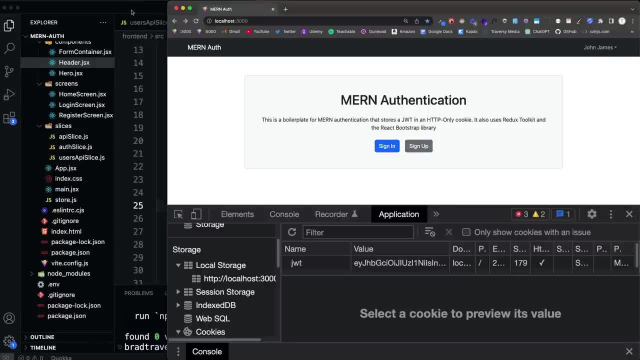 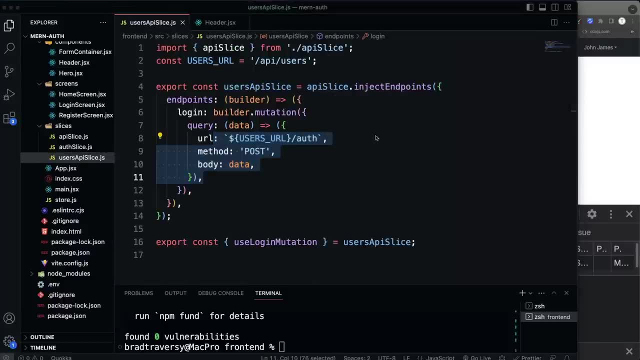 But at least we can see that we're logged in. So now to do the log out, what we can do is go back to our user's API slice and we can add a new mutation for a log out. So I'm going to go under the log in. 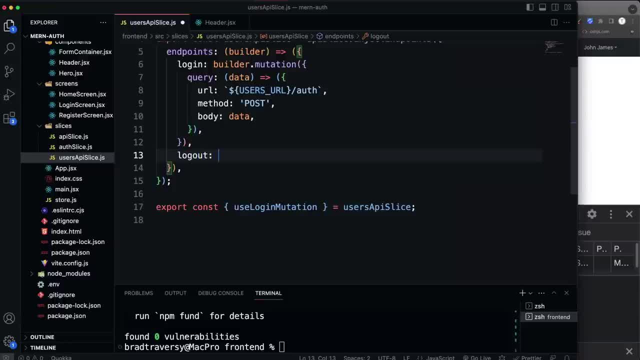 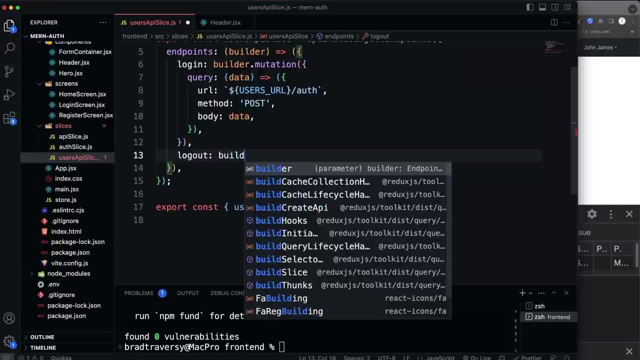 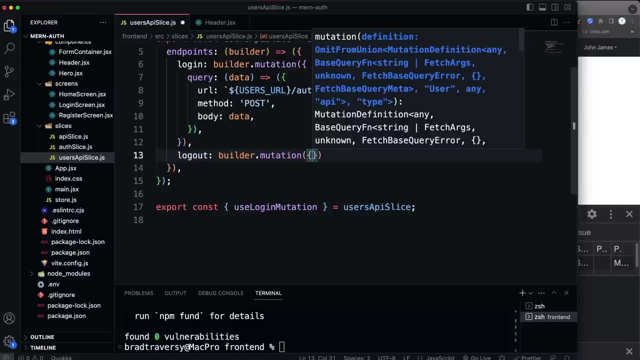 which ends right here, And you'll see the pattern and you'll start to see that it's easy to add new functionality and new requests. So we're going to say builder dot mutation And in here we're going to pass in. 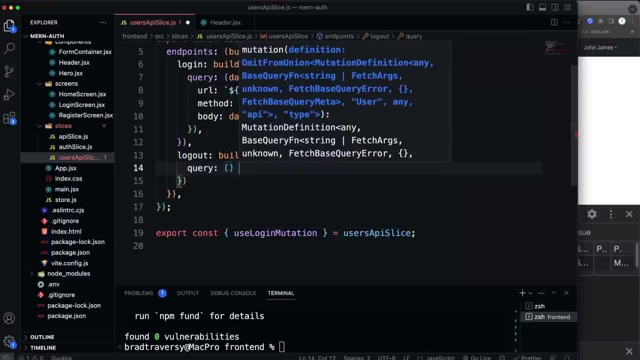 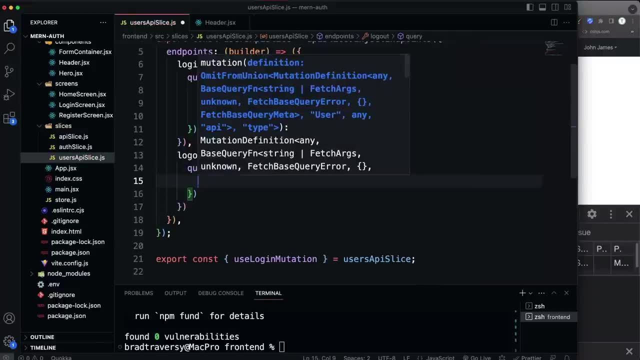 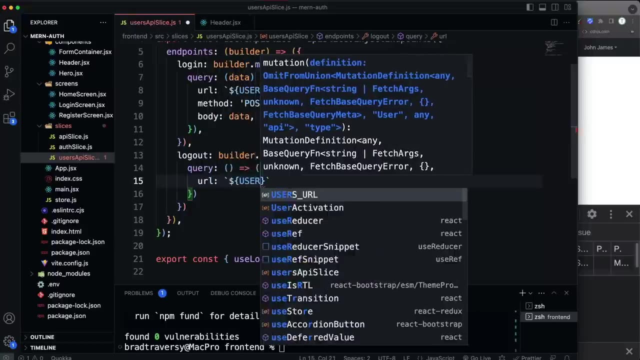 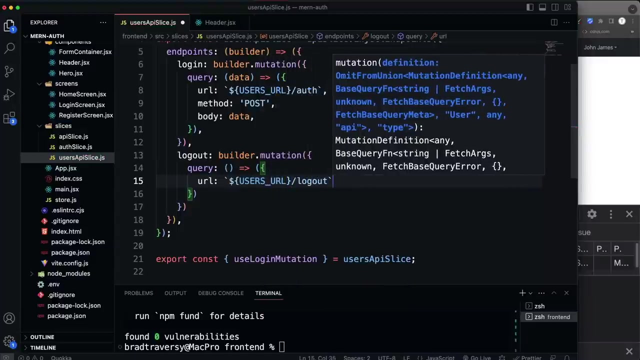 say query. Actually, we want to set that to parentheses and then curly braces. So the URL for this is going to be the user's URL. User's URL: slash log out. Okay, Because we're hitting that endpoint And we want it to be a post request. 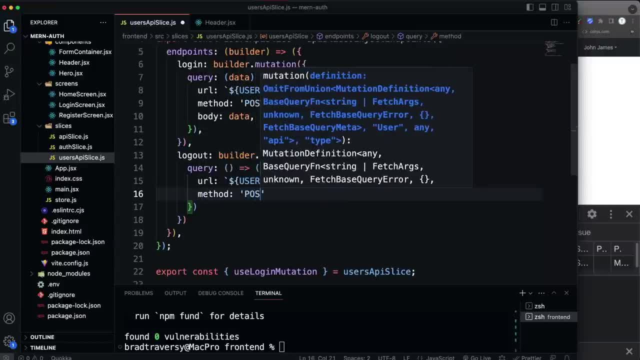 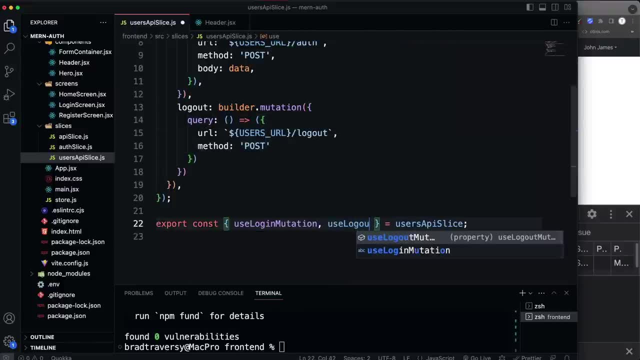 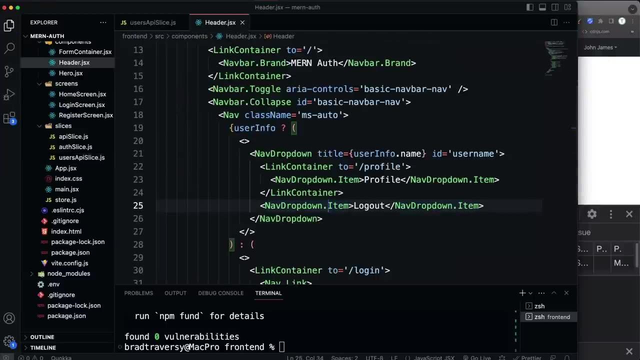 So let's say method and set that to post. Now we need to export this. So remember the convention. It's use log out mutation. Now I'm going to go back to the header and I'm going to bring in that mutation. 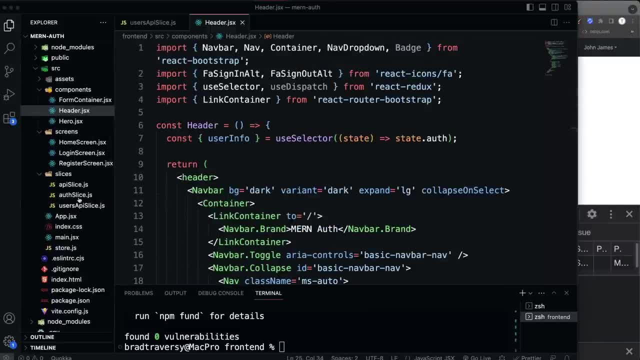 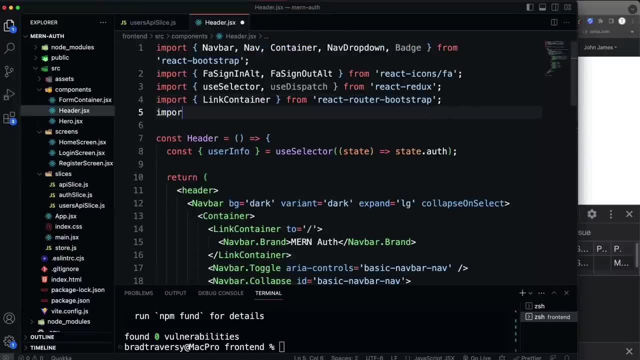 And I also want to bring in the log out from the auth slice, the local one Right, This log out which just removes it from local storage. So let's say in the header import And we want use log out mutation. 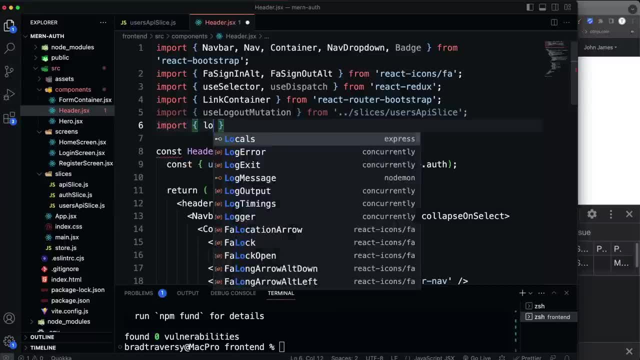 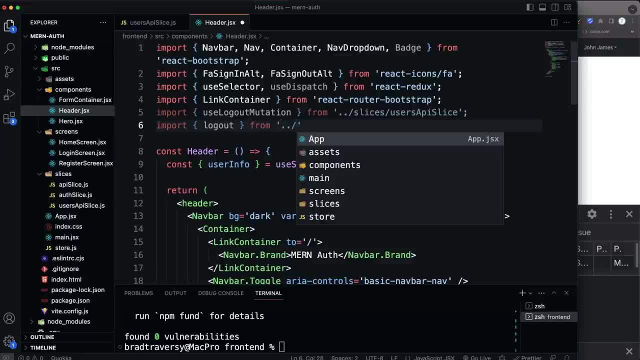 And then I'm also going to import log out from let's see where are we. We want to go up to slices, Slices, slash, and then users- I'm sorry, no, auth, slice, Okay, And we want to call both of those. 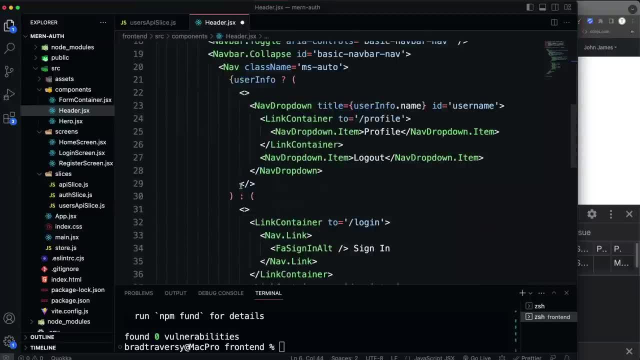 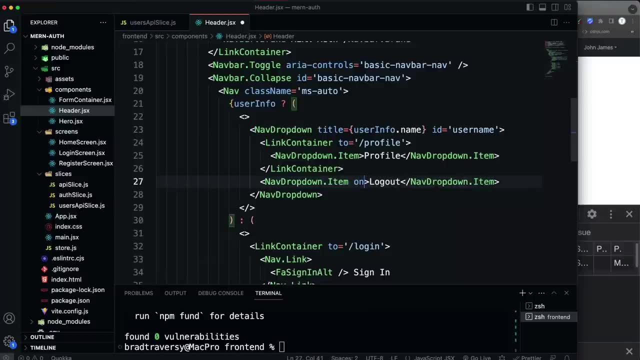 In our handler. So let's go down to the log out Which is right here. So this nav bar drop down item I'm going to say on click And we'll set that to, let's say, log out handler And then we'll go up here. 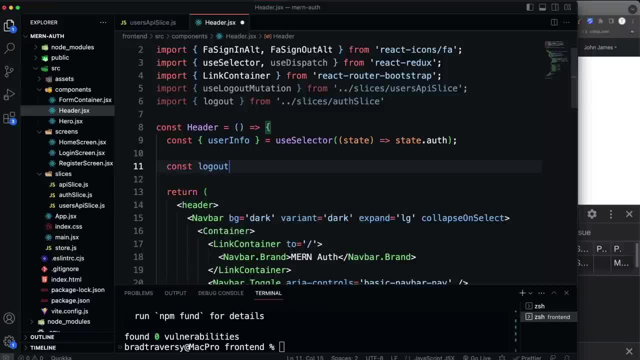 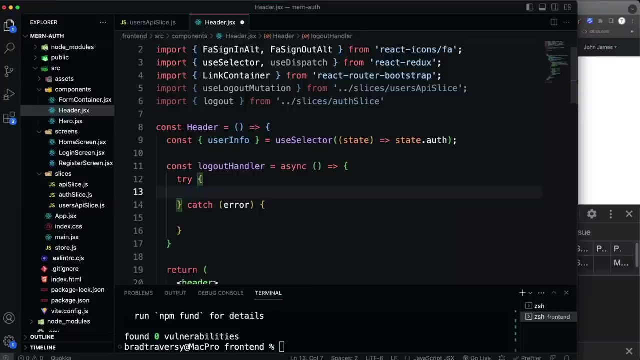 We'll add that Log out handler And that's going to be asynchronous, Okay, And then we'll put that in a try catch, And what we're going to do here is await. Now I haven't created the function to call for this mutation yet. 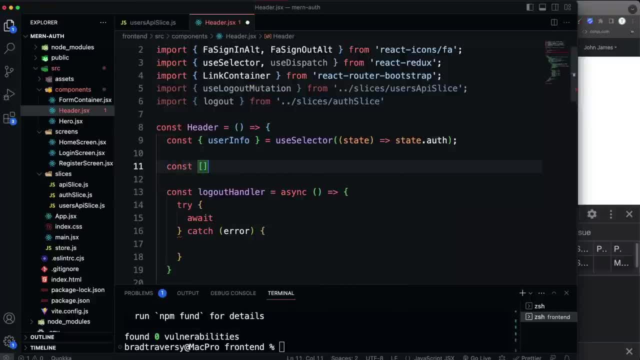 So that's something we have to do. So let's say const, And in brackets, I'm going to call that. I'm not going to call it log out, because this one is called log out. So I'll call it log out- API call. 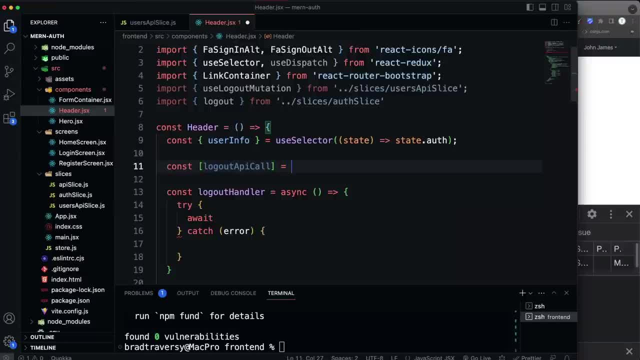 And then, yeah, that's all we need And we'll set that to use log out mutation, All right. And then I also just need to initialize dispatch, because we do need to dispatch that, this log out When we have a mutation or a query in an API slice. 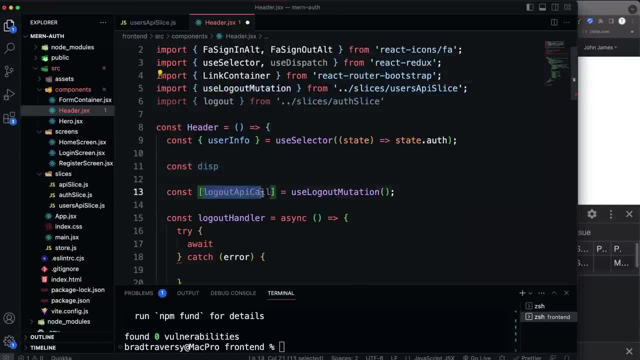 we don't need to use dispatch, We just we create it here. But when we just have a regular function where we're not making asynchronous requests, then we need to call dispatch around it. So we need to set that to use dispatch. 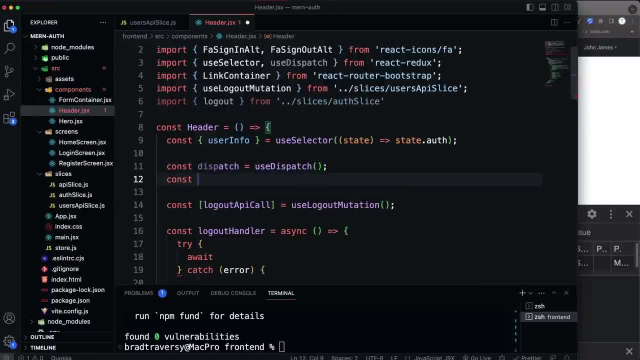 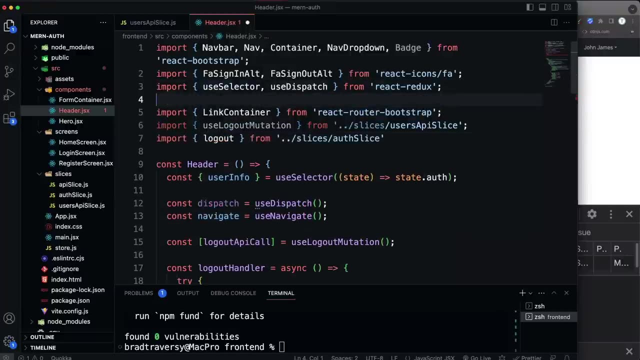 And then if we want to navigate, we need to create, let's say, navigate set that to use navigate. Did I bring that in? No, I didn't bring in navigate, use navigate. So we need to say: import, use navigate. 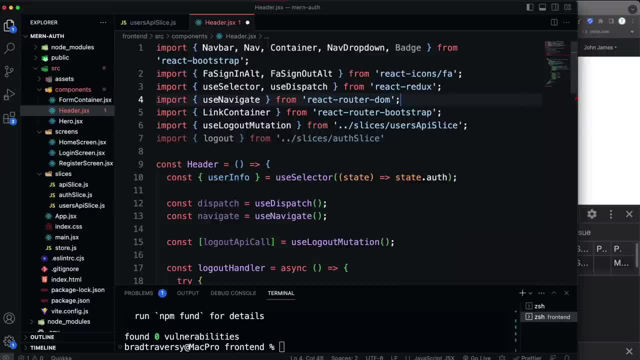 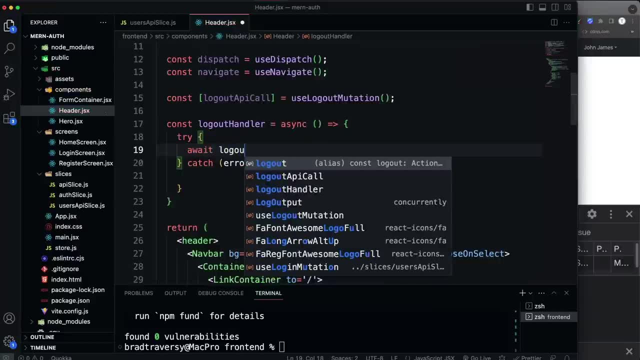 from react router DOM, Okay, And then down here. So I'm going to await on the log out API call And again I'm just going to call dot unwrap. So that will actually make the request, which will destroy the cookie. 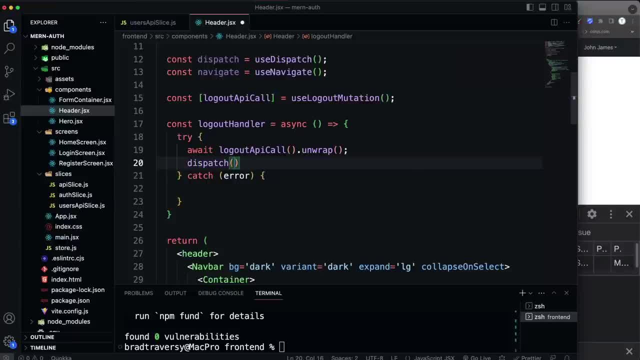 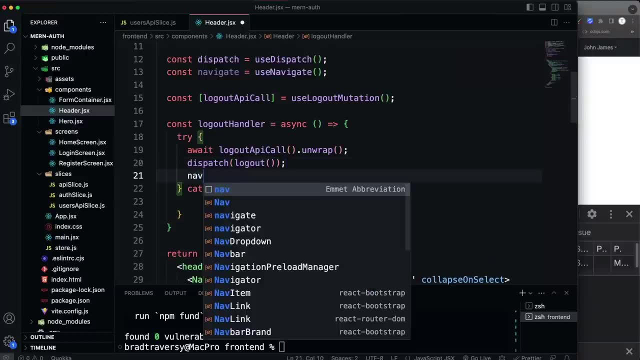 And then we're going to dispatch the log out, the, I guess the local log out, which will just clear the local storage, And then we're going to navigate to the, to the index page, And then, if there's an error, 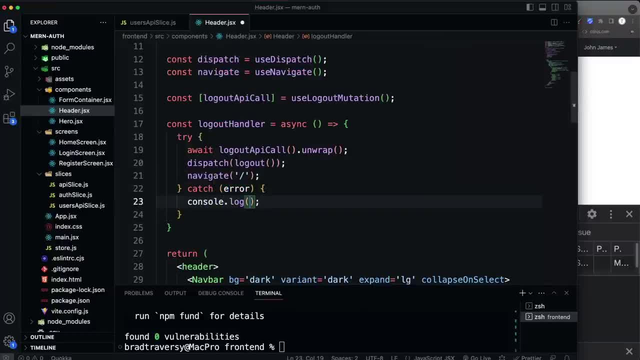 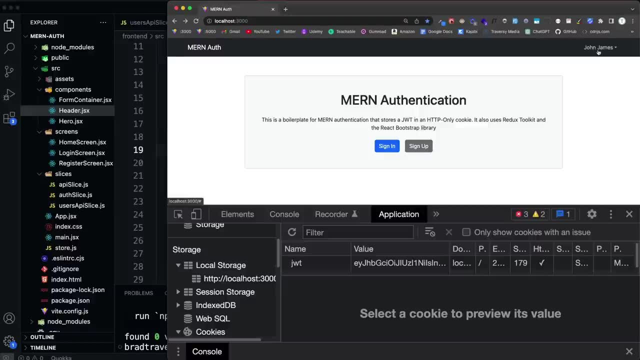 then let's just console log error, All right, So now we'll come over here and I'm going to go and click log out, And there we go And you can see that the token, the cookie, just disappeared when I did that. 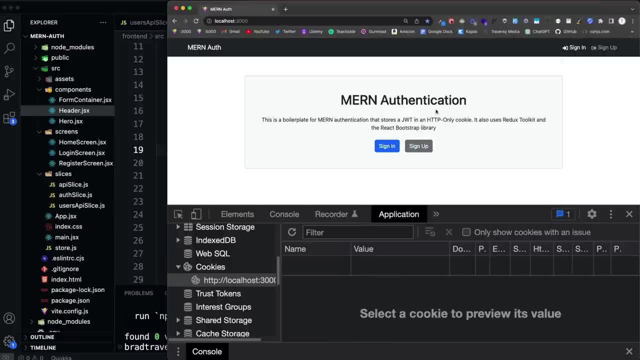 Now, one thing I want to do is have the a spinner. So when we sign in, like right now, if I do that, there is a point where it is loading and we actually brought that in into the login screen. So right here is loading. 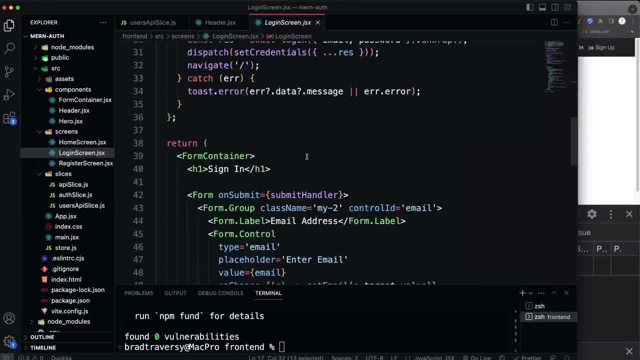 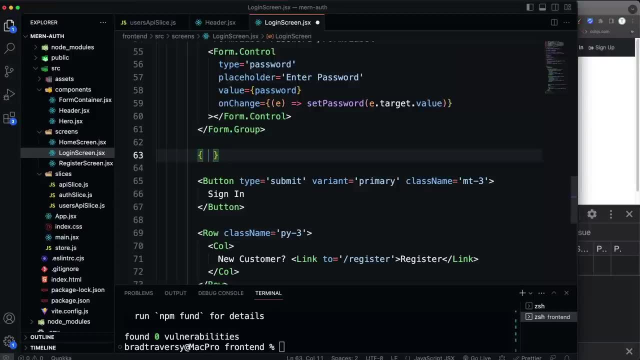 So we might as well take advantage of that And let's put it. Let's see, I'm going to put it right above the button So we can just check and say if is loading then. So I'm just using the double ampersand. 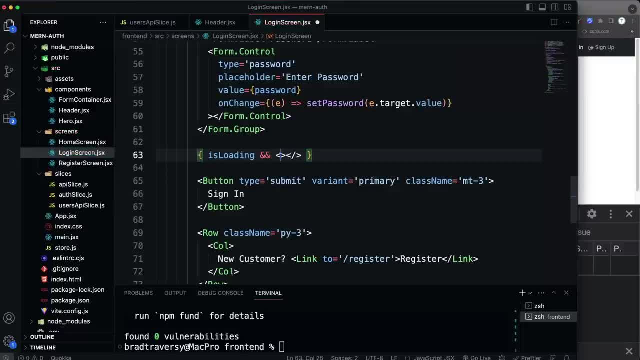 So if loading then show, I guess for now just an H2 and loading, We'll create a spinner in a minute, but let's just see if that works. So yeah, you can see, it flashes loading. So let's create a quick loader or spinner component. 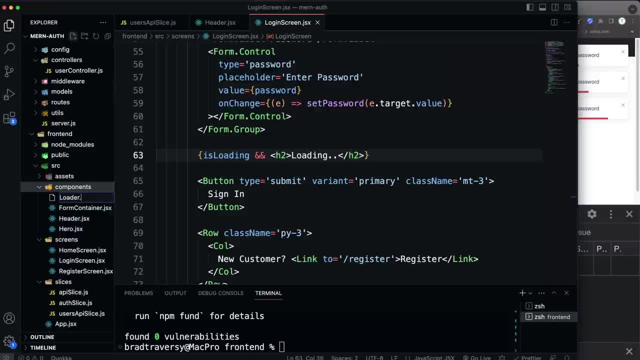 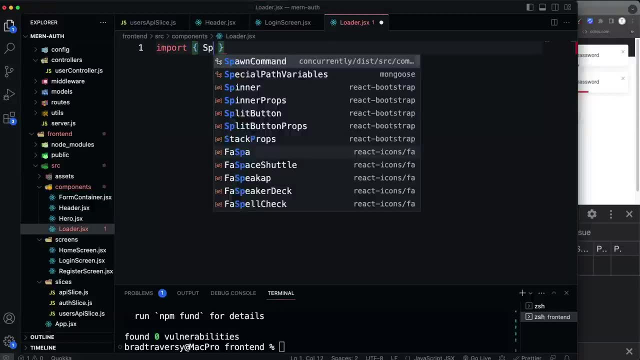 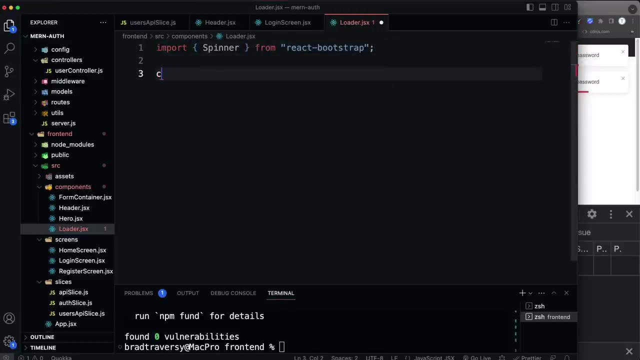 So I'm going to create a new component called loader dot JSX and React Bootstrap actually has a spinner component, So we're going to bring that in. So let's say import spinner from React Bootstrap And we'll call this function. Actually, let me just do R-A-F-C-E. 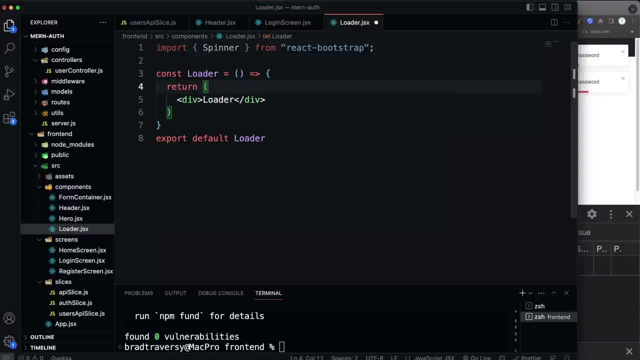 So loader And let's see, we're going to return a spinner, Spinner, And we don't have to put anything in there. What we need to do is just add some props- So I'm going to say animation- and set that to border. 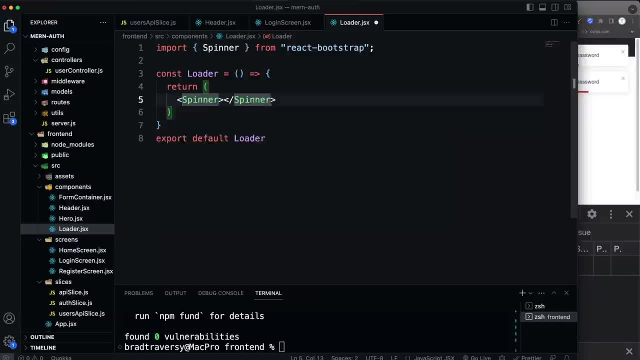 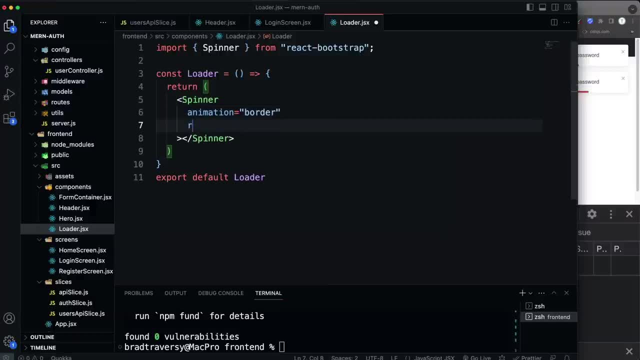 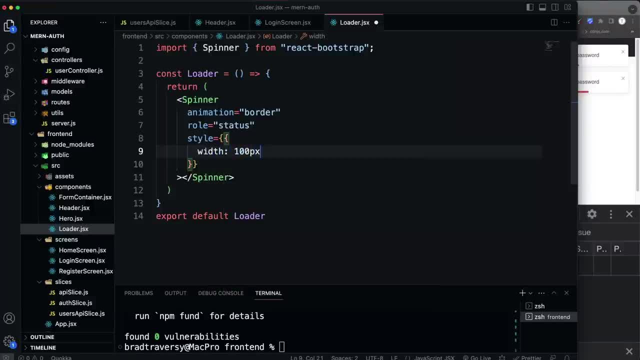 Let's set a width of hundred pixels. This needs quotes. Win it with. Why is this? Yeah, that should be good. So, with 100 pixels and then comma, then the height, which I'm also gonna set to a hundred pixels, and what else do we want? margin? 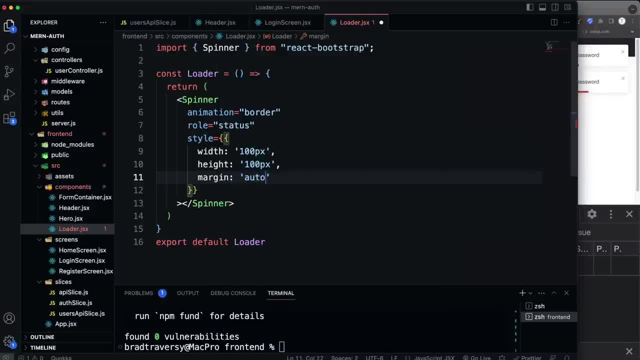 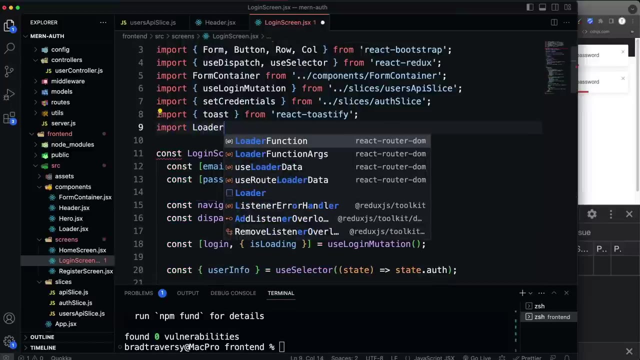 let's set that to auto, because we want that to be in the middle, and we'll set display to block. okay, so now let's close that up and bring the loader into the login screen. so import loader. why isn't it popping up? port loader from dot dot. 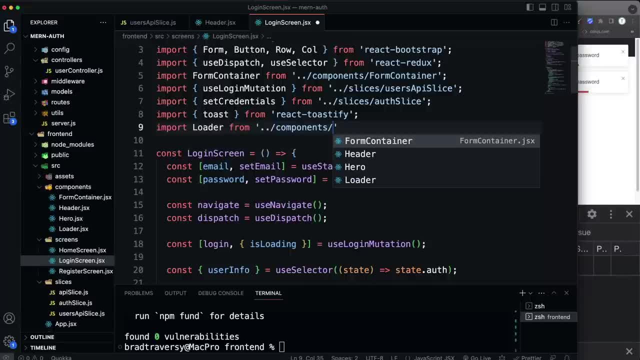 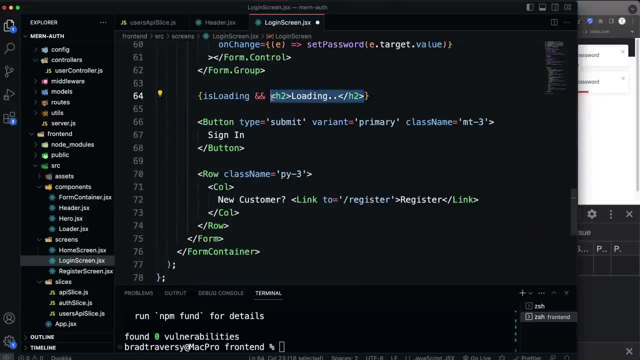 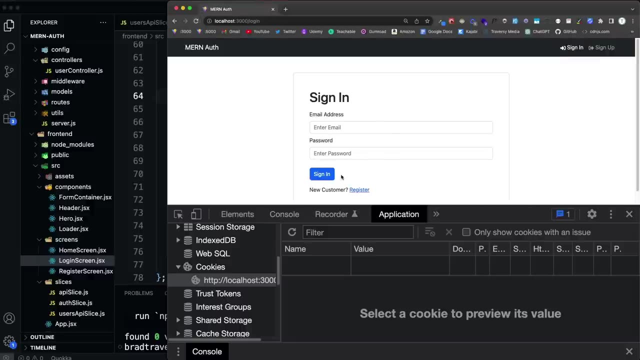 slash components, slash loader, and then down here instead of this h2, let's change that and say: if is loading, then we want the loader, so we'll save. let's see what happens. so if I click sign in, you can see it flashes real quick. alright, now we want to do the register next. so the sign up and first step. so you again. 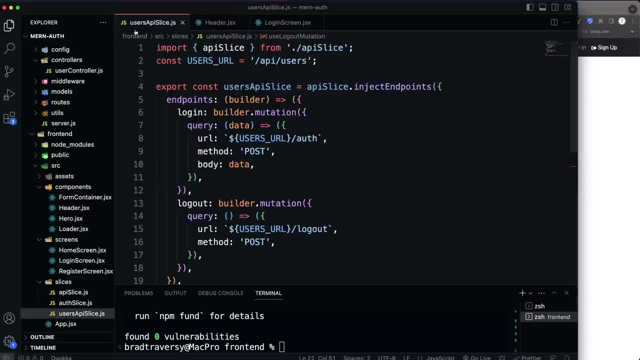 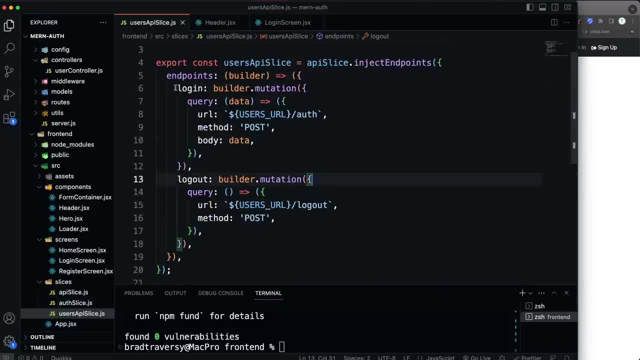 you're gonna start to see a workflow here. the first step is to put the, the endpoint in here and the slice. so we have login, we have logout. I'm actually just gonna copy this login and then we'll go right under it and paste it in at the waypoint data. so I'm actually just going to send it to the. 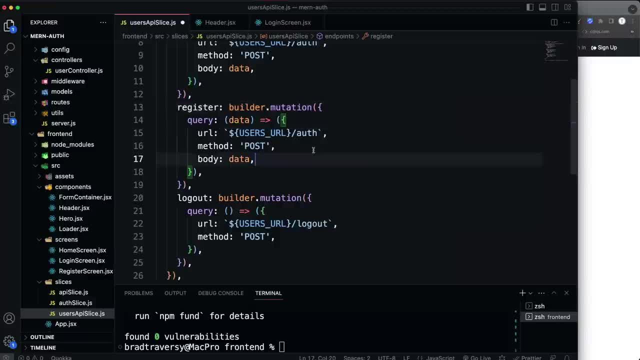 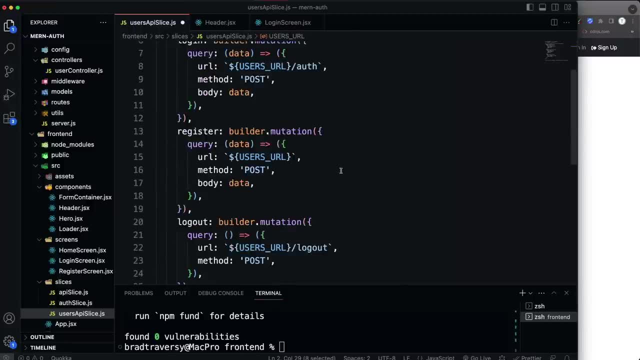 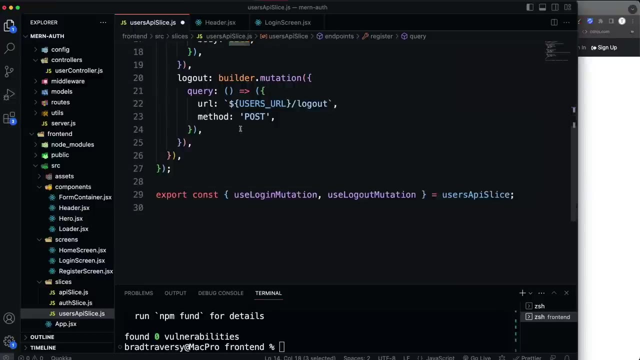 that in and let's call this register and the endpoint is just going to be the user's url because, remember, if we make a post request to api users, that's our register and we're going to keep body data and passing in the data, because that's going to be the name, email and password, and then 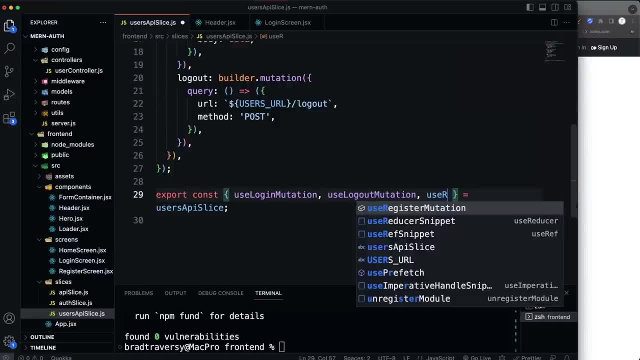 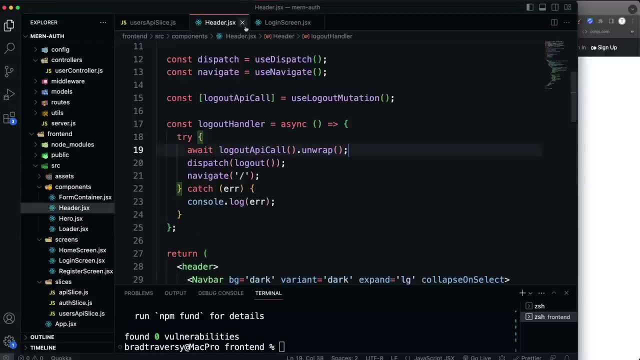 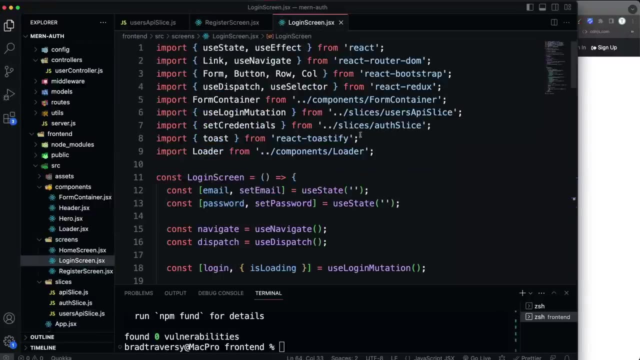 to export. remember the convention. it's going to be use register mutation and then we can go into our register screen. let's see we can close the header up. let's go into our register screen and we can probably copy some stuff from our login screen. so like, for instance, this: use use selector and. 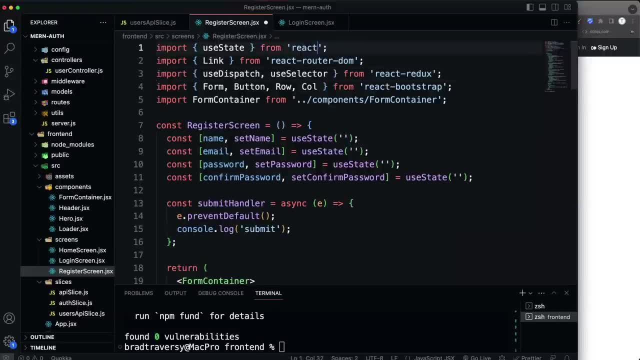 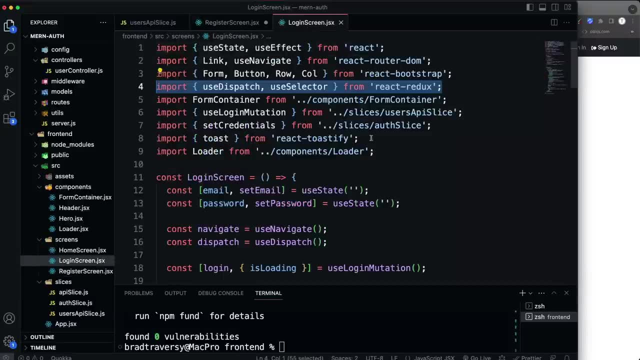 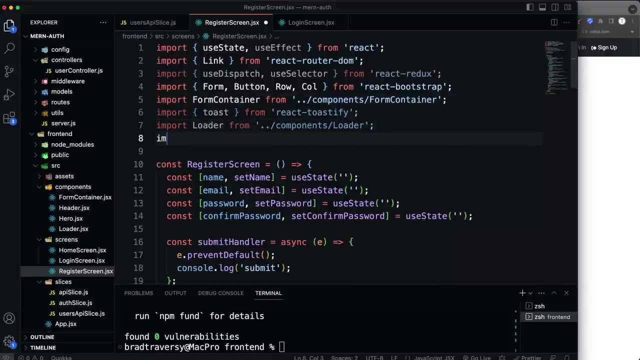 use dispatch. we're going to need that. let's see, we're going to need use effect. so, right here, use effect. and then what else? the toast and the loader, we can bring those in, and then we want to bring in the mutation that we just created. so that's going to be use register mutation and we're also going. 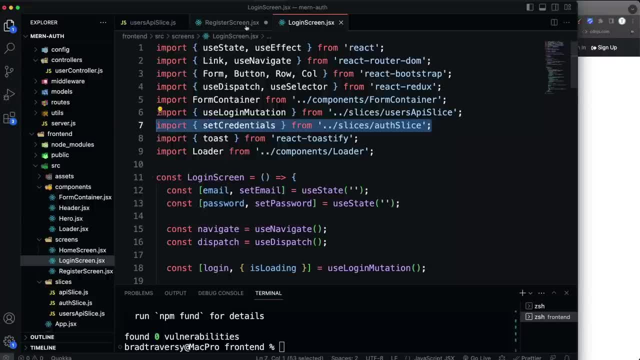 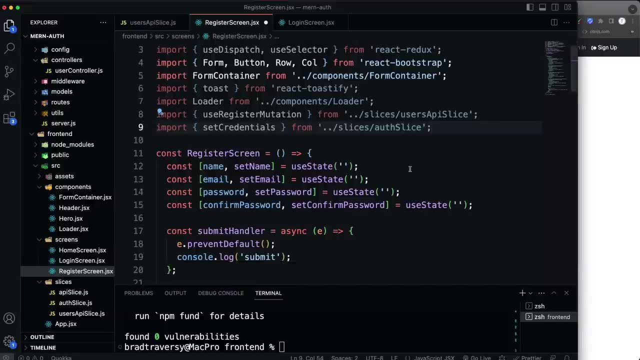 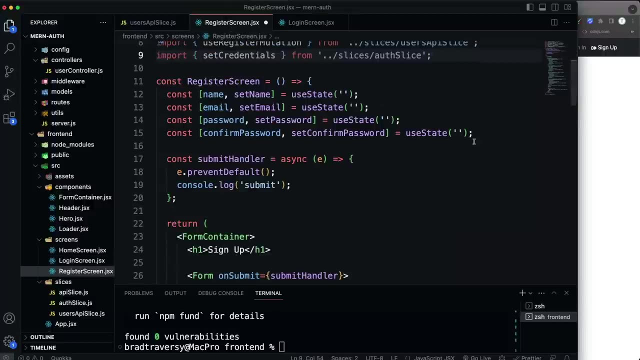 to want this: set credentials because, remember, when we register, we log in directly after. so we're going to want to set those credentials once we register. so I want to bring that in as well. and then, let's see, we also want to initialize our navigate and dispatch, so that I'll put right here the let's see. 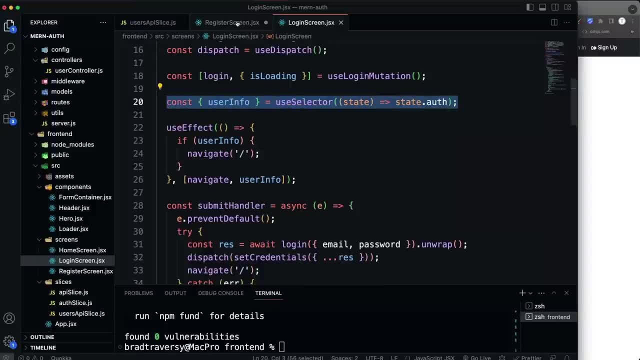 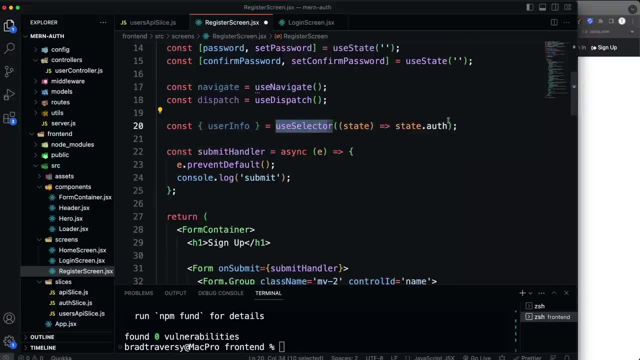 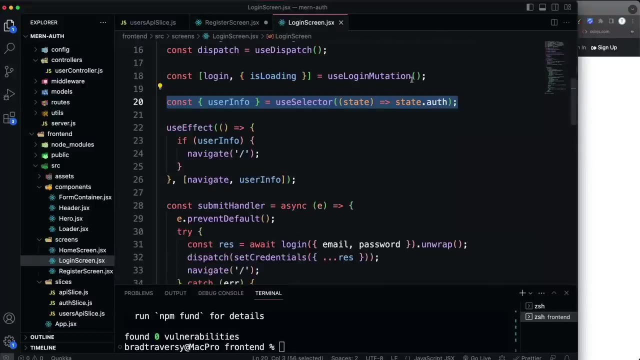 the user info. so we're going to want that. any component where you want to get the user info, it's just this single line here and breath course bringing in you selector now to get the register mutation. we're going to do similar to what we did right here, so I'll actually copy that. 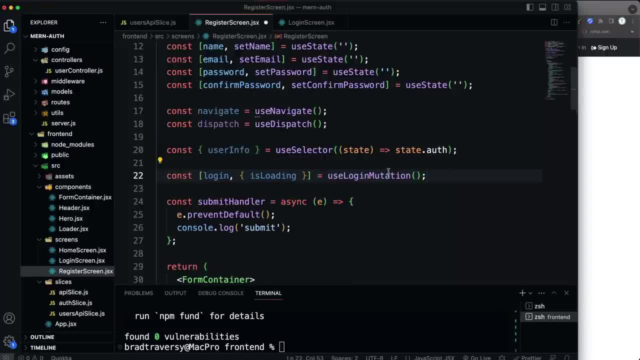 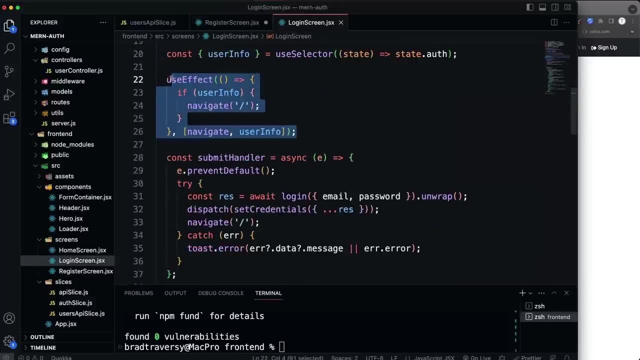 and you register. what we'll do is change this to our register mutation and we'll call this instead of login. we'll call this register and then, for the use effect, just like we did here, we're going to check for the user and if there is a 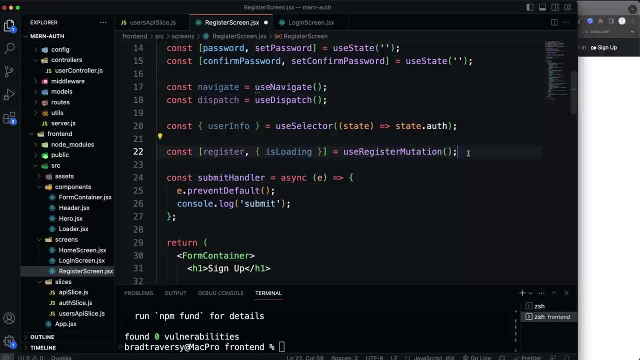 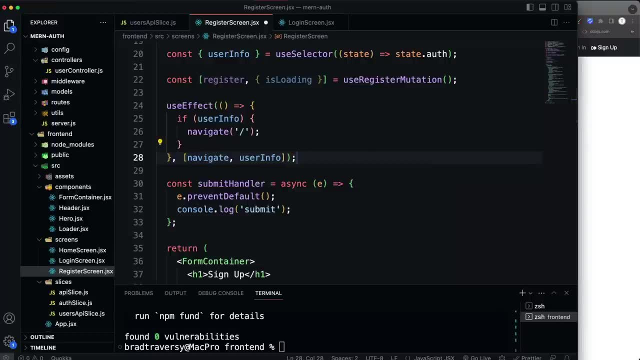 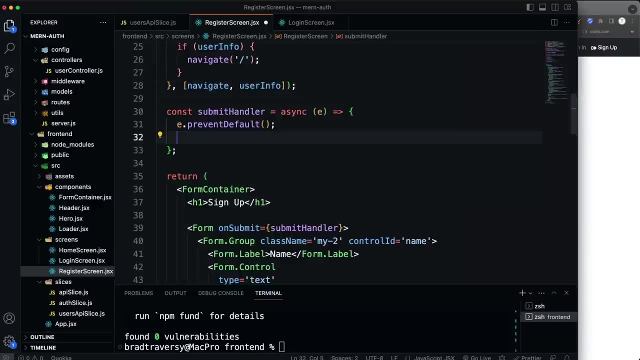 user, we want to navigate to the home page because obviously we don't want you to go to the register page. if you're already logged in, you're already registered, so that can stay the same. and yeah, and then in the submit handler, let's get rid of this console log and let's just do. let's check the password. 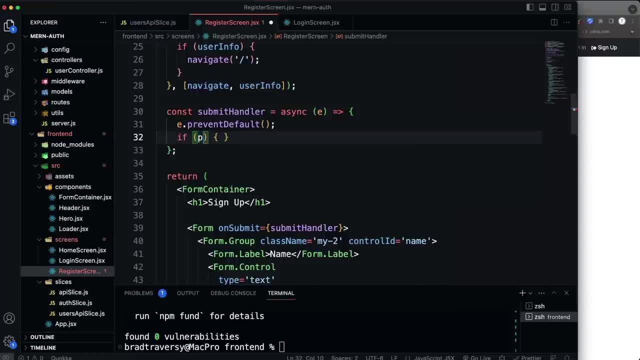 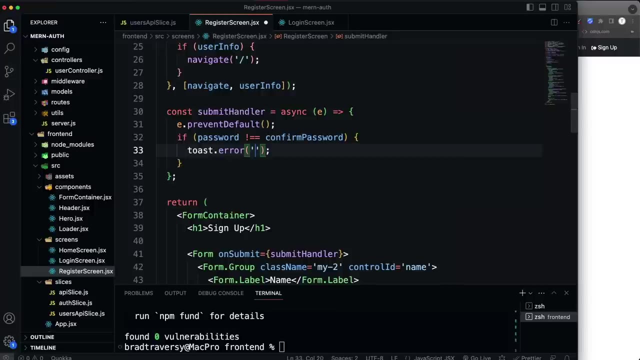 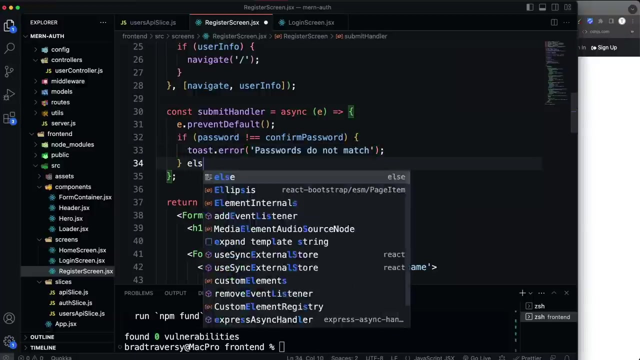 first because we have a confirmed password field. so we'll say: if password is not equal to confirm password, then we'll show an error. let's say toast dot error and we'll say passwords, passwords do not match, else they do match. then we'll do a try. 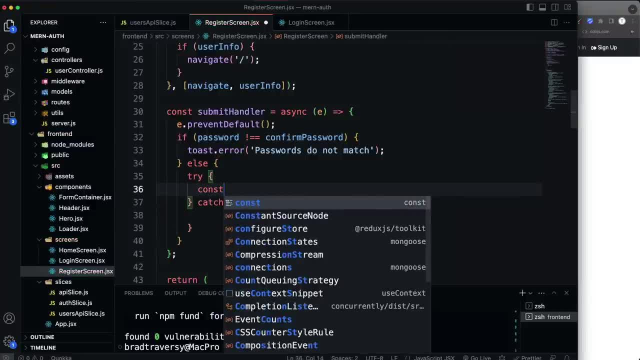 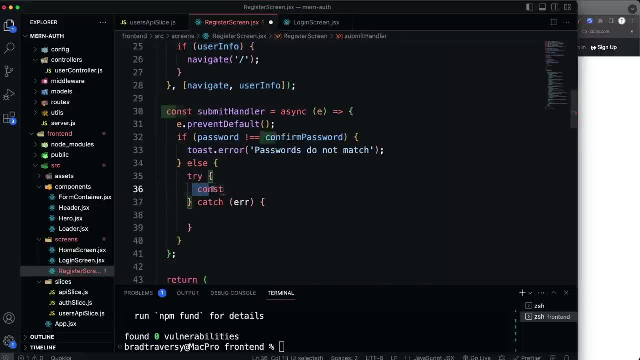 try catch. and in here we're going to basically do the same thing we did here, right, in fact? i'll copy these three lines, except instead of login we're going to call register and instead of just the email and password we're going to pass in name, email and password. same thing: here we're going. 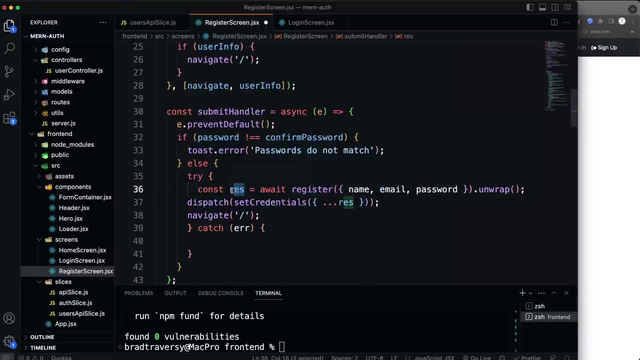 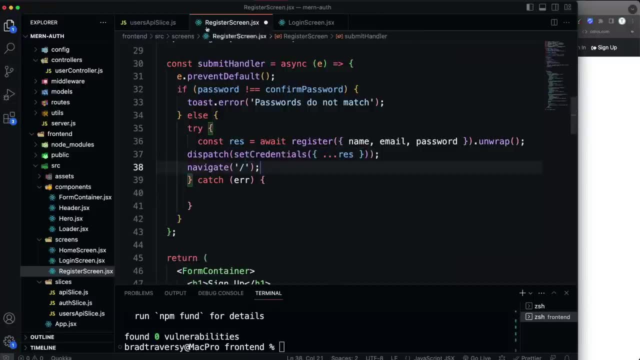 to dispatch, set credentials, because register will give us the user data back. and then we're going to set the credentials, meaning we're going to log them in, and then we're going to navigate to slash, all right, and then if there's an error, we'll just show it in a toast, just like we did here. 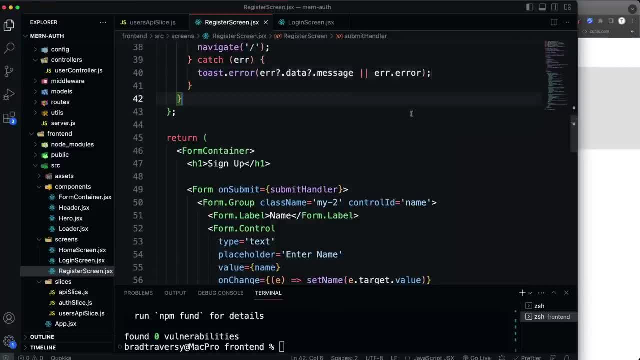 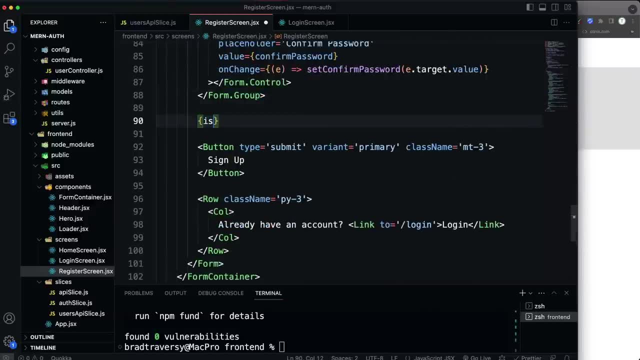 so very, very similar to what we did in login, and also we can add the loader. so down, right up above the button, we can say: if is loading, then show the loader. so i think we're ready to try to register a user. what's this use navigate not defined. 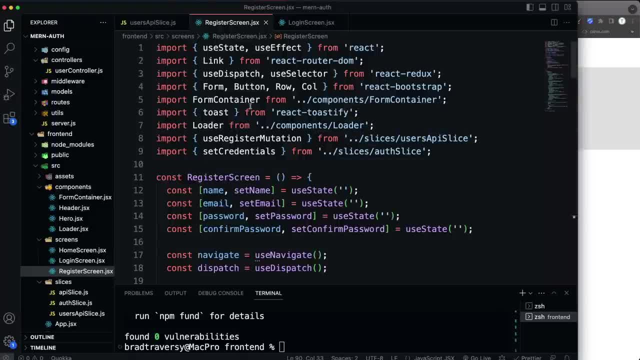 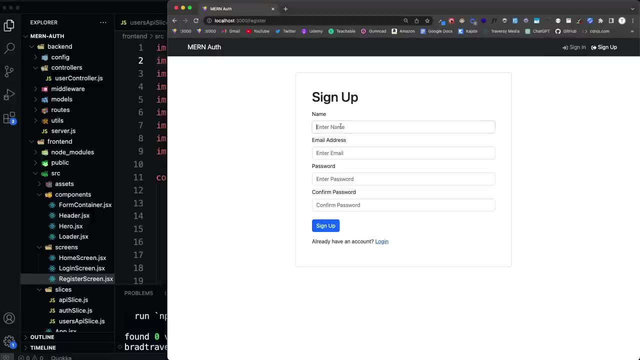 did i not bring that in? i thought i did. oh right, here we need to bring in use navigate, alright, so now i'm going to try to register a new user. so say brad. of course you can put whatever you want here. say brad at gmail: one, two, three, four, five, six. one, two, three. 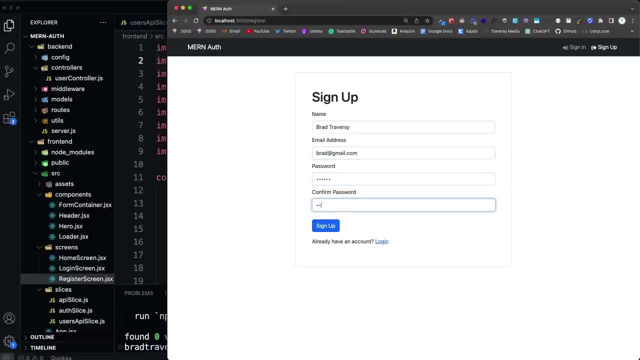 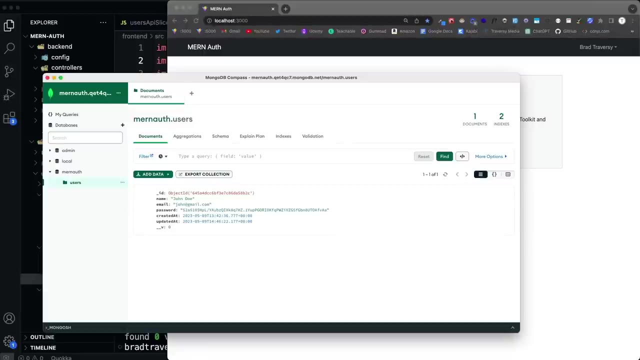 four, five, six. stone two, two, three, four, five, six stone two, four, five, six primera: sign up and there we go. we saw that it it did, the little spinner, and now we see brad traversey at the top here. so it looks like everything went okay. and if i were to open up compass and reload my 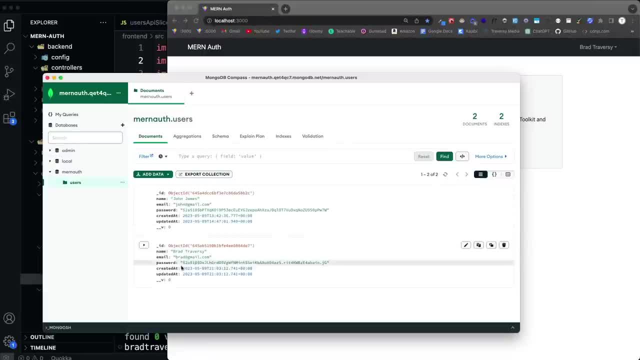 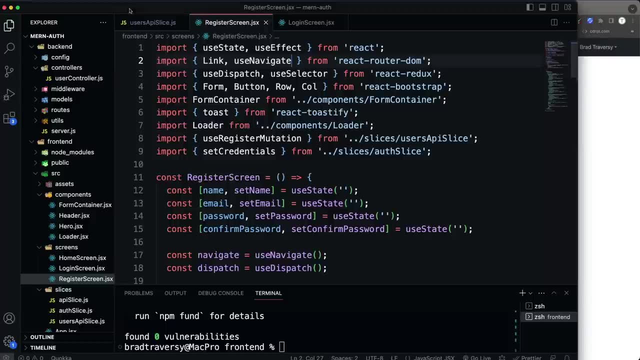 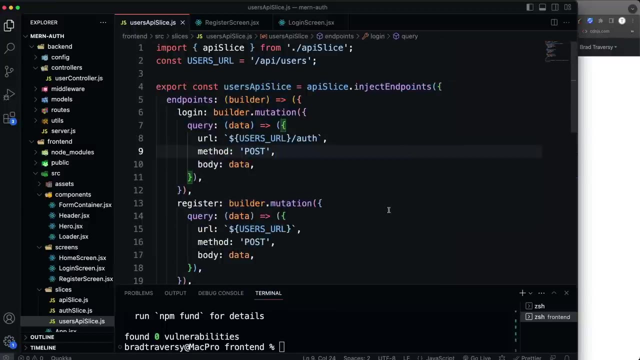 data. now i have this brad traversey user and i registered this user through the front end, through our application, so hopefully this is starting to kind of make sense to you. i think that this, this is pretty neat, as opposed to what we would do with just vanilla redux having like an actions. 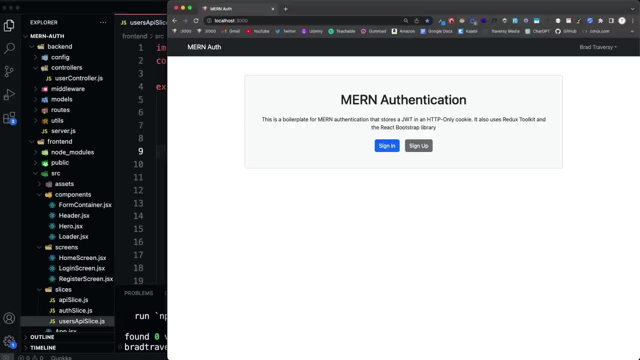 file and so on. it kind of with the thunk middleware, and it can get quite messy all right now, the last thing that we want to do is have the ability to see the, the profile, which is basically just going to be a form that has our email and name, and we also want the ability to update our email. 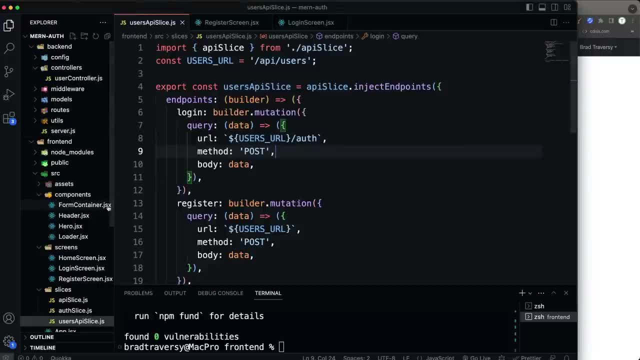 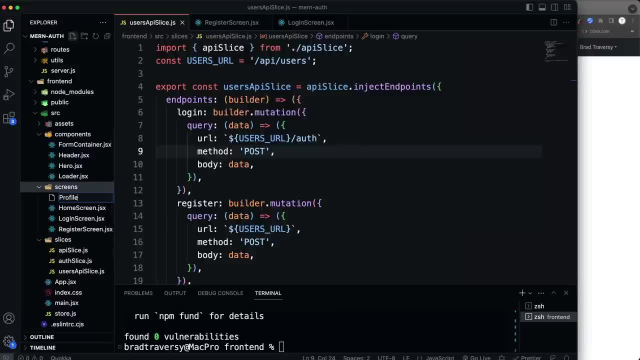 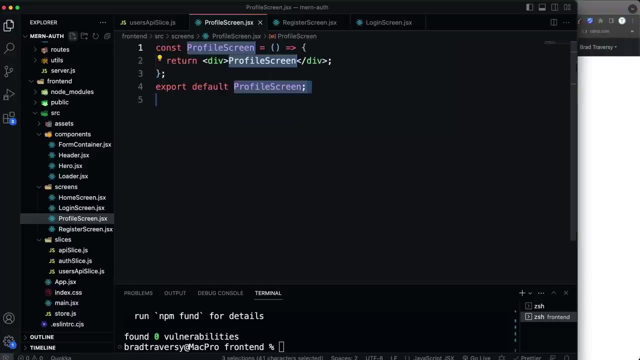 name and password, password. so let's create a new screen. so let's see screens. we're going to say new, call it profile screen, dot jsx, and for now i'm just going to do rafce and then i want to add the route. however, i don't want just anyone to be able to go to this. 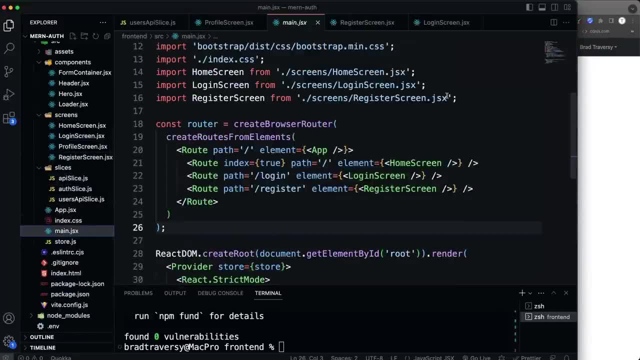 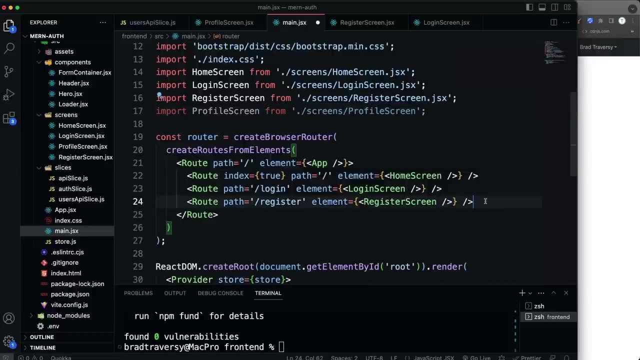 right, if i go to my main dot jsx and i bring in, we're going to want to do this anyway, so we might as well. so let's import profile screen and then, if i, you know, go ahead and do profile screen, path is going to be slash profile if i do that and then i log out. 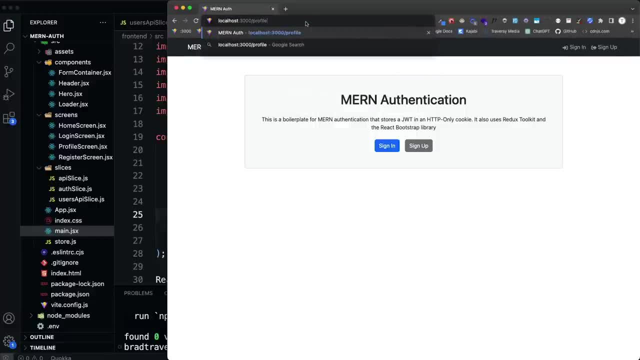 so right now i'm not logged in and if i go to profile it lets me go there, and i don't want that. i we have to be logged in now. even though in the back end we have protection against updating your profile, you still want for the user experience. you still don't want the users. 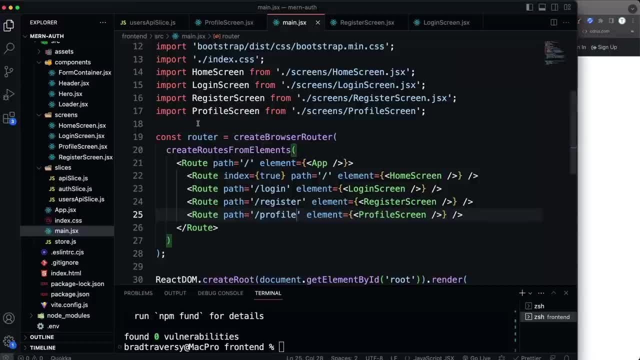 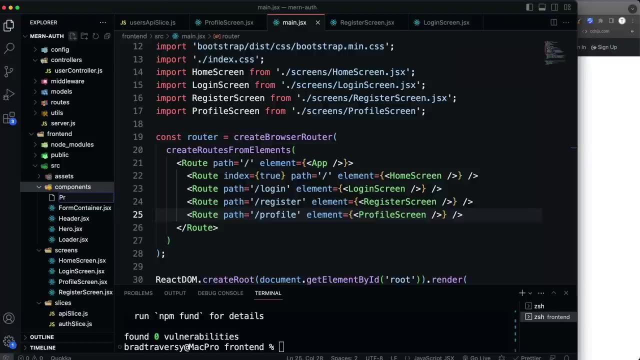 to be able to come to the profile page because there could be data that you don't want them to see or whatever. so you want to have a private route component, and that's what we're going to create. so in components, let's create a new file called private. so it's going to be called private. 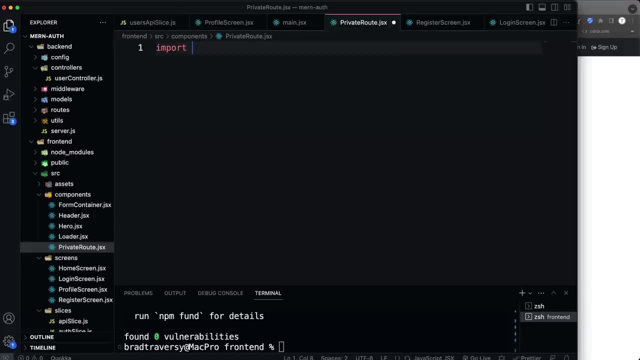 and this is actually going to be pretty simple. so we're going to just import a couple things from react router. we want navigate- not use navigate, but navigate- which is actually a component that you can use to redirect rather than a function- and then we also want the outlet, and that's going. 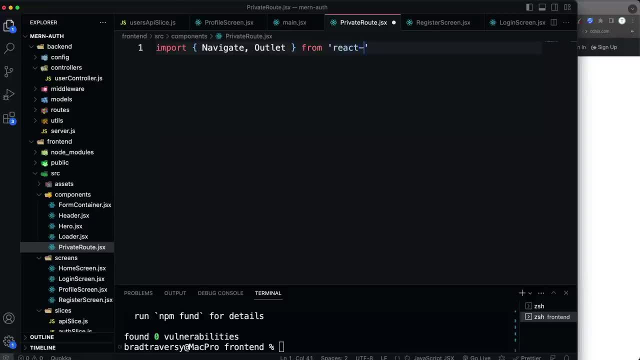 to be from react dash. why isn't it popping up? react router dom, all right, and then we're also going to use selector. i don't know why it's not popping up, but that's going to be from react dash, redux. because we want to be able to get the the user info from the state, because if there's user info, then we 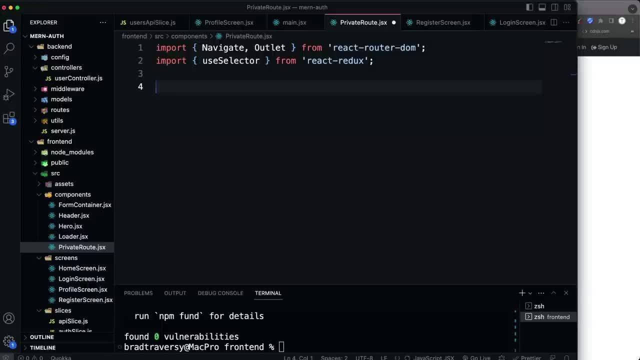 want to allow it. if there's not, we want to redirect them. so let's say, rafce, we have our private route and we're going to go above the return and get the user info. so in brackets and curly braces here we want user info and we can get that from use selector and that takes in. 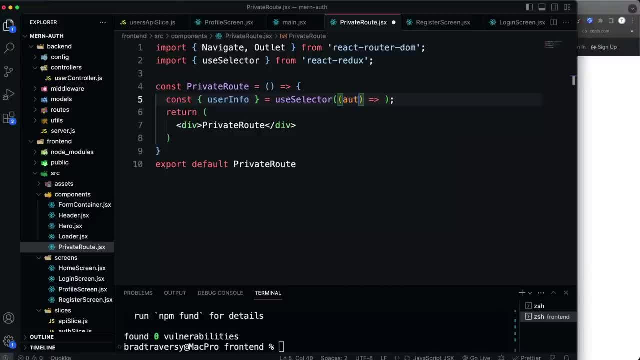 a function with off- i'm sorry- state, and then we want to get state dot off that'll give us the user info. then what we want to return here depends on if there's user info or not. if there is, then we just want this to be the outlet which will show us the state dot off and then we want to get the. 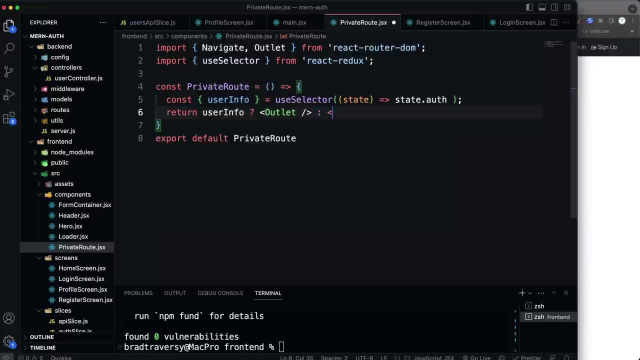 user info and then we're going to do that inside of the port and we're going to show whatever the route is. else then we want it to navigate, so we're going to use the navigate component which takes in a to at two prop and that'll go to slash login and we're just going to add, replace onto. 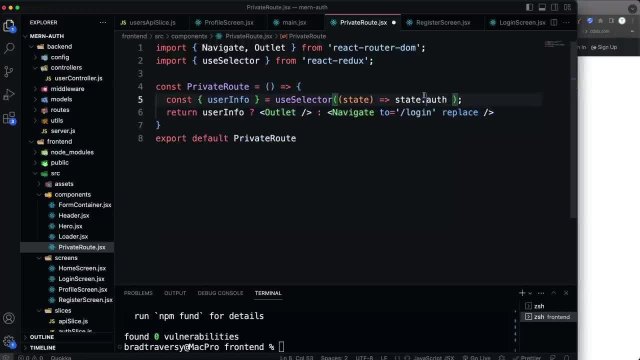 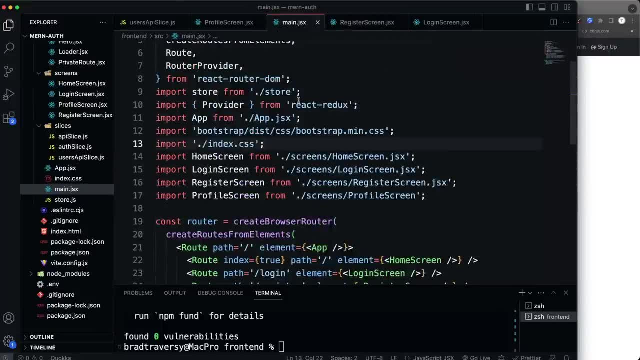 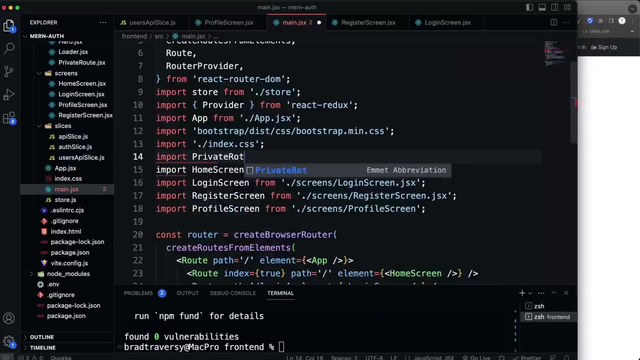 this too, or it could give us some crazy stuff. so now, and that's pretty simple, so to implement this, we go back to our main dot jsx and we need to bring that component in. so let's say, import private route. it's really annoying that's not auto completing. import that from dot slash. 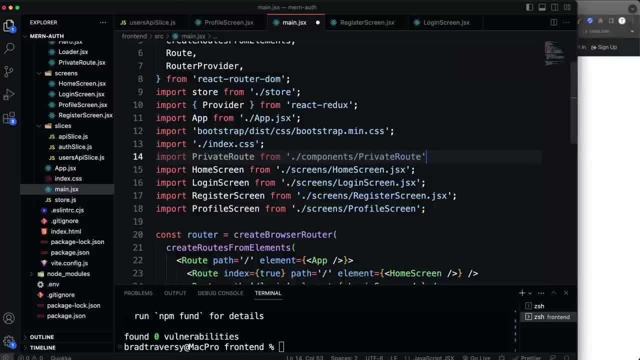 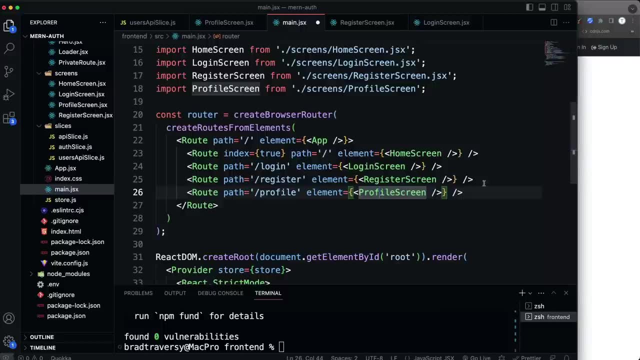 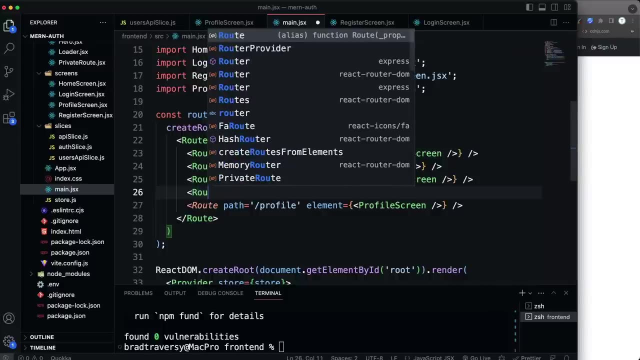 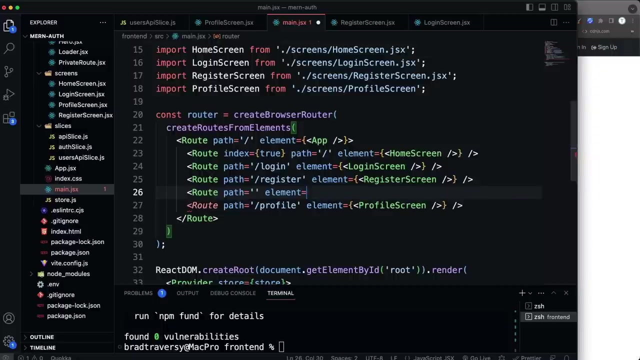 component slash private route, and then what we have to do is just basically wrap whatever. whatever routes we want to be private, we just want to wrap with that, with a route component, and for path we can just put an empty string and then for element we want to set. 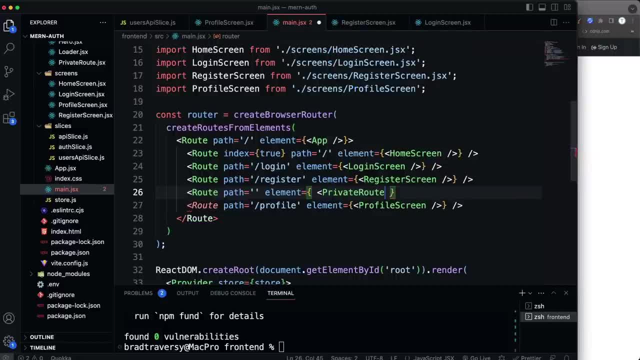 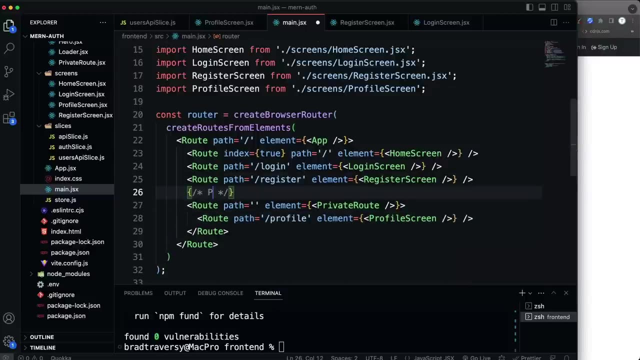 that to the private route. so we want to say private route, make sure you put an ending angle bracket. and then we want to move that into there. okay, and we could even put: we could put a comment right here and just say: private routes, okay you. so anything else private, just make sure you put it in between here. 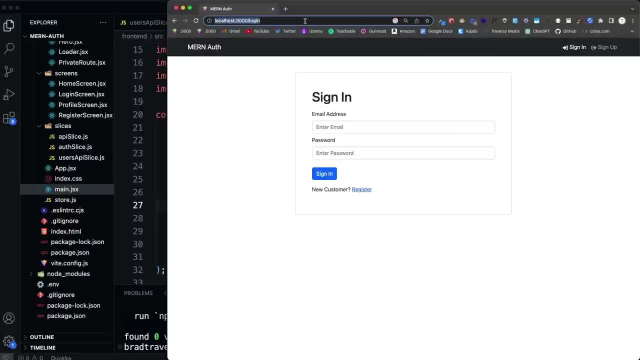 now i'll save that and notice it took me to the login. if i try to go to profile, i can't now log in. i'm going to log in as brad at gmail and now, if i go to profile, it lets me. okay, now the profile screen. 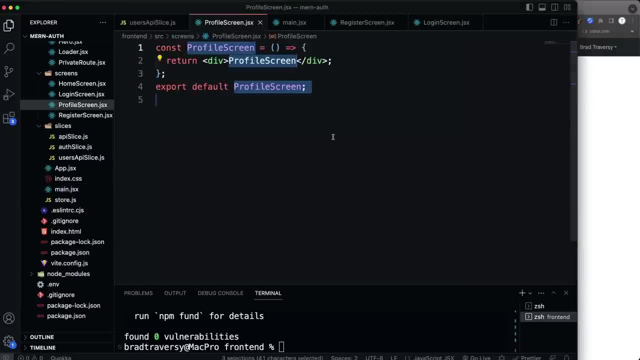 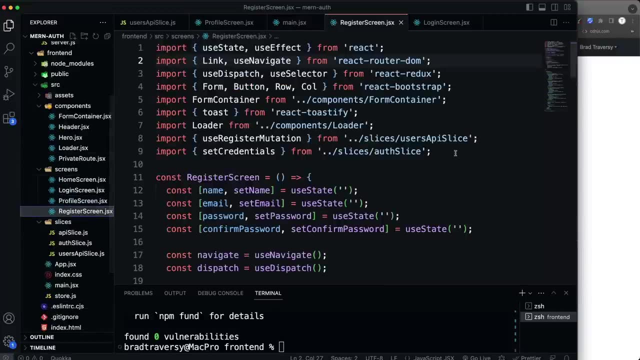 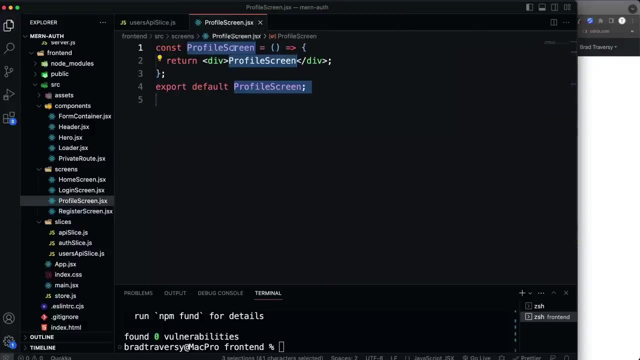 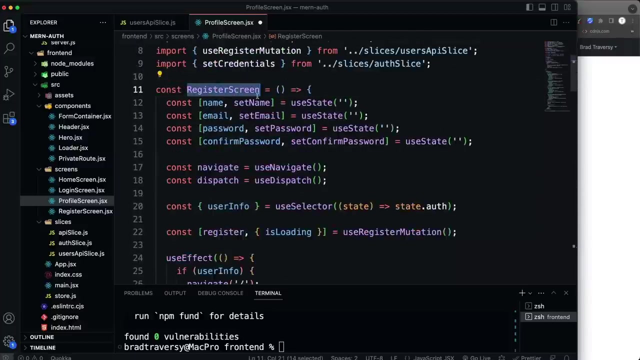 is going to be pretty similar to the other forms, um. so i think what i'll do is copy. let's see, let's copy the register screen here, and then we'll go and close that up. close that up, yeah. so i'm just going to paste in the register screen, but i'm going to change the name of the component here. 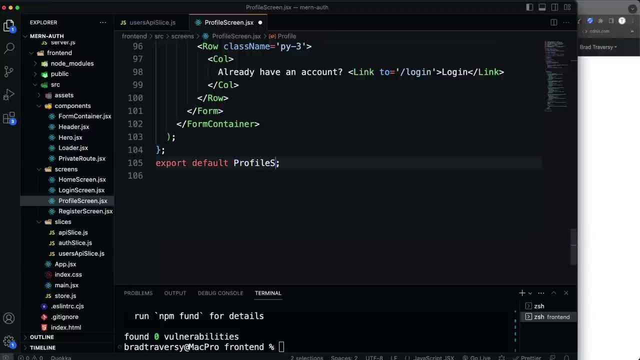 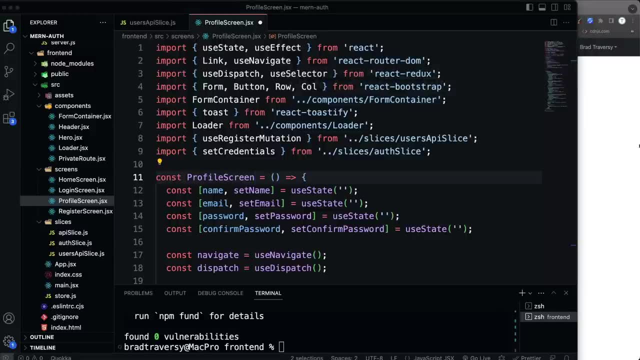 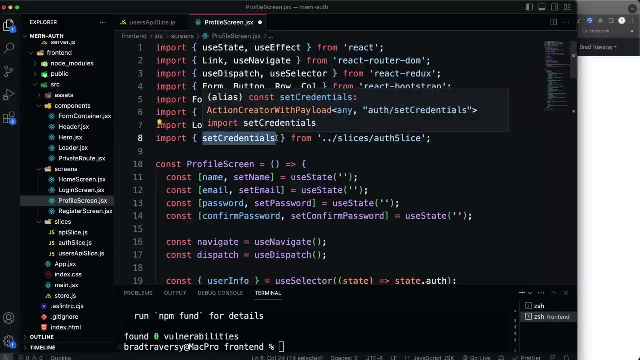 and then at the bottom to profile screen and let's see we're going to go up to the top here and figure out what we don't need. we don't need the register mutation. we're going to keep set credentials because if they change their info we want to reset the credentials, right, um loader will. 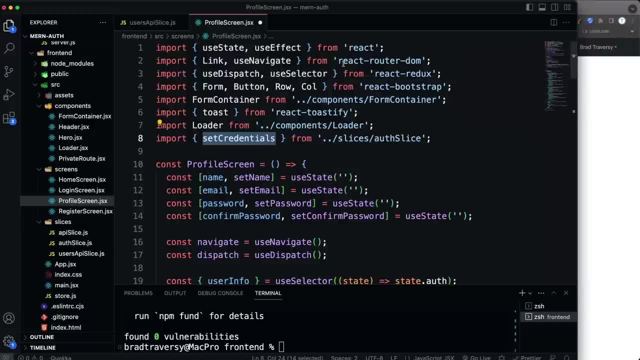 keep that toast form. yeah, i think we're going to pretty much keep all of this stuff. we don't need row and column though, so we're going to keep that, and then at the bottom to profile screen, and then we're going to go and close that up, close that up, and then at the bottom to profile screen, and then. 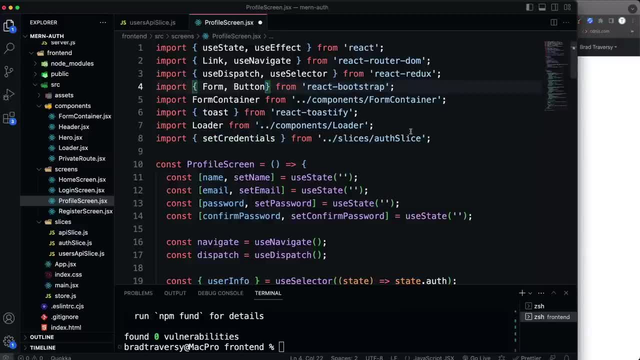 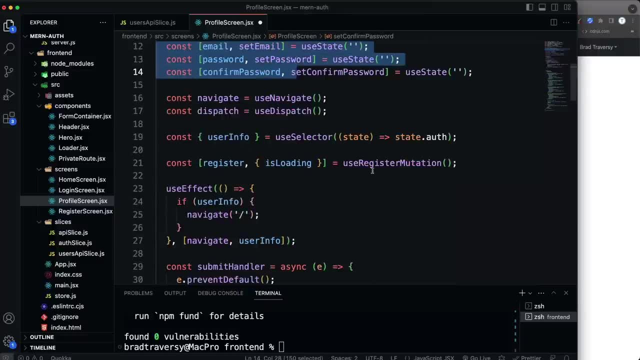 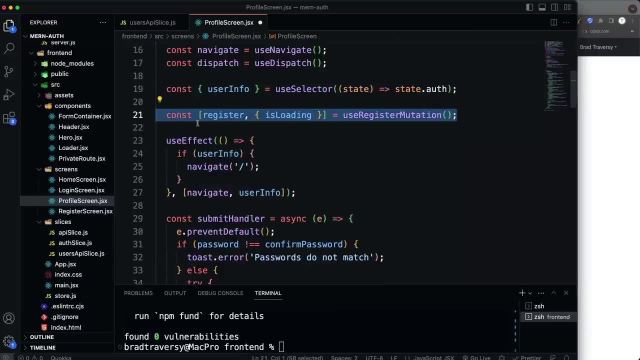 because we don't need that last part where it says you know not registered. then log in and then let's see for the state. we're going to keep the same stuff here. we're going to keep that. we want to get the user info. we don't want the register mutation. we can get rid of that. 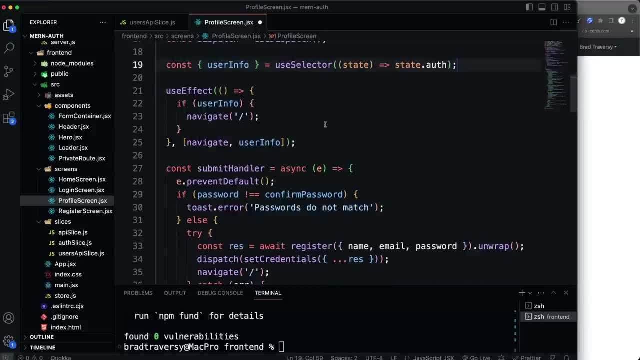 so for the use effect, what i want to do is fill. we're not going to redirect here, because obviously, if you're logged in, if the user info is there, you don't want to get the user info, and then you can just go ahead and do that, and then you can. 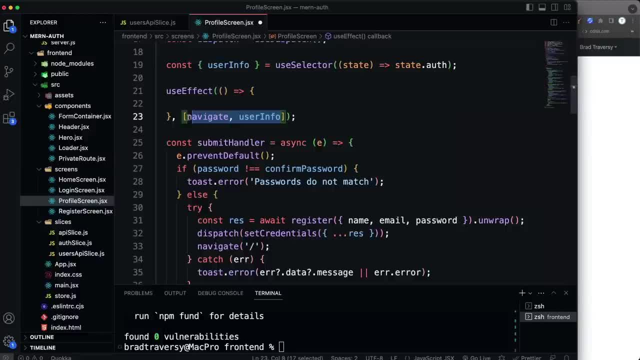 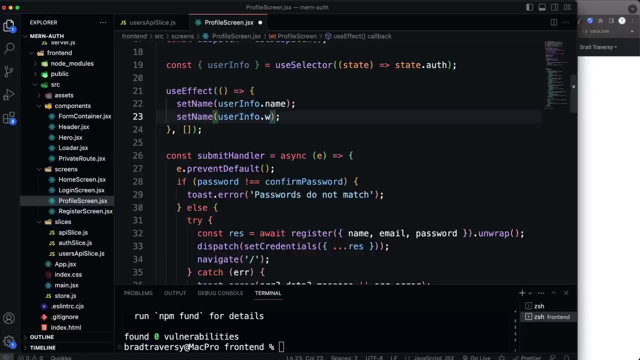 redirect so we can get rid of that and get rid of these dependencies. but what i do want to do here is set the name to whatever is in user info dot name, and i want to do the same for email, so this one will be set email, and then we just need to add into here user info. 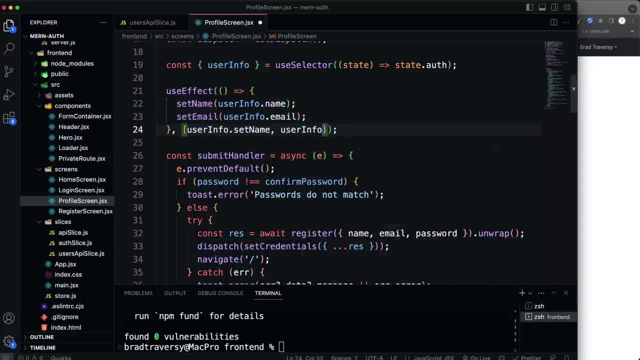 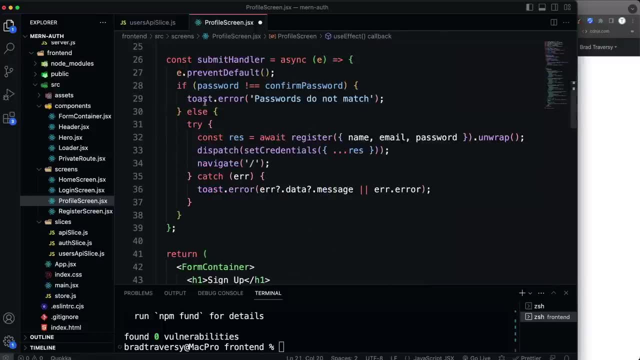 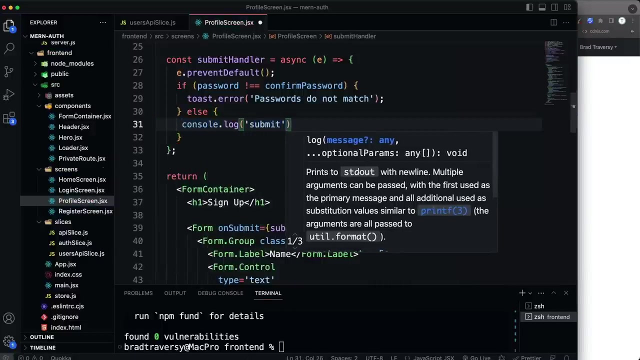 dot set name, user info- dot set email. okay, and then let's see: submit handler. we're just gonna. we want to keep the password check, but this stuff here, the try catch, i'm going to just get rid of for now and just say: consolelog submit. i just want to get the form displayed right now, so moving. 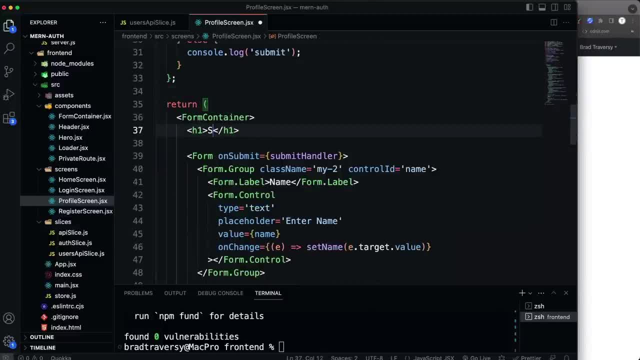 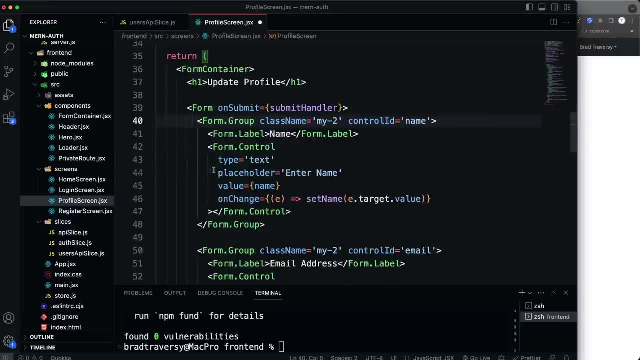 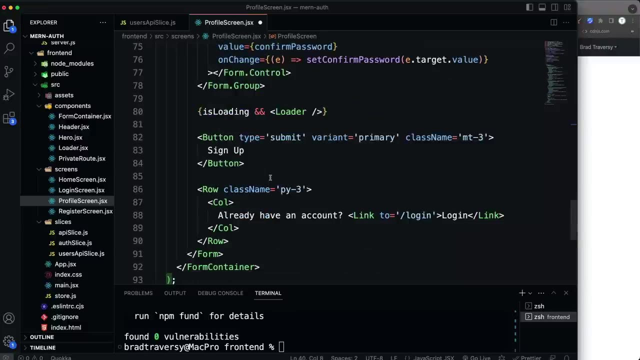 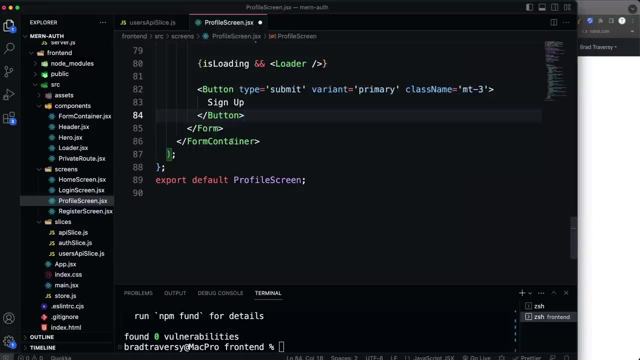 on down here. let's change the title here, the h1- to update profile, and then let's see we have our form group for the name, so this stuff can pretty much- yeah, this can all stay the same, except at the very bottom where we have this row. we don't need this part, so we can get rid of that and let's change. sign up to update. 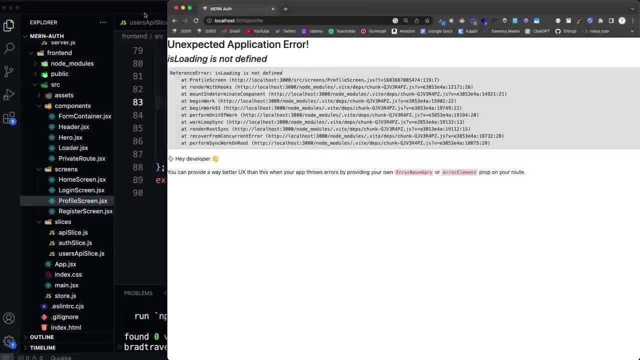 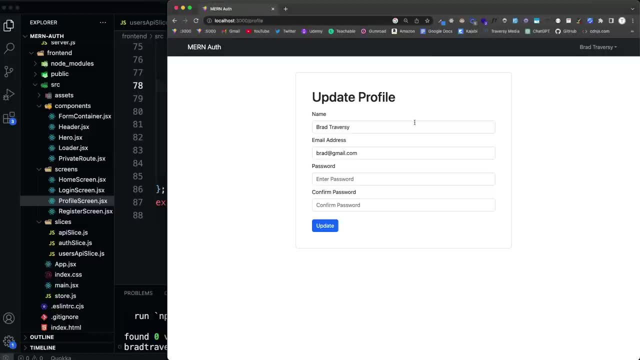 to update. to update is loading is not defined. oh so right here, we're going to get rid of that as well. And there we go. So we have user profile and it has my name and email. We're not going to pre-fill the password, but we will be able. 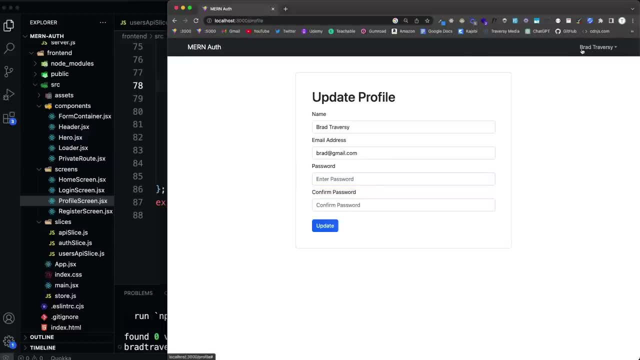 to update the password. We're going to do that in a second, But yeah, so now we're logged in, we can go to our profile screen here and the last step is to be able to update this. So, again, in order to do that, we're going to go to our user API slice and we're going to 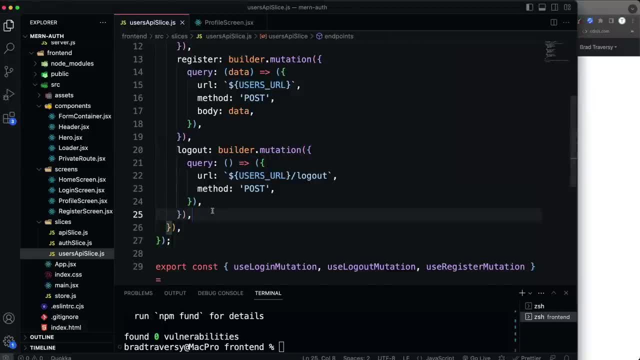 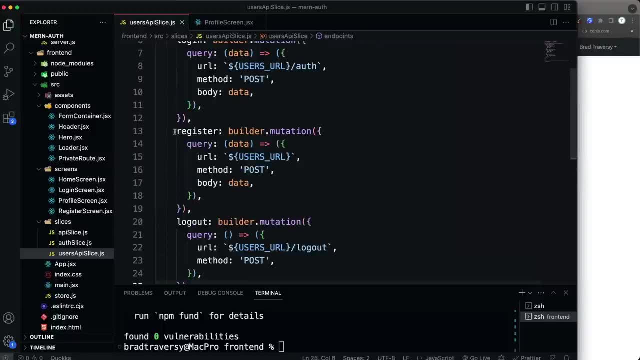 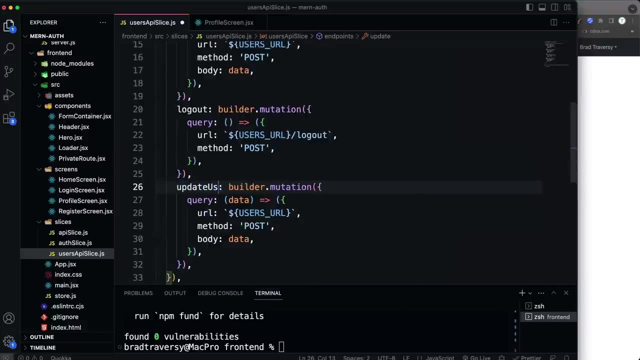 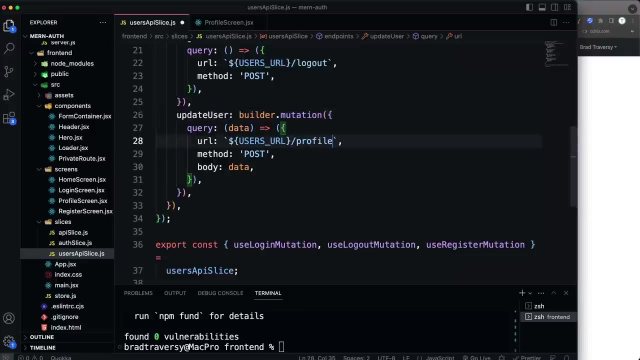 add to this. Let's go under logout and let's say update user. Actually, I'm just going to copy, I'll just copy register And we'll call this Update user And let's see it's going to be users URL slash profile, but it's going to be a PUT request. 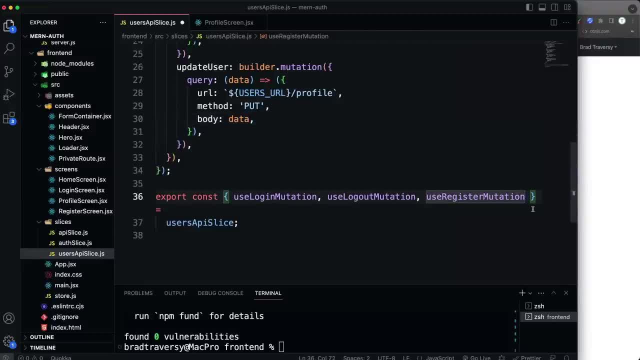 And we're going to send data And then we're 006必須罄 W изв, then it's going to be a PUT request And in that case we don't have to want to export it with use. let's see what are we going to call it: use- update- user mutation. 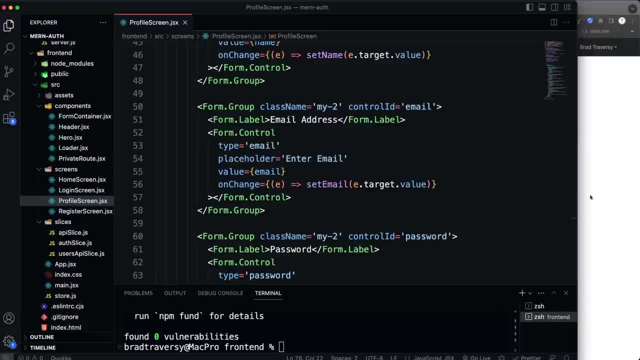 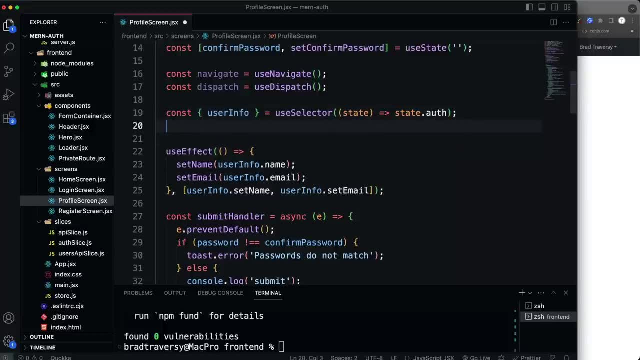 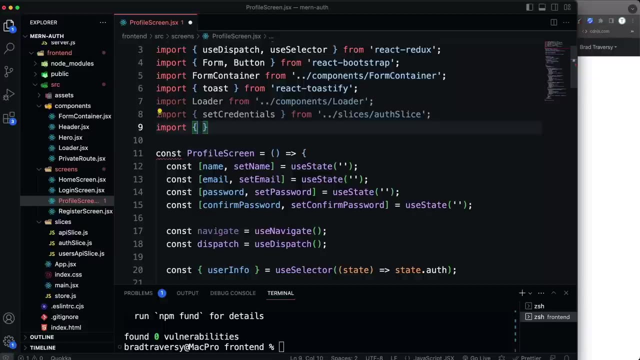 and we can close that up. so now in our profile here, let's bring in up at the top. we'll go right here and say, con. actually, first of all we need to bring the mutation in. so let's import, use, use, update, user mutation from dot dot slash slices. 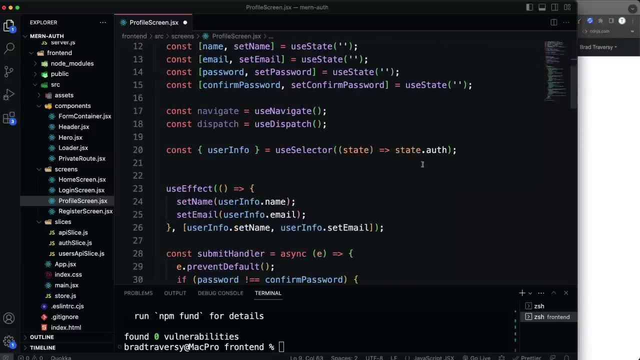 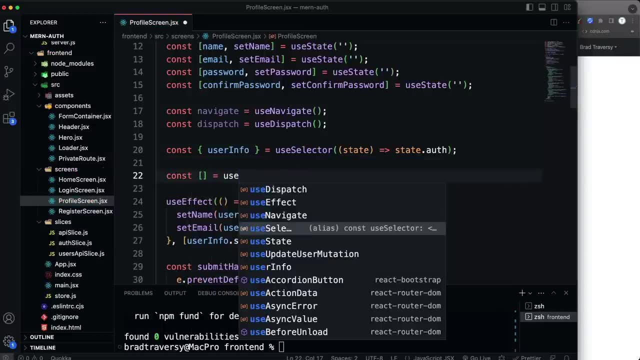 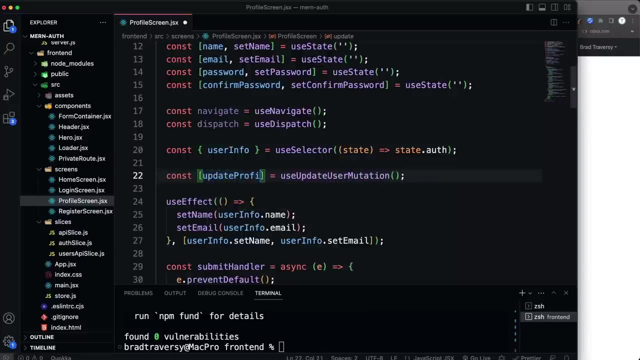 users api slice and then we'll go right under where we get our user info and let's say cons with brackets, set that to use update user mutation and i'm going to call this update profile and we can also get is loading so that we can put that loader back. 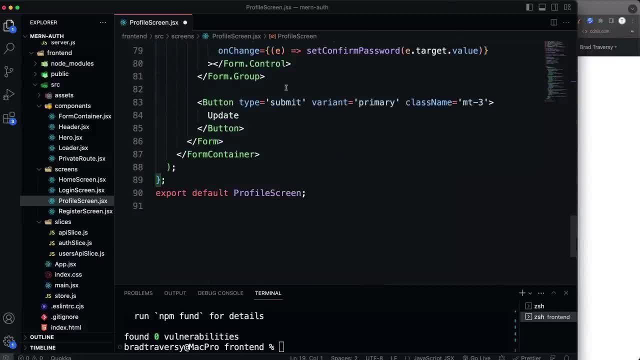 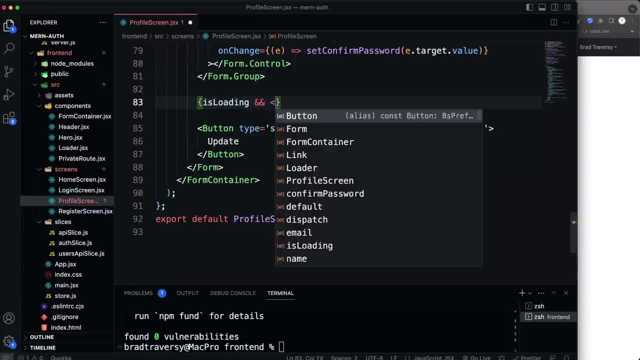 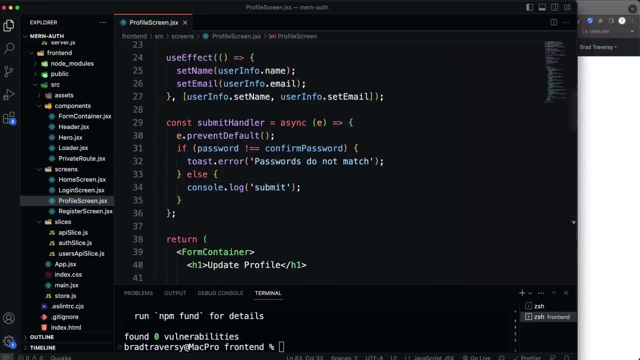 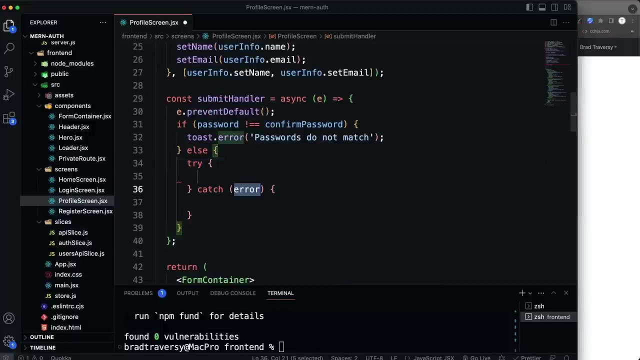 okay. and then, yeah, let's put the loader back. so right above the button oops, we'll say is loading? then show loader. okay now in this submit. so right here in the submit handler, we're gonna get rid of this console log and let's put our try catch back and in the try we're going to say const res. 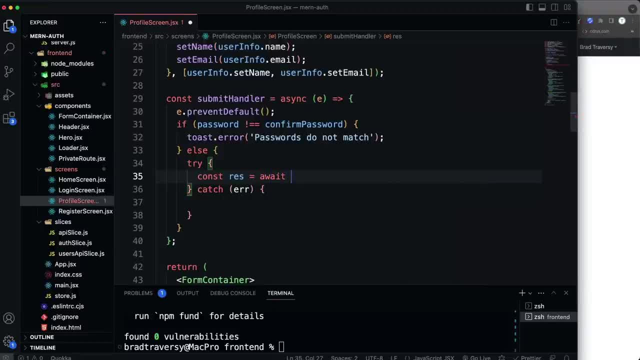 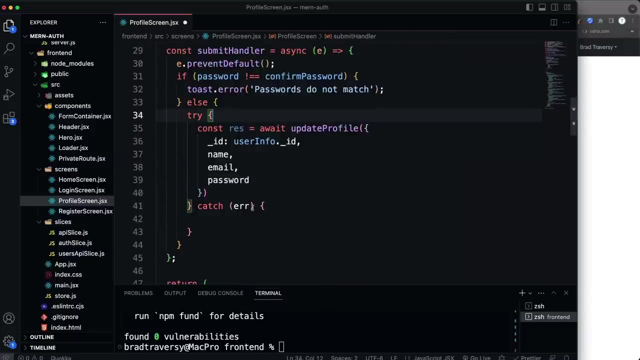 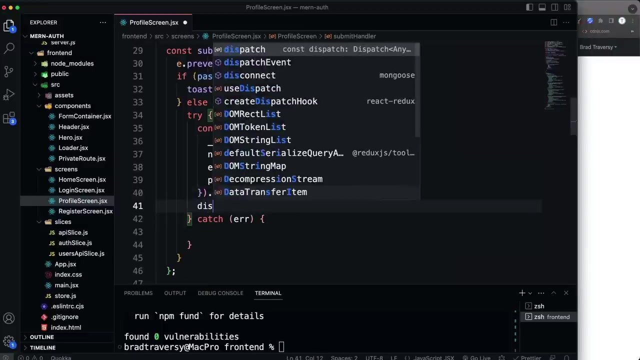 set that equal to await and call update profile. now that's going to take in an object with underscore id. set that to user info dot underscore id and then name- uh name, email and password. okay, and we do want to unwrap that as well. and then we want to dispatch. 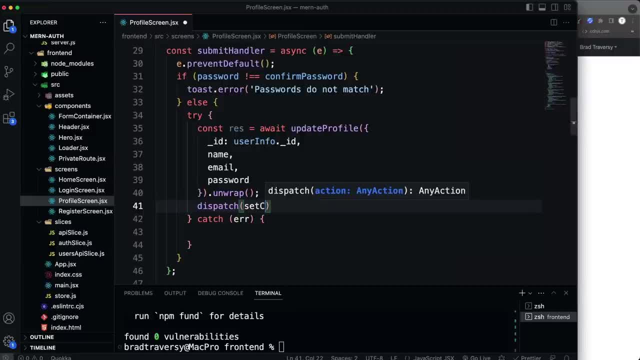 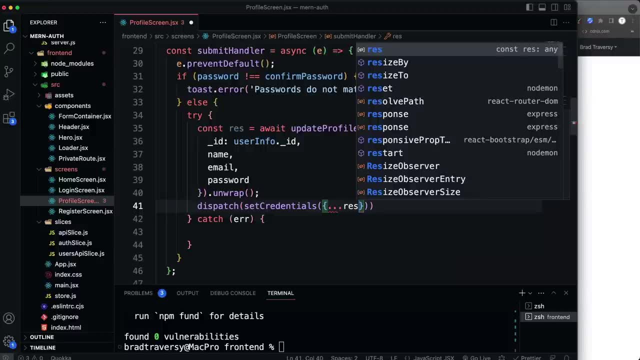 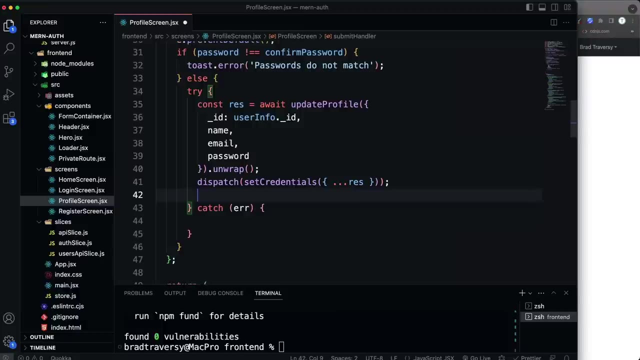 we will open those and then, once they show, now we will go back in here and we will功 to slowly index this number. so if we click on this type set credentials and then here we will actually be able to attach the set credentials, so set credentials and we're going to pass in there an object spread across res. 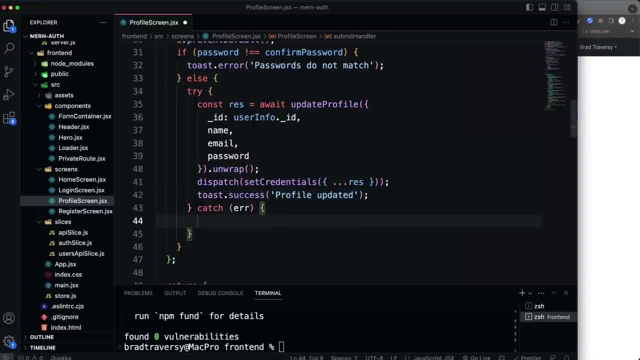 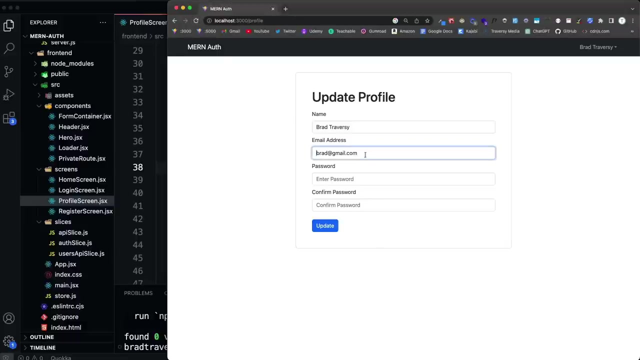 or we could just pass in res and then let's do a success toast, so we'll say toast, say toast dot error, and we'll pass in here err dot data dot message or err dot error, so that should let us update. so let's come over here now and i'm just going to change my email to: 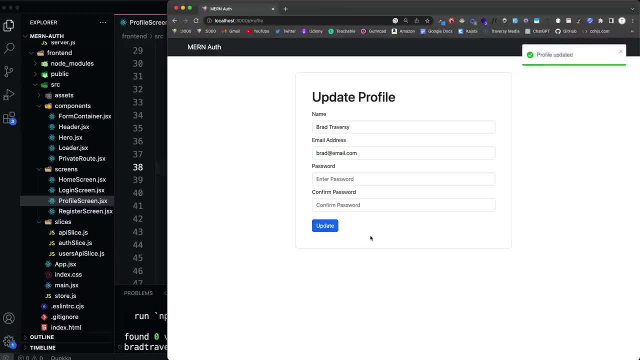 brad at emailcom and update. so it says profile updated. if i reload, it's still brad at email. now if i log out it it we should be able to log in now with brad at email instead of the gmail. so there we go. i was able to update it, so if i want to update my name, i'll just say: 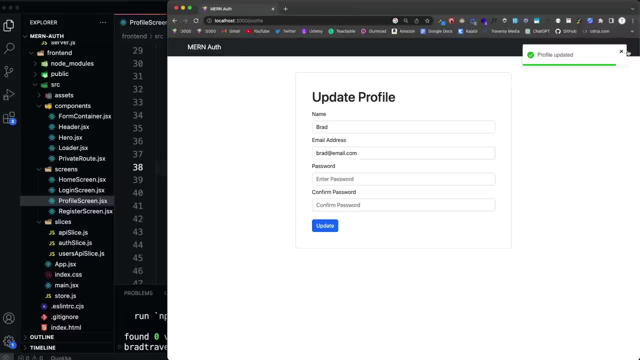 just change it to brad and click update and notice it also updated right here as well. this reacted to to our update. okay, so i'm mean that's pretty much it and it's. you know this took a while and i mean it's quite a bit of code. 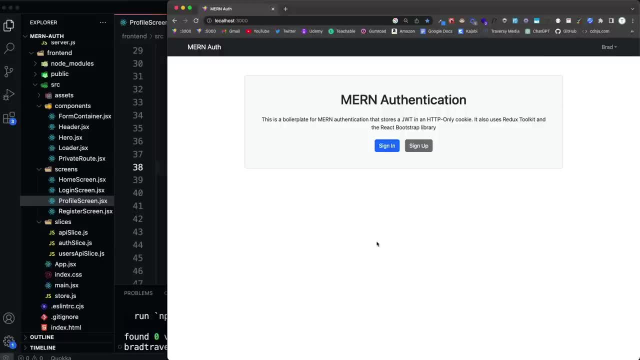 for small functionality, but you can now use this as a starting point for other single page applications- mern, stack applications- where you want to use this authentication system and it's easy to protect your routes because we created that off middleware in the back end. it's easy to create private routes on the front end. so, yeah, that's that. so in the final part of 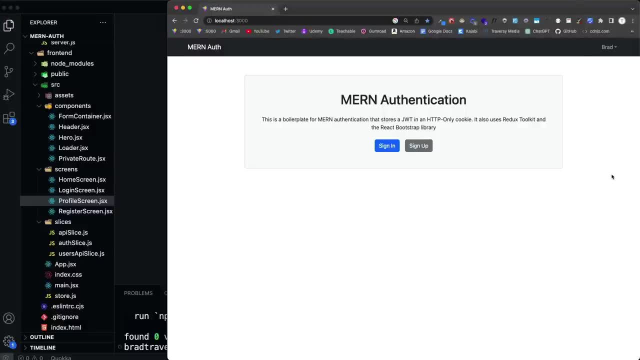 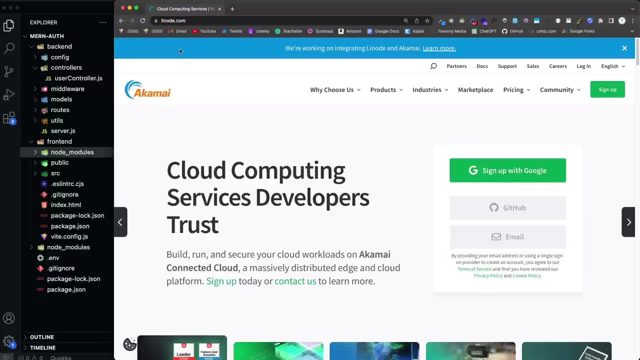 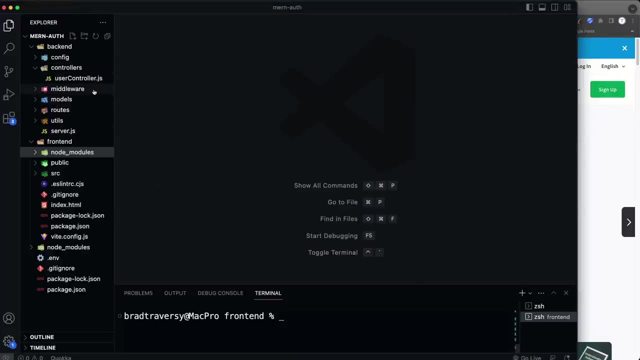 this video in this project we're going to deploy to linode. all right, so we're going to get ready to deploy to linode, slash akame, and there's just a couple of things we need to do to prepare for production. so right now, what's going on is we have our back end that runs on localhost 5000. 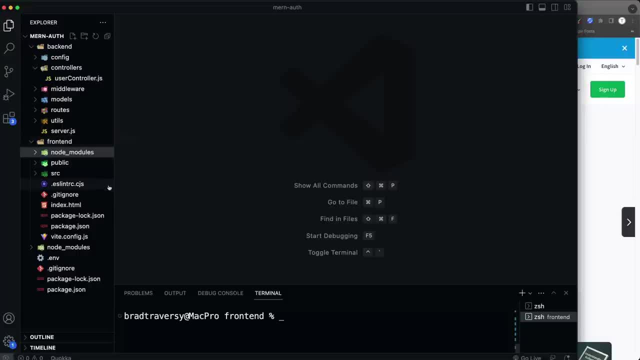 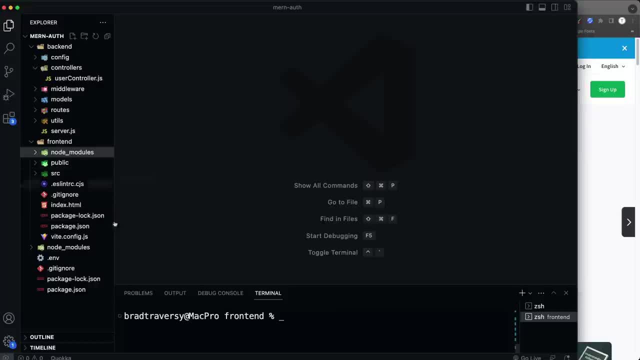 dev server. so what we need to do is build out our static assets with npm run build, and then we need our back end server to point to the index html that's in that build folder or that dist folder. so let's go into the terminal and make sure you're in your front end and let's do npm run build. 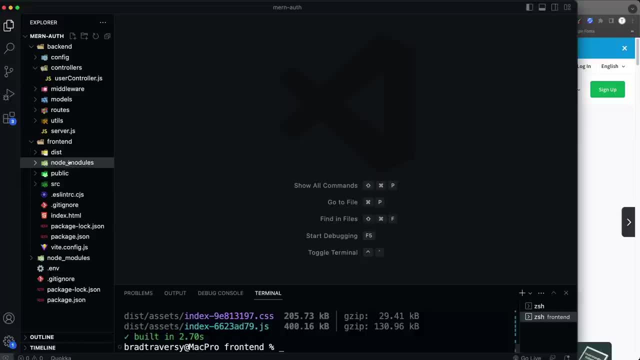 and what this is going to do is build out our static assets. if you're using veet, it'll be in this dist folder, right? and if you're using create react app, it'll be called build. okay, the folder will be be called build and inside that is the index html, which is basically the entry point to our react. 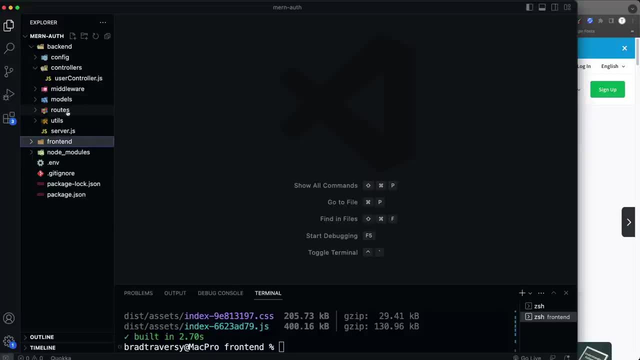 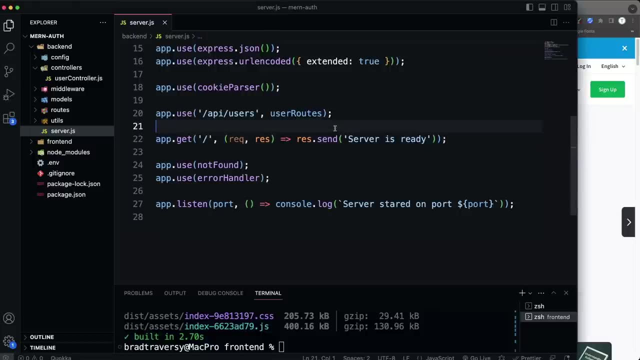 application in production. so we're going to open up our serverjs and we're going to go down here where i just have this, this index route that says server is ready. i'm going to go right above that and i'm going to open up our serverjs. and i'm going to go right above that and i'm going to. 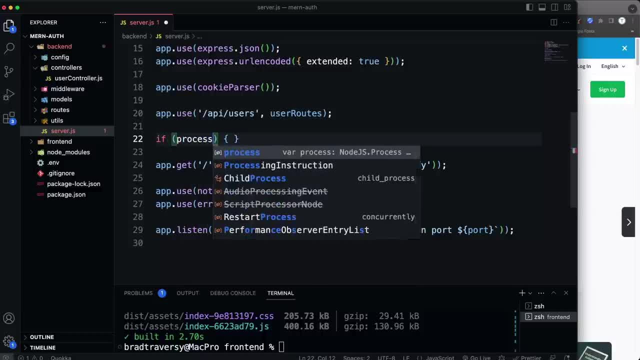 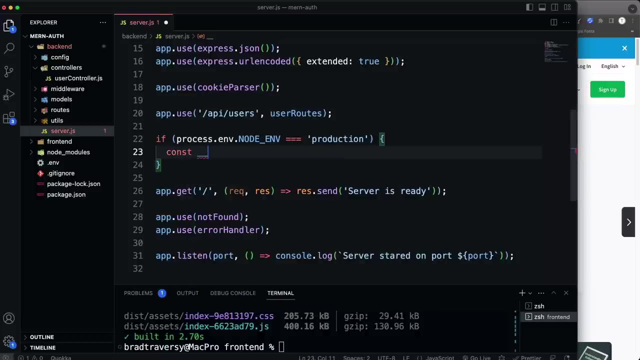 check to see if we're in production. so let's say, if process dot env, dot node underscore env is equal to production, okay, so if that's true, then first thing i'm going to do is just set a variable of double underscore dirname and set that to path dot resolve. 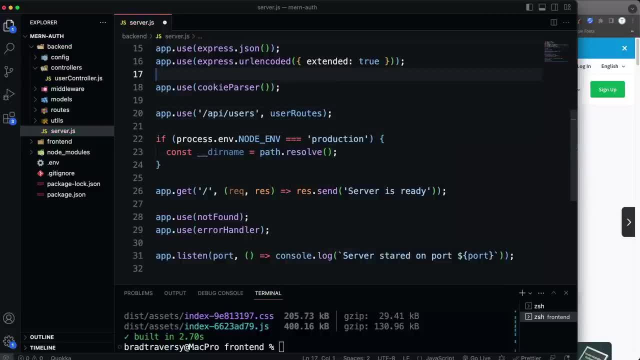 now the path module is part of nodejs, so we just need to bring it in up to that field. now that we've added that Muse개 root ela keyword in ourği module and a second небaba, i could go ahead and addzzo: do we pops this worked or not? we need to install that as well, so we can go on to bit morelite. let's go ahead. 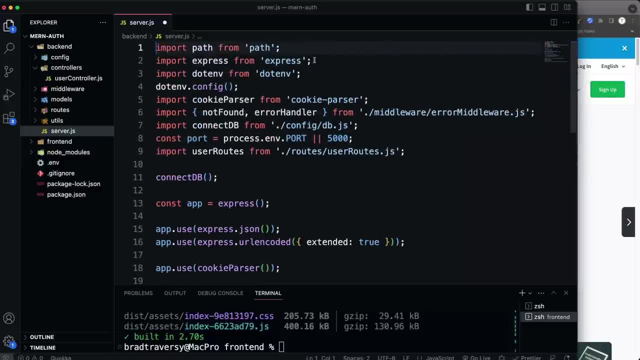 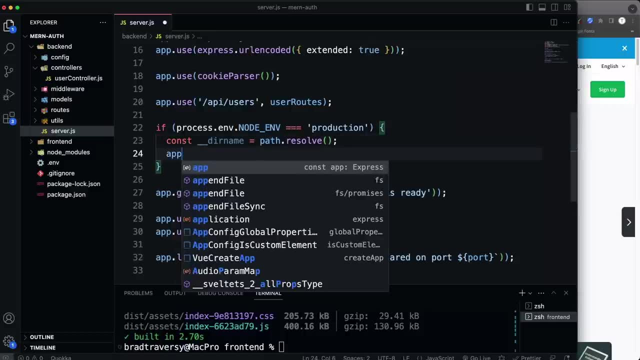 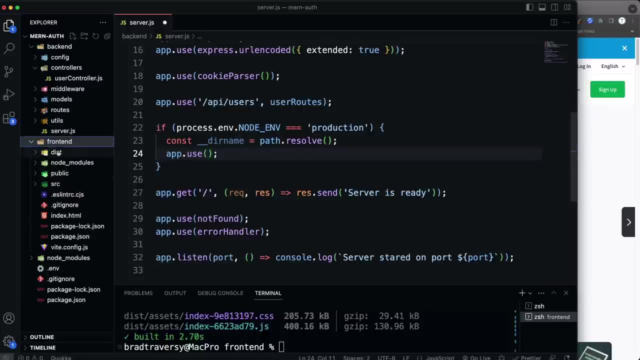 to bring it in up top. we don't have to. oh, i actually already did so. just make sure you import path and then we're just setting the root directory and then we're going to run appuse and we want to make this folder so front end dist. we want to make that a static folder so we can. 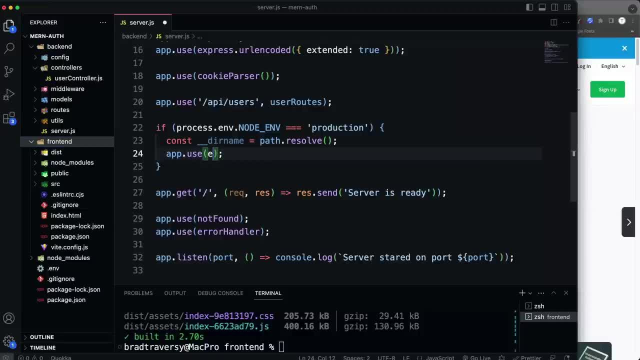 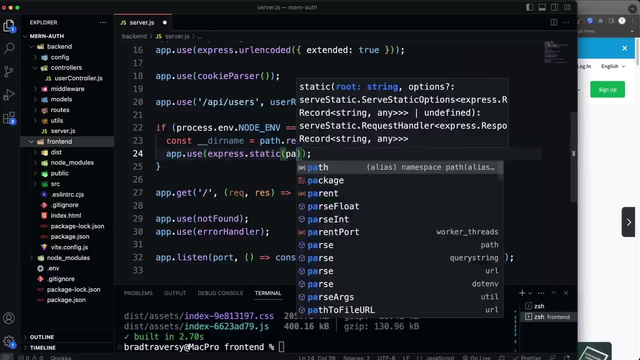 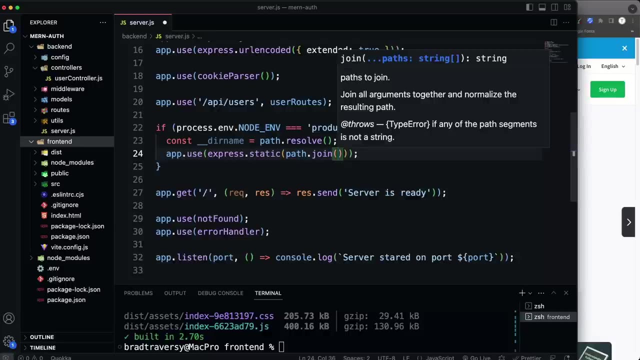 just access it directly. so in appuse we can say express, dot, static and then we just basically want to point to that dist folder. so i'm going to use pathjoin to join together our folders and files and in the join we're going to add our double underscore dir name and then we're going to add: 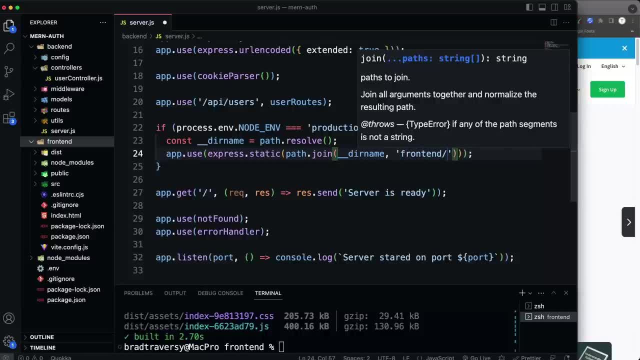 front end slash and then dist for me because i'm using veet. if you're using create react app, you'll want to put front end slash build, all right, and then what i'm going to do is add a route. so make sure you're in this if statement. 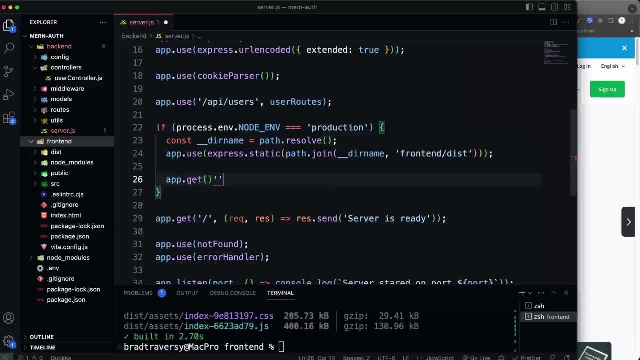 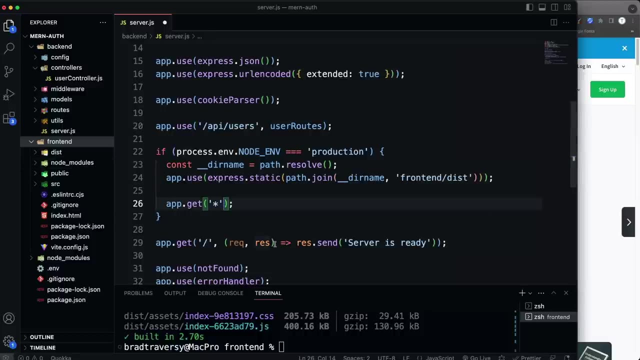 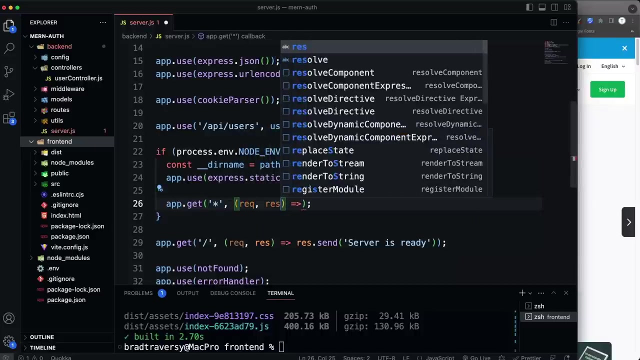 and we're going to say appget and we're going to use just the universal wildcard character, the asterisk. so if we get any routes- that's not, you know, api slash users- then we want to just show the dist index html. so let's add our callback here. so request response and then what i want to do here. 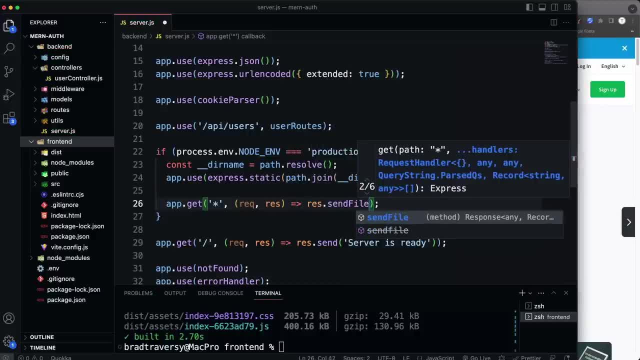 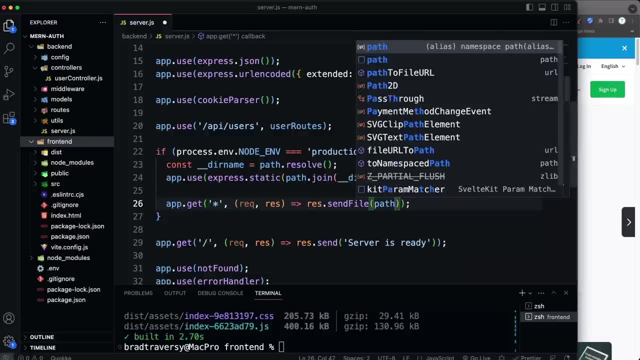 is res dot. and then we have a send file method, because that's what we want to do, is we want to basically direct them to that index html. so now in here we can say path dot resolve and let's close that up and in the path resolve. 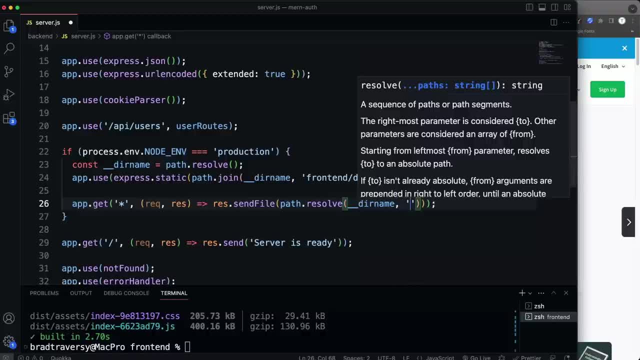 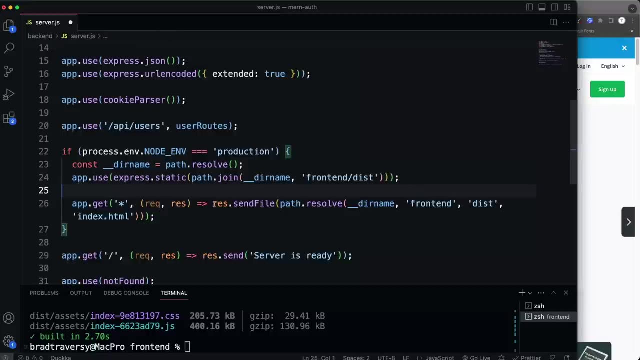 i'm going to add double underscore dir name and then from there we want to go to front end, and from there we want to go to the dist folder or the build folder, and then from there we want our index html. okay, so we're, we're making this disc folder a static folder with this line. and then here we're. 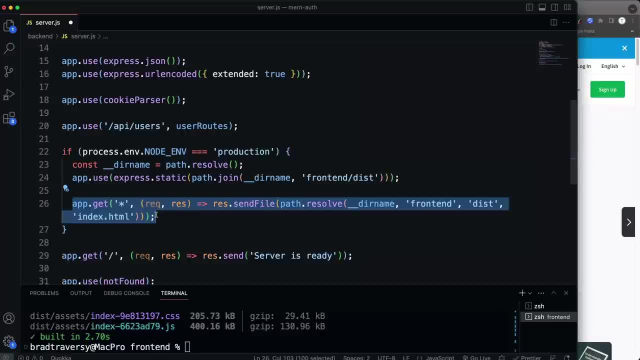 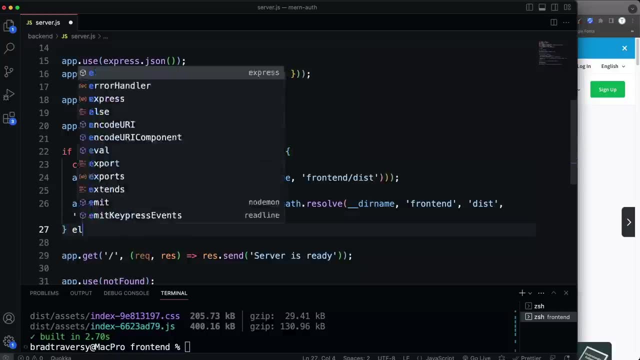 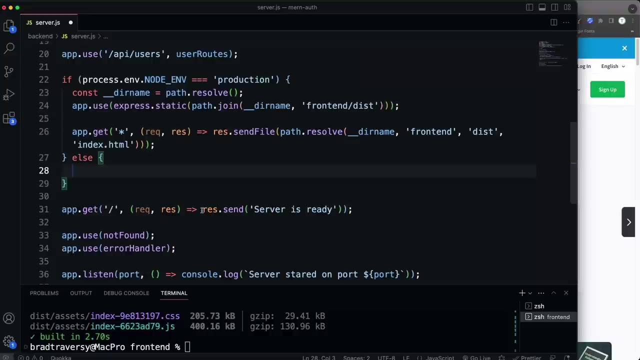 saying any route that we hit. that's not this. api users is going to load that index html now in the else, so else meaning we're in development, then we don't really need to load that index html because we're using the v dev server or the create react app dev server. so what i'll do is: 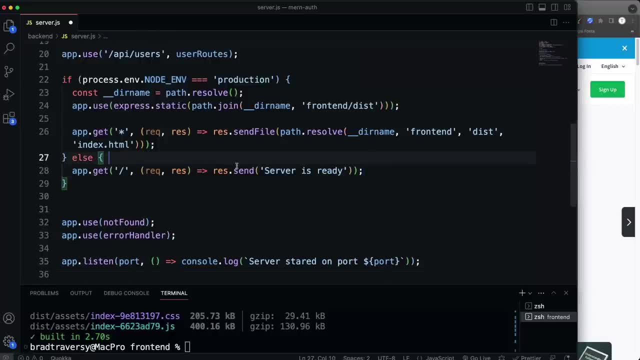 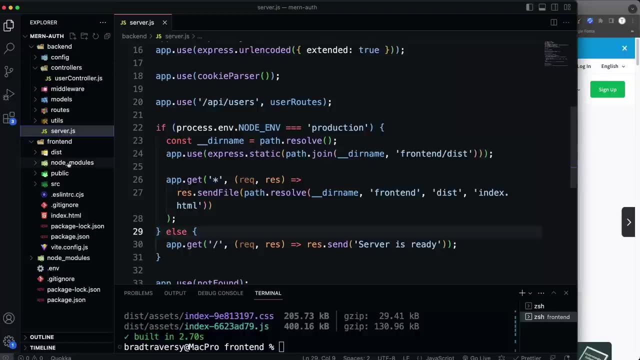 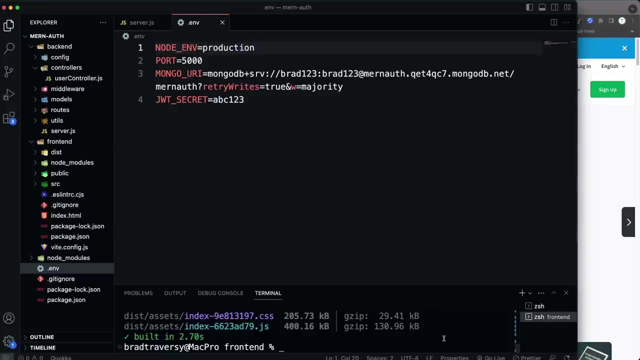 just put this in here and it will just say: server is ready. all right, so now to kind of test this out before we actually deploy. excuse me, we're going to go to our env and let's set it to production. so now, if i run just the server so i'll go into my other terminal here. i can stop that. 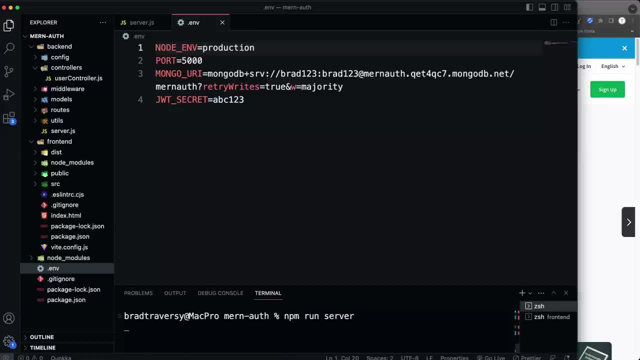 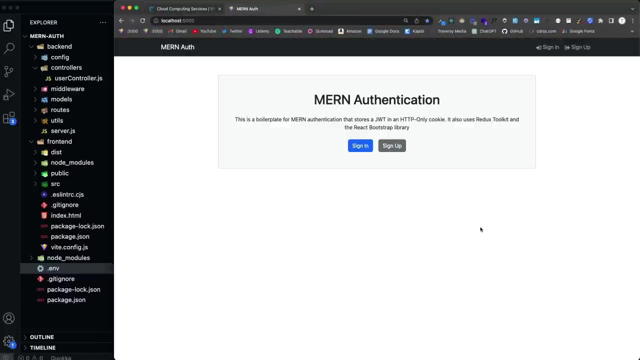 and if i run npm run server, remember that runs just express our localhost 5000. but since we compiled our front end into this disc folder and we set that as a static folder and we set it to point to it now if i go to localhost 5000 it takes us to our application and if you have the react, 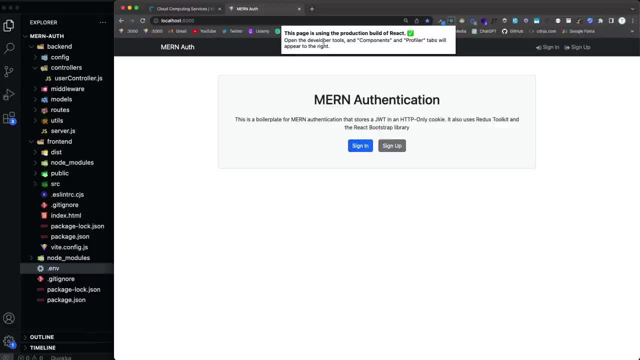 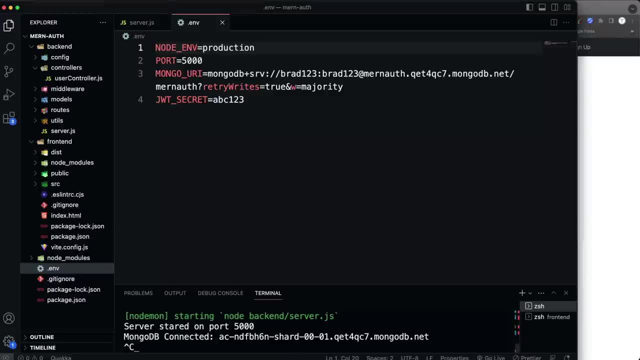 extension installed in chrome. you can see it's. it will say: this page is using the production build of react rather than the dev server. all right, so now we should be ready for production or to deploy. so i'm gonna just uh, you know, this dot env really doesn't matter, it's not gonna go onto the server, we're gonna. 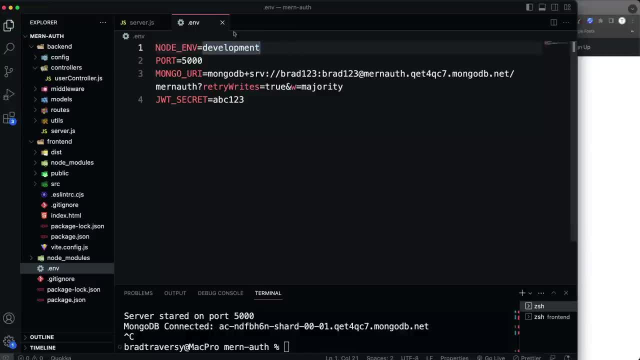 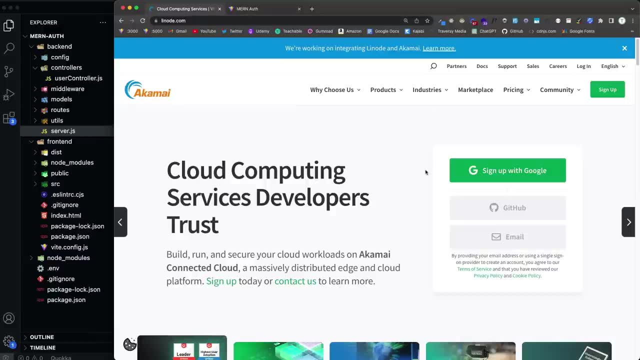 create our own dot env on the server, so i'm gonna set this back to development. okay, now what we want to do is go to linodecom and, of course, if you don't have an account, create one and again. i have that link in the description to give you a hundred dollars free over 60 days. 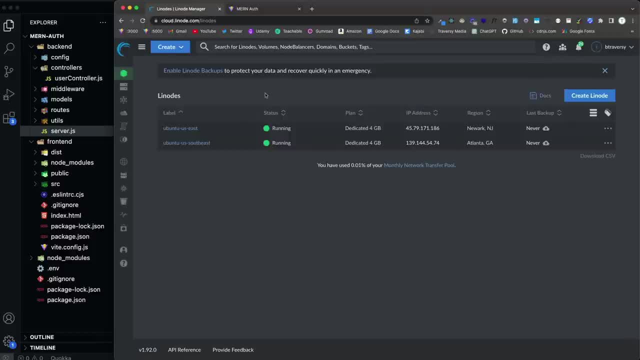 so i'm going to go ahead and log in and you're going to see a dashboard like this and you can see i already have a couple of nodes here, and linode is just what they call these little servers. they're basically just linux instances and they can be different, uh, different. 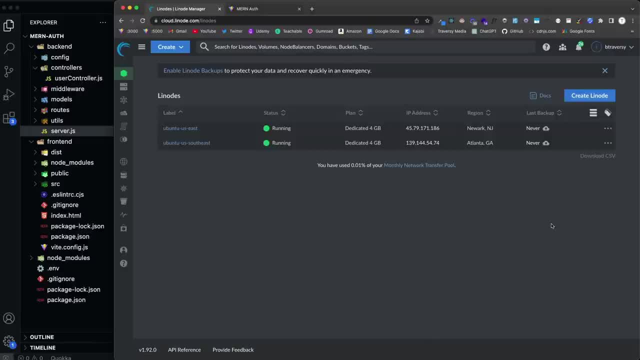 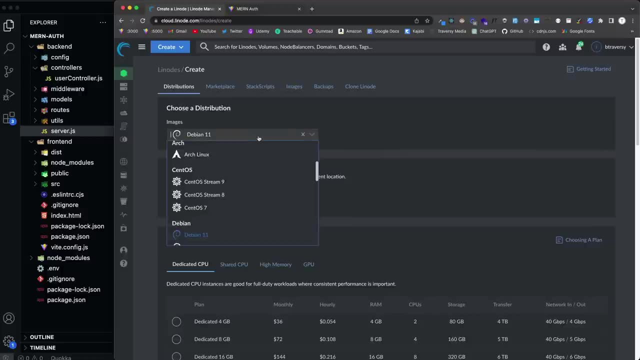 distros too. i like to use ubuntu, but you can use just about anything. so first thing you're going to want to do is create a new linode, and the default distribution is debian 11, but again, i like to use ubuntu, so i'm going to choose ubuntu 2304, and then you want to select a region, that's. 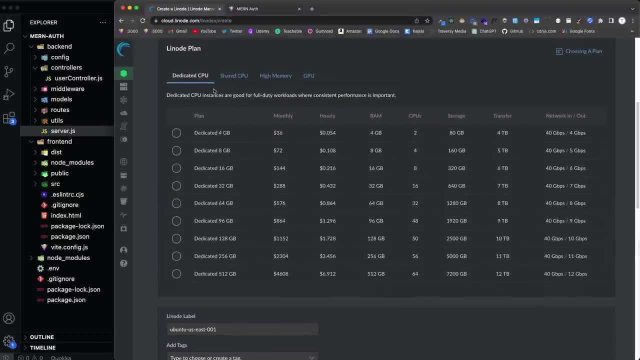 close to you, select new jersey. and then, as far as the plans go, i'd suggest this one here: dedicated four gigabytes, which has a cap of 36 a month, and remember with that, that link that i gave you- you're going to get a hundred dollars free over two months, so you'll be able to use this package. 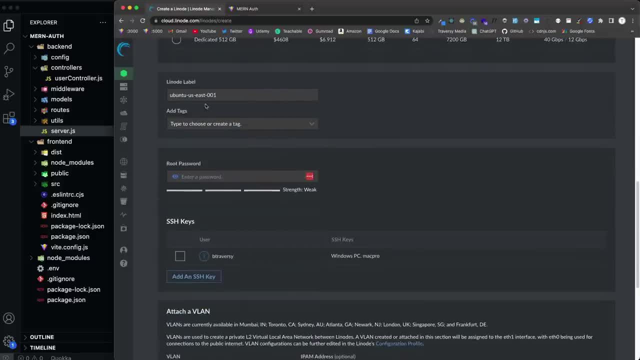 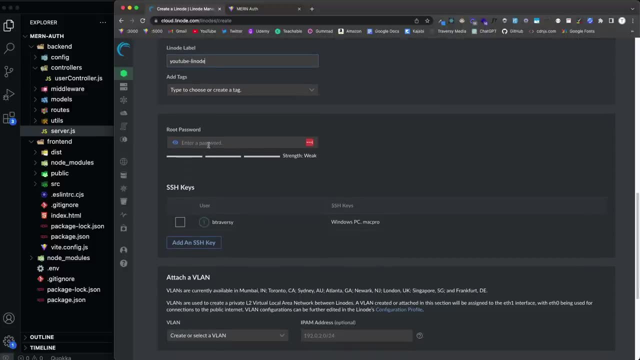 for free for two months. okay, and then let's come down here. you can rename it if you want. i'm just going to call it youtube dash linode and then enter a root password. make sure it's secure. actually, i don't think i typed that right. 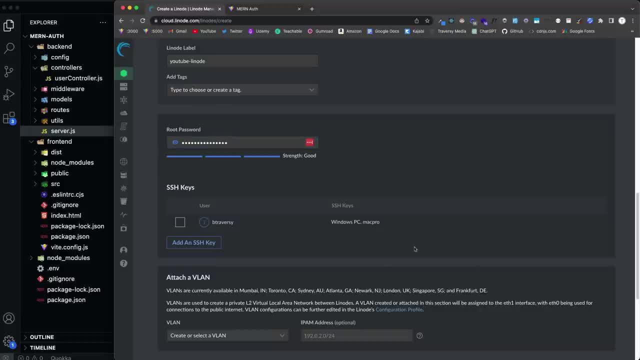 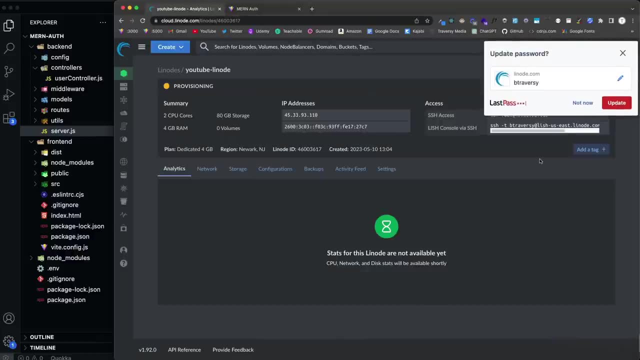 all right, and you can also set up ssh keys. you can see i i do have one set up, and then that's it. let's click on create linode and it will just take a few minutes for your analytics to show up, but your server should be ready and this is your ip address. 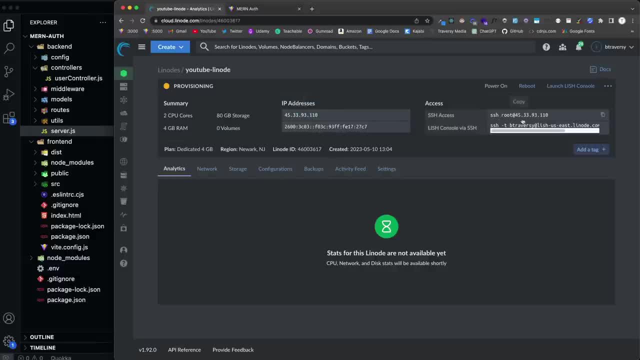 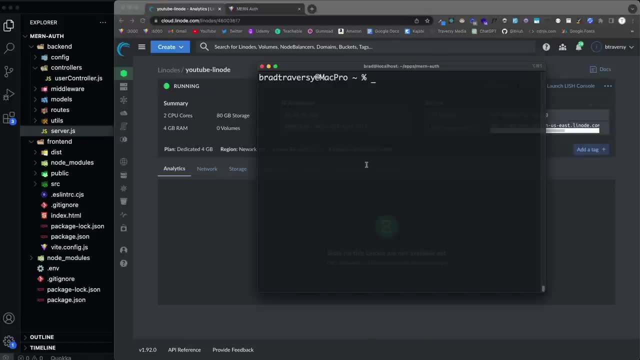 okay, make sure you use your own, and this is the ssh command that you can use to connect to your server. so let's actually copy that and then open up a terminal and then i'm going to paste that in here and connect to my server. the first time you log in it's going to ask if you want to continue. 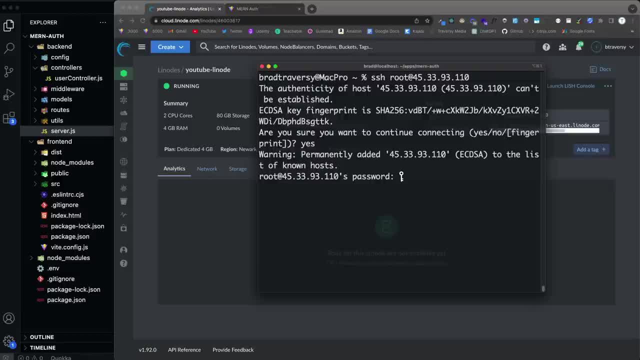 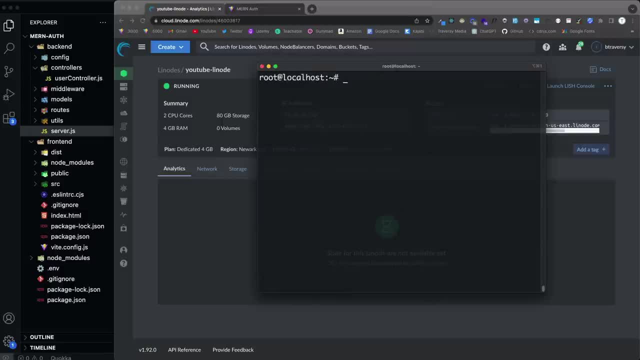 just say yes, and then you want to put in your password. okay, so now we're logged into our server and there's just a little provisioning that i want to make sure that you're going to be able to see the i want to do for one. i don't want to stay using the root user. it's good practice to create a. 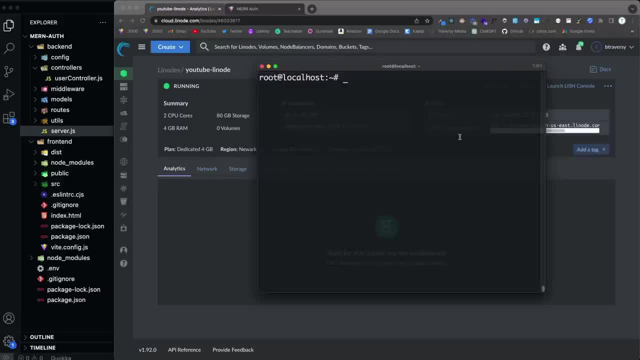 separate user and if you're going into production, i would suggest using ssh keys and disabling passwords. it's just an extra security step, but we're not going to do that for this tutorial. but we will create a new user. but before we do that, let's just update everything, all of our. 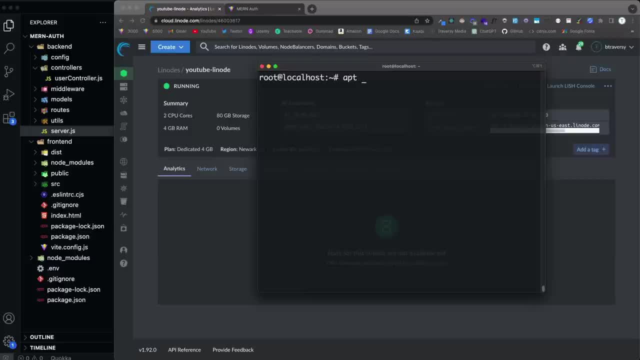 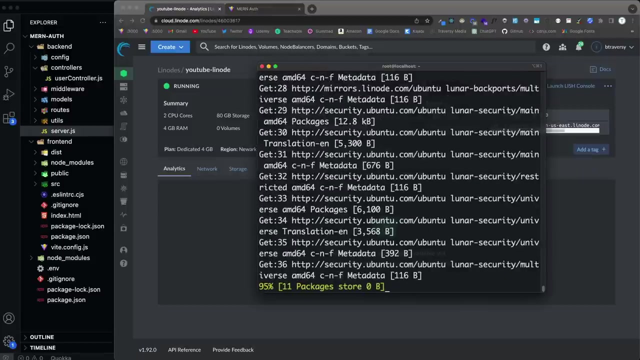 packages, our lists. so we're going to say apt, which is, you know, the aptitude package manager, and then we'll say update and apt, so you can do apt or app dash get, but we're going to do apt upgrade and that will just get everything up to date. okay, so the next thing i want to do: 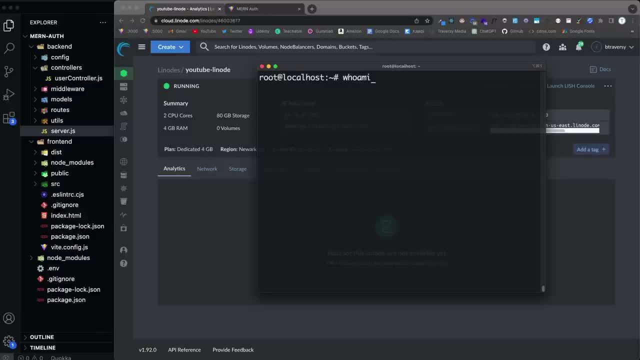 is: create a new user. and if you do, who am i? i mean, it says it right here: root at localhost. but if we run, who am i? you see i'm logged in as root, so i'm going to add a new user with the add user command. 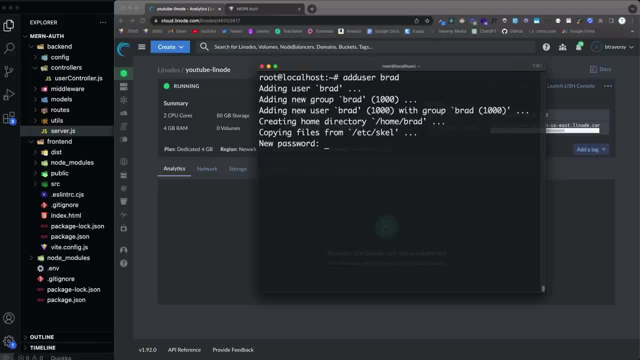 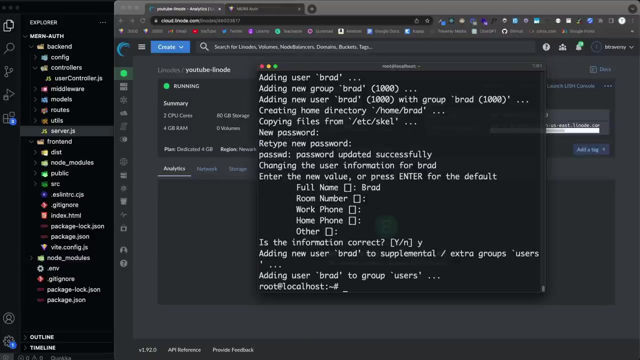 and i'm going to call my user brad- of course you can call it whatever you want- and then you want it a password and repeat that, okay, and then it's just going to ask for some information. you can just enter through this and say yes, okay. so now we have a new user named brad and it's added to the group of users. 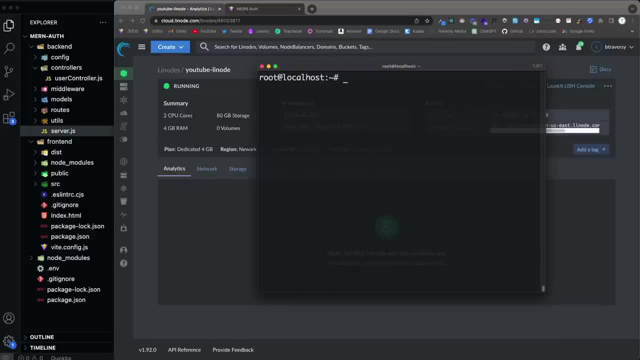 now i want this user to be, i want it to be able to make commands as root. so you want to add it to the sudo group. so to do that, we can say user mod and then dash lowercase, a, uppercase, g, and then sudo, because that's the group i want to add this user to, and then the user name, which for me is: 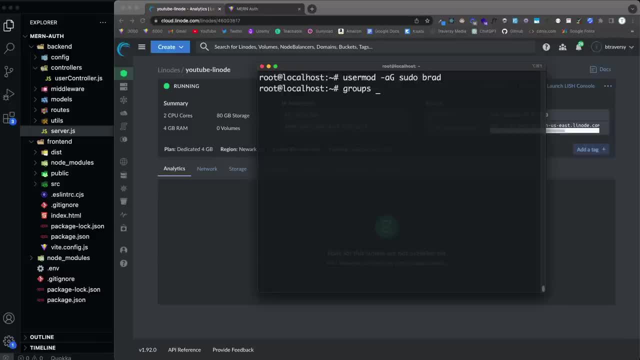 brad. okay. so now if i do groups, brad, it shows me the groups that i'm in and you're going to be in a group with the same name as your user- also the users group, and now also sudo. okay, so next thing we'll do is log in as that user so we can do that with su, and then space, hyphen space. 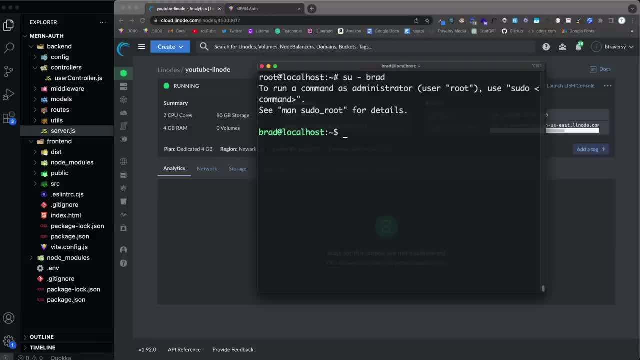 and then the username that we want to log in as. so it's just telling us that now we have to use sudo to run commands as administrator. but you can see, now it says brad at localhost. also, if i say who am i, it'll give me brad. so now that we've done that, let's start with our application, and of course we 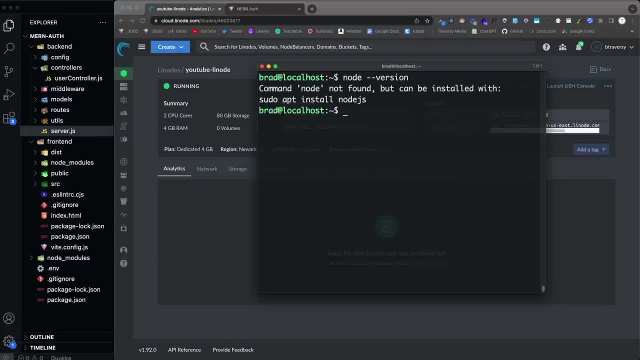 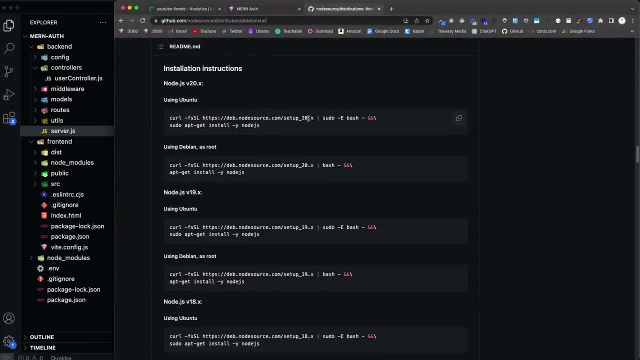 nodejs installed. if we say node version, by default it's not, it's not found. so we do have to install it and i'm going to just show you a page real quick that shows us how to install on ubuntu. so we want version 20, which is the latest, so we need to run these two commands, this curl. 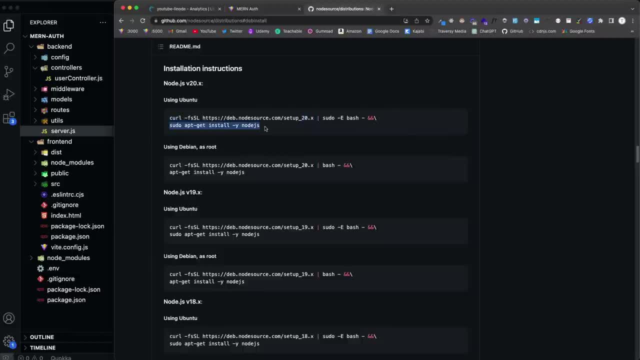 command which will get us the package and then we install it with this command here. all right, so you can either copy this- you can copy it from my blog post or, if you want to go to this url, like, if i click this button it'll actually grab both commands. 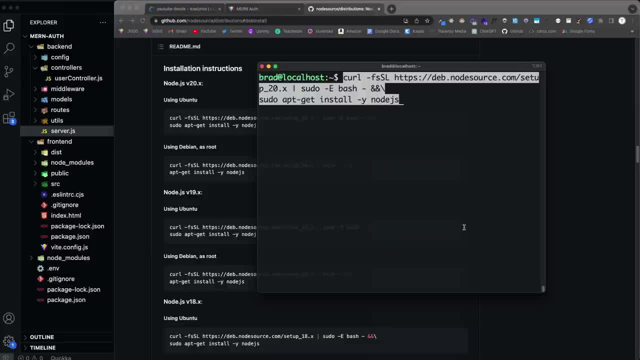 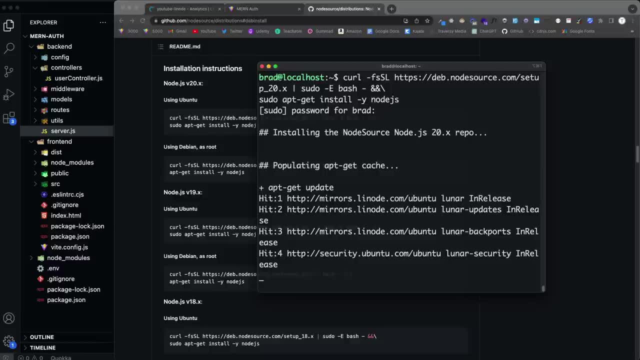 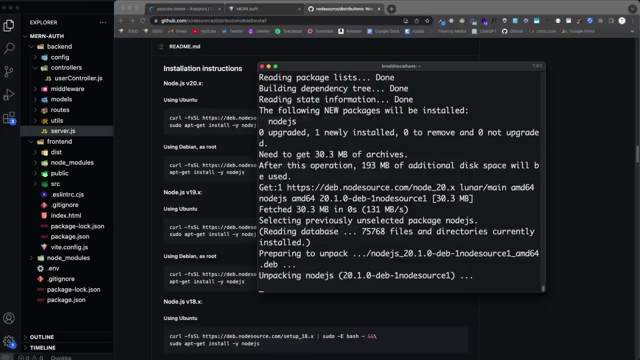 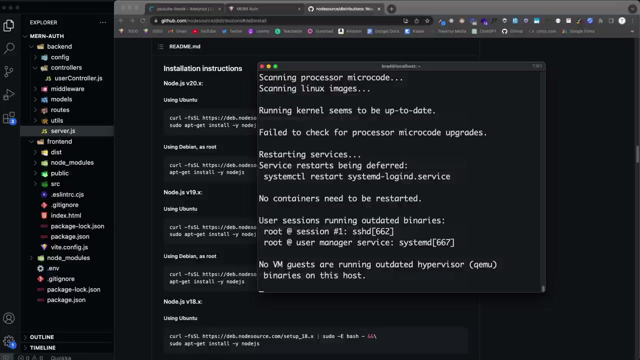 so let's go ahead and paste that in password. all right, so it's going to grab the package and then it's going to go ahead and install it and if you see this screen, just hit enter. all right. now, if i do node dash dash version, you can see i have version 21: 0 and if i do npm dash dash version, we should also. 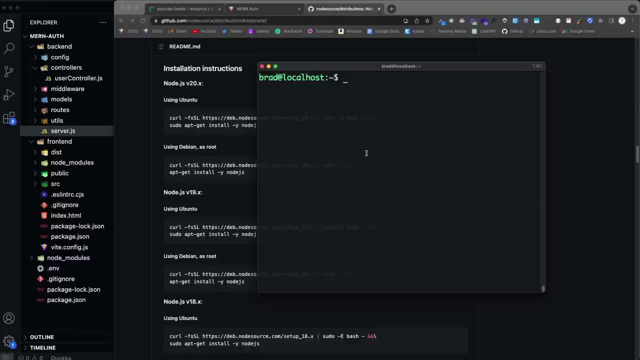 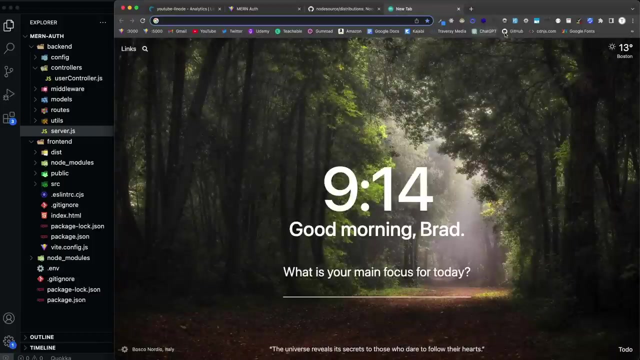 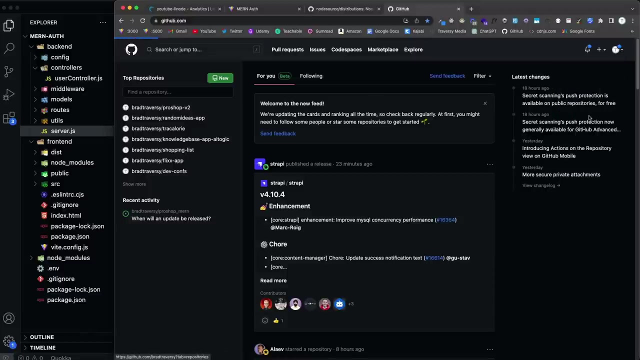 have npm, all right. now we need a place to put our application. so we're in the, the root directory. now that's what this tilde means. so i'm going to make a directory, so mkdir, called apps, and we're going to have everything sistema as a whole. so we're going to use the. 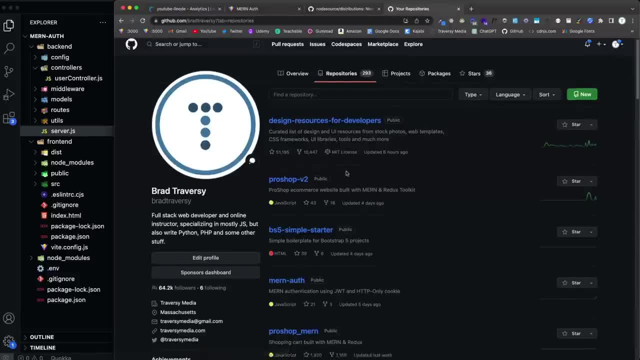 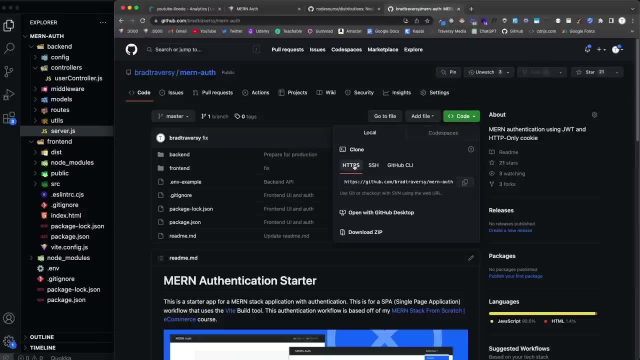 node to do that, and btn2, and this is where i want to put the application. so i'm going to use git to get my files on the server. so if i go to github, i'm going to go to that repository and you guys should have already pushed your app to github. 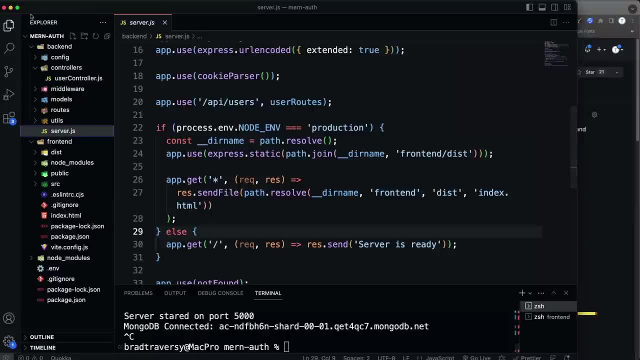 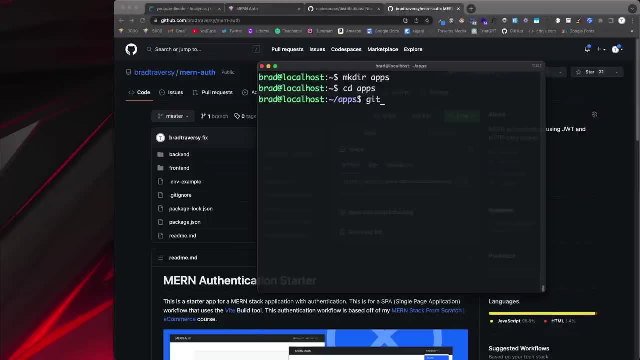 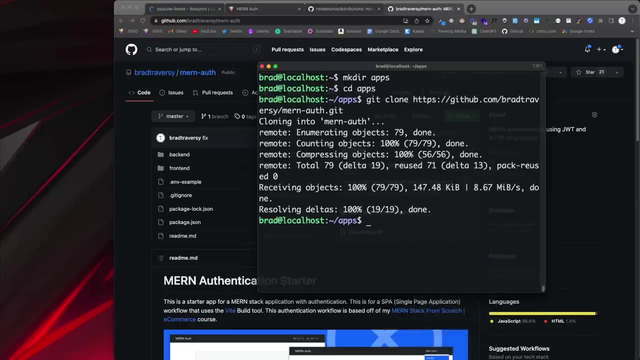 just copy that link. okay, so now actually we can close that up. so now we can go ahead and just do a git clone and then i'm going to paste in that link i just copied. and now, if i do an ls, you'll see we have the mern off folder. let's cd into mern off. do an ls, dash a, that'll show us everything. 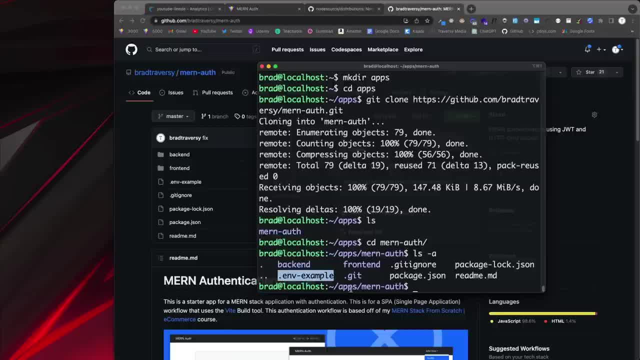 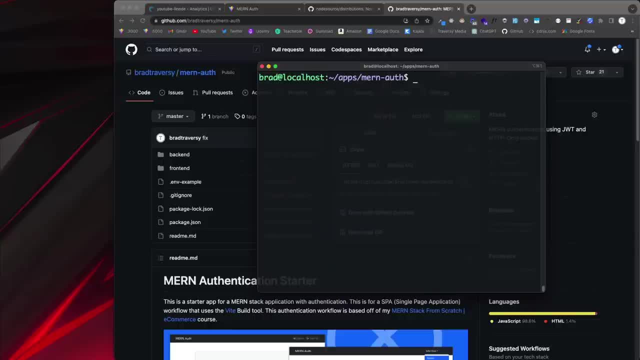 so we have a dot env dash example, because i didn't push my dot env to github. so what we want to do is rename that to dot env on the server. so let's say mv and then dot env- dash example, and we want to rename it to dot env. so now, if i do ls dash a, you can see dot env. so let's edit that file. i'm going 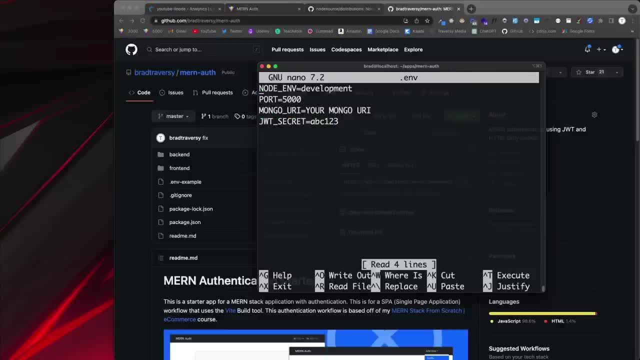 to use nano, so nano dot env. and then i'm going to change- and there's different ways to use environment variables on the server, but this, this one, is really easy. so we're just going to change this to production and it's going to run on on port 5000. however, we're going to set up nginx as a proxy so that we can. 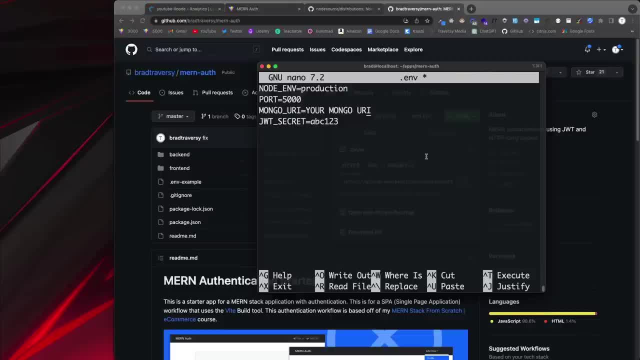 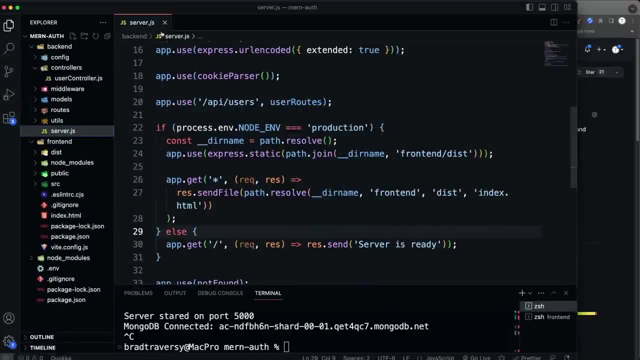 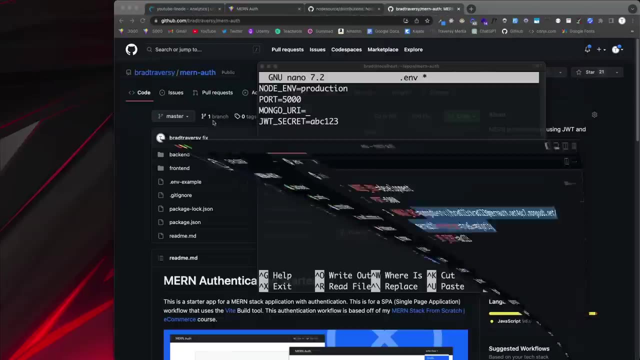 access our app through port 80, which is the http app port. so the mongo uri, we're going to need that. so going to grab mine from this dot env file right here so if we go ahead and copy that and i should be able to paste it in. 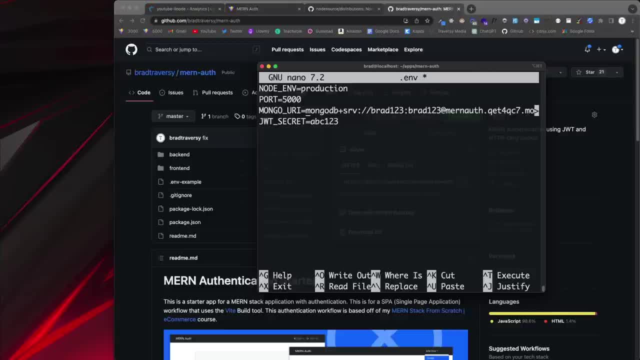 yep. so now we have that set and if you want to change this secret, jwt secret, you can. but that should do it. so i'm going to do command or control x and then hit y for yes, i want to save and then enter. and if you want to check, make sure the file is saved, you can use the cat command. 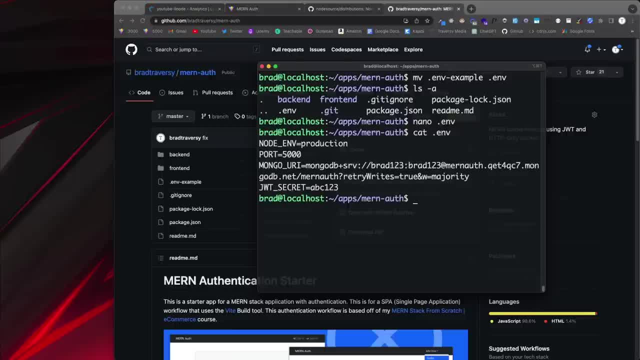 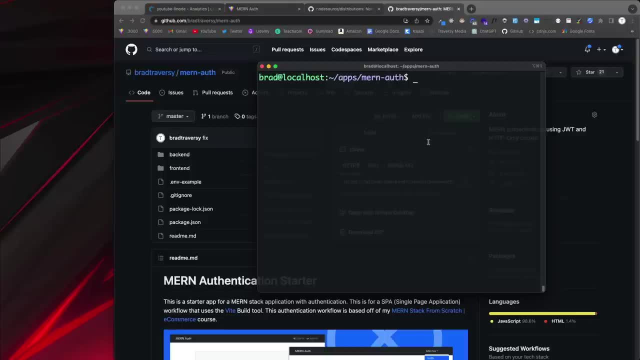 and do env. that'll just show you what's in that file. okay, so the next thing we want to do is install our dependencies and build out our front end assets. so we'll start off with npm install in the root, so that will install all of our server dependencies. it's just going to create a node. modules folder, just like it did in the past. so we're going to go ahead and create a node modules folder, just like it did in the past. so we're going to go ahead and create a node modules folder, just did locally. but we don't push our node modules to github, so we don't have that, so we have to run. 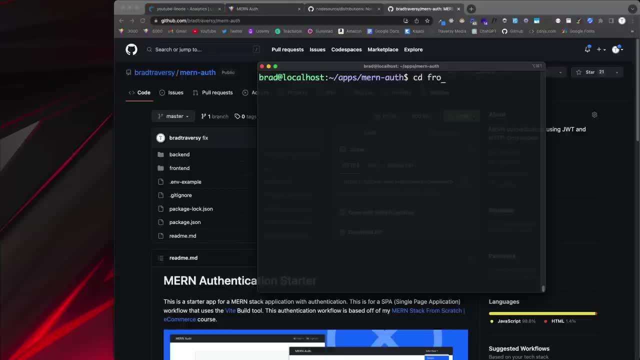 this again on the server and then we're going to cd into front end and run npm install or npm i. all right, and now let's run npm- run build from the front end, and that will create a dist folder. all right, and now let's run npm- run build from the front end, and that will create a dist folder. 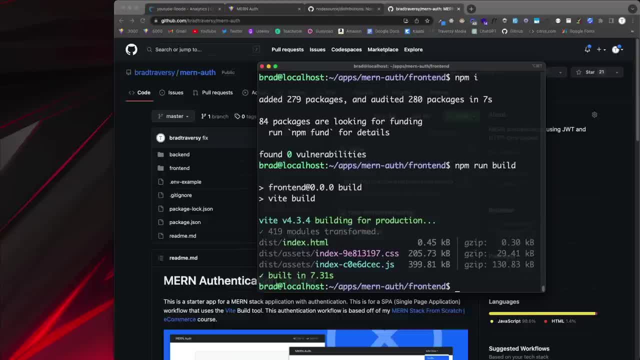 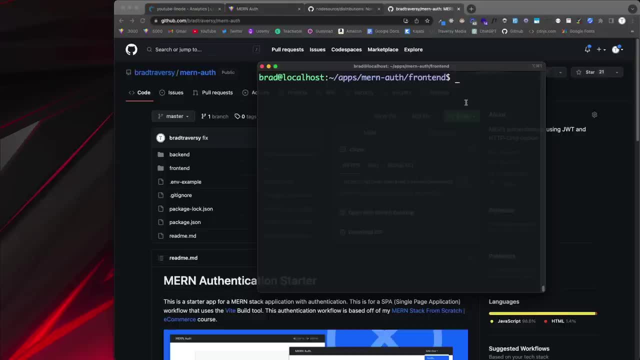 and that disk folder has the index html, which is the front end of our application. all right, cool. now, before we go ahead and run or try to run our application, you need to make it so that your mongodb atlas will actually accept connections from our server. because, right. 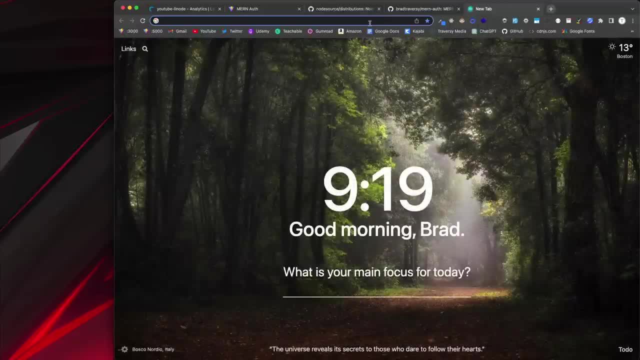 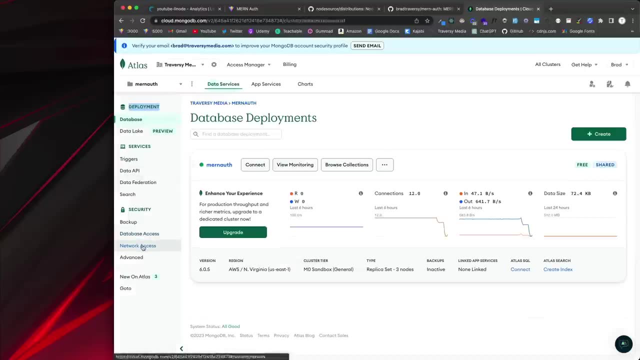 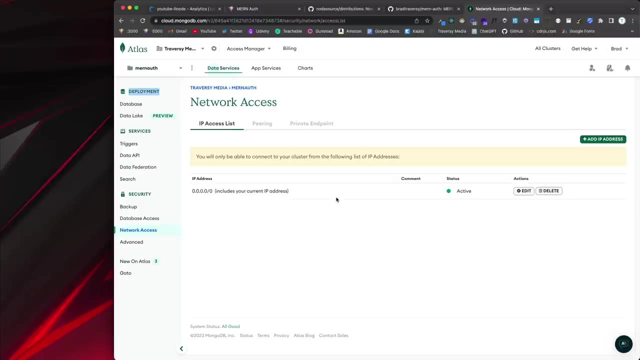 now you probably have it set up to just your. you know your local machine. so if we go to mongodb and log in right now, you probably have. if you go to network access, you probably have just your local ip address, like your, your machine at home or wherever you're you're building from, so you're. 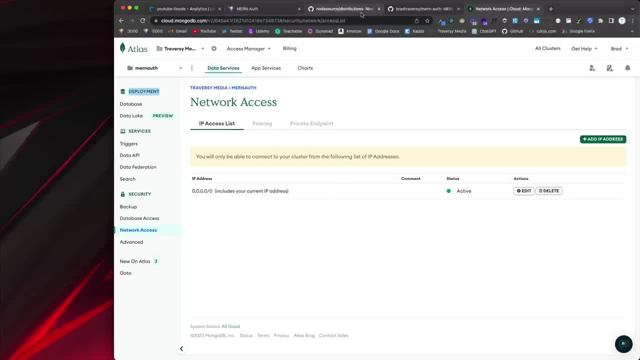 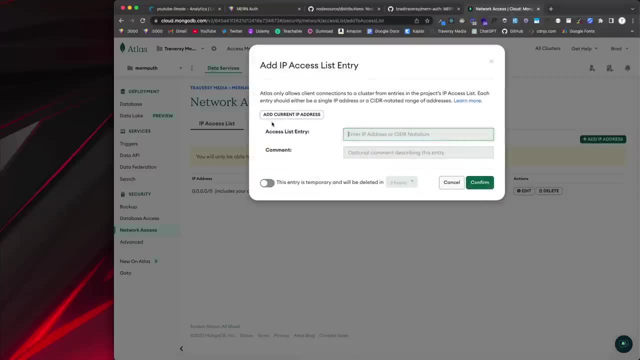 going to have to do one of two things: you can either add the ip address of the server, which would be, you know, whatever you have here, or you could just allow from anywhere, which is what i did. so that's why you see this zero, zero, zero. um, because i clicked this and then i said: allow from. 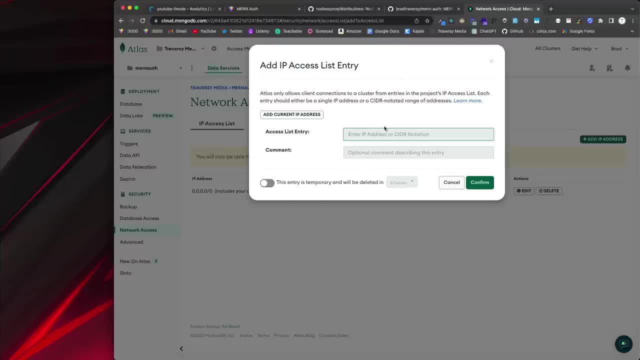 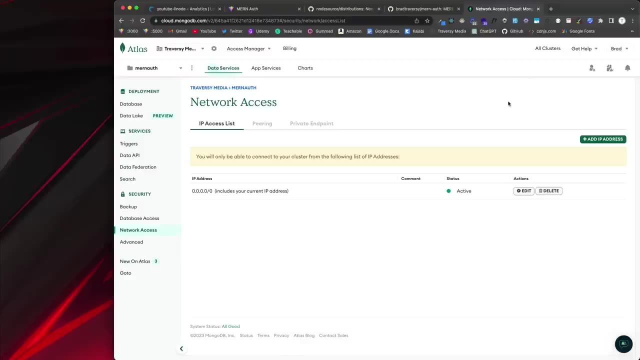 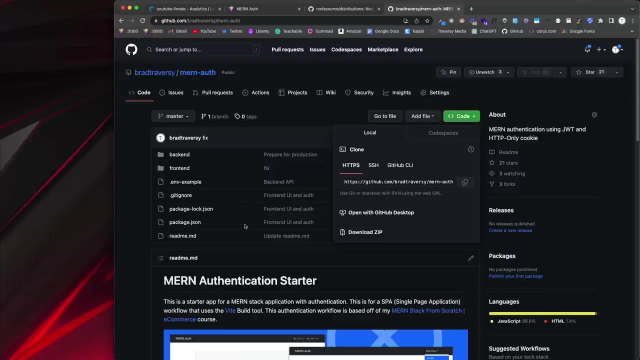 anywhere. i don't have that option anymore because i already chose it, but you can do that. or again, you can just put the server ip address, but you need to. your server needs to be allowed access to your database, all right. so once you do that, let's- uh, we can close that up. let's jump back over to 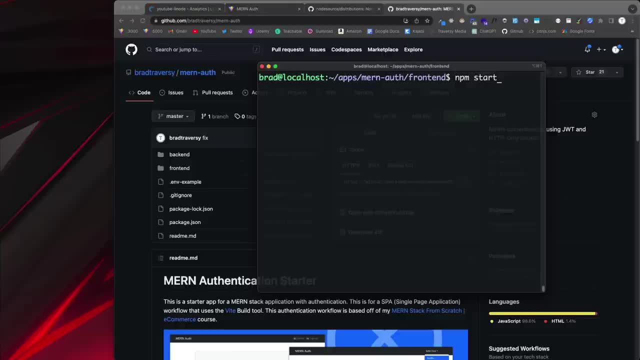 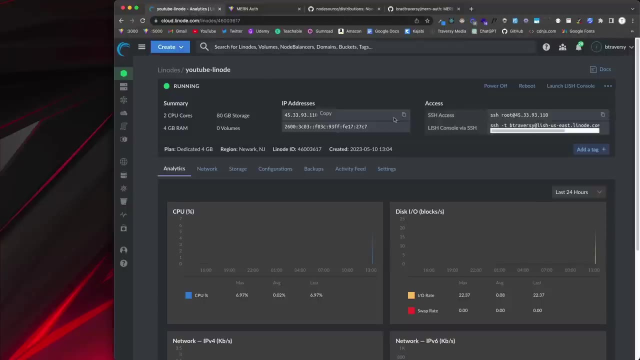 our terminal and let's. for now we're just going to run npm start. actually you need want to do this. run our server js and you can see mongodb connected. now it's running on port 5000. so if i go to my ip address, i'm going to copy that. make sure you use your own and then, if i go to colon, 5000, you should see your application. but you don't want to have to go to colon 5000 and you also don't want to have to keep it running in your terminal, because if i stop this then i try to go there. it's not going to work. 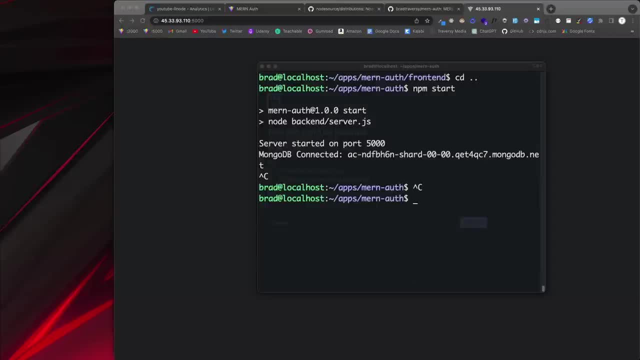 all right. so what we need to do are two things. we need to set up a process manager so that we can run our app as a process in the background. so even if we close the terminal and you know we get rid of our connection here, it'll still be running. and then we also want to 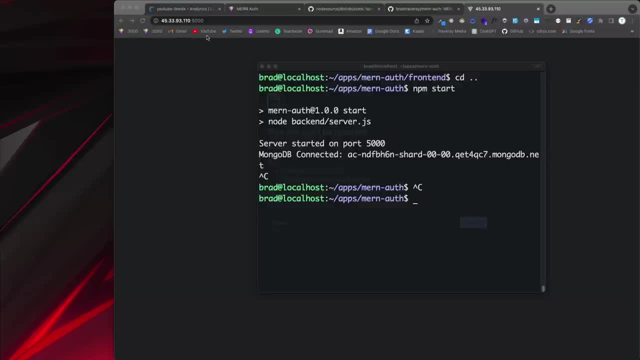 use nginx as a proxy so that we can go through port 80, so that we don't have to add a colon in a port, and then if you, of course, if you want to add a domain name, you can move on and do that. so let's start off with the. 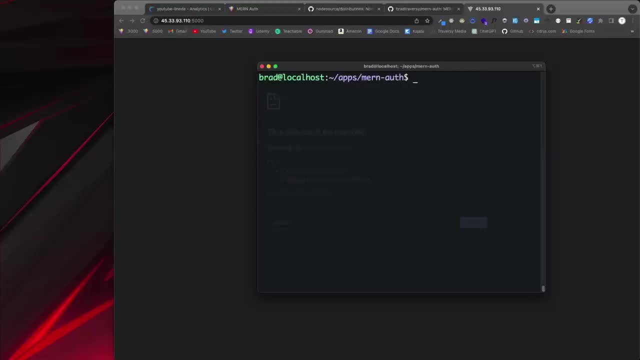 process manager. so we're going to npm. actually, now that we're a lot, we're using a, not the root user. we can say sudo, or we have to say sudo, npm install and i'm going to install this globally. so dash g and then pm2 is the name of the process manager and this is really simple. so, basically, 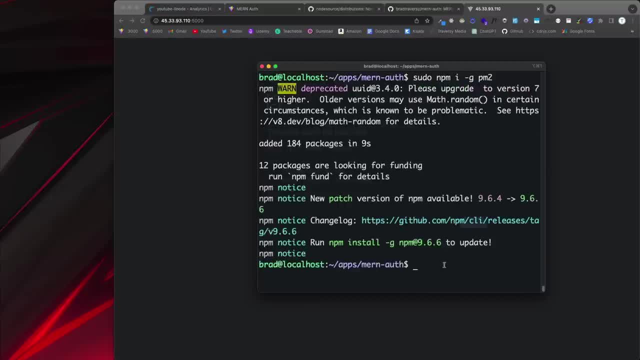 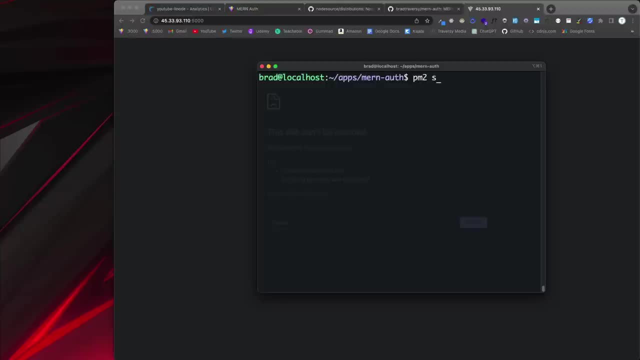 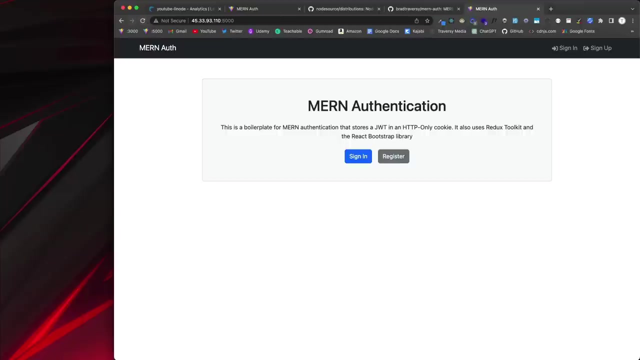 we can just use this like we do: npm to start the application, but it will be ran as a process. so we can say pm2 and we want to start and then backend slash serverjs and now it's bit that the application is running. if i go back here and reload, it should work. 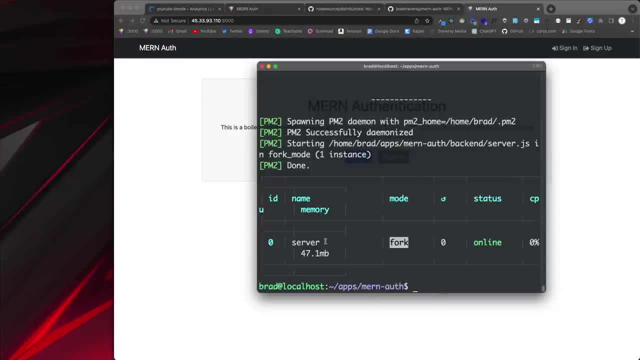 and my terminal is freed up and i can exit out of this and it will still be running as a process. okay, so now we have the issue of 5000. i don't even want people to access port 5000, so that's the next step. is we're going to enable? 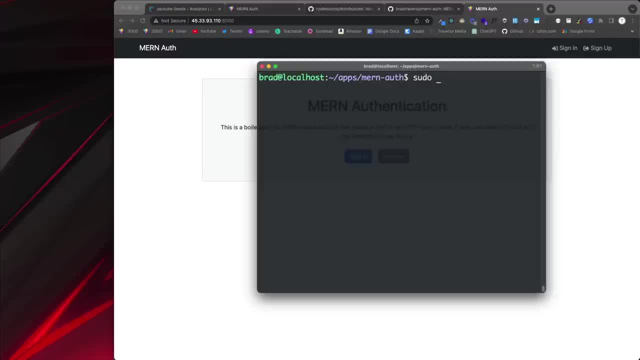 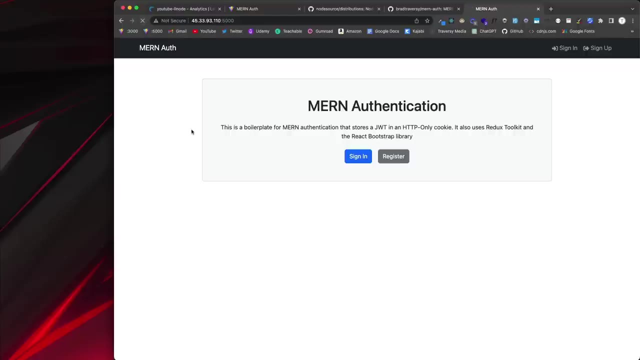 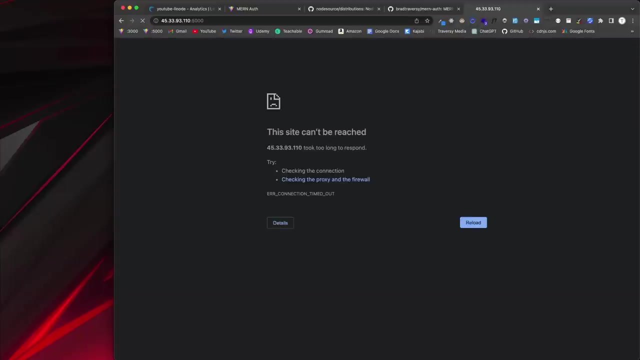 our firewall. so let's say sudo and then ufw is the default firewall, so we're going to enable it and it says it may disrupt connections. we'll say yes for that. all right now. if i reload this, you'll see it's still trying to to connect. it doesn't work because i enabled the firewall, which. 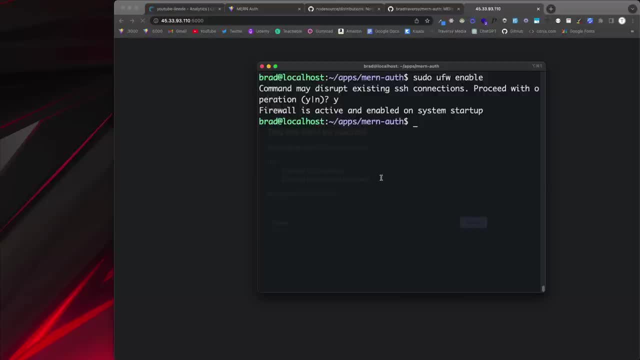 by default, all the ports are blocked. so we do want to enable the ports for http, https and ssh. so to do that we can say sudo, ufw allow, and let's say ssh, and then we want to do allow http, and then we want to do allow http. 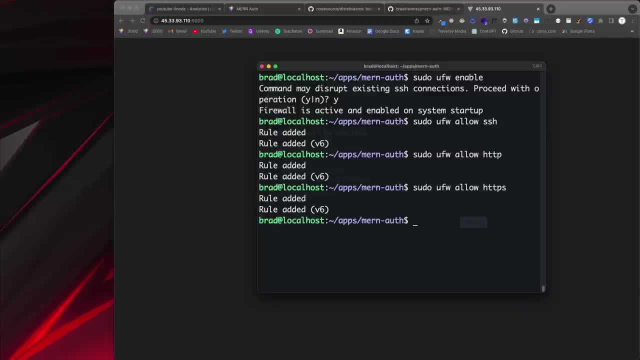 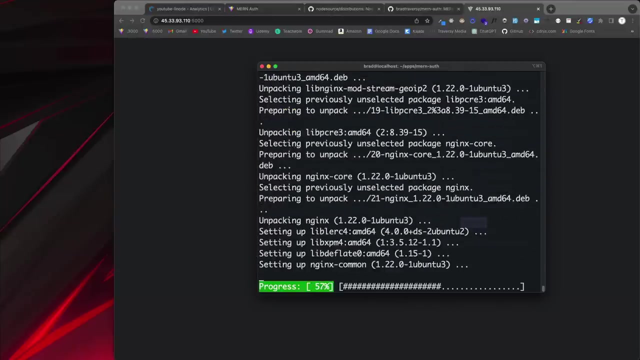 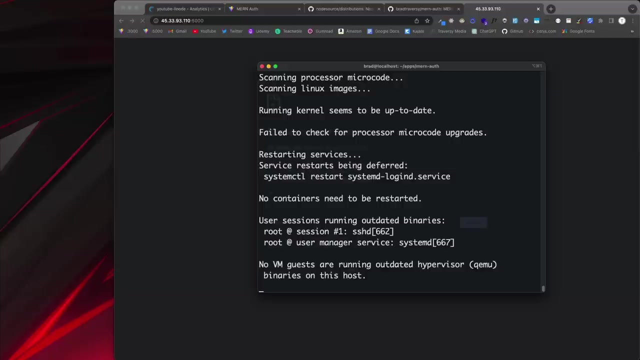 ps, you can also put the actual port numbers. so the next thing is to set up nginx, because that's how we can have our app basically run through port 80. so let's say sudo apt, install nginx, say yes, and for this just hit enter. all right. so now we have nginx installed. and if we were to go to 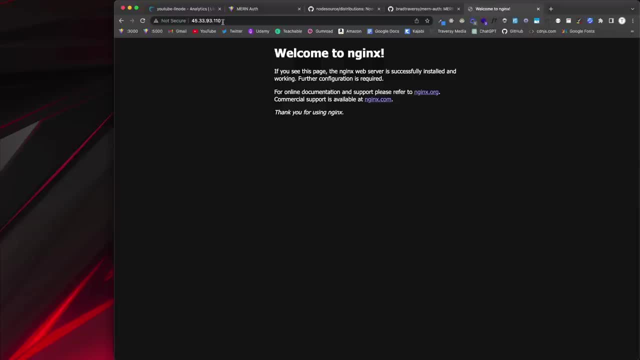 just our root domain here, you should see. just welcome to nginx. so the next step is to configure our application so that we can access it through through the root domain. so we're going to edit a specific file, let's say sudo, nano, and then it's going to be slash, etc, slash. 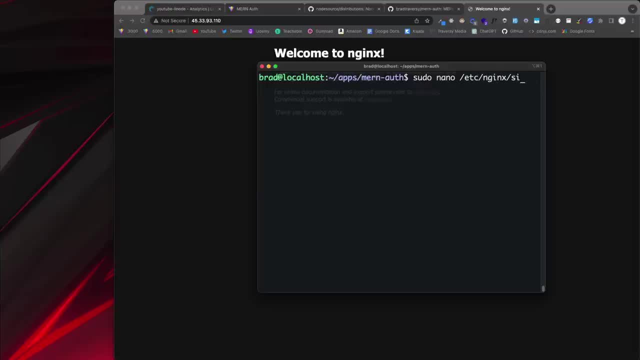 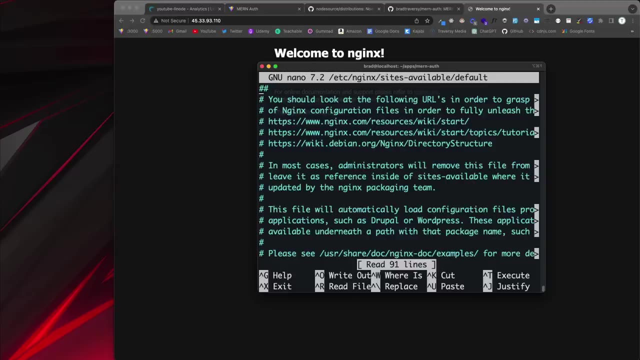 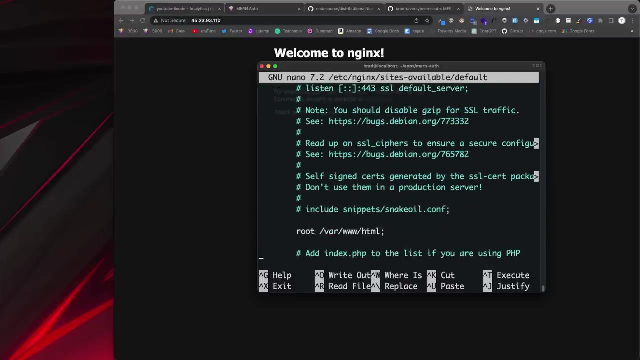 nginx, slash sites, dash available and then slash default. so you should see a file like this, and what we want to do is go down to where we have the location, the location block, which is right here. okay, and if you add a domain name, you would put the domain here. so, for instance, if i were to use 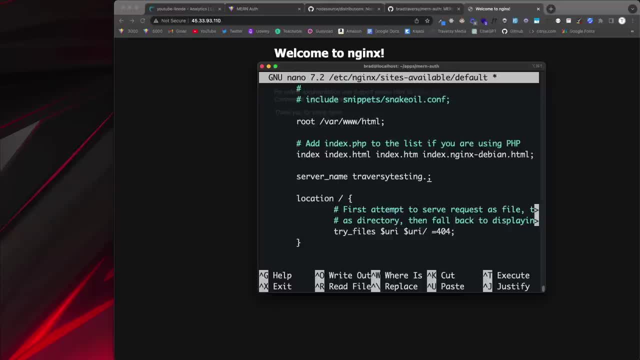 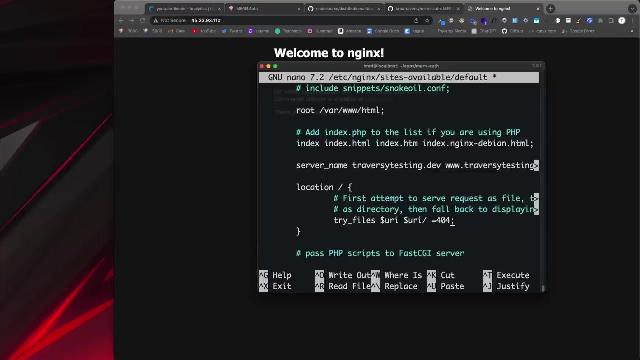 traversy, testing, dot, dev, and i would also put the www version all right. so that's if i wanted a domain now in the location block. we're actually gonna get rid of this stuff, so we're going to clear out everything in here. excuse me, i don't know why my 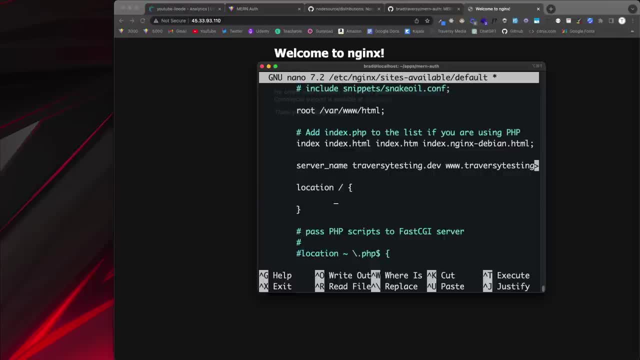 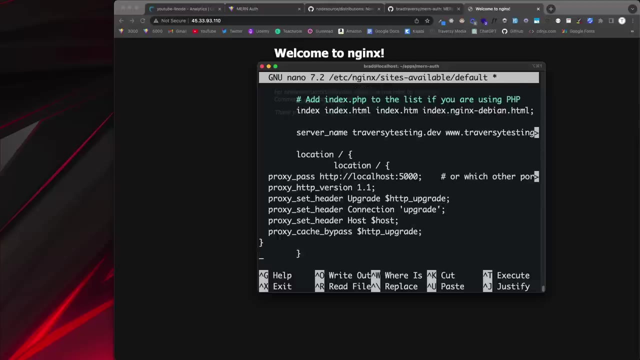 option isn't working all right, so we want to clear that out, and what i'm going to paste in here you can get from the blog post in the description or you can type it out if you want. so i'm going to just paste this in: whoops, this also has the location, so i want to make sure i don't have 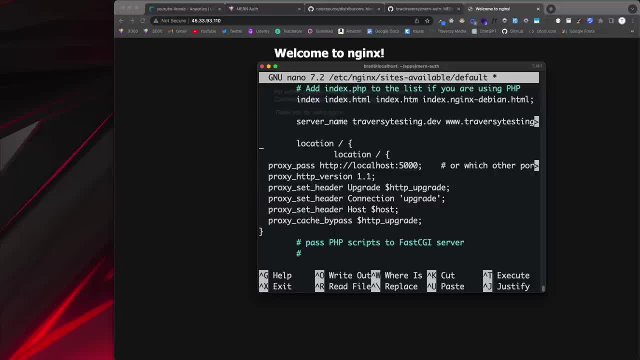 that twice. so i'm going to get rid of that last one. and there it is. there. i don't want to paste it and i'm going to hit open and get rid of that, all right, so in location slash you should have this proxy pass. so, basically, our, our app is running on the server, which is localhost, because 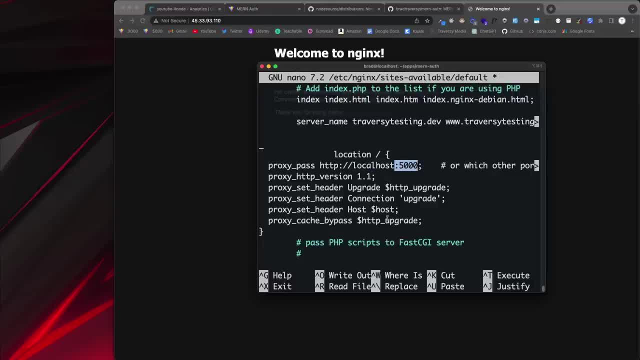 we're logged into the server and on port 5000, but adding this here will allow us to access it through the root domain, through, basically, our http port. all right, so that should be all we need to do. so we can go ahead and do Control-X Yes to save and then Enter. 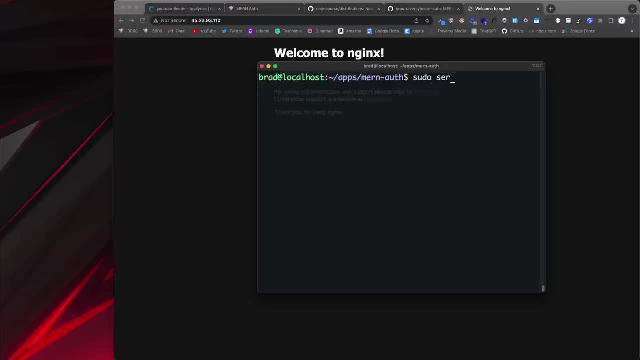 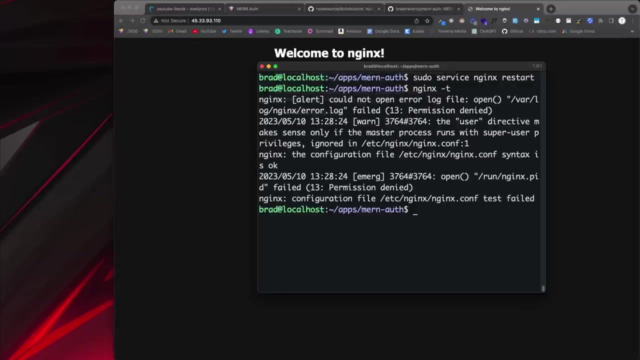 And then we just want to reload NGINX, and we can do that with sudo service, NGINX restart, And you can check the NGINX config file by just saying NGINX-T. Let's see alert: Could not open log file. 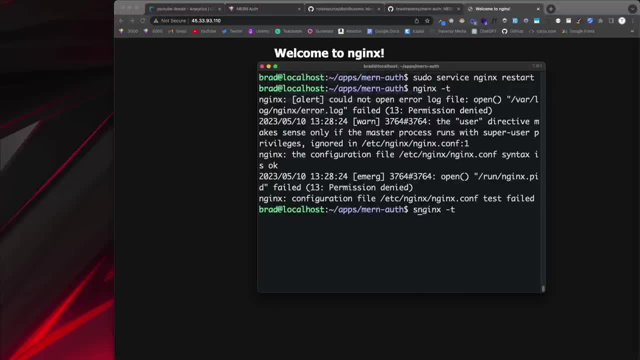 Oh, I just need to do sudo. So sudo, Okay. so it says the configuration file syntax is okay. Test is successful, So we should be ready. So now let's go to the browser and let's reload this page. And there we go. 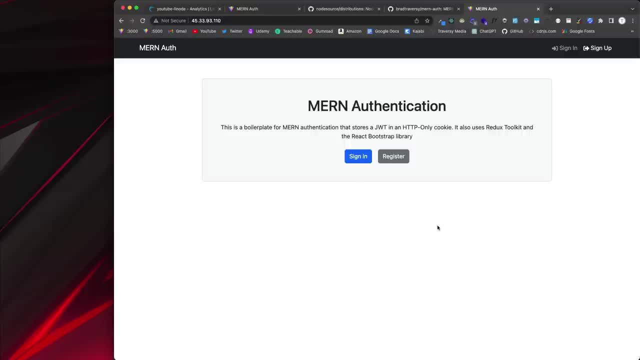 So our project is now deployed. However, I do want to mention that your JSON web token isn't going to get stored in the HTTP-only cookie unless you have a domain and an SSL certificate, because it has to be HTTPS. So that's another level. 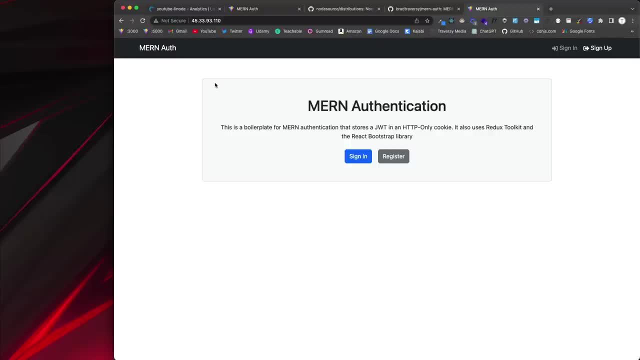 So you should be able to log in or create a user. You just won't be able to access any protected routes, And our protected routes are the. Actually, the only one we have that we're using is the update profile, So we should be able to create an account. 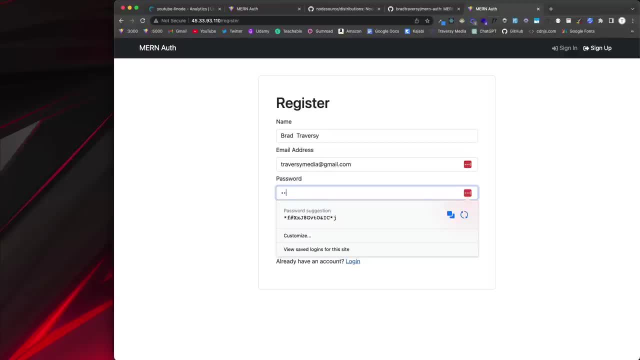 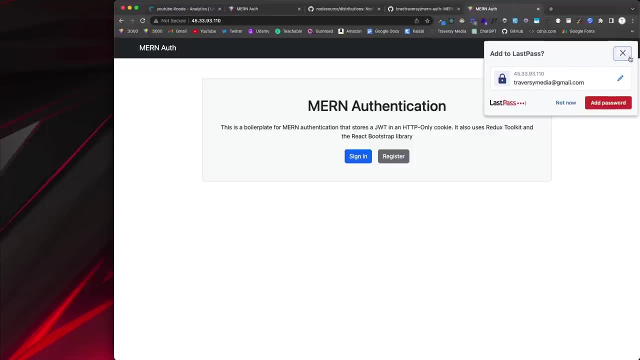 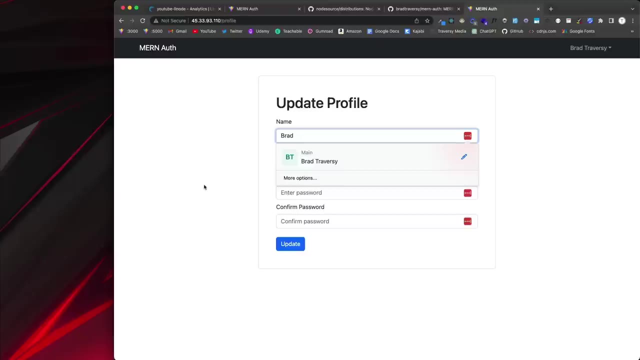 Let's just go ahead and do that real quick. So I'll register, So I am logged in. I'm logged in to the front end, But if I try to make a request, like, let's say, I want to change my name here and update, 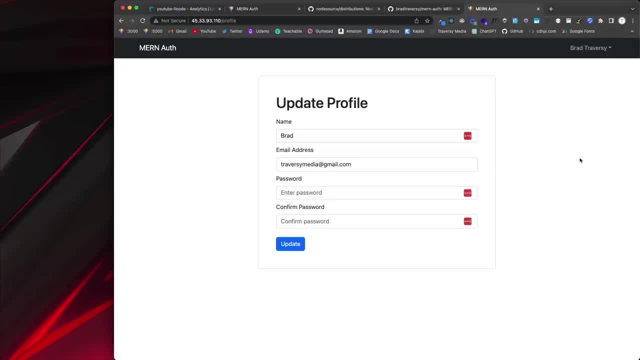 you'll see it says not authorized, not no token, because that HTTP-only cookie was not created. because I'm not secure right now, I'm not using HTTPS Now. if you did want to move further and add a domain and an SSL, you can look in Linode documentation. 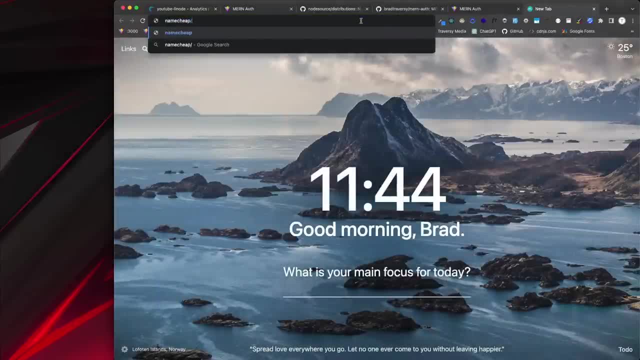 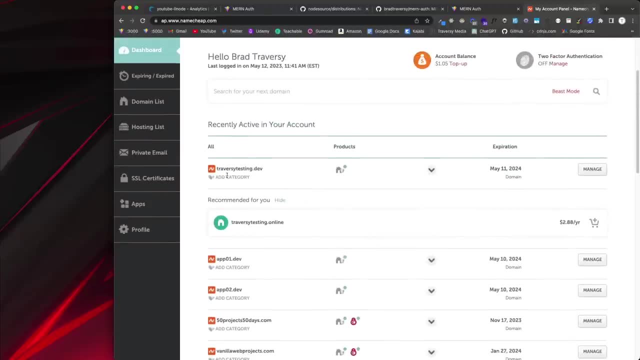 but I'll just show you real quick. So I'll use Namecheap for my domains, But of course you could use whatever you want. And if I go to my dashboard here and let's just say I want to use this Traverseetestingdev. 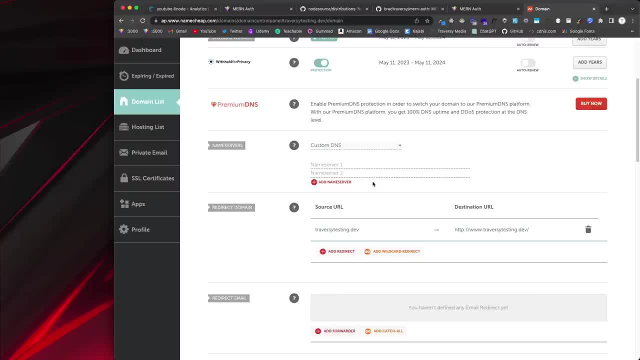 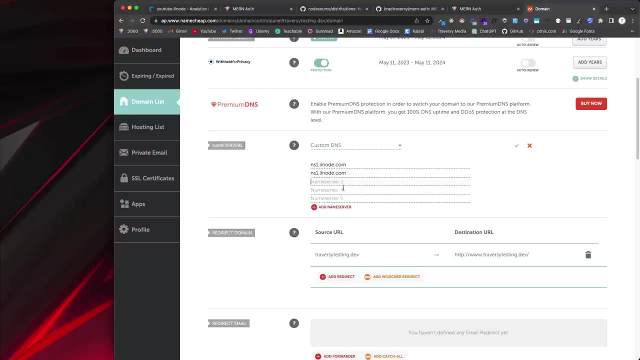 So if I go to Manage and then under Name Servers you want to add your custom DNS name servers And the ones you want to add for Linode are going to be ns1.linodecom through ns5.. So we can just copy that and paste those in. 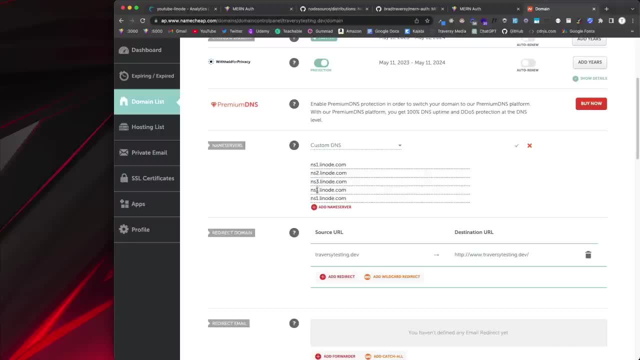 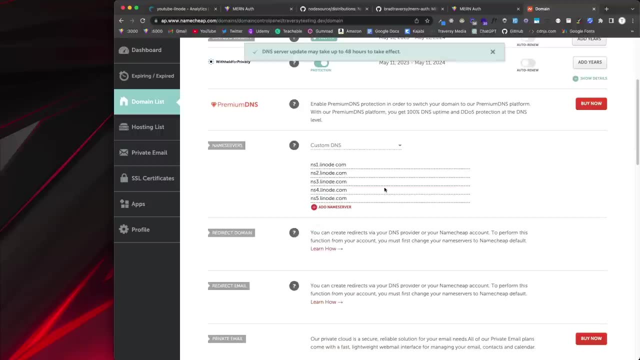 and then just change this to 2.. Change that to 3,, 4, and 5.. So once you do that, that will take up to 48 hours to propagate, as you can see here, But once you do that you can go over to Linode. 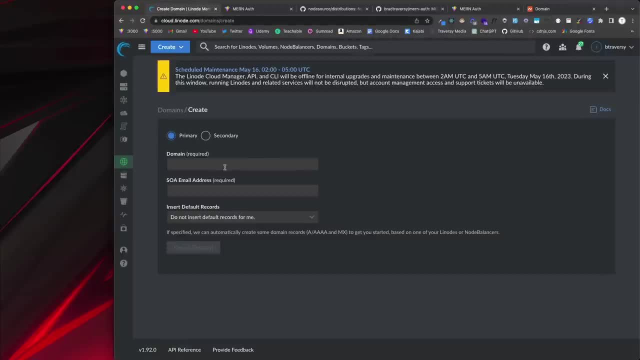 and just go to Domains, Create Domain. add in the domain you want to use, like Traverseetestingdev, and then your email address. I'll just put that in there And then here. you just want to insert your default records from one of your Linodes. 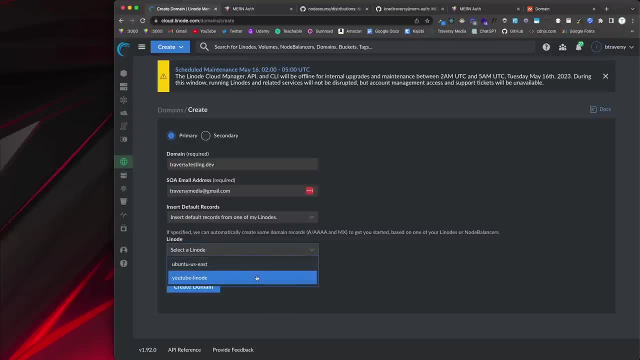 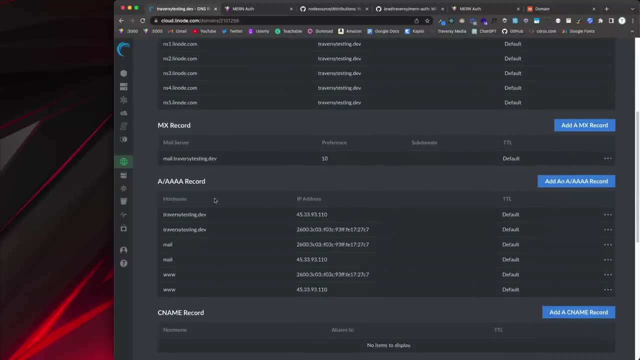 and then make sure you choose the one that you want, because you could have multiple domains in multiple servers. Once you do that, it will create the domain here and it will add the correct records for you, the correct A records and all that.